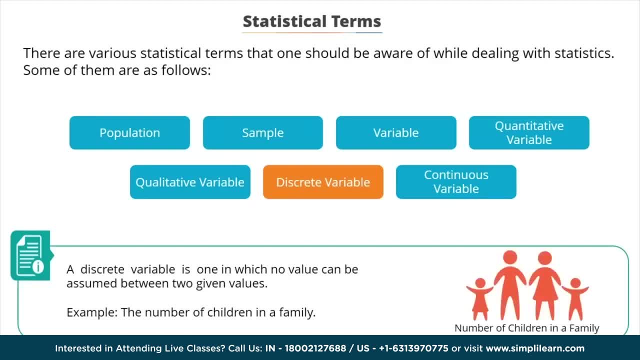 and an aspiring data scientist looking for online training and certifications from the present, then this course is for you, And if you are a professional with minimum one year of experience. For example, the number of children in a family, A continuous variable, is one in which any value can be assumed between the two given values. 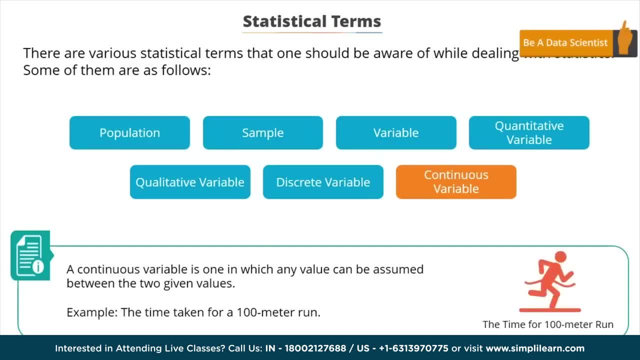 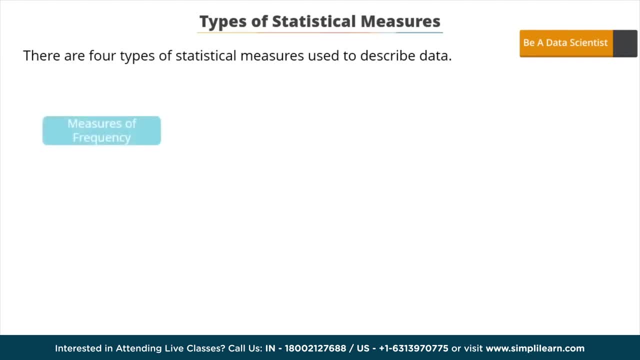 For example, the time taken for a 100-meter run. Typically, there are four types of statistical measures used to describe the data. They are measures of frequency, measures of central tendency, measures of spread, measures of position. Let's learn each in detail. 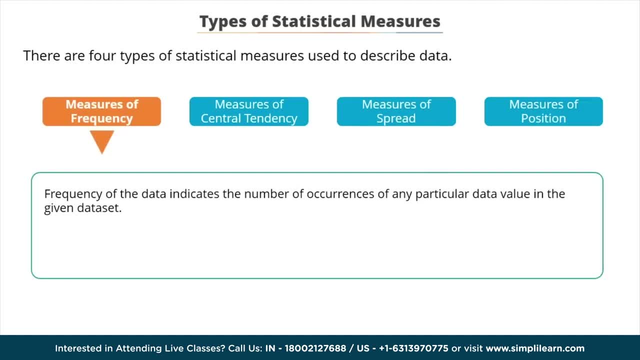 Frequency of the data indicates the number of times a particular data value occurs in the given dataset. The measures of frequency are number and percentage. Central tendency indicates whether the data values tend to accumulate in the middle of the distribution or toward the end. The measures of central tendency are mean, median and mode. 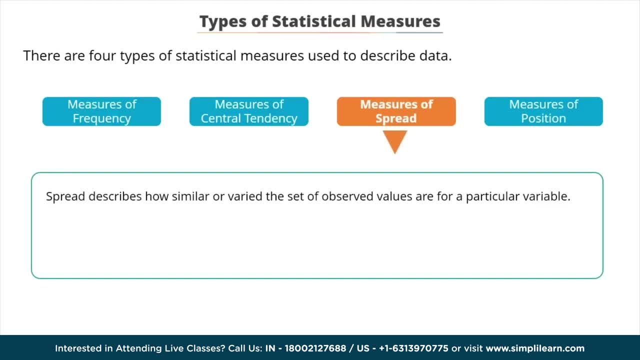 Spread describes how similar or varied the set of observed values are for a particular variable. The measures of spread are standard, deviation, variance and quartiles. The measures of spread are also called measures of dispersion. Position identifies the exact location of a particular data value in the given dataset. 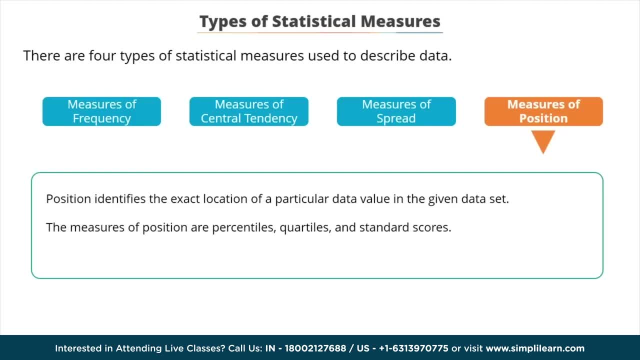 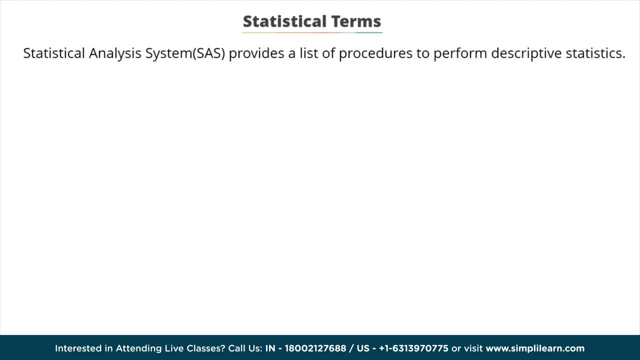 The measures of position are percentiles, quartiles and standard scores. Statistical Analysis System, or SAS, provides a list of procedures to perform descriptive statistics. They are as follows: Proc print, Proc contents, Proc means, Proc frequency, Proc univariate. 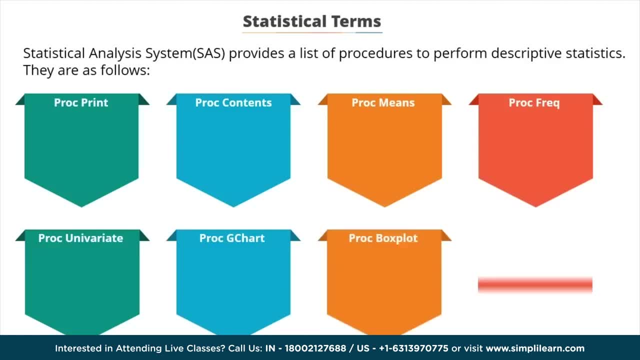 Proc, gchart, Proc, boxplot, Proc, gplot, Proc print: It prints all the variables in a SAS dataset. Proc contents: It describes the structure of a dataset. Proc means: It provides data summarization tools to compute descriptive statistics for variables across all observations. 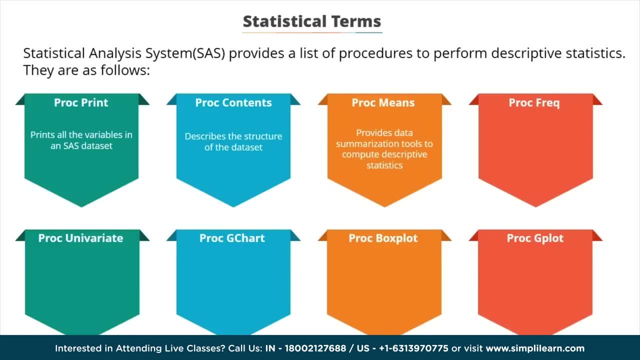 and within the groups of observations. Proc frequency: It produces one-way to n-way frequency and cross-tabulation tables. Frequencies can also be an output of a SAS dataset, Proc univariate. It goes beyond what proc means does and is useful in conducting some basic statistical analyses and includes high-resolution graphical features. 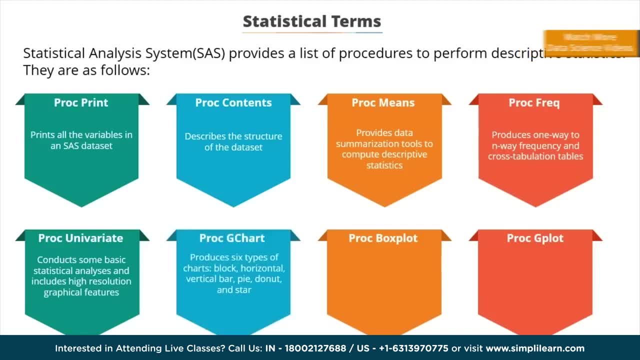 Proc gchart. Proc gchart Proc gfbr. Proc ggm, Proc g 0.. Proc ggdl です node Proc gdlothes. node Start the classification: Proc gsr candle, Proc gsr candle. Procầu candle Birch. coincidence假 Reg לצ'. 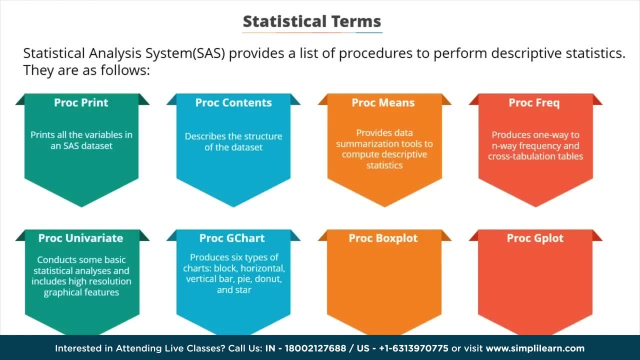 So the typical prosecution procedure produces six types of charts: Block charts, horizontal vertical bar charts, Pie-donut charts and star charts. These charts graphically represent the value of a statistic calculated for one or more variables in an input SAS dataset. So you can compute these, but they are numbers. 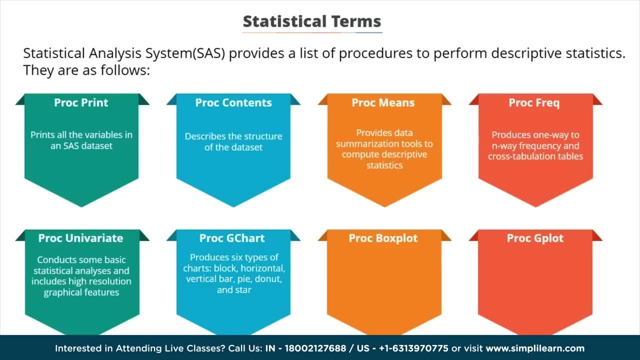 The numbers are the index of an input SAS dataset. The chart could be limited or the number of individual input. Proc. boxplot. The boxplot procedure creates side-by-side box-and-whisker plots of measurements organized in groups. A box and whisker plot displays the mean, quartiles and minimum and maximum observations for a group. 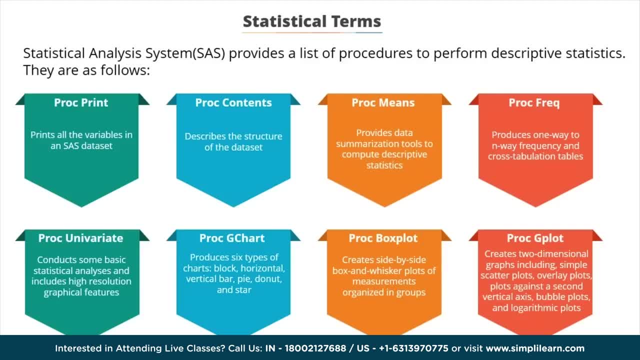 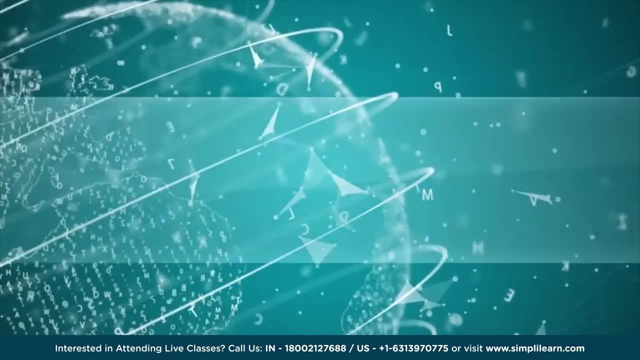 PROC GPLOT. GPLOT procedure creates two-dimensional graphs including simple scatter plots, overlay plots in which multiple sets of data points are displayed on one set of axes, plots against a second vertical axis, bubble plots and logarithmic plots. In this demo, you'll learn how to use descriptive statistics to analyze the mean from the electronic dataset. 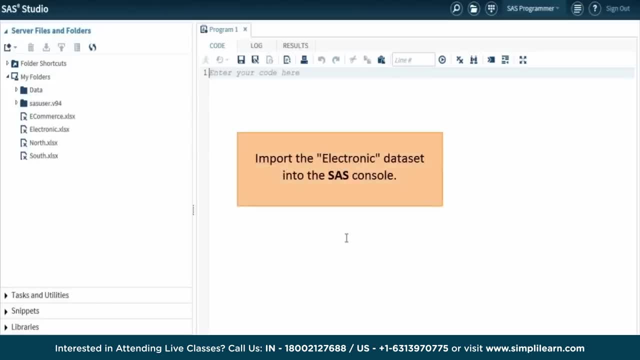 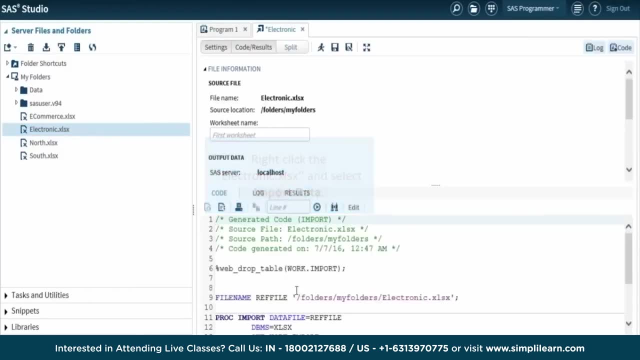 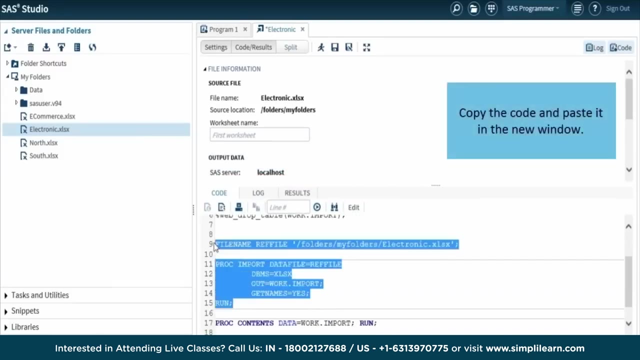 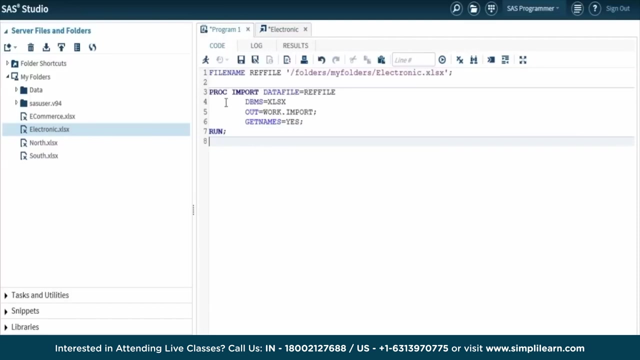 Let's import the electronic dataset into the SAS console. In the left plane, right-click the electronic xlsx dataset and click Import Data. The code to import the data generates automatically. Copy the code and paste it in the new window. The PROC MEANS procedure is used to analyze the mean of the imported dataset. 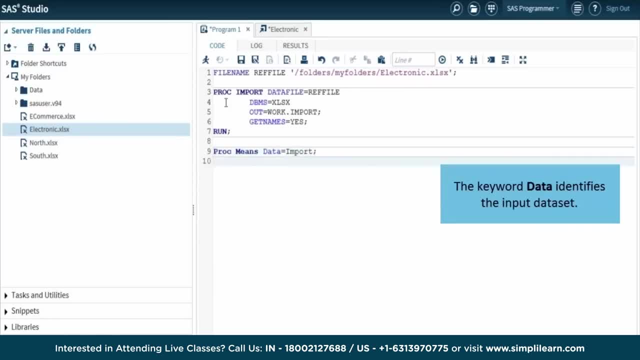 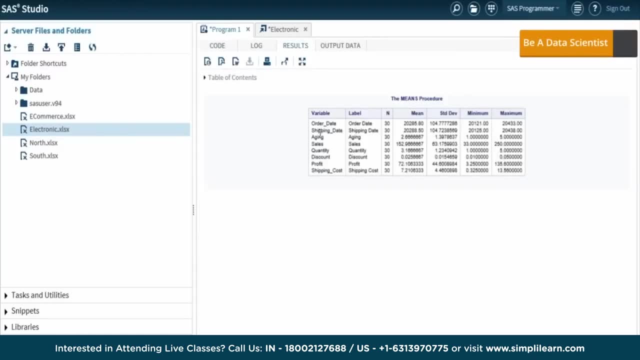 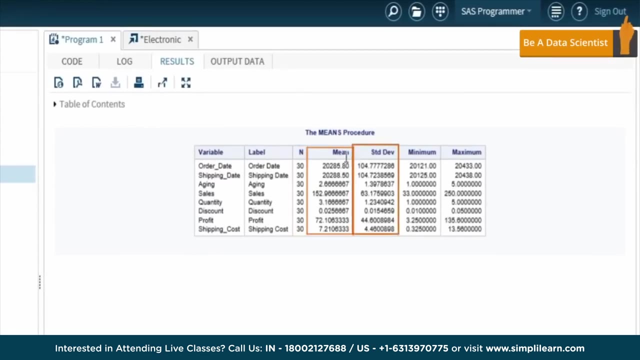 The keyword DATA identifies the input dataset. In this demo, the input dataset is electronic. The output obtained is shown on the screen. Note that the number of observations mean standard deviation and maximum and minimum observations. The data values of the electronic dataset are obtained. 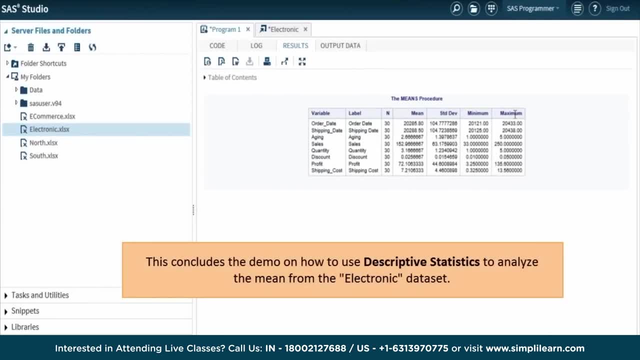 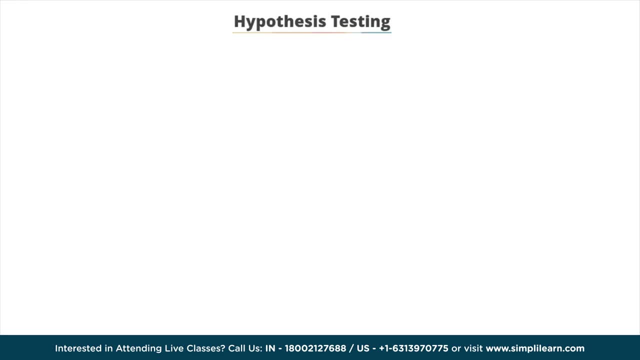 This concludes the demo on how to use descriptive statistics to analyze the mean from the electronic dataset. So far you have learned about descriptive statistics. Let's now learn about inferential statistics. Hypothesis testing is an inferential statistical technique to determine whether there is enough evidence in a data sample. 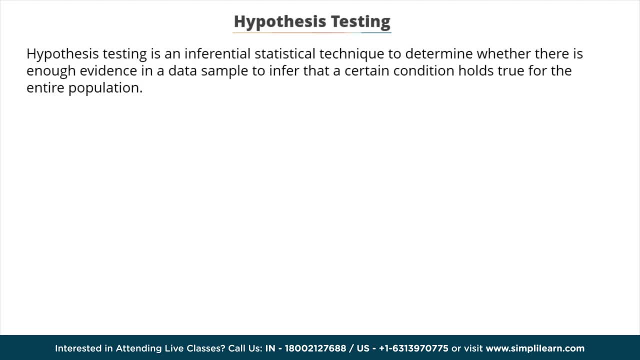 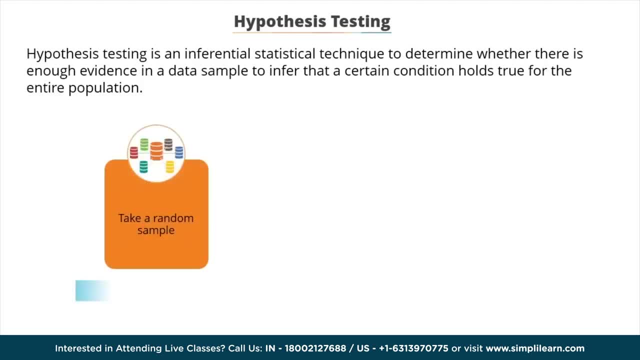 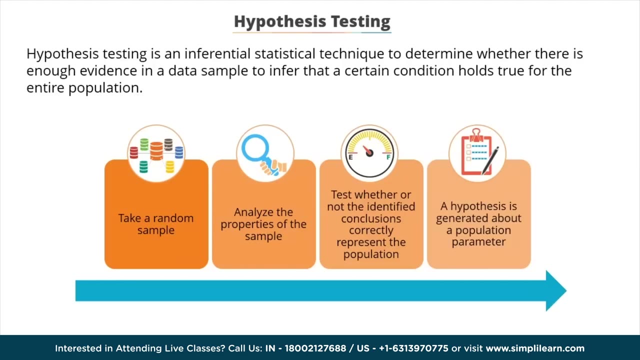 the characteristics of the general population. we take a random sample and analyze the properties of the sample. we then test whether or not the identified conclusions correctly represent the population as a whole. the population of hypothesis testing is to choose between two competing hypotheses about the value of a population parameter, for example. one hypothesis might 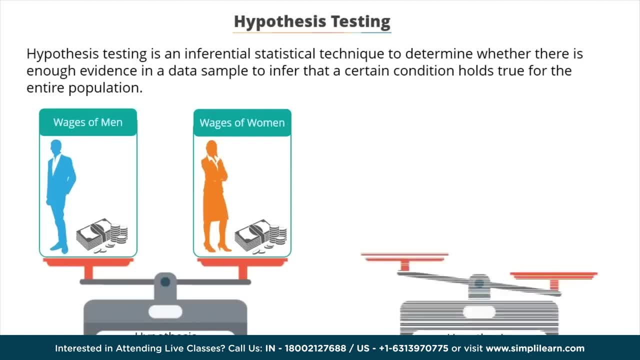 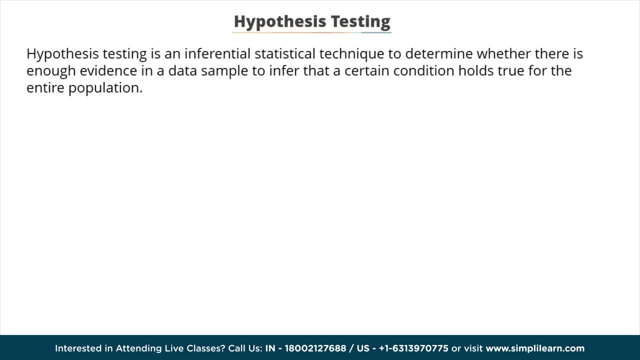 claim that the wages of men and women are equal, while the other might claim that women make more than men. hypothesis testing is formulated in terms of two hypotheses: null hypothesis, which is referred to as h. null alternative hypothesis, which is referred to as h1. the null hypothesis is: 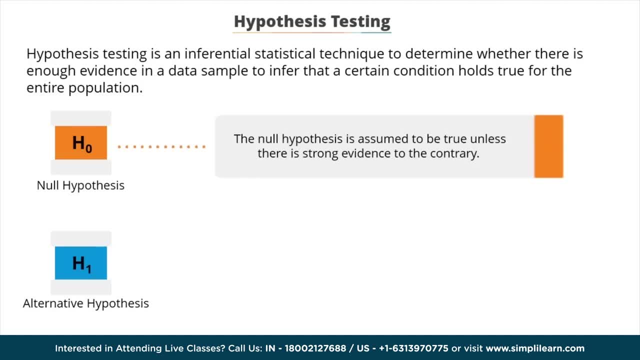 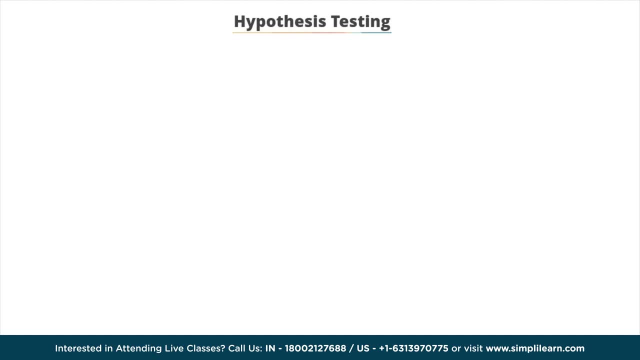 assumed to be true unless there is strong evidence to the contrary. the alternative hypothesis is assumed to be true when the null hypothesis is proven false. let's understand the null hypothesis and alternative hypothesis using the null hypothesis a general example. null hypothesis attempts to show that no variation exists between variables. 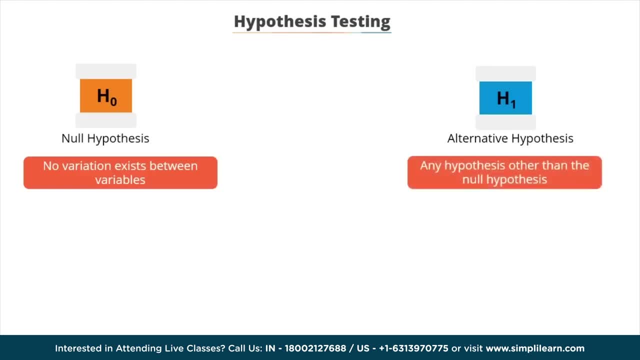 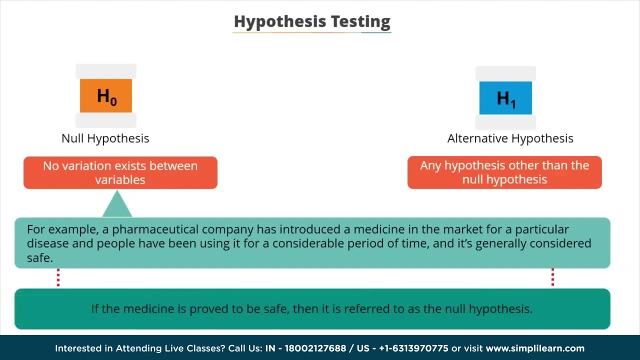 and alternative hypothesis is any hypothesis other than the null. for example say, a pharmaceutical company has introduced a medicine in the market for a particular disease and people have been using it for a considerable period of time and it's generally considered safe. if the medicine is proved to be safe, then it is referred to as null hypothesis. to reject null hypothesis: 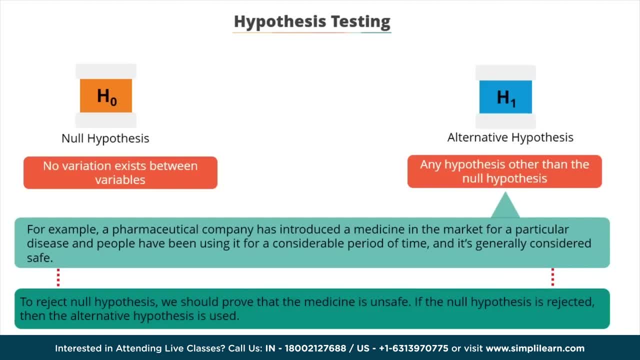 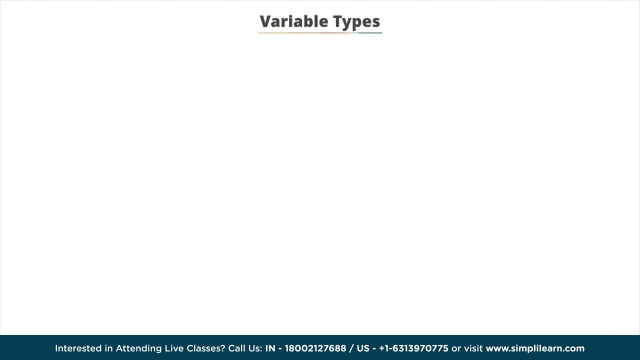 we should prove that the medicine is unsafe. if the null hypothesis is rejected, then the alternative hypothesis is used. before you perform any statistical tests with variables, it's significant to recognize the nature of the variables involved. based on the nature of the variables, it's classified into four types. they are categorical or nominal variables. ordinal variables interval. 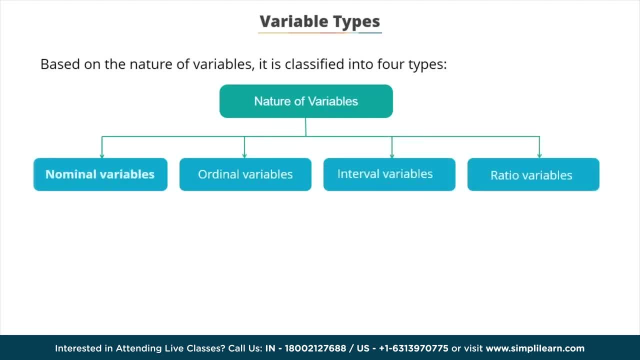 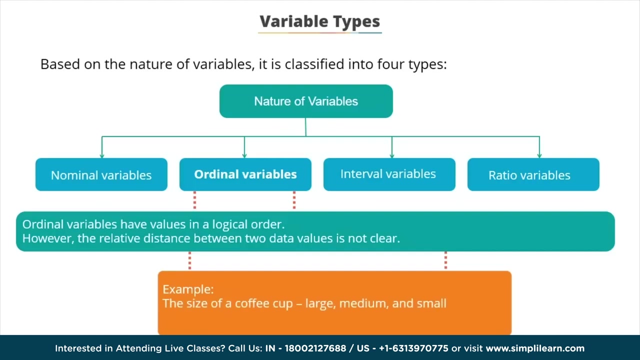 variables and ratio variables. nominal variables are ones which have two or more categories and it's impossible to order the values. examples of nominal variables include gender and blood group. ordinal variables have values ordered logically. however, the relative distance between two data values is not clear. examples of ordinal variables include considering the size of a coffee cup. 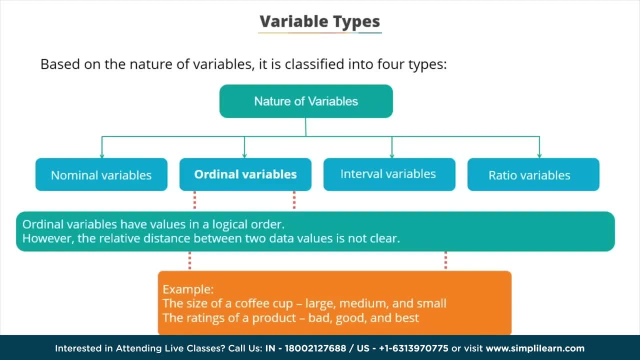 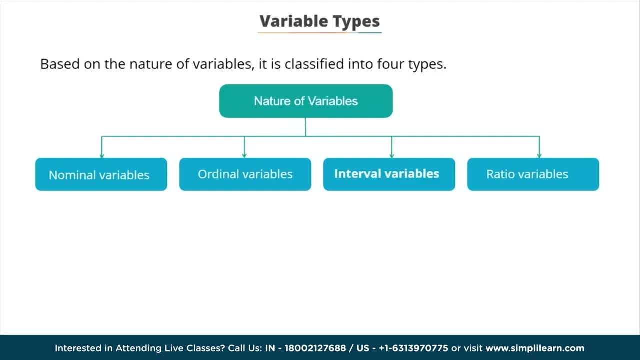 large, medium and small- and considering the ratings of a product- bad, good and best- interval variables are similar to ordinal variables, except that the values are measured in a way where their differences are meaningful, with an interval scale. equal differences between scale values do have equal quantitative meaning. for this reason, an interval scale provides more quantitative. 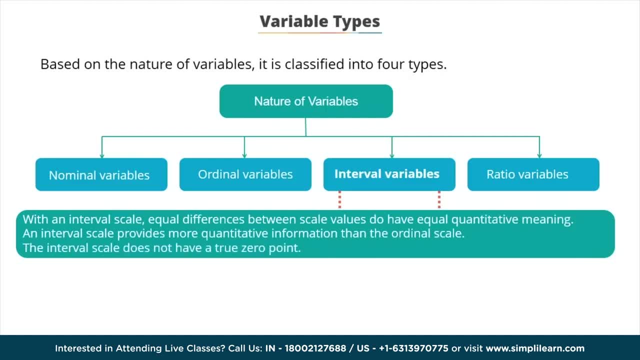 information than the ordinal scale. the interval scale does not have a true zero point. a true zero point means that a value of zero on the scale represents zero quantity of the construct being the related value. as long as the rolled Ohio today EN 來 FACTORY. 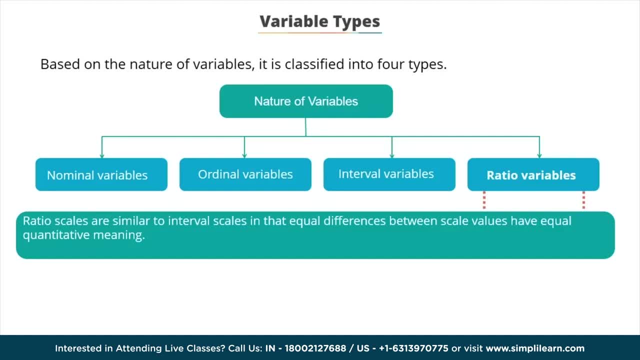 ratio scales are similar to interval scales in that, equally, differences between scale values have equal quantitative meaning. however, ratio scales also have a true zero point, which gives them an additional property. for example, the system of inches used with a common ruler is an example of a ratio scale for mao. 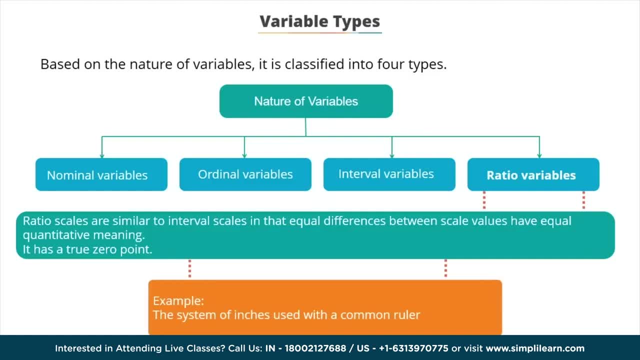 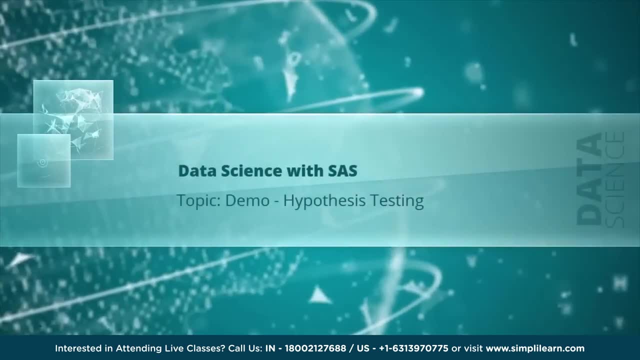 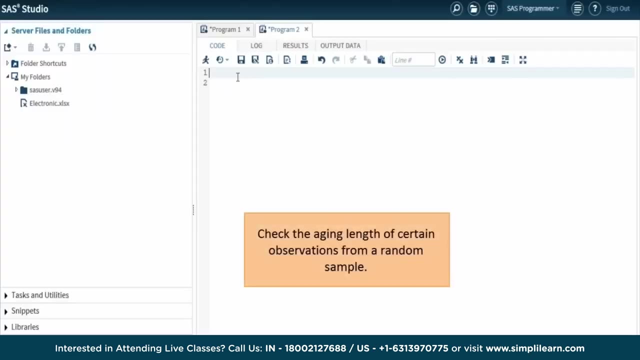 MOPE ROW, 치가 Gs. substitute Vfare y point, because 0 inches does in fact indicate a complete absence of length. In this demo, you'll learn how to perform the hypothesis testing using SAS. In this example, let's check against the length of certain observations from a random sample. 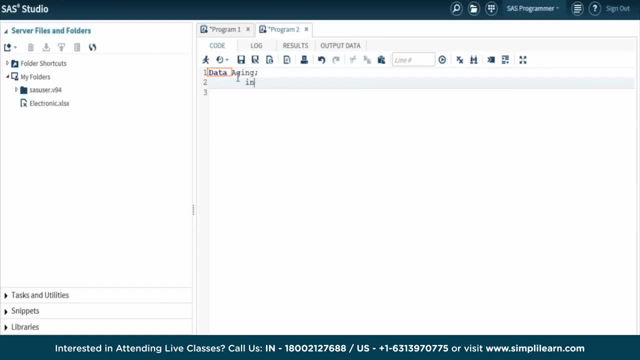 The keyword data identifies the input dataset. The input statement is used to declare the aging variable and cards to read data into SAS. Let's perform a T-test to check the null hypothesis. Let's assume that the null hypothesis runs well, hypothesis to be that the mean days to deliver a product is 6 days. 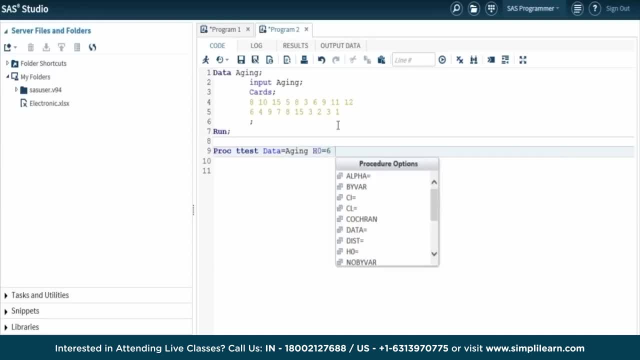 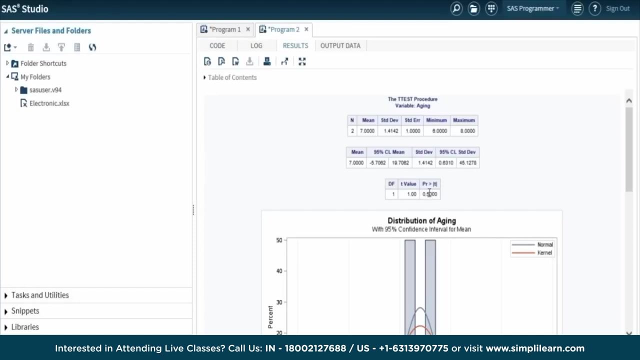 So null hypothesis equals 6,. alpha value is the probability of making an error, which is 5% standard, and hence alpha equals 0.05.. The variable statement names the variable to be used in the analysis. The output is shown on the screen. 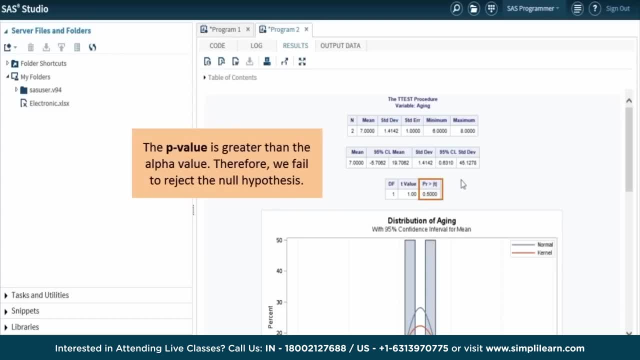 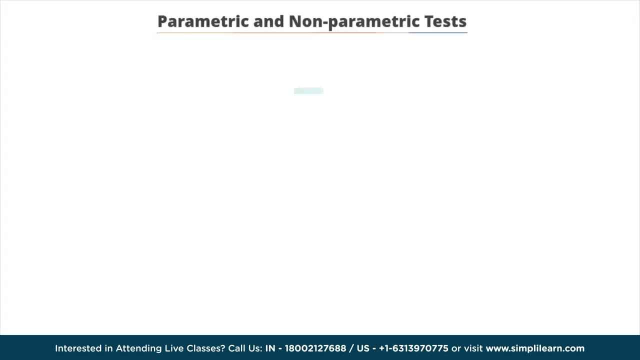 Note that the p-value is greater than the alpha value, which is 0.05.. Therefore, we fail to reject the null hypothesis. This concludes the demo on how to perform the hypothesis testing using SAS. Let's now learn about hypothesis testing procedures. 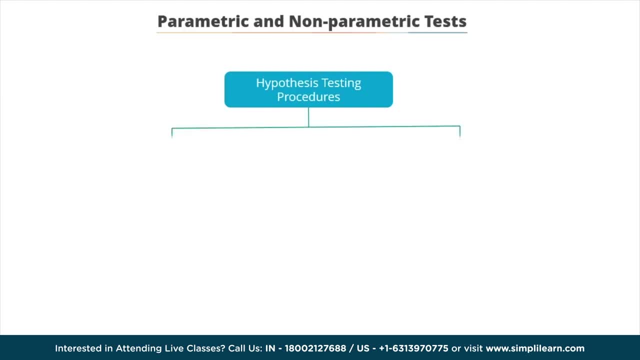 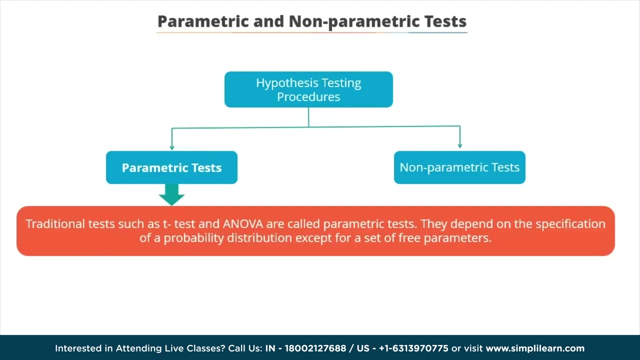 There are two types of hypothesis testing procedures. They are parametric tests and non-parametric tests. In statistical inference or hypothesis testing, the traditional tests, such as t-test and ANOVA, are called parametric tests. They depend on the specification of a probability distribution, except for a set of free parameters. 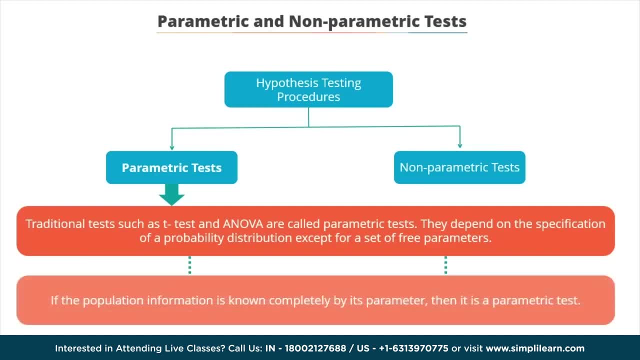 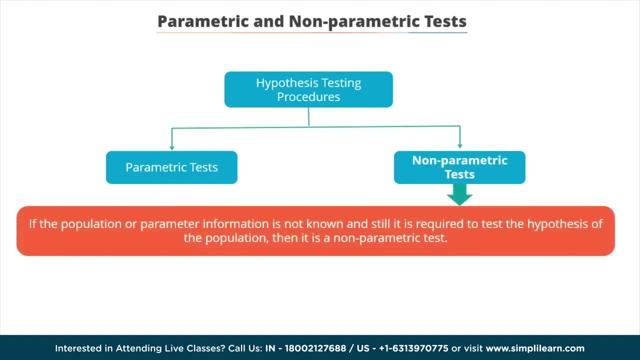 In simple words, you can say that if the population information is known completely by its parameter, then it is called a parametric test. If the population or parameter information is not known and you are still required to test the hypothesis of the population, then it is called a non-parametric test. 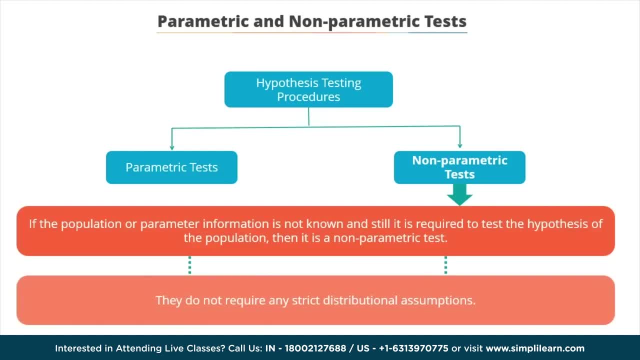 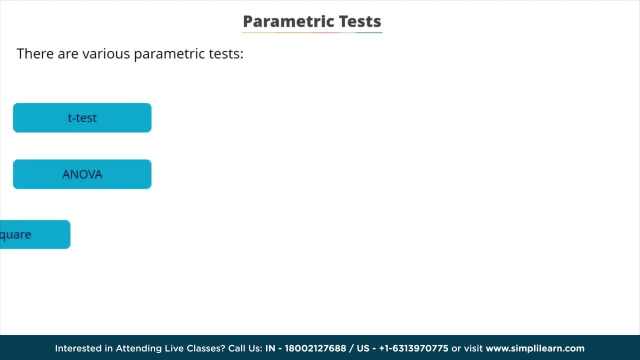 Non-parametric tests do not require any strict distributional assumptions. There are various parametric tests. They are as follows: t-test, ANOVA, chi-squared, linear regression. Let's understand them in detail. t-test: A t-test determines if two sets of data are significantly different from each other. 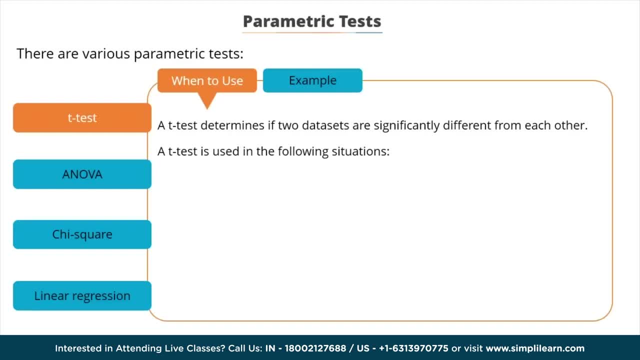 The t-test is used in the following situations: To test if the mean is significantly different than a hypothesized value. To test if the mean for two independent groups is significantly different. To test if the mean for two dependent or paired groups is significantly different. 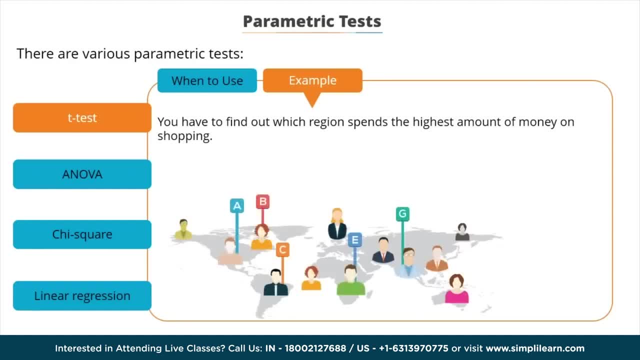 For example, Let's say you have to find a t-test, You can find out which region spends the highest amount of money on shopping. It's impractical to ask everyone in the different regions about their shopping expenditure. In this case, you can calculate the highest shopping expenditure by collecting sample. 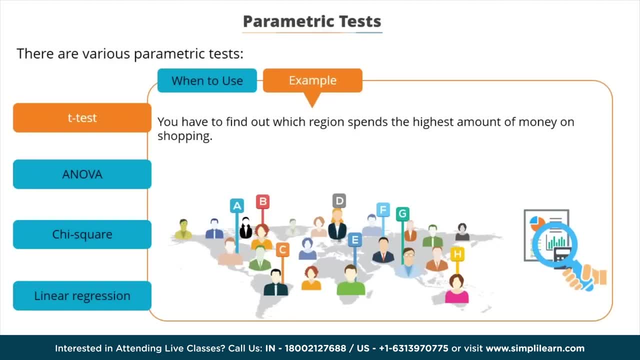 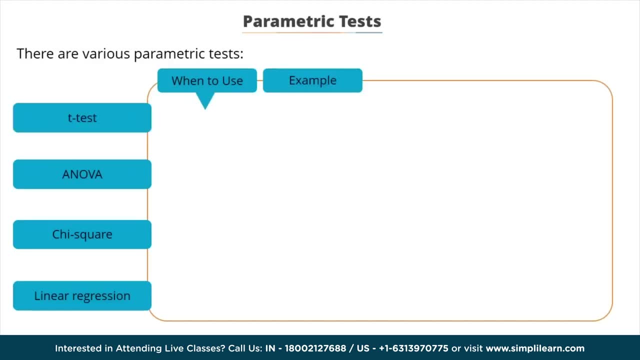 observations from each region. With the help of the t-test, you can check if the difference between the regions are significant or a statistical fluke. ANOVA. ANOVA is a generalized version of the t-test. ANOVA is a generalized version of the t-test. 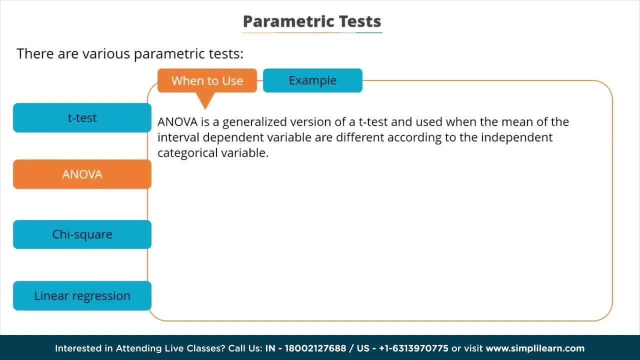 Also, it is used when the mean of the interval dependent variable is different to the categorical independent variable. When we want to check variance between two or more groups, we apply the ANOVA test, For example. let's look at the same example of the t-test example. 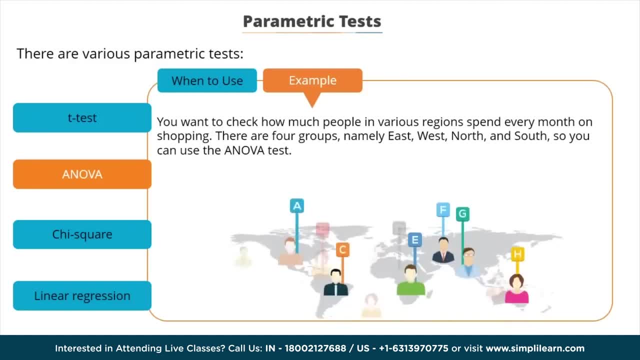 Now you want to check how much people in various regions spend every month on shopping. In this case, there are four groups, namely east, west, north and south. With the help of the ANOVA test, we can calculate how much people spend an entire month shopping. 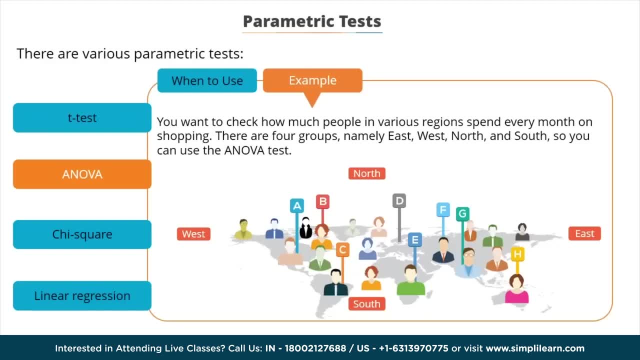 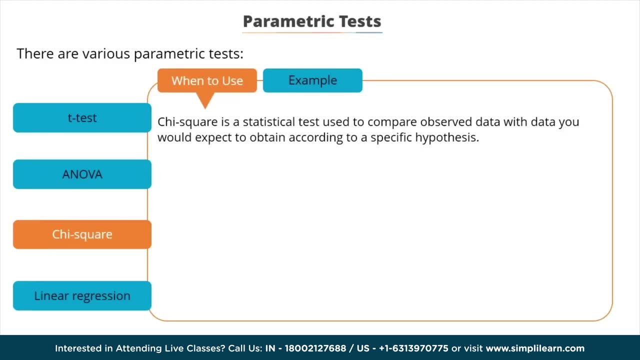 test you can check if the difference between the regions is significant or a statistical fluke- Chi-square- Chi-square is a statistical test used to compare observed data with data you would expect to obtain according to a specific hypothesis. Let's understand the chi-square test. 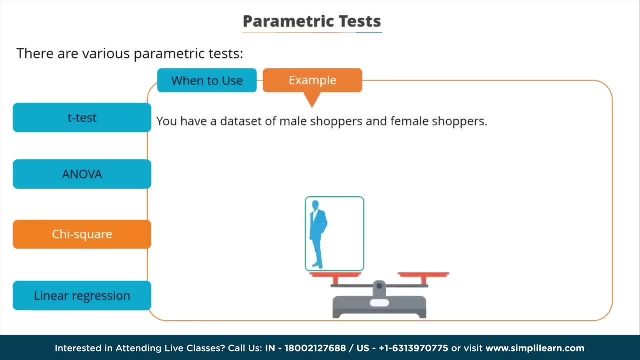 through an example. You have a data set of male shoppers and female shoppers. Let's say you need to assess whether the probability of females purchasing items of $500 or more is significantly different from the probability of males purchasing items of $500 or more. 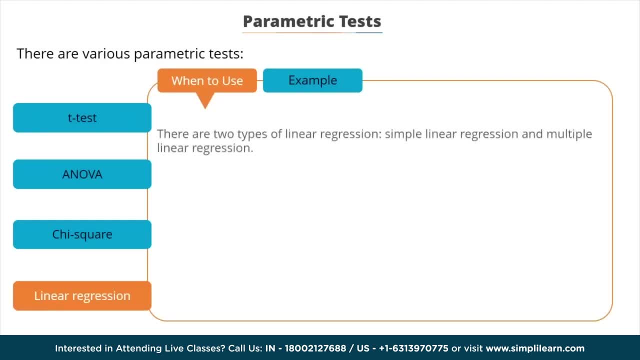 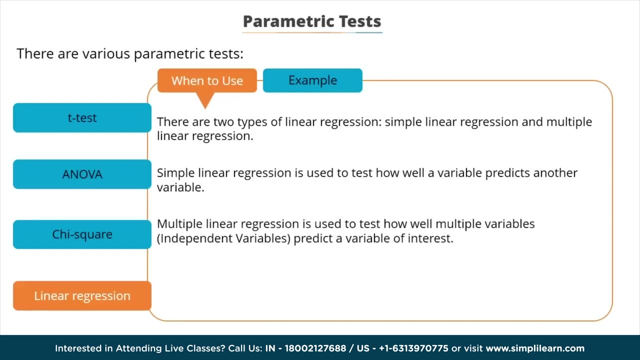 Linear regression. There are two types of linear regression: simple linear regression and multiple linear regression. Simple linear regression is used when one wants to test how well a variable predicts another variable. Multiple linear regression allows one to test how well a variable predicts another variable. 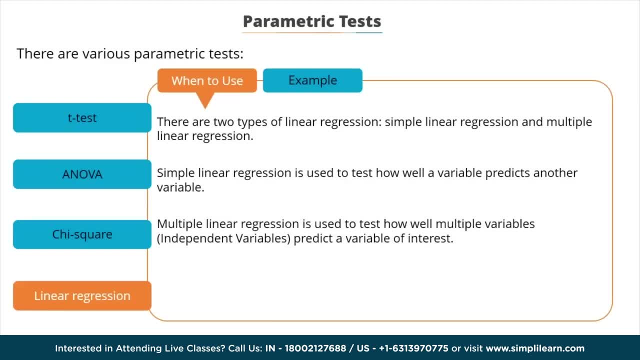 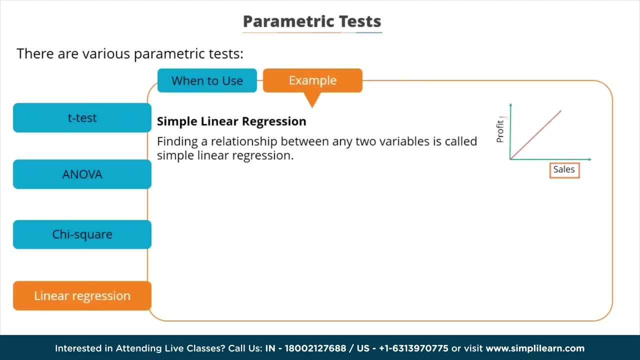 multiple variables or independent variables predict a variable of interest. When using multiple linear regression, we additionally assume the predictor variables are independent. For example, finding relationship between any two variables, say sales and profit, is called simple linear regression. Finding relationship between any three variables, say sales, cost, telemarketing, is called 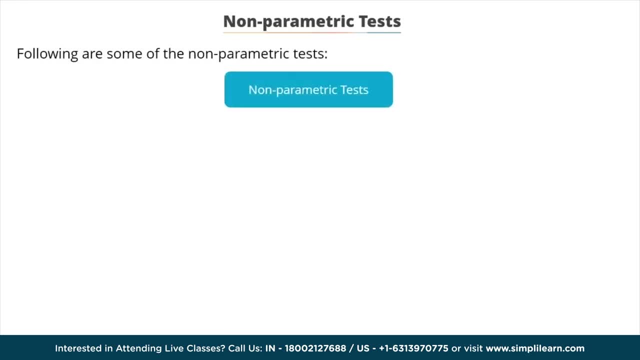 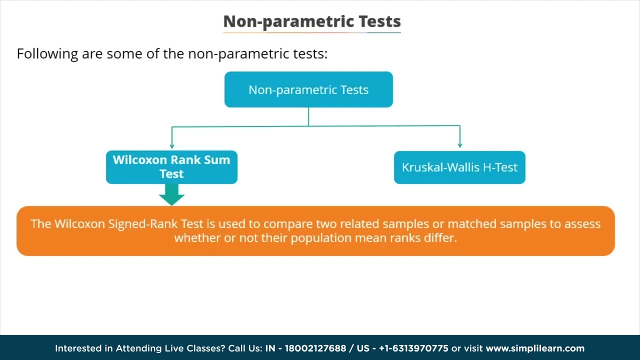 multiple linear regression. Some of the nonparametric tests are Wilcoxon Rank Sum Test and Kruskal-Wallis H-Test. Wilcoxon Rank Sum Test: The Wilcoxon-signed Rank Test is a nonparametric statistical hypothesis test used to compare. 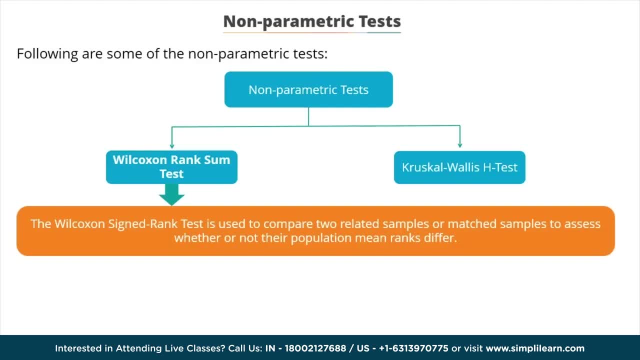 two related samples or matched samples to assess whether or not their population mean ranks differ. In Wilcoxon Rank Sum Test, you can test the null hypothesis on the basis of the ranks of the observations. Kruskal-Wallis H-Test: Kruskal-Wallis H-Test is a rank-based nonparametric test used to compare independent samples of 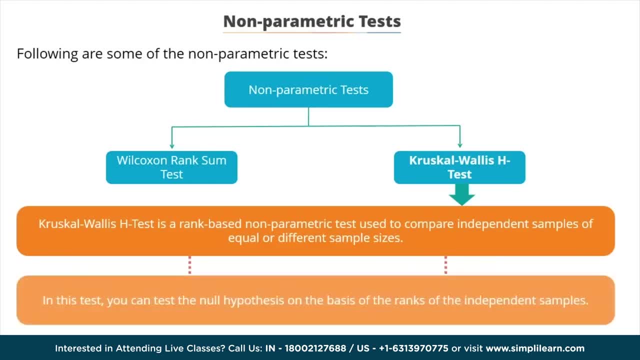 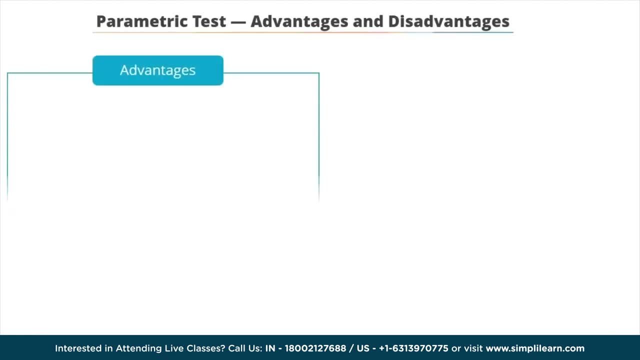 equal or different sample sizes. In this test, you can test the null hypothesis on the basis of the ranks of the independent samples. The advantages of parametric tests are as follows: Provide information about the population in terms of parameters and confidence intervals. Provide data information about the population. 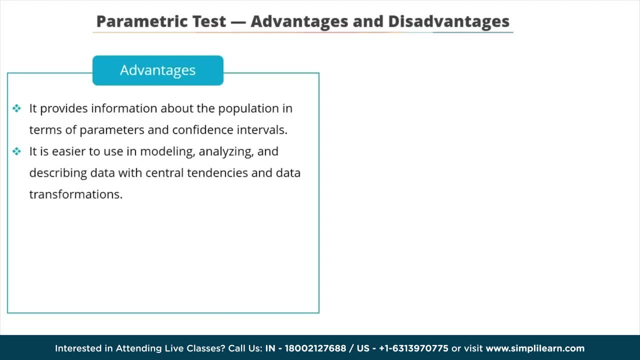 Easier to use in modeling, analyzing and for describing data, with the data used to with central tendencies and data transformations. Express the relationship between two or more variables. Don't need to convert data into rank order to test. The disadvantages of parametric tests are as follows: 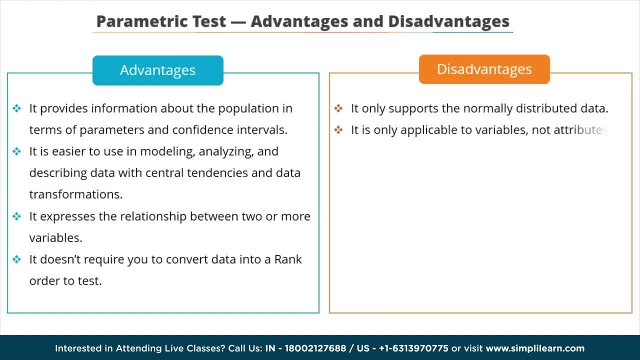 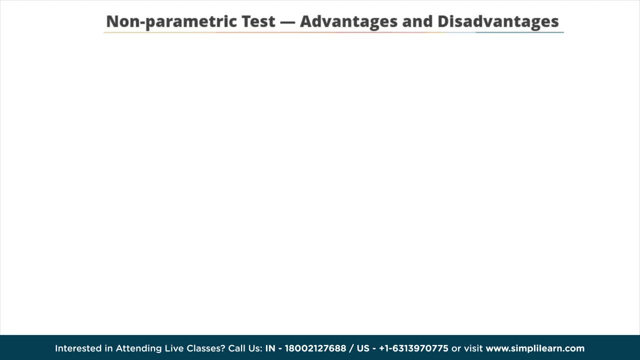 Only support normally distributed data, Only applicable on variables, not attributes. Let's now list the advantages and disadvantages of nonparametric tests. The advantages of nonparametric tests are as follows: Simple and easy to understand, Do not involve population parameters and sampling theory. 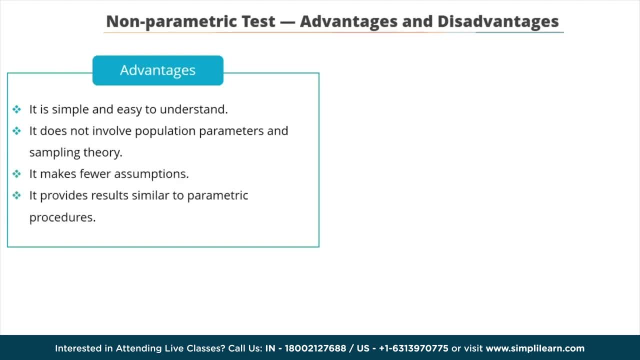 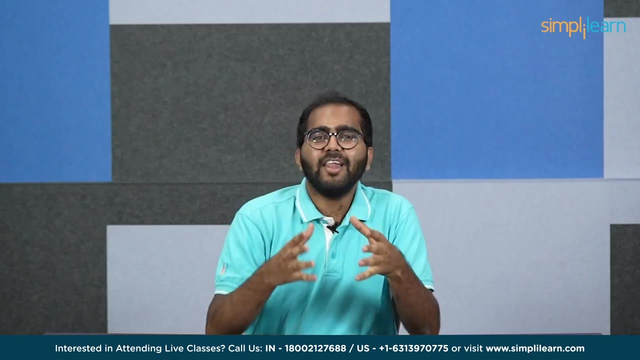 Make fewer assumptions, Provide results similar to parametric procedures. The disadvantages of nonparametric tests are as follows: Not as efficient as parametric tests. Difficult to perform operations on large samples manually. Hello everyone, Welcome to Simply Learn You. 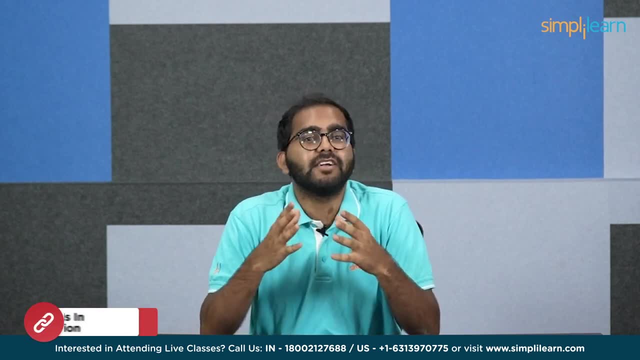 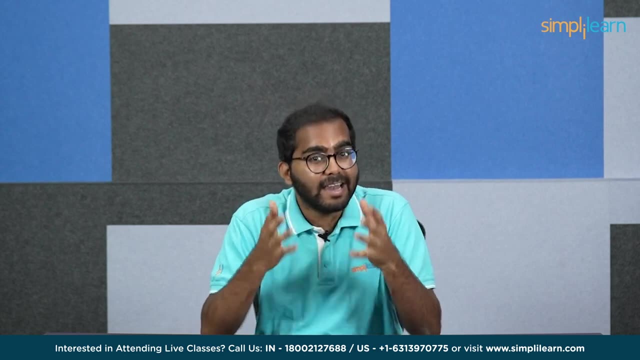 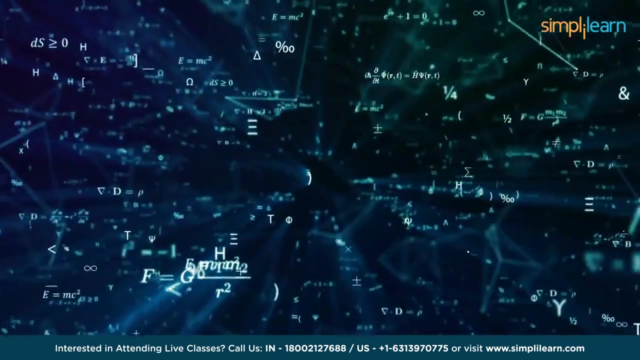 Welcome to Simply Learn. Today, we will delve into statistics and uncover the 10 most essential concepts every data scientist should know. Statistics form the backbone of data science, allowing us to extract valuable insights and make informed decisions from raw data. In this video, we will explore various fundamental statistical concepts, essential for any aspirant. 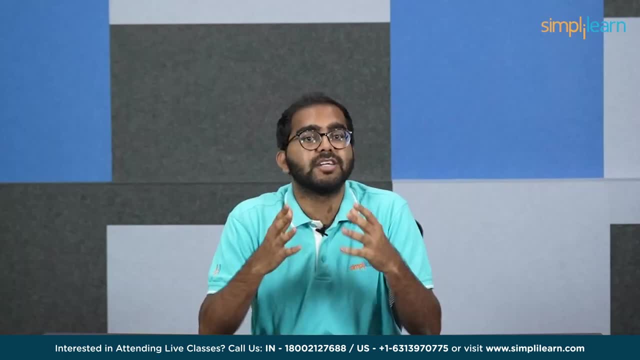 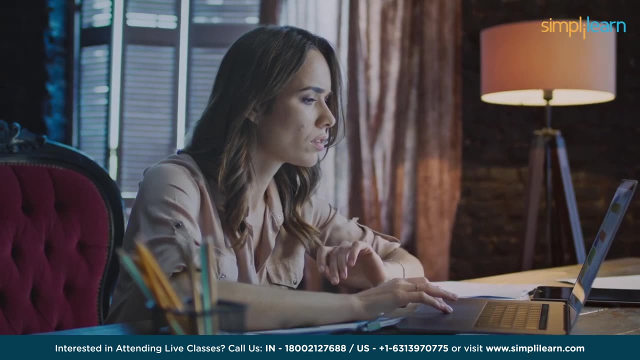 data scientist. We will start with descriptive statistics, which helps us understand the essential characteristics of a dataset. From there we will move on to inferential statistics, enabling us to make predictions and draw conclusions. We will also explore statistical patterns and conclusions about larger populations based 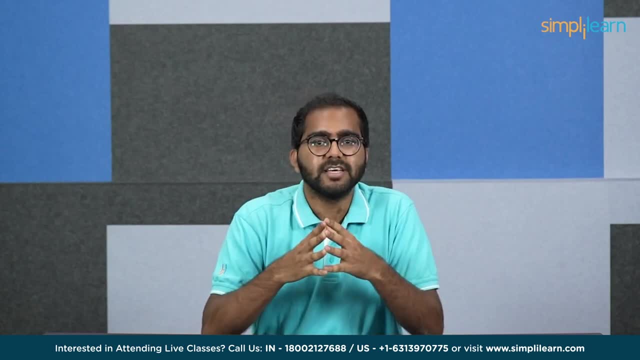 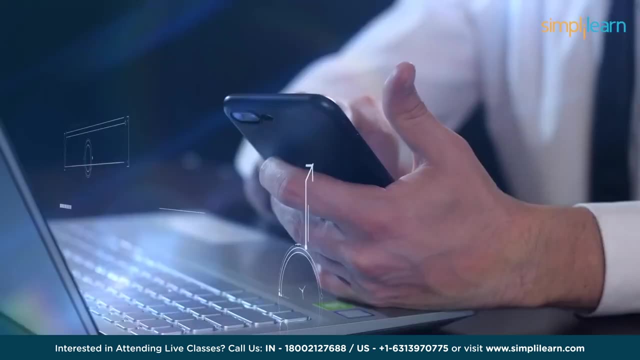 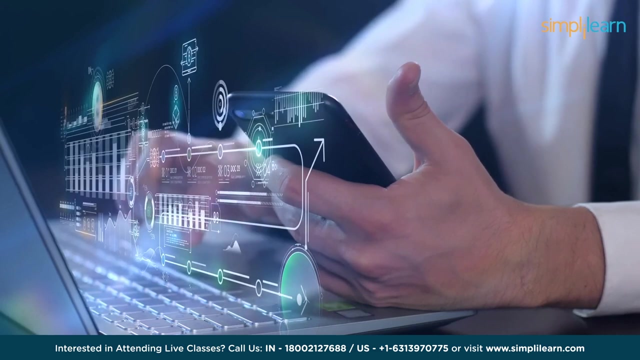 on sample data. Probability, a cornerstone of statistics, will be our next stop. We will uncover how it quantifies uncertainty and plays a crucial role in data analysis. We will also cover sampling techniques, regression analysis and hypothesis testing, which are indispensable tools for understanding relationships, making inferences and validating hypotheses. 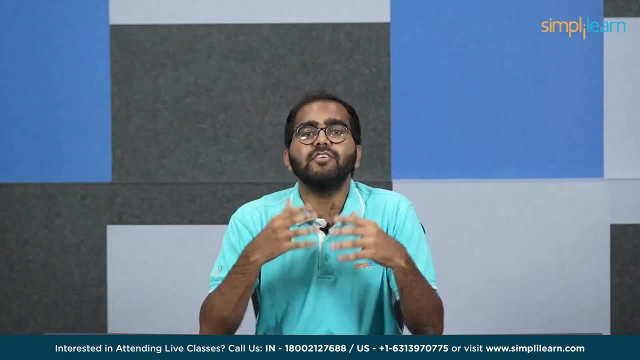 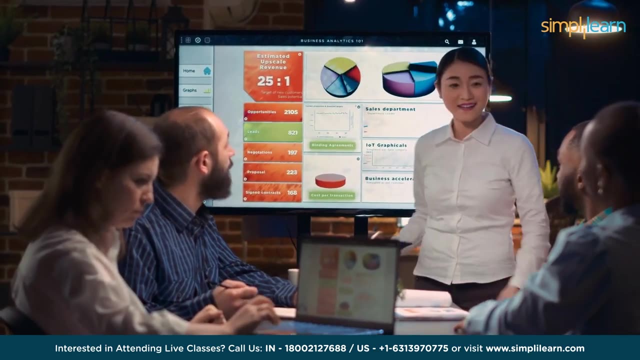 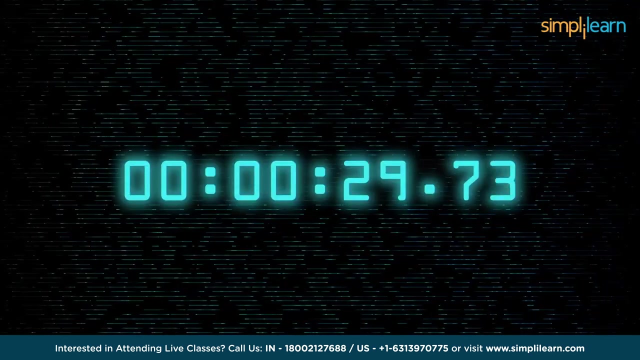 Furthermore, we will dive into statistical distributions, which provide a framework for understanding data patterns and behavior. statistical inference and experimental design will be explored, emphasizing the importance of drawing meaningful conclusions and ensuring reliable results. Finally, we will touch upon time series analysis, a vital skill for analyzing and forecasting. 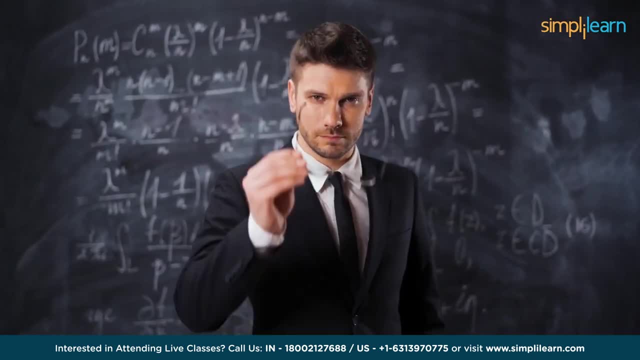 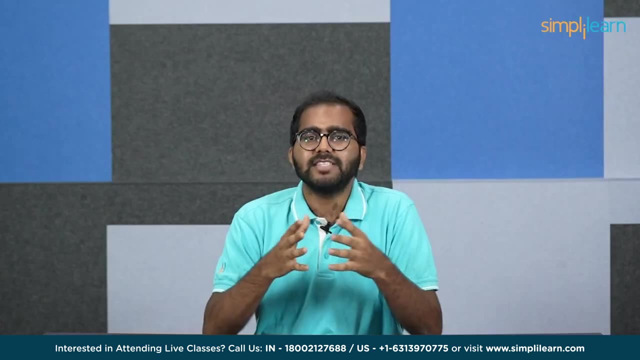 data collected over time. By the end of this tutorial, you'll have a solid foundation in these 10 key statistic concepts, empowering you to confidently embark on your data science journey. So let's dive in and unlock the power of statistics in data science. 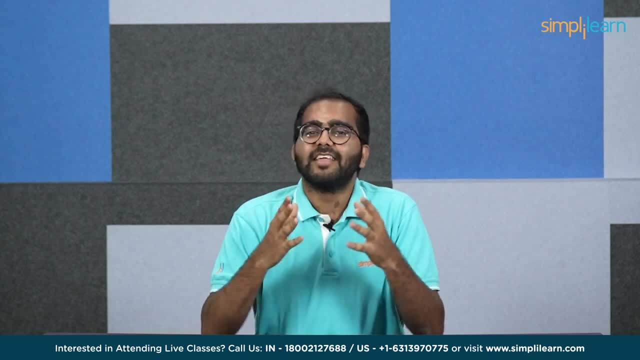 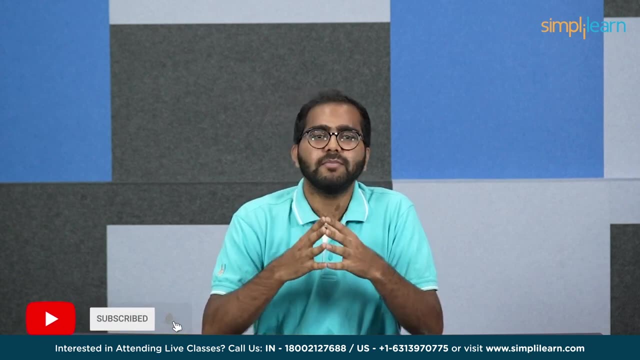 But before we get started, if these are the types of videos you'd like to watch, then you know how YouTube algorithm works. Let's do the drill: get subscribed to our YouTube channel, like our videos and hit the bell icon to never miss an update from Simply Learn. 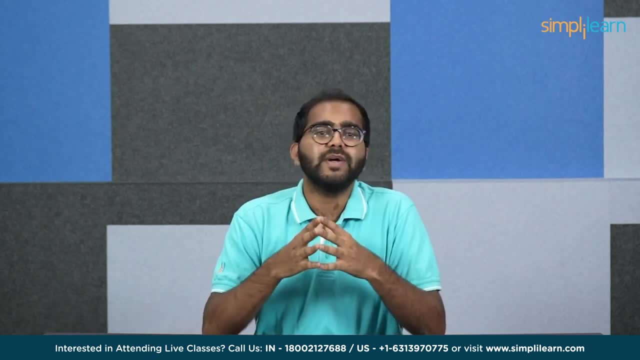 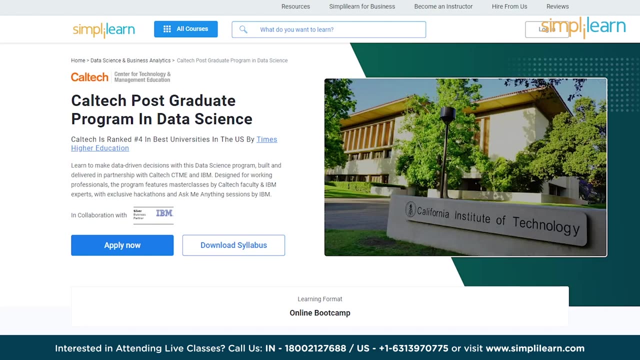 If you're one of the aspiring data scientists looking for online training, graduating from the best universities, or a professional who elicits to switch careers with data science by learning from the experts, then try giving a shot to Caltech postgraduate program in data science from Simply Learn, in collaboration with IBM. 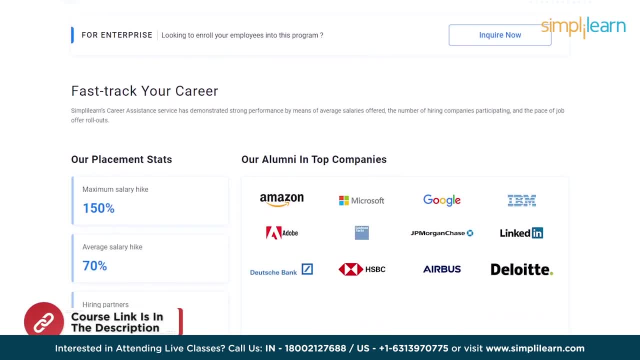 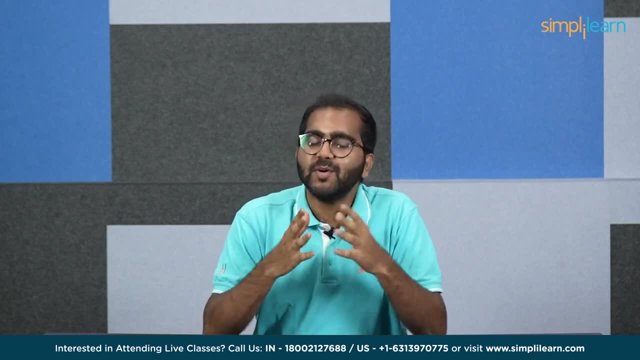 The link in the description box should navigate you to the link, And on the homepage you can find a complete overview of the program being offered. Let's begin with discussing the top 10 most important statistics concepts for data science Over to our training experts. 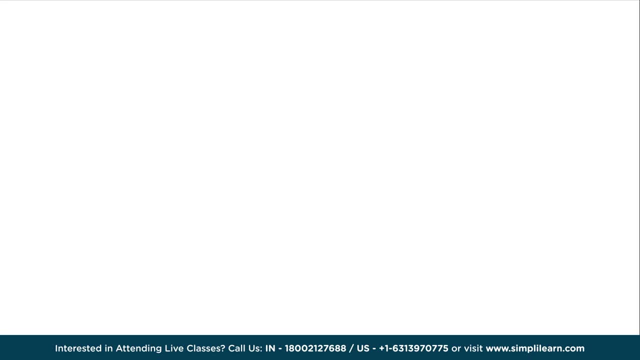 Hello all. Let's get started with the top 10 most important statistics concepts for data science. First on the list is Descriptive statistics. Descriptive statistics involves summarizing and describing the main features of a data set. It includes measuring, such as mean, median mode, sketch and accuracy. 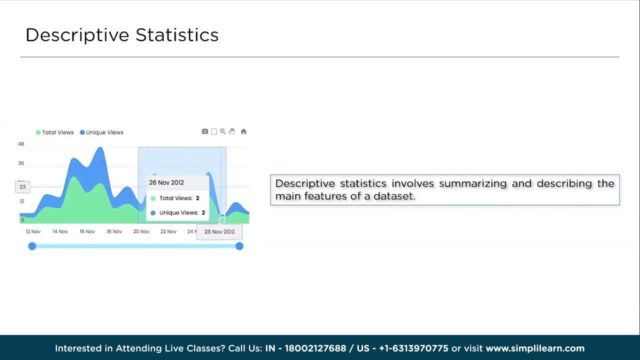 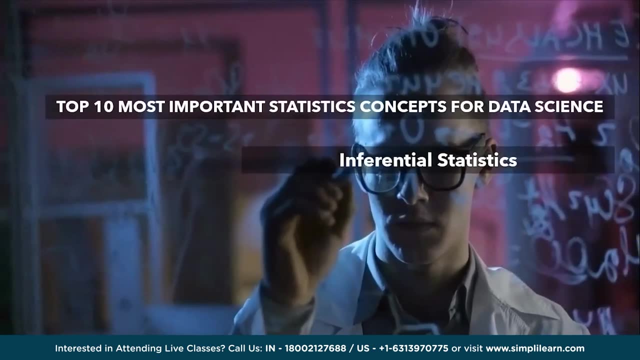 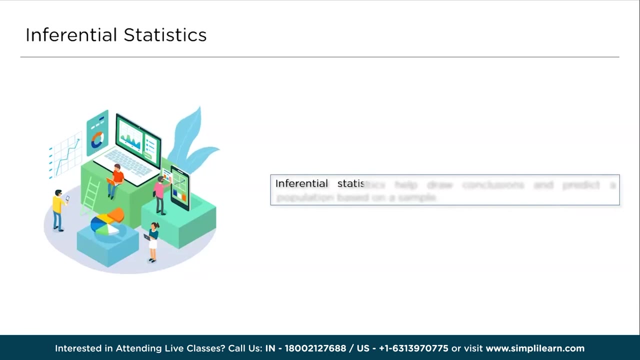 standard deviation and range, which provide insights into the data's central tendency, spread and distribution. Now, proceeding ahead, we have inferential statistics. Inferential statistics help draw conclusions and predict a population based on a sample. It involves hypothesis testing, confidence intervals and p-values allowing data scientists 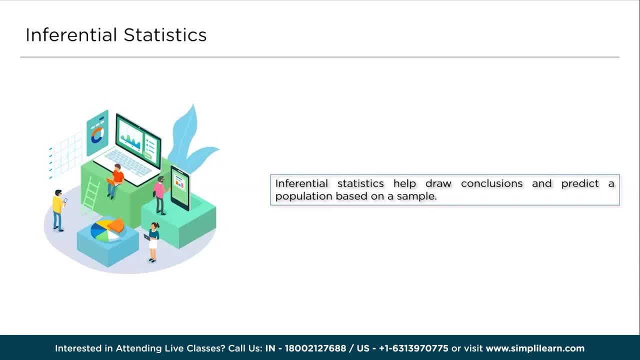 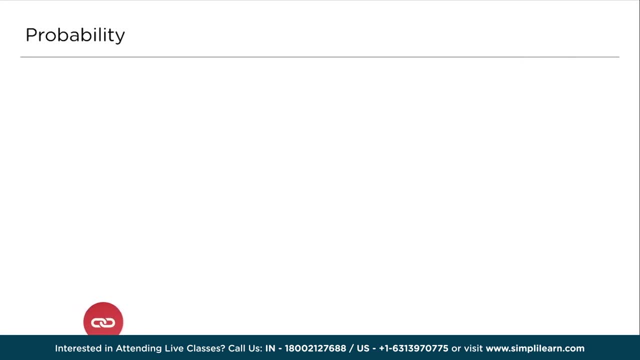 to make informed decisions and statements about the population from which the sample was drawn. Next on the docket is probability. Probability is the foundation of statistics. It measures the likelihood of an event occurring and enables data scientists to qualify uncertainly. Understanding probability is crucial for tasks such as estimating probabilities. 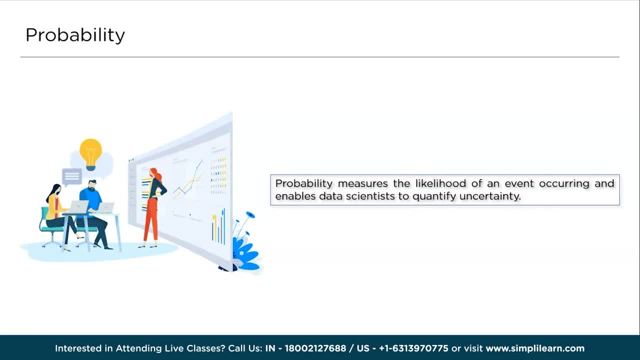 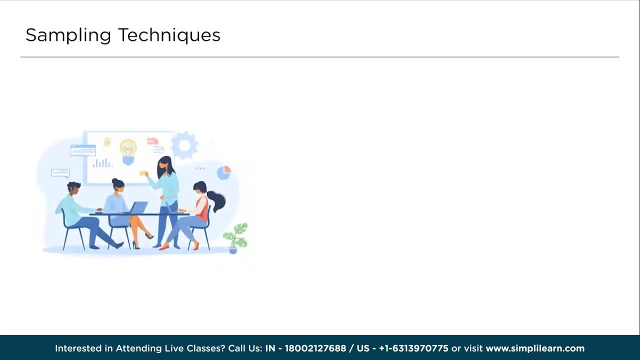 calculating expected values and conducting Bayesian analysis. The fourth one on the list is sampling techniques. Sampling techniques are essential for collecting representative data from a population. Simple random sampling, satisfied sampling, cluster sampling and systematic sampling are standard techniques used to ensure that the sample accurately reflects the characteristics. 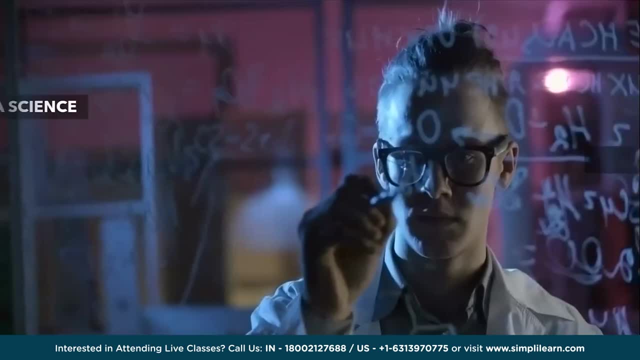 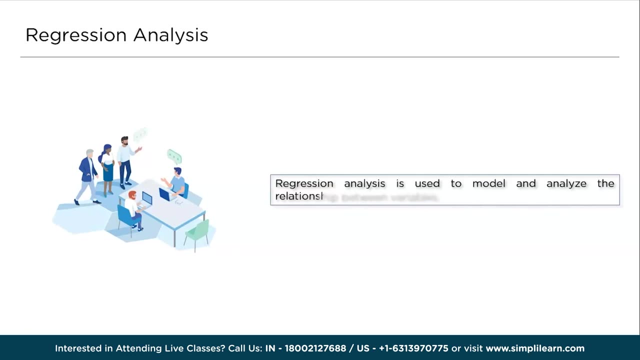 of population. The fifth one on the docket is regression analysis. Regression analysis is used to model and analyze the relationship between variables. Simple, linear, multiple and logistic regression are commonly used techniques to understand how one or more variables in a population can be calculated. The sixth one on the list is performance and outcome, or dependent. 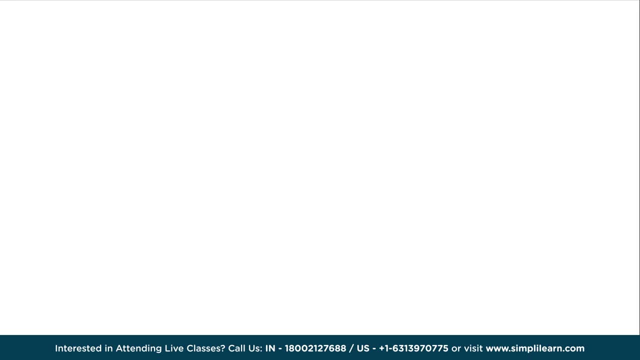 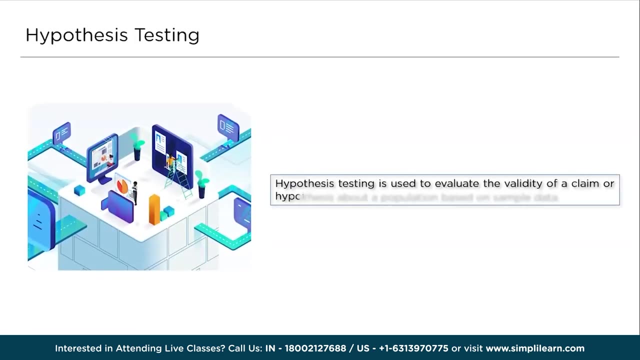 variable Proceeding ahead. we have hypothesis testing. Hypothesis testing is used to evaluate the validity of a claim or hypothesis about a population based on sample data. It involves setting up a null and alternative hypothesis, calculating test statistics and make decisions. 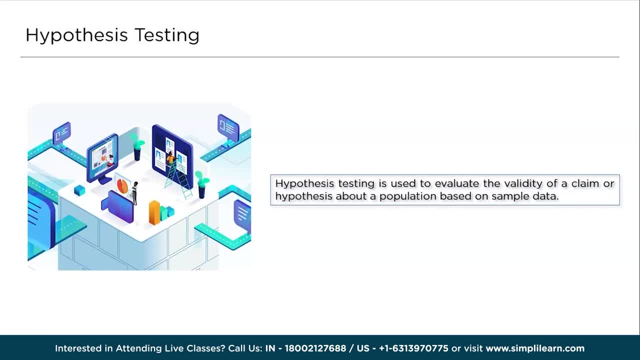 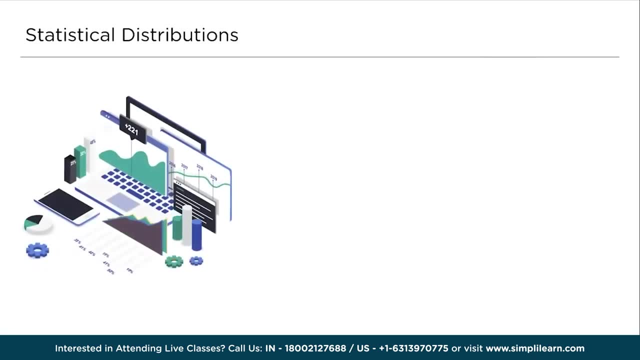 based on p-values and significance levels. With that we can move on to the next one, that is, statistical distributions. Statistical distributions describe data patterns and behavior. Understanding distributions such as the normal binomial and Poisson distribution is crucial for analyzing and 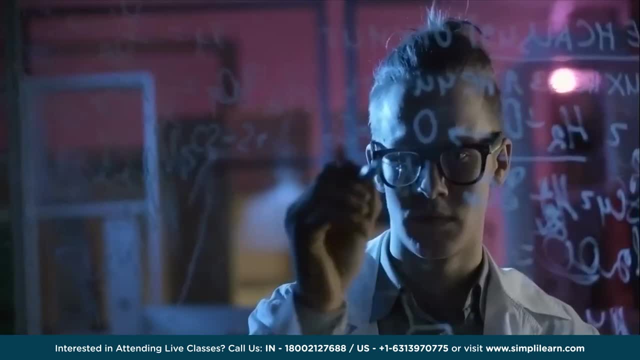 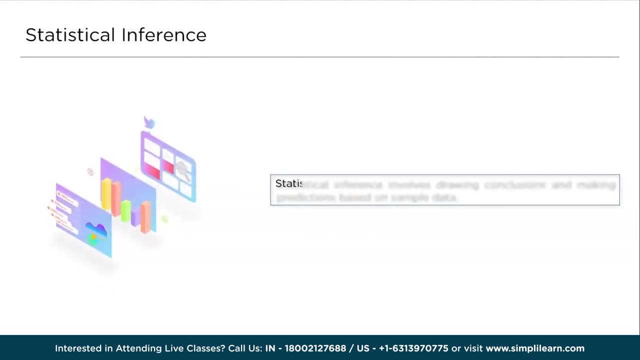 modeling various data types. Now we have the statistical inference in the eighth place. Statistical inference involves drawing conclusions and making predictions based on sample data. It includes concepts such as confident intervals, margin of error and sample size determination, which help quantify the precision and 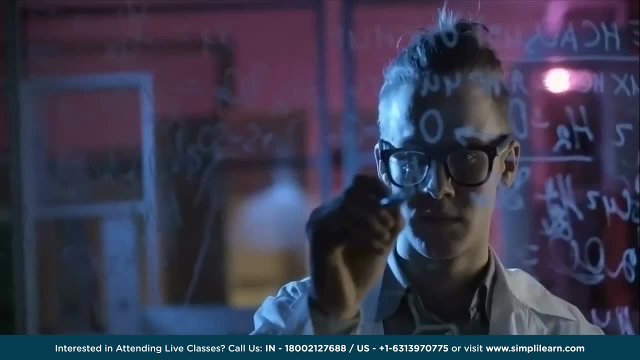 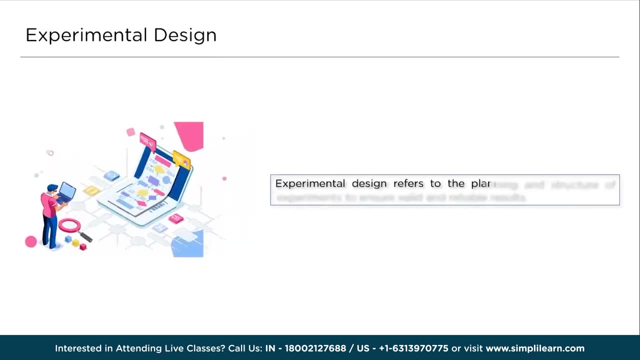 reliability of estimates and predictions. Proceeding to the ninth one, we have experimental design. Experimental design refers to the planning and structure of experiments to ensure valid and reliable results. Concepts such as randomization, control groups and replication are used to minimize bias, and cofounding variables allow data scientists to make casual. 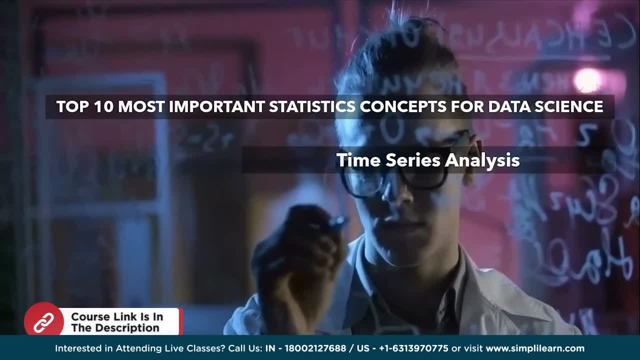 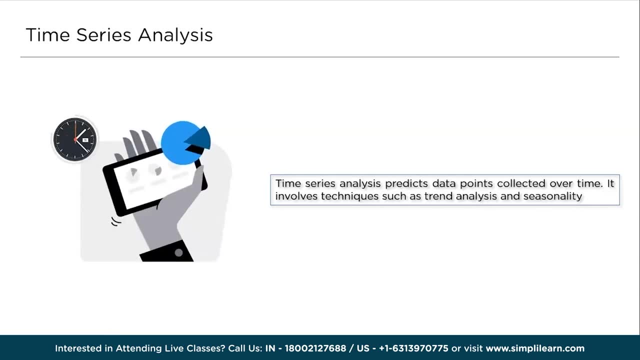 inferences. Finally, we have the most important one on the tenth place: Time series analysis. Time series analysis analyzes and predicts data points collected over time. It involves techniques such as trend analysis, seasonality and auto-regressive integrated move and auto-regressive integrated moving average or ARIMA models, which are useful. 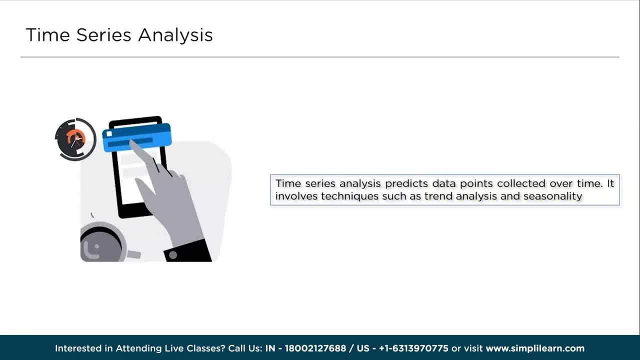 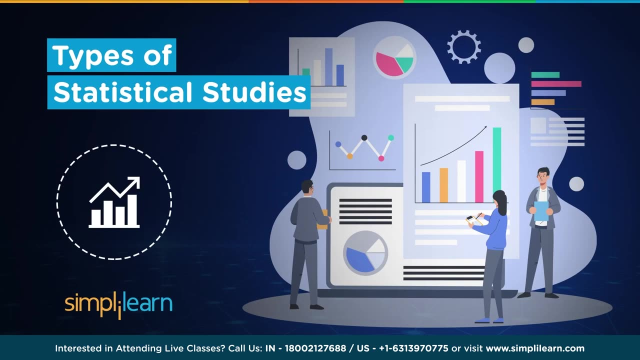 for forecasting and understanding temporal patterns in data. These 10 statistics concepts will provide a solid foundation for data scientists to explore, analyze and draw meaningful insights from data. In today's session, we will discuss about types of statistical studies. A statistical study is a four-step process that begins by asking the right questions. 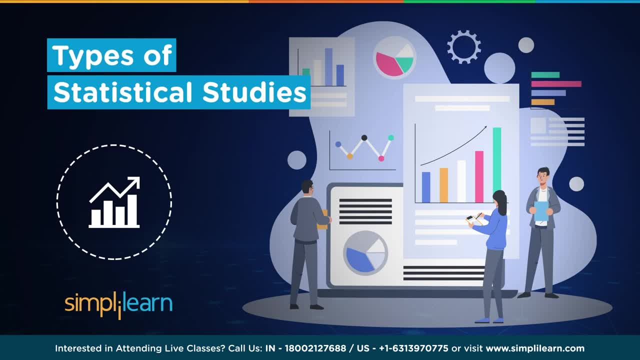 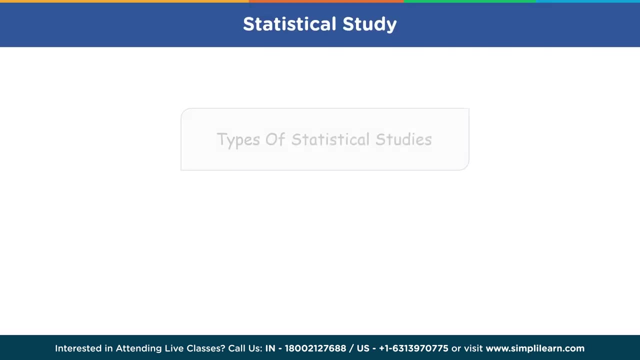 The steps are to collect appropriate data and organize and analyze the data to arrive at a proper conclusion. So in this session we will discuss what types of statistical studies are used to finally arrive at the conclusion. There are mainly three types of statistical studies. 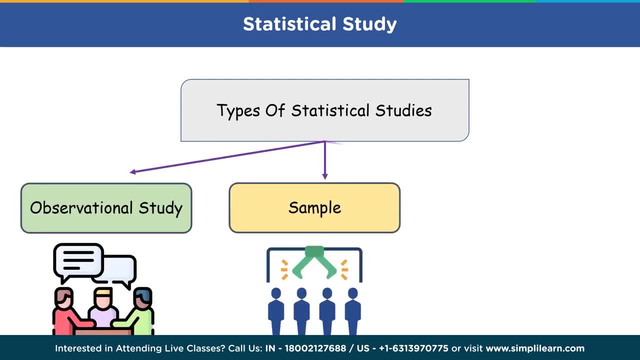 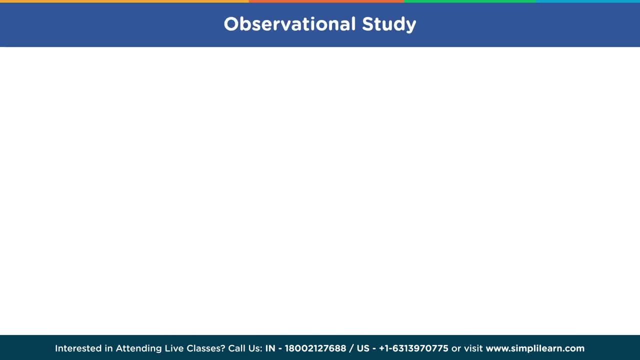 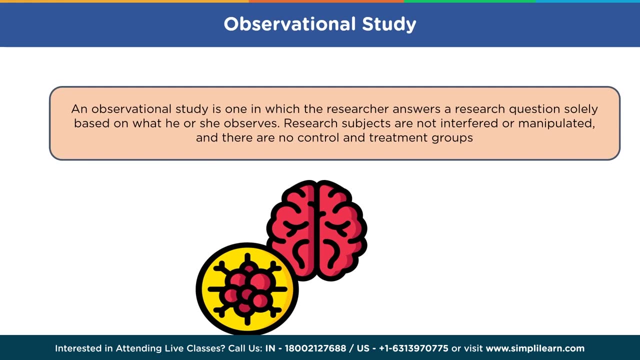 The first one is observational study, the second one is sample and the third are the experiments. Let's discuss each one of them in detail. Observational Study: An observational study is when researchers are looking at the effect of some types of intervention, risk, a diagnostic test or treatment, without trying to manipulate who or what. the 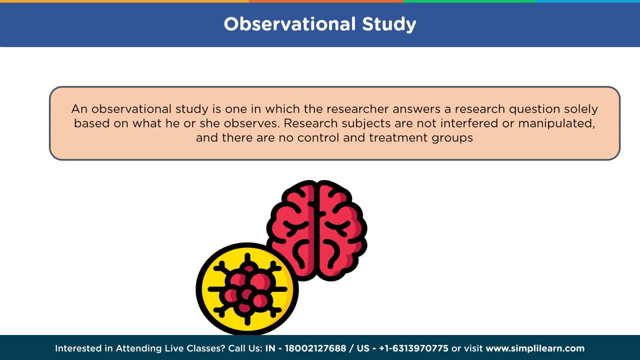 subject is: There is no interference on the research subjects. Let's try to understand this with the help of an example. Suppose a researcher investigates the link between the use of cell phones and the brain cancer. There are two variables in this study. One is the extent of the cell phone usage and the second one is whether the person has. 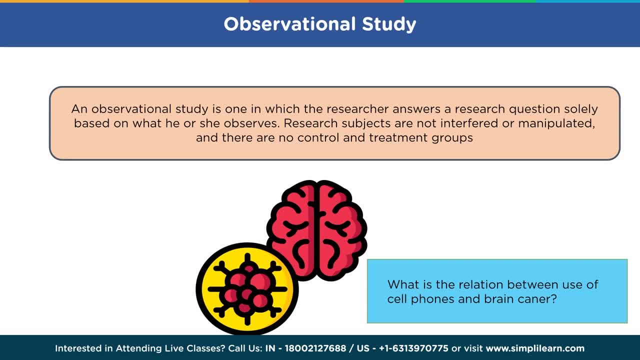 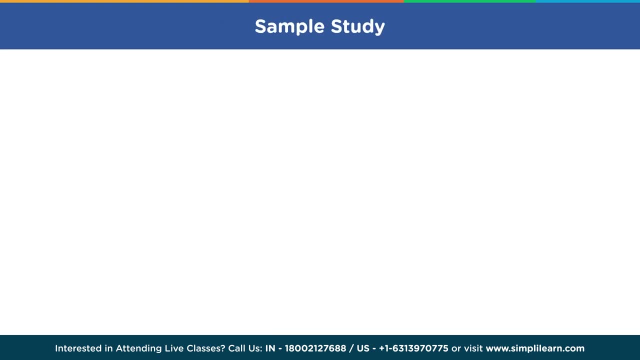 a brain cancer previously or not. Both variables are measured for the group of people. This is an observational study. There was no attempt to influence the study. There was no attempt to influence people's cell phone usage to see if different levels of usage made any difference in whether or not a person developed the brain cancer. 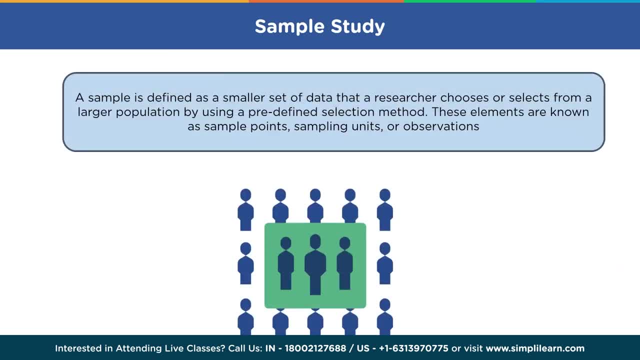 Sample Study. In statistics, a sample is an analytical subset of a larger population. The use of samples allow researchers to conduct their studies with more manageable data and in a timely manner. Randomly drawn samples do not have much bias if they are large enough. but achieving such 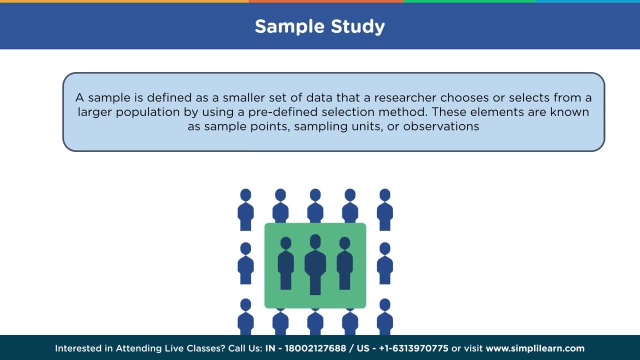 a sample may be expensive and time-consuming. The results of this study show that the use of samples in a larger population is more effective and time-consuming. Let's understand this with the help of an example. Suppose a company has 800 female employees and 200 male employees. 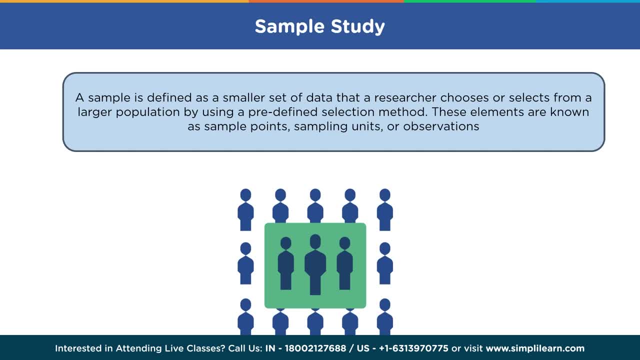 You want to ensure that the sample reflects the gender balance of the company, So you sort the population in two strata based on gender. Then you use random sampling on each group by selecting 80 women and 20 women respectively, which will give you the representative sample of 100 people. 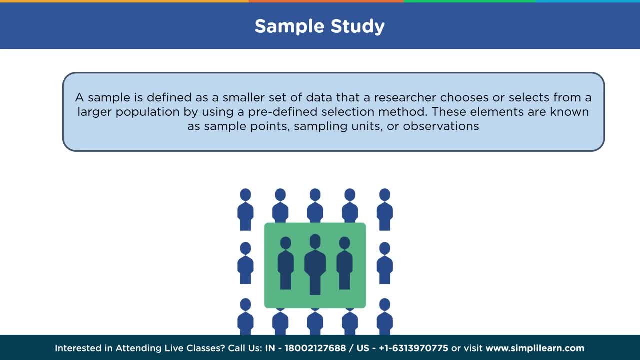 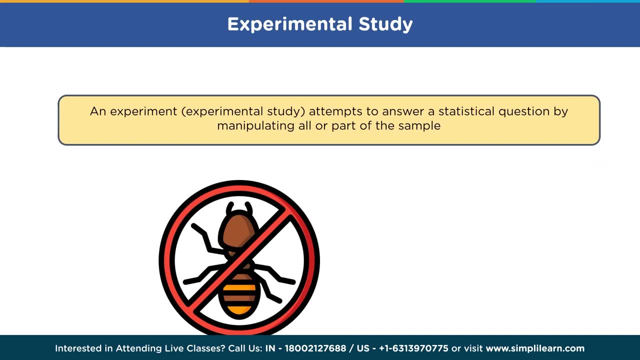 Now you can conduct your statistical analysis on these 100 people to arrive at a larger conclusion. The last one is Experimental Study. Experimental studies involve the random assignment of participants into different groups in order to determine the casual effect of a certain condition on a certain outcome. 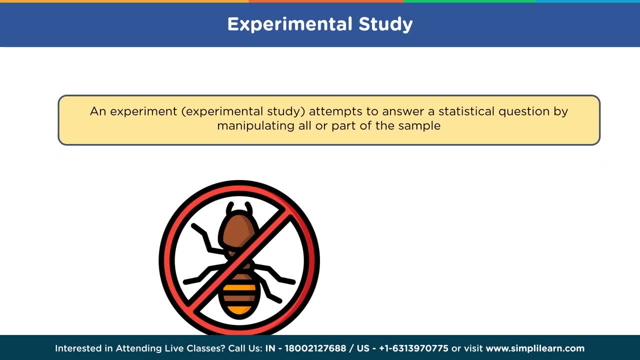 Suppose that an observational study indicated that a certain type of tree did not have much termite damage as the other trees, Researchers wondered if the resin from the trees was toxic to termites, So they decided to do an experiment where they exposed some termites to the resin. 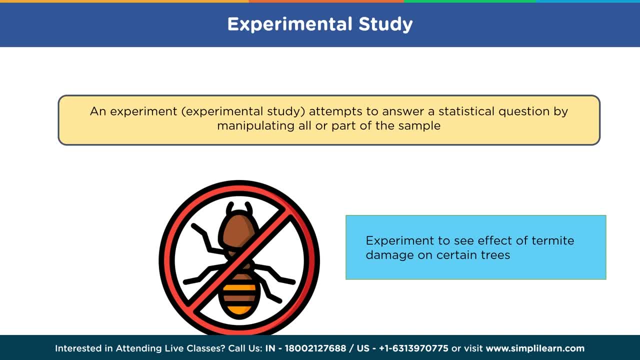 The results of the experiment showed that the resin from the trees was toxic to termites. So they decided to do an experiment where they exposed some termites to the resin And the other were the plain water and recorded whether the termites survived, And the other were the plain water and recorded whether the termites survived. 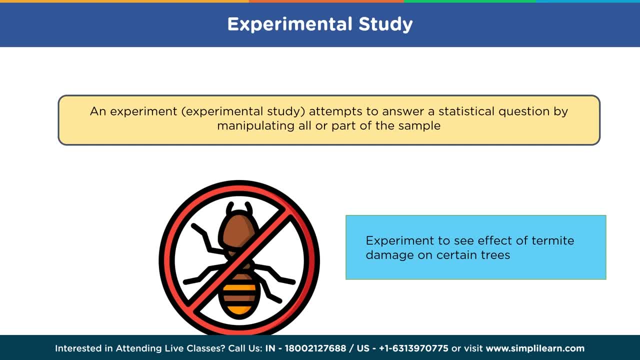 And the other were the plain water- and recorded whether the termites survived. The explanatory variable, ie the treatment variable, is the exposure type- Resin- Plain water- and the response variable is whether or not the termite survived. We can state that this is an experiment because the researchers imposed a treatment on the 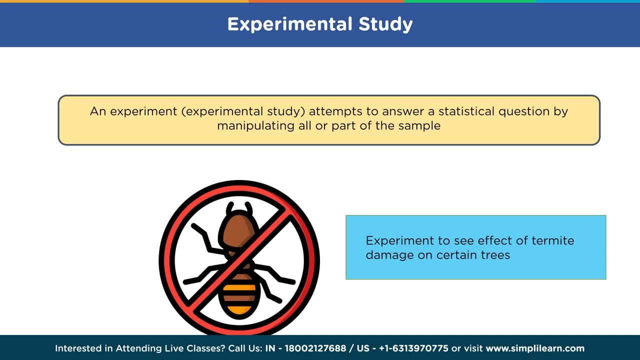 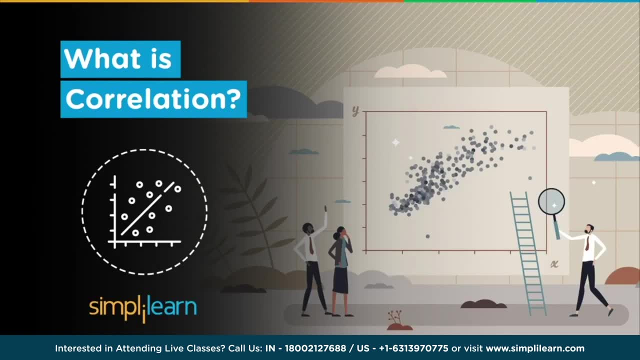 subjects. This can be termed as an Experimental study. In this session, we will discuss a very widely used term in statistics, ie correlation, And we will also see what is the significance of correlation. What is the significance of correlation and where it is used. 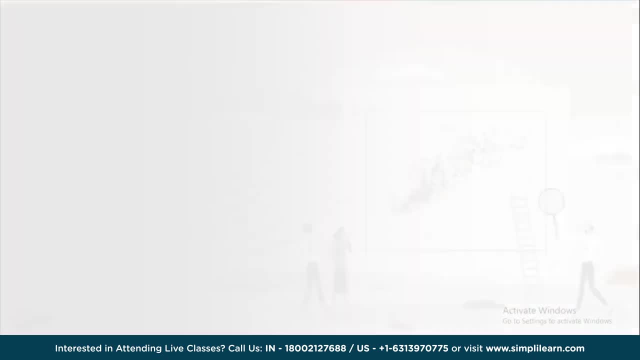 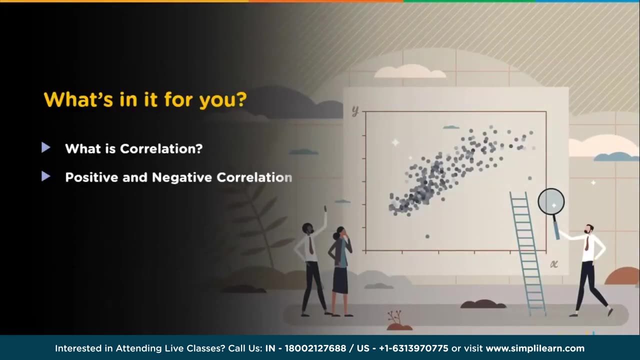 So let's discuss the agenda for today's session. We will start this tutorial by understanding what is correlation. Then we will move on to discuss the two types of correlation and correlation coefficient. After that we will see the limitations of correlation and some real-life applications. 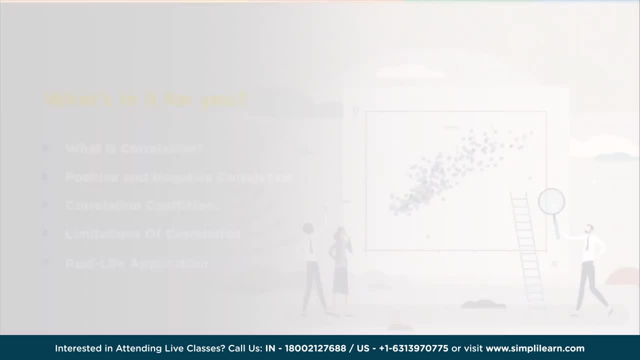 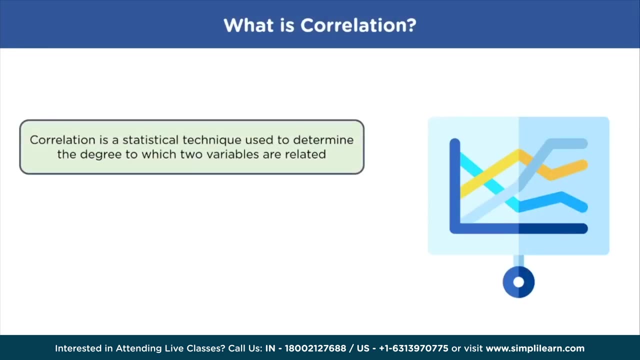 of correlation. So let's get started. What is correlation? Correlation refers to a statistical relationship between the two entities. It measures the extent to which the two variables are linearly related. For example, the price and demand of a product is in correlation. 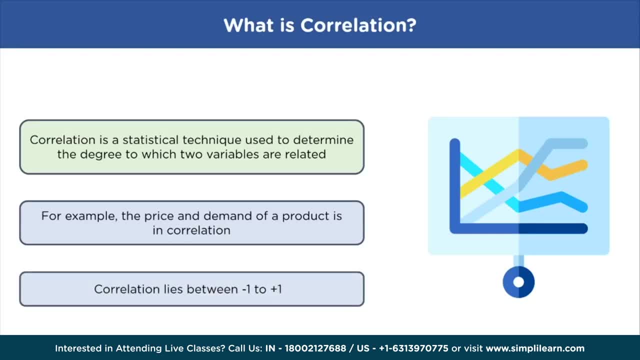 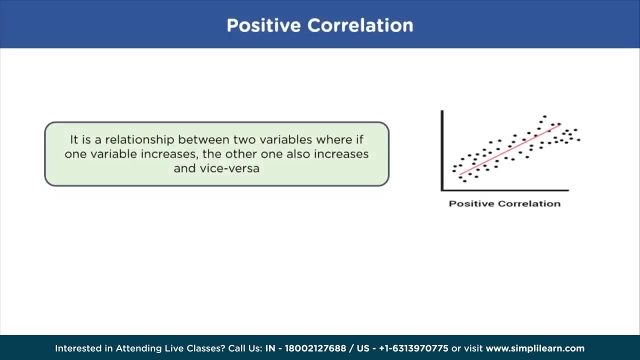 They are linearly related. The value of correlation always lies between minus one to plus one. There are mainly two types of correlation. The first one is positive correlation. A positive correlation means that the linear relationship is positive And the two variables increases or decreases in the same direction. 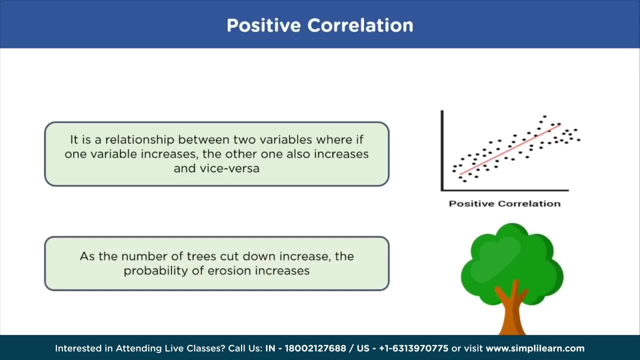 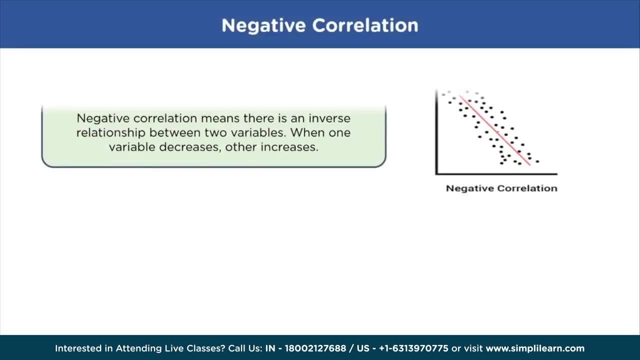 The number of trees cut down and the probability of erosion are in correlation. When one increases, other also increases, and vice versa. Negative correlation- A negative correlation is just the opposite. The relationship line has a negative slope and the variables change in opposite directions. 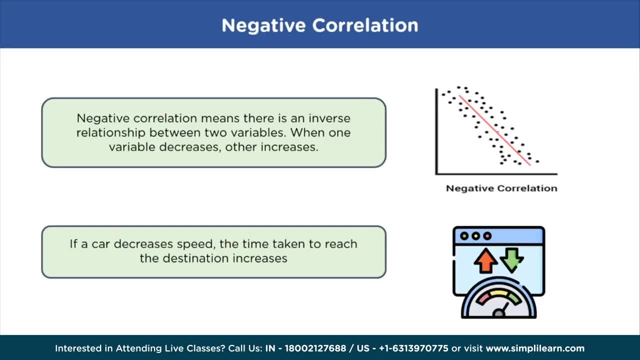 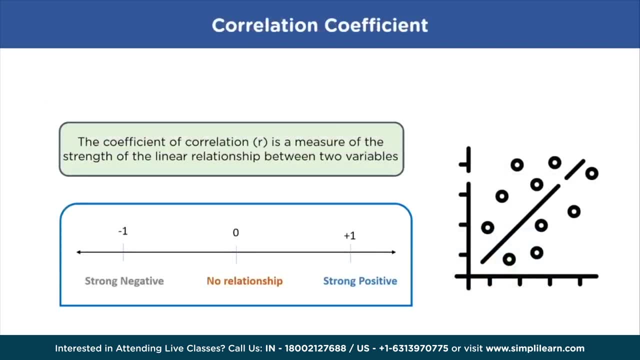 For example, if you decrease the speed of the car, the time taken to reach the destination increases. This is a negative correlation Correlation coefficient. The correlation coefficient, which is denoted by r, gives us a measure of the strength of the linear relationship between the two variables. 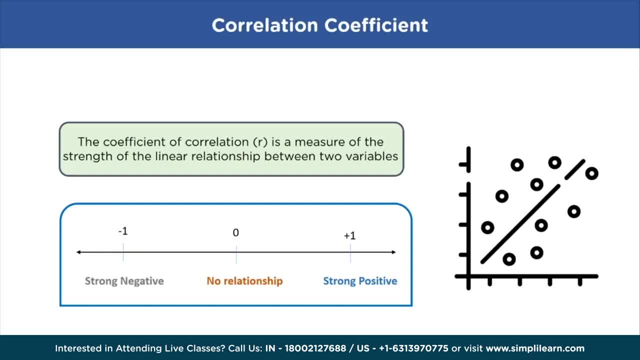 The value is denoted by the letter r and it ranges from minus one to plus one. If it is less than zero, it implies that there is a negative correlation. The minus one indicates there is a strong negative correlation between the variables. If r is greater than zero, it implies there is a positive correlation and plus one is. 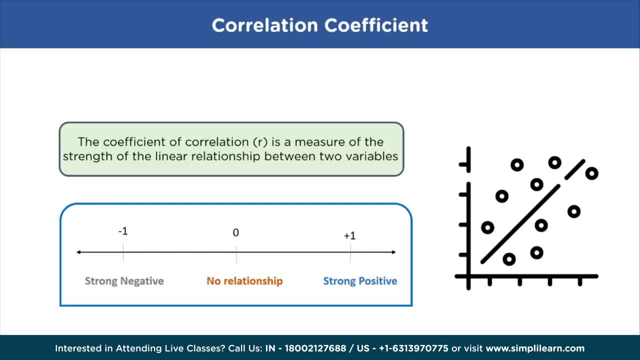 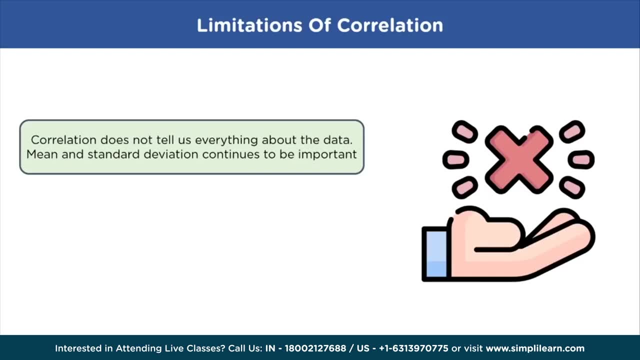 the strongest point of a positive correlation. When r is equal to zero, we can say that there is no correlation between the variables. There are also some limitations of correlation. The first one is: correlation does not give you every insight on the data. 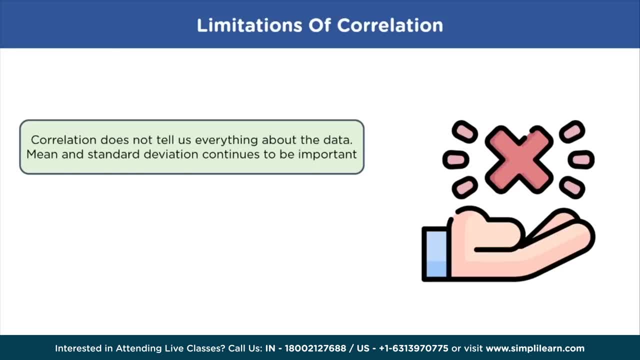 Mean and standard deviation are still the important parameters to get the insight of a data. The second one is the data will not produce a straight line every time and it will be difficult to predict the value of r just with the straight line or the slope of the graph. 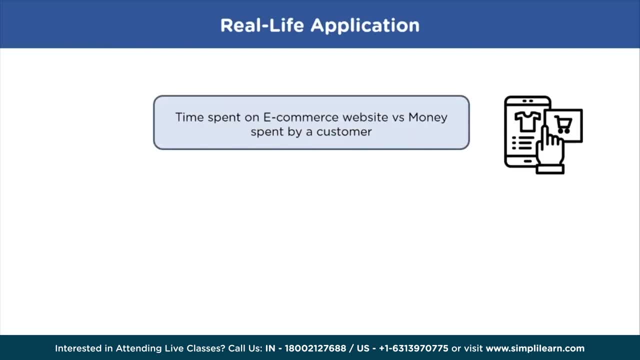 Now let's look at the next one. The second one is the data will not produce a straight line every time, and it will be difficult to predict the value of r just with the straight line or the slope of the graph. Now let's see some real-life applications of correlation. 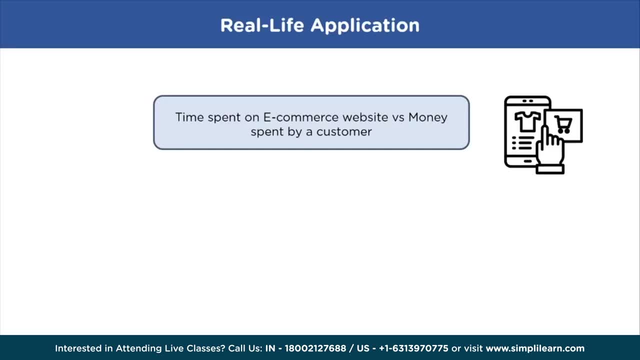 If you take any e-commerce company whose website is accessed by millions of users all over the world, the company can look at all the data and they can measure how much time was spent by the customer and the respective money spent by the customer. We can also predict the unique users that visited the website and how it affected the 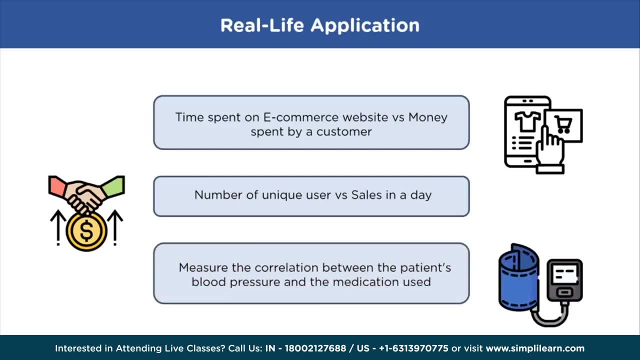 sales in a day. The third application can be the patient blood pressure and the medication used, the level of patient blood pressure and the efficiency. The third application can be the patient blood pressure and the medication used. the level of patient blood pressure and the effecct of medication on it can be in correlation. 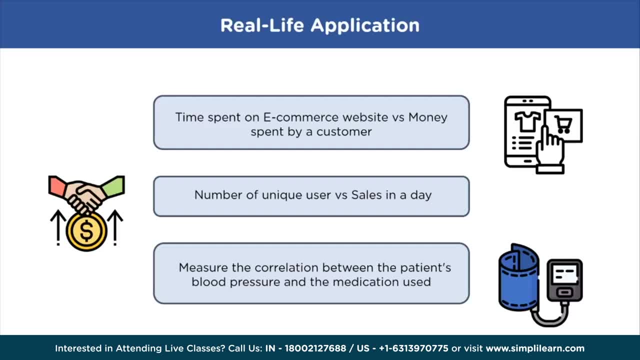 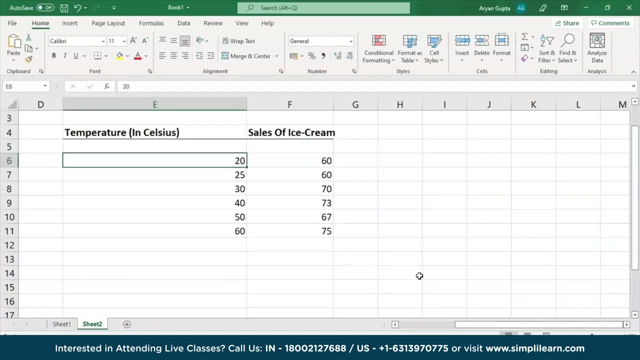 Now let's jump on to excel workbook to calculate how we can calculate correlation. Here we are on excel workbook. You can see we have the temperature, den antiquity, Celsius at 20,, 25,, 30,, 40,, 50 and 60, and the 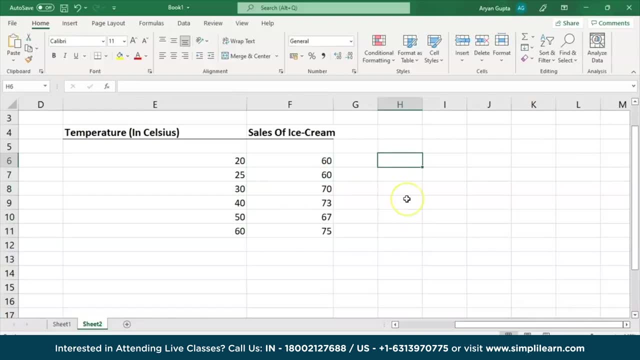 corresponding sales of ice cream in the units. To calculate the correlation we will use the co relevant function i, student function, ψ- speeds, Since the ice cream- isaney ice cream- can carry the full measure according to the rate at a number of grades. 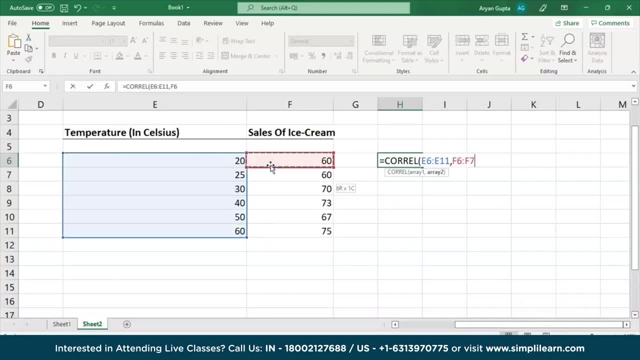 ber 70. Celsius, and the array 2 will be our sales of ice cream. So you can see there's a very strong correlation between the temperature of a day and the sales of ice cream unit. If the temperature increases, the sales of ice cream unit. 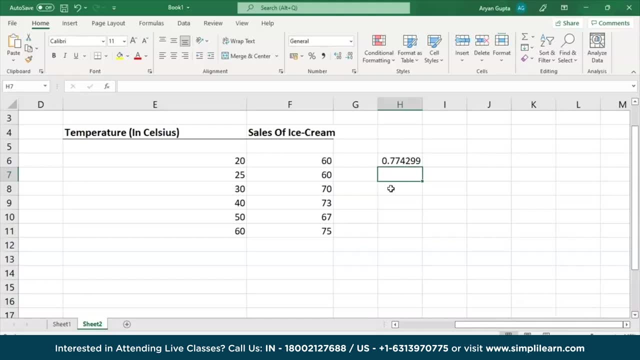 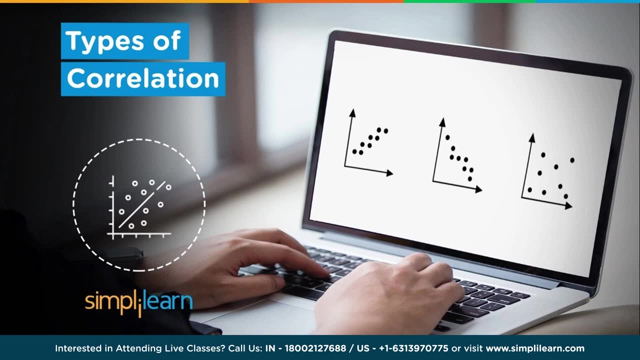 increases and if the temperature decreases, the sales of ice cream unit decreases. In this session we will continue the discussion and look into different types of correlation. So let's discuss the agenda for today's session. We'll start the tutorial by understanding what is correlation, then? 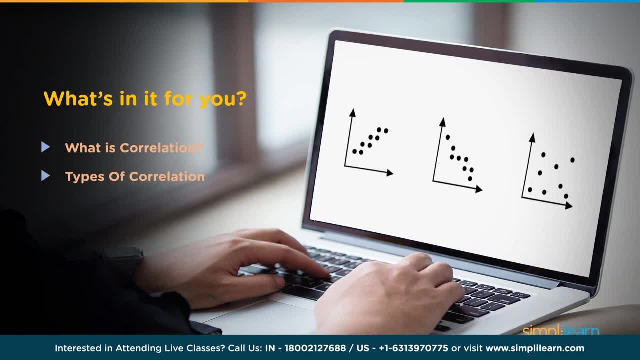 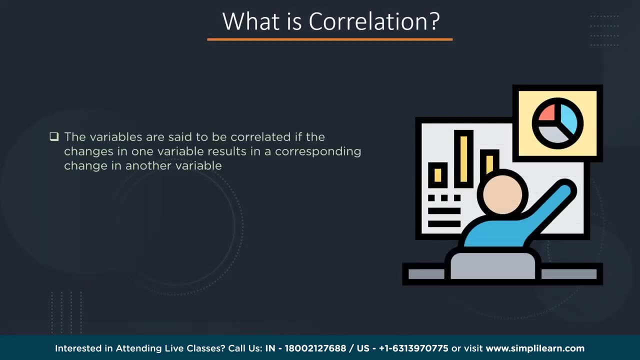 we'll move to discuss types of correlation and discuss each of them one by one. After that, we'll learn the two major methods to calculate correlation coefficient, ie Spions-1 correlation as Spions-1 Rank correlation. So let's get started. what is correlation? Correlation refers to the statistical relationship. 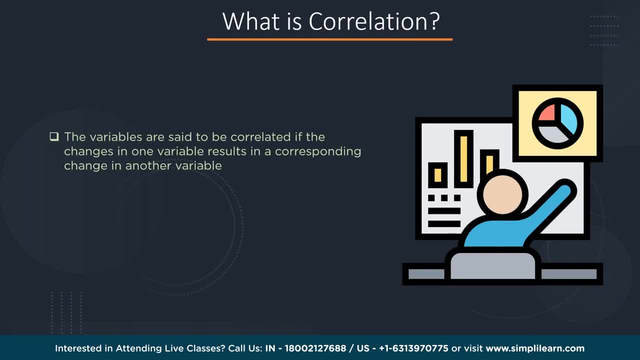 between the two entities. It measures the x-axis in a y-axis in order to estimate correlation coefficient extent to which two variables are linearly related. For example, the increase in the height of the children is accompanied often by the increase in weight. The value of the 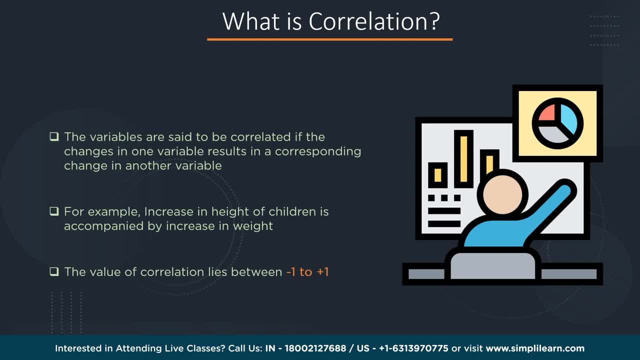 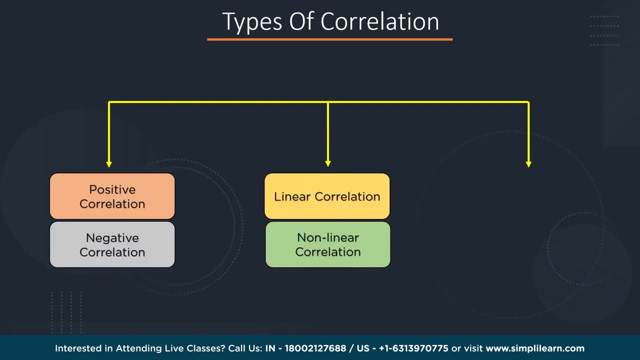 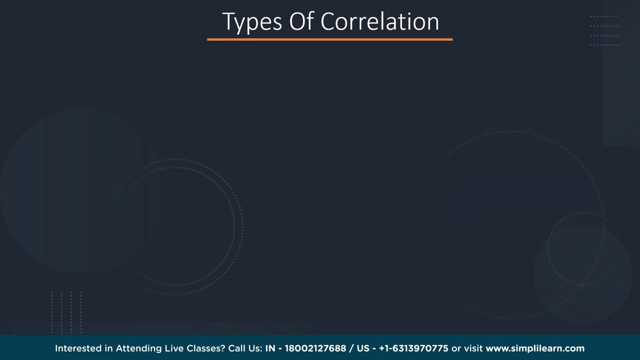 correlation always lies between minus one to plus one. There are mainly three categories of correlation. The first one is positive correlation and negative correlation. The second one is linear and nonlinear correlation, And the third one is simple, multiple and partial correlation. Let's discuss each of them one by one. 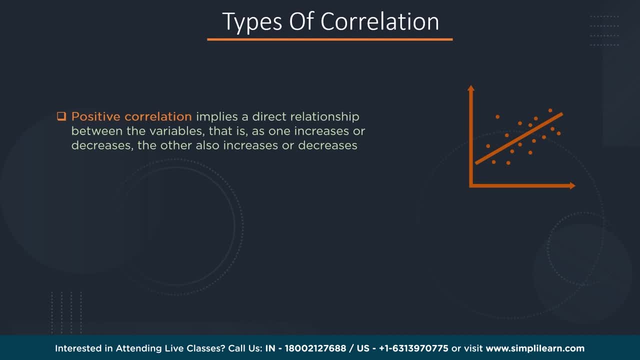 Positive correlation. A positive correlation means that a linear relationship is positive and the two variables increases or decreases in the same direction, as you can see from the graph, For example, the calories you burn is directly proportional to the amount of time you run on a treadmill. On the other hand, a negative correlation- 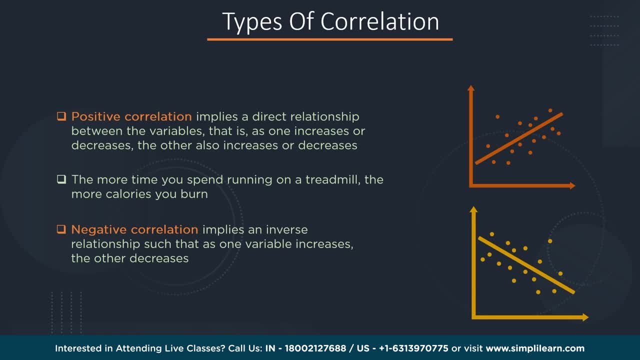 is just the opposite. The relationship line has a negative slope and the variable changes in the opposite direction. That is, one variable decreases while the other increases. An example can be a student who has many absences has a decrease in grades. Now let's move. 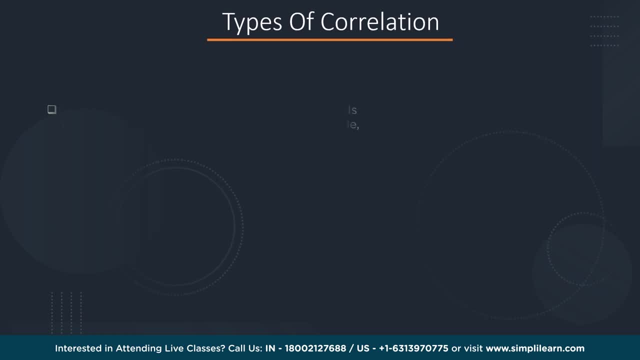 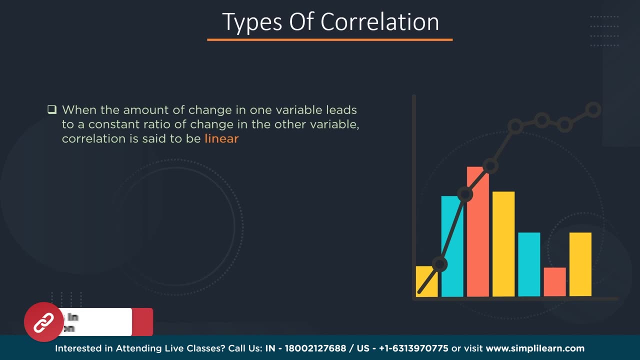 on to discuss linear and nonlinear correlation. When we change the value of a variable which leads to a constant ratio change in other variables, then that relation is said to be linear, For example, the fact that the value of the variable actually doubles its output by doubling the number of workers. On the other hand, 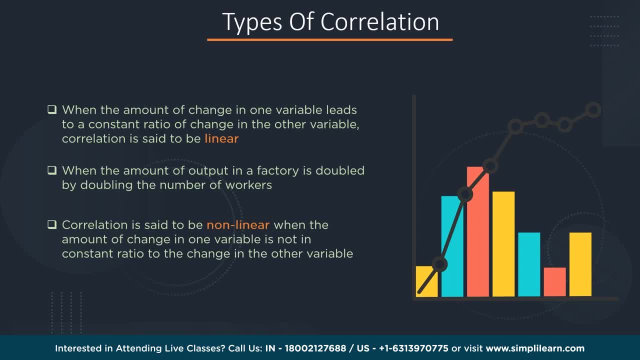 correlation is said to be nonlinear when the amount of change in one variable is not in constant ratio to the change in the other variable. For example, the change in radius of the sphere and the change in volume of the same sphere does not happen to be in the 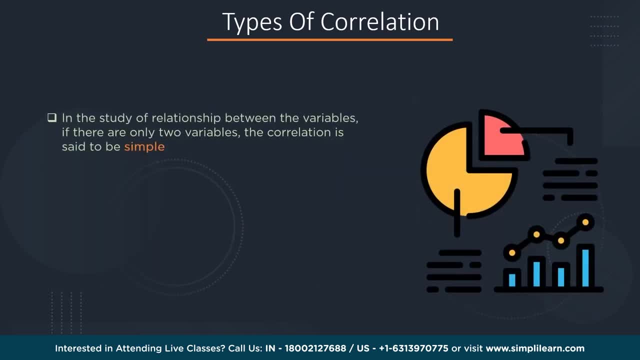 same ratio. Now let's discuss simple multiple and partial correlation When studying the relationship between the variables. when only two variables are involved, the correlation is said to be simple. In the multiple correlation, we measure the degree of association between one variable on the one side and all the variables together on the other side. And for the partial correlation, 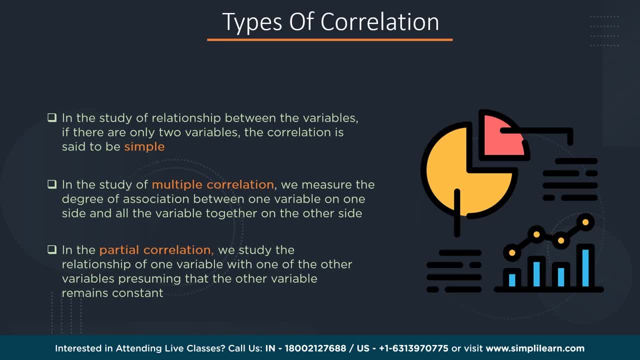 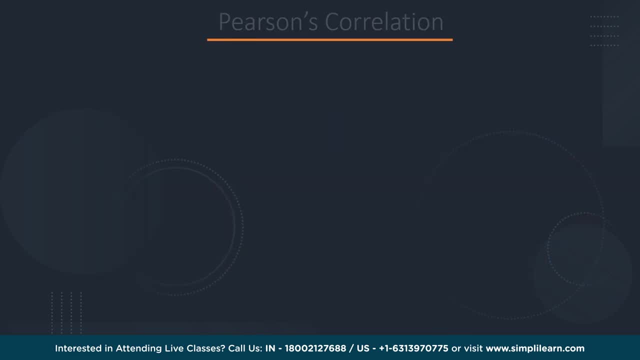 we study the relationship of one variable with one of the other variables, presuming that all the variables remains constant. Now that we know all the types of correlation, let's discuss the two major types to calculate the correlation coefficient. The first one is Pearson's correlation. 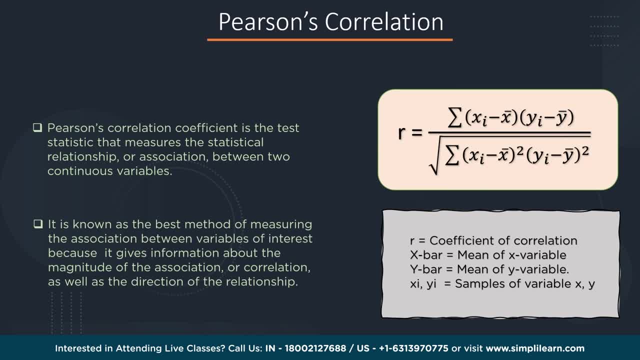 Pearson's correlation coefficient is the correlation coefficient of the two variables that are related. The correlation coefficient is the test statistic that measures the statistical relationship between the two continuous variables. The Pearson's correlation coefficient is often denoted by R and the formula to calculate the Pearson's correlation coefficient is: 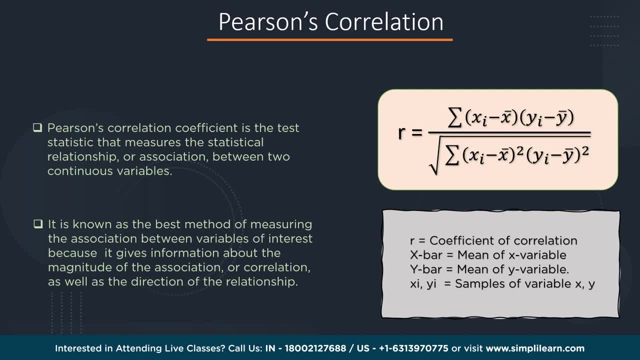 sigma x, i minus x bar into i minus y bar. divided by under root, sigma x, i minus x bar whole square and y- i minus y bar whole square. Where R is the coefficient of correlation, x, y is the mean of x variable and y bar is the mean of y variable, And x, i and y y denotes. 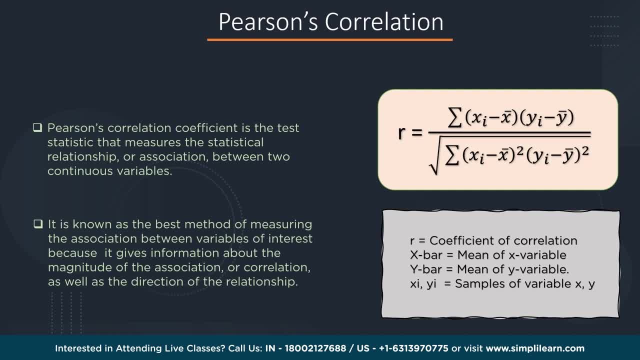 the samples of variable x and y respectively. The Pearson's correlation coefficient is the best method to measure the association between two variables of interest, because it gives information about the magnitude of the association or correlationship, as well as the direction of the relationship between the two variables. 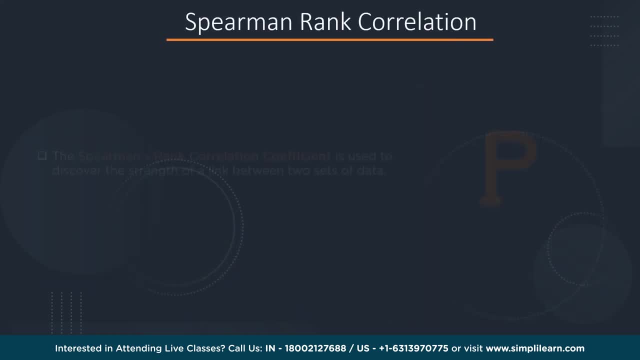 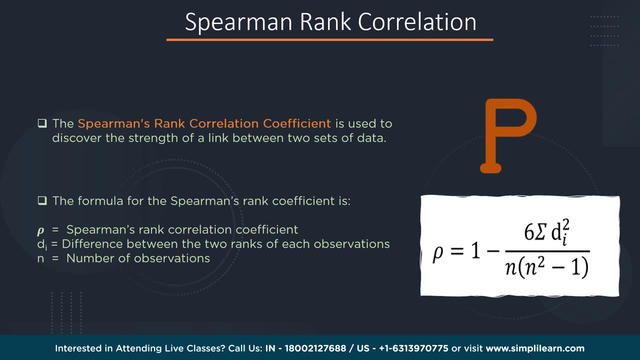 The second best method is the PSN rank correlation. This PSN rank correlation is used to discover the strength of a link between the two sets of data. The formula to calculate this PSN rank correlation coefficient is: rho is equal to 1 minus sigma. 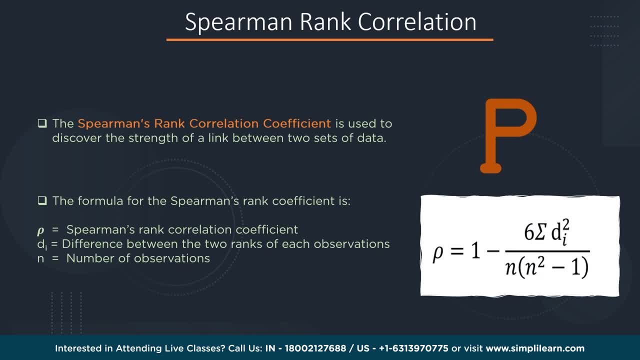 d i whole square divided by n bracket, n square minus 1.. Where, rho, is this PSN rank? correlation coefficient. d? i is the difference between the two ranks of each observation and n is the number of observations. In our previous two sessions we discussed what is correlation, correlation coefficient. 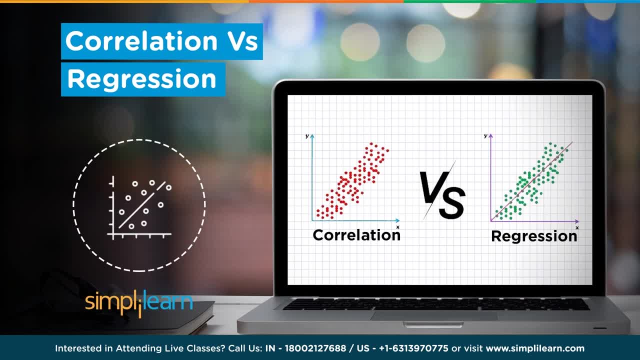 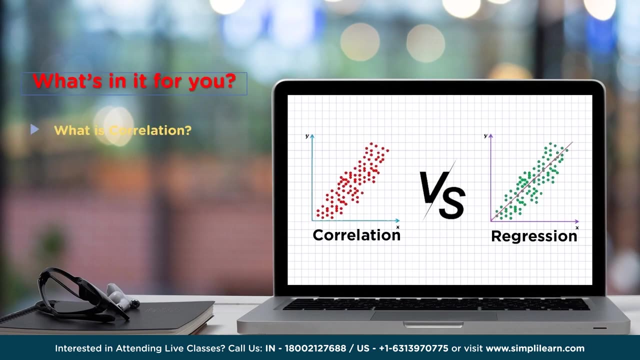 and types of correlation. In this session, we will continue the discussion and try to understand the difference between correlation and correlation And discuss it with the help of an example. So let's discuss the agenda for today's session. We will start this tutorial by discussing what is correlation. 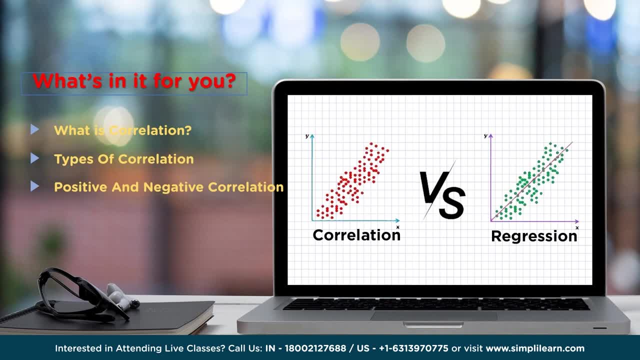 Then we will move on to understand types of correlation, and we will discuss one major type, that is, positive and negative correlation. After that we will move on to what is regression, lines of regression, and then we will discuss a simple regression model with its equation. 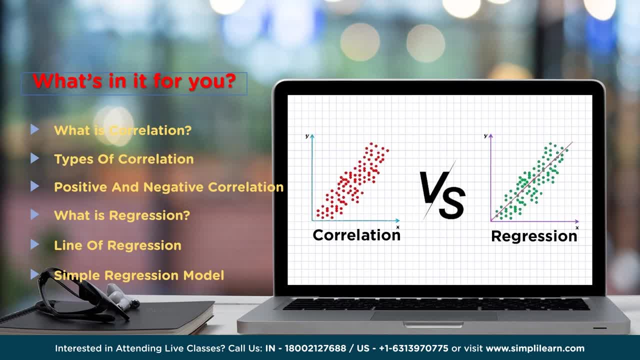 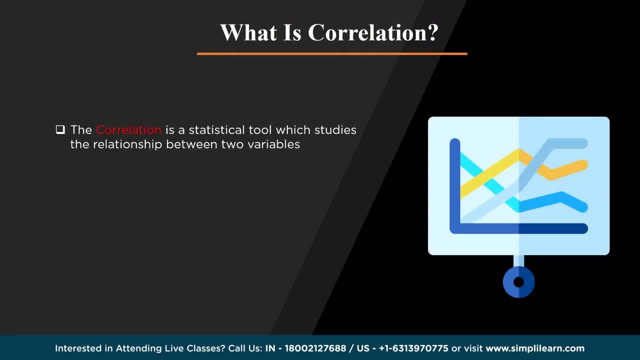 Finally, we will move on to excel, to discuss how we can calculate the regression using an example. So let's begin. What is correlation? A correlation is a statistical relationship between two entities. It measures the extent to which the two variables are linearly related. In simple words, it is the measurement of 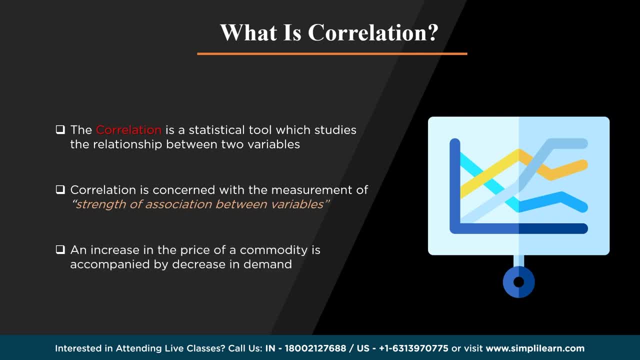 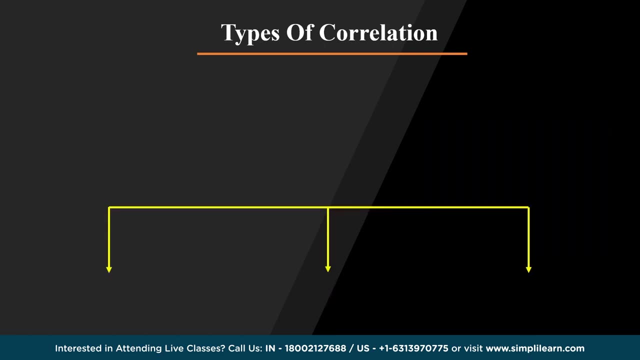 strength of association between the two variables. For example, an increase in the price of commodity is always accompanied by decrease in demand. The value of the correlation always lies between minus 1 to plus 1.. Types of correlation. So there are mainly three categories of correlation. 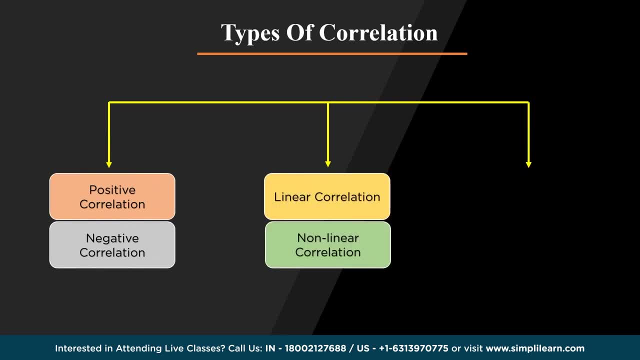 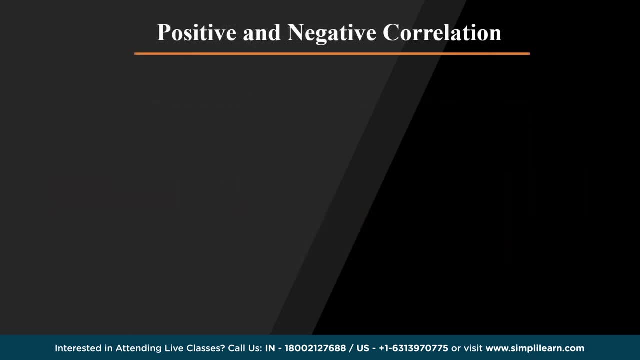 The first one is the positive and negative correlation, The second one is linear correlation and nonlinear correlation. And the third one is simple, multiple and partial correlation. The third one is simple, multiple and partial correlation. Lets discuss positive and negative correlations. A positive correlation means that a linear relationship is positive and the two variables 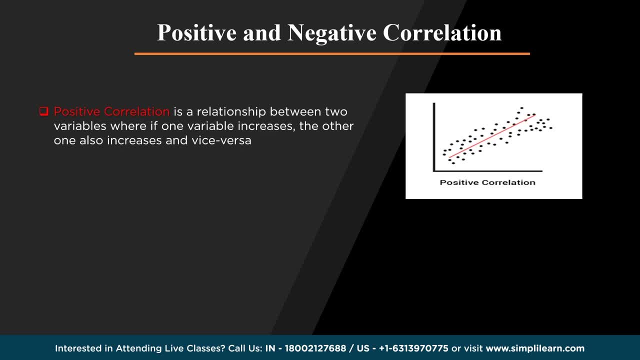 increase or decrease in the same direction, as you can see from the graph. An example can be: As the number of trees- scriormal dow- increases, the probability of soil erosion also increases. It means that the tip of the tree not only gets rest in the nut. should stayborgsthe value of 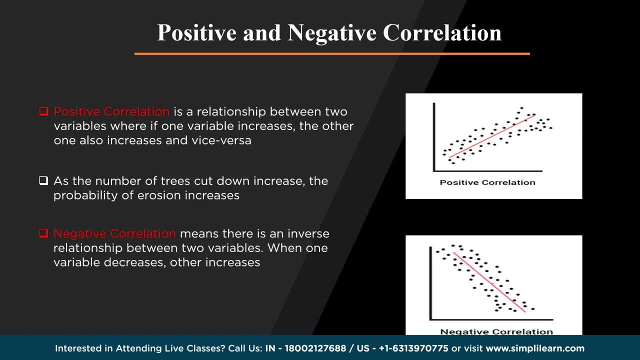 one row, but that two mandibles are not. Let's see now In the same manner. a negative correlation is just the opposite. The relationship line has a negative slope, as you can see from the graph, And the variables changes in the opposite direction. 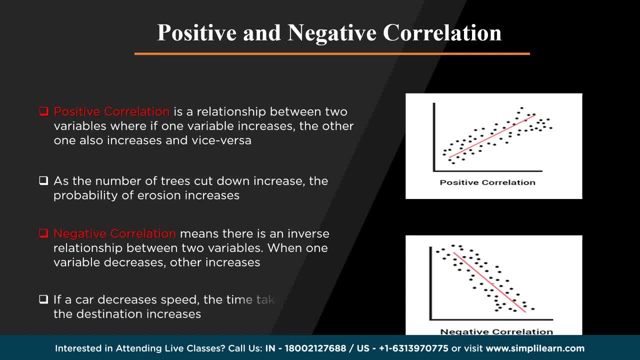 That is, one variable decreases while the other increases. To understand this, an example can be: if a car decreases the speed, the time taken to reach the destination increases. To know more about the types of correlation, you can refer to our previous videos and you. 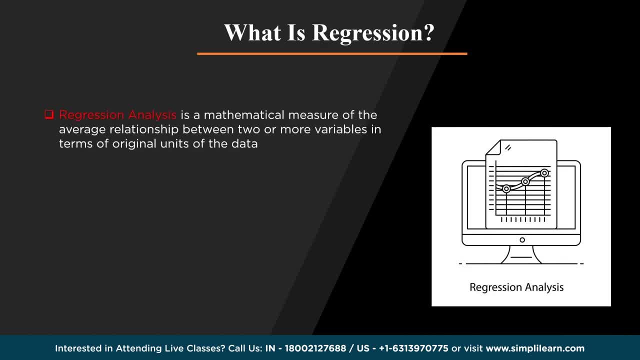 can find the link in our description. Now, what is regression? Regression analysis, like most multivariate statistics, allows you to infer that there is a relationship between two or more variables. These relationships are seldom exact because there is a variation caused by many variables. 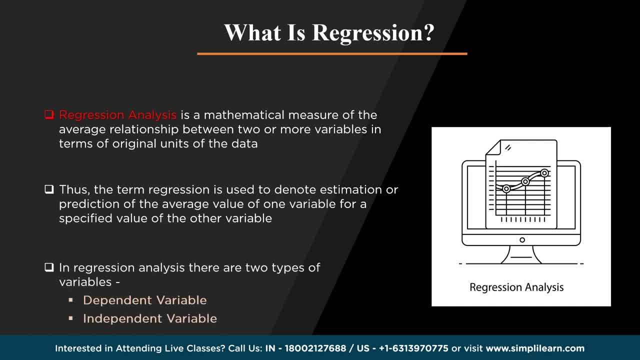 not just the variables being studied In regression analysis. there are two types of variables. One is dependent variable and other is independent variable. Let's discuss what the both variable represents. A dependent variable is a variable whose value is influenced or to be predicted. 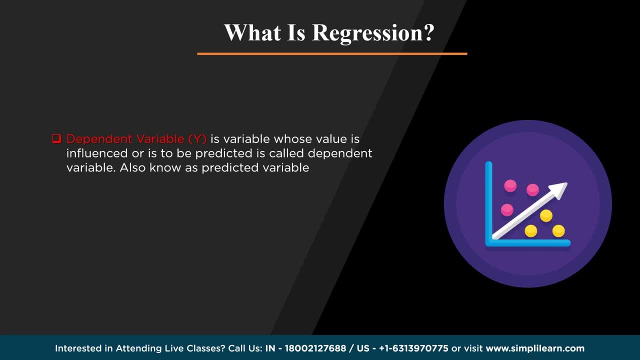 The dependent variable is often denoted by y and is also known as a predicted variable, Whereas independent variable, which is denoted by x, is a variable which influences the value or is used for prediction. The independent variable is also known as a predictive variable. 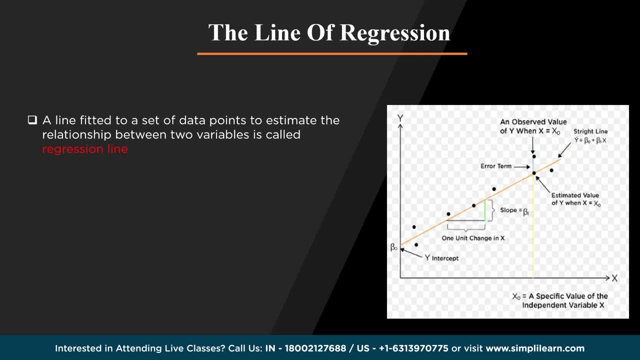 The line of regression. The regression line is a line which is used to describe the behavior of a set of data. In other words, it gives the best trend of the given data. Regression lines are useful in forecasting procedures. Its purpose is to describe the regression. 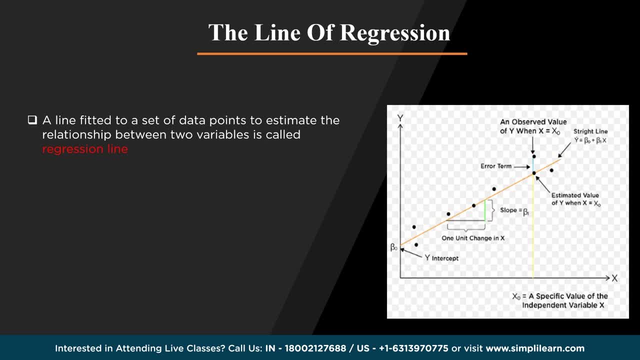 It is the best way to understand the relationship between different variable and independent variables. The regression equation of y and x describes the change in the value of y for given changes in the value of x and vice versa. In the regression line equation, x and y are the variables of interest in our data, with. 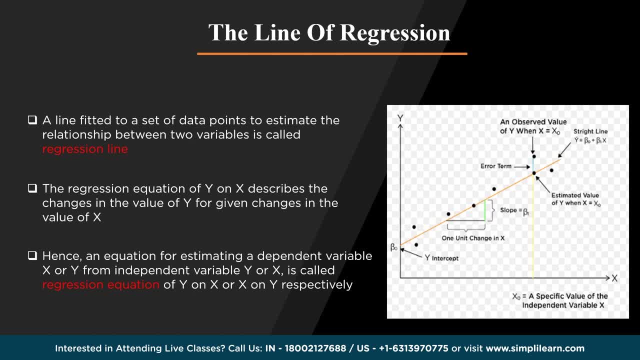 y, the unknown or dependent variable, and x, the known or independent variable. Let's discuss the two key terms in this graph. The first one is slope. Slope is the ratio of the vertical and horizontal distance between two variables. Slope is the ratio of the vertical and horizontal distance between the two variables. 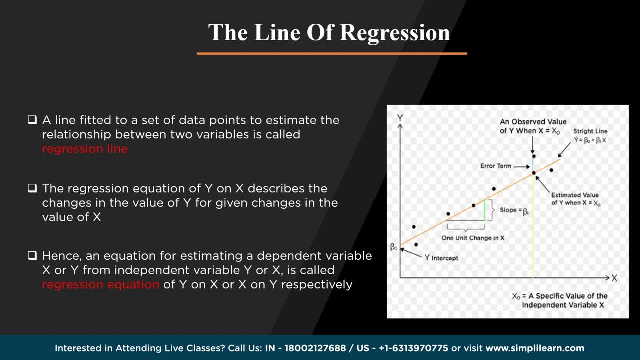 The second one is the direction of a energy flow. Slope is the direction of the energy flow between the two points on a line and you can see y-intercept, which is the coordinate of the point at which the curve intersects an axis. There are some. 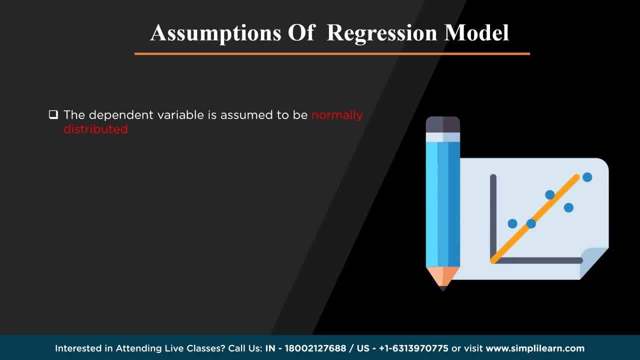 assumptions we take to create the regression model. The first one is the dependent variable is assumed to be normally distributed. The values of the dependent variable are statistically independent. This means that when we select the sample of a particular X, it does not depend on any other value of Y. 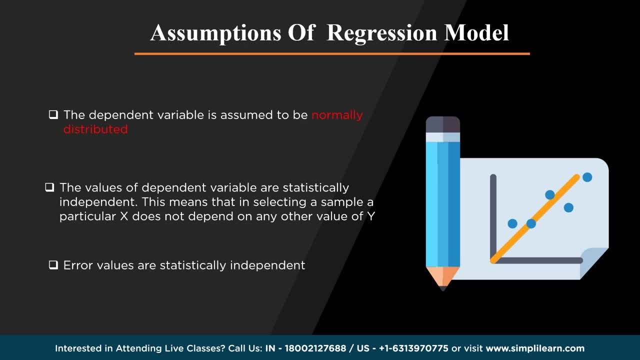 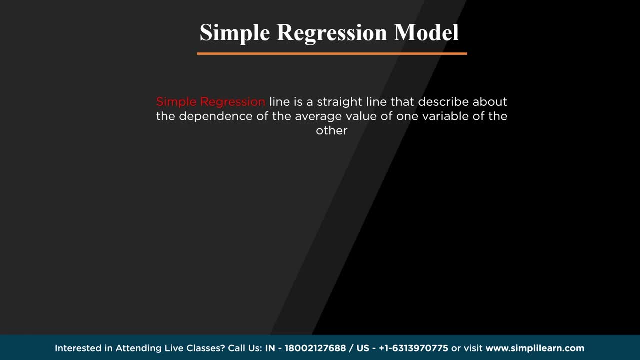 And the third one is error values are statistically independent. Now let's discuss a simple regression model. A simple regression model is used to depict a relationship between variables which are proportional to each other, Meaning the dependent variable increases, decreases with the independent variable. The equation of a simple regression model is: y is equal to b0 plus b1x plus. 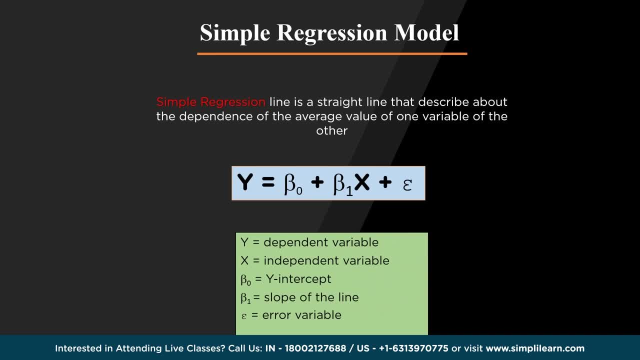 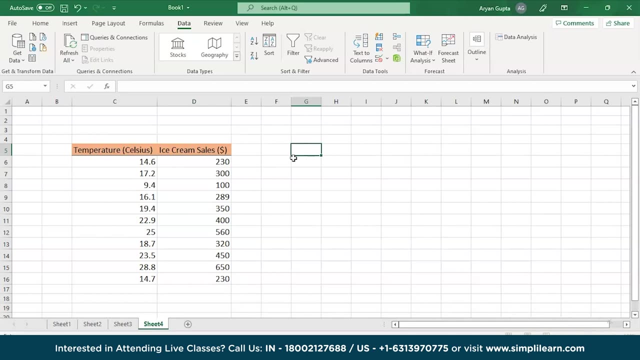 e, Where y is dependent variable, x is independent variable. b0 and b1 represents y-intercept and the slope of the line respectively, and e is the error variable. Now let's move on to Excel To calculate the regression coefficient of a given data. we are on our excel. 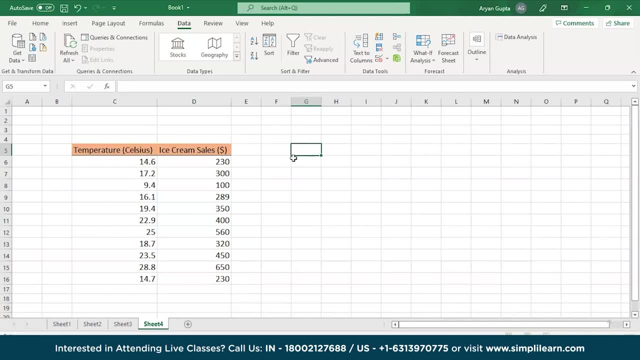 workbook In front of us. we have the data of temperature of the day and sales of the ice cream on that day. Let's try to understand this regression, analysis and summary output using this data. The first step is to go to the data tab and 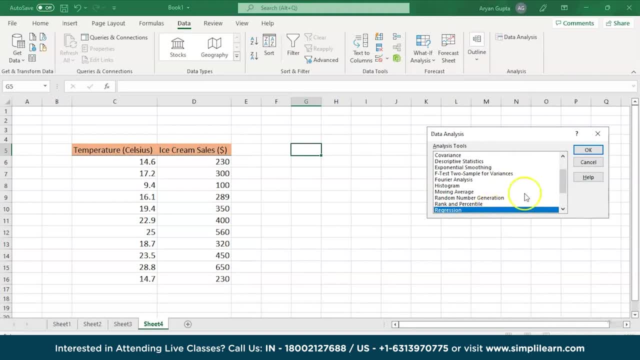 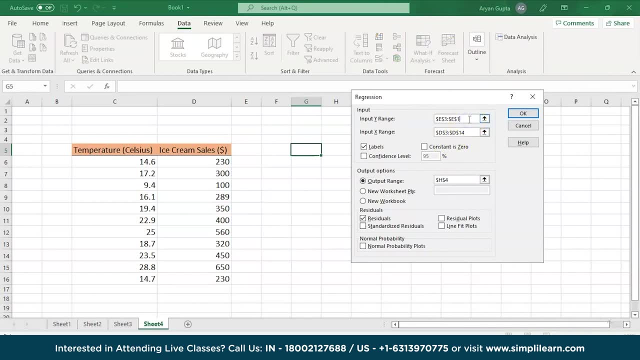 select data analysis, Then select regression and click OK. We'll get this table. Select the y-range, then select data analysis and select y-intercept to show the y-intercept range as the ice cream sales. This y range is predictable variable, also called as dependent. 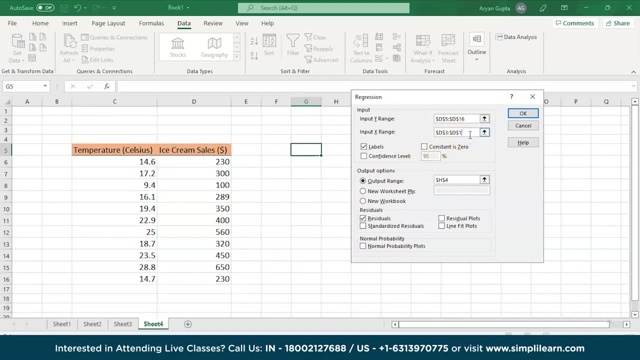 variable For the input x range, we will select the temperature in degree Celsius. This is the explanatory variable, also called as the independent variable. One thing you should keep in mind is that both the x and y column must be adjacent to each other. We have the 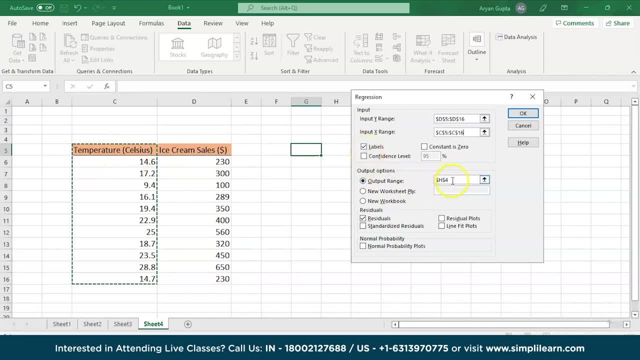 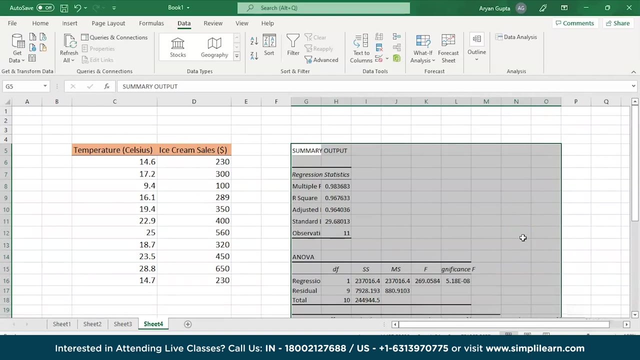 labels. so we will check the label and we will select the output range from G5.. Check the residuals and click OK. Excel produces the following output. Let's analyze some key data. We got the R-square value to be 0.9676, which is very good. This shows that the 96% 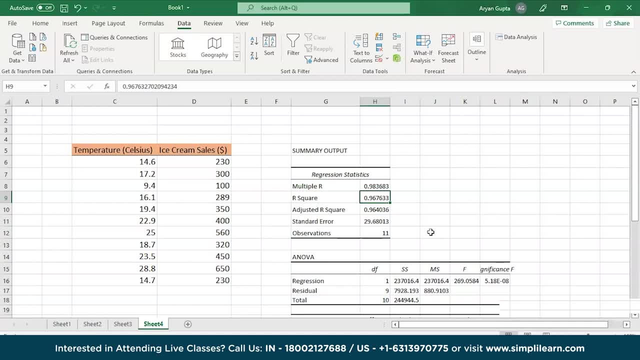 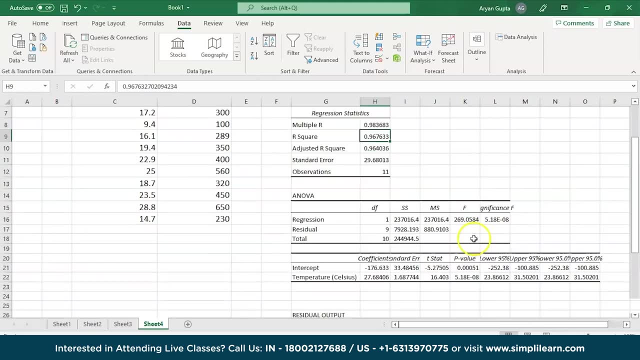 of the variation in ice cream sales is explained by the temperature of the day. Closer to the one, the better the regression line fits the data. Now let's move little more and analyze this coefficient. If you look at the coefficient, you will get the equation of the regression. 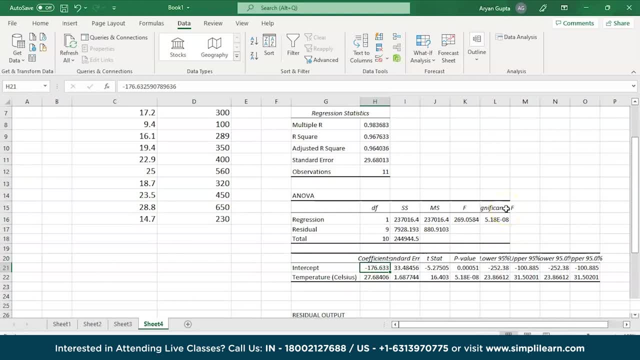 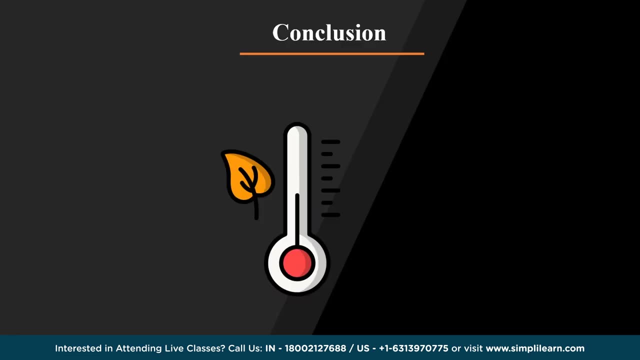 line. In this case it is minus 176.33, plus 27.68 into temperature of the day. Substituting the temperature of the day for any given day, we can find the sales of the ice cream. With the above discussion we can conclude that there is a big difference between the correlation. 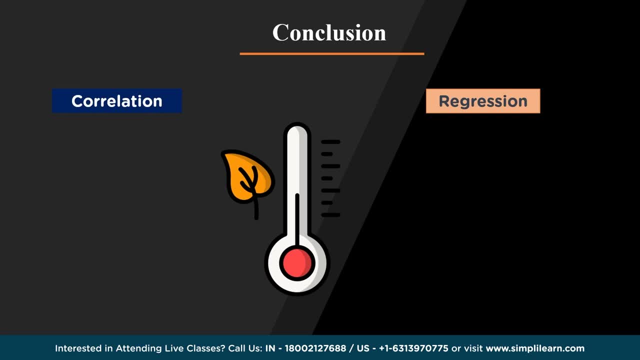 and regression, although these are studied together. Correlation is used to study whether the variables under study are correlated, Whereas regression is used to establish a functional relationship between the two variables. The equation of the regression line is of form: y is equal to fx plus c Correlation. 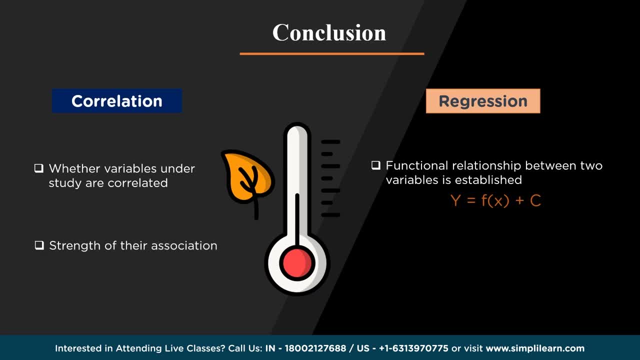 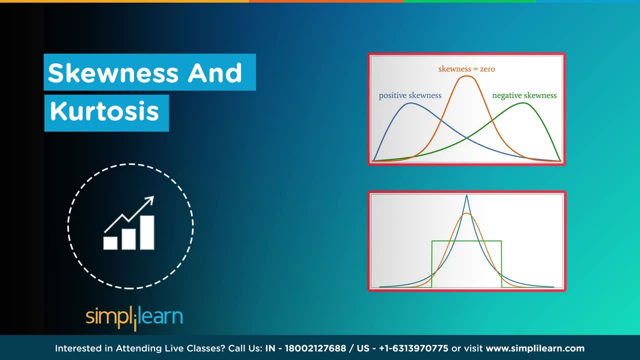 is used to establish the strength of the association between the two variables that are being studied, Whereas regression is used to make the future predictions on the any given event. As you know, in today's world, data is becoming increasingly important- Entire professions. 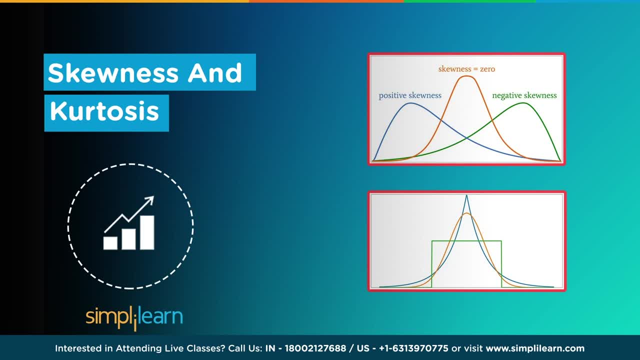 are dedicated to studying, understanding and evaluation of data. As you know, in this form, understanding and manipulating the data. Hence it is important to know about the different types of data and their associated properties. So in this session, we will discuss how to 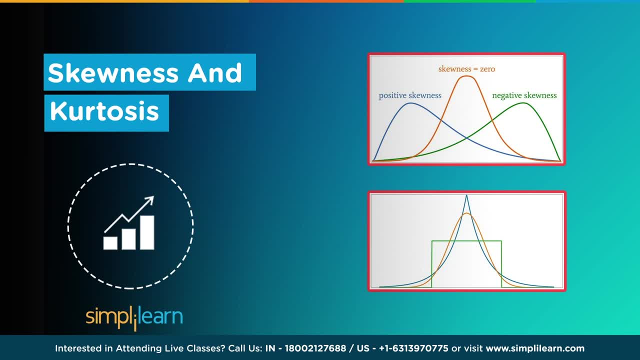 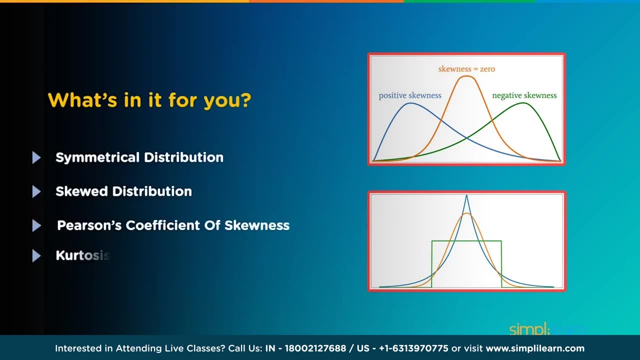 calculate the distortion in the normal curve using skewness and kurtosis. So let's get started. We will start this tutorial by understanding symmetrical distribution. Then we will move on to discuss skewed distribution and Pearson's coefficient of skewness. Finally, we will discuss kurtosis. So let's get started. 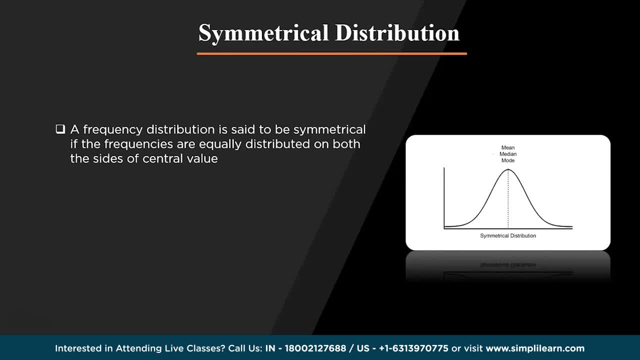 Symmetrical Distribution. A distribution is said to be a symmetrical distribution when it is equally distributed on both the sides of the mean value. The distribution shape can either be a bell-shaped or U-shaped. In symmetrical distribution, the values of mean, median and mode are all equal, as you can see in the graph. 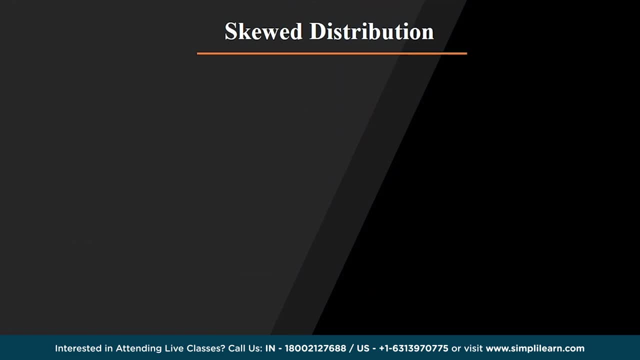 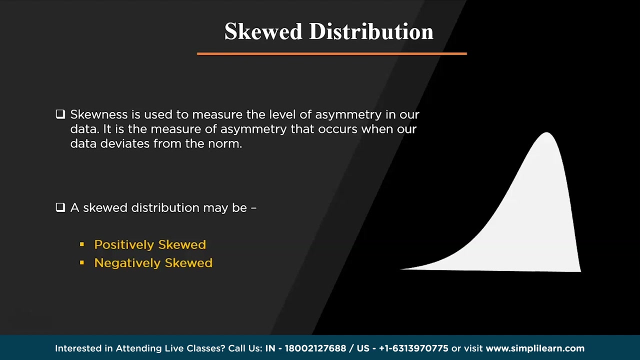 Skewed Distribution. Skewness is used to measure the level of asymmetry in our graph. It is the measure of asymmetry that occurs when our data deviates from the norm. Sometimes, the normal distribution tends to be tilted more on one side. This is because the probability of data being more 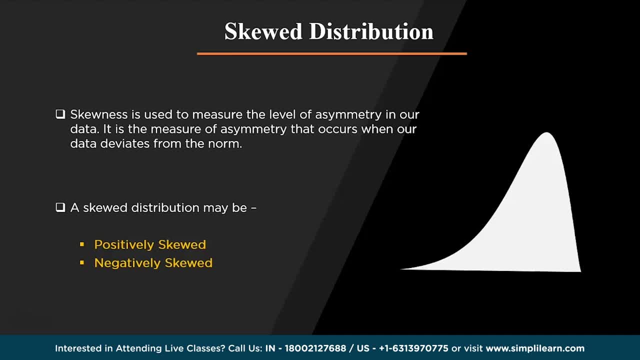 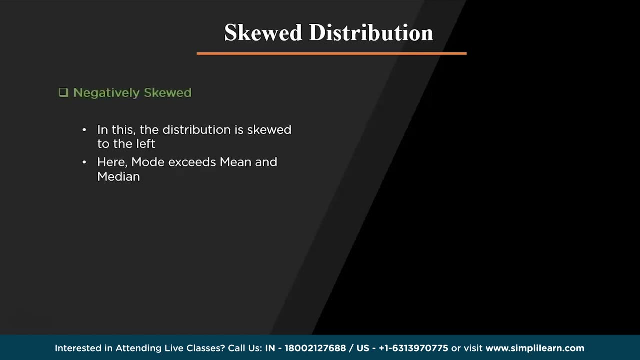 or less than the mean is higher and hence makes the distribution asymmetrical. This also means that the data is not equally distributed. The skewness can be of two types: Positively skewed and negatively skewed. Let's discuss them separately. Negatively Skewed: In a negatively skewed distribution, the data 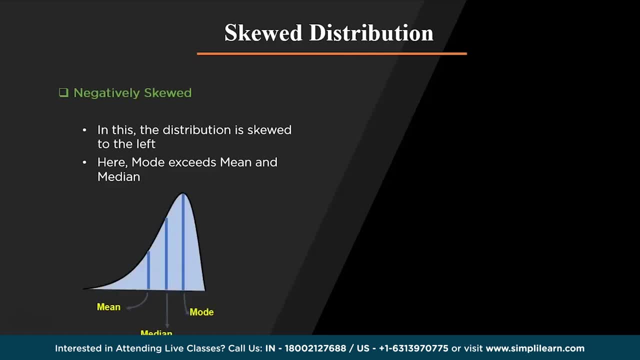 points are more concentrated towards the right hand side of the distribution. As you can see in the graph, this makes the mean, median and mode bend towards the right Hence these values are always negative. In this distribution, mode is greater than median and median is. 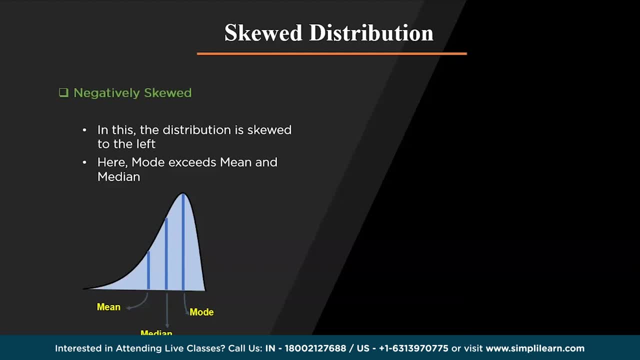 greater than mean. Positively Skewed Distribution. Positively Skewed Distribution. Positively Skewed Distribution. In a distribution that is positively skewed, the values are more concentrated towards the right side and the left tail is spread out, as you can see in the graph. 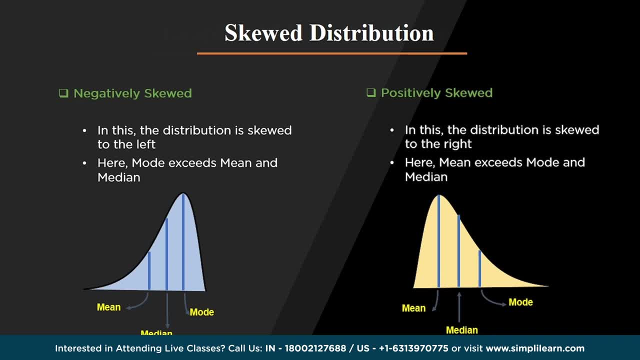 Hence the statistical results are bent towards the left hand side. Therefore, the mean, median and mode are always positive. In this distribution, mean is greater than median and median is greater than mode. The measure of skewness always helps us to know to what degree and in which direction. 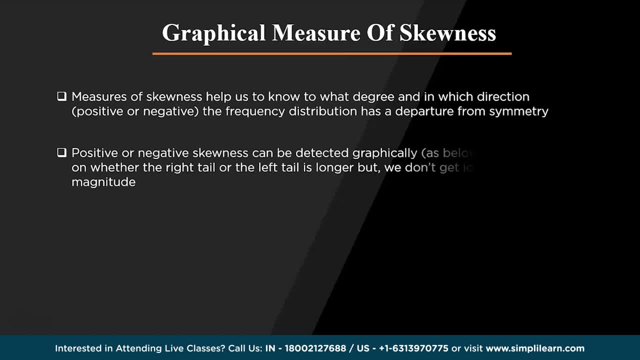 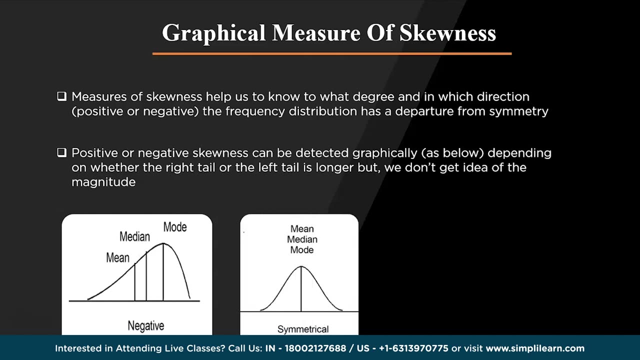 positive or negative. the frequency distribution has a departure from symmetry. Positive or negative skewness can be detected graphically, depending on whether the right tail or the left tail is longer, but we don't get the idea of the magnitude. In a negatively skewed symmetry, the values are always negative. 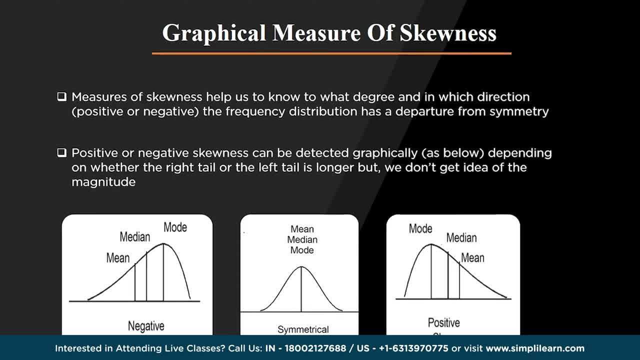 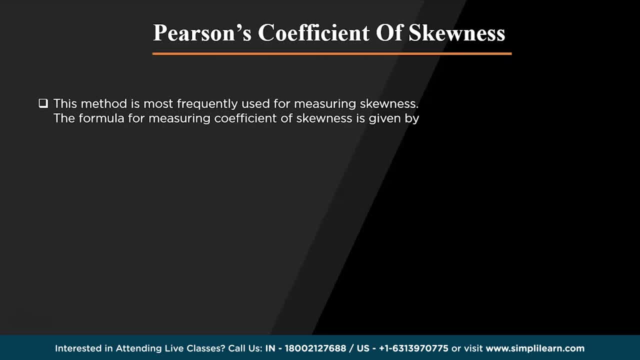 This is the symmetrical distribution and in a positively skewed the values are always positive. Now let's discuss PSU's coefficient of skewness. The median is always the middle value And the mean and the mode are the extremes. So we can derive the formula to capture the horizontal distance between the mean and the. 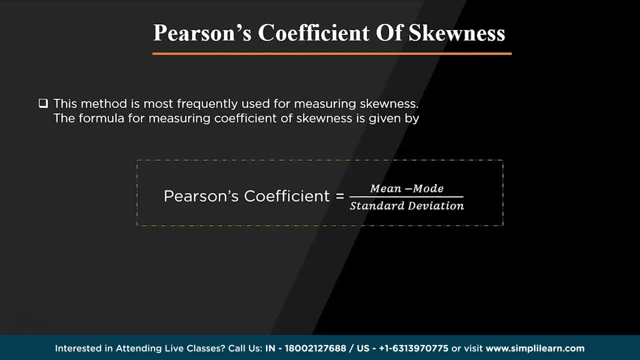 mode using the PSU's first coefficient. So the formula to calculate the PSU's coefficient is mean minus mode divided by the standard deviation. The division by the standard deviation will help you to scale down the difference between the mode and the mean. This will scale down their values in the range of minus 3 to plus 3.. 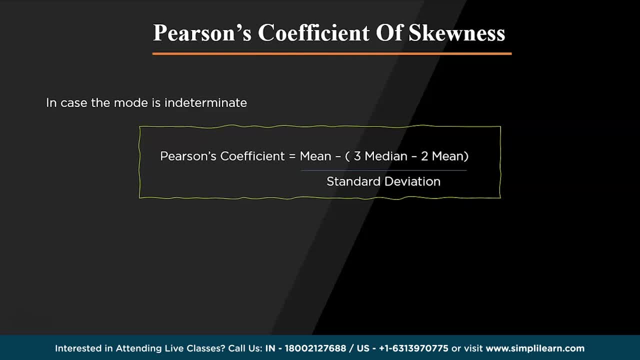 In case where the mode is indeterminate, we can calculate the PSU's coefficient by mean minus 3, median minus 2. mean divided by the standard deviation. If the value of coefficient is between minus 0.5 and 0.5, the distribution of the value 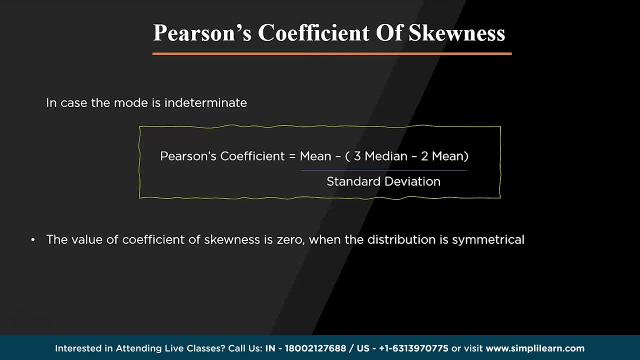 is always symmetrical. If the value of coefficient is 0,, then the distribution is symmetrical. If the value of coefficient is positive, then the distribution is positively skewed, And if the coefficient is negative, then the distribution will be negatively skewed. 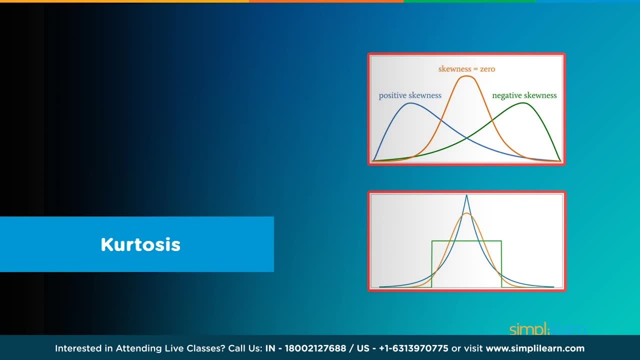 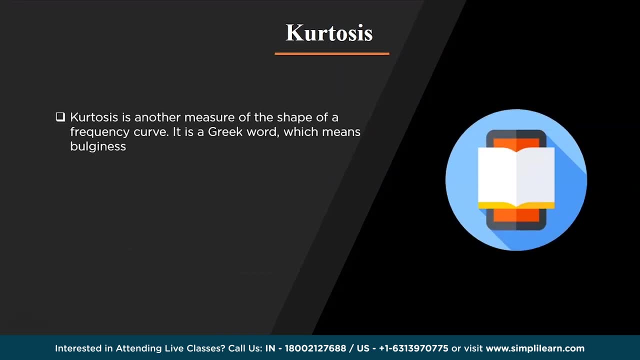 Now that we have discussed the symmetrical and skewed distribution, Let's move on to understand what is kurtosis? Kurtosis is used to find the presence of outliers in our data. It gives us the total degree of outliers present. The data can be heavily tailed and the peak can be flatter, almost like punching a distribution. 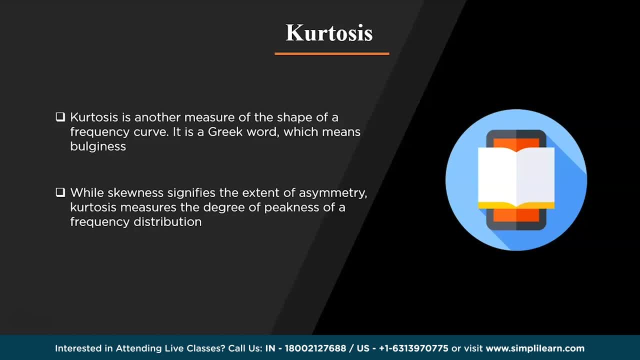 or squishing it. While skewness signifies the extent of the symmetry, kurtosis measures the degree of peakness of a frequency distribution. When the peak of the curve becomes relative to the peak of the curve, then the peak of the curve becomes relative to the peak of the curve. 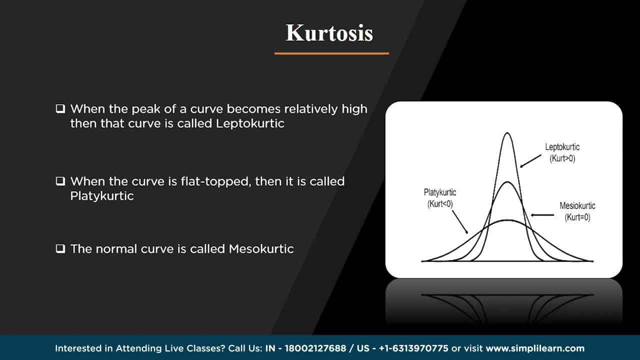 When the peak of the curve becomes relatively high, then the curve is called leptokurtic, And when the curve is flat, it is called platykurtic. When the curve is similar to the normal curve, it is called mesokurtic. 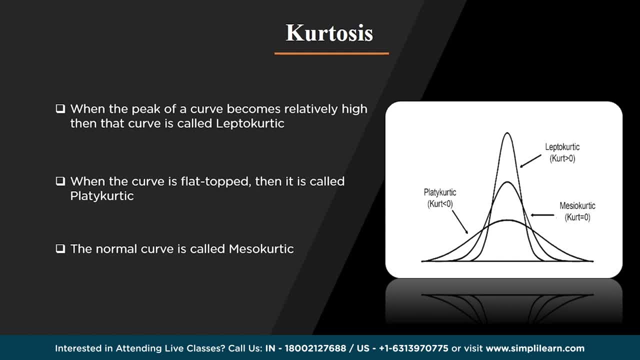 The expected value of kurtosis is 3.. This is observed in a symmetrical distribution. A kurtosis greater than 3 will indicate positive kurtosis. Further, a kurtosis less than 3 will mean a negative kurtosis. 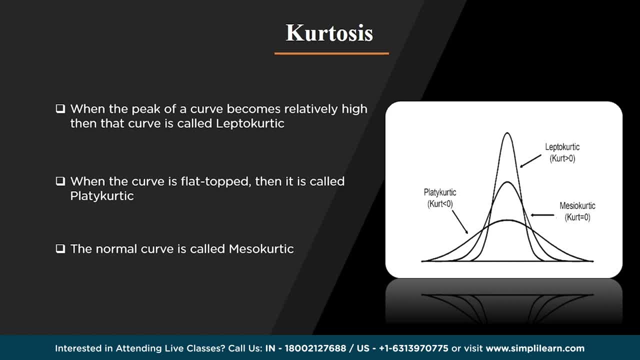 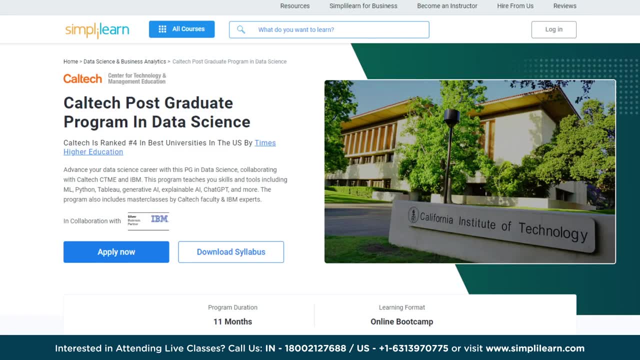 The range of value for a negative kurtosis is from minus 2 to 1.. The greater the value of kurtosis, the higher is the peak, as you can see from the graph. Simply Learn's postgraduate program in data science offered by Caltech University in collaboration. 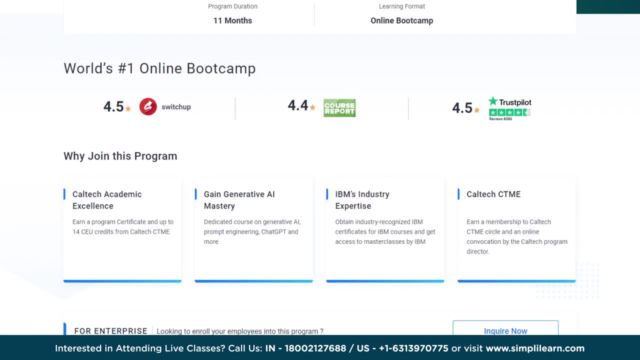 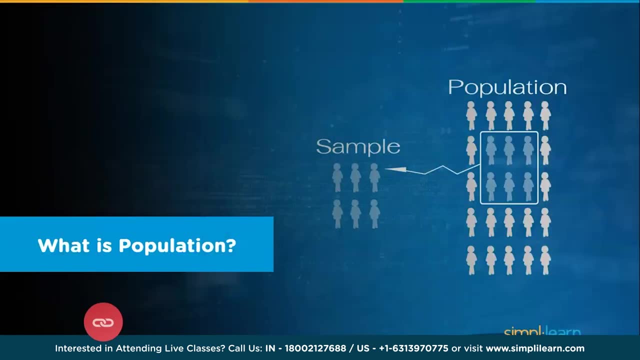 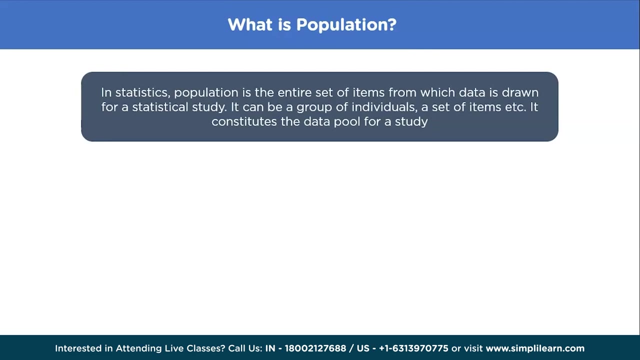 with IBM is just what you need For more details. head straight to our homepage and search for data science postgraduate program, or simply click on the link in the description box below. So what is a population? In statistics, population is the entire set of items from which data is drawn. 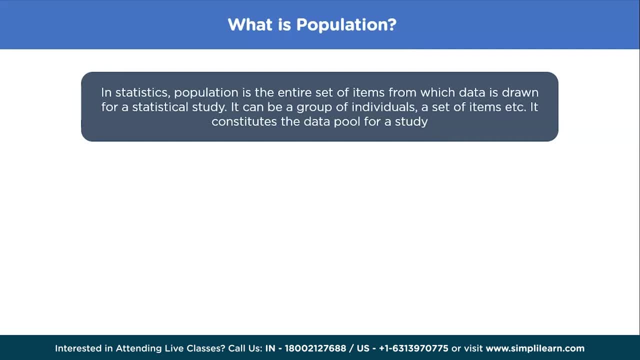 For a statistical study. it can be a group of individuals, a set of items, etc. It constitutes the data pool for a study. In general, a population is the entire group that you want to draw conclusions about. Usually, when we talk about population, you think about the people living in an area at 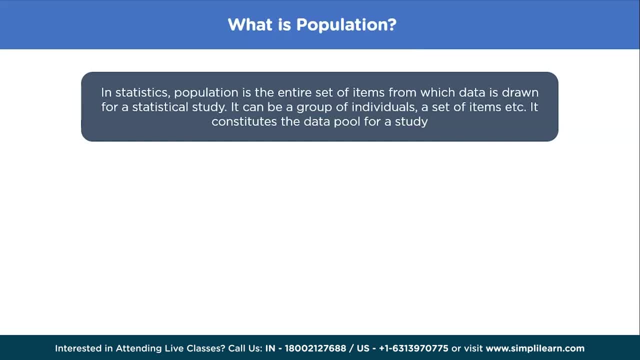 a time, But in research a population doesn't always refer to people. It can mean a group containing elements of anything you want to study, such as objects, events etc. Organizations, countries, species, organisms etc. For example, all undergraduate students in the Netherlands. 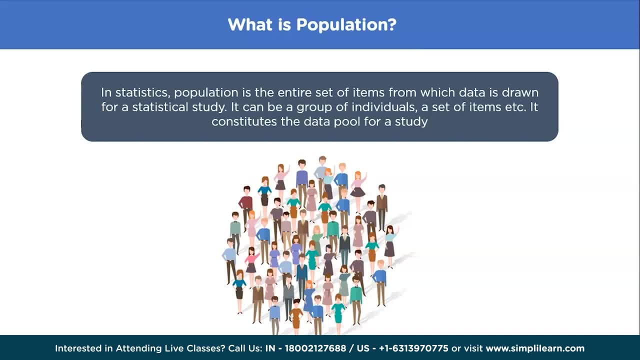 Or say you would like to know whether there is an association between job performance and the amount of home working hours per week in the specific case of Belgian data scientists. In this case, the population may be Belgian data scientists. However, if the scope of the study is more narrow, then the population will be more specific. 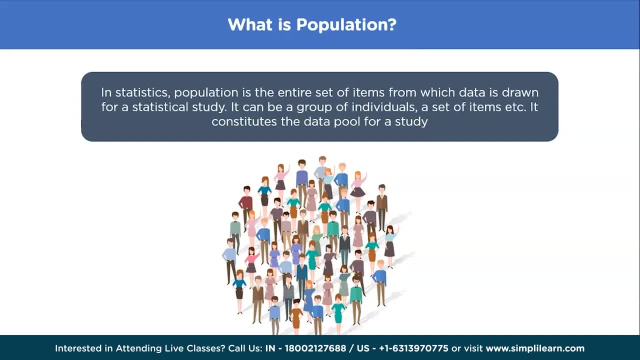 and include only workers who meet that certain criteria. The point is that the population should only include people to whom the results will apply, Since, in this case and many others, it is impossible to observe the entire statistical population due to time constraints, constraints on geographical accessibility and constraints on the researcher's. 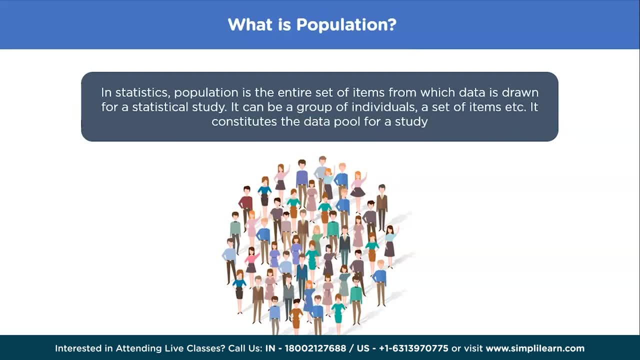 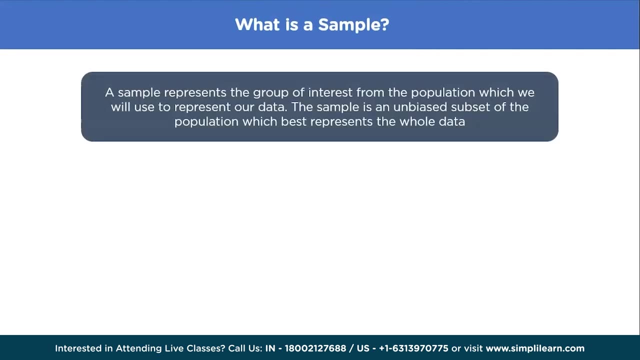 resources. a researcher would instead observe the statistical sample from the population in order to attempt to learn something a bit better. We can發 from here: population as a whole. This brings us to the topic. what is a sample? A sample represents the group of interest from the population which we will use to represent. 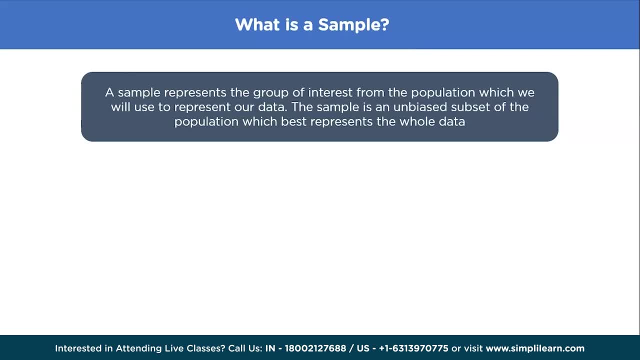 our data. The sample is an unbiased set of the population which best represents the whole data. A sample consists of some observations drawn from the population, So a part or a subset of the population. The sample is the group of elements who actually participated. 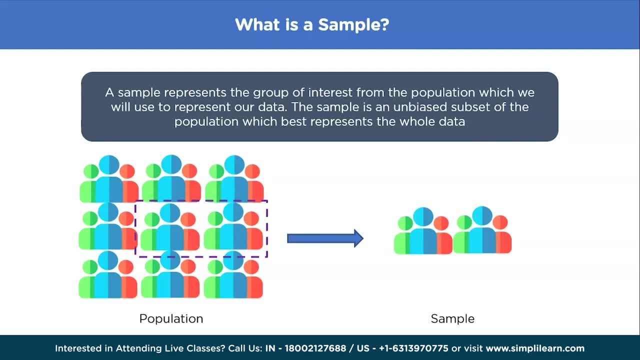 in the study, The size of the sample is always less than the total size of the population. Typically, the population is very large, making a census or a complete enumeration of all values in the population impractical or impossible. The sample represents a subset of manageable 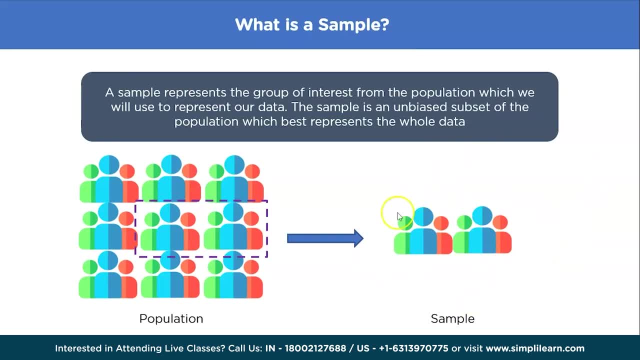 size. Samples are collected and statistics are calculated from the sample so that one can make interferences or extrapolations from the sample to the population. This process of collecting information from a sample is referred to as sampling. Say, you are testing the effects of a new fertilizer on crop yield. All the crop fields represent your population. 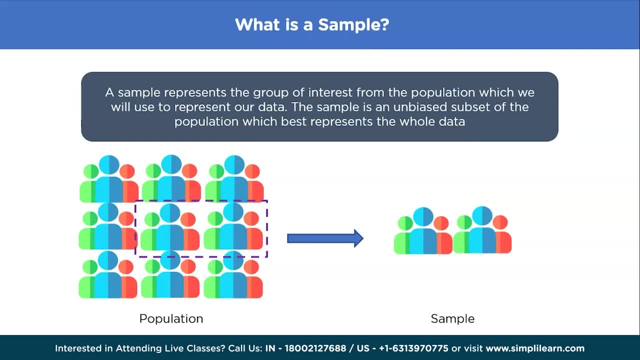 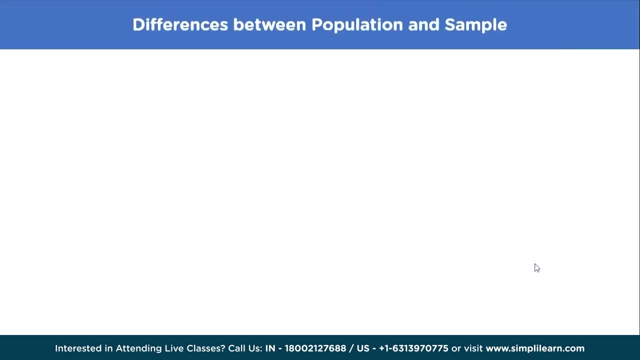 whereas the 10 crop fields you tested correspond to your sample. Now let's look at the differences between population and samples with the help of some examples. The first example would be that all students in a class would constitute the population of that class. Samples are easiest toihuld to allow you to calculate your sant layouts. A sample would: 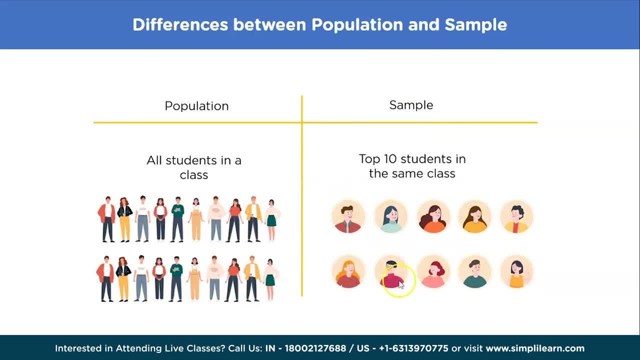 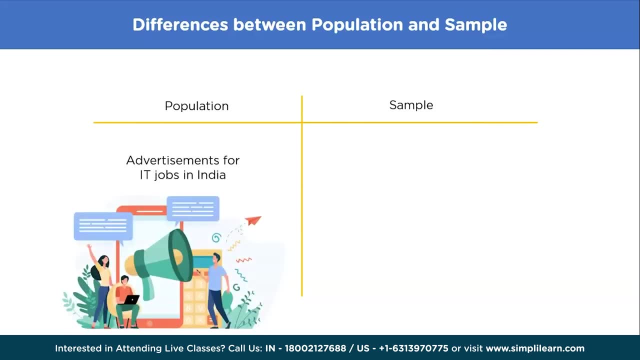 be only the top 10 students within the same class. The sample is a small subset of the population. in this case, Advertisement of IT jobs in India are the average for JEE search results, which we do here. A sample of that would be the Top Fifty Advertisements for the same job from policy. 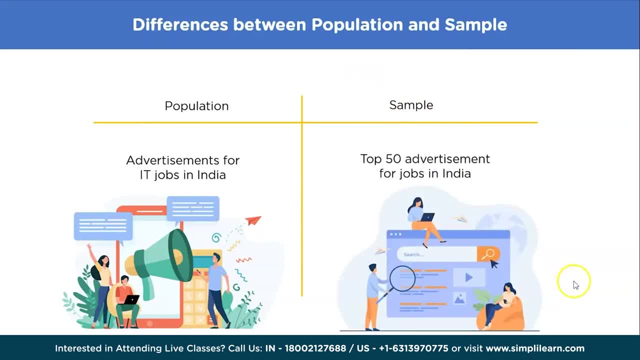 India. The sample would also represent the state of the country. The rate of completion of good or bad atom for AND jobs in India is also counted. Sample of all the students in an India would be the comparisons and all the test results are жеendereh starter results for. 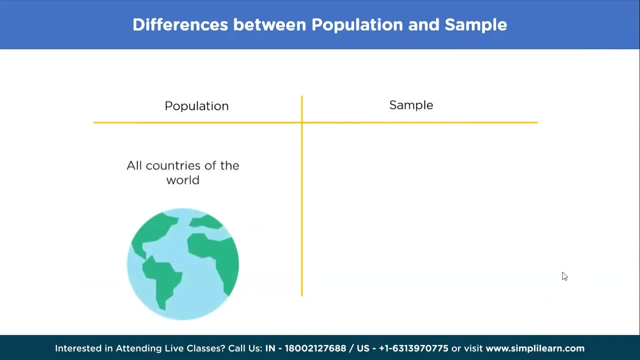 for the same jobs. Another example is all countries of the world. This represents a population of all the countries. A sample would be countries with published data on birth rates and GDP since 2000s. Next, let's look at how to collect data from a. 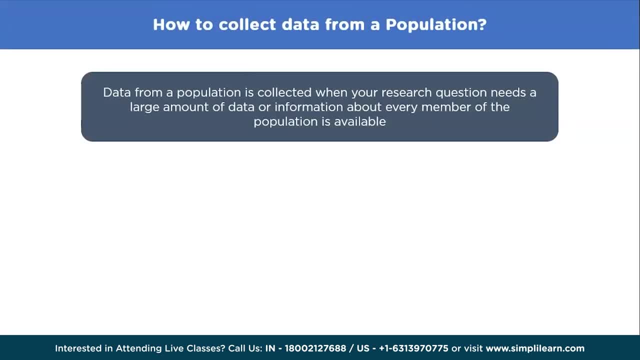 population. Data from a population is collected when your research question needs. a large amount of data or information about every member of the population is available. Populations are used when your research question requires or when you have access to data from every member of the population. 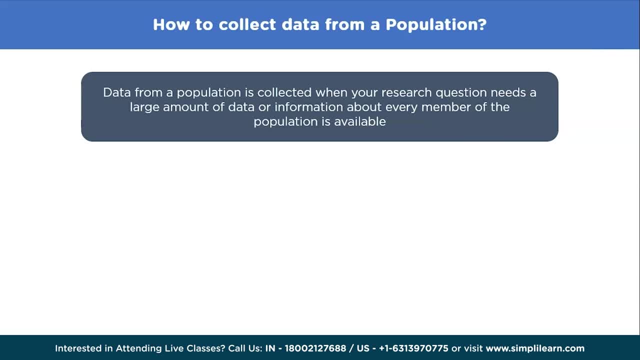 Usually, it's only straightforward to collect data from a whole population when it is small, accessible and cooperative. Population data is used when the data pool is small and cooperative to giving all of the required data. For larger populations, we can use sampling to represent part of the population and 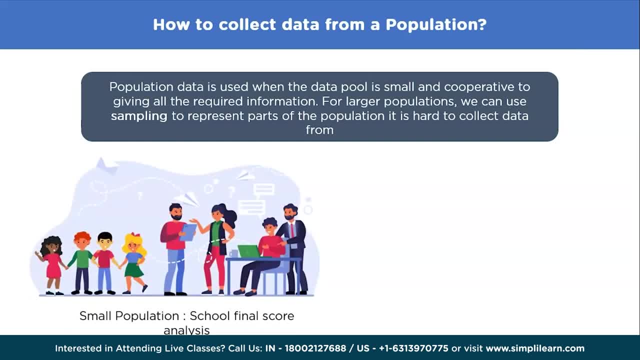 it is hard to collect data from. For example, a high school administrator wants to analyze the final exam scores of all graduating seniors to see if there is a trend. Since there are only interested in applying the findings to the graduating seniors in this high school, they can use the whole population. 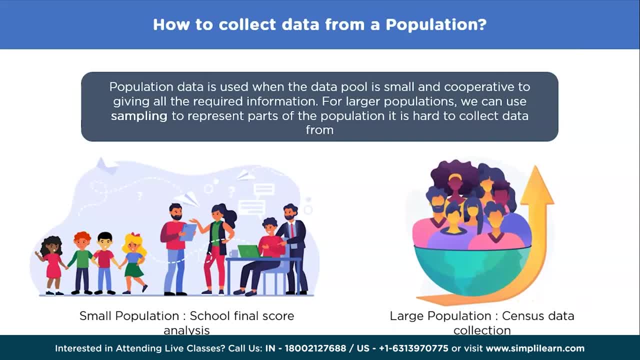 data set For larger and more dispersed populations. it is often difficult or impossible to collect data from every individual. For example, every 10 years the federal US government aims to count every person living in the country using the US Census. This data is used to distribute funding across the nation. 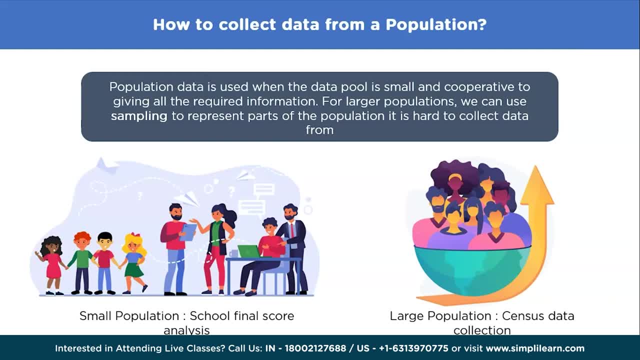 However, historically marginalized and low-income groups have been difficult to contact, locate and encourage participation from. Because of non- responses, the population count is incomplete and biased towards some groups, which results in disproportionate fundings across the country. In cases like this, sampling can be used to make more. 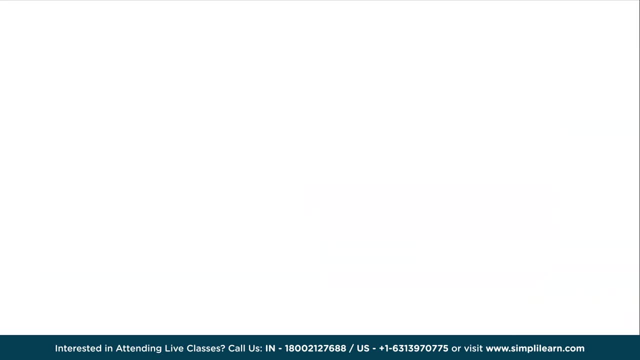 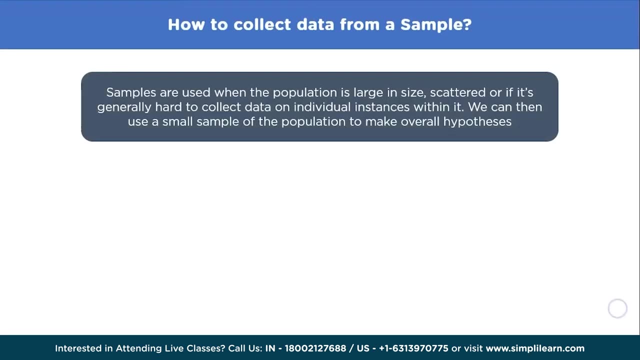 precise interferences about the population, And for that we can collect data from a sample. How do we go about collecting data from a sample? Samples are used when the population is large in size, scattered, or it's generally hard to collect data on individual instances within it. We can use a small sample of 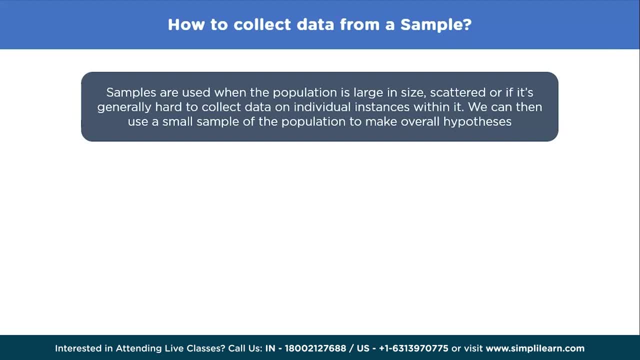 the population to make overall hypotheses. When your population is too large in size, geographically dispersed and the population is too large in size or difficult to contact, it is necessary to use a sample. With statistical analysis, you can use sample data to make estimates or test hypotheses about. 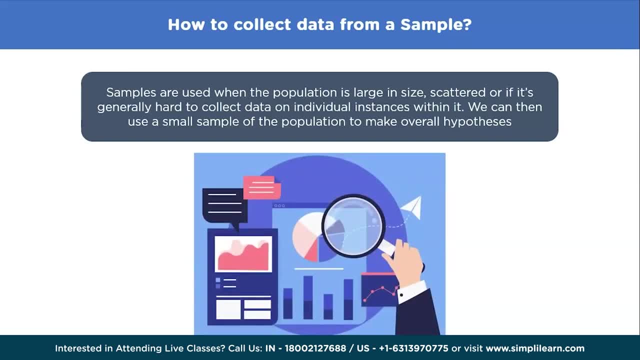 population data. For example, you want to study political attitudes in young people. Your population is the 3,000 undergrads in the Netherlands. Because this is not practical to collect data from all of them, you use a sample of 300 undergraduate volunteers from 3,000 undergraduates. 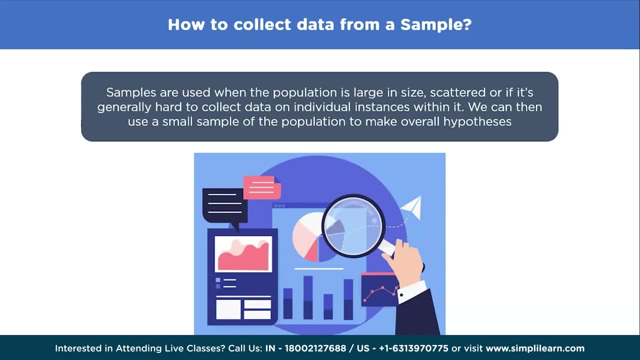 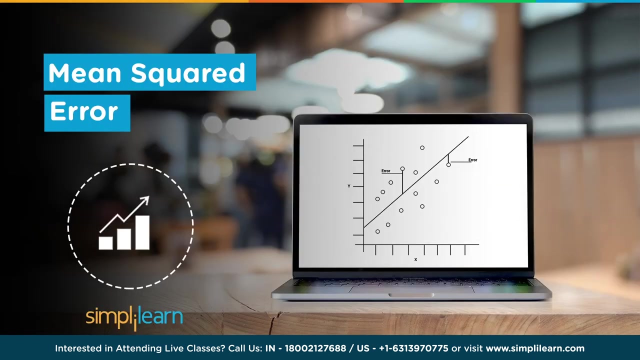 This is the group who will complete your online study. Ideally, a sample should be randomly selected and representative of the population. Using probability sampling methods such as simple random sampling or stratified sampling reduces the risk of sampling bias and enhances both internal and external validity. We'll discuss a very interesting and a very 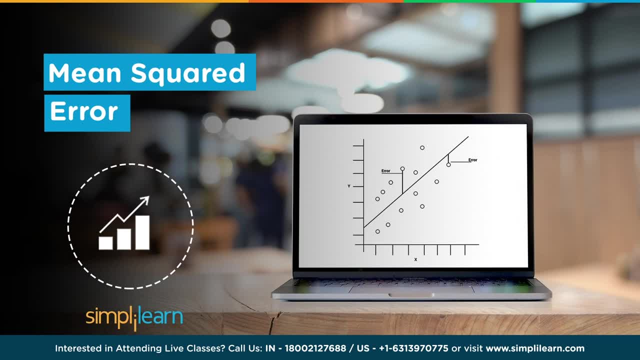 important topic, that is, the mean squared error, where it is used, and why do we actually need this mean squared function when there are already so many methods to evaluate the model? So watch this video till the end and, if this is your first visit to 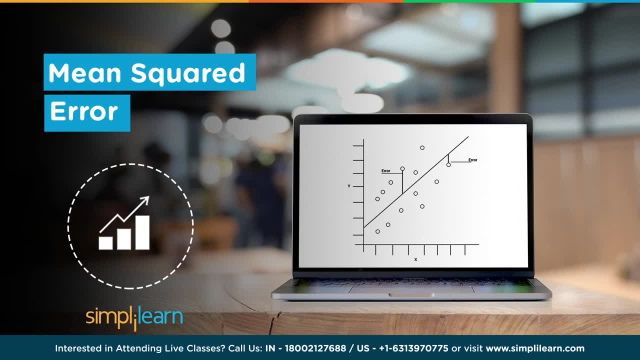 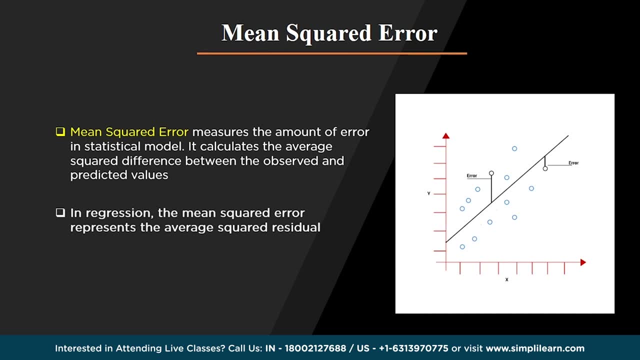 our channel. please click on the subscribe button so that you do not miss any update. Let's start by defining what is mean squared error. Mean squared error measures the amount of error in a statistical model. It calculates the average squared difference between the observed and predicted error. It is used to 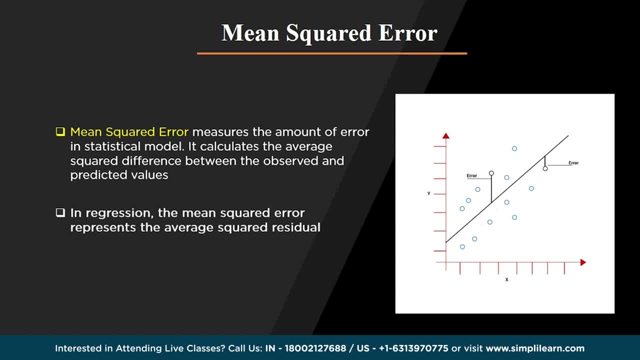 calculate the number of predicted values. In regression line, the mean squared error represents the average squared residual. As you can see in the graph, as the data points fall closer to the regression line, the model has less error, decreasing the mean squared error. A model with less error produces more precise predictions. 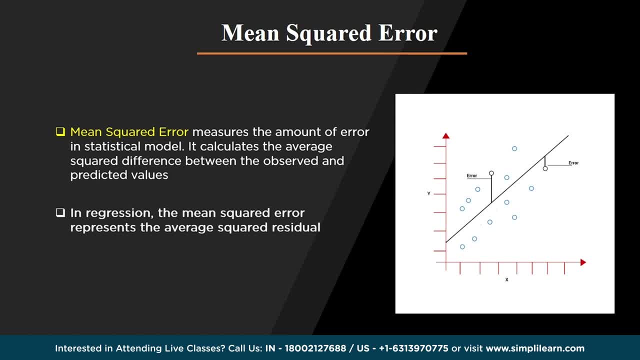 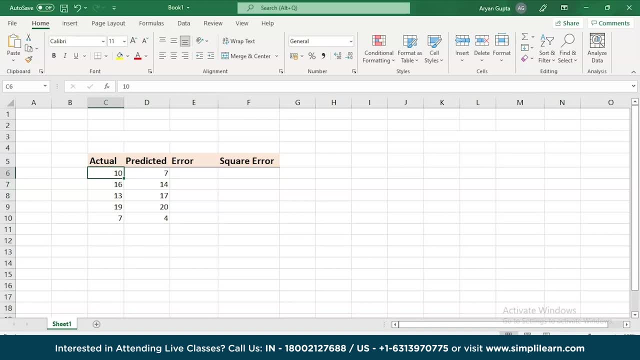 Now let's jump to our excel workbook and discuss it with an example. Here we have a small table with the actual and predicted values. We will start by finding the error between the actual and predicted values, which will be the difference between the actual minus predicted values. So here 10-7 will become. 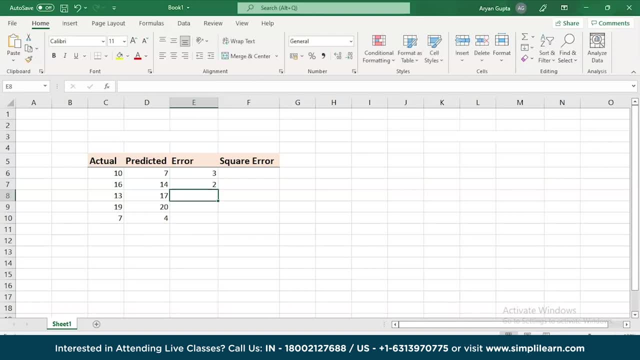 3,, 16-14 will become 2,, 13-17 will become minus 4, 19-20 becomes minus 1, and 7-4 becomes 3.. Now just calculate the total of the errors. While calculating the total, we will treat. 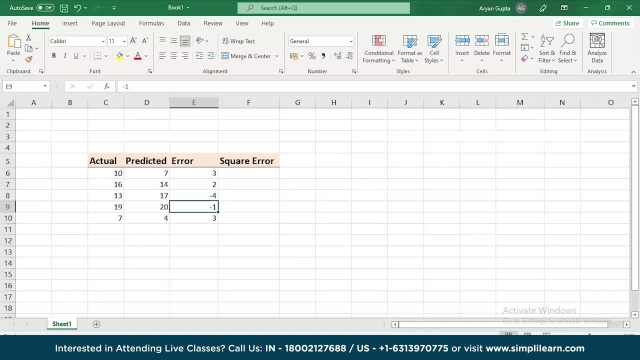 this negative value as a positive value. We will also find the error between the actual and predicted values, which will be the difference between the actual and predicted values. So value. So here the total of the errors will become 3 plus 2,, 5 plus 4,, 9,, 10 and 13.. Then 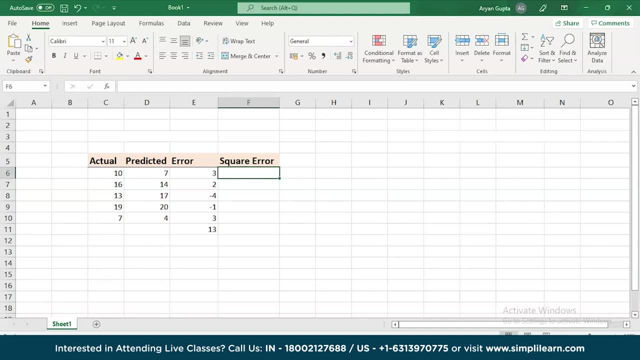 we will calculate the square of the errors. So here 3 square will become 9,, 2 square will become 4,, 4 square will become 16, 1 square will become 1 and 3 square again is 9.. And 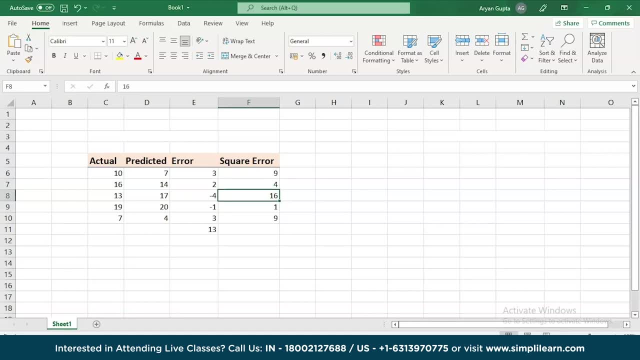 we will do the total of the square errors. So this will become 9 plus 4,, 13,, 13 plus 1,, 14,, 14 plus 16,, 30 and 39.. To find the MSE, that is the mean squared error, we will divide. 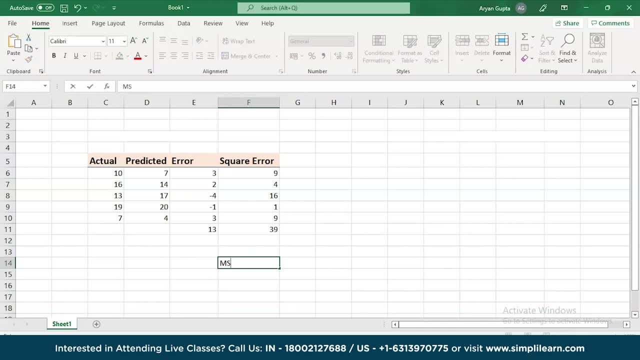 the total of the square error values with the total number of records. So here, MSE will be equal to 39 divided by, and we have the total number of records, that is, 5,, which will be 7.8.. Let's. 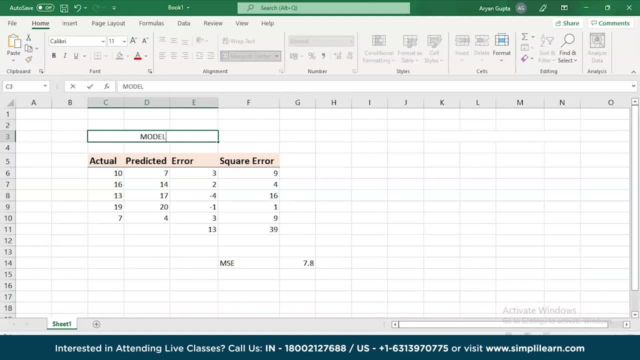 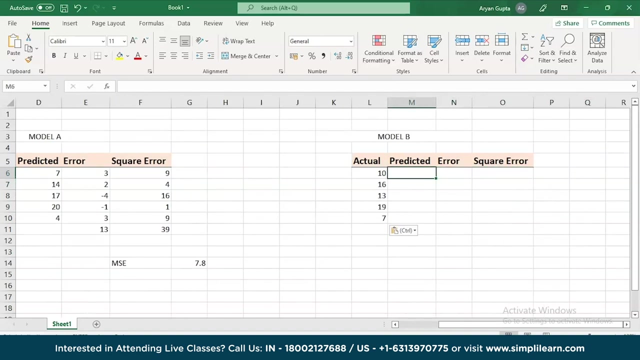 name this as model A. Now, for the comparison purpose, we will create another model, that is model B. We will have all the columns here And we will keep the actual values here same. We will just change the predicted values. So let's take some random values. We will keep this as 13,. we will take this as 20,. 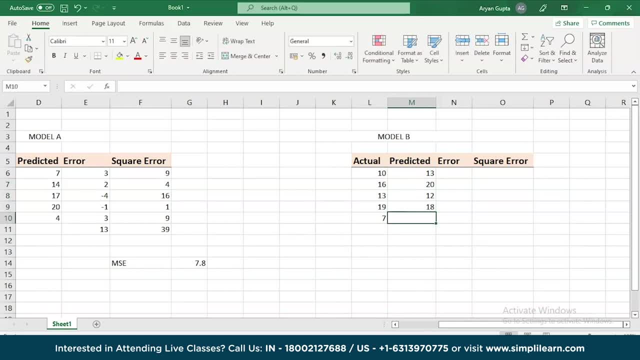 we will take this as 12, 18 and 3.. Now, to calculate the error, we'll subtract the predicted values from the actual values. So 10 minus 13 wil become minus 3, 16 minus 20 will become minus 4.. This will become 1,. 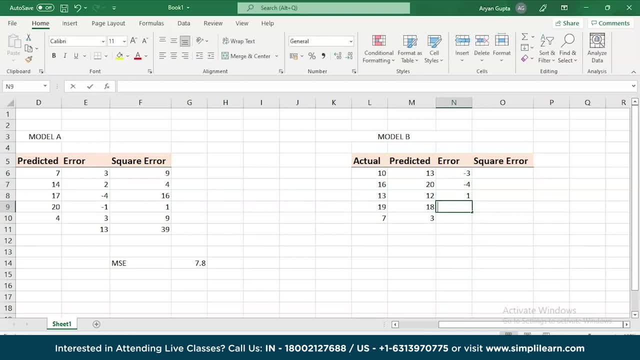 this will be 1 and this will be 4.. Now to calculate the square error, we will just square the error values. So this will be 9,, this will be 16,. this will be 1, this will be 1.. 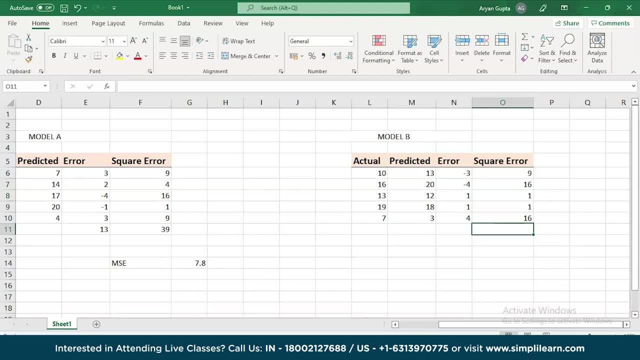 And this will be 16.. ри, The total of all the square values will come out to be 43.. Now to calculate the MSE again, we will divide the total square values with the total number of records. So here this will be equal to 43 divided by 5, which will come out to be 8.6.. 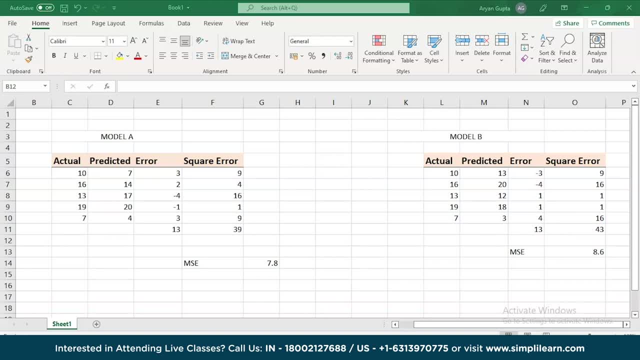 If you observe here, the total of the errors in both Model A and Model B is same. that is, 13.. So which model to prefer? Since the MSE of Model A is lesser than Model B, we will prefer Model A because we are okay with a model that has small, small errors, but in Model B there are some significantly large. 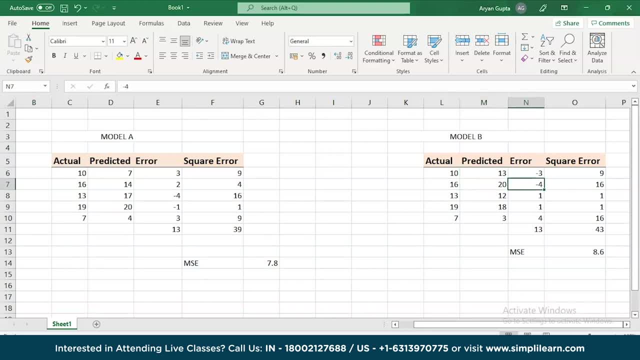 errors. suppose in this case 16-20, that is minus 4,, minus 3 and this here 4.. So we do not want a model where the errors, large errors specifically, are more frequent. We can have a model with the small errors, that will be okay. 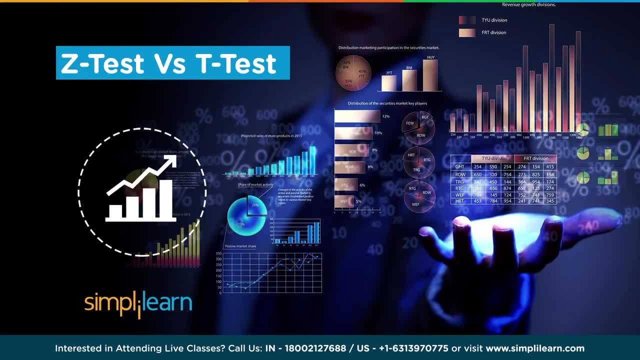 So we will prefer Model A over Model B. We will discuss about the two important parametric tests that are Z-test and T-test, and what are the major difference between them. We will also work out an example to understand how the Z value and the critical value plays. 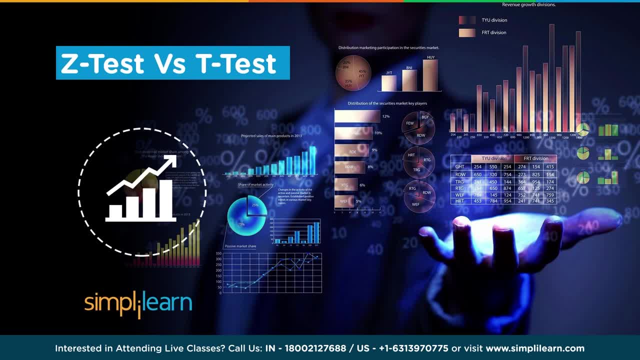 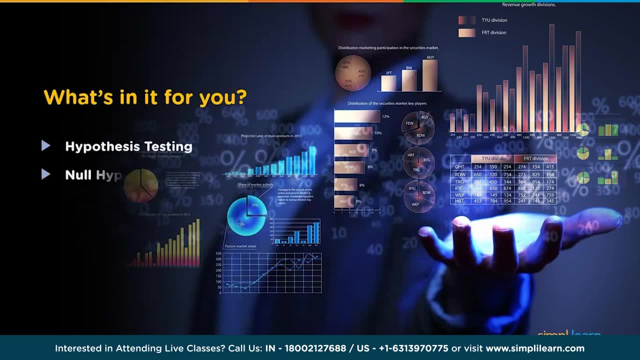 an important role in the hypothesis testing. So let's start. We will start by discussing what is hypothesis testing and what is the importance of null hypothesis, Then we will discuss the example for the same, and then we will move on to Z-test and T-test. 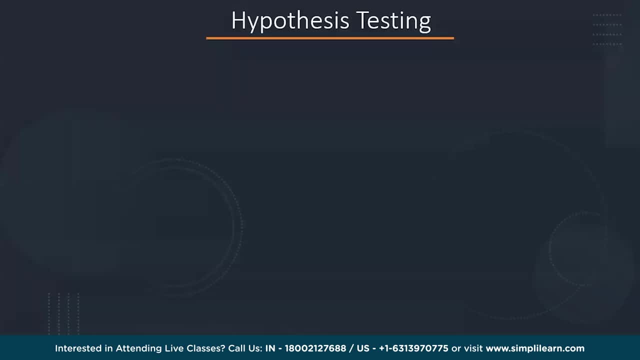 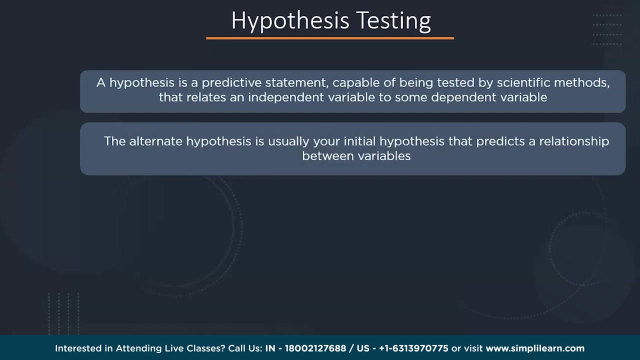 and understand the difference and the major points regarding it. So what is hypothesis testing? A statistical hypothesis is an assumption about the population parameters. this assumption may or may not be true. Hypothesis testing refers to the formal procedures used by statisticians to accept or reject the 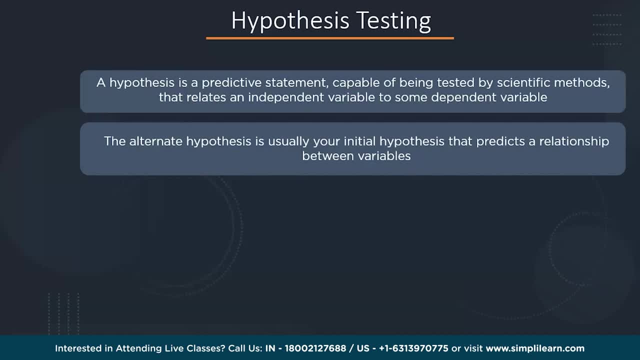 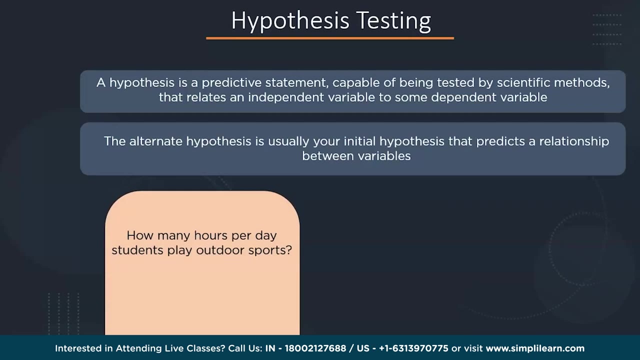 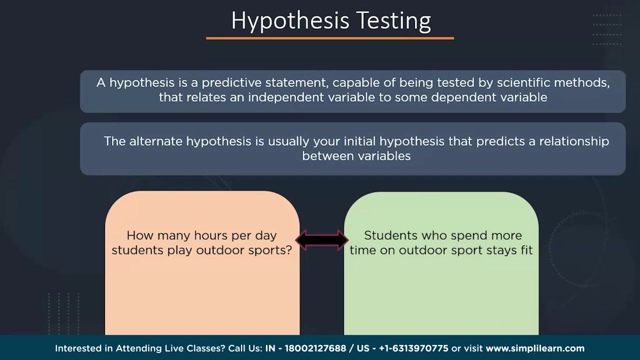 statistical hypothesis. Here the alternate hypothesis is usually your initial hypothesis that predicts the relationship between the two variables. For example, suppose you answer the question how many hours per day a student plays outdoor sports. With this data you can make a hypothesis: students who spend more time on outdoor activities. 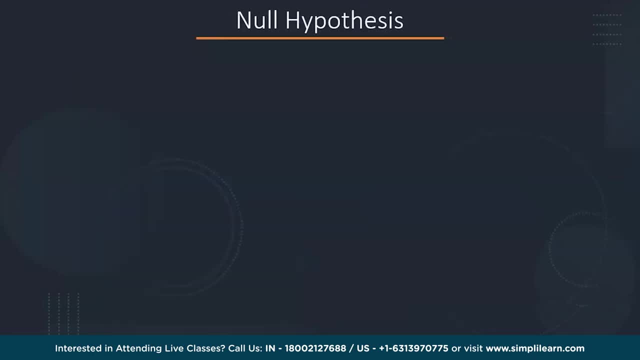 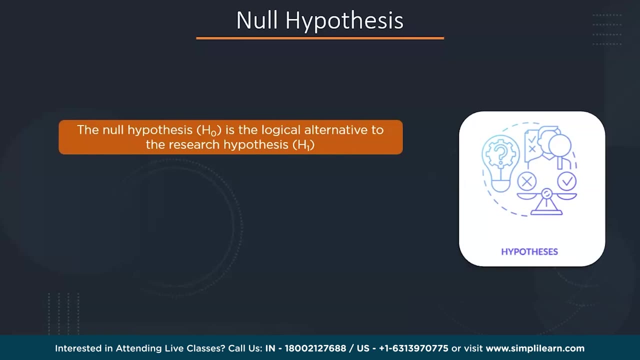 stays fit In this hypothesis testing there is one major term, that is null hypothesis. So what is hypothesis testing? A null hypothesis expresses the opposite of what a researcher or experiments predicts or anticipates. It essentially defines the statement that no exact or actual relationship exists between 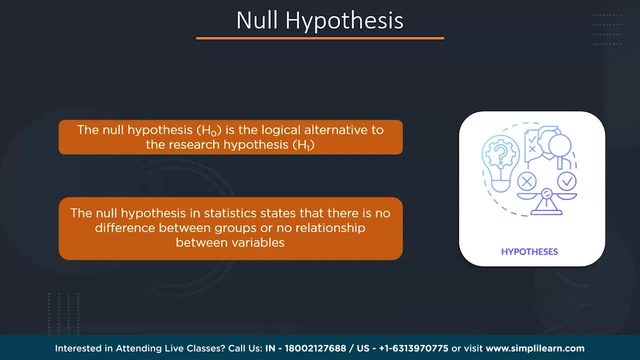 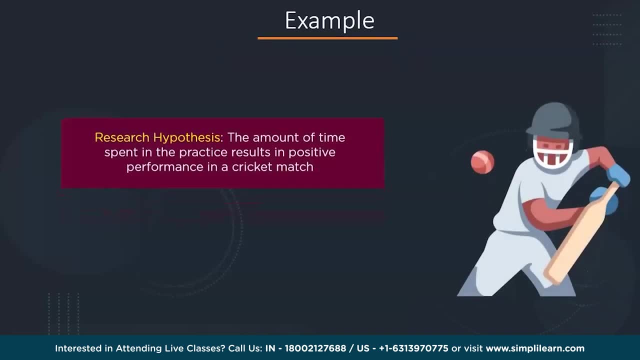 the variables. Usually it is denoted by H0.. Let's try to understand the research and null hypothesis with the help of an example. Suppose a research hypothesis says the amount of time that is spent On a cricket practice results in a positive performance in the actual cricket match. 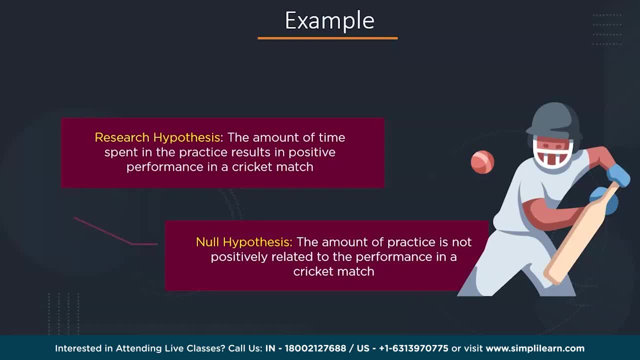 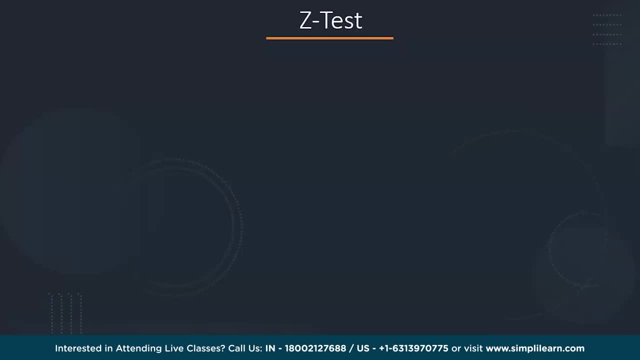 So, in accordance with it, a null hypothesis can be that the amount of practice is not positively related to the performance in the cricket match. Now that we know about the null and research hypothesis, let's move on to z-test. So what is z-test? 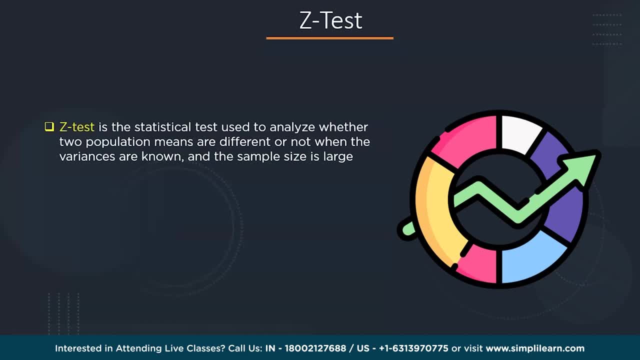 A z-test is a statistically significant test for hypothesis testing. It is used to analyze whether the two population means are different or not, when the variances are known and the sample size is very large. In this, the sample size should be usually more than 30.. 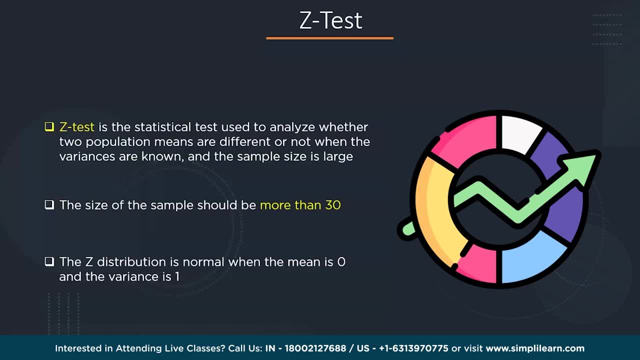 And when the z-distribution is normal, the mean is 0 and the variance is 1.. There are few assumptions that we take into consideration when calculating the z-test. The first one is: although observations are independent, there are merely three steps in the 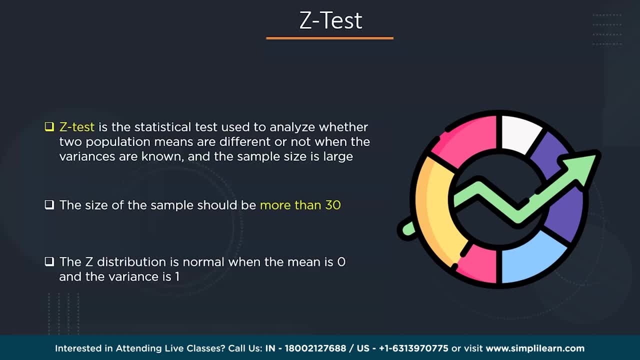 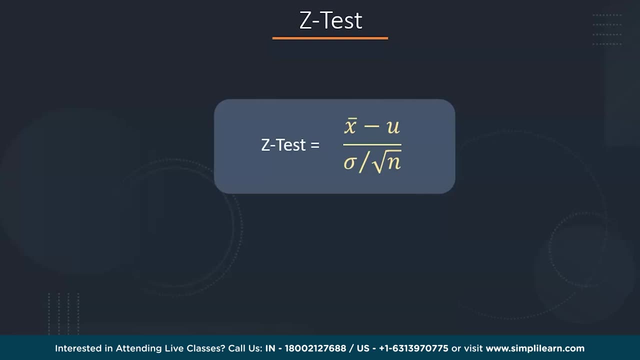 hypothesis testing. The first one is state the null and alternate hypothesis and perform the statistical test And with the help of a z-value we can accept or reject the null hypothesis. Let's discuss this more clearly with the help of an example, But before that let's discuss the formula. So to calculate the z-value we 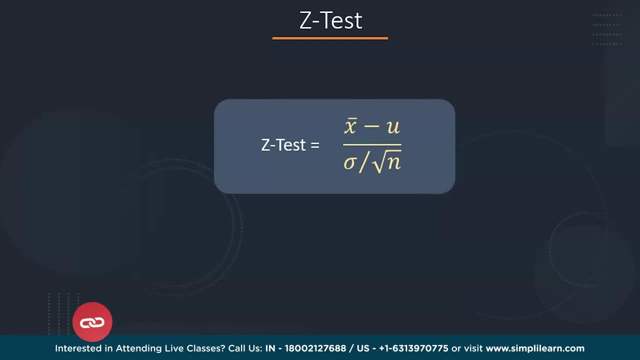 have this formula, that is, x bar minus mu, divided by sigma, divided by root n, Where x bar represents the sample mean and the sigma is the population standard deviation. n is the sample size and mu is the population mean. Let's see how you can use this formula to arrive at a null or alternative. 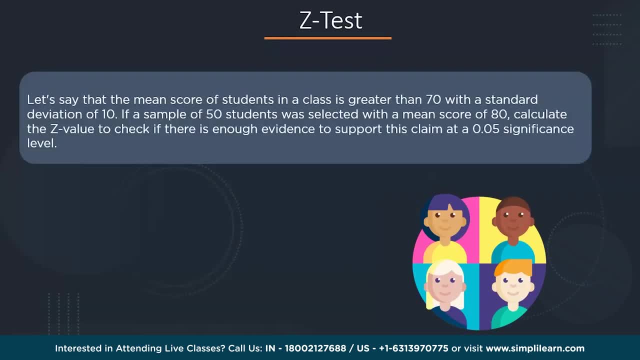 hypothesis. Let's say that the mean score of students in a class is greater than 70, with a standard deviation of 10.. If the sample of 50 students was selected with a mean score of 80, we have to calculate a z-value to check. 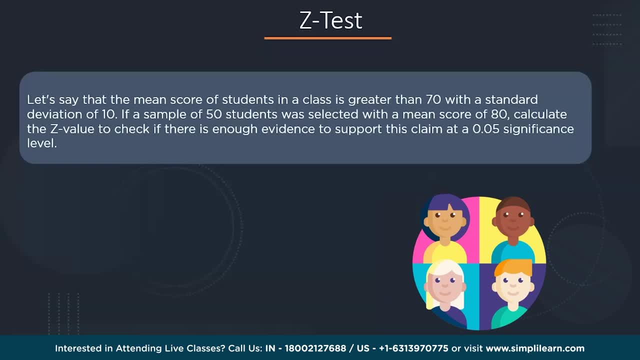 if there's enough evidence to support this claim, at 0.05 significance level. So let's point down the important data. We have: the x bar, that is sample mean, equal to 80.. The sigma is given to be 70,. that is the 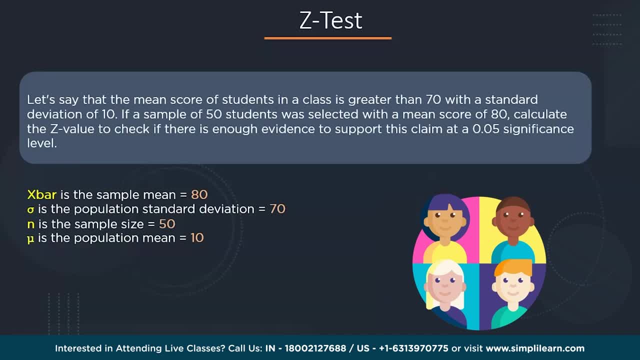 population standard deviation. n is the sample size, which is equal to 50. And mu is the population mean, that is equal to 10.. Putting all the values into the formula, we get z-value to be 7.09.. Now, at the significance level of 0.05, the critical value is 1.645, which is 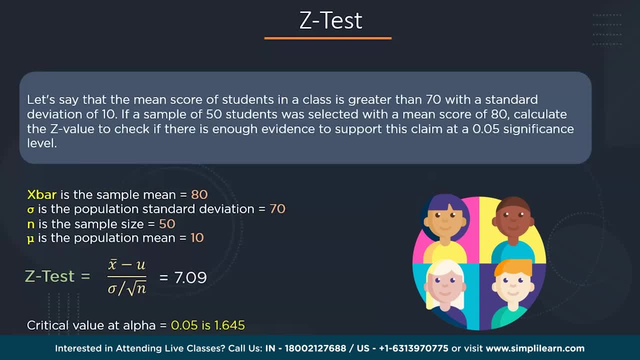 calculated with the help of a z-table. You can get this z-table simply by searching in google. So we have a z-value to be 7.05.. and the critical value to be 1.645.. Since 7.09 is greater than 1.645, we can simply. 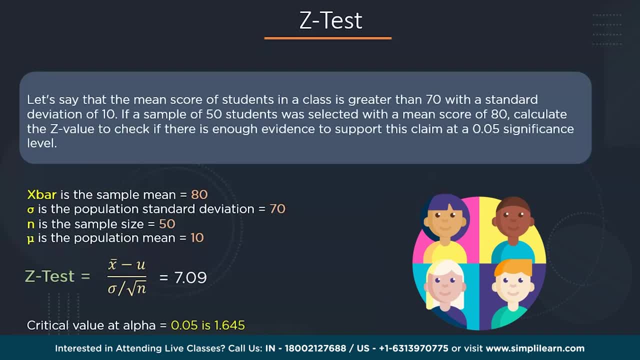 reject the null hypothesis and come to a conclusion that there is enough evidence to support that the mean of the class is greater than 70. This is how you can use the z-value to arrive at a proper conclusion. Now let's move on to t-test. T-test in statistics. 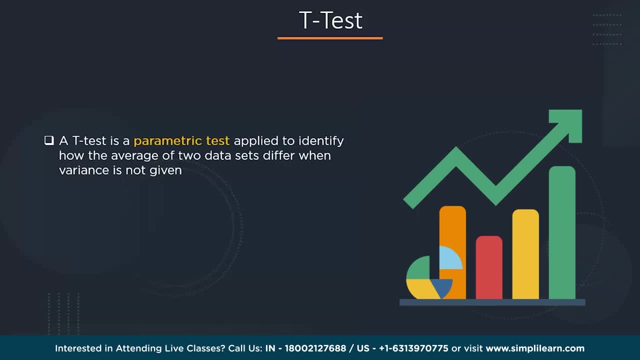 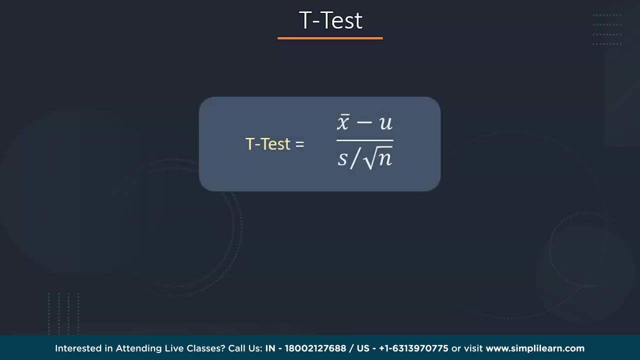 is a method of testing hypothesis about the mean of a small sample drawn from a normally distributed population when the population's standard deviation is not known. In this case, the data is continuous. The formula to calculate the t-value is x-bar minus mu divided by s. 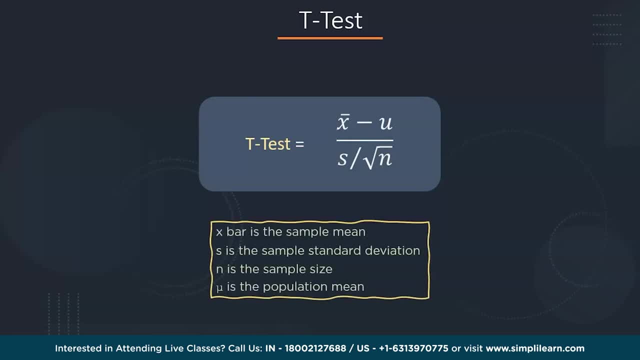 divided by root n, where x-bar is the sample mean, s is the sample standard deviation, n is the sample size and mu is the population mean. Let's discuss with the help of an example. Suppose a store wants to use a sample standard deviation. 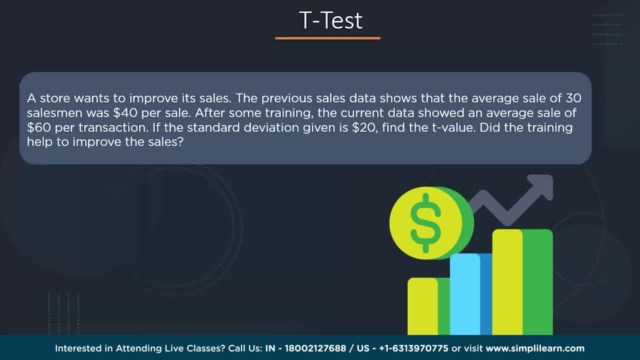 The previous sales data shows that the average sales of 30% was $40 per sale. After some corporate training, the current data showed an average sale of $60 per transaction. If the standard deviation is given to be $20, we have to calculate the t-value and we have. 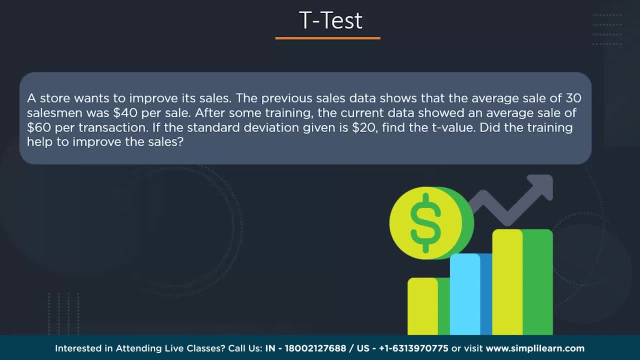 to arrive at a conclusion that: did training improve the sales or not? So in this case we have the sample mean to be 60,, standard deviation to be 20,, the sample size is taken as 30, and the population mean is 40.. 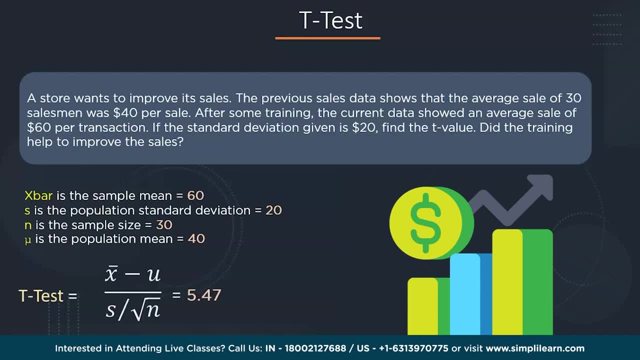 Putting all the values in the formula will arrive at a value of 5.47.. In this case also, we assume the significance value to be 0.05.. Now, moving from right to left in a Z-table, the critical value will come out to be 1.711, which is less than 5.47.. So in this case also, 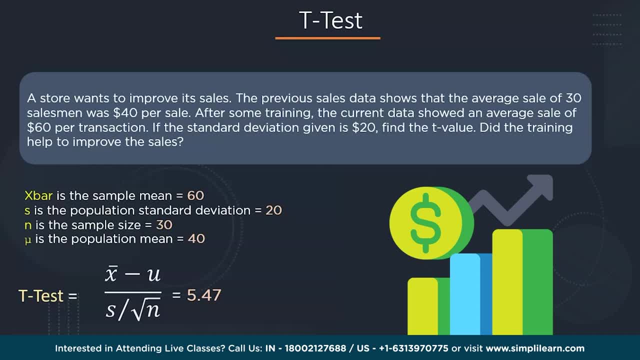 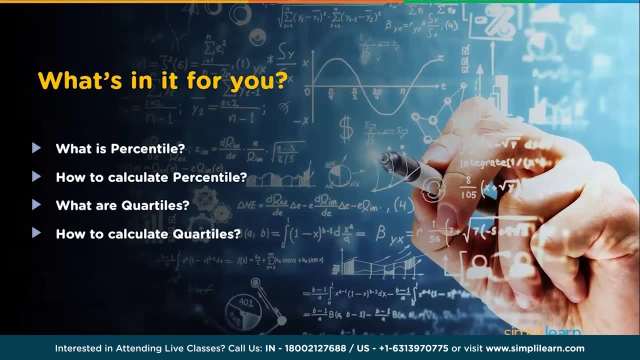 we can reject the null hypothesis and we can conclude that the training did affect the sales and the training was helpful. In this tutorial we are going to learn what is percentile and how we can calculate the percentile with the formula. Then we will move on to quadratiles and we will see what are quadratiles and how we can calculate the. 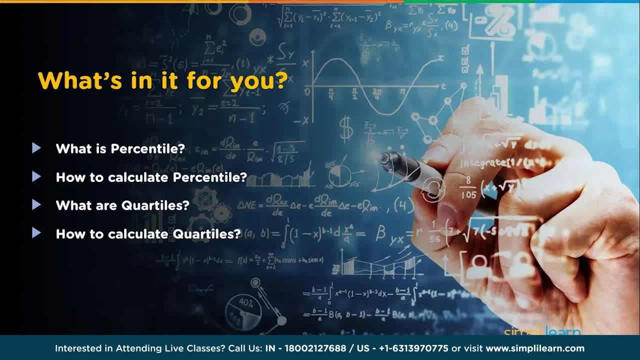 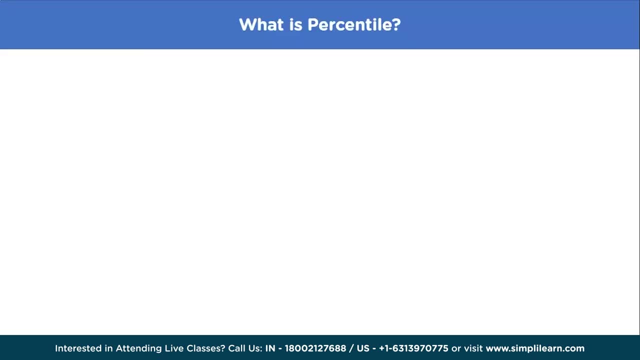 quadratiles with the help of the formula. So, without further ado, let's get started. We'll start with percentile. So what exactly is a percentile? A percentile is a term used in statistics to express how a score compares to other scores in the same dataset. So we 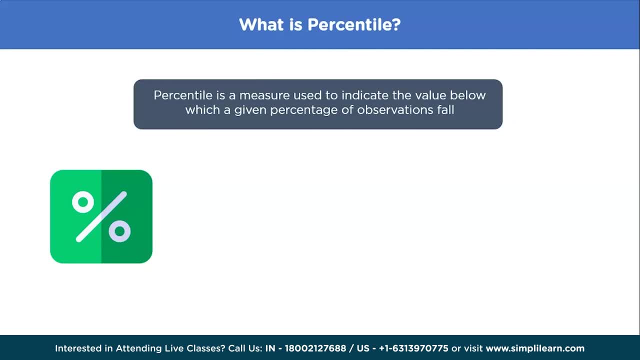 will start with percentile. While there is technically no standard definition of percentile, it is typically communicated as a percentage of values that fall below a particular value in a set of data scores. Percentiles are commonly used to report values from a non-referenced test. The formula to calculate a percentile is: px is equal to x. 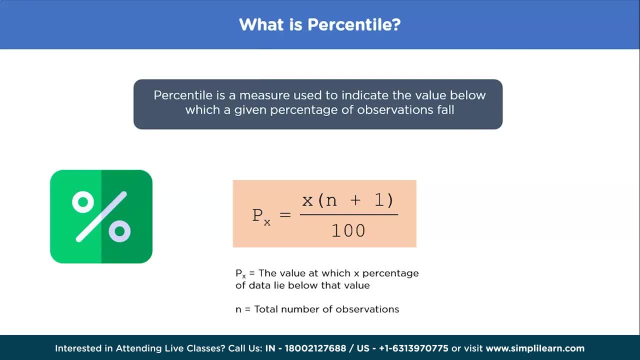 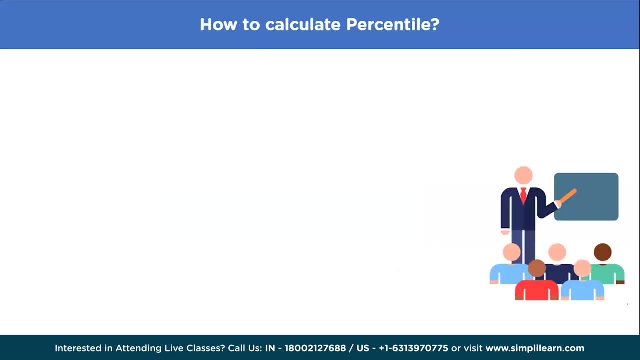 n plus 1 divided by 100, where x is the percentile you want to calculate and n is the total number of observations. Let's understand this formula better with the help of an example. So let's see how to calculate a percentile. Suppose you have marks of 20 students. Here we have 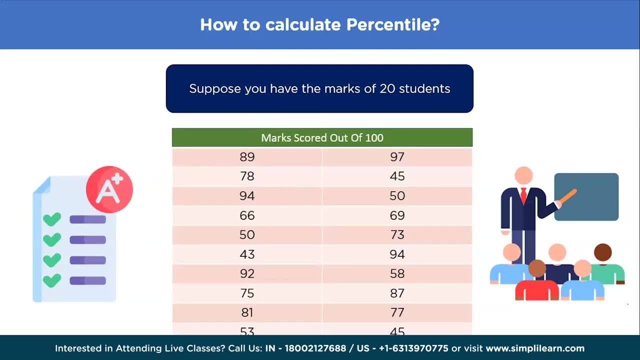 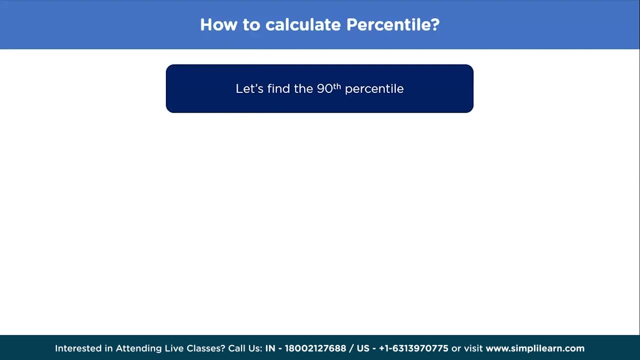 the marks of 20 students: 89,, 78,, 94 and so on. The marks are scored out of 100.. Let's try to find out the 90th percentile. So the first step to calculate the 90th percentile. 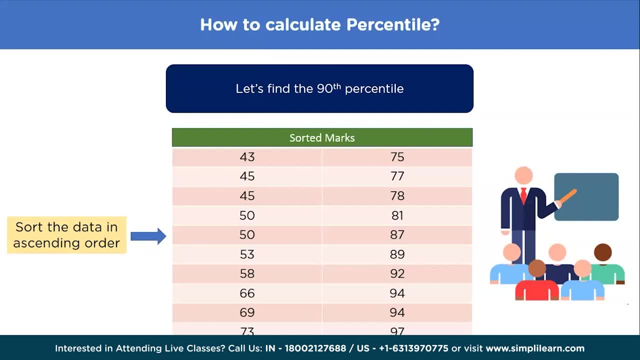 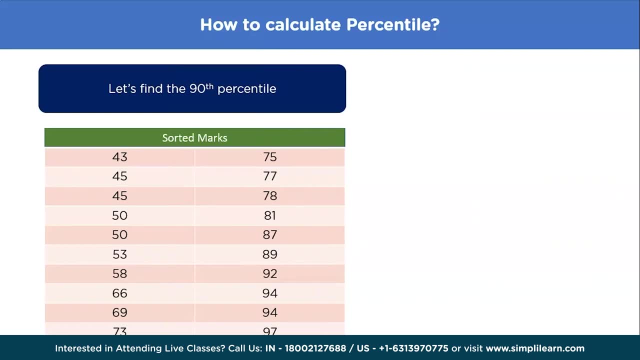 is to sort the data in ascending order. So here we have sorted the data in ascending order from 43, 45,, 45 till 97.. Next step is to substitute the values in the formula, So p90 will be is equal to 90,. 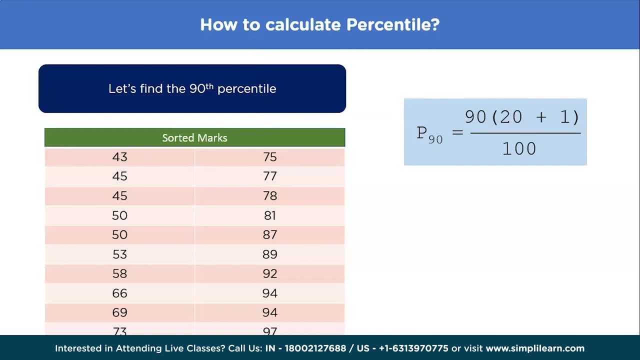 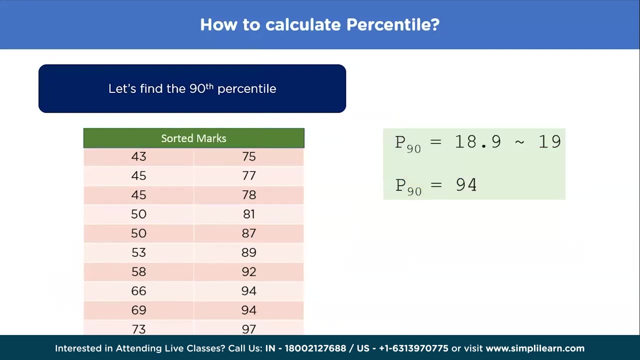 20 plus 1 divided by 100, where 90 is the percentile you want to calculate and 20 is the number of observations, It will come to 1890 divided by 100, which will be approx to 94. So our 90th percentile is the 94 marks in the data set. What exactly does this 94? 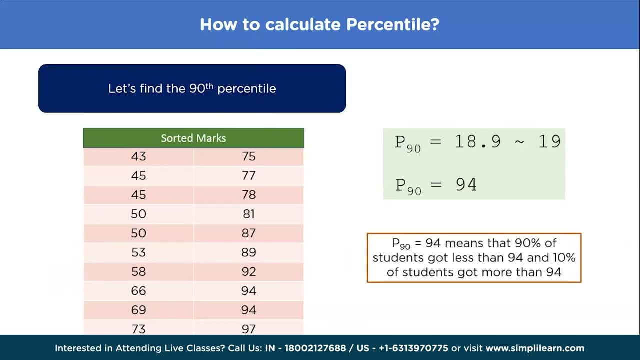 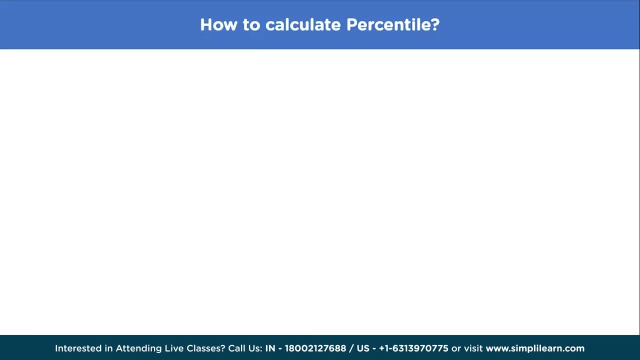 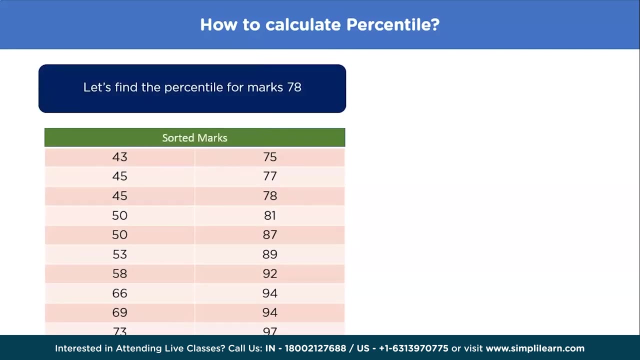 marks signify p90. equal to 94 means that the 90% of the students got less than 94 marks And the 10% of the students got the marks more than 94. There is another way to calculate the percentile. Let's see how we can do that. Suppose we want to calculate at what percentile. 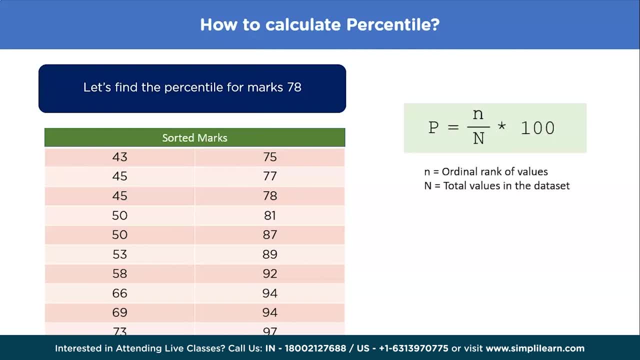 range the 78 marks fall. So to calculate this we have the formula: p is equal to n divided by N into 100, where n is equal to ordinal rank of values and N is equal to total values in the data set. So, substituting the values in the above formula, we get 12 into 100 divided. 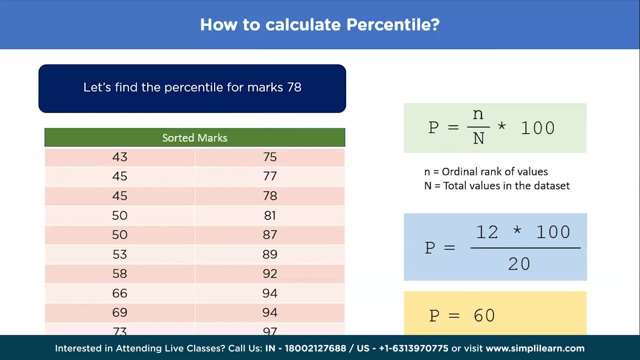 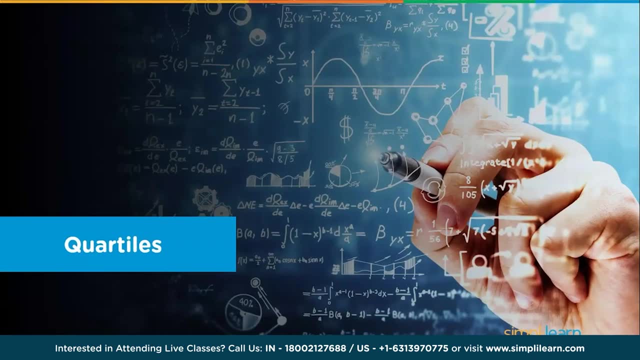 by 70,, which will be equal to 60. So this means that the 78 marks signify the 60th percentile in the data set. Now that we have discussed the percentiles and know how to calculate the percentile, let's move on to quartiles. What are quartiles? Quartile as the name. 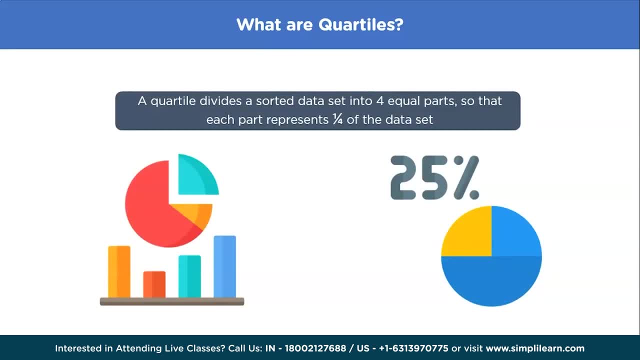 suggests is a statistical term that divides the data into the 4 quarters. It basically divides the original data points into the 4 quarters. on the number line, The Q1, which is also called the first quartile, is the 25th percent of the data set. So this is. 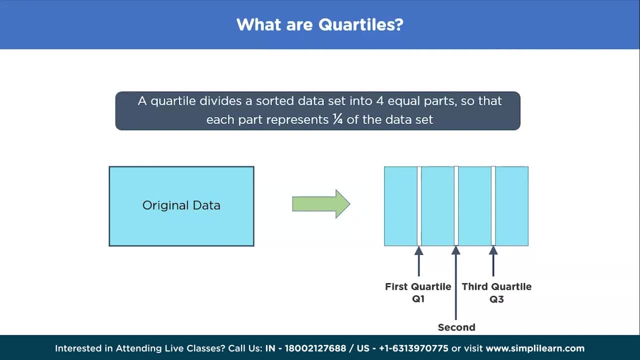 the 50th percent of the data set. The second quartile, which is Q2,, signifies the 50th percent of the data set and the third quartile, which is Q3, signifies the 75% on the data set. The 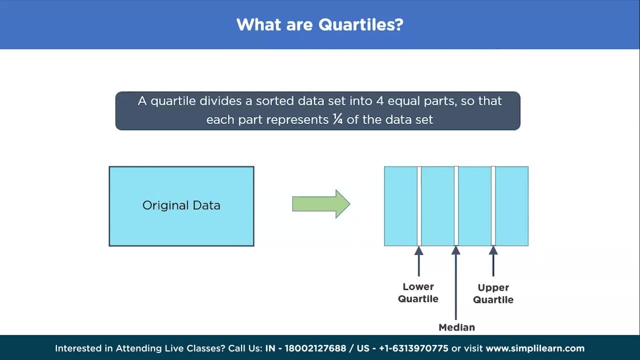 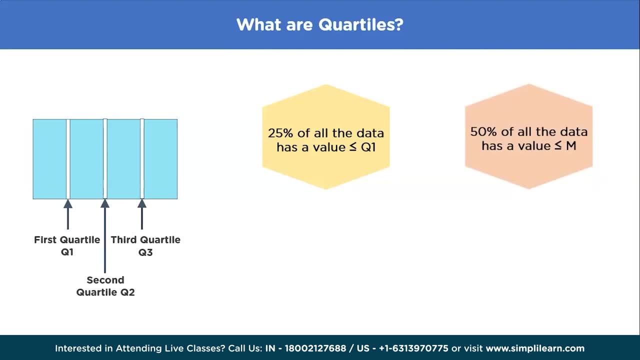 Q1 is also called the lower quartile and the upper quartile is also called as Q3.. 25% of all the data has a value less than or equal to Q1.. Second quartile, which is also the median, has 50% of all the data less than M. 75% of all the data has a value less than. 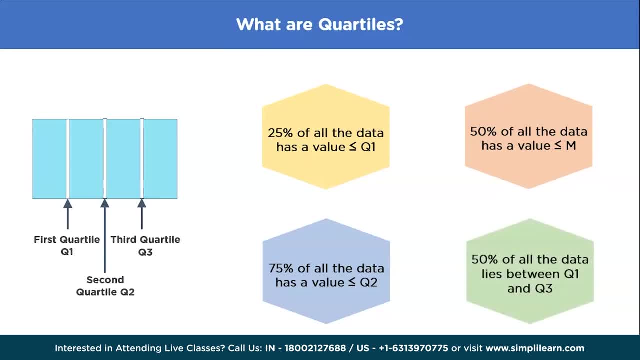 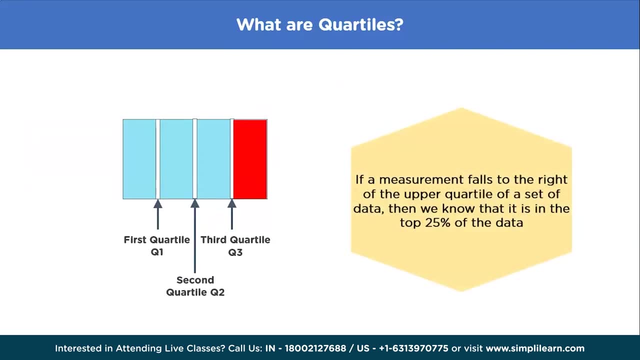 or equal to Q2.. And the 50% of all the data lies between Q1 and Q3.. If the measurement falls on the right side of the upper quartile in a set of data, then we know that it is in the top 25% of. 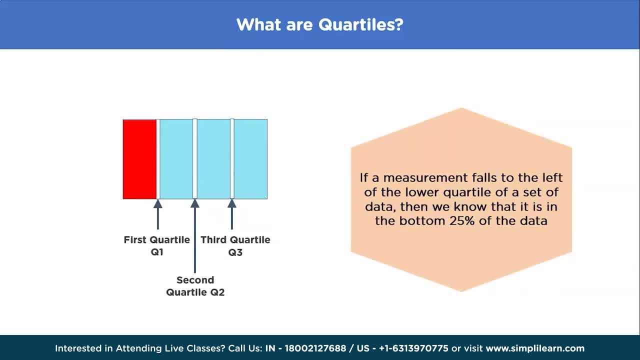 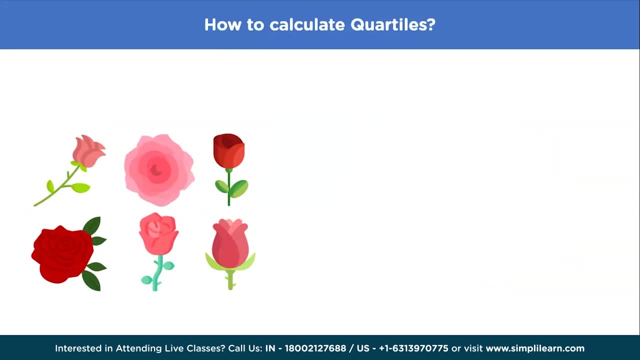 the data. If the measurement falls to the left of the lower quartile of a set of data, then we know that it is in the bottom 25% of the data. Now that we have discussed the theoretical aspect of quartiles, let's understand how. 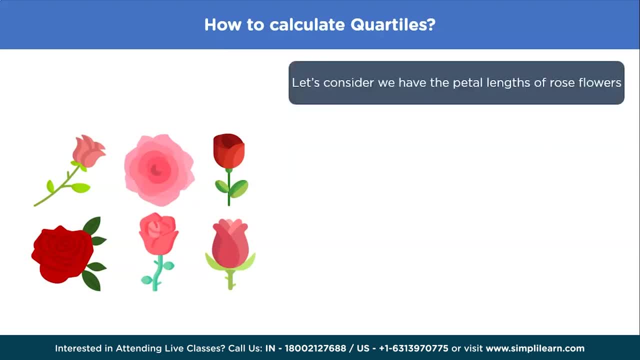 we can calculate the quartiles For this. we have taken one famous example. Let's consider it. We have the petal length of rose flowers. Here we have the petal length of rose flowers. We have the petal length in centimeters. 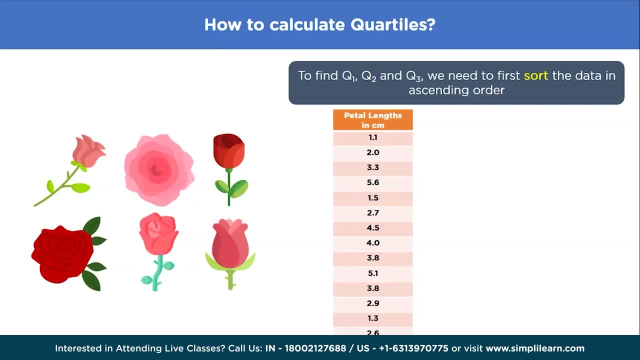 To find the Q1,, Q2, and Q3, we first need to sort the data in ascending order. So when we sort the data in ascending order, we get the following values: 1.1,, 1.3,, 1.5, till 5.6.. 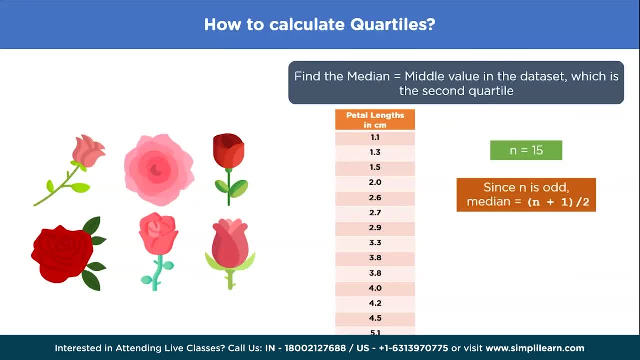 To find the M we have two formulas: First when the N is odd and the second when the N is even. Since here the N is odd, which is equal to 15,, we will calculate the median by N plus 1 by 2.. 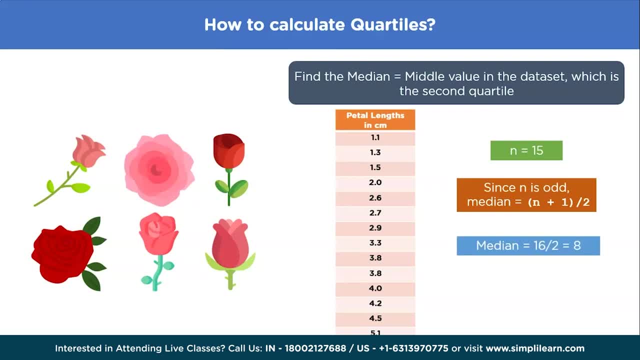 It will be 16 by 2.. It will be 16 by 2, which is equal to the eighth value in the data set. So the Q2 is the eighth observation, which is equal to 3.3 in the data set. To find the first quartile value we have the formula: Q1 is equal to N plus 1 into 1. 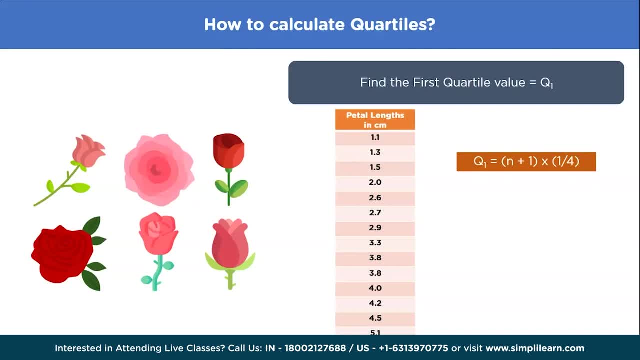 by 4.. N plus 1, because we have the N as odd, which is equal to 15.. So dividing 16 by 4,, we get the value equal to 4.. So Q1 is the fourth observation, which is equal to 2.0.. 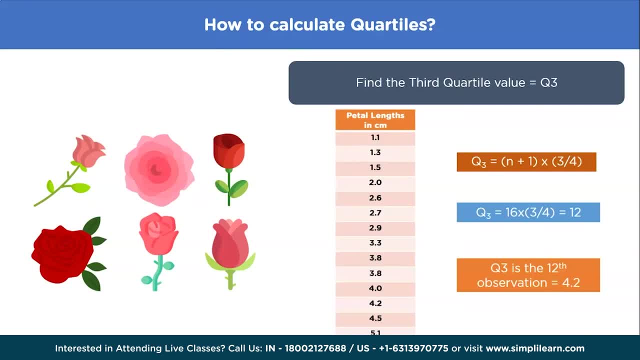 So this point is our first quartile. Now to calculate the Q3, which is the top 25% of the data set, we multiply the N plus 1 into the 3 by 4.. So Q3 is the twelfth observation, which will come out to be 4.2. 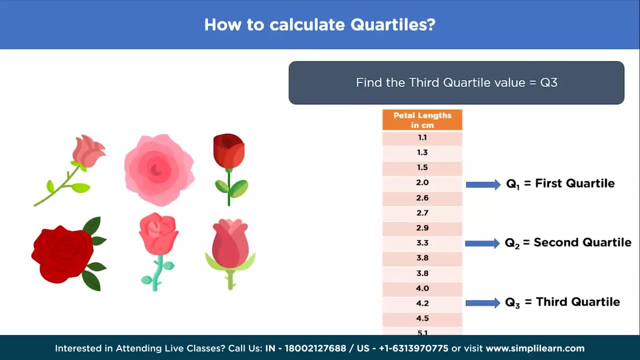 So we have our Q1, which is the first quartile- 2.0, Q2, the second quartile, which is also the median as 3.3, and we have the Q3 is equal to third quartile, which is 4.2.. 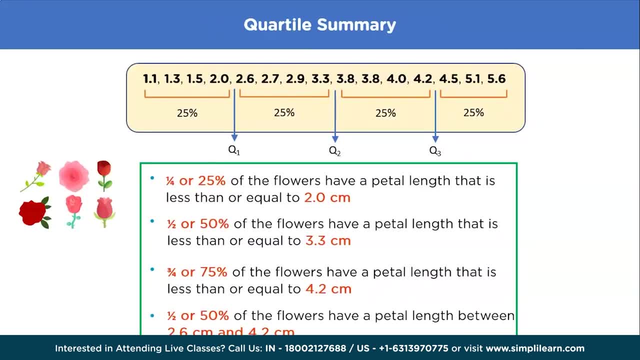 So what does this point signify? 1 by 4 or 25% of the flowers have a petal length that is less than or equal to 2.0.. 50% of the flowers have a petal length that is less than or equal to 2.0.. 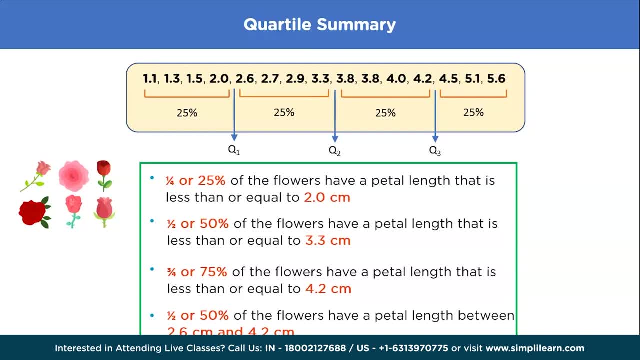 50% of the flowers have a petal length that is less than or equal to 2.0.. 50% of the flowers have a petal length that is less than or equal to 3.3 cm. 3 by 4. or 75% of the flowers have a petal length that is less than or equal to 4.2.. 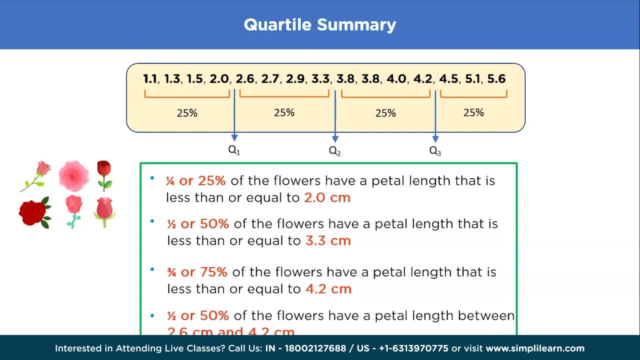 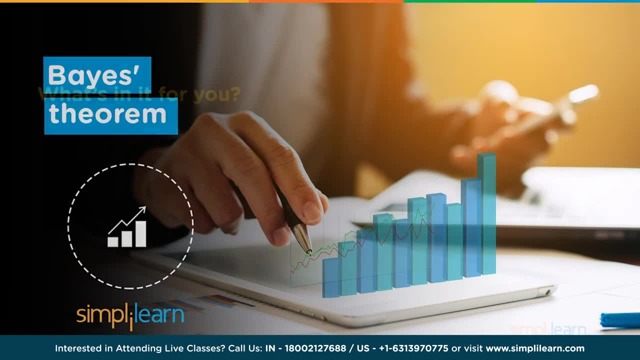 And half, which is also 50% of the flowers, have a petal length between 2.6 cm and 4.2 cm. Going to discuss the Bayes theorem, an important sub-topic that comes under Probability Theory, We'll start this video by talking about Probability and Conditional Probability. 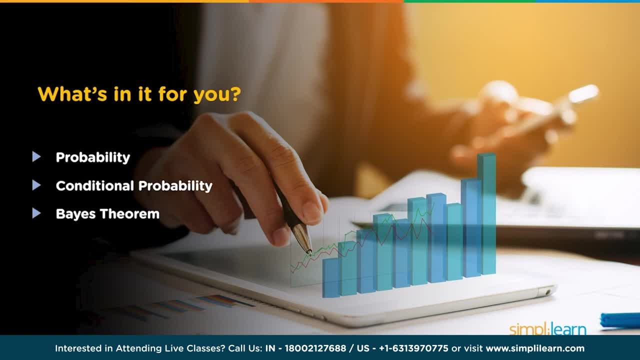 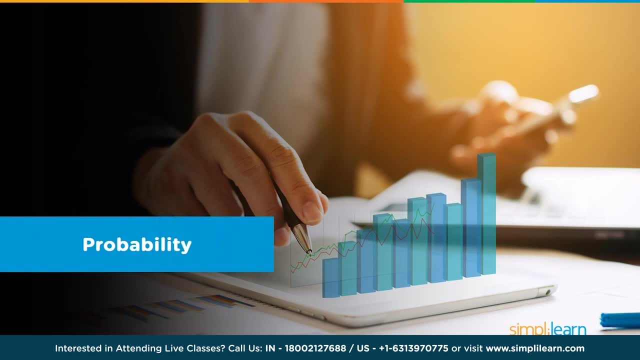 After that we'll move on to the Bayes theorem and understand its formula and understand how it works- real-life example where the base theorem can be used. So let's get started. What is probability? Probability is the branch of mathematics concerning 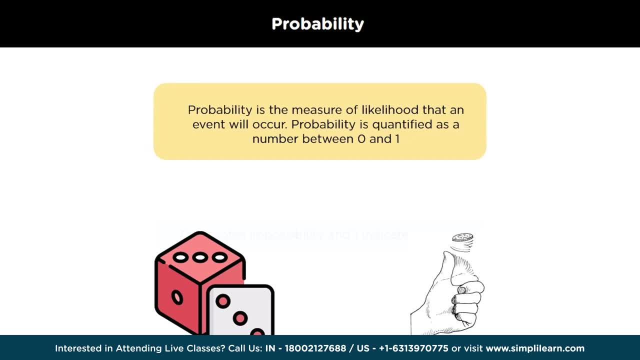 numerical descriptions of how likely an event is to occur or how likely it is that a proposition is true. The probability of an event is a number between 0 and 1, where, roughly speaking, 0 indicates the impossibility of the event and 1 indicates certainty. The higher the 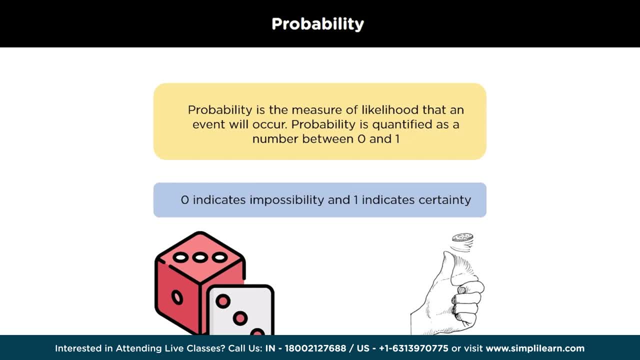 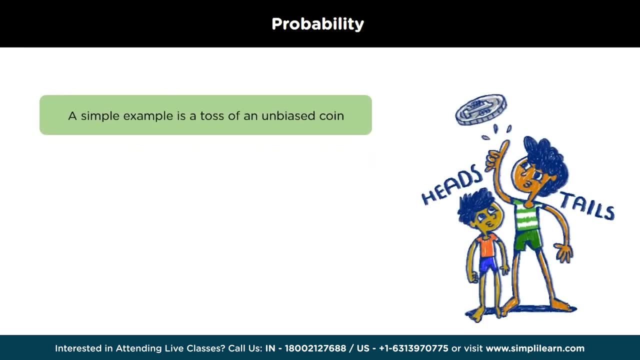 probability of an event, the more likely it is that the event will occur. Let's look at an example. A simple example is the tossing of a fair, unbiased coin. Since the coin is fair, the outcome, that is, heads and tails are both equally probable. The probability: 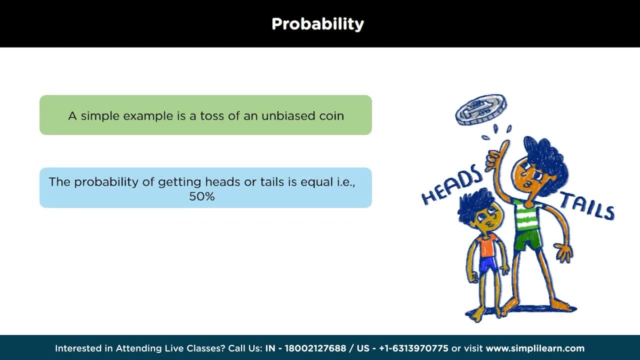 of heads equals the probability of tails and, since no other outcomes are possible, the probability of either heads or tails can be said to be 1 by 2, which is also 50%. The probability of an event can be calculated by supposing that the probability of head is equal to probability. 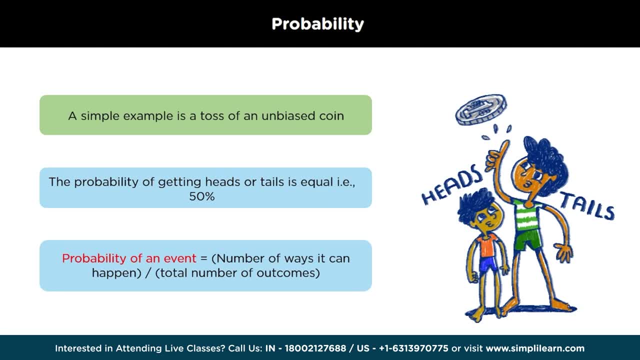 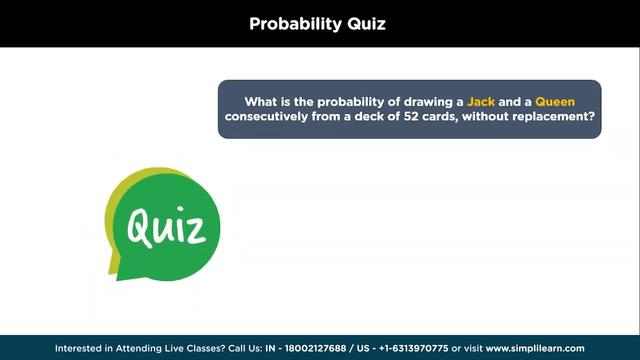 number of ways it can happen divided by the total number of outcomes. Now that we know about the probability, let's see if you can answer this question: What is the probability of drawing a jack and a queen consecutively from a deck of 52 cards without? 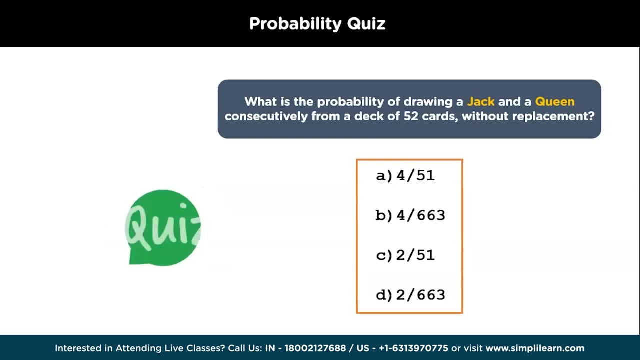 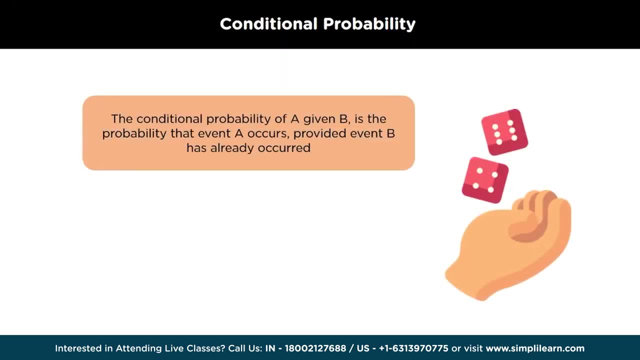 replacement. Here are your options: Post your answers in the comment section and let us know. Now let's move on to conditional probability. Let A and B be the two events associated with a random experiment. Then the probability of A's occurrence, under the condition that B has already occurred, and probability of B is not. 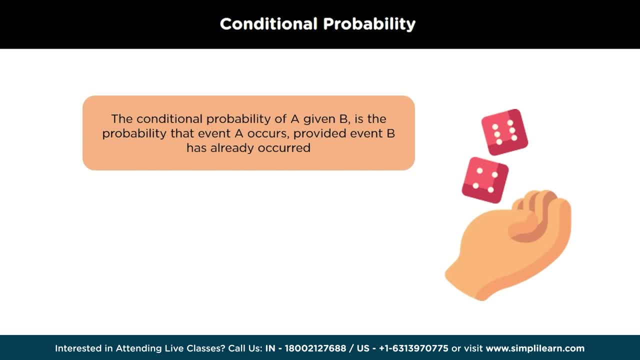 equal to zero is called the conditional probability. It is denoted by PA slash B. Thus, we can say that PA slash B is equal to PA intersection B divided by P of B, where PA slash B is the probability of occurrence of A, given that B has already occurred, and PB is the probability of occurrence of B. 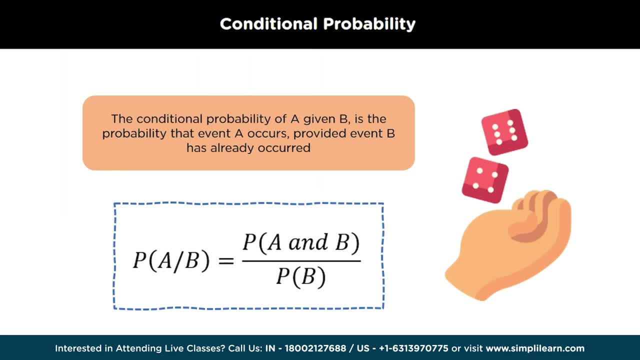 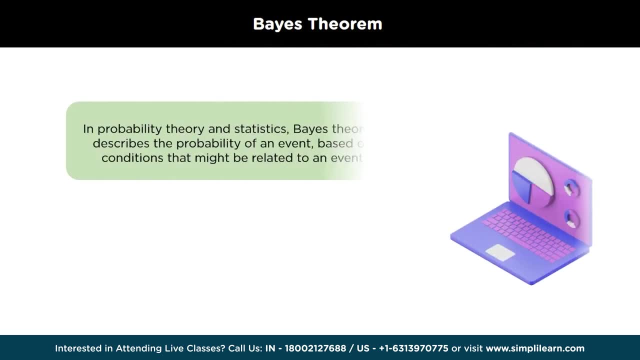 To know more about conditional probability, you can check our previous video, Which is specifically on conditional probability. Now let's move on to Bayes theorem. The Bayes theorem is the mathematical formula for calculating conditional probability in probability and statistics. In other words, it is used to figure out how likely an event is associated. 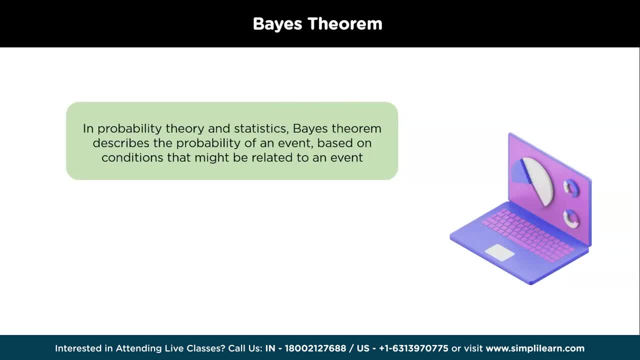 on its proximity to another. Bayes law or Bayes rule are the other names of this theorem. The formula for the Bayes theorem can be written in a variety of ways. The most common version is the Bayes rule. The most common version is PA. slash B is equal to P of B. slash A into P of A divided by P of B. 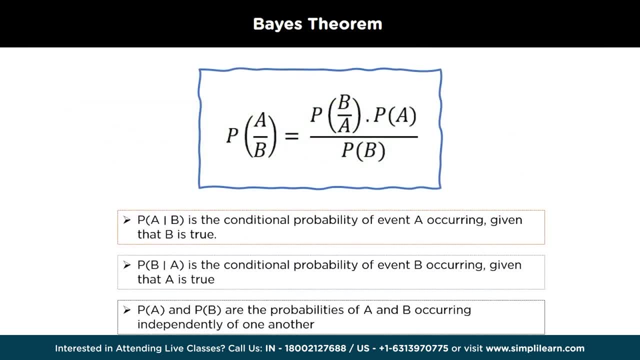 where PA slash B is the conditional probability of event A occurring. given that B is true and PA and P of B are the probabilities of A and B occurring independently of one another. Let's solve a problem using the Bayes theorem to understand it better. 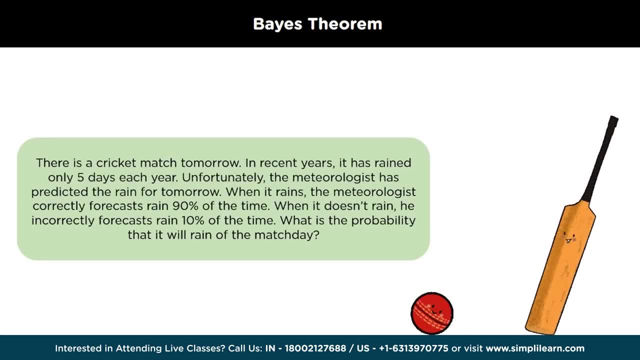 There is a cricket match tomorrow and in recent years, it has rained only five days each year. Unfortunately, there is no cricket match tomorrow And in recent years, it has rained only five days each year. Unfortunately, there is no cricket match tomorrow and in recent years, it has rained only five days each year. 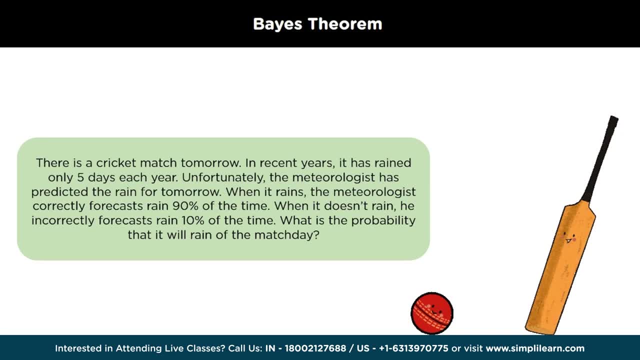 Unfortunately, the meteorologist has predicted the rain for tomorrow. Now, when it rains, the meteorologist correctly forecasts rain 90% of the time, And when it doesn't rain, he incorrectly forecasts rain 10% of the time. Let's calculate: what is the probability that it will rain on the match day. 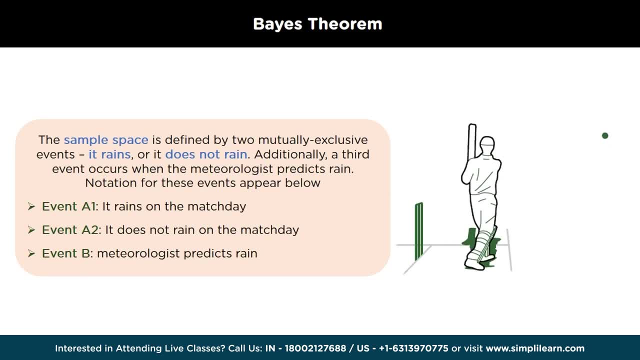 So the two sample spaces here are the events that it rains and it does not rain. Additionally, a third event is also there, that meteorologist predicts the rain. So the notation for these events appear below: Event A1 is equal to it rains on the match day. event A2, that it does not rain on the match day. 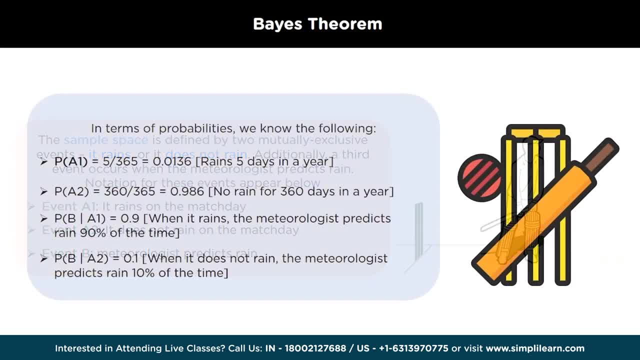 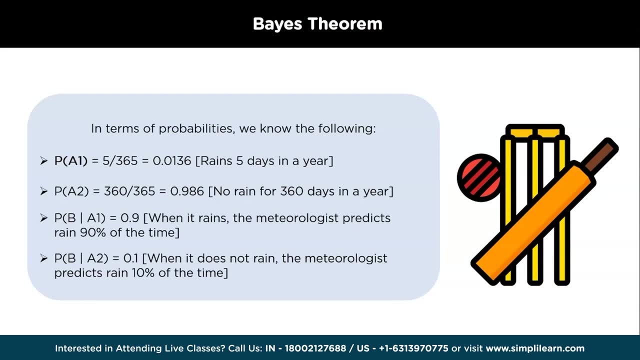 and event B is the meteorologist predicting the rain. Now, in terms of probability, we know the following: Probability of A1 is 5 by 365, that it rains 5 days in a year, which will come out to be 0.0136. 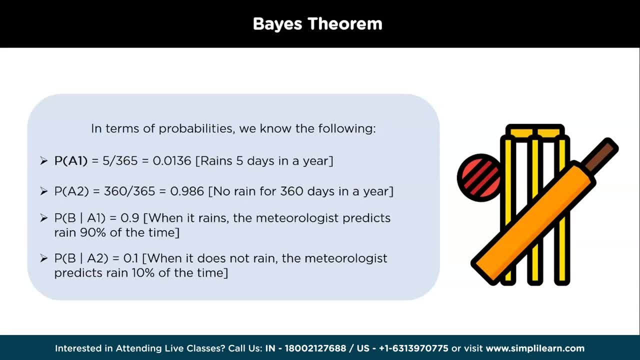 P is 360 by 365,, that is no days for 360 days in a year, which will come out to be 0.986.. P is 360 by 365, that is no days for 360 days in a year, which will come out to be 0.986., 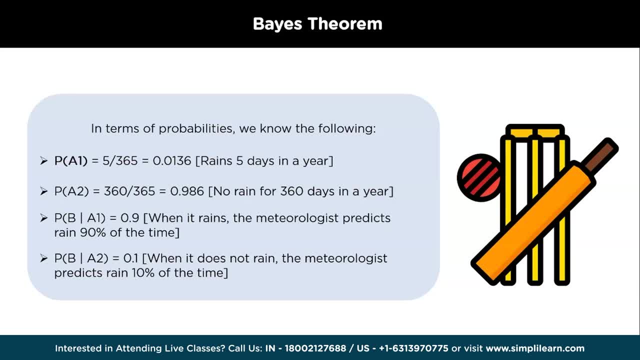 P is 360 by 365, that is, no days for 360 days in a year, which will come out to be 0.986.. P is 0.9.. This signifies when it rains, the meteorologist predicts the rain 90% of the time. 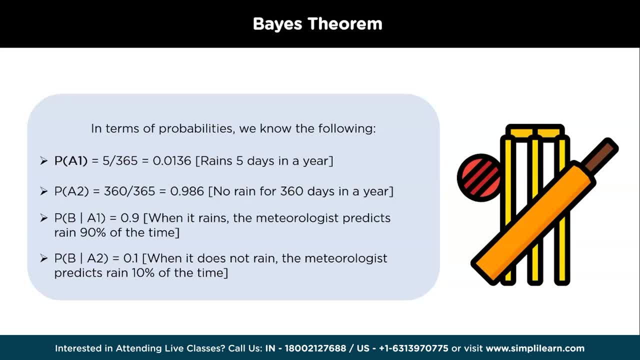 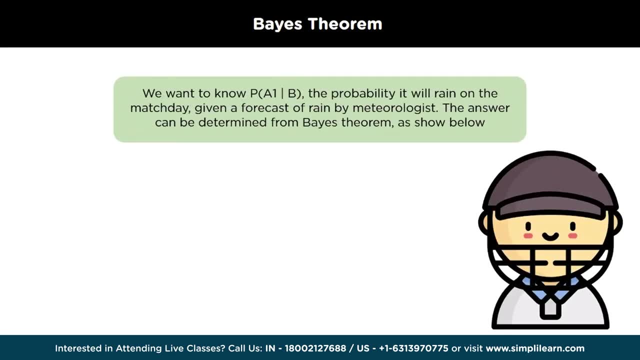 In a similar manner. P is 0.1, that it does not rain. the meteorologist predicts the rain 10% of the time. Combining all this we can calculate P. that is the probability it will rain on the given match day. 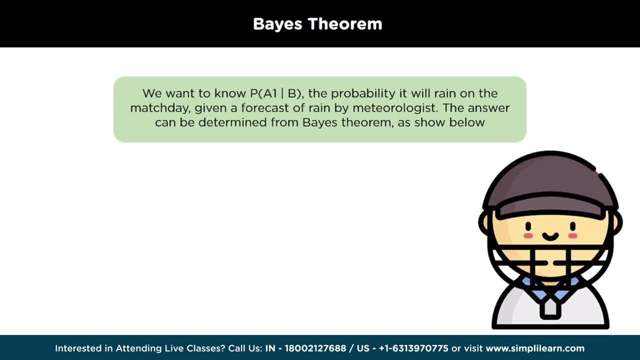 given a forecast of rain by meteorologist. The answer can be determined using the Bayes theorem, as shown below. So here is the formula of the Bayes theorem and, putting all the values that we have calculated in the previous slide, the probability that it will rain on the match day given a forecast of the rain by meteorologist will come out to be 0.111,. 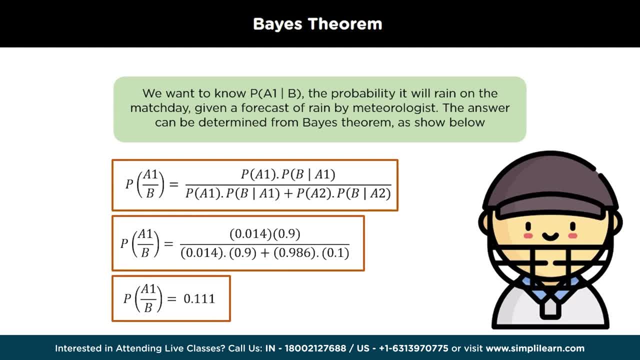 which will be equal to 11.11%. So there is an 11% chance that it will rain on the match day, given that the meteorologist has predicted the rain. I hope this example is clear to you. We will discuss a very widely used term in statistics, that is, confidence interval. 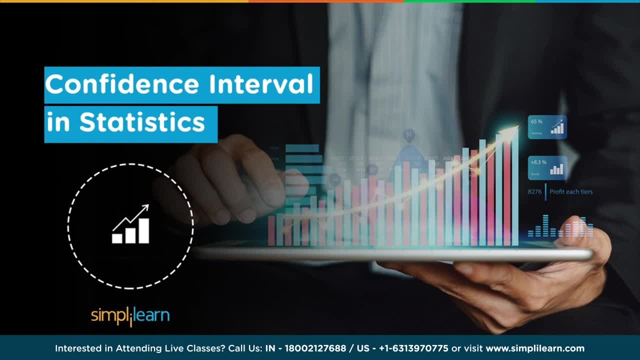 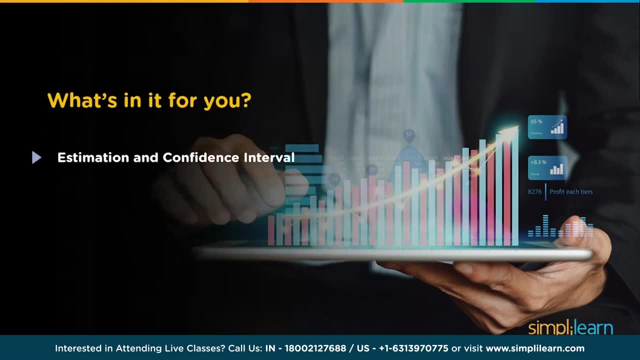 And we will see what is the significance of confidence interval and how to calculate it. So let's discuss the agenda for today's session. We will start this tutorial by understanding estimation and confidence intervals. Then we will move on to discuss the level of confidence. 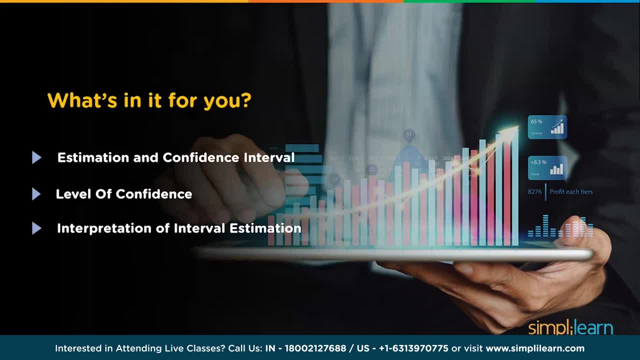 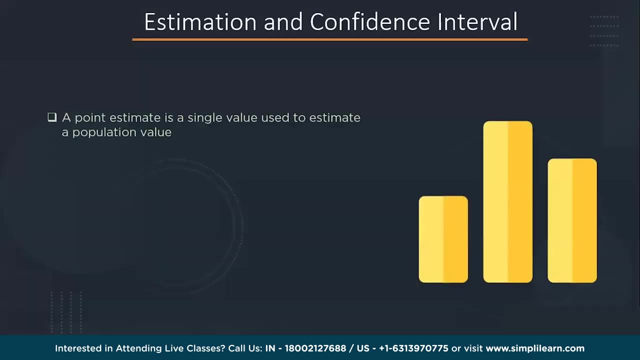 After that, we will discuss the importance of interval estimation and margin of error, And finally, we will learn how you can calculate confidence interval with the help of an example. So let's move further ahead: Estimation and Confidence Interval Using descriptive and inferential statistics. 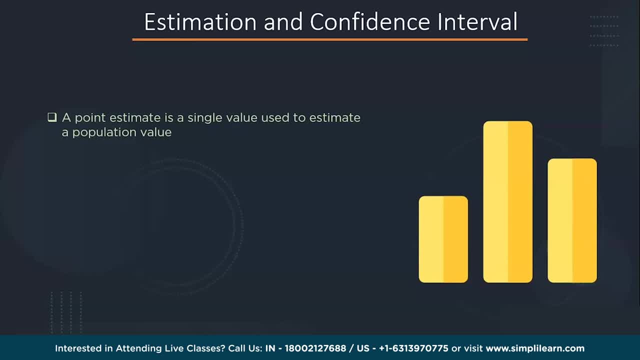 you can make two types of estimate about the population. One is point estimate and other is interval estimate. A point estimate is a single value estimate of a parameter. For instance, a sample mean is a point estimate of a population mean. An interval estimate gives you a range of values where 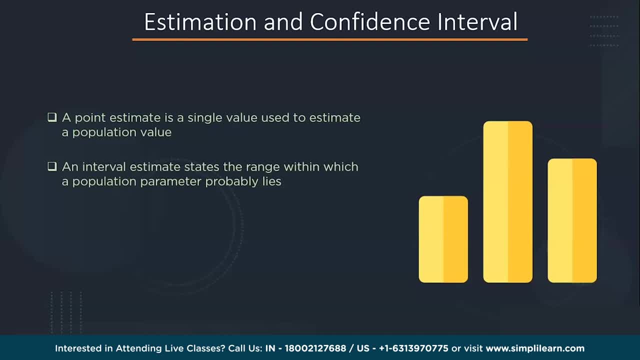 the parameter is expected to lie. A confidence interval is the most common type of interval estimate. Both the types of estimate are important for gathering a clear idea of where a parameter is likely to lie. The confidence interval is a range of values, It is expressed as a percentage and it is expected to contain the best estimate of a statistical parameter. 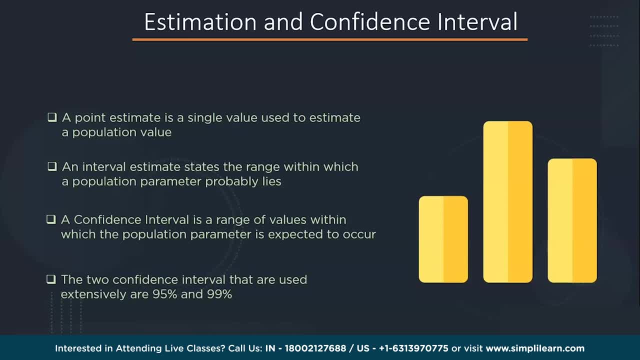 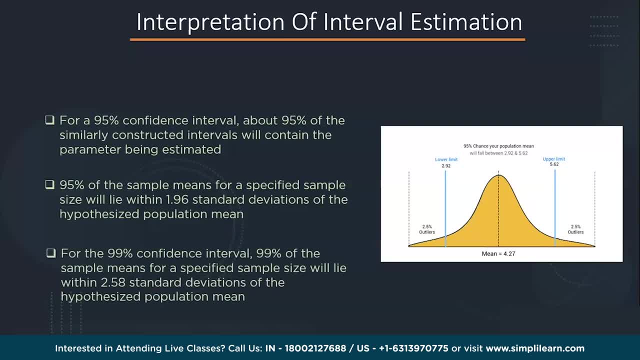 A confidence interval of 95% means that it is 95% certain that our population parameter lies in between this confidence interval. Similarly, for the 99% confidence interval, 99% of the sample means will lie within the 2.5 standard deviations from the population mean. 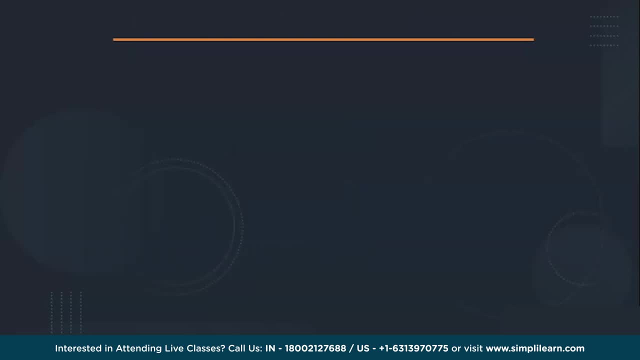 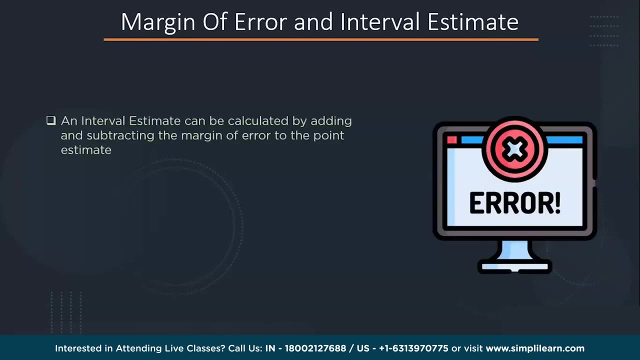 Now let's see how you can calculate the interval estimates. The interval estimate can be calculated by adding and subtracting the margin of error to the point estimate. It gives us the idea of how close the point estimate is to the value of parameter. The general form of the interval estimate is x-bar plus minus margin of error. 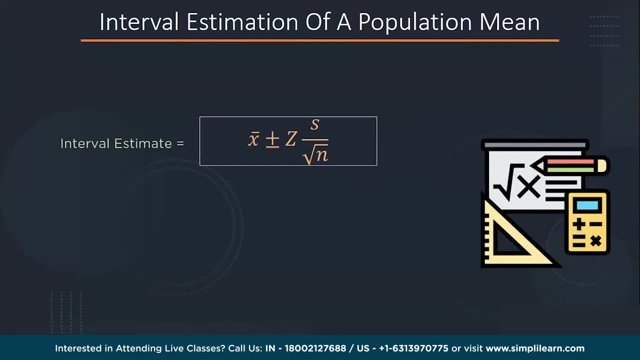 To calculate the interval estimate we have the formula x-bar plus minus z s, divided by root n, where x-bar is the sample mean, z is the number of standard deviations from the sample mean, s is the standard deviation and n is the size of the sample. 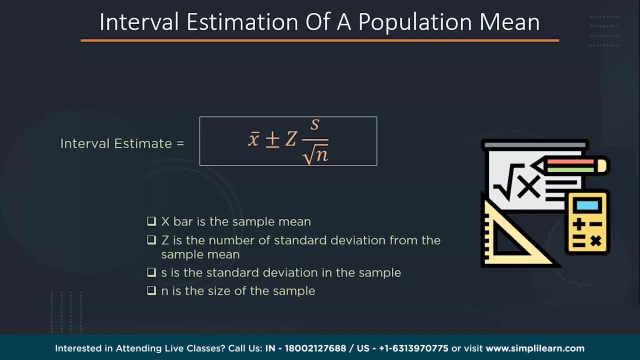 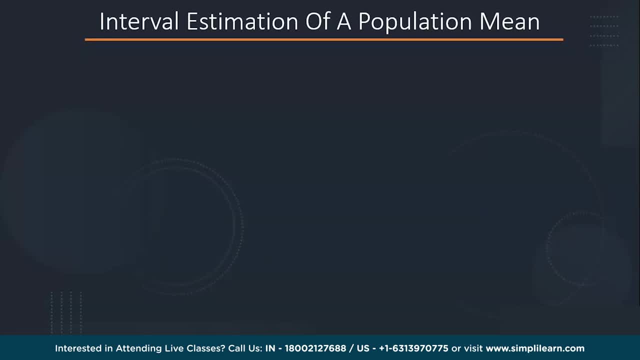 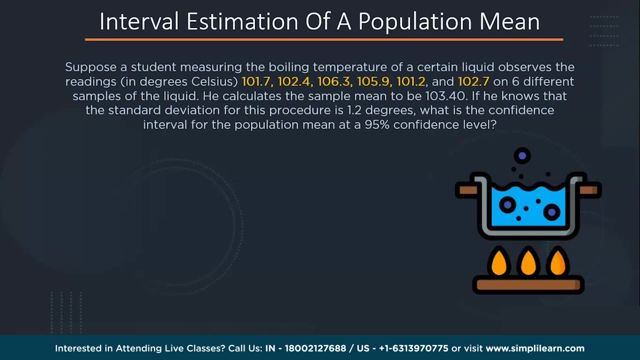 Now that we have discussed the interval estimate and the margin of error, let's understand all this concept with the help of an example. Suppose a student, measuring the boiling temperature of a certain liquid, observes the readings on 6 different samples of the liquid. He calculates the sample mean to be 103.4. and if he knows that the standard deviation 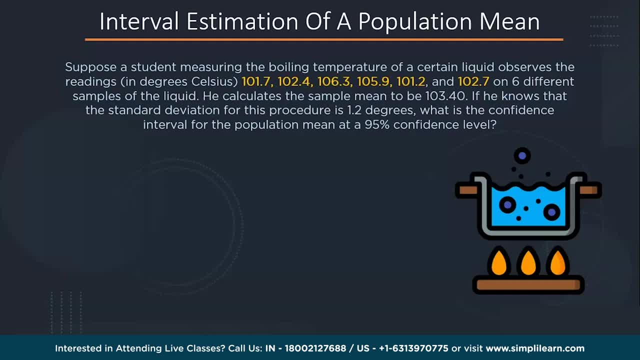 of this procedure is 1.2 degrees. we have to calculate the confidence interval of the population mean at a 95% confidence interval. So using this formula of interval estimate, x-bar plus minus z into s by root n, we will. 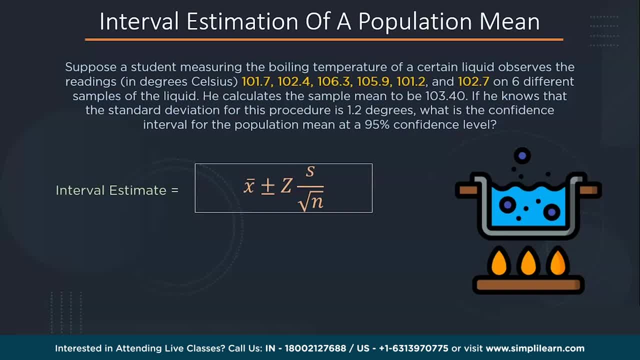 find the confidence interval Here, x-bar is 103.4 and z value is 1.96, corresponding to 95% confidence interval, and standard deviation is 1.2 divided by root 6, which is the sample size. So, calculating, we will get the value to be 102.47 and 104.33, which shows that it is 95%. 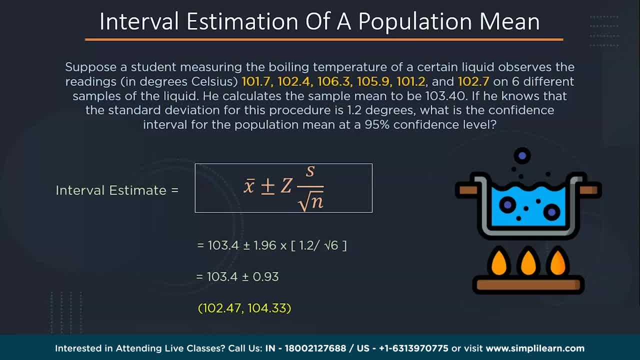 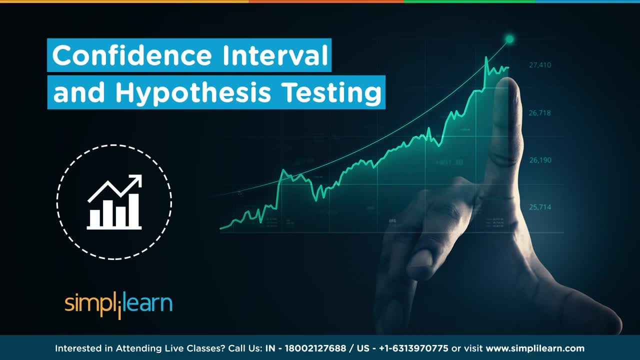 certainty. So let's calculate the confidence interval. We can see that the confidence interval is 2.6 degrees and the data population parameter lies between this confidence interval. Maths and statistics for data science are essential, because these topics form the basic foundation of all the machine learning algorithms. 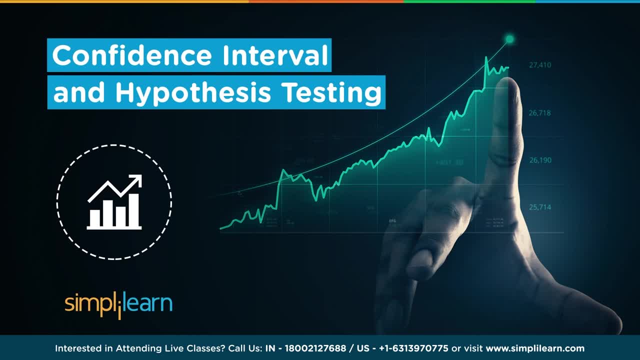 In fact, mathematics and statistics is behind everything from shapes, patterns, colors and algorithms. So today we will discuss two important topics of statistics, that is, confidence interval and hypothesis testing. We will discuss how to use it, when to use it and what are the advantages of using it. 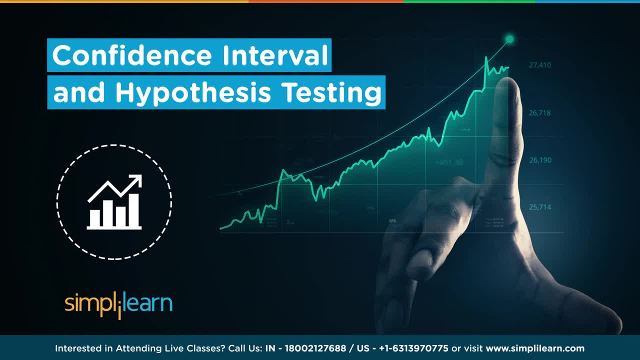 So let's start with the first topic: use it, when to use it, and the real life application of the same. But before we begin, if you haven't already subscribed to our channel, please do so so that you never miss an update. 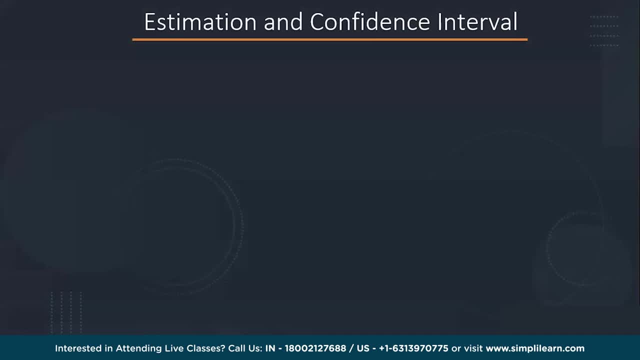 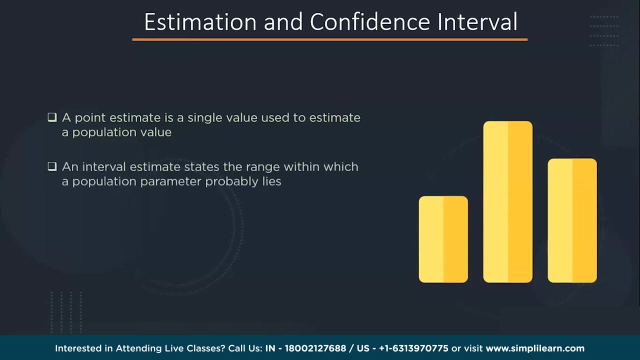 Let's move forward. Estimation and Confidence Interval. Using descriptive and inferential statistics, you can make two types of estimate about the population. One is point estimate and other is interval estimate. A point estimate is a single value estimate of a parameter. For instance, a sample mean is a point estimate of a population mean. 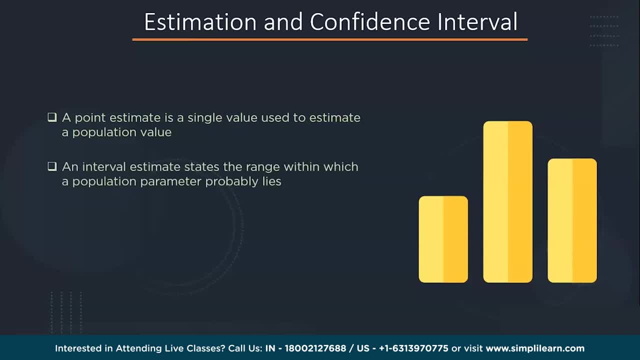 An interval estimate gives you a range of values where the parameter is expected to lie. A confidence interval is the most common type of interval estimate. Both the types of estimate are important for gathering a clear idea of where a parameter is likely to lie. The confidence interval is the range of values. 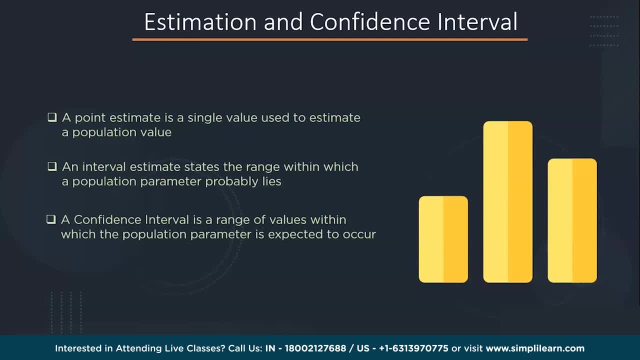 It is expressed as a percentage and it is expected to contain the best estimate of a statistical parameter. The two most frequently used confidence interval are 95% and 99%. A confidence interval of 95% mean that it is 95% certain that our population parameter. 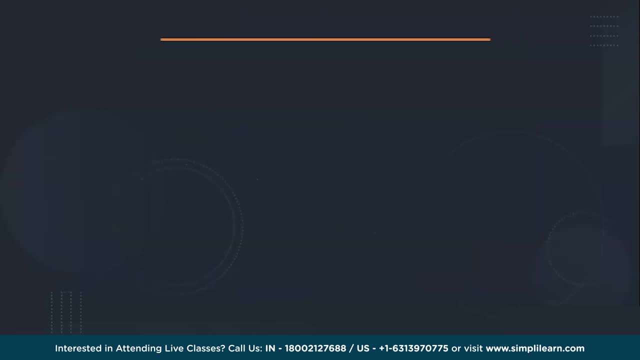 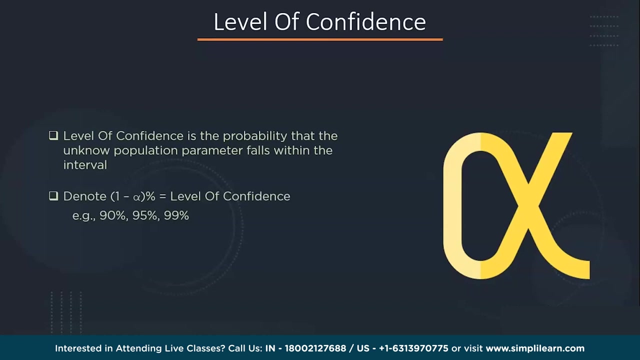 lies in between this confidence interval. Now, what is level of confidence With respect to estimation problems? alpha refers to the likelihood that a true population parameter lies outside the confidence interval. The level of confidence is denoted by 1-alpha, and it is usually 90%, 95% or 99%. 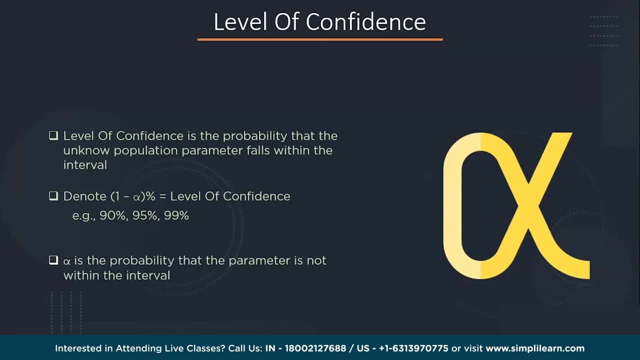 Alpha is usually expressed as a proportion. So if the confidence level is 95%, then alpha will be equal to 1-0.95, that is 0.05.. Now let's move on to discuss what this confidence interval is. Let's move on to discuss what this confidence interval is. 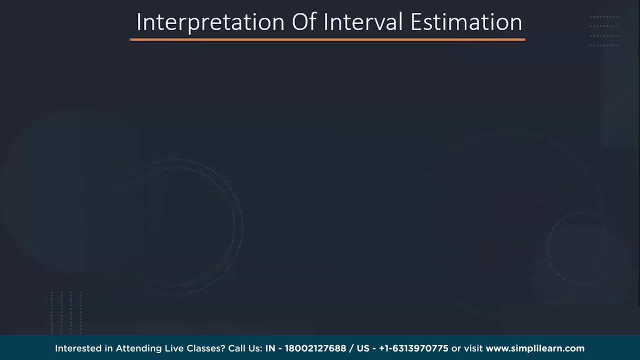 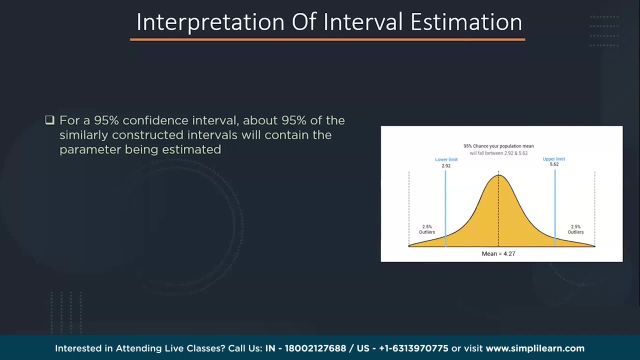 Now let's move on to discuss what this confidence interval is. A 95% confidence interval of the mean is a range with an upper and lower number calculated from a sample, Because the true population mean is unknown. this range describes the possible values that 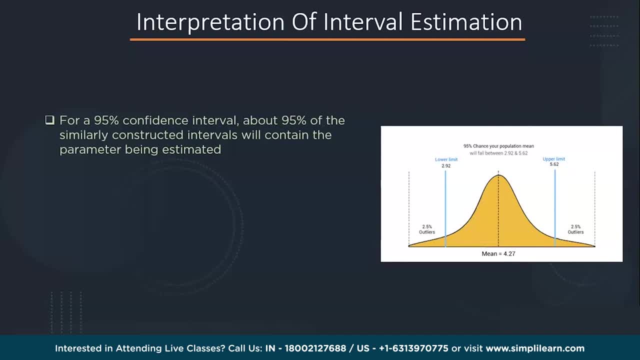 a mean could be If multiple samples are drawn from the same population and a 95% CI calculated for each sample. we would expect the population mean to be found within 95% of these confidence intervals. 95% of the sample means for a specific sample. 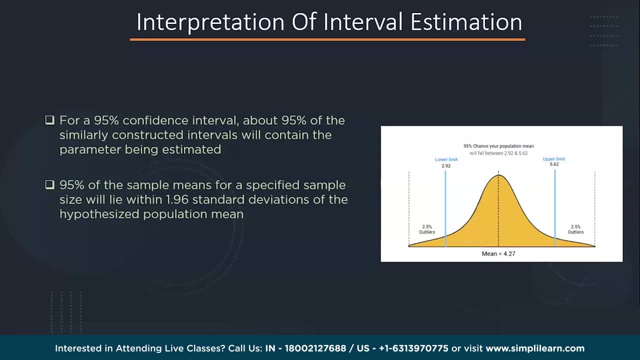 95% of the sample means for a specified sample size will lie within 1.96 standard deviations of the hypothesized population mean. Similarly, for 99% confidence interval, 99% of the sample means will lie within the 2.5s. 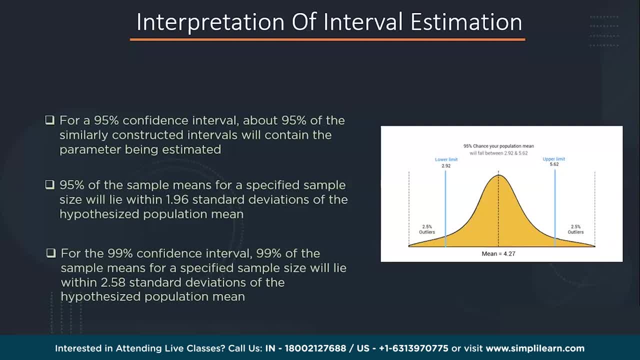 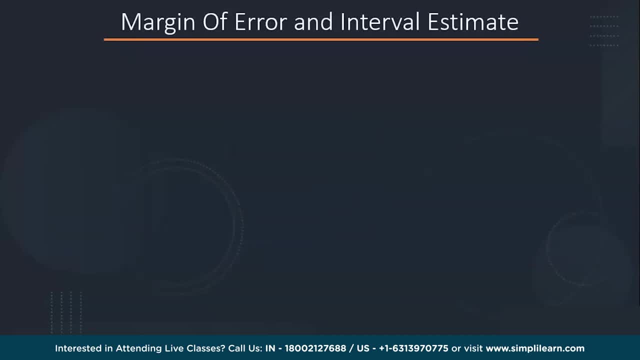 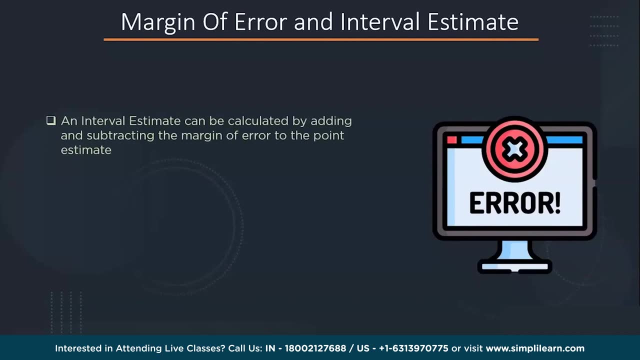 standard deviations from the population mean. Now let's see how you can calculate the interval estimates. The interval estimate can be calculated by adding and subtracting the margin of error to the point estimate. It gives us the idea of how close the point estimate is to the value of parameter. 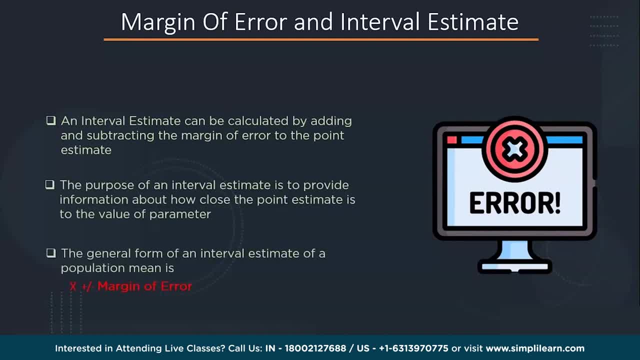 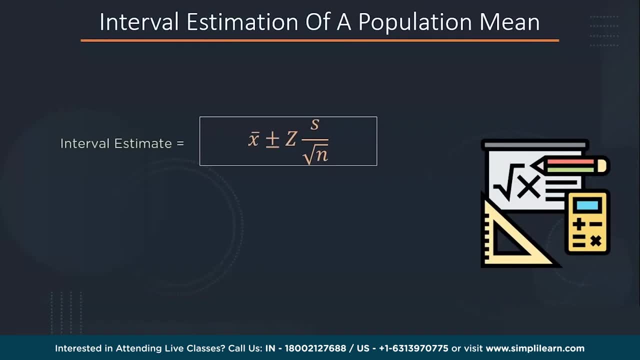 The general form of the interval estimate is x-bar plus minus margin of error. To calculate the interval estimate we have the formula x-bar plus minus z s divided by root n, Where x-bar is the sample mean, z is the number of standard deviations from the sample mean. 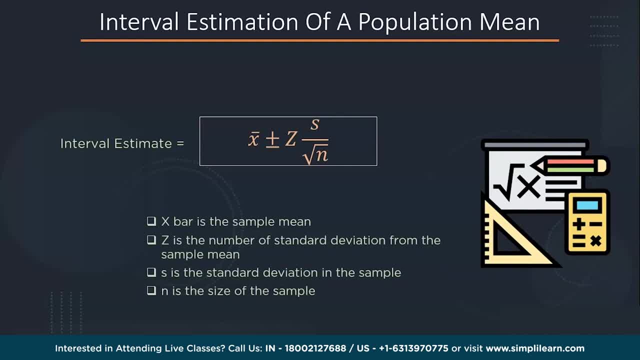 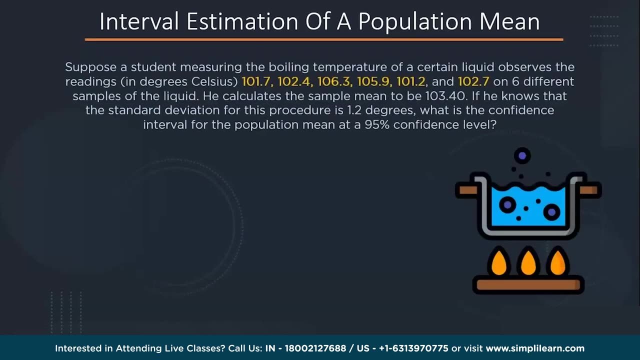 s is the standard deviation and n is the size of the sample. Now that we have discussed the interval estimate and the margin of error, let's understand all this concept with the help of an example. Suppose a student, measuring the boiling temperature of a certain liquid, observes the readings on: 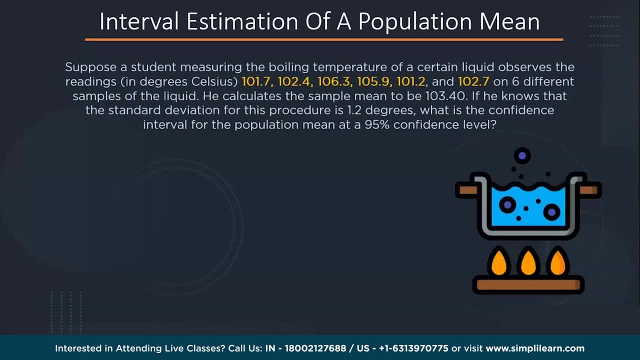 6 different samples of the liquid. He calculates the sample mean to be 103.4, and if he knows that the standard deviation of this procedure is 1.2 degrees, then he can calculate the sample mean to be 103.4.. 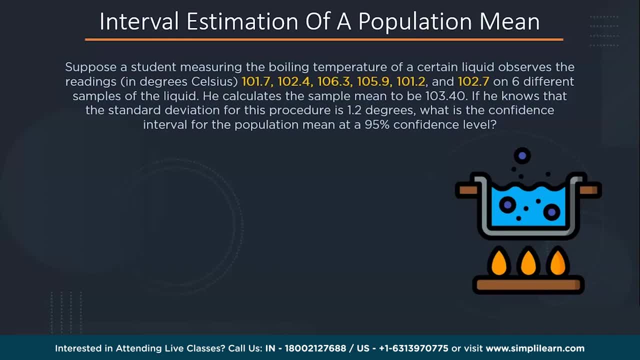 He can also calculate the standard deviation of the sample mean to be 103.4. and if he knows that the standard deviation of this procedure is 1.2 degrees, then he can calculate the sample mean to be 103.4.. We have to calculate the confidence interval of the population mean at a 95% confidence. 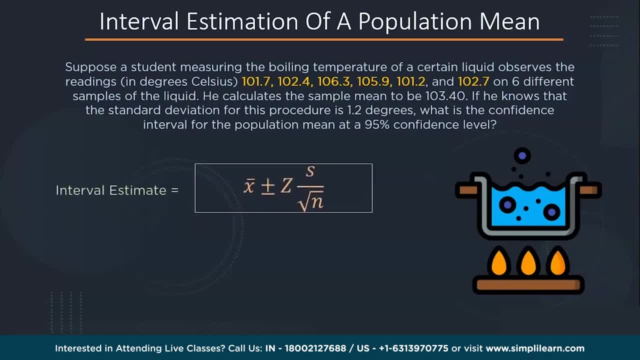 interval. So using this formula of interval estimate x-bar plus minus z into s by root n, we will find the confidence interval Here. x-bar is 103.4 and z value is 1.96, corresponding to 95% confidence interval and standard deviation. 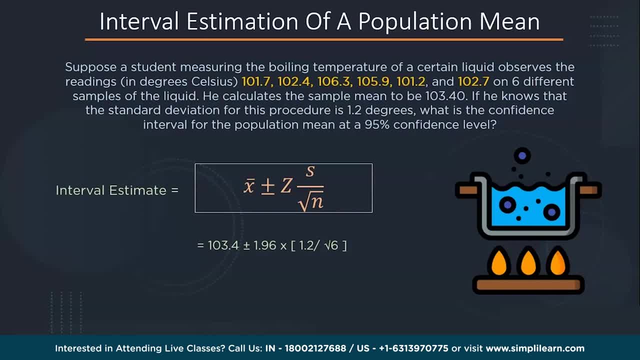 is 1.2 divided by root 6, which is the sample size. So, calculating, we will get the value to be 102.4.. So we have to calculate the confidence interval of the population mean at a 95% confidence interval, that is, 1.2 degrees to 2.47, and 104.3c which shows it is 95% certain that 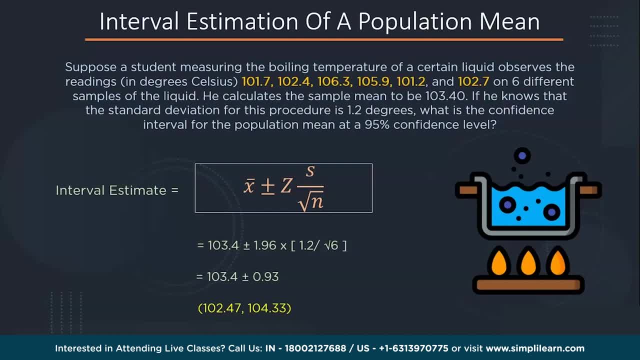 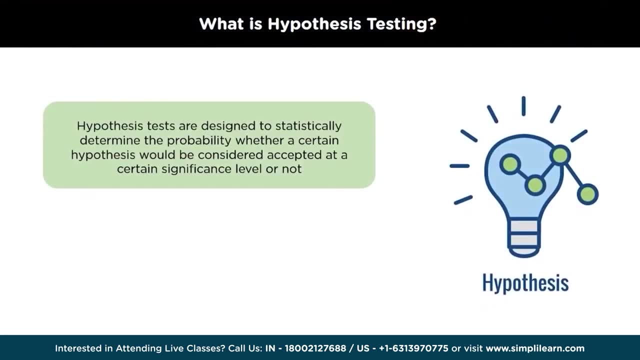 a population parameter lies between this confidence interval. What is Hypothesis Testing? Hypothesis testing or significance testing is the method for testing a claim or hypothesis about a parameter in a population using data measured in a sample. The purpose of the hypothesis testing is to check if there is enough statistical evidence. 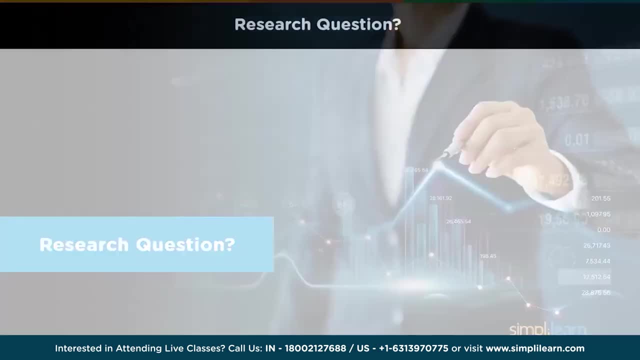 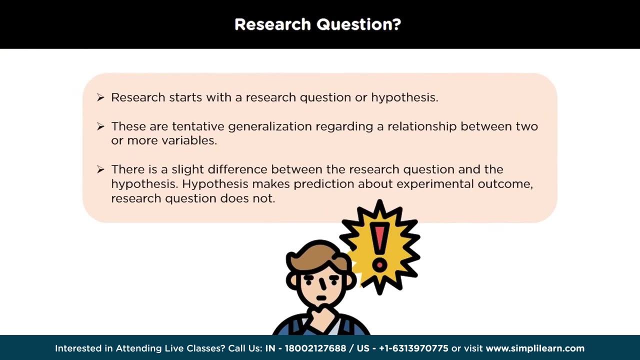 in a favour of a hypothesis on the parameters of the given population that we have came. Now we will move on to the research question. A research problem is a broad issue that you would like to address through your research. It identifies a difficult doubt or area. 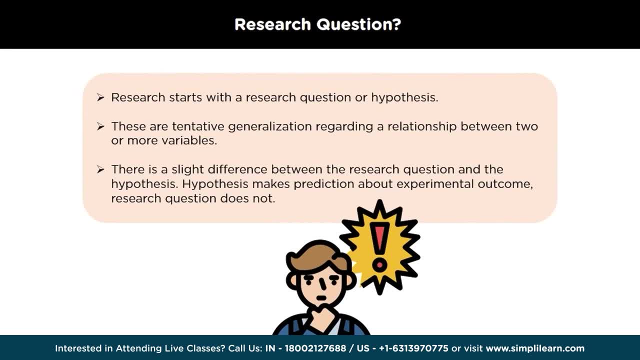 of concern in the theory or in practice. that requires thought and investigation. Research objectives are clear statements of what you aim to achieve through your research. There are specific actions that you will take and act as a milestone that will help you complete your research. A research question is a specific concern that you will answer through research. It is derived 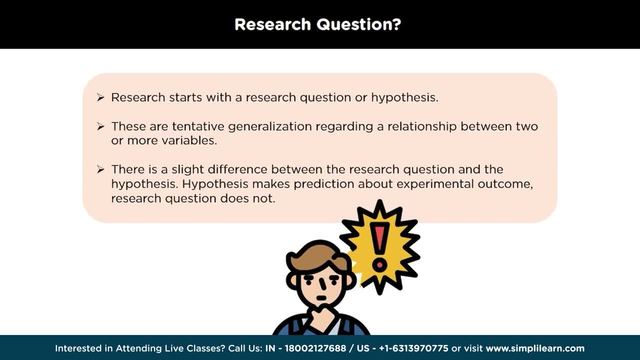 from a research problem but is based on a study design. When you narrow down on a research problem to a specific idea that points towards a feasible way to investigate or address your research problems, you will get your research question. Now, what you should really take care of is there. 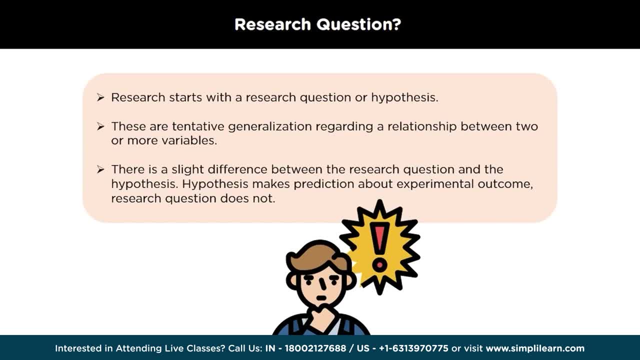 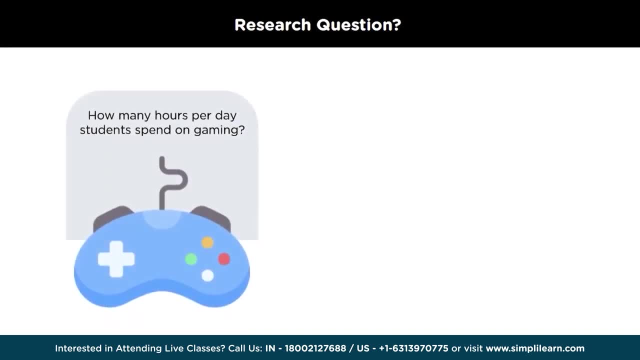 is a slight difference between a research question and a hypothesis. Hypothesis makes prediction about an experimental outcome, whereas research question doesn't. Let's understand with the help of an example. Suppose your research question is how many hours per day a student spends on a gaming and you want the answer for that. Another research question may. 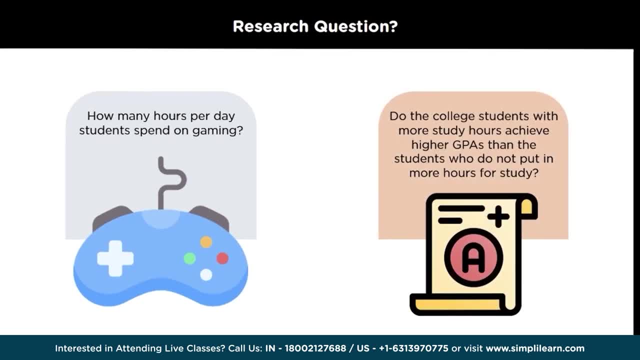 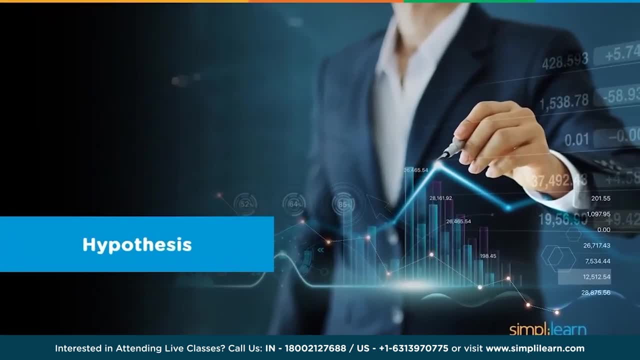 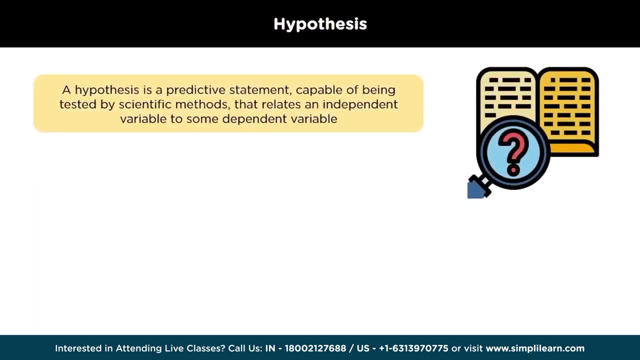 be. do the college students with more study hours can achieve a higher GPA than the students who do not put in more hours for study? These questions can be answered by framing a hypothesis. So let's understand what a hypothesis is. A hypothesis is a tentative statement about the results of a 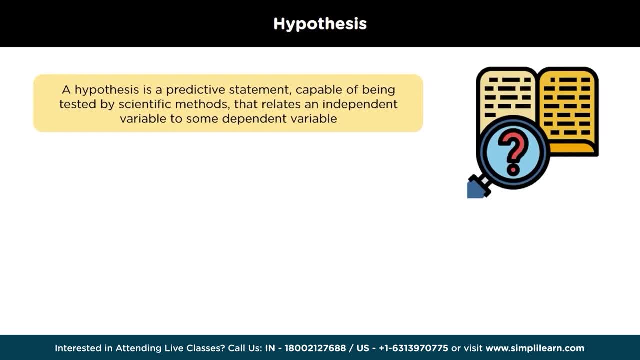 relationship between two or more variables. It is a specific, testable prediction about what you expect to happen in a study. The hypothesis is a prediction, but it involves more than a guess. Most of the time, a hypothesis begins with a question, which is then explored. 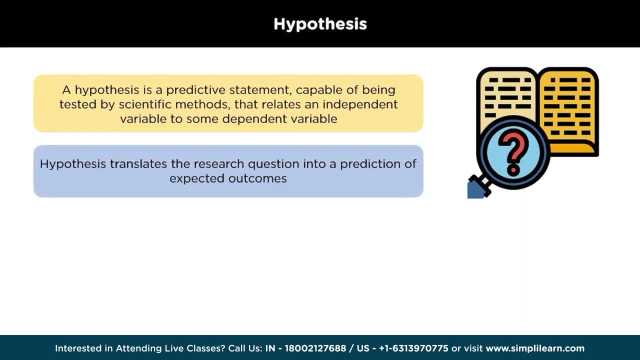 through a background research Hypothesis translates a research question into a prediction of expected outcomes. Unless you are creating an exploratory study, a hypothesis should always explain what you expect to happen. On the right side, we have framed a question that how many hours per day students spend on a gaming. 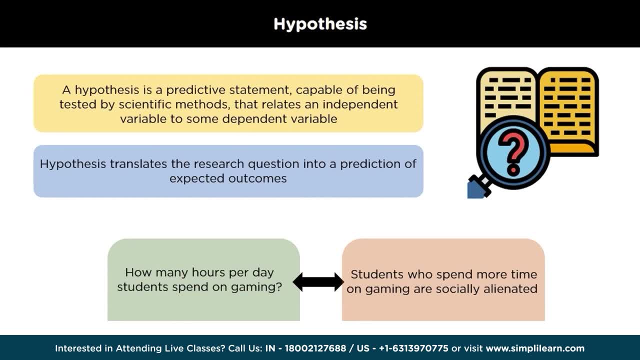 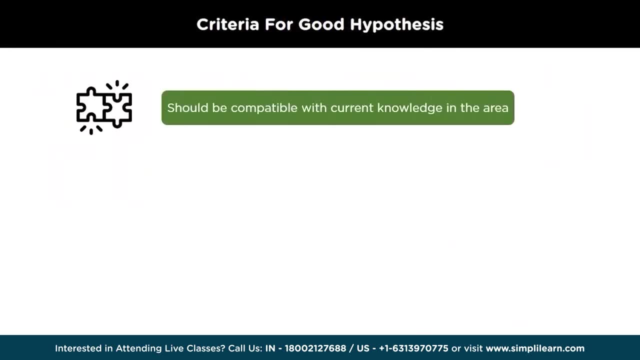 Relating to this question, we can create a hypothesis that students who spend more time on gaming are socially alienated. So there are some good criteria's for a good hypothesis. Let's discuss what are those. A hypothesis should be compatible with the current knowledge in the area and it should follow the 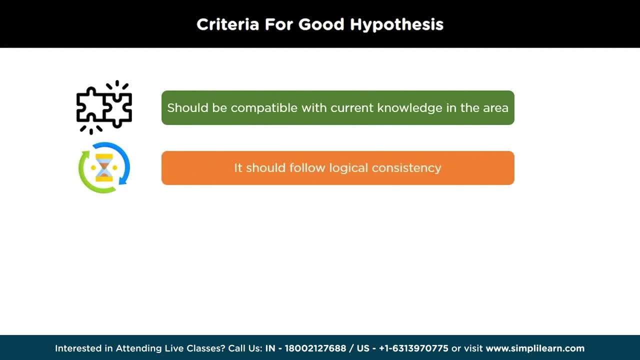 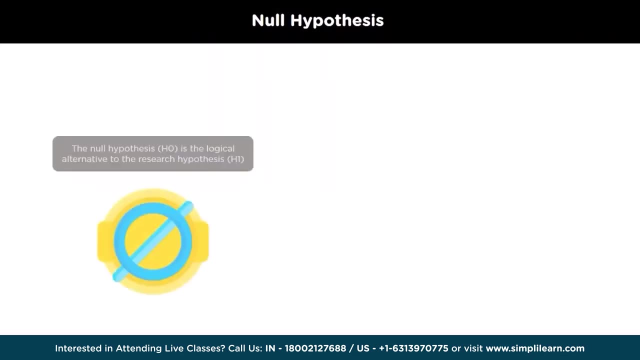 logical consistency. It should not be inconsistent in places. A good hypothesis must be shaded briefly and clearly And it should be testable. Now we will understand what a null hypothesis and alternative hypothesis is. The null hypothesis is the assumption that an event will not occur. 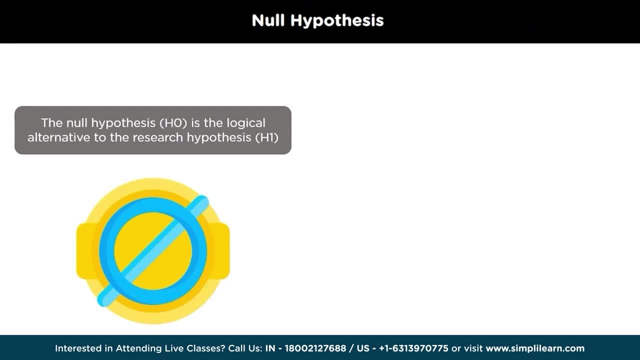 A null hypothesis has no bearing on the study's outcome unless it is rejected. H0 is a symbol for null hypothesis. The alternative hypothesis or a research hypothesis is a logical opposite of the null hypothesis. The acceptance of the alternative hypothesis follows the rejection of the null hypothesis. Let's understand the null hypothesis with the help of an example. 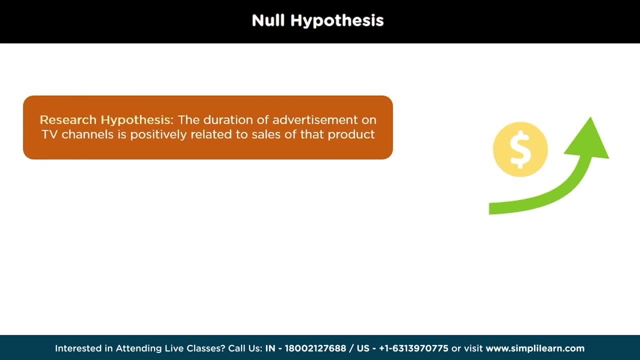 Suppose you have a research hypothesis that the duration of an advertisement on the TV channels is positively related to the sales of the product. The more the duration, the more the sales of that product. So the null hypothesis of this assumption would be that the duration of the advertisement on the TV channels are not related to the sales of the 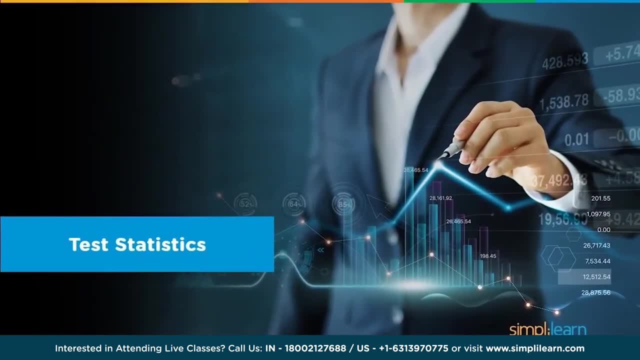 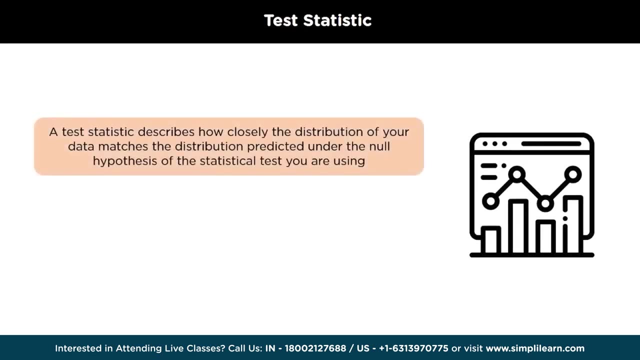 product. They are not related at all. Now we will move on to the test statistics that I explained. Test statistics is a number calculated from the statistical test of a hypothesis. It shows how closely your observed data matches the distribution expected under the null hypothesis. 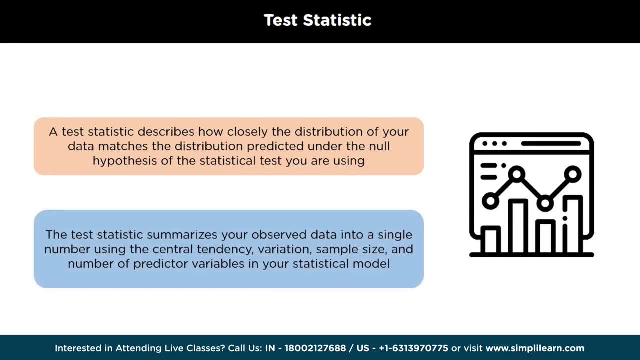 of data statistical test. The distribution of the data is how often each observation occurs and can be described by its central tendency and variation around the central tendencies. The test statistics summarizes your observed data into a single number using the null hypothesis testing. The test statistics summarizes your observed data into a single. 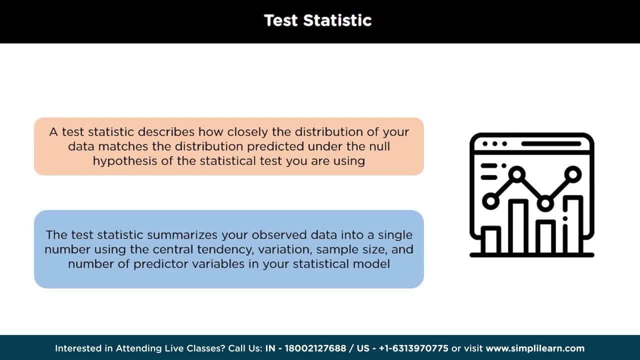 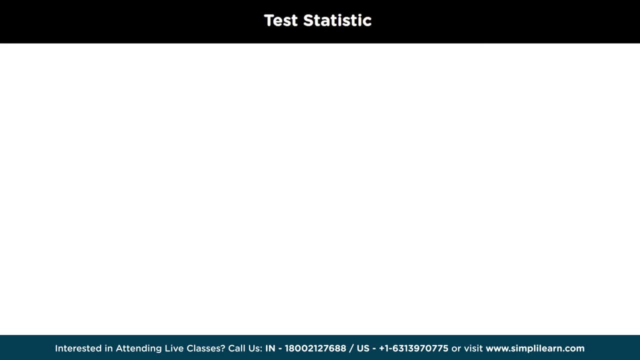 number using the null hypothesis test, שמ�lig, tendency, variation, sample size and the other number of predictable variables in a statistical model. They are broadly 3 steps of statistical test. Different statistical tests have slightly different ways of calculating these test statistics, but the underlying hypothesis and interpretation of the test. 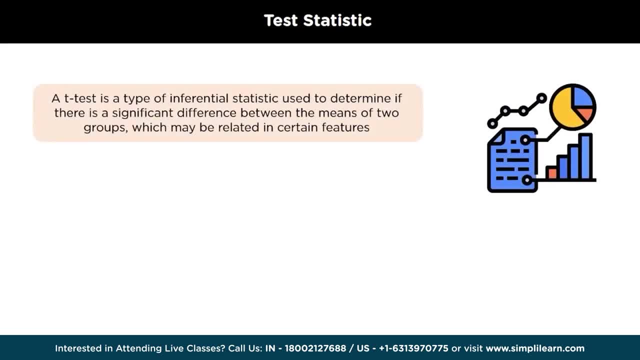 statistics stay the same. The first one is a t-test. A t-test is a statistical test that is used to compare the means of two groups. It is often used in hypothesis testing. klede: multiply how many toasts are found, or zero is common. The teenagers at least 20%. The average rate of 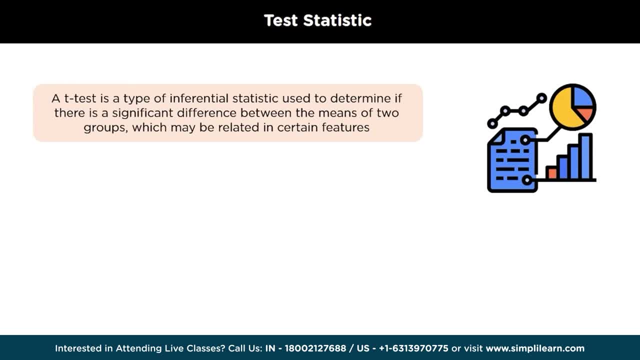 whether a process or treatment actually has an effect on the population of interest or whether the two groups are different from one another. The null hypothesis is that the true difference between these group means is zero, and the alternative hypothesis is that the true difference is different from zero. 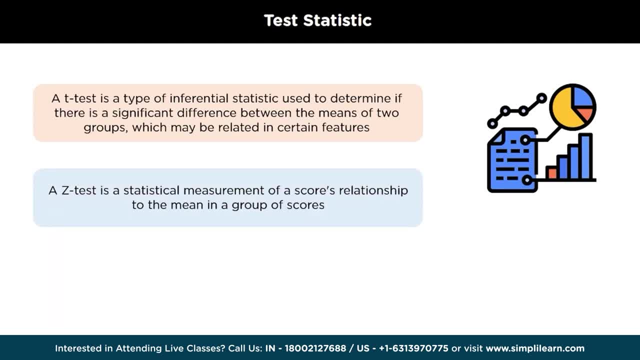 Now let's move on to Z tests. Z tests are a statistical way of testing a hypothesis: that either we know the population variance or we don't know the population variance, but our sample size is greater than 30. We perform the Z test when we want to compare a sample mean with the population mean. 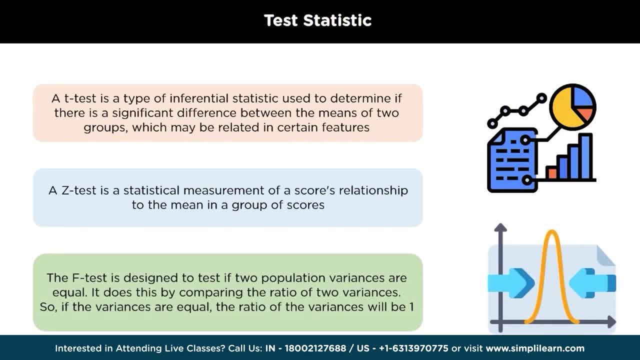 The next is an F test. The F test, or the F statistics, is simply a ratio of two variances. Variances are the measure of dispersion, or how far the data are scattered from the mean. Larger values represent the greater dispersion. Despite being a ratio of variances, you can use the F test in a wide variety of situations. 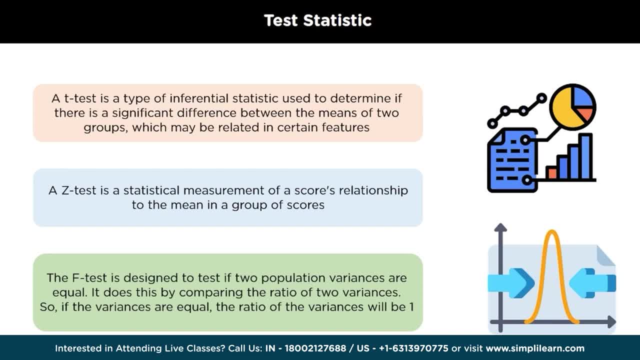 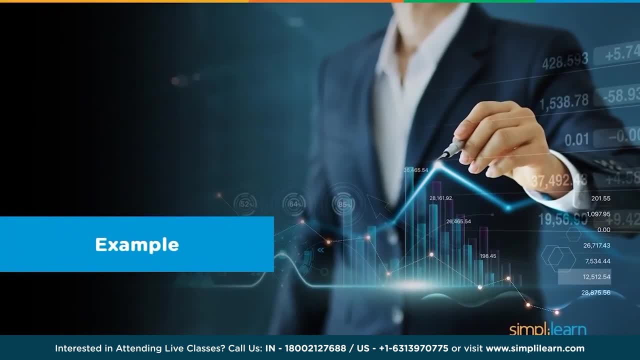 F test can assess the equality of variances. However, by changing the variances that are included in the ratio, the F test becomes a very flexible test. Now that we have discussed all the theories related to the hypothesis testing, let's take an example to understand them more clearly. 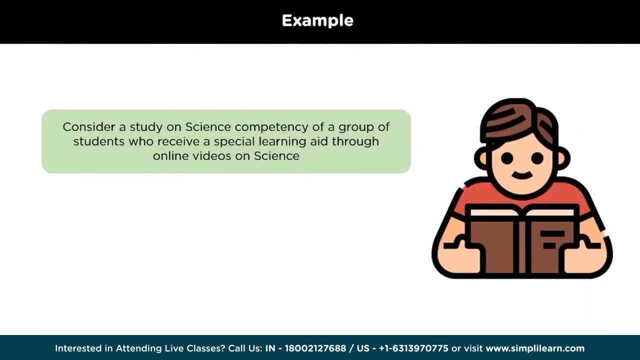 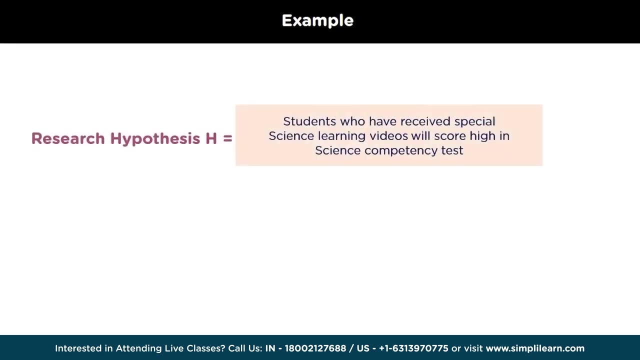 Consider a study on a group of students where the students receive a special learning aid through the online videos on science. It is hypothesized that after viewing this online video, the group of students score better than the one who have not seen the videos. So in this case, 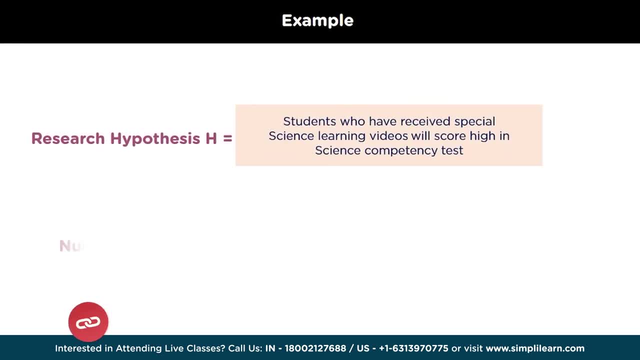 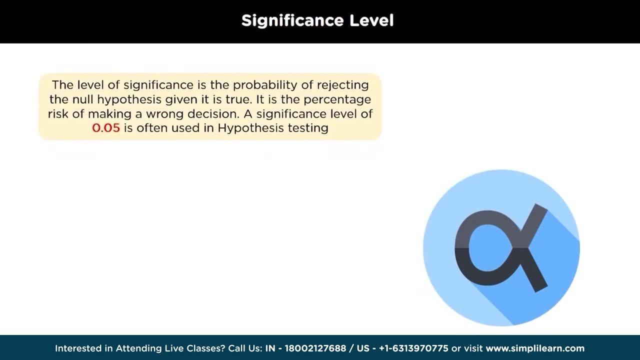 the research hypothesis will be students who have received the special science learning videos will score higher in the science competency test, And its null hypothesis will be: the special science learning videos made no impact on the scores of the students. Now we will discuss what a significance level is. 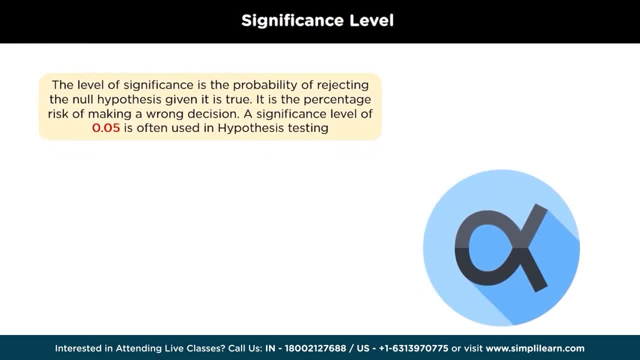 Level of significance, or significance level, refers to a criterion of judgment upon which a decision is made regarding the value stated in the null hypothesis. This criteria is based on the probability of the result. This is based on the probability of obtaining a statistic measured in a sample. 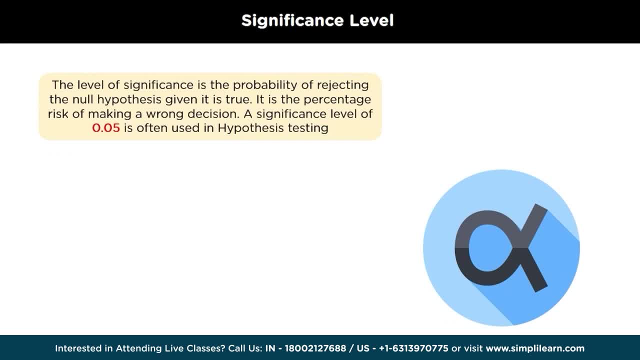 if the values stated in the null hypothesis were true. Generally, the criterion of the level of significance is typically set at 5% or 0.05.. This value of significance level can also be taken as 1% or 10%, depending upon your requirement. 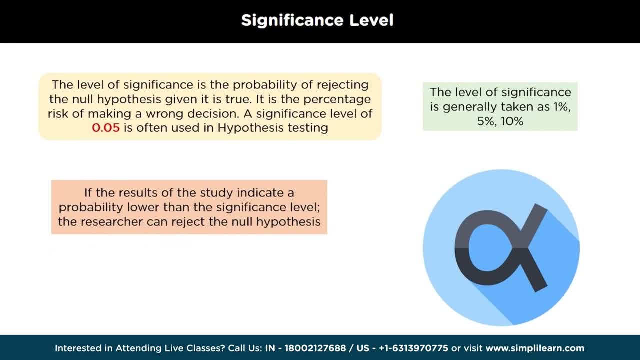 If the result obtained from the study indicates a probability lower than the significance level, so in this case a researcher can reject a null hypothesis. Otherwise, if the result of the study indicates a probability higher than the significance level, the researcher can support the null hypothesis. 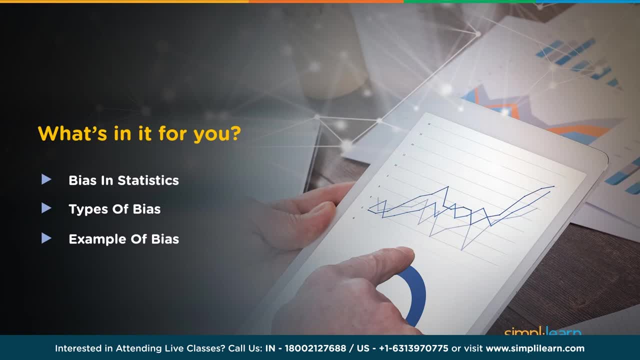 We will start the discussion by discussing what is bias in statistics and some examples and reasons for the same. Then we will move on to discuss what is types of biases and the examples to understand these types better. So, without further delay, let's begin. 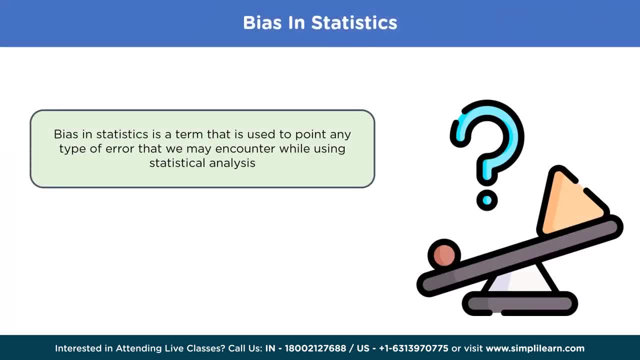 What is bias in statistics? Bias in statistics is a term that is used to refer any type of error that we may find when we use the statistical analysis. We can say that it is an estimator of a parameter that may not be confusing with its degree of precision. 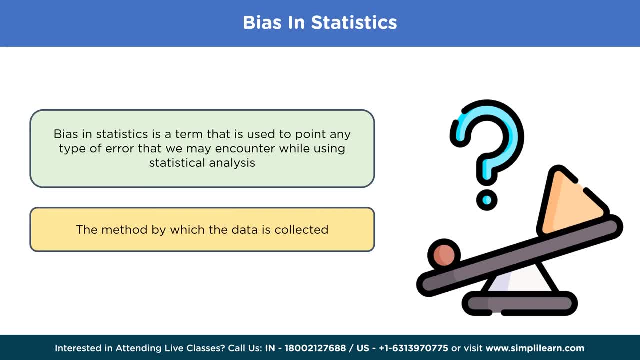 The reasons for this bias may be that the method by which the data is collected may be faulty, or the way the question is phrased may be not accurate. Let's see what are the types of biases. The first one is the measurement bias. 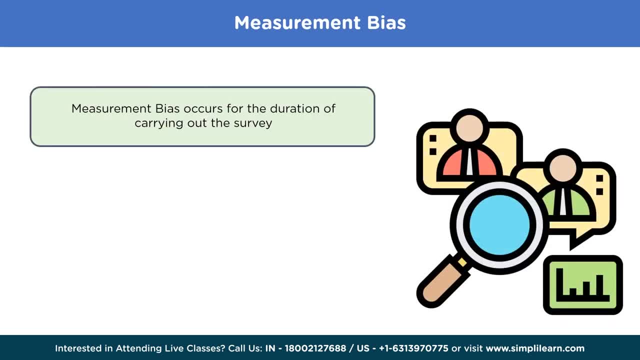 Measurement bias refers to any systematic or non-random error type that occurs in the collection of data in a study. Another term that is used for this type of bias is the detection bias. This difference in observation might be because of unseen reasons. Some of them can be the error that happens while recording the data or the leading questions that follows after the data. 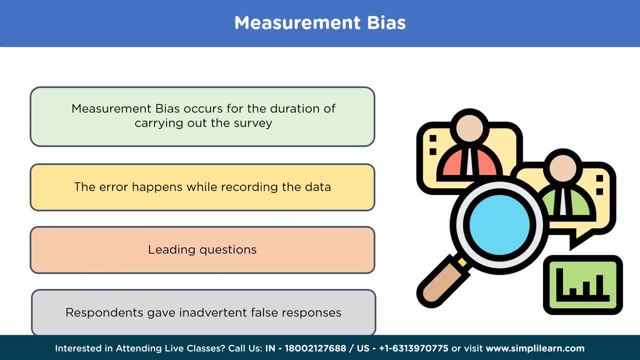 The error can also occur because the respondents gave the false answers. Suppose you conduct a survey to determine whether or not someone voted for President Obama. Some may have voted for him, but the way the question was put confused the respondents and they answered wrong. In this case, the measurement bias can occur. 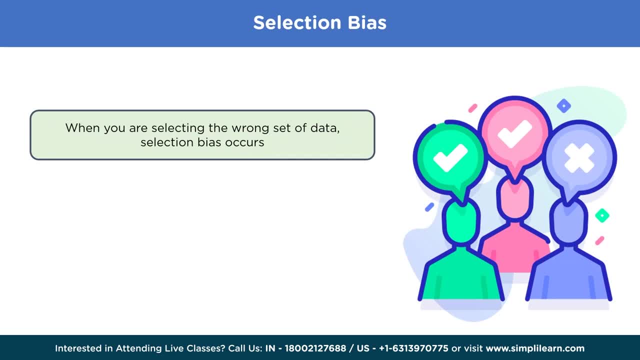 The next type of bias is the selection bias. When you choose your sample or data incorrectly, selection bias occurs. There can be many reasons for this, but the most common reason is when the people try to work with the data that are easily available And 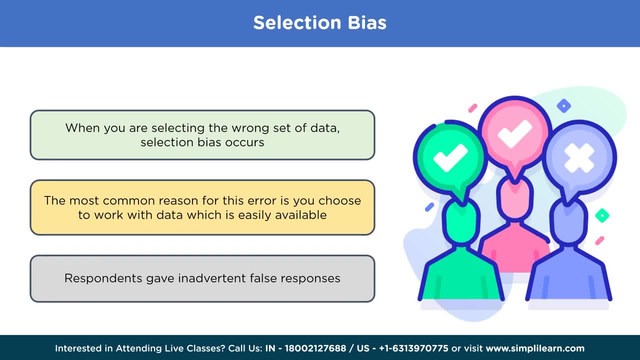 because of that, the respondents gave the false response. Let's try to understand this concept with the help of an example. Suppose you are conducting a poll to determine how people feel about the current ruling government. You have gathered all the information that you need. 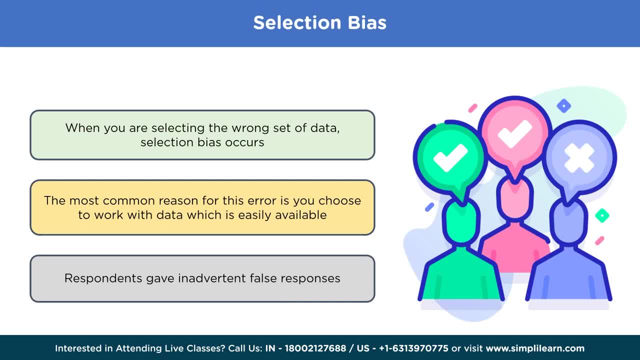 Unfortunately, many of them say that Twitter is the primary source for the information. Now, social media is not considered trustworthy because it is in public opinion, but their friends' opinion. As a result, this type of data can be classified as a traditional selection bias. 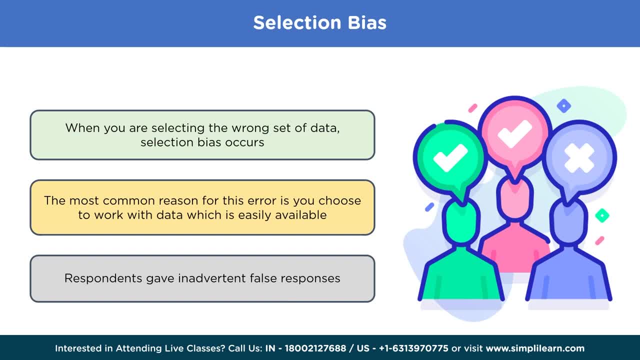 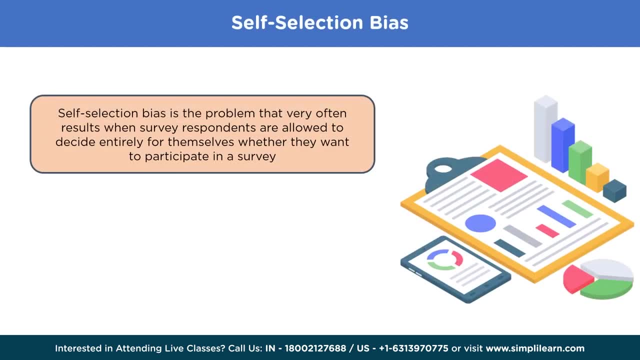 Easily accessible, but not for unrepresentative and specific subsets of the overall population. The next type of bias is the self-selection bias. Self-selection bias occurs when the respondents are allowed to decide entirely for themselves whether they want to participate in the survey or not. 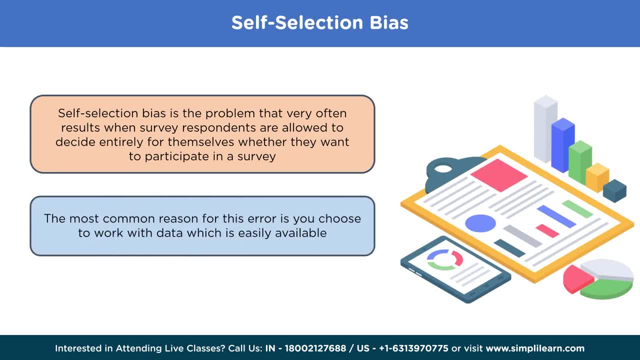 The reasons for this error may be same, that the data may be collected which are easily available. Let's try to understand this type of bias with the help of an example. Suppose you want to assess a program for improving the eating habits of the shift workers. 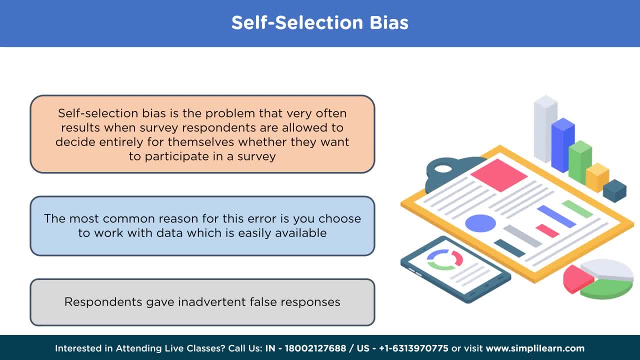 You put up posters where many workers nice shifts and invite them to participate. However, those who sign up may be different from those who don't. They may be more health conscious to be with, which is why they are interested in a program for improving eating habits. 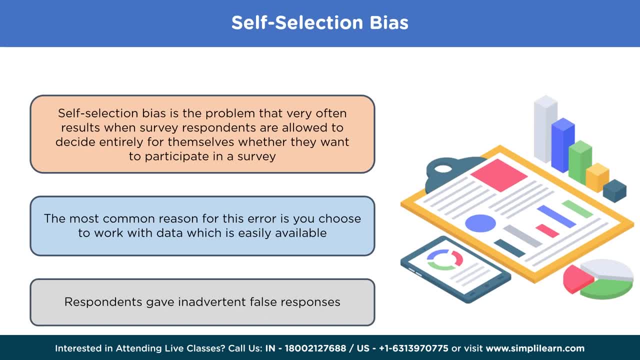 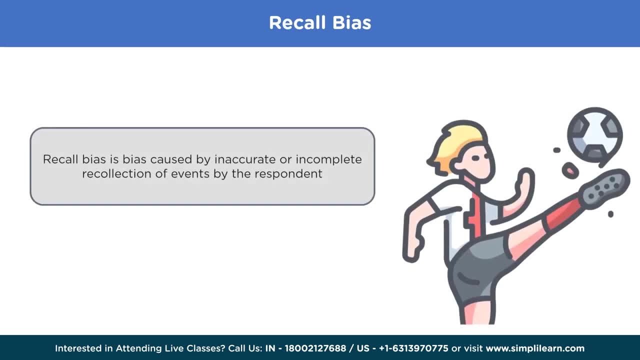 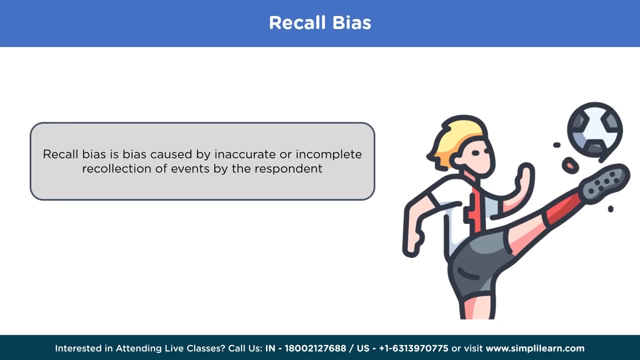 If this was the case, it wouldn't be fair to conclude that a program was effective or not. In this case, a self-selection bias occurs. Recall bias: Self-selection bias occurs when respondents' recollection of events is inaccurate or incomplete. It's especially problematic when it comes to retrospective surveys. question. 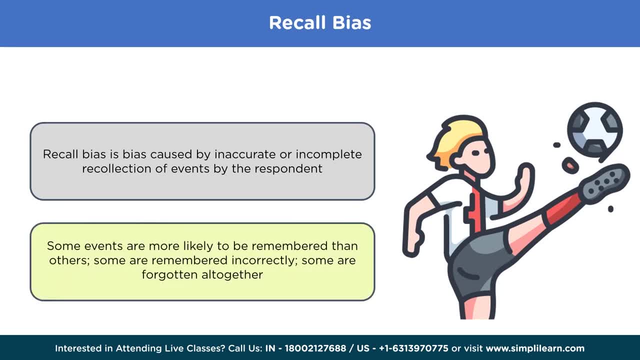 For example, suppose you are asked for a football match that happened three years back Now. you may remember the goals and the good moments of the football match, but might not be able to recall the bad moments or the fouls or the mistakes that happened in that match. 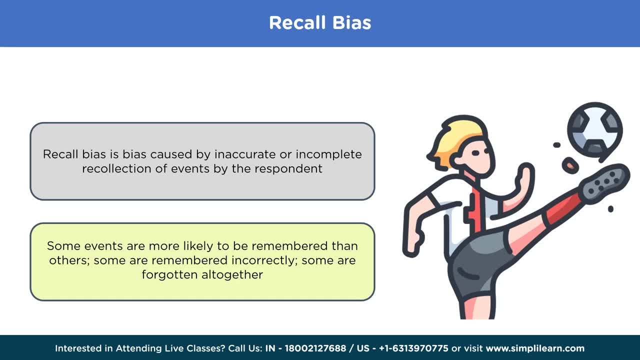 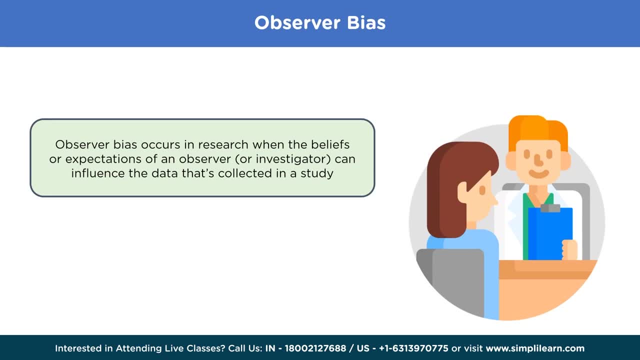 So if you try to guess work here, in this case a recall bias can occur. Another one is the observer bias. When a researcher subconsciously projects their expectation onto the research, this is known as the observer bias. In this case, the beliefs or expectation of an observer can influence the data that is collected for the study. 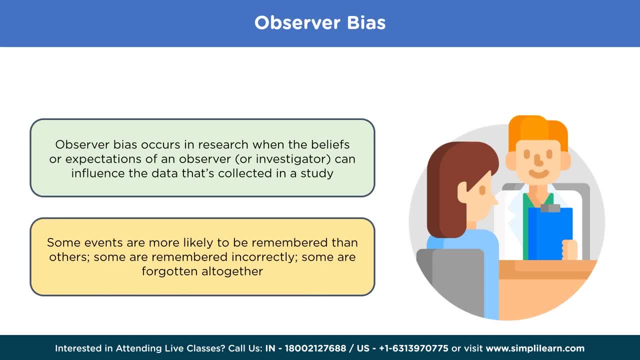 Let's try to understand this observer bias with the help of an example. Suppose there is a certain news channel Now in the race of TRP. certain news might not be accurate or may be even false. To prove his point, he may try to prove that this news is correct and the data that are given are accurate. 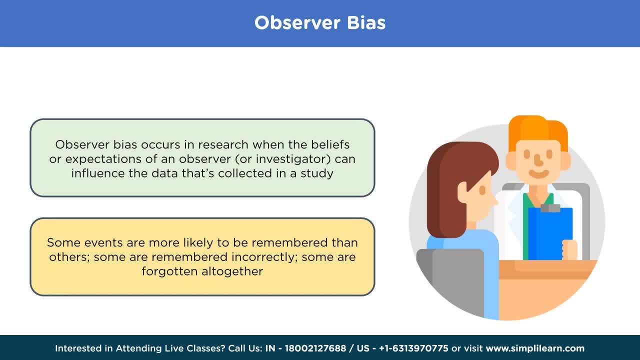 In this case, the observer, which is the news channel, is trying to force his opinion on the data And in this case the observer bias can occur. So with this we have discussed all the types of biases with the help of an example. 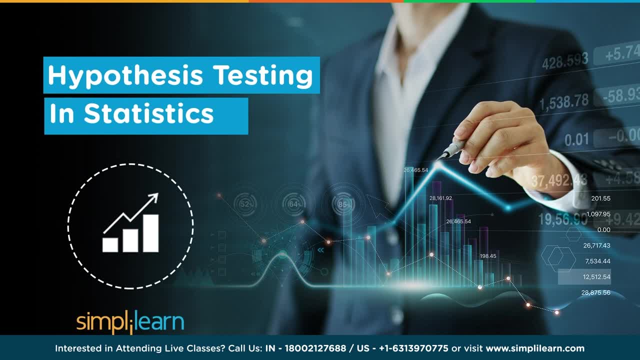 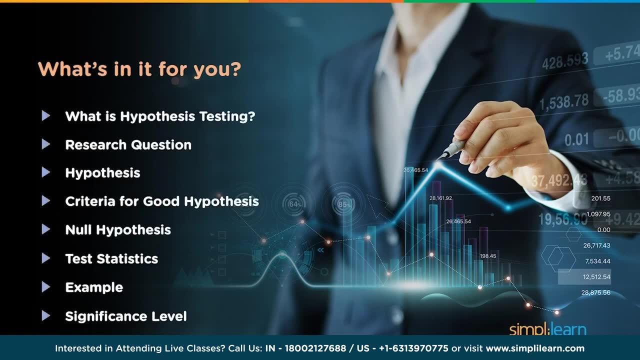 In this video we will be discussing about the hypothesis testing. We will start by talking about the hypothesis testing and how a research question can help you come with a good hypothesis. Then we will discuss the hypothesis testing. We will look at the hypothesis and the criteria for developing a good hypothesis. 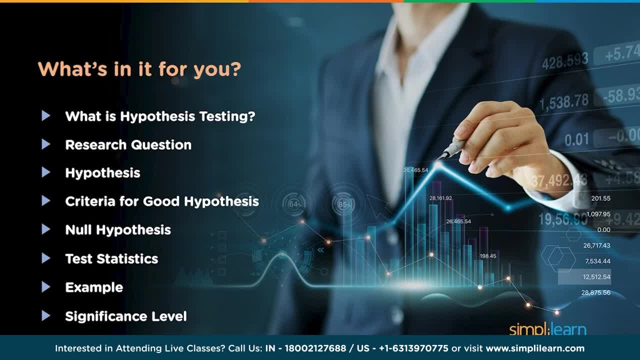 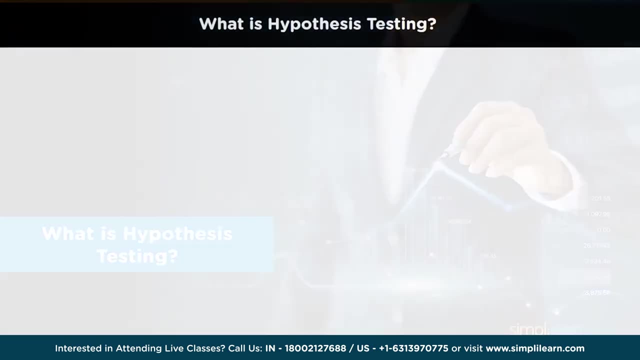 Following that, we will look at the null hypothesis concept test statistics and understand it with the help of an example. Finally, we will conclude this video by briefing you about the significance level. So let's get started. What is hypothesis testing? 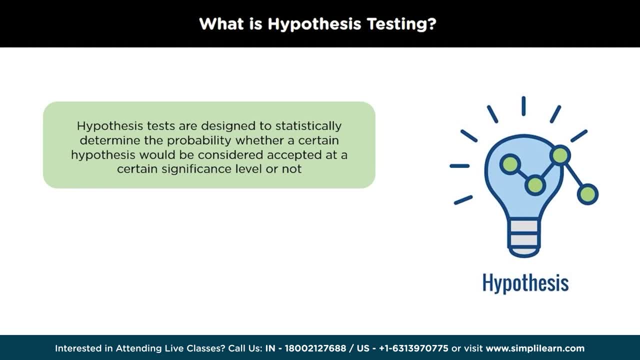 Hypothesis testing or significance testing is the method for testing a claim or hypothesis about a parameter in a population using data memory. The purpose of the hypothesis testing is to check if there is enough statistical evidence in favor of a hypothesis that we have claimed. 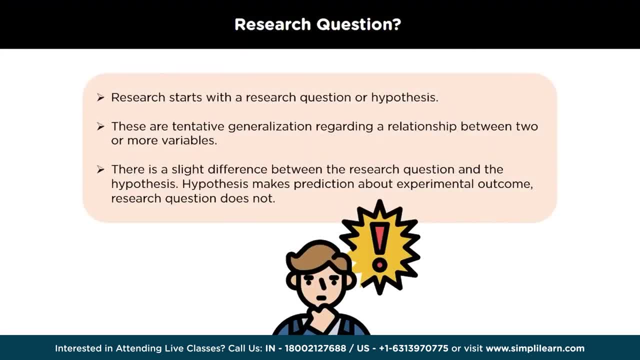 Now we will move on to the research question. A research problem is a broad issue that you would like to address through your research. It identifies a difficult doubt or area of concern in the theory or in practice that requires thought and investigation. Research objectives are clear statements of what you aim to achieve through your research. 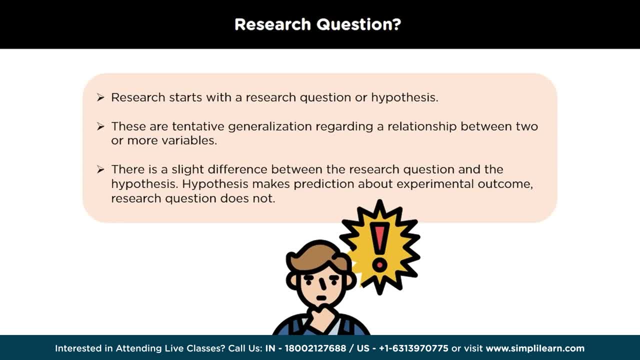 There are specific actions that you will take and act as a milestone that will help you complete your research. A research question is a specific concern that you will answer through your research. It is derived from your research problem but is based on your study design. 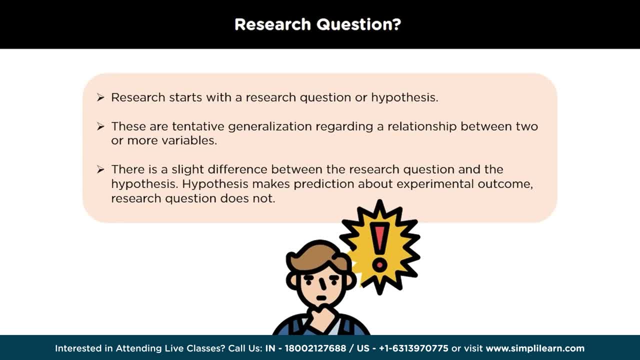 When you narrow down on your research problem to a specific idea that points towards a feasible way to investigate or address your research problems, you will get your research question. Now, what you should really take care of is: there is a slight difference between a research question and a hypothesis. 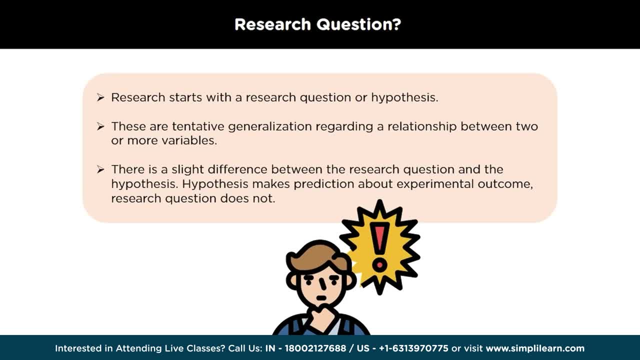 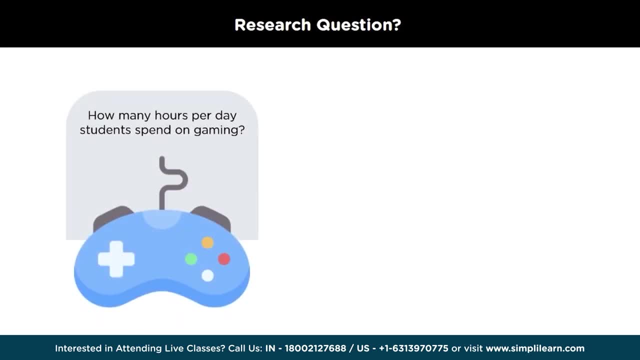 Hypothesis makes predictions about an experimental outcome, whereas a research question does not. Let's understand with the help of an example. Suppose your research question is how many hours per day a student spends on a gaming and you want an answer for that. 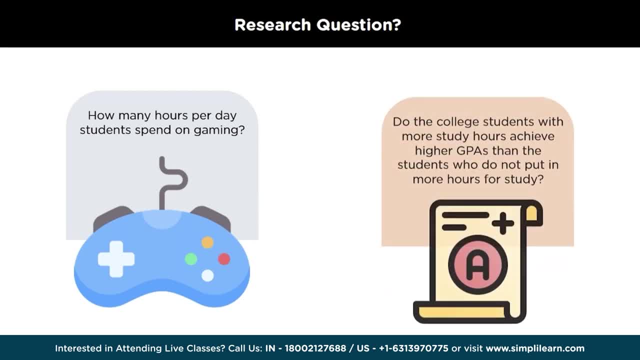 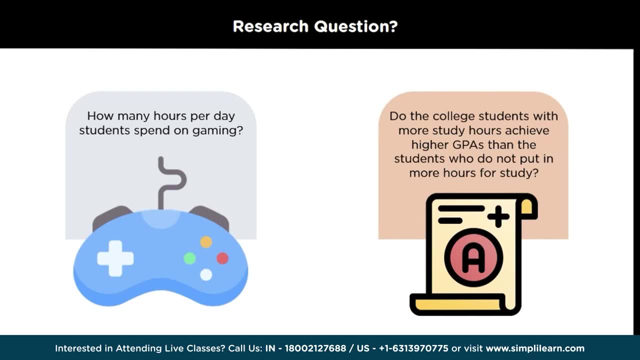 Another research question may be: do the college students with more study hours can achieve a higher GPA than the students who do not put in more hours for study? These questions can be answered by framing a hypothesis. So let's understand what a hypothesis is. 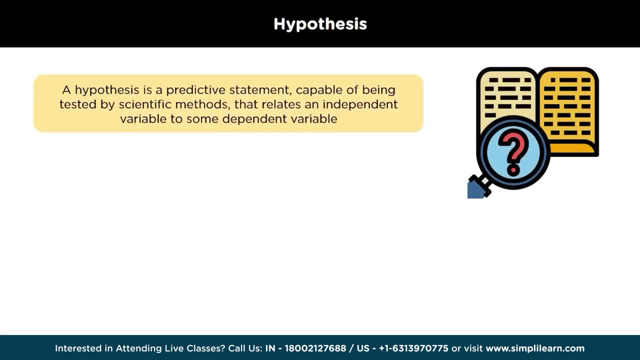 A hypothesis is a tentative statement about the relationship between two or more variables. It is a specific, testable prediction about what you expect to happen in a study. The hypothesis is a prediction, but it involves more than a guess. Most of the time, a hypothesis begins with a question, which is then explored through a background research. 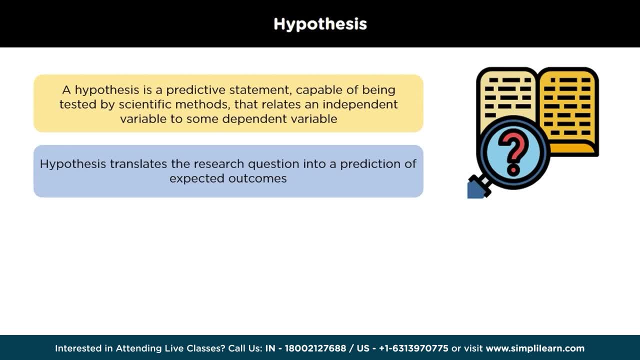 Hypothesis translates a research question into a prediction of expected outcomes. Unless you are creating an exploratory study, a hypothesis should always explain what you expect to happen. So, as in the previous slide, we have framed a question that how many hours per day a student spends on a gaming. 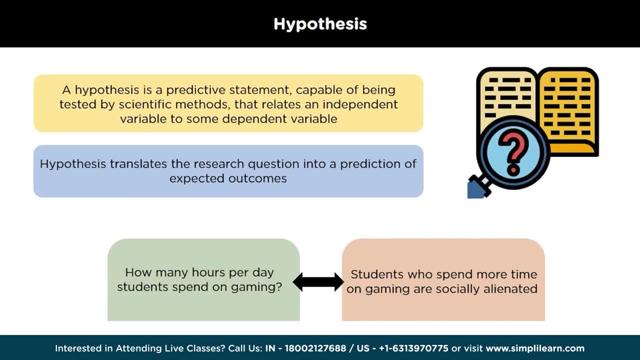 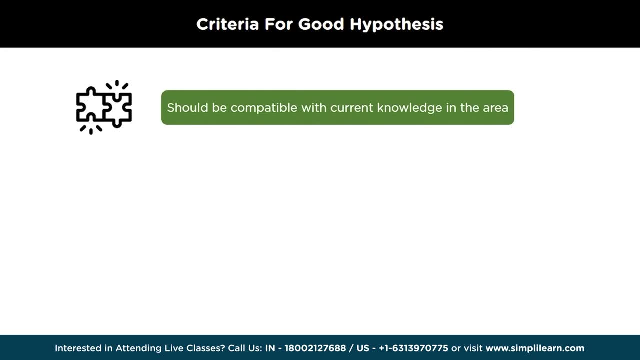 Relating to this question, we can create a hypothesis that students who spend more time on gaming are socially alienated. So there are some good criteria for a good hypothesis. Let's discuss what are those. A hypothesis should be compatible with the current knowledge in the area. 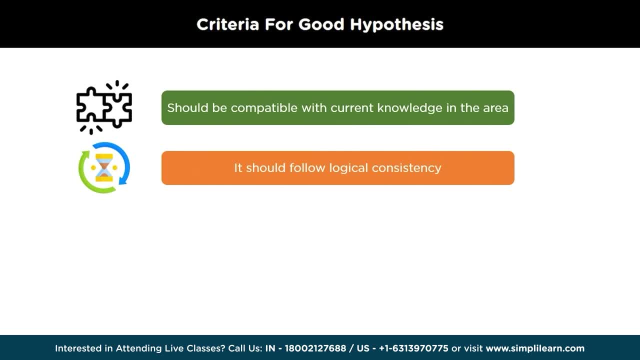 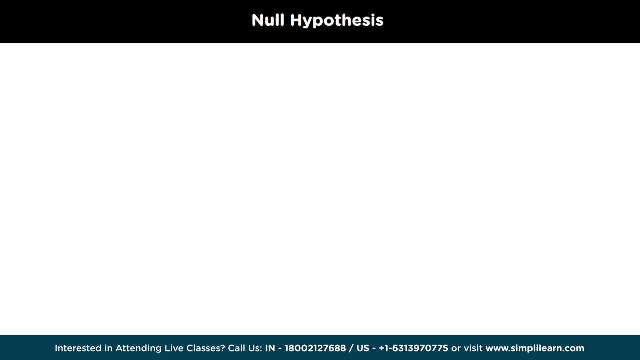 And it should follow the logical consistency. It should not be inconsistent in places. A good hypothesis must be stated briefly and clearly And it should be testable. Now we will understand what a null hypothesis and alternative hypothesis is. The null hypothesis is the assumption that an event will not occur. 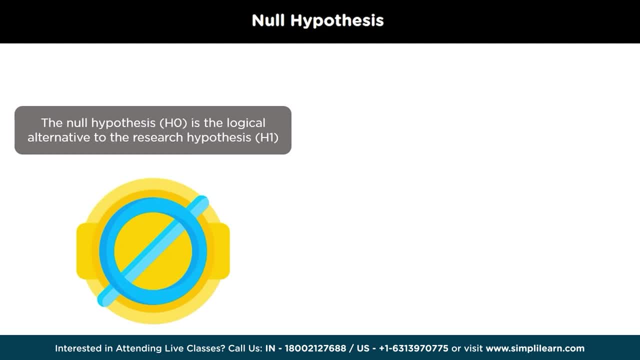 A null hypothesis has no bearing on the study's outcome unless it is rejected. H0 is the symbol for null hypothesis. The null hypothesis on a research hypothesis is the logical opposite of the null hypothesis. The acceptance of the alternative hypothesis follows the rejection of the null hypothesis. 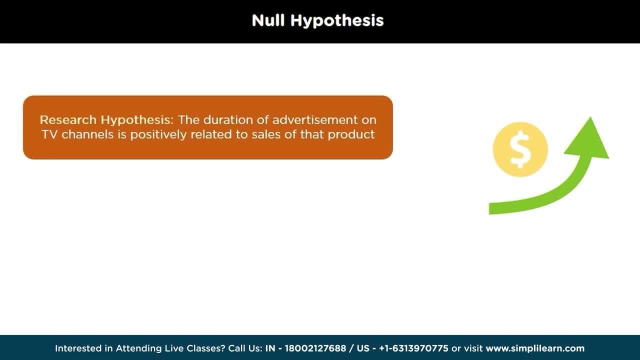 Let's understand the null hypothesis with the help of an example. Suppose you have a research hypothesis that the duration of an advertisement on a TV channel is positively related to the sales of the product. The more the duration, the more the sales of that product. 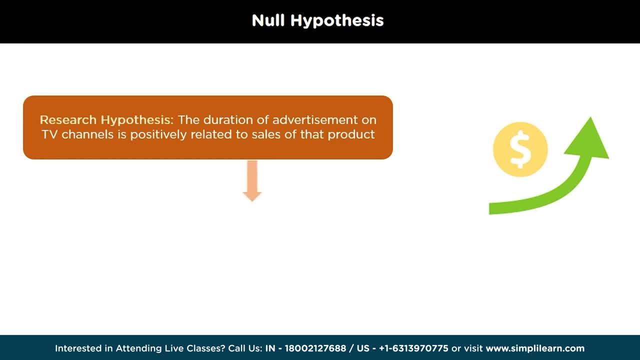 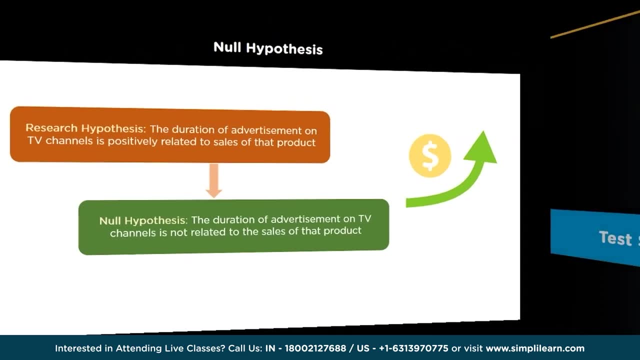 So the null hypothesis of this assumption would be: The duration of the advertisement on the TV channels are not related to the sales of the product. They are not related at all. Now we will move on to the test statistics that are frequently discussed when creating hypothesis testing. 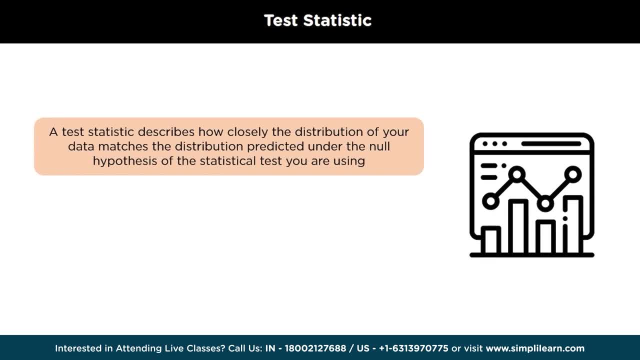 The test. statistics is a number calculated from the statistical test of a hypothesis. It shows how closely your observed data matches the distribution expected under the null hypothesis of that statistical test. The distribution of the data is how often each observation occurs And can be described by its central tendency and variation around the central tendencies. 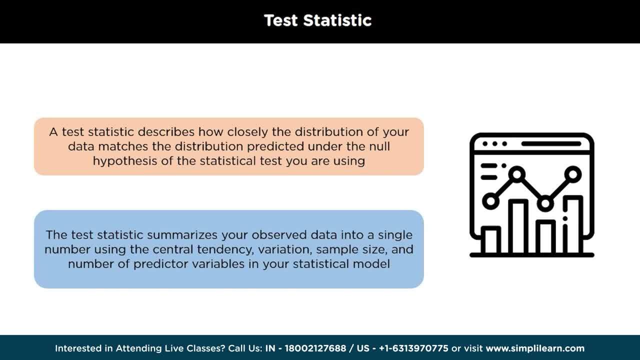 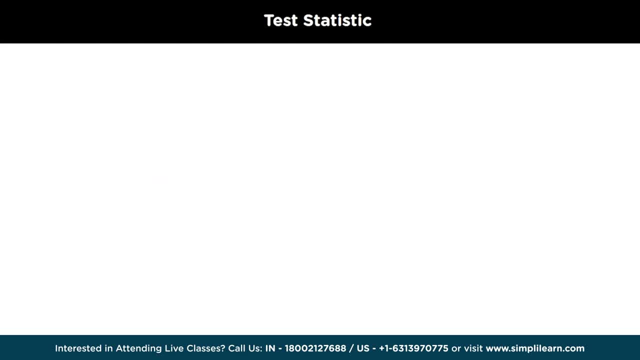 The test statistics summarizes your observed data into a single number using the central tendency variation of sample size and the other number of predictable variables in your statistical model. There are broadly three types of statistical tests. Different statistical tests have slightly different ways of calculating these test statistics. 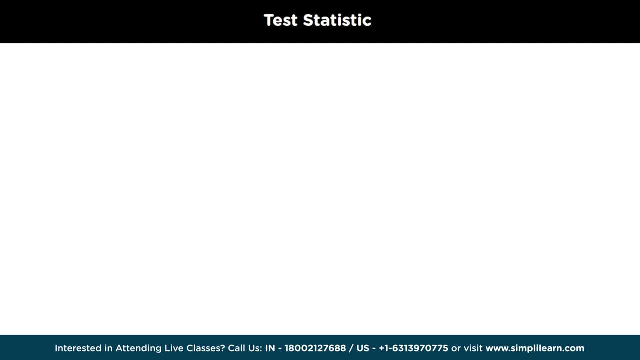 But the underlying hypothesis and interpretation of the test statistics stay the same. The first way is a t-test. A t-test is a statistical test that is used to compare the means of two groups. It is often used in hypothesis testing to determine whether a process or treatment actually has an effect on the population of interest or whether the two groups are different from one another. 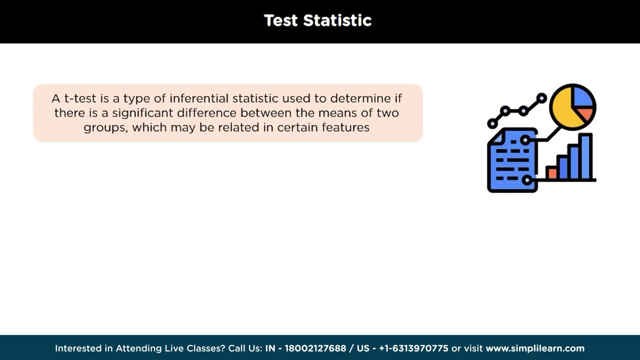 The null hypothesis is that the true difference between these group means is zero, and the alternative hypothesis is that the true difference is different from zero. Now let's move on to z-tests. Z-tests are statistical tests. There is a different way of testing a hypothesis than either we know the population variance or we don't know the population variance, but our sample size is greater than 30.. 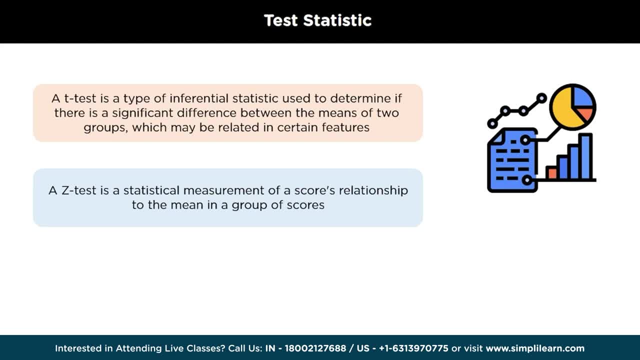 We perform the z-test when we want to compare a sample mean with the population mean. The next is an f-test. The f-test, or the f-statistics, is simply a ratio of two variances. Variances are the measure of dispersion, or how far the data are scattered from the mean. 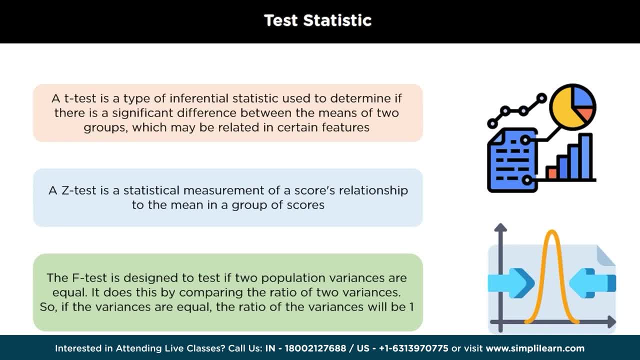 Larger values represent the greater dispersion. Despite being a ratio of variance, you can use the f-test in a wide variety of situations. F-test can assess the equality of variances. However, by changing the variances that are included in the ratio, the f-test becomes a very flexible test. 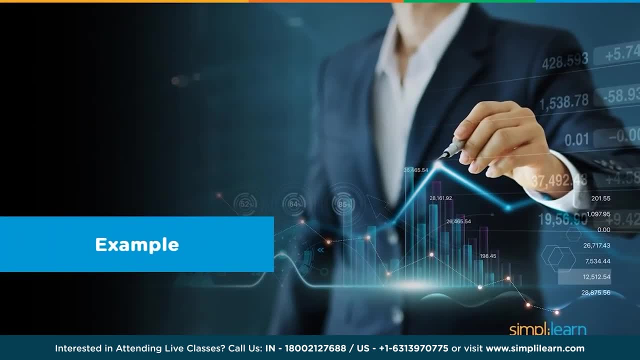 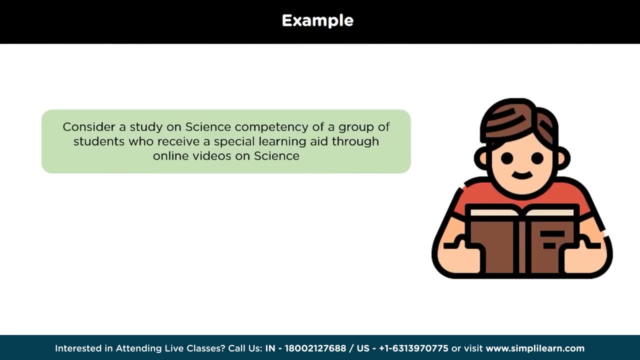 Now that we have discussed all the theories related to the hypothesis testing, let's take an example to understand them more clearly. Consider a study on a group of students where the students receive a special learning aid through the online videos on science. It is hypothesized that after viewing this online video, 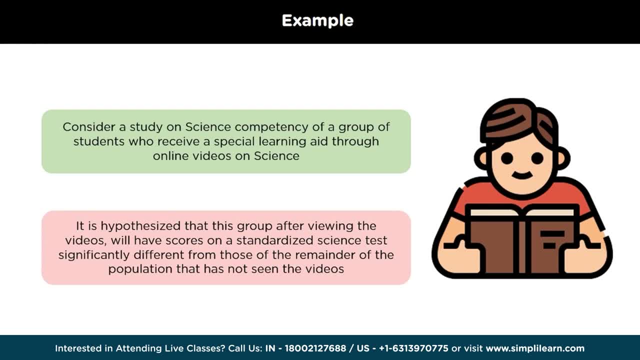 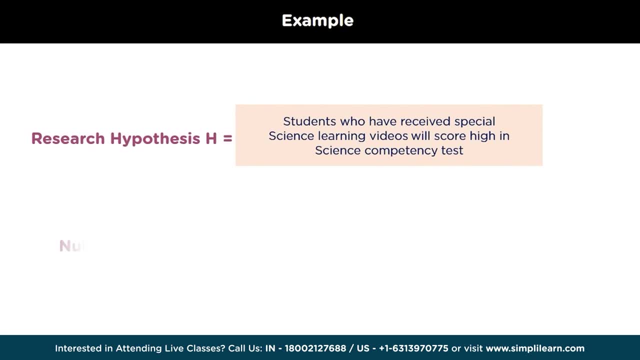 the group of students score better than the one who have not seen the videos. So in this case, a research hypothesis will be: students who have received the special science learning videos will score high in the science competency test And its null hypothesis will be. 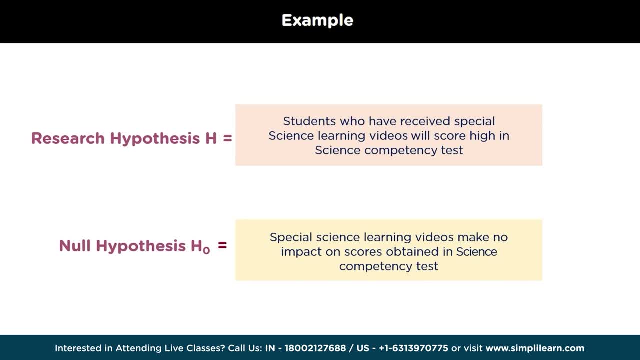 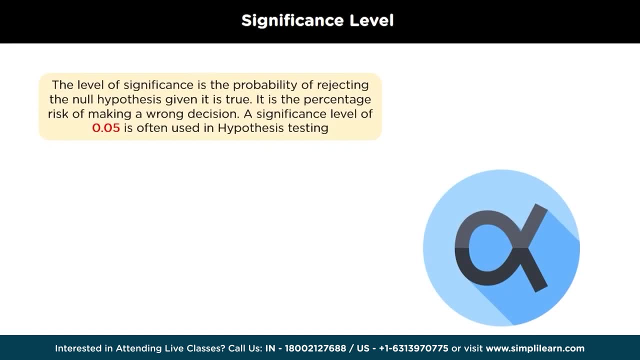 the special science learning videos made no impact on the scores of the students. Now we will discuss what a significance level is. Level of significance or significance level is the level of significance or significance level of a student. Now we will discuss what a significance level is. 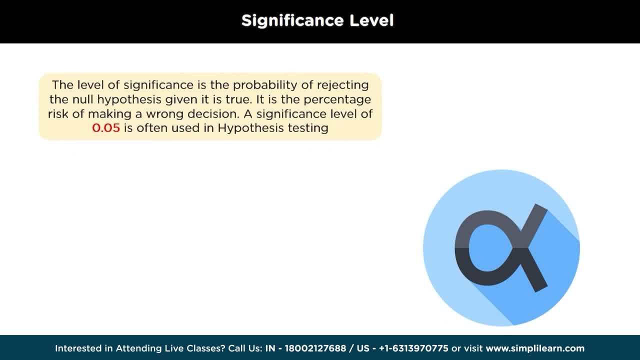 Level of significance, or significance level, refers to a criterion of judgment upon which a decision is made regarding the value stated in the null hypothesis. This criteria is based on the probability of obtaining a statistic measured in a sample if the values stated in the null hypothesis were true. 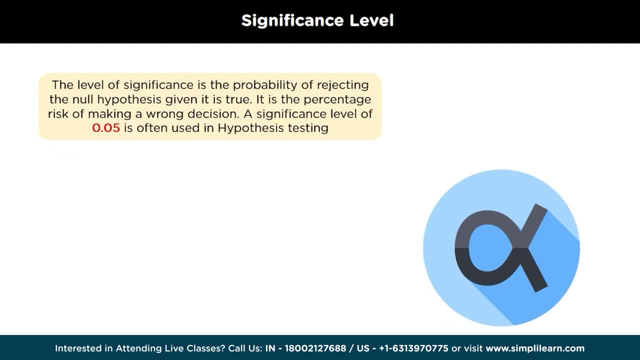 Generally, the criterion of the level of significance is typically set at 5% or 0.05.. This value of significance level can also be taken as 1% or 10%, depending upon your requirement, If the result obtained from the study indicates the probability lower than the significance level. 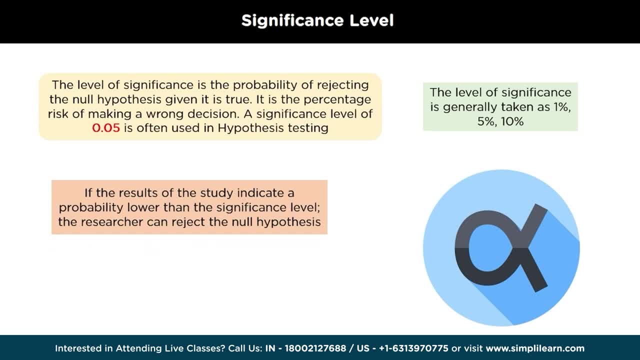 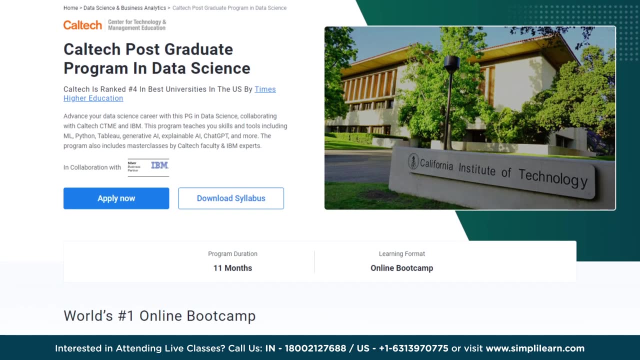 so in this case, a researcher can reject the null hypothesis. Otherwise, if the result of the study indicates the probability higher than the significance level, the researcher can support the null hypothesis. SimplyLearn's postgraduate program in data science, offered by Caltech University in collaboration with IBM, is just what you need. 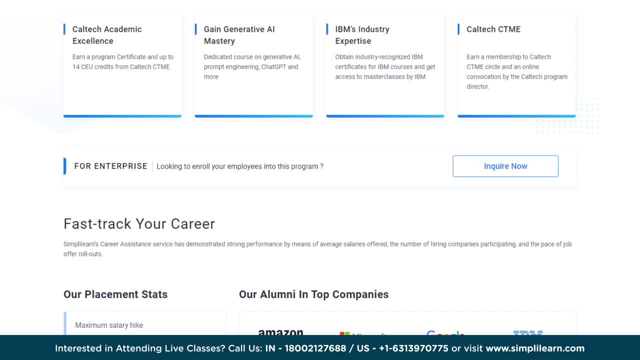 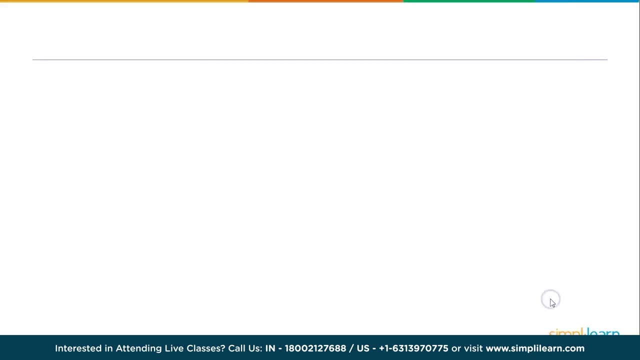 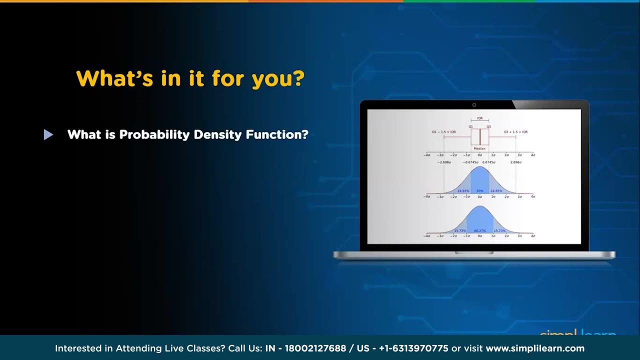 For more details, head straight to our homepage and search for data science postgraduate program, or simply click on the link below. So let's get started. So what can you expect from this video? What's in it for you? First, we will go over the basic definition of the probability density function. 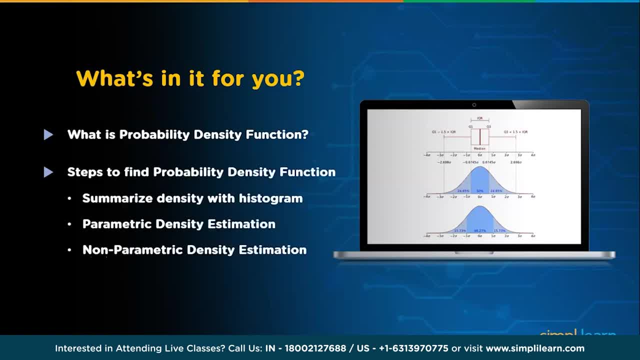 followed by the steps to find the probability density function. There are three main steps, which is summarizing the density using histograms, parametric density estimation and non-parametric density estimation. And finally, we will see how to implement all three of these steps in Python. 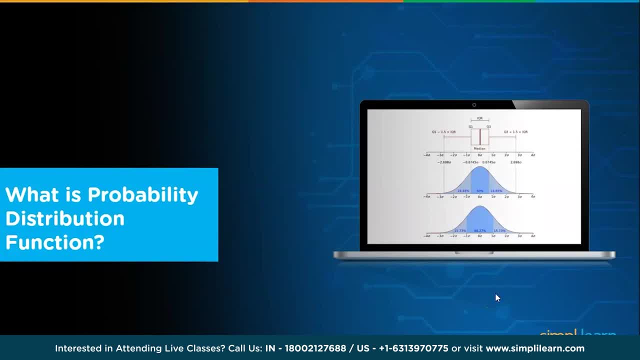 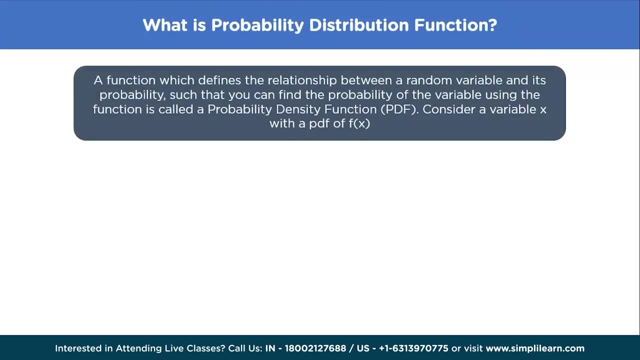 So now let's dive into the definition of the probability distribution function. What is probability distribution function? A function which defines the relationship between a random variable and its probability, such that you can find the probability of the variable using the function, is called a probability density function. 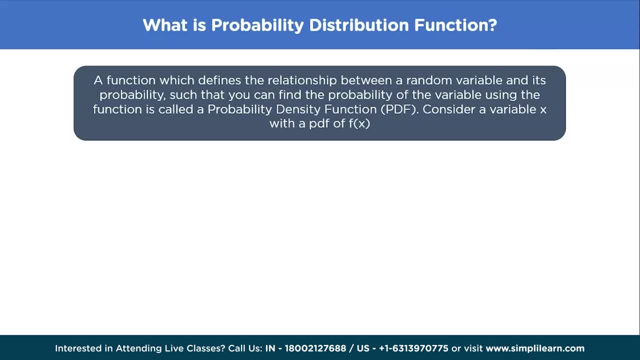 In simple words, probability density is the relationship between an observation and the probability. Some outcomes of a random variable will have low probability density and other outcomes will have a very high probability density. Basically, the probability of a variable x happening or occurring will vary. 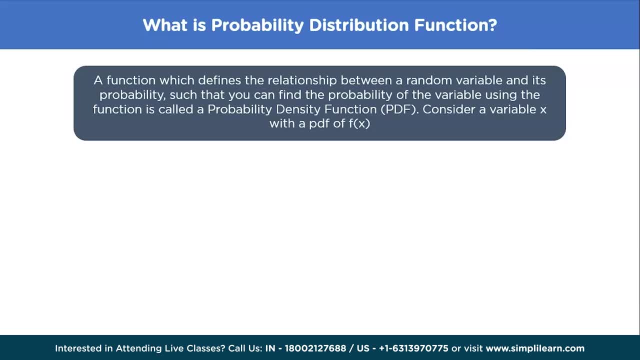 and it can sometimes take on a lower value or it can take on a way higher value. The overall shape of the probability density is referred to as probability density function. The probability distribution and the calculation of probabilities for specific outcomes of a random variable is performed by a probability density function. 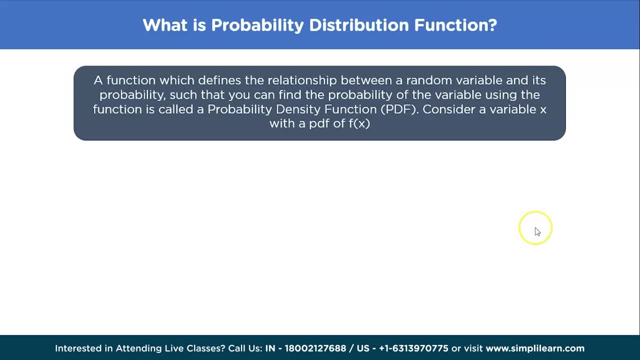 or PDF for short. Now consider a variable x with a PDF of f of x. This is what your probability density function will look like. There might be a point where the probability of x occurring is very high, Hence your probability distribution function or f of x. 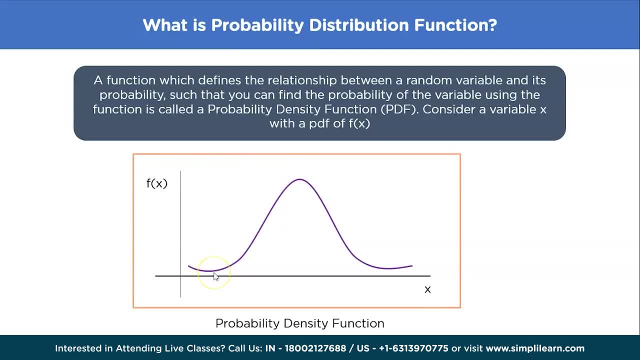 will also be very high. At other points, the distribution or the probability of x happening or occurring is going to be very low. Hence your f of x is also going to have a very small value, Basically, given the random sample of a variable. 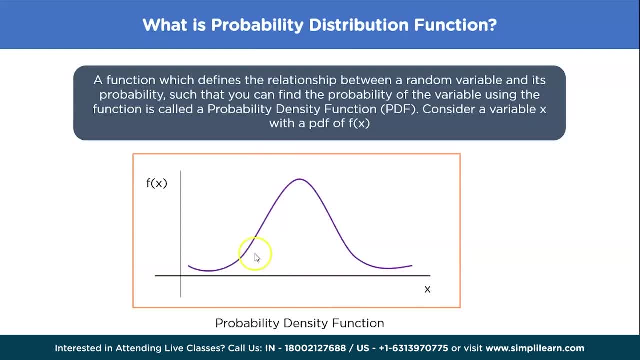 we might want to know things like the shape of the probability distribution. This here is something called a normal distribution, where your probability distribution function takes on a bell shape. However, this is not the probability density function. that might always occur. There are different probability distribution functions. 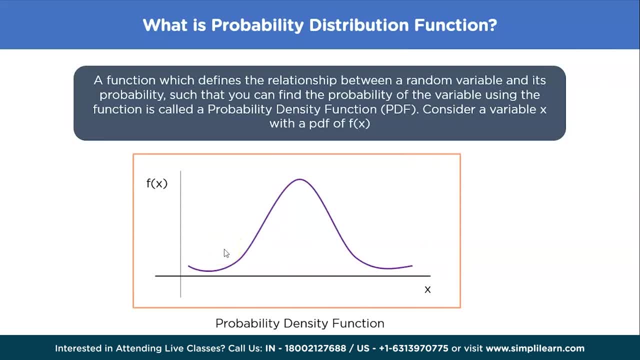 and all of their graphs look very different from each other. Knowing the probability distribution for a random variable can help you calculate movements of the distribution, like the mean and variance, But it can also be useful for other more general considerations, like determining whether an observation is unlikely or very unlikely. 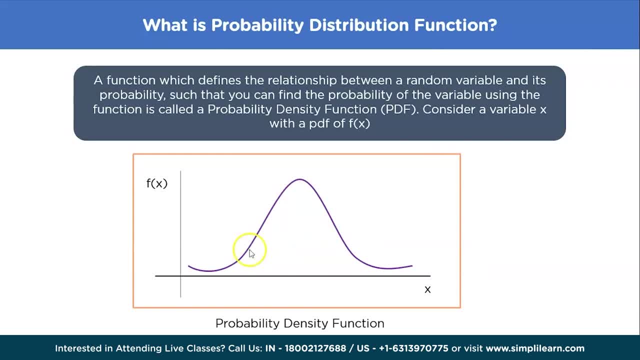 and might be an outlier or an anomaly like consider this graph itself. In this graph, these points over here which have very less probability distribution are outliers, which means that the chance of them occurring is very low and basically, this is not something that you are going to see. 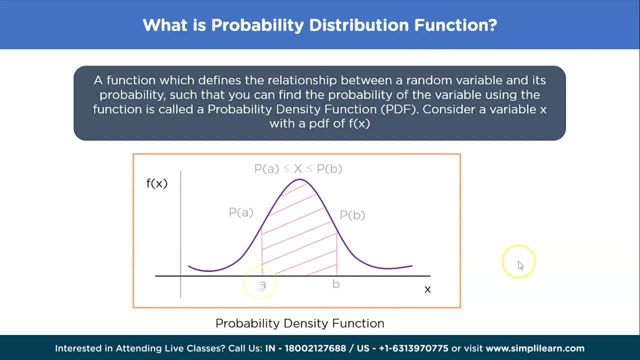 in your regular scenario for your variable x. Now let's consider two points, a and b, which are values that our variable x can take. p of a and p of p just represent the probability of a and the probability of b, which can be found out by drawing a straight line. 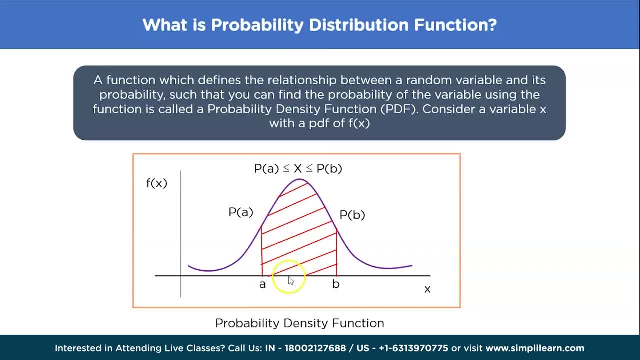 and coinciding it with our graphs. The area under the graph over here, which is going to give you your probability of this region occurring, can be written as probability of a less than equal to x, which is the probability that we are searching for here- less than equal to probability of b. 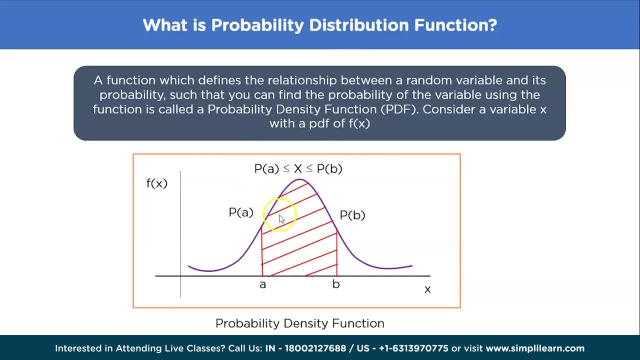 What does this mean exactly? This means that this area is always going to be greater than or equal to the probability of a, but less than or equal to the probability of b. This gives us the narrow region of the probability which is present over here. and doing this, 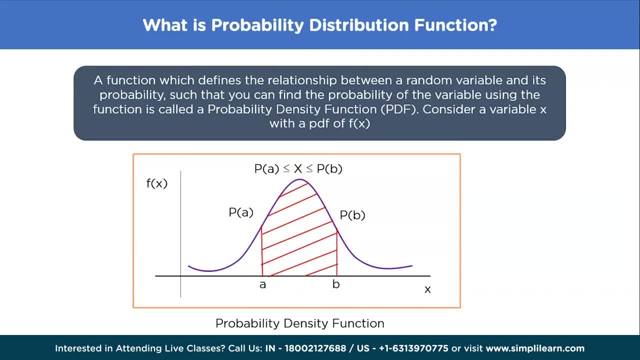 we can find the probability of occurrence for any value of x. Suppose you want to find the probability of b happening For a probability distribution function, the probability of b happening is not simply this point here, but the entire area of the graph which is taking place before this point itself. 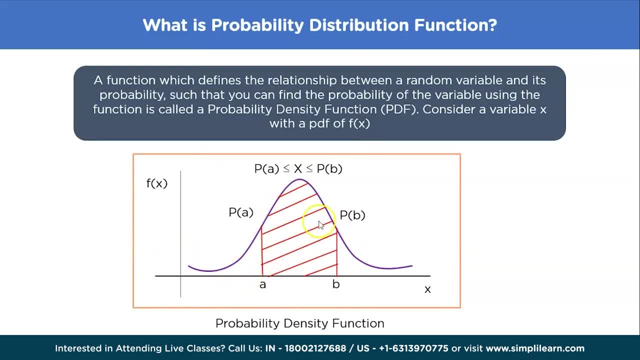 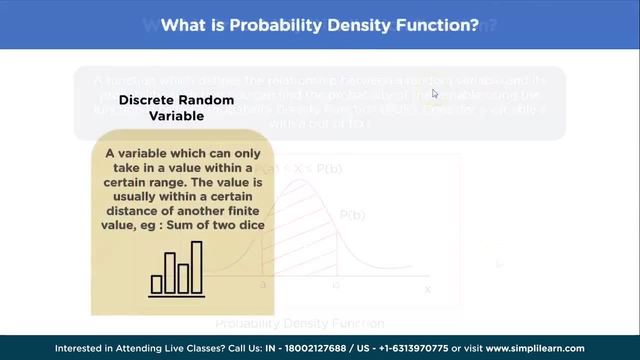 So if you want to find the probability between these regions, you are going to have to find the entire area and not simply the probability at one point. Now, so far, we have been talking about different types of variables, which is discrete, random variables and continuous variables. 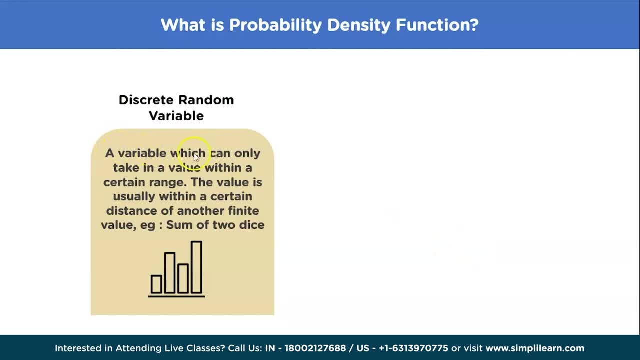 What exactly do these mean? A variable which can only take a value within a certain range is called a discrete, random variable. The value is usually within a certain distance of another finite value. An example of this would be the sum of two dices. 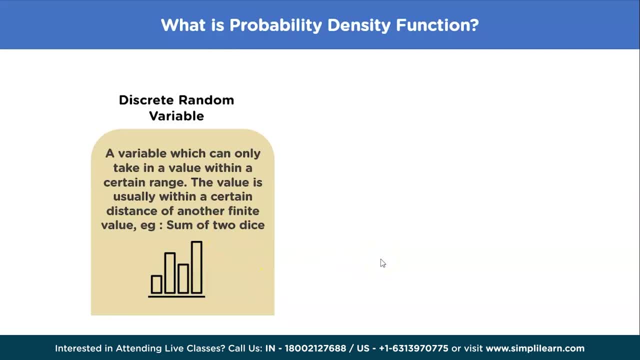 Basically, values which are well defined are called discrete values, and a variable which has well defined values will be called a discrete, random variable. This variable can only take values which fall within a certain set of values. Let's say you roll a dice, the dice can only give you specific outcomes. 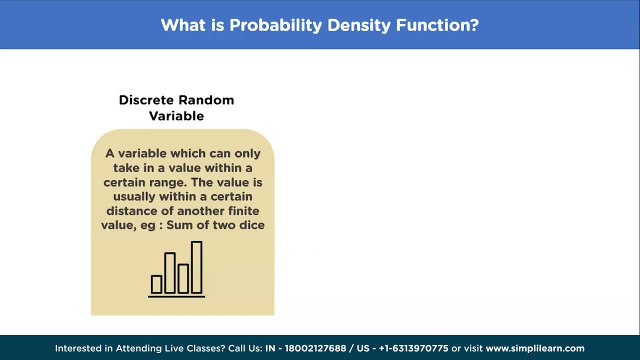 which range from 1 to 6.. This is what you would call a discrete output. On the other hand, a continuous random variable can take on infinite different values within a range of values, for example, the height of a student. The height of a student is not fixed. 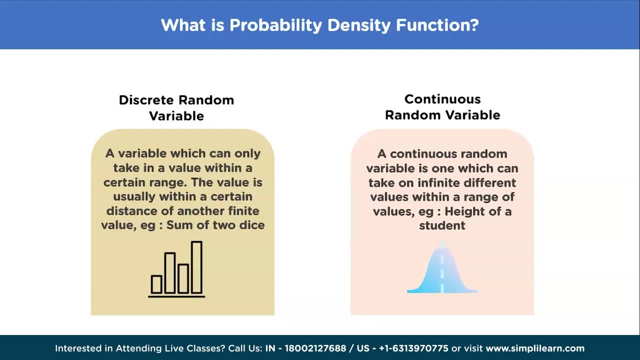 even if the height is 1.7 m, in reality the height can be 1.7 m or 1.765 or 1.789. The exact height is very hard to determine because it's not easy for us to find the precise value of the height of a student. 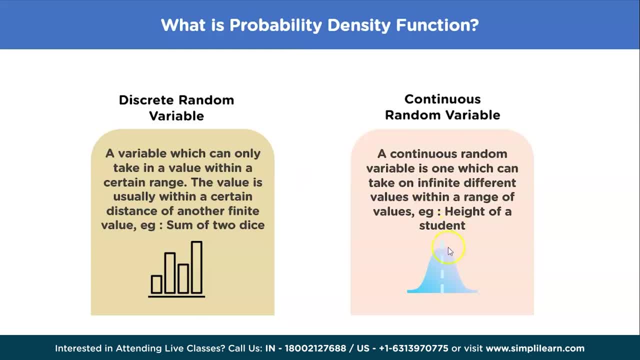 So basically, the height can take on an infinite different range of values. When we are trying to define the values that a continuous random variable can take, we usually say it in the form of a range of values, which means that the value can fall in that range. 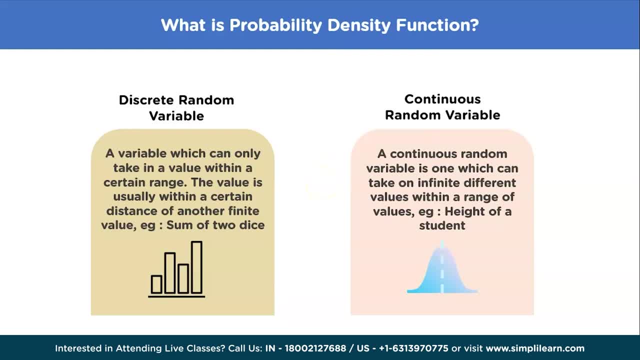 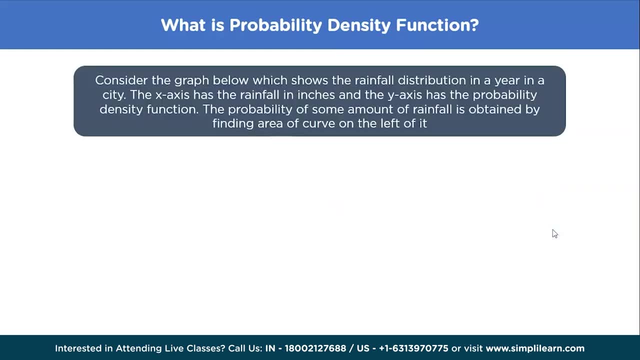 and can take on any value in that range. It's not like a discrete, random variable where you can define definitive values. Now let's understand a probability density function with the help of a graph. Consider the graph below, which shows the rainfall distribution in an year in a city. 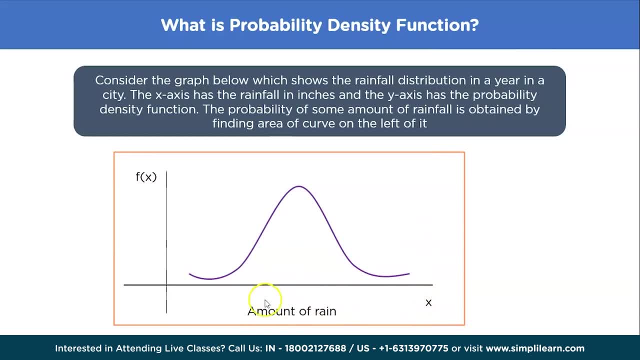 The x-axis has the rainfall in inches, or the amount of rain that we are getting, and the y-axis has the probability density function of getting that amount of rain. The probability of some amount of rain is obtained by finding the area of the curve to the left of it. 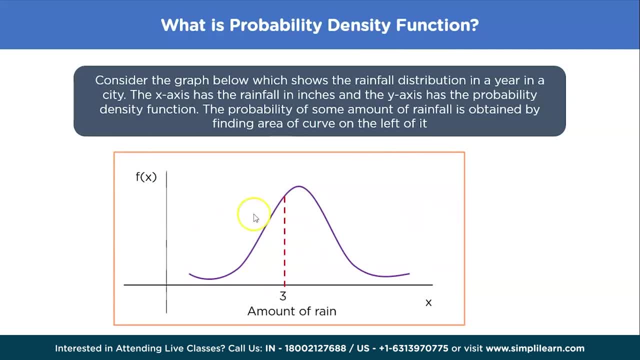 So let's say we have a point 3. If we want to find the probability of 3 inches of rainfall occurring, we would have to find the area of the curve which falls to the left of 3.. When we draw a line from 3, 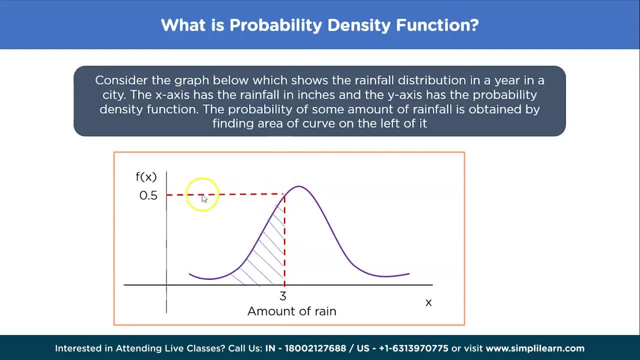 which intercepts the graph and further extend it onto the y-axis, we get a value of 0.5.. Simply put, this means that the probability of 3 inches of rainfall occurring is going to be lesser than or equal to 0.5.. 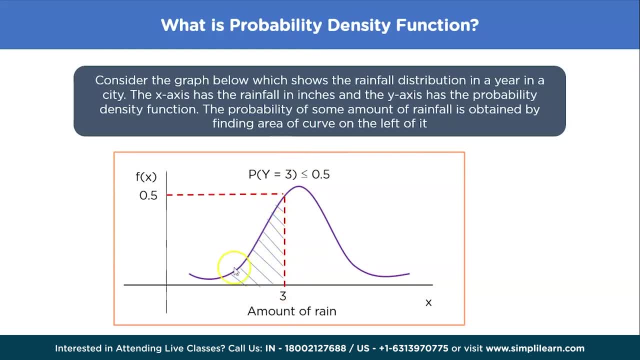 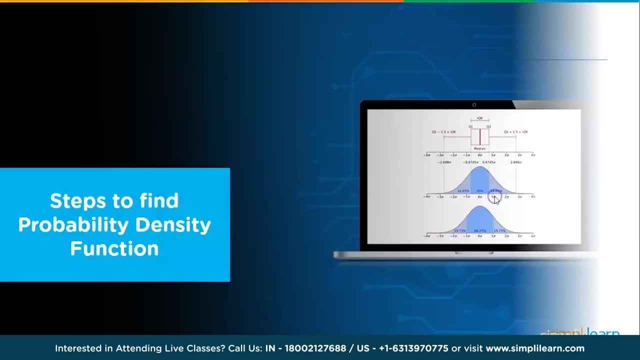 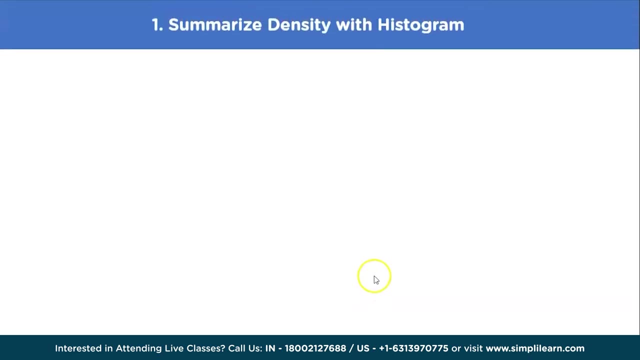 The exact probability can be found out by finding the area of the curve which falls to the left of 3.. How do we find the probability distribution function? The first step is to summarize your density with the help of a histogram. The first step in a density estimation: 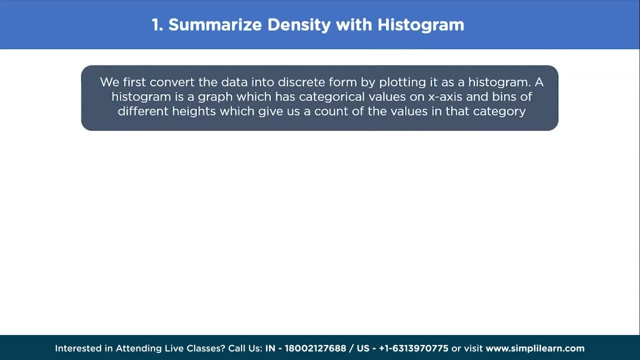 is to create a histogram of the observations in the random sample. Now, what is a histogram? A histogram is a plot which involves first grouping the observation into bins and counting the number of events that fall in each bin, The counts of frequency of observation in each bins. 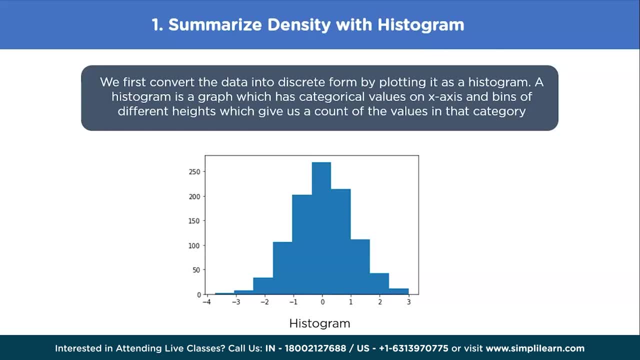 are then plotted as a bar graph, with the bins on the x-axis and the frequency on the y-axis. The choice of the number of bins is important, as it controls the coarseness of the distribution and, in turn, how well the density of the observation. 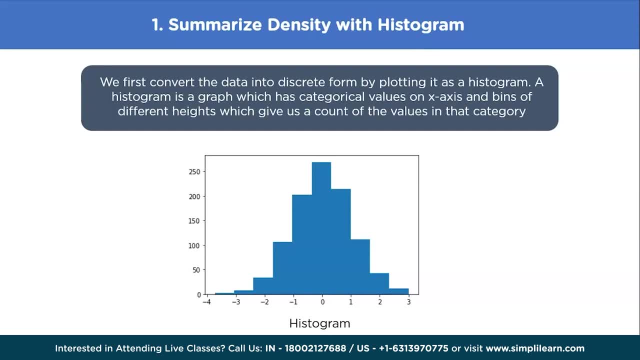 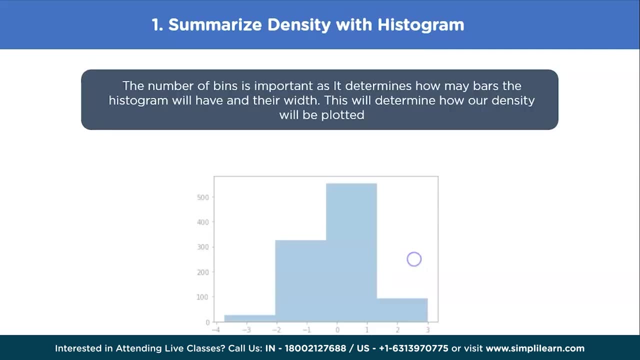 is plotted. It is a good idea to experiment with different bin sizes for a given data sample to get multiple perspectives or views on the same data At the same time. the number of bins is important as it determines how many bars the histogram will have. 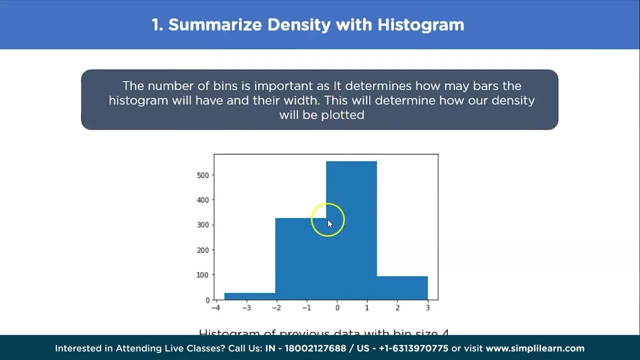 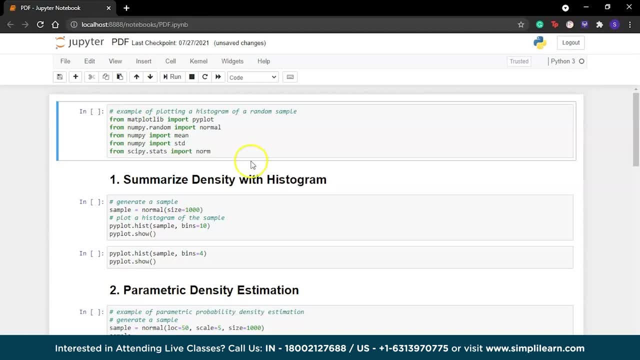 and their widths. This will change not only the shape of the graph, but also how the graph will spread. This will also determine how our density is plotted. Now let's see how we can summarize our density with histograms using Python. First, let's import all of our 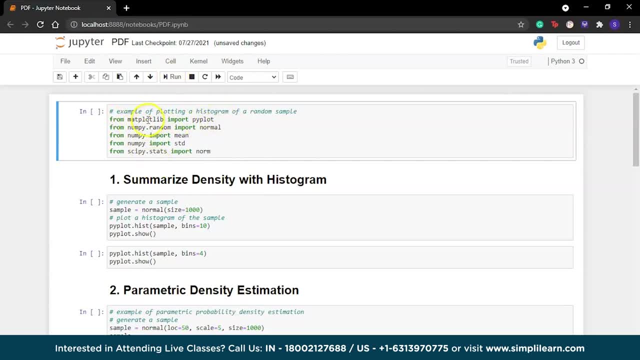 necessary modules which we are going to require. We are going to require matplotlib to plot graphs. We are going to need the normal random function so that we can get a normal distribution. We are going to import mean and standard deviation from numpy to use on our graphs. 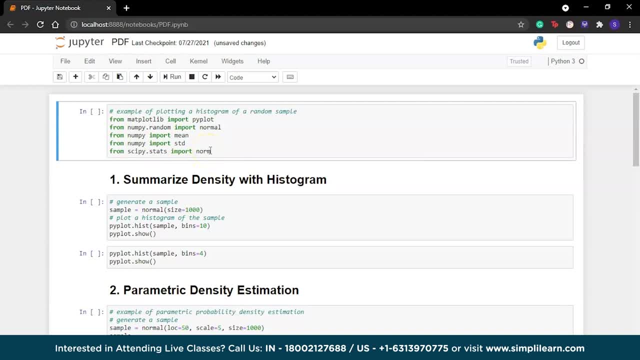 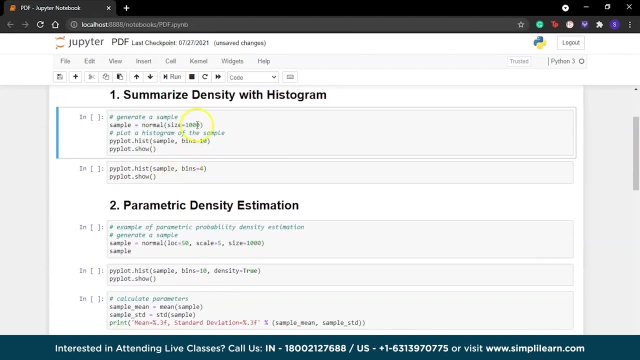 We are also going to normalize the data, so we are going to import the norm function from scipy. We have finished importing all of our necessary modules. Now let's generate a sample which has a size of 1000 and it is going to be a normal distribution. 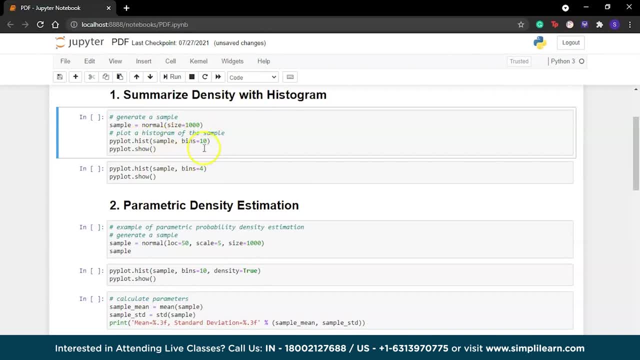 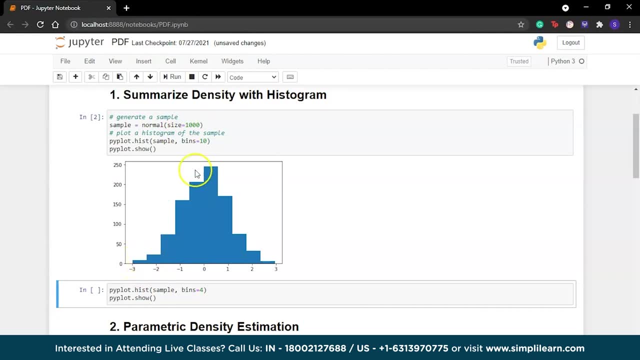 We are going to also plot this with the help of a histogram in bins of 10.. As you can see here, you get a normal distribution which is nothing but an almost bell-shaped curve, and we have 10 bins here which are centered at 0 and which extend. 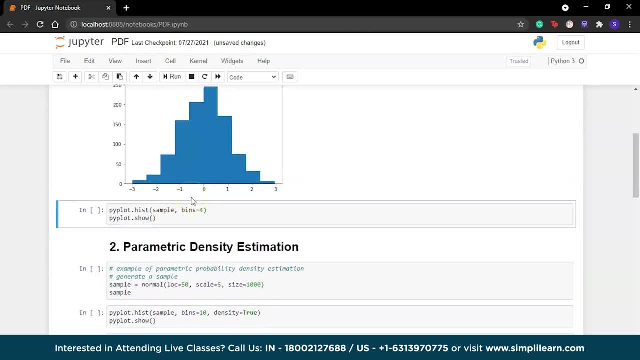 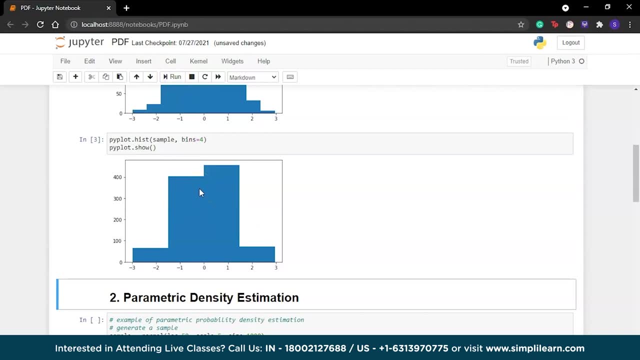 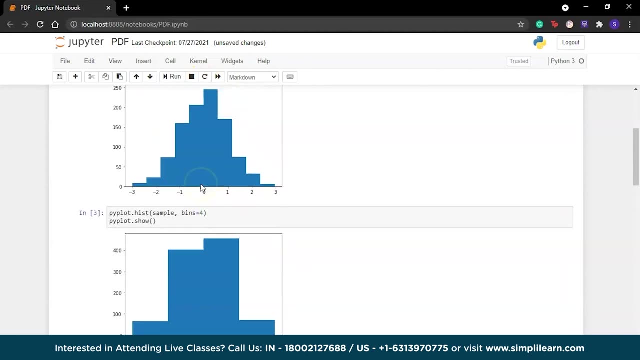 from minus 3 to 3.. How will our graph look if we change the number of bins, though? Let's run it and see. So you still have a normal distribution, but it is not as well defined because of how less the number of bins are. you lose a. 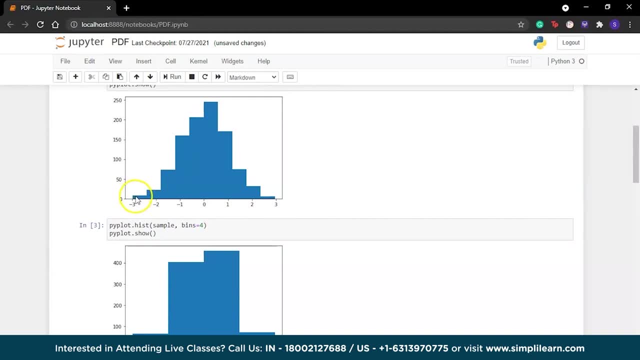 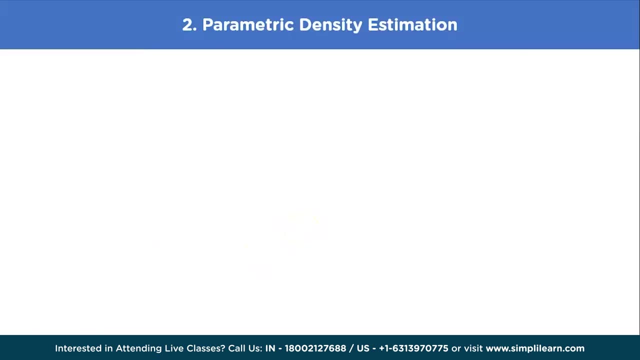 majority of the data which will contribute to your normal distribution. It doesn't look like a proper normal distribution, but looks more like a discrete data at this point. Now let's take a look at the next step of finding our probability distribution function. The next step is called: 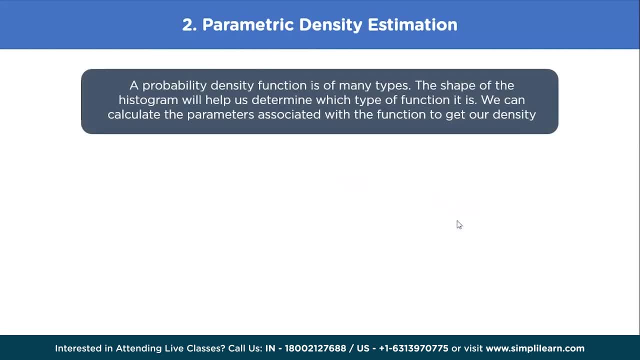 parametric density estimation. What exactly is parametric density estimation? The probability density function is of many types. The shape of your histogram will help you determine what type of a function it is. We can also calculate the parameters associated with the function to get our density. 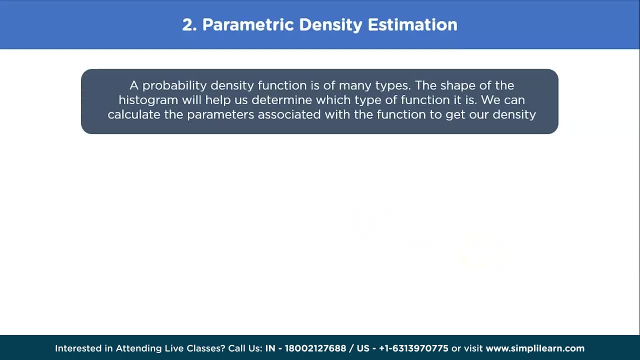 Now, different probability distribution functions will have different graphs, which will have different shapes and which will also have different parameters, like mean, standard deviation, etc. associated with them. Using these parameters, we can find important points of our data. Hence it is very important for us to 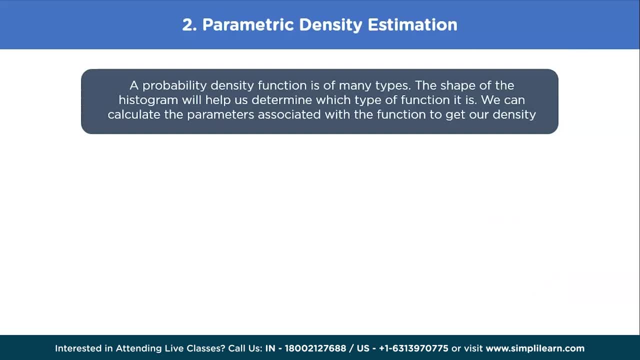 recognize what type of a distribution it is. Common distributions will occur again and again in different and sometimes unexpected domains. Getting familiar with common probability distributions will help you identify a distribution from a histogram and, once identified, you can attempt to estimate the density of the random variable. 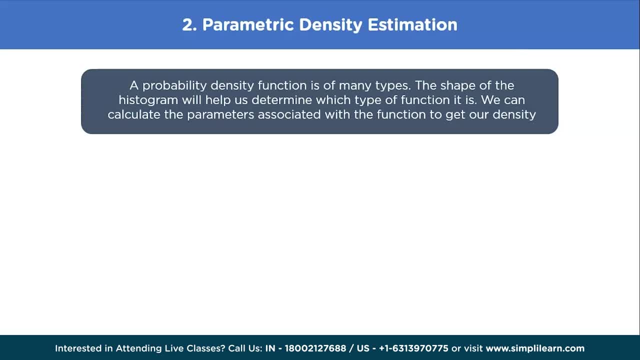 with a chosen probability distribution. This can be achieved by estimating the parameters of the distribution from a random sample of data. Now, an example of this would be a normal distribution which has two main parameters: the mean and standard deviation. Given these two parameters, we will now know. 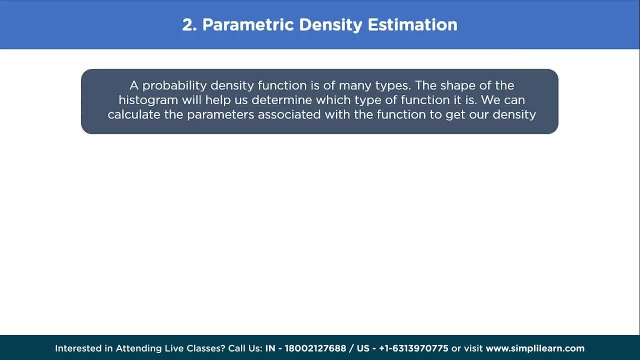 the probability distribution function. These parameters can be estimated from data by calculating the sample mean and sample standard deviation. This entire process is known as parametric density estimation, and it includes identifying your probability distribution function and getting the parameters which are associated with it. Now, once we have 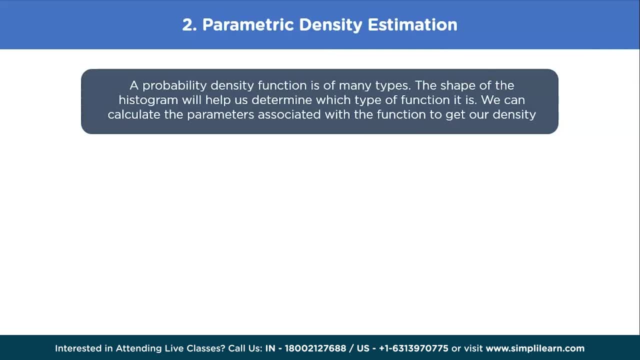 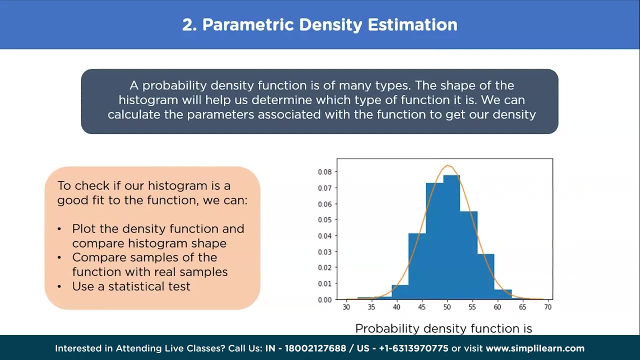 estimated the density, we can check if it's a good fit. This can be done in three different ways. One is plotting the density of the function and comparing the shape to the histogram. The next is sampling the density function and comparing the generated sample to the real sample. 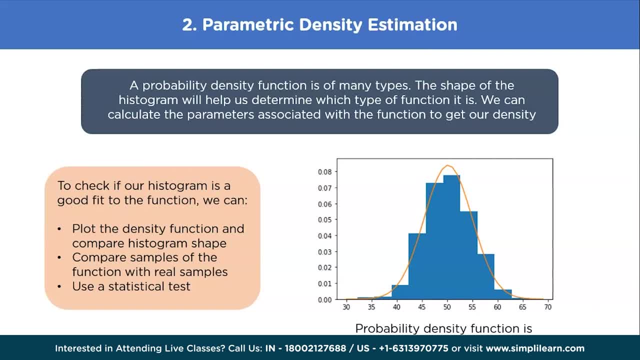 and the last one is using a statistical test to confirm if the data fits the distribution. Now, over here, as you can see, all we've done is taken our data and plotted the density function on top of our histogram and we've compared the shape, So the distribution, so the 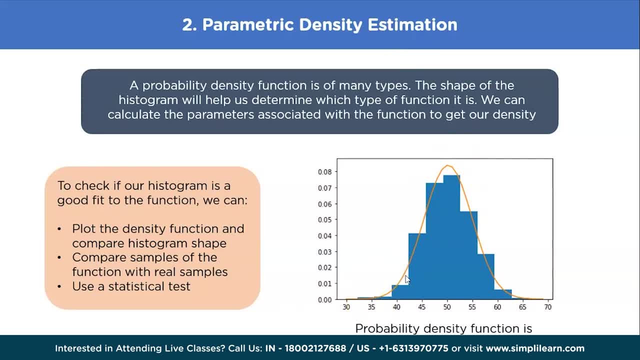 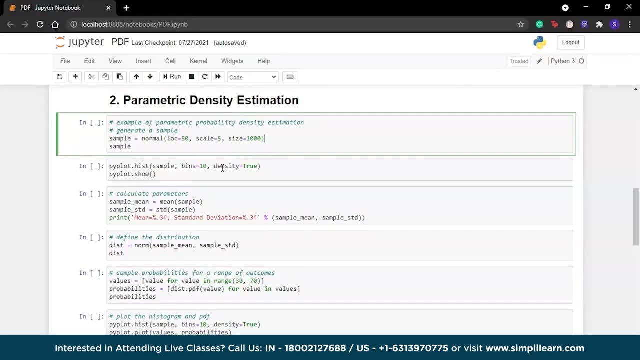 density function that we're actually considering. here is a normal distribution, And from this graph we can see that it's almost an exact fit to our histogram. Now let's see how we can perform parametric density estimation using Python. To begin with, let's generate a. 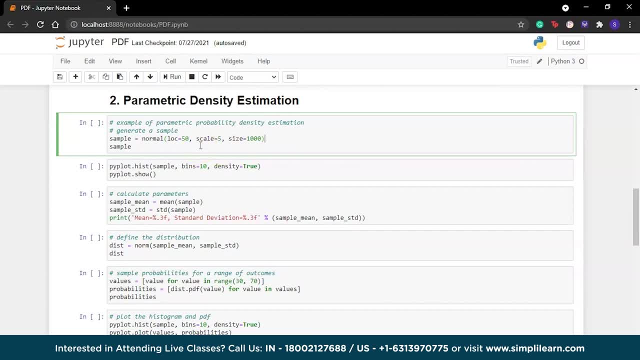 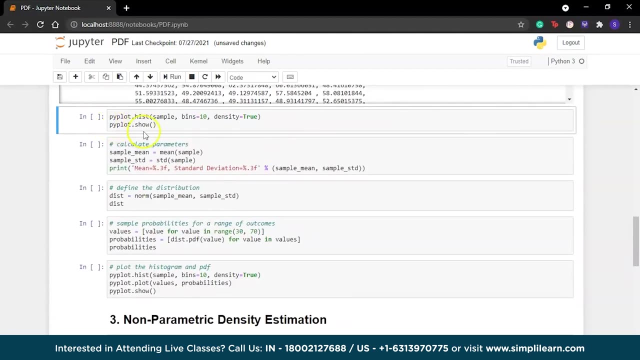 random sample of thousand observations from a normal distribution with a mean of 50, which is determined by the LOC parameter, and a standard deviation of 5, which is determined by the scale parameter. Now, just to show you what the distribution looks like, we're gonna plot it in the form of a histogram. 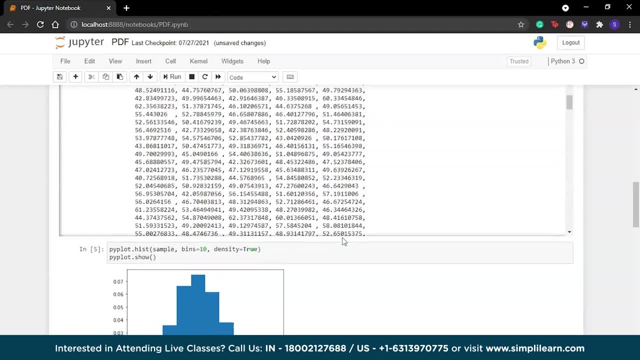 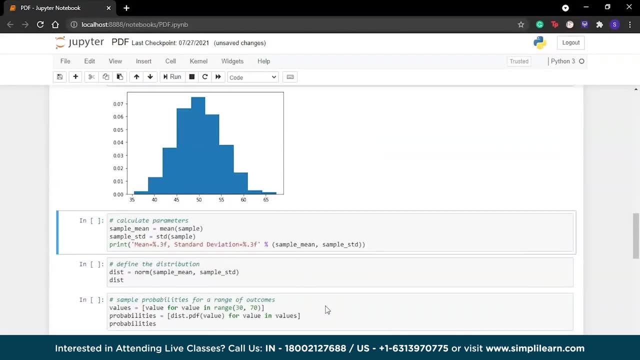 So this is what the histogram looks like, But this is just to give you a basic idea of our data and what it looks like once plotted. But let's assume that we don't know the probability distribution and we don't know what it looks like. 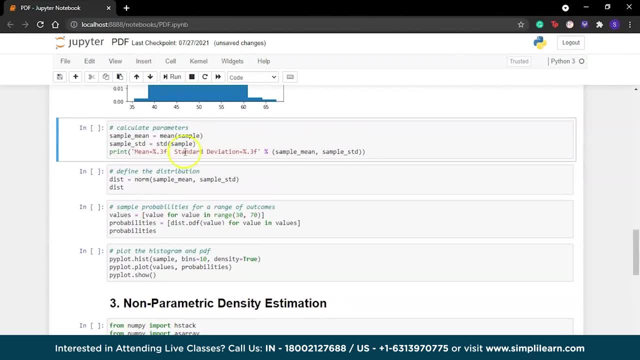 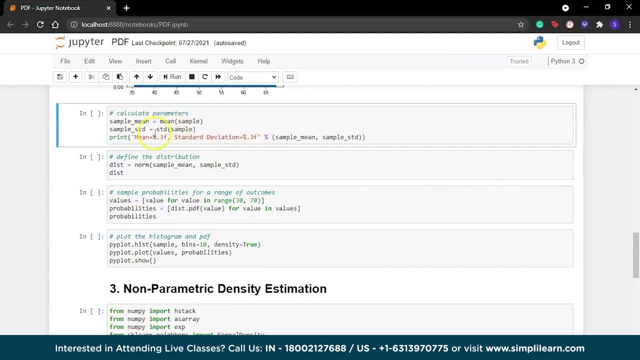 as a histogram and we don't know that it's normal. So now, if we just assume that it's normal, we can calculate the parameters of the distribution, specifically the mean and the standard deviation. We would not expect the mean and standard deviation to be 50 and 5. 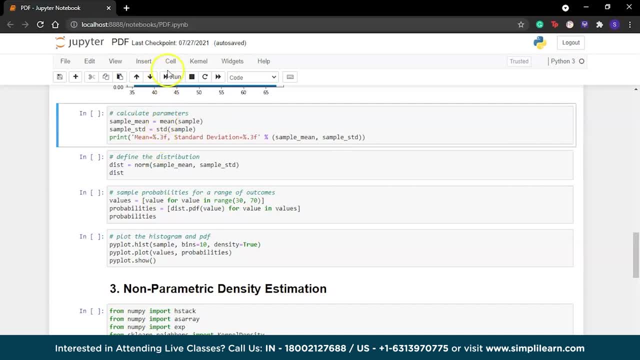 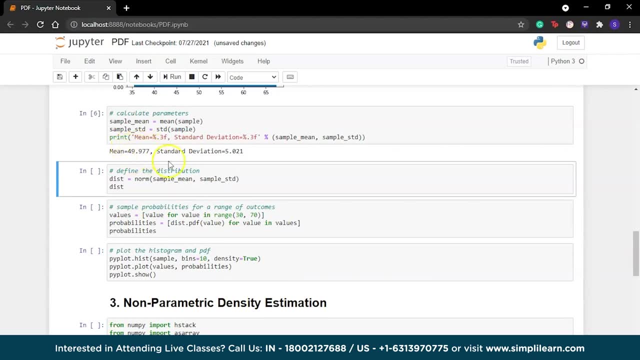 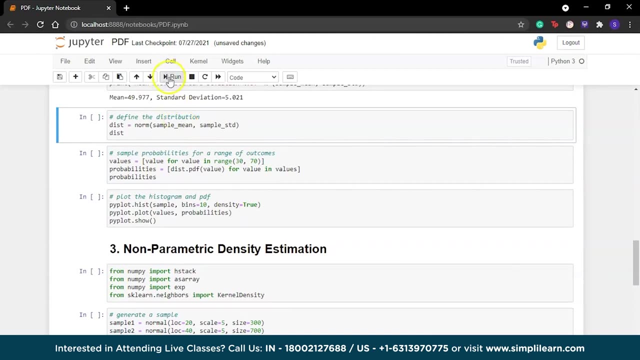 exactly, given the small sample size and the noise in the sampling data. So because of this noise and the small sample size, we have a mean of almost 50 and a standard deviation of a little more than 5.. Now let's define the distribution as: 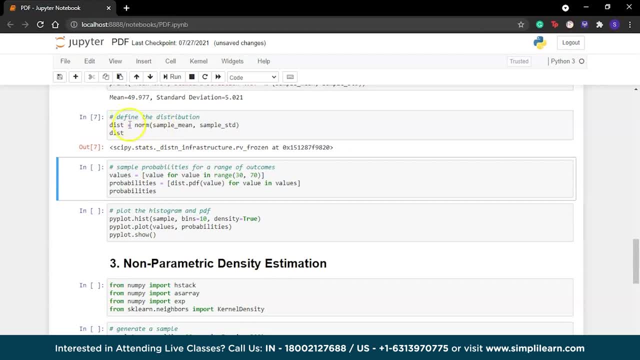 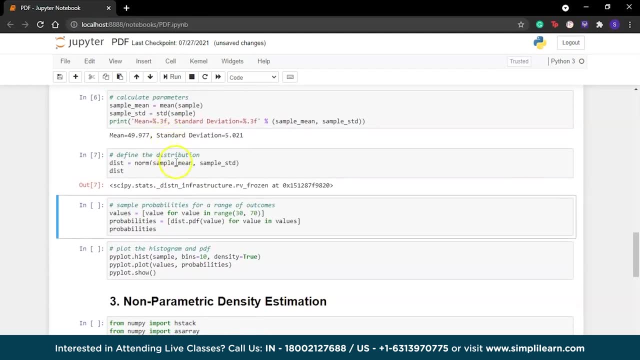 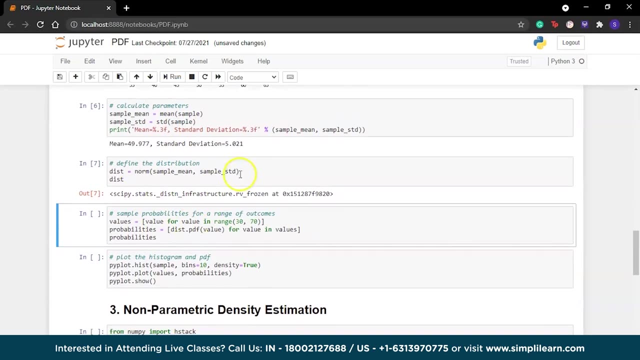 normal. So now, using this, we've defined a normal distribution, We've used the norm method of the sci-fi library, and we're doing this with the mean and the standard deviation that we've obtained from our samples. So up until now, we're just 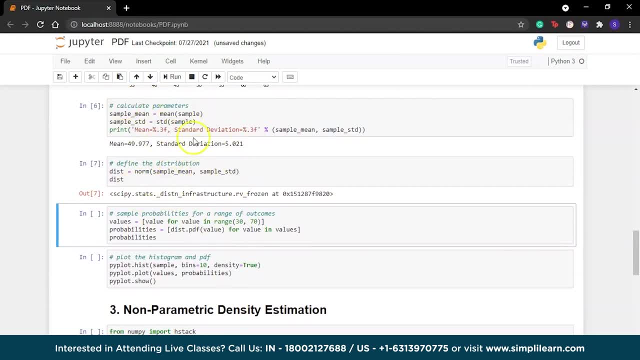 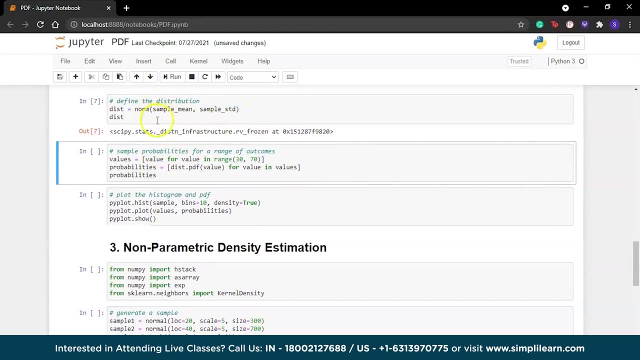 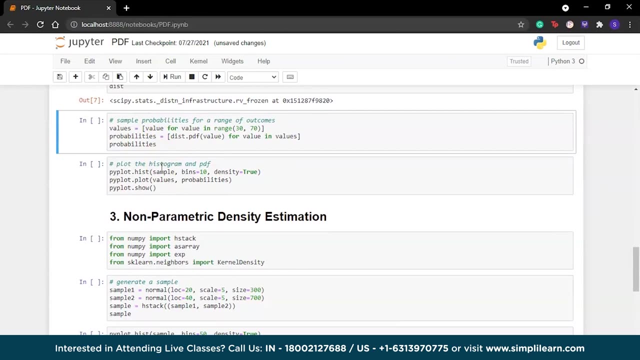 assuming that it's a normal distribution and because of that, the parameters that we've calculated is the mean and standard deviation, And using the calculated mean and standard deviation we've gotten a normal distribution. And up until now again, keep in mind, we do not know for certain. 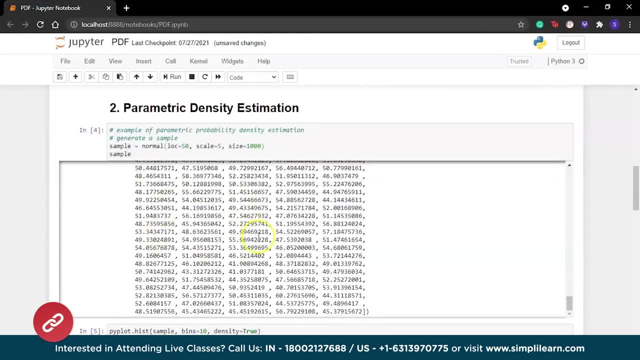 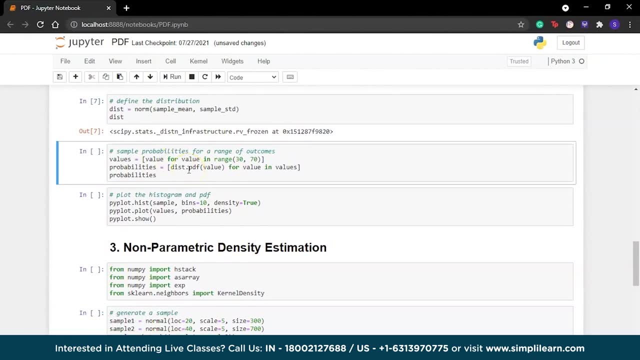 that it is a normal distribution. So far, all we have is this data, So the next thing that we're gonna do is fit the distribution with these parameters and then sample the probabilities for a distribution for a range of values in our domain, which, in this case, is: 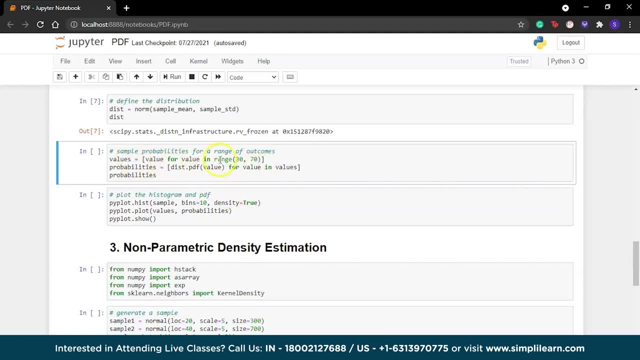 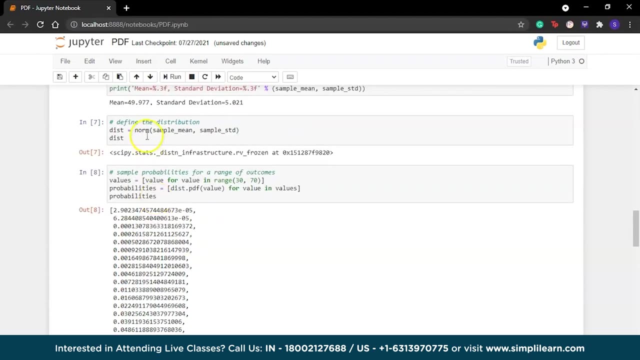 30 and 70.. So all we're doing is we're calculating probabilities for a range of outcomes and in this case we've taken 30 and 70 as our domain. So these are the probability distribution values for the normal distribution that we've defined over here. 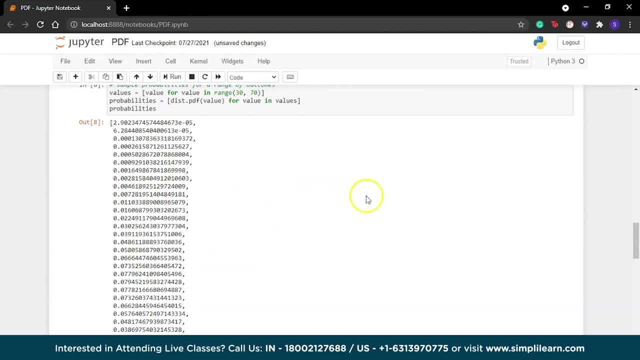 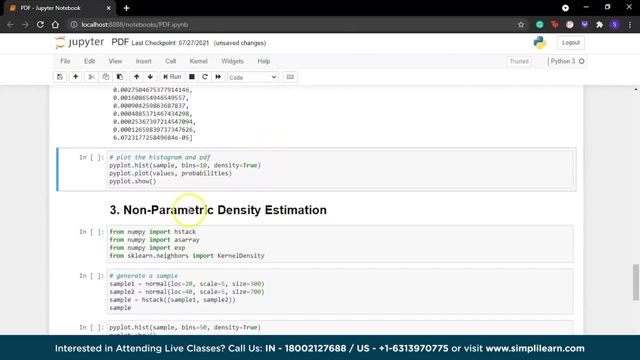 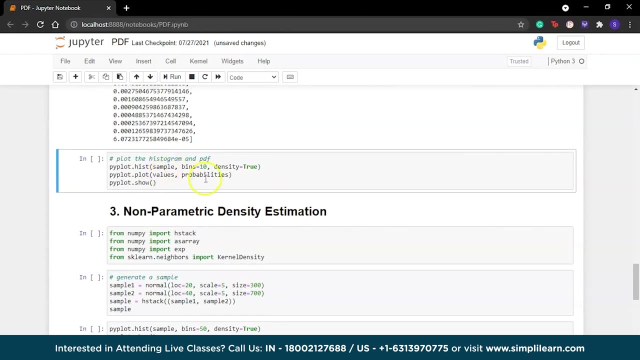 and this is gonna give you the outline of your normal distribution. These are the points at which your normal distribution will be plotted. Now, what we're basically gonna do is we're gonna plot our histograms using the samples that we've already generated, along with the values and probabilities. 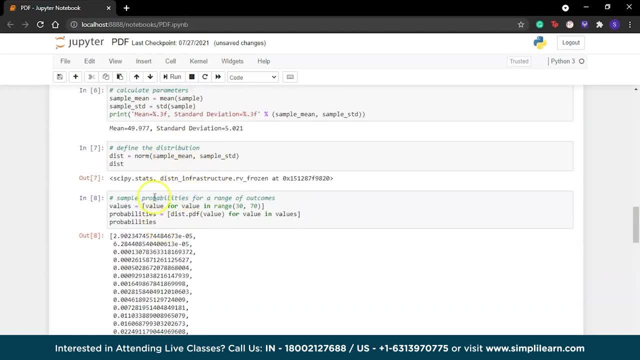 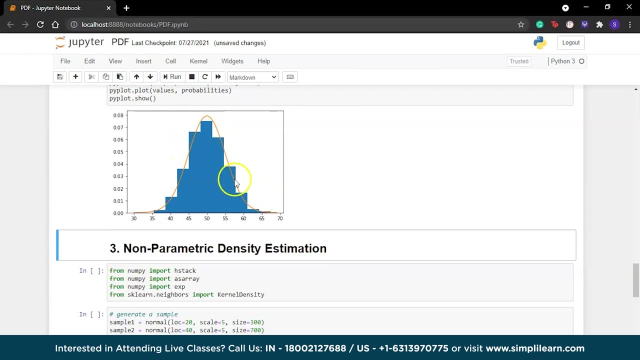 of the normal function that we defined over here. So, as you can see, it's almost a complete fit. The normal distribution that we have here is made using the mean and the standard deviation of our actual samples. The reason we took mean and standard deviation was: 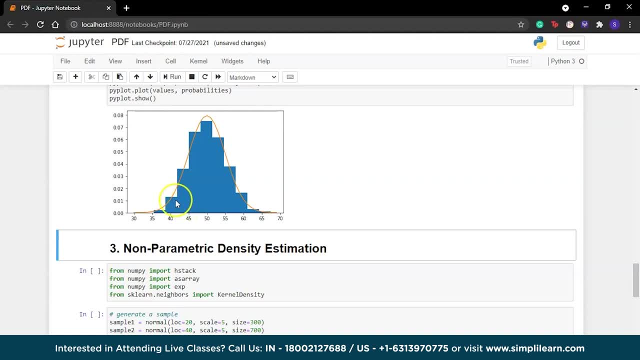 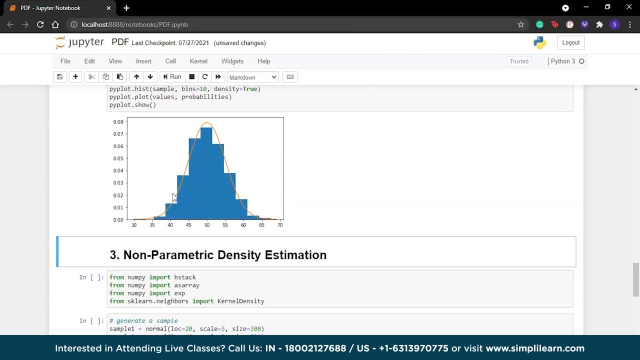 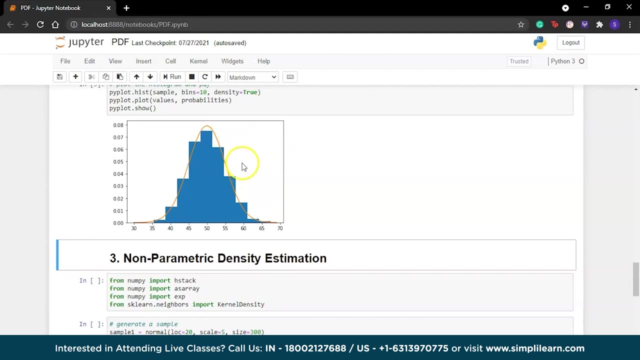 because we assumed it was a normal distribution and the parameters associated with the normal distribution are mean and standard deviation. Using the mean and standard deviation, we got the normal distribution. we calculated probabilities for this normal distribution using a random domain of 30 and 70 and we 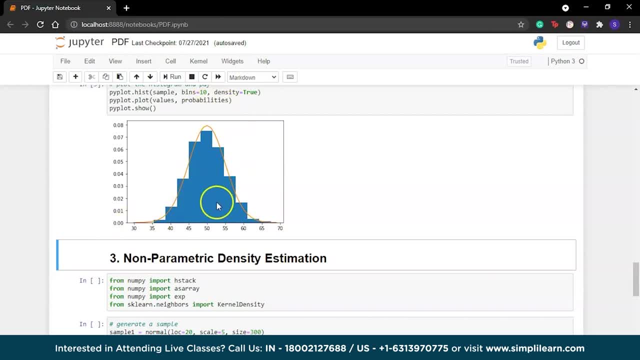 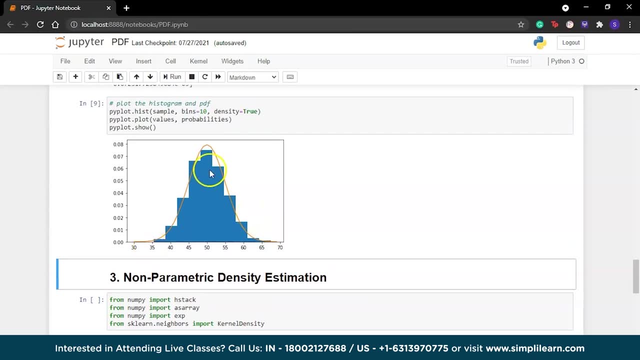 plotted the probabilities and the values on top of our histogram to see if the normal distribution was a fit to our histogram. If it was not a fit, you would have to go and do the same procedure with other common probability density functions until you found a function. 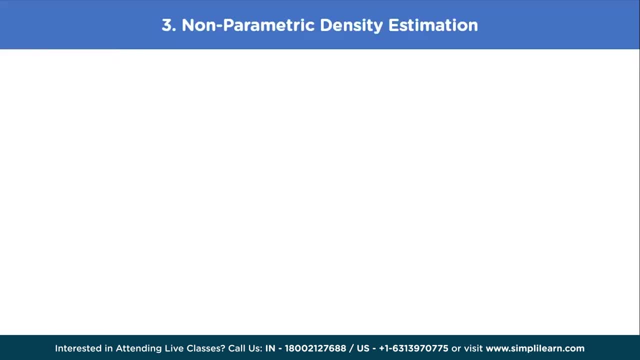 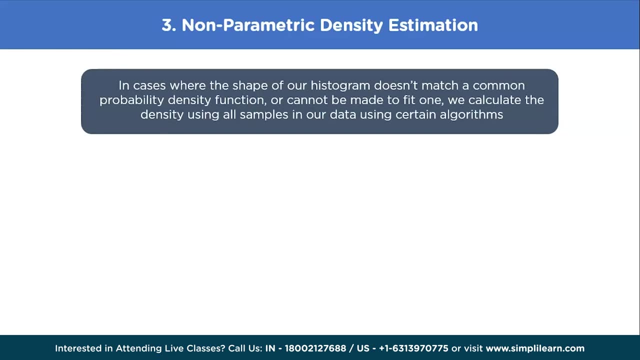 which was a proper fit to your histogram. Now let's move on to the final step, which is used in the calculation of our PDF. This final step is called nonparametric density estimation and it's only used when the shape of our histogram doesn't match a common 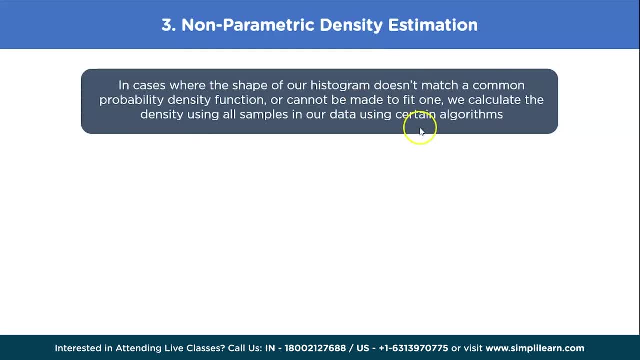 probability density function or it cannot be made to fit one. In this case, we will calculate the density using all samples in our data. using certain algorithms, This is only done when a data sample does not resemble a common probability distribution or it cannot be easily made to fit the 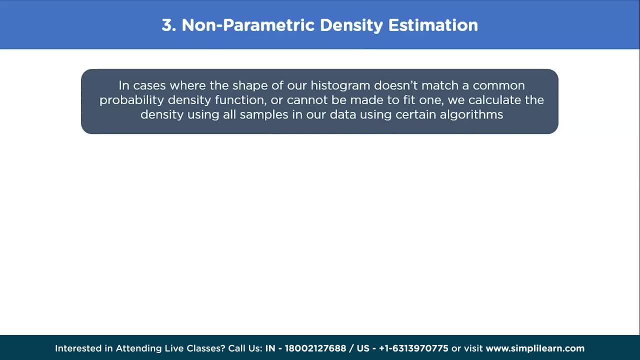 distribution. This is often the case when the data has two peaks- this is also called a bimodal distribution- or it has many peaks, which is also called a multimodal distribution. In this case, the parametric density estimation will not be feasible and alternative methods can be. 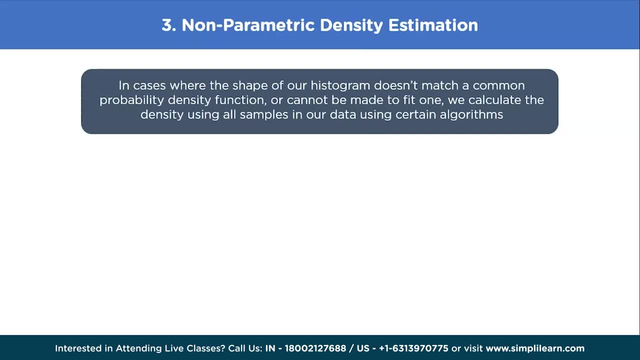 used that do not use a common distribution. Instead, you will use an algorithm which is used to approximate the probability distribution of the data without a predefined distribution, which is also referred to as a nonparametric method. because we are not using any predefined parameters, The distribution will still have. 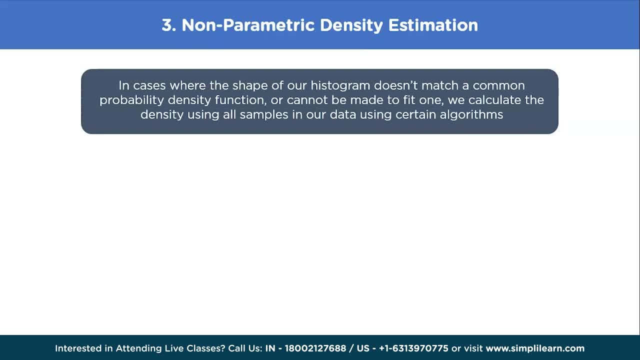 parameters, but these are not controllable in the same way as a simple probability distribution, For example. a nonparametric method might estimate the density using all observations in a random sample, in effect, making all observations in the sample parameters. Now consider this graph, which has: 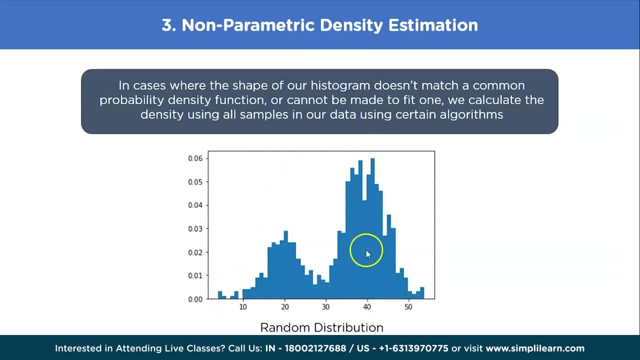 two peaks. This is not a normal distribution or any other sort of distribution that we are familiar with. So for this we are not going to use a parametric estimation method, but which is going to calculate the parameters for every single sample point in this. 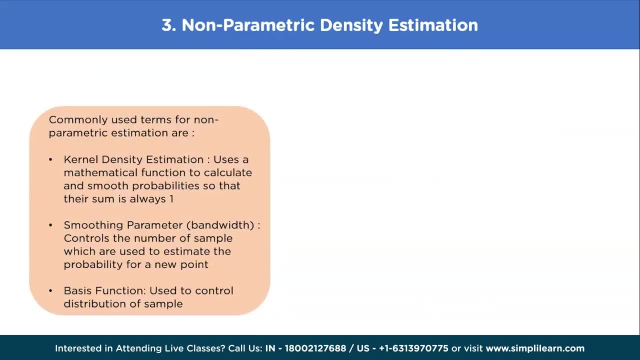 Perhaps the most common nonparametric approach for estimating the probability density function of a continuous random variable is called kernel smoothing or kernel density estimation, or KDE for short. Kernel density estimation is a nonparametric method for using a dataset to estimate probabilities for new data points. 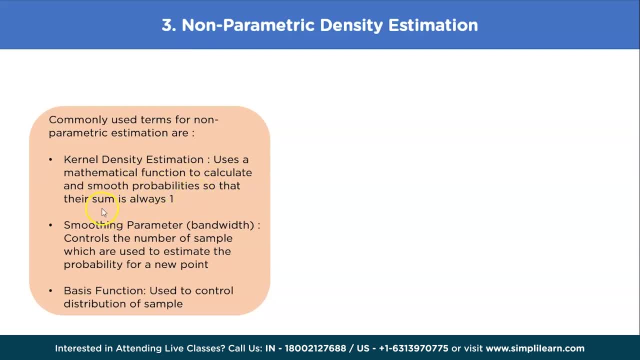 It uses a mathematical function and smoothing probabilities, so the sum of the resultant probabilities is always 1.. Now, in this case, a kernel is a mathematical function that returns a probability for a given value of a random variable. The kernel effectively smooths or interpolates. 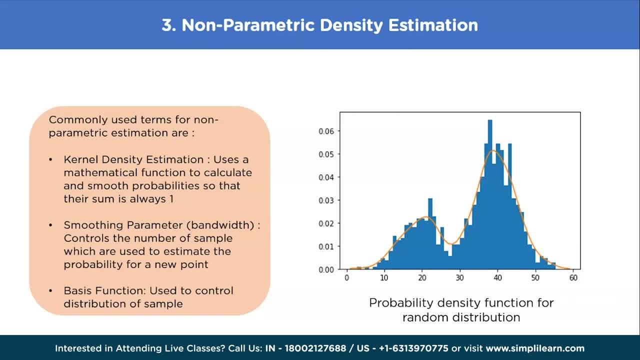 the probabilities across the range of outcomes for a random variable, such that the sum of probabilities always equals 1. A requirement of well behaving probabilities. You also have a parameter called the smoothing parameter, which controls the scope or the window of observations from the data samples. 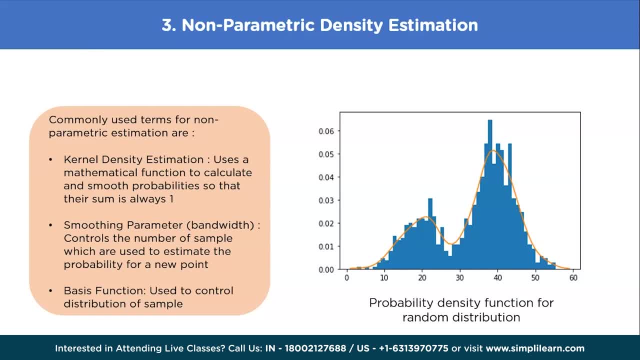 that contributes to estimating the probability for a given sample. As such, the kernel density estimation is sometimes referred to as your Parzen-Rosenbald window. Now, at the end, you also have a basis function, which is a function which is chosen to control the contribution of. 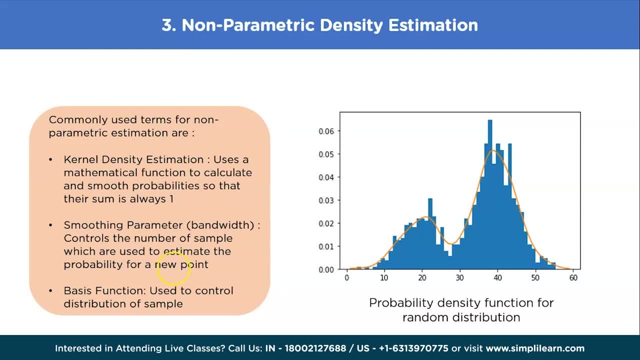 samples in the dataset towards estimating the probability of a new point. This is only done to make sure that you are not learning from a lot of noise and that you are not using a lot of the outliers. Again, let's see how we can perform nonparametric density estimation. 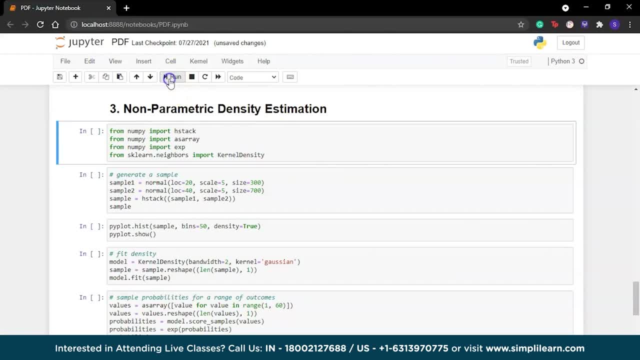 with the help of python. So first we will start by importing all the necessary modules, along with the kernel density estimation, which can be imported from sklearn. Now let's create a bimodule distribution by combining two different samples, sample 1 and sample 2.. 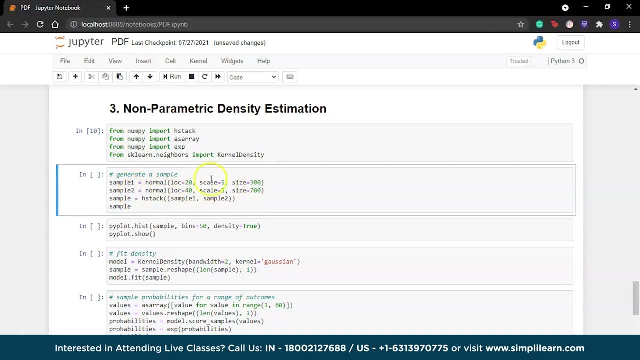 Sample 1 has 300 examples, with a mean of 20 and a standard deviation of 5, while sample 2 has 700 examples, with a mean of 40 and a standard deviation of 5.. We are then going to use hstack to 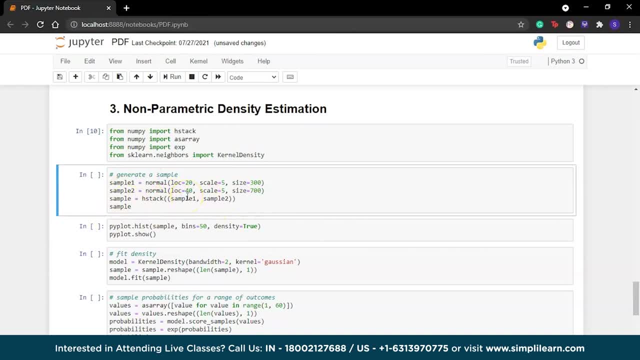 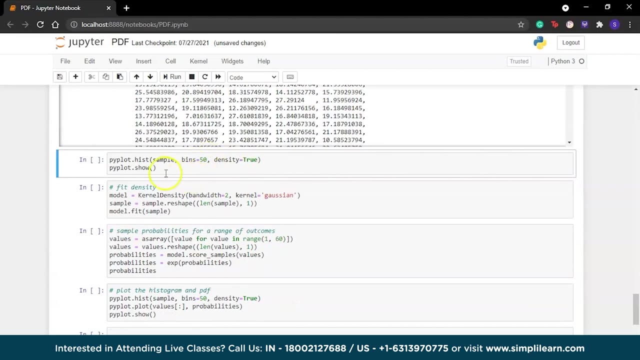 merge both of them together to get a final sample. The means that we have chosen, which is 20 and 40, are chosen close together to ensure that the distributions overlap in the combined sample. So this is what our distribution is. Let's just plot it. 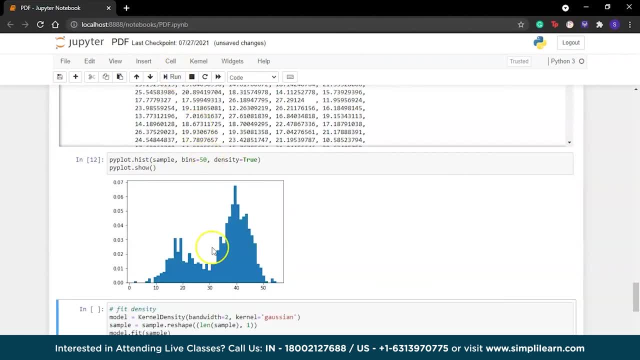 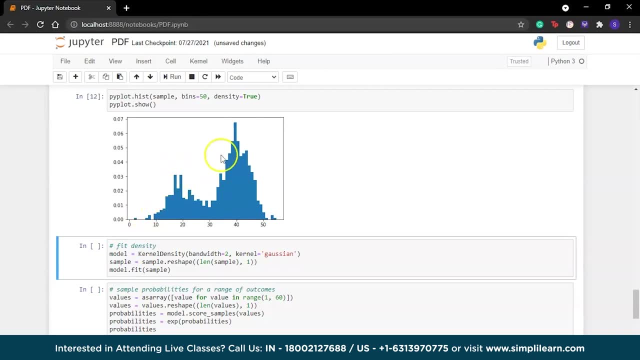 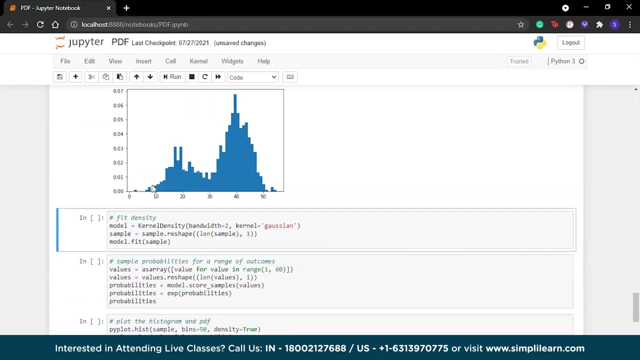 so you get a basic idea of what our graph looks like. So this is what our graph looks like. Now we already know that none of the various different probability distribution functions fit these graphs, So now we are going to perform non-parametric estimations. 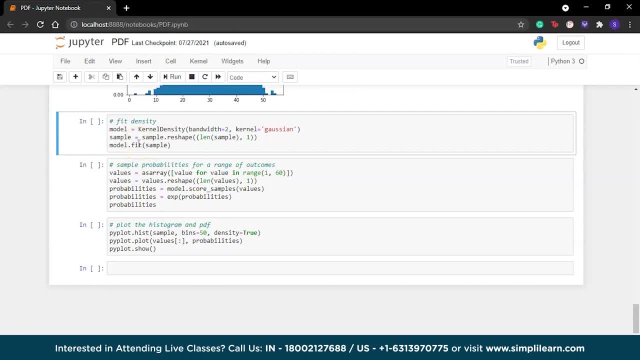 To perform non-parametric estimations, we are going to use the scikit-learn machine learning library, which provides the kernel density class that implements kernel density. sorry, that implements kernel density estimation. First, the class is constructed with the desired bandwidth or window size of 2.. 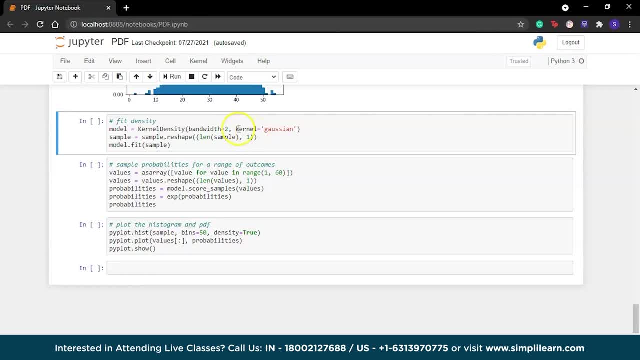 And your basis function, which in this case is a Gaussian function. It's a good idea to at least test different configurations to your data, and in this case we are only going to try a bandwidth of 2 and a Gaussian kernel, But usually there are multiple different. 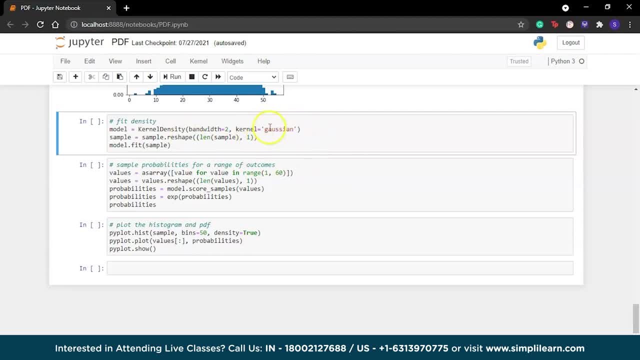 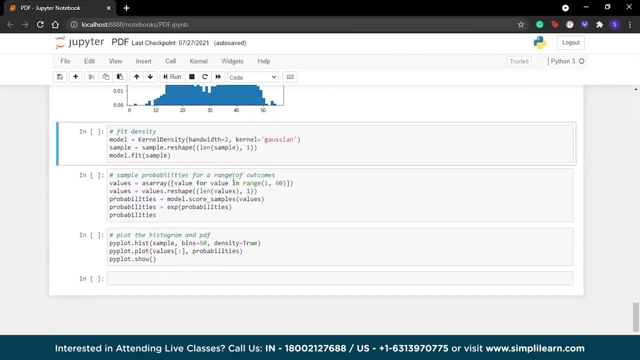 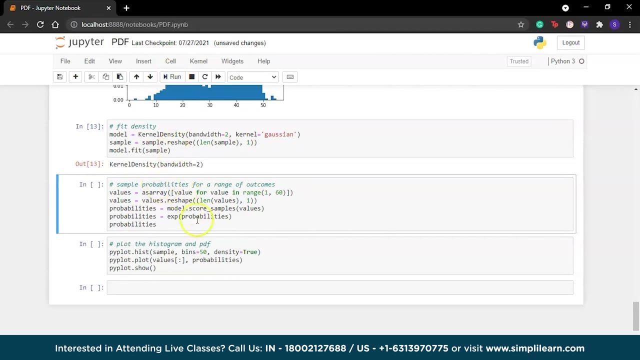 kernels that you can play around with, and you can also tweak your bandwidth to exactly fit the distribution that you have. Now let's run this. So now we have gotten our kernel density estimation. Now we can evaluate how well the density estimates matches our data by calculating. 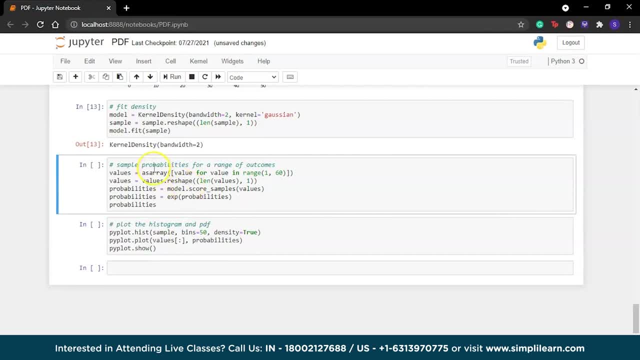 probabilities for a range of observations and comparing shapes to the histogram, Just like we did for the parametric case before. So again, we are going to just calculate different probabilities using the kernel density function And we are just going to plot it on top of our 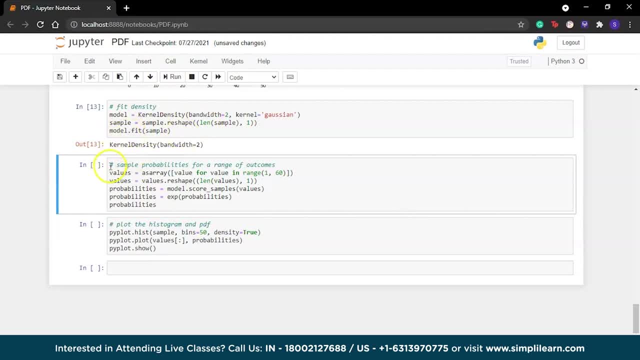 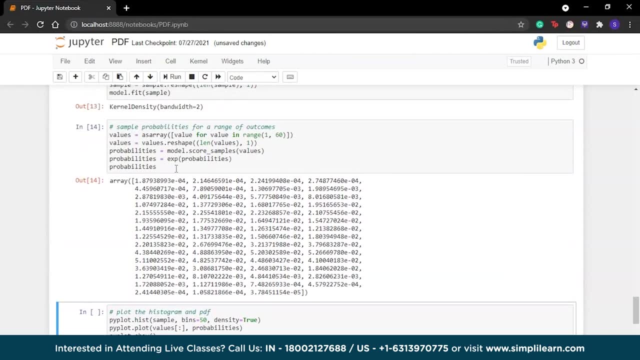 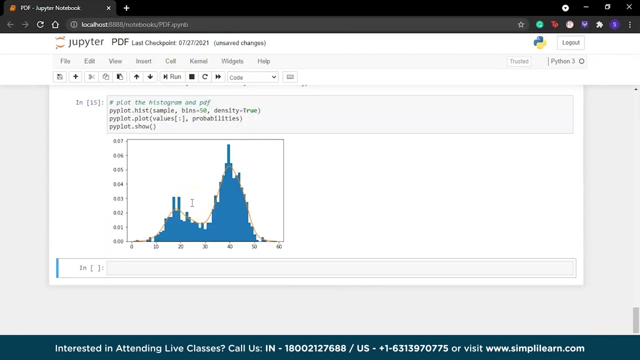 histogram to see how well this, the kernel density function, is estimating for our data. So these are the probabilities that we have gotten finally with the kernel density estimation And now we are going to plot it on top of our histogram. As you can see, it's almost a complete 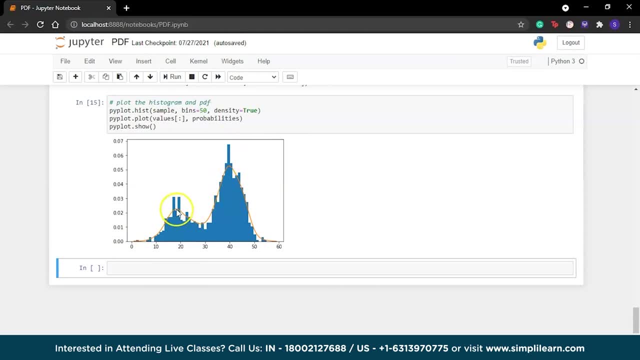 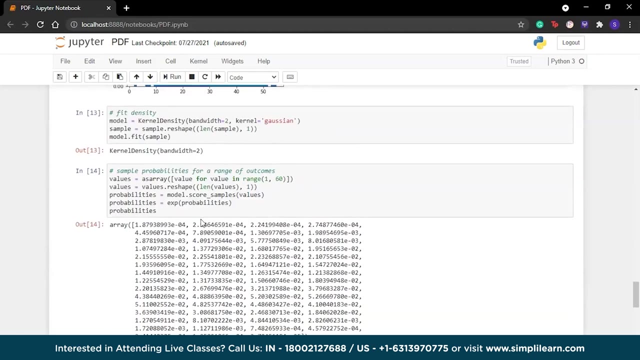 fit. It's just left out some of these outlier values, which again are ranging very high, But overall we have a pretty good fit. So the only problem is it's not very smooth and you can again try tweaking the bandwidth to different values. So let's just, in this case, try tweaking. 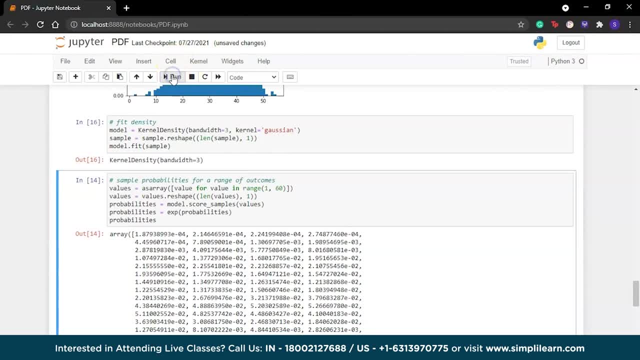 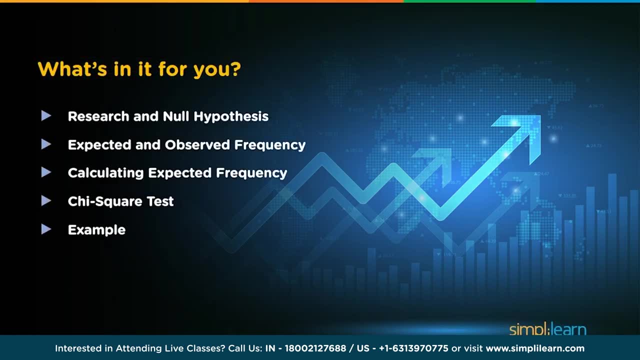 it to 3 and see how well it runs. In this video we will be discussing the chi-square test. We will start by defining what is research and null hypothesis. Then we will move on to learn about observed and expected frequencies. You will see. 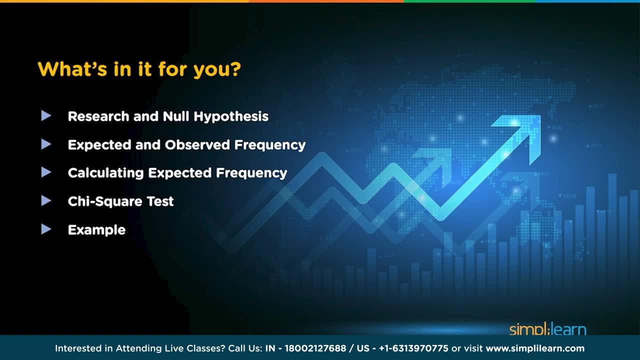 how you can calculate the expected value using a formula. Then we will move on to chi-square statistics. We will learn its limitations, its formula and its basic concept. After grasping every theoretical knowledge. we will discuss an example, step by step, to see. 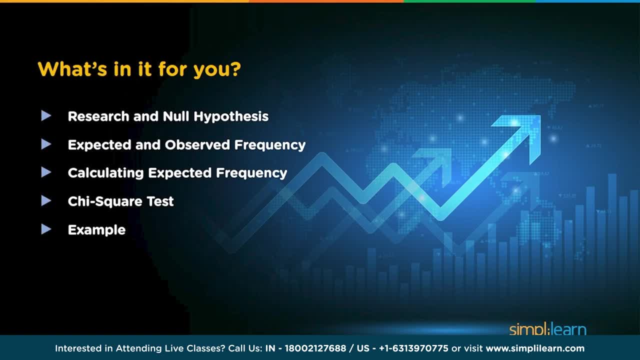 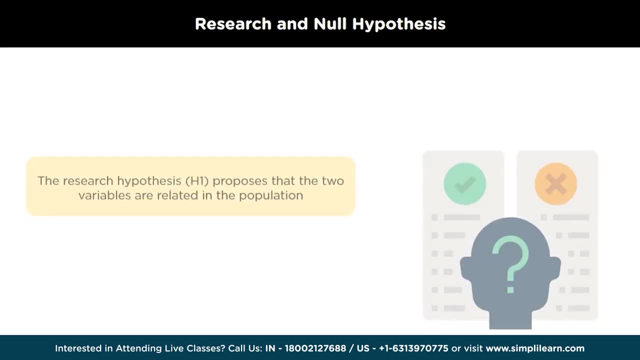 how you can calculate the chi-square statistics and the conclusion you can draw from the calculated value. So let's get started. Research and null hypothesis. The research hypothesis, which is also denoted by H1, says that the two variables are related: in the population, The 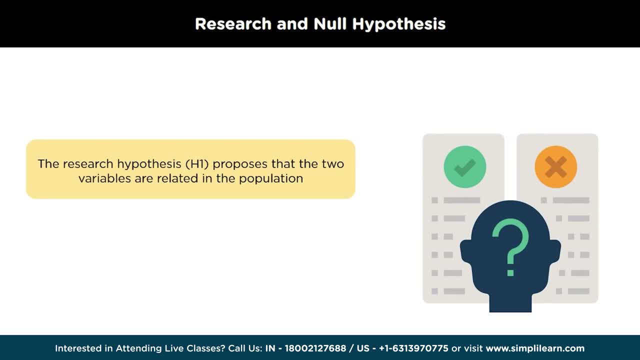 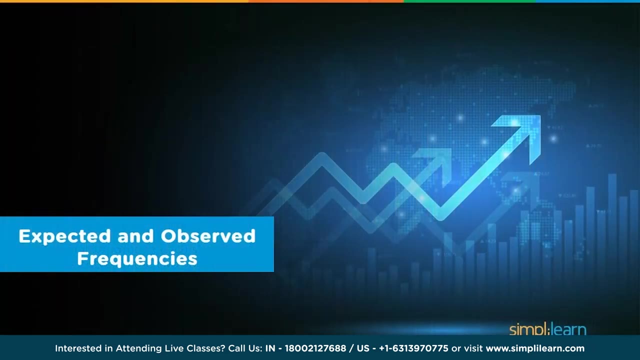 acceptance of the research hypothesis follows the rejection of the null hypothesis. The null hypothesis H0 says that there is no association between the two variables and they are statistically independent. The null hypothesis has no bearing on the study's outcome unless it is rejected. Now let's define expected and observed frequencies. 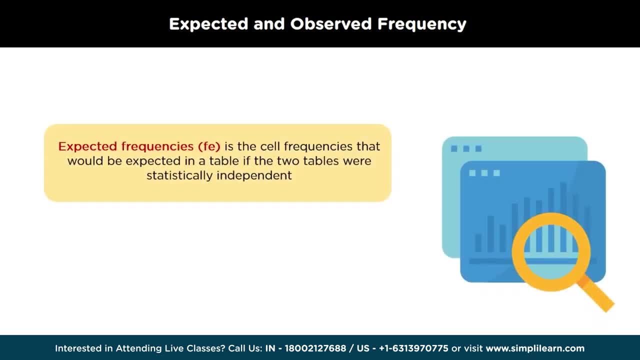 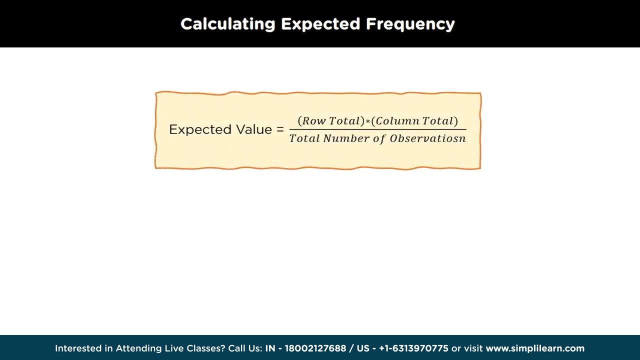 Expected frequencies are the value that we would get if the two tables were statistically independent. The expected values are calculated based on our null hypothesis. The observed frequencies are those frequencies that we gather ourselves from our observation. To calculate the expected frequency, we have a 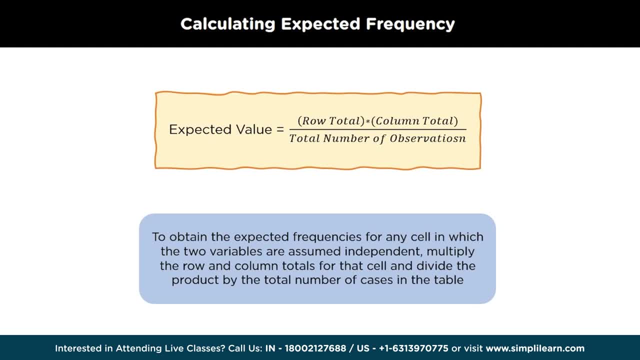 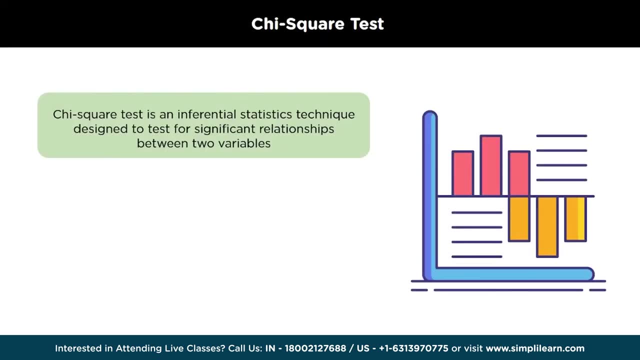 direct formula: We multiply the row total by the column total and divide the whole value by the total number of observations. Now let's move on to chi-square test. The chi-square test is a statistical procedure for determining the difference between observed and expected data. 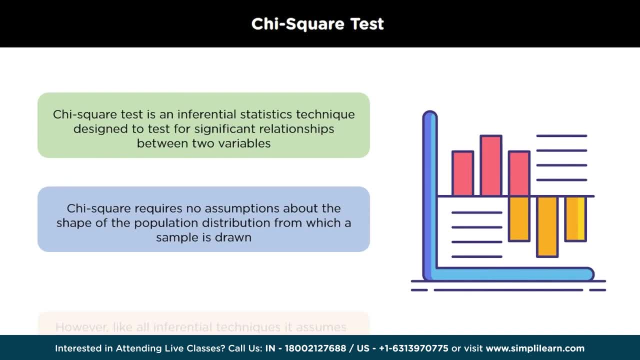 This test can also be used to determine whether categorical variables in our data are correlated. It helps to find out whether a difference between two categorical variables is due to chance or a relationship between them. The chi-square test required no assumption about the shape of population. 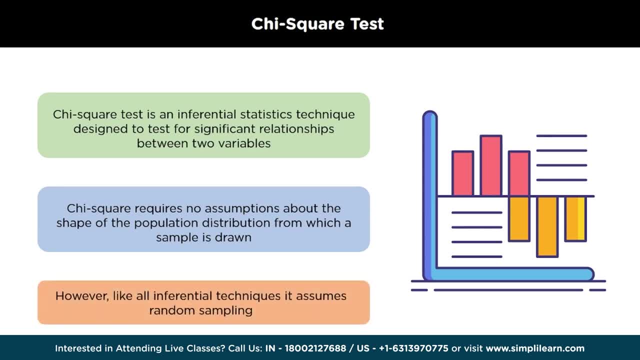 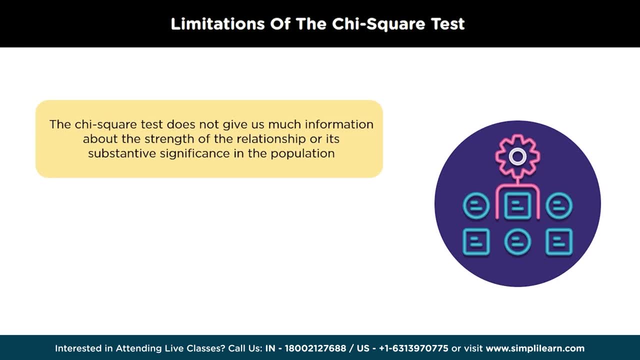 distribution from which the sample is drawn. However, like all inferential techniques, they assume the random sampling. The chi-square test do have some limitations. Firstly, the chi-square test does not give us much information about the strength of the relationship or its 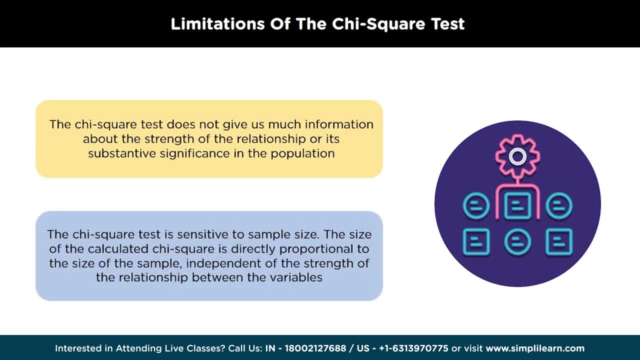 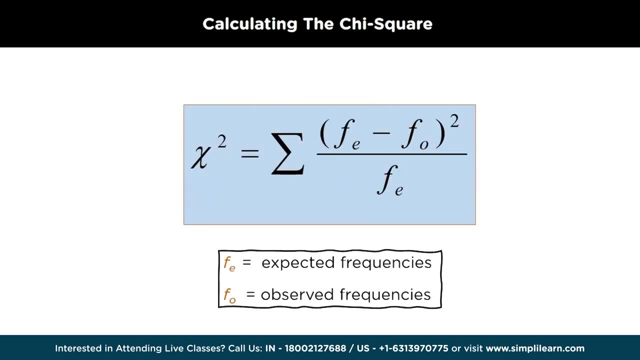 significance in the population. The chi-square test is also sensitive to sample size. The calculated chi-square statistics is directly proportional to the size of the sample, which is independent of the strength of the relation between the variables. So to calculate the chi-square statistics, we have a direct formula. 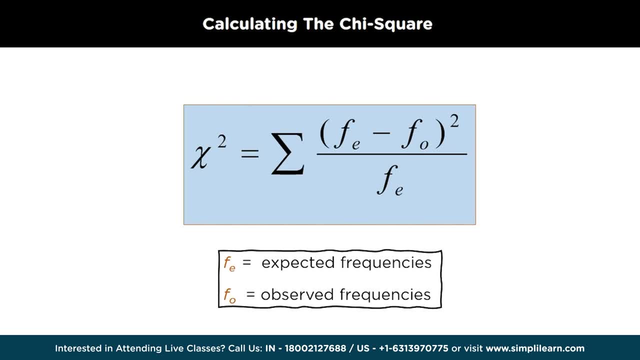 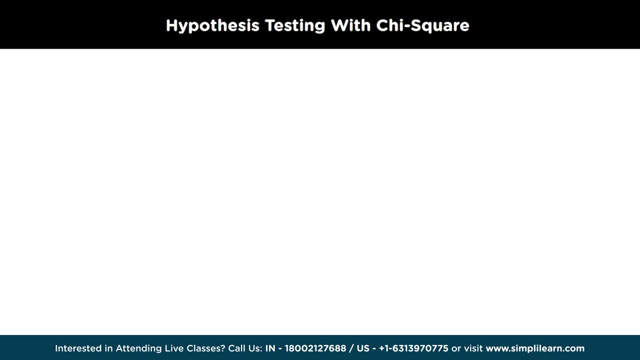 The chi-square statistics, which is also denoted by x. square is equal to summation of expected frequencies minus observed frequencies, whole square divided by expected frequencies. The chi-square test statistics follow these five steps. First, we make assumptions about random sampling and state its research and 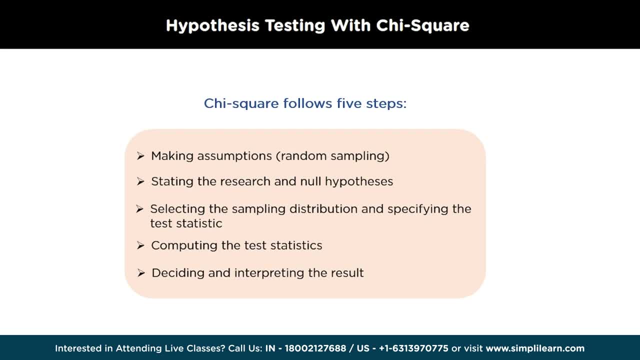 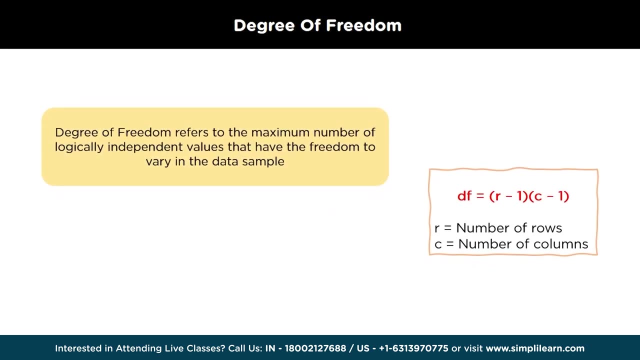 null hypothesis, Then we select the sampling distribution and specify the test statistics, and after that we compute the test statistics. The value we get is used to decide and interpret the results. Degree of freedom: The degree of freedom is a statistical calculation which represents the number of variables that 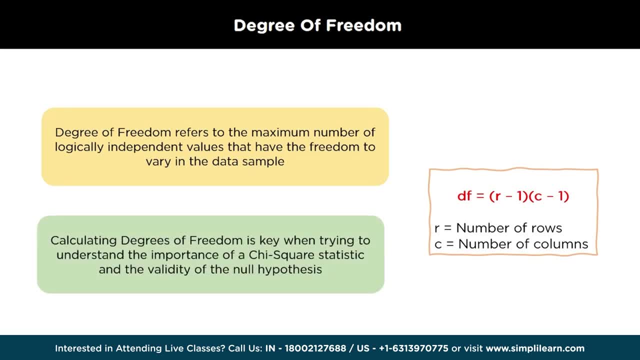 can vary in a calculation. The degree of freedom can be calculated to ensure that the chi-square test is statistically valid. These tests are frequently used to compare observed data with the data that would be expected to be obtained if a particular hypothesis were true. The formula to calculate: 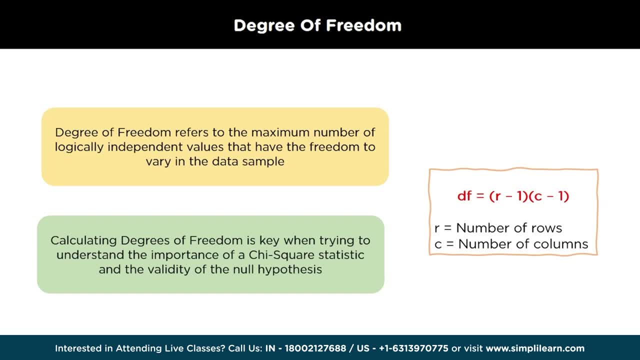 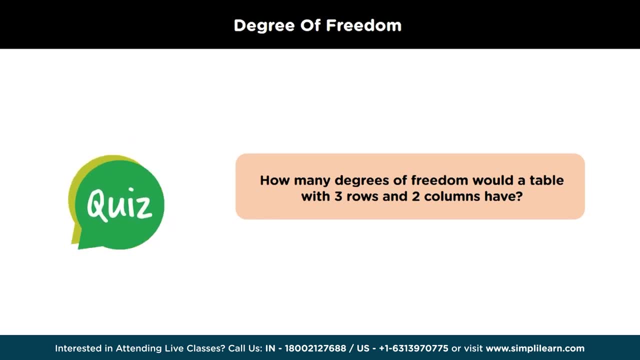 degree of freedom is number of rows minus one multiplied by number of columns minus one. So, after knowing the formula, we have a question for you: How many degree of freedom would a table with three rows and two columns would have? Post your answers in the comment section. 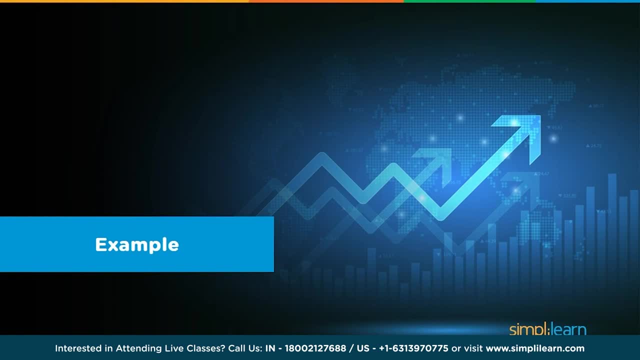 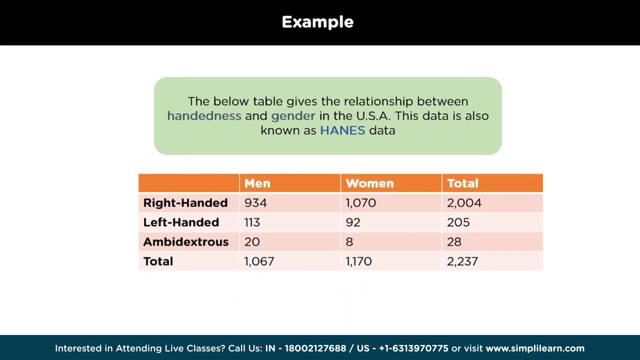 Now that we have learnt all the theoretical concepts regarding chi-square test, let's understand this more clearly with the help of an example. Let's say we want to know if the gender has anything to do with the handedness of the people. We have the data of. 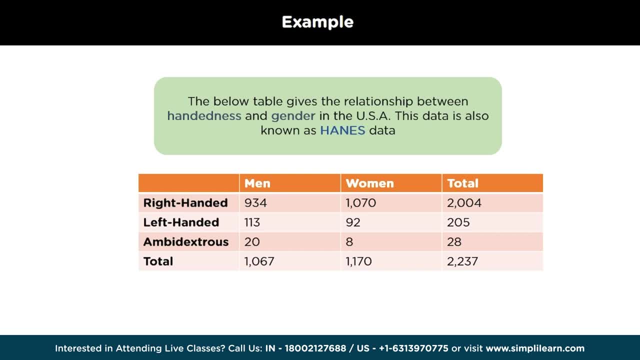 2237 people in a simple random sample to find out if they are left-handed, right-handed or both. The results of the survey are shown in the table below. To see if the gender is related to handedness, we perform the chi-square test. 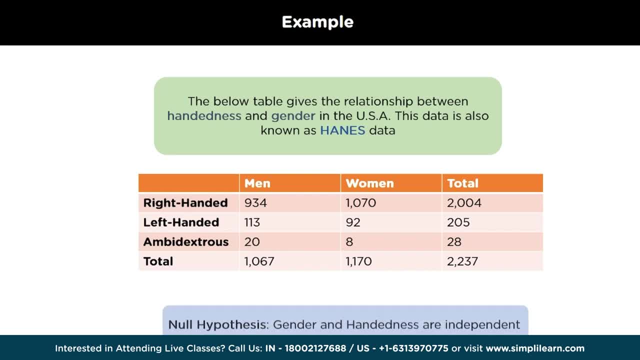 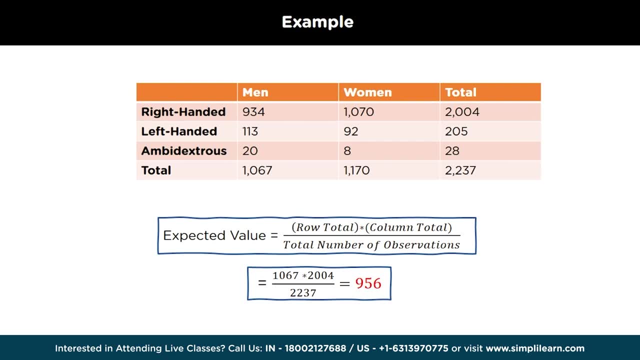 The first step is to define the null hypothesis. The null hypothesis says that the gender and handedness are independent to each other. The next step is to calculate the expectation values. The expected value is calculated using the formula that is shown in the slide. 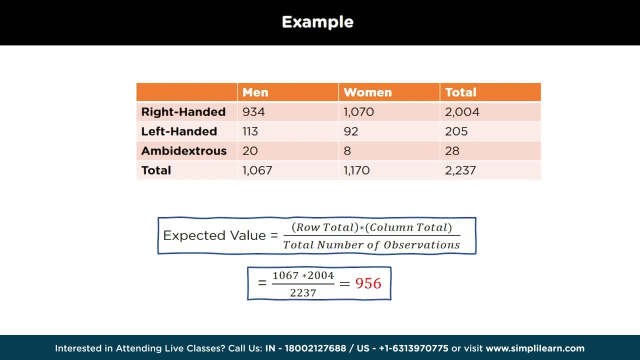 Which is row total, into column total divided by the total number of observations. For example, the expected value of a right-handed man can be calculated by multiplying 1067 into 2004, divided by 2237, which comes out to be 956.. 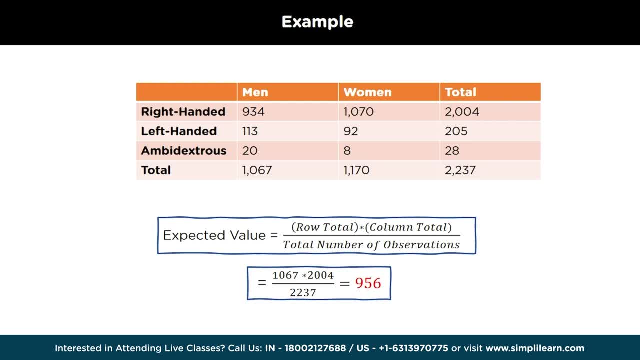 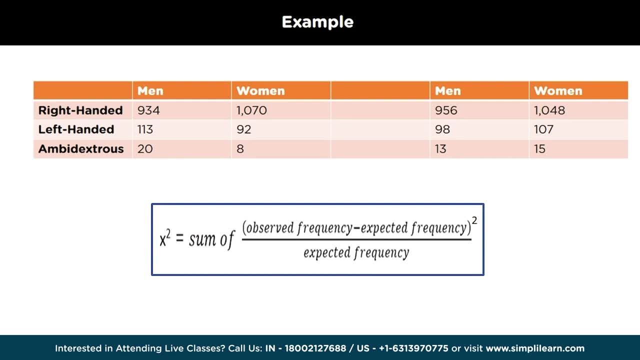 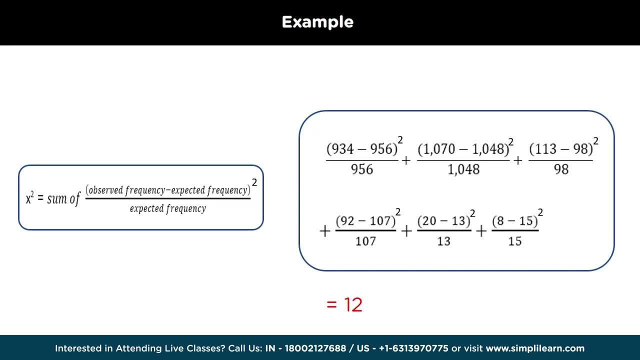 In a similar manner, you can calculate the expected value for each of the cell. After calculating the expected value, we calculate the value of x-square. x-square is calculated by the following formula: Observed frequency minus expected frequency, whole square divided by expected frequency. 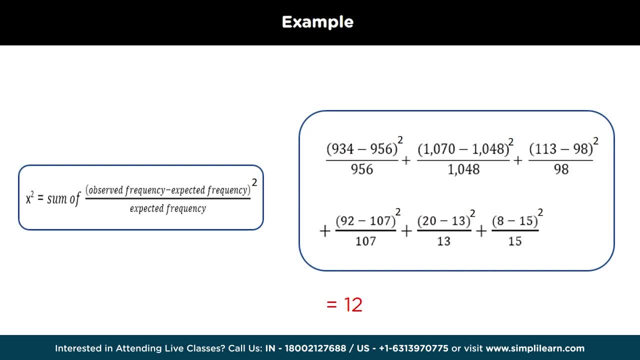 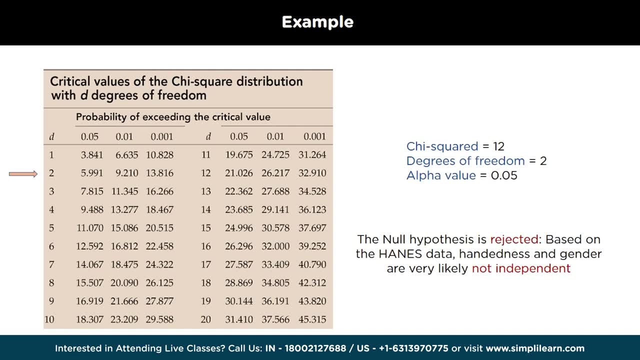 By putting the values in the formula, we get the x-square value to be 12.. Now we got our x-value, which is also the chi-square value, to be 12, and the degree of freedom is equal to 2., Which is calculated by: 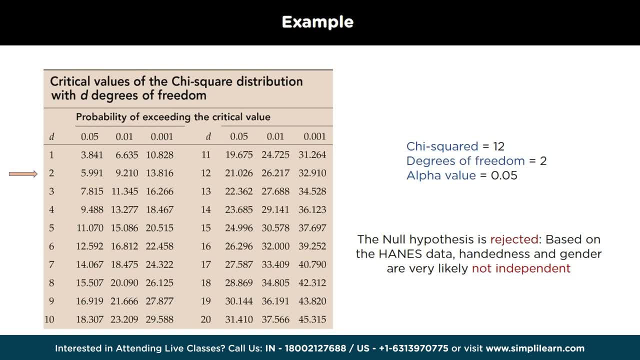 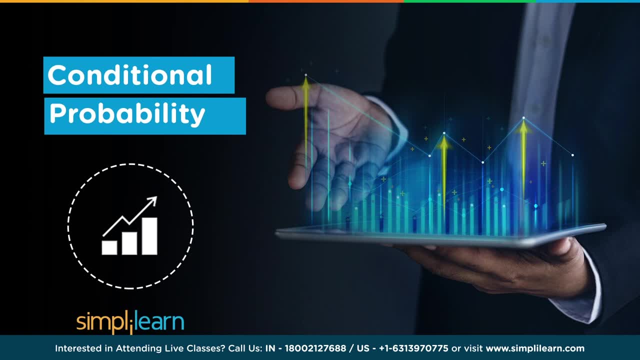 R-1 into C-1, where R and C were rows and columns respectively. We will be discussing conditional probability, which is one of the most important areas in probability theory. We will start by talking about random experiments and then move on to events and sample space. 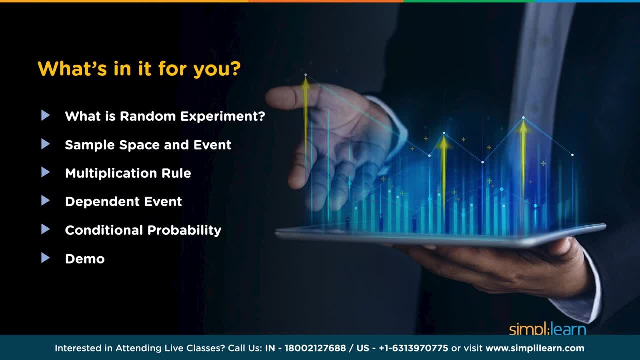 Then we will try to understand the multiplication rule with the help of an example. After that, we will learn about dependent events and the multiplication rule associated with them. After that, we will learn about conditional probability with the help of an example. So let's get started. 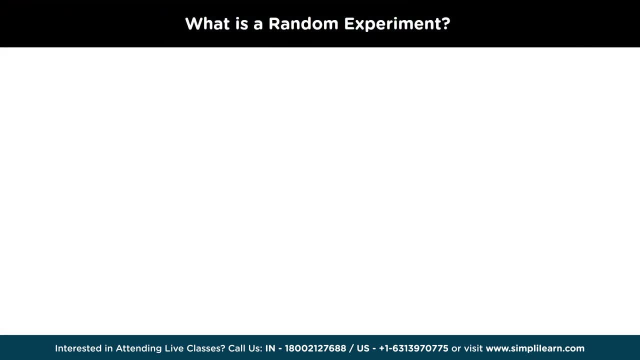 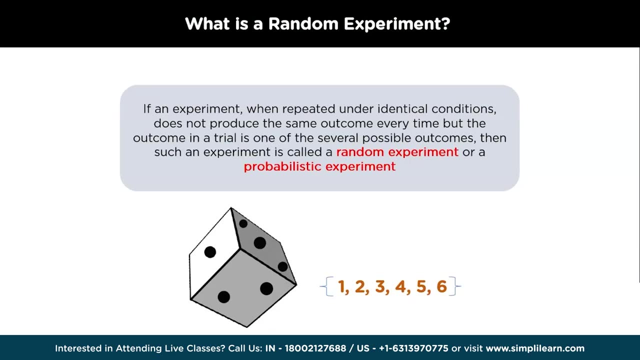 What is a random experiment? Let's say that you roll a fair die and there are 6 possible outcomes. You can get a number from 1 to 6. But it is impossible to accurately predict the outcome. In mathematical theory, we consider only those. 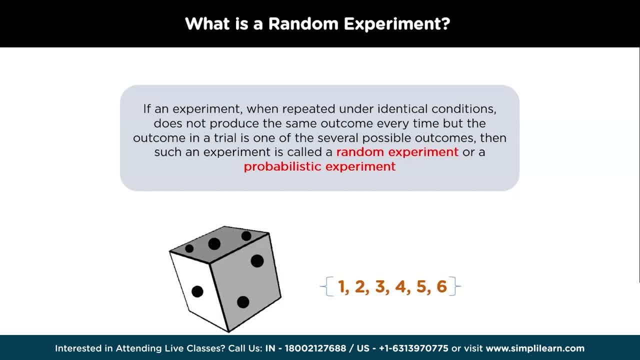 experiments or observations for which we know the set of possible outcomes. Also, it is important that predicting a particular outcome is impossible. Such an experiment, where we know the set of all the possible results but find it impossible to predict any one particular execution, is a random experiment. 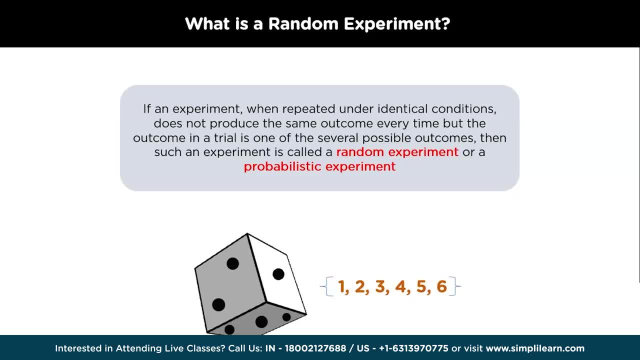 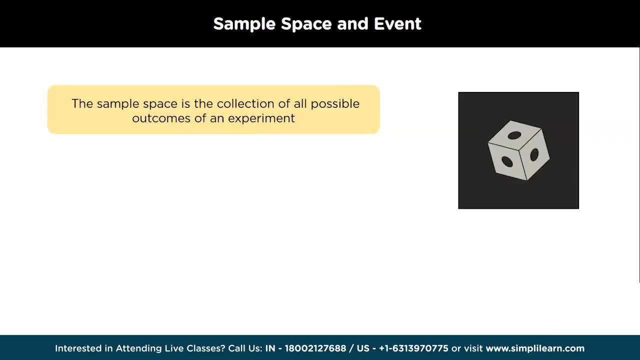 Even if a random experiment is repeated under identical conditions, the outcomes or results will fluctuate randomly. Sample space and events. The sample space associated with a random experiment is the set of all the possible outcomes. Suppose you roll a die, So the sample space for a single throw-up die. 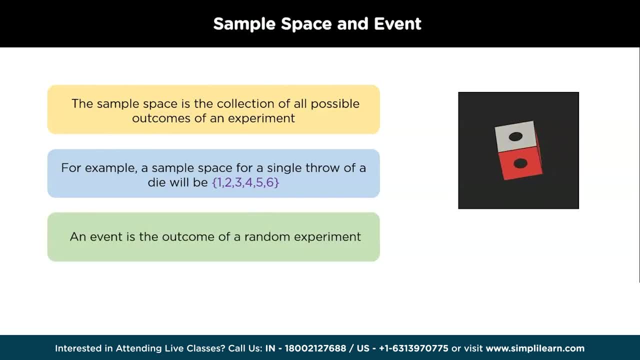 will be 1,, 2,, 3,, 4,, 5 and 6.. An event is a subset of the sample space, or you can say it is an outcome of a random experiment. Getting a heads when we toss a coin is an event. 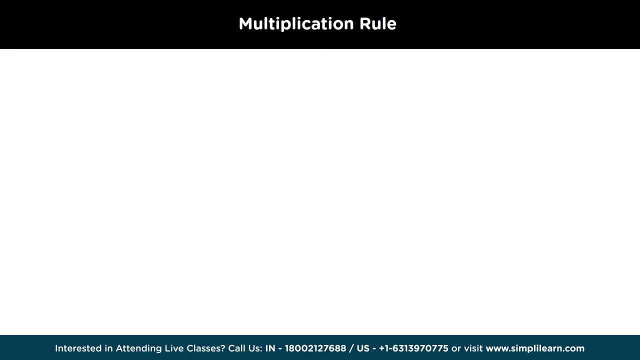 Let's discuss about the multiplication rule. in probability, The multiplication rule says that when two events are independent, the probability of both occurring simultaneously is given by probability of A. intersection B will be equal to probability of A into probability of B. Let's understand this with the help of an example. 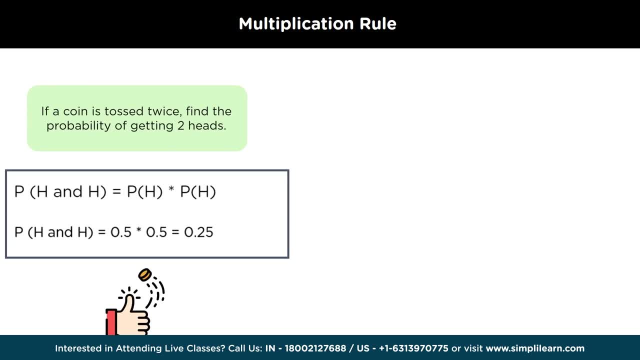 If a coin is tossed twice, what will be the probability of getting two heads? So in a single throw, the probability of getting a heads is 1 by 2, ie 0.5. So the probability of getting the two heads 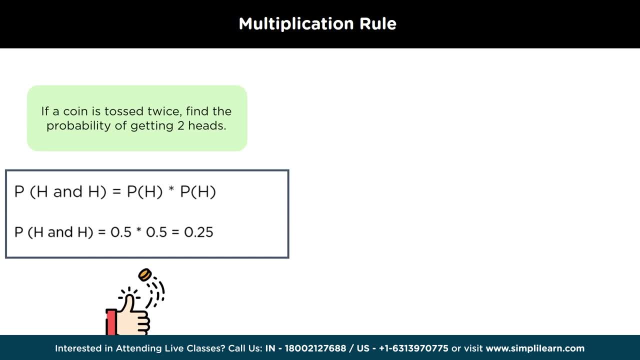 in both the coins will be 0.5 into 0.5, which will be equal to 0.25.. Let's look at another example. Suppose a coin is flipped and a die is rolled at the same time. So what will be the probability of? 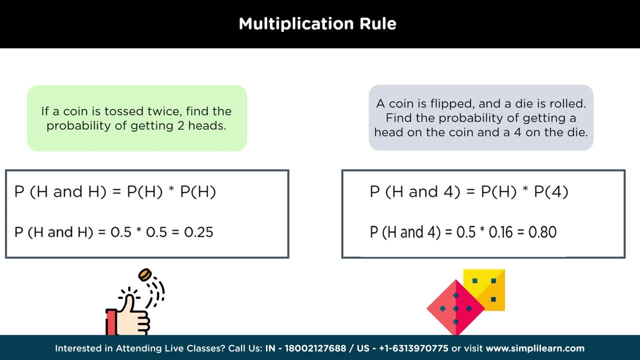 getting a head on the coin and 4 on the die. So the probability of getting a heads, as discussed in the previous example, will be equal to 0.5 and the probability of getting a 4 on a single throw-up die will be 1 by 6. 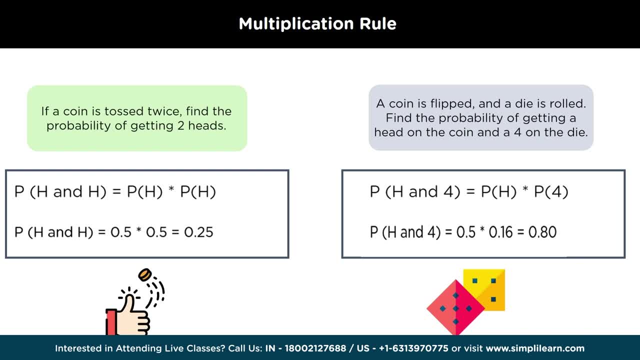 since there are 6 sample space. So the probability of getting a head on a coin and 4 on a die will be equal to 0.5 into 0.16, which will come out to be 0.80. Now let's move on to dependent events. 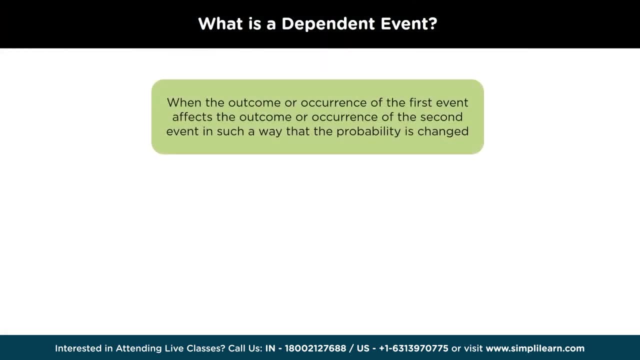 Two events are said to be dependent if the outcome of the first event affects the outcome of the second event, so that the probability is changed. Let's understand this with the help of an example. Let's understand this with the help of an example. Suppose you have a deck of cards. 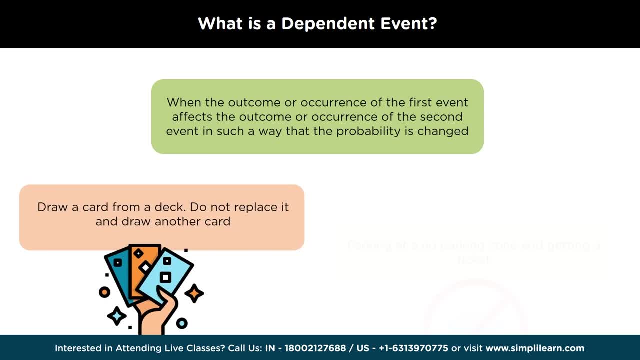 The probability of drawing a card from a deck of cards is 1 by 52. Now, if you do not replace the card, the probability of drawing another card changes to 1 by 51.. Another example of it can be parking at a no parking zone. 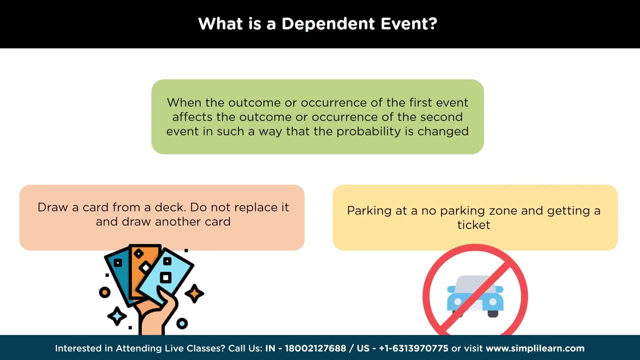 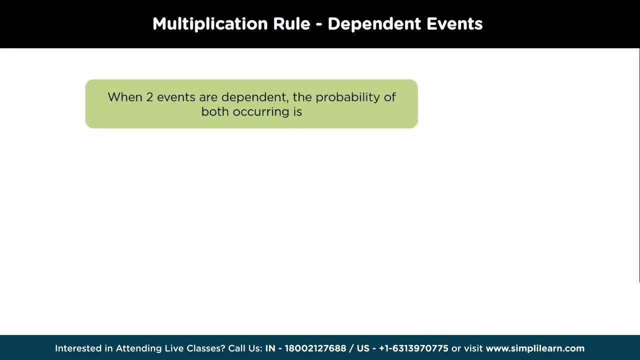 and getting a ticket. When you park at a no parking zone, the probability of getting a ticket increases. There is a multiplication rule associated with the dependent events. It says that when the two events are dependent, the probability of both occurring is given by this formula. 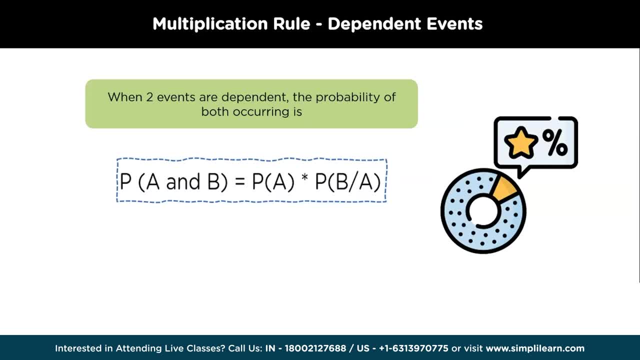 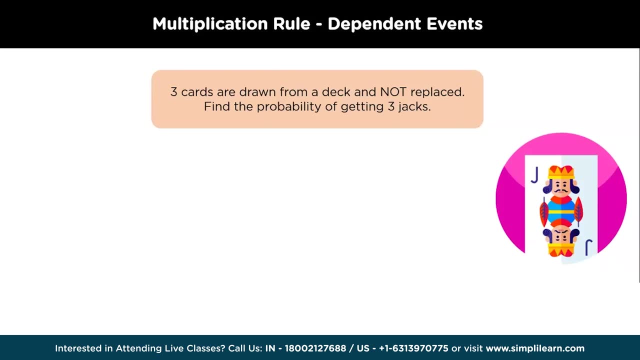 which is P A. intersection B is equal to probability of A into probability of B. slash A. The slash reads the probability that B occurs, given that A has already occurred. Let's look at an example. Three cards are drawn from a deck and are not replaced. 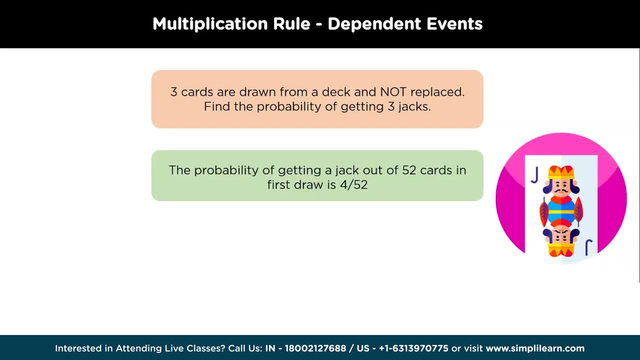 What will be the probability of getting three jacks? So in this case, the probability of getting a jack out of 52 cards in the first draw will be 4 by 52.. Now, after we have drawn the first card, there are 51 cards left. 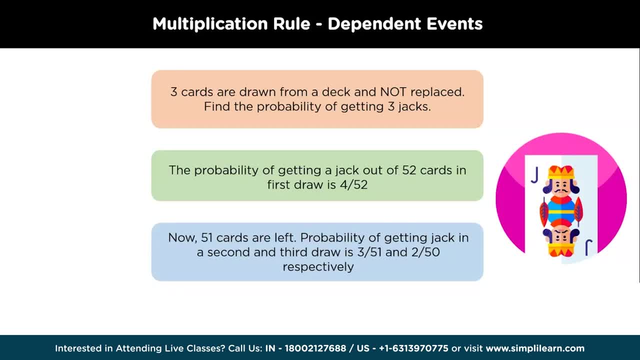 The probability of getting a jack in a second and third draw will be 2 by 51 and 2 by 50 respectively. So, according to the formula, the probability of getting the three jacks will be P 0.76 into 0.058 into 0.04. 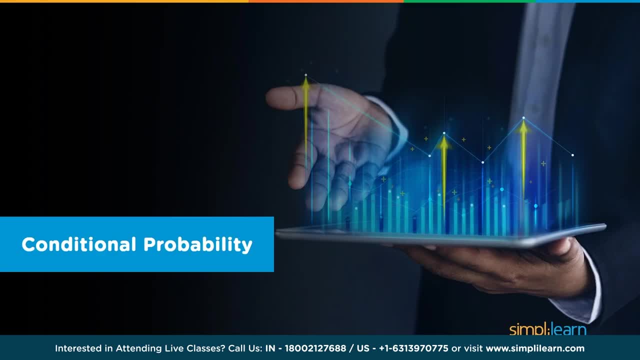 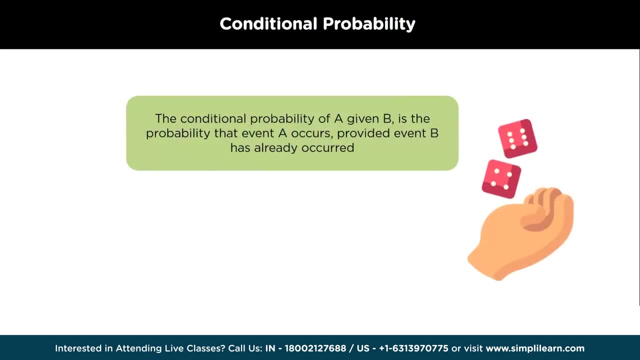 which will come out to be 0.00176.. Now that we know all the basic concepts in probability theory, we will move on to conditional probability. Let A and B be the two events associated with a random experiment. Then the probability of A's occurrence. 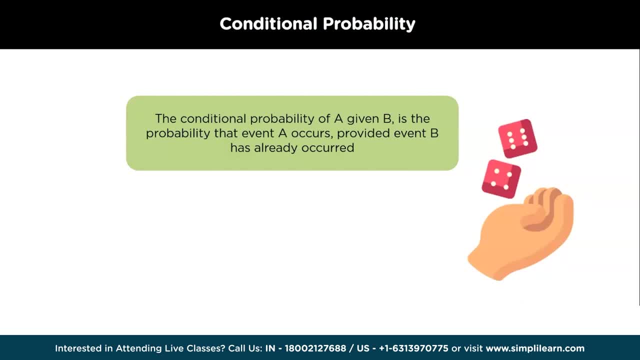 under the condition that B has already occurred is called the conditional probability. It is generated by the probability of P. Thus we have: P is equal to P divided by P. P is read as probability of occurrence of A, given that B has already occurred. 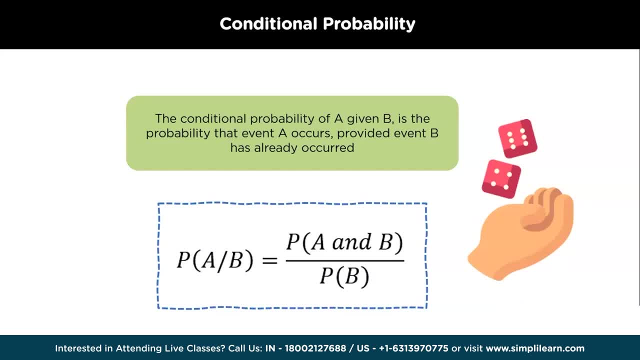 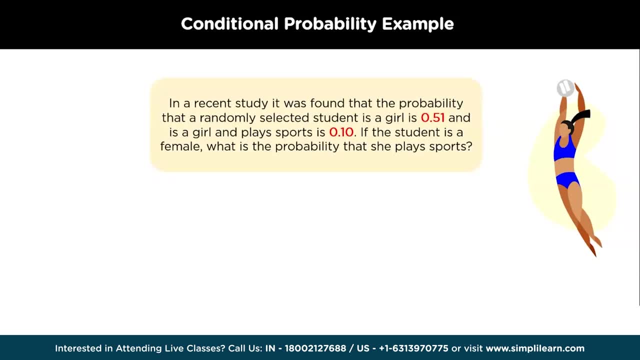 Similarly, P can be called as probability of occurrence of B, given that A has already occurred. Let's look at an example. In the recent study, it was found that the probability of a randomly selected student is a girl is 0.51 and is a girl and plays sports. 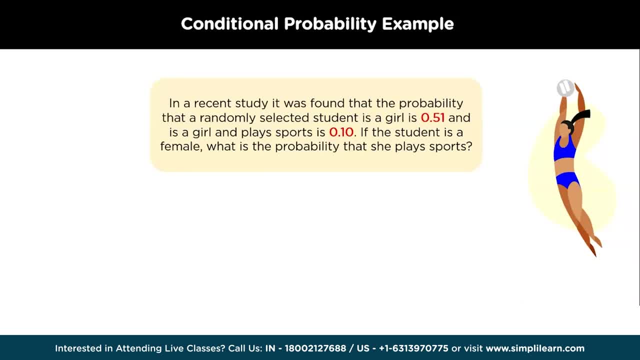 is 0.10.. So if the student is a female, what is the probability that she plays sports? In this case, the probability that a student is female and plays sports is 0.1 and the probability that a student is female is 0.51. 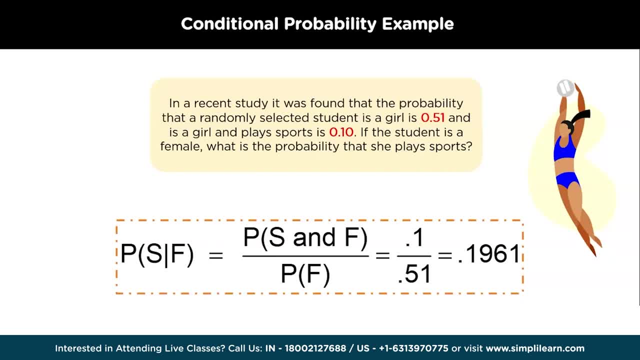 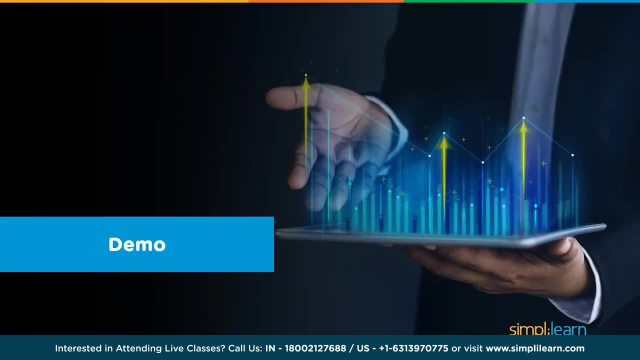 So the probability that a student plays a sport, given that she is a female, will be 0.1 divided by 0.51, which will come out to be 0.1961.. Now that we are done with all the theories related to conditional probability. 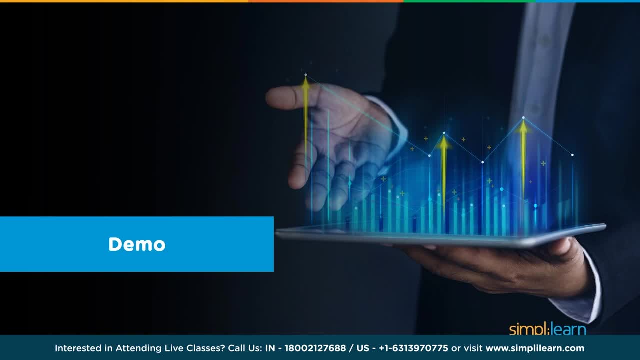 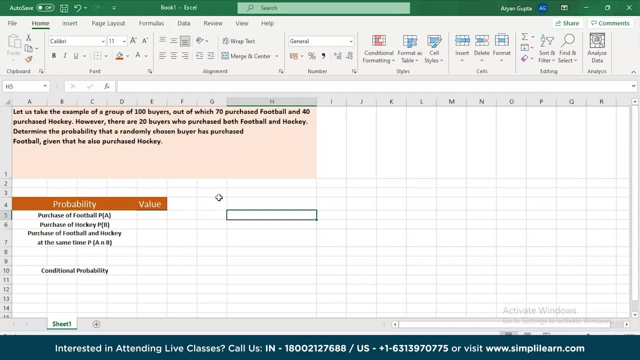 we will move on to the demo in excel. Suppose there are a group of 100 buyers, out of which 70 purchased football and 40 purchased hockey. However, there are 20 buyers who purchased both football and hockey. Determine the probability that a randomly chosen buyer has purchased football. 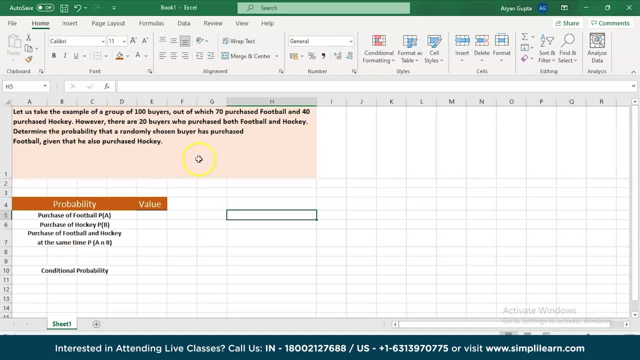 given that he also purchased hockey. So this is a clear example of a conditional probability. Let's fill in this table. So the probability of purchasing a football is 0.70 and that of hockey is 0.20.. It is also given that there are 20 buyers. 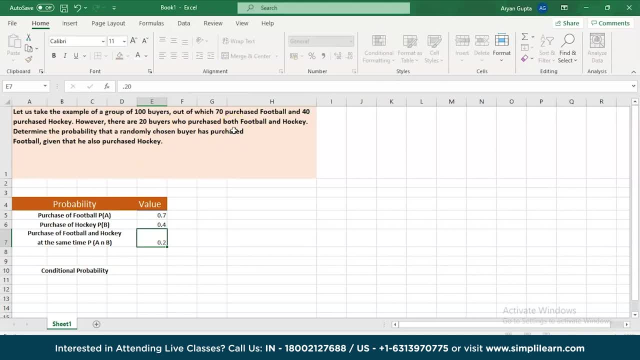 who have purchased both football and hockey. So 0.20 is the probability of PA intersection B. Now, if you remember the formula of the conditional probability, the A slash B is equal to PA intersection B divided by PA of B. where PA intersection B 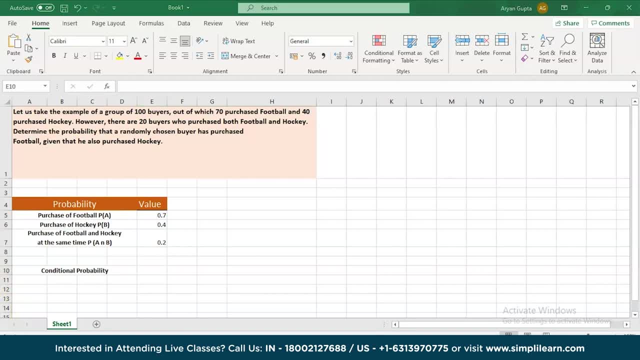 is the probability of occurrence of both A and B. TB is the probability of occurrence of B. So we have all the values Let's fit in. So this will be equal to. this is cell E7.. So we will divide the cell E7. 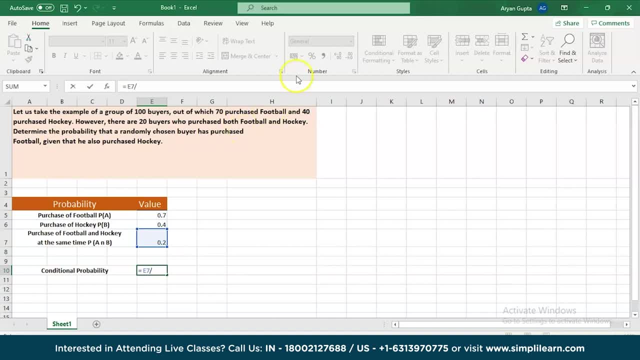 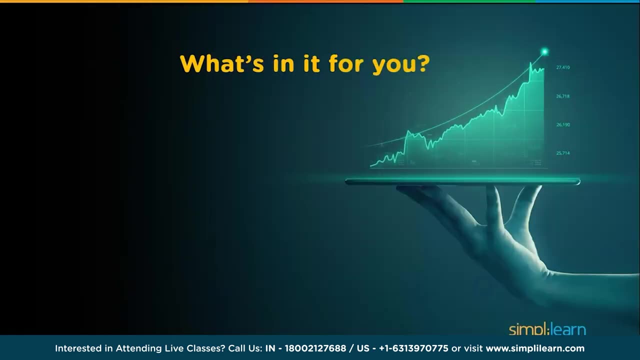 by cell E6, which will come out to be 0.5.. So the probability that a randomly chosen buyer has purchased football, given that he also purchased hockey, is 0.5.. So what can you expect from this video? What's in it for you? 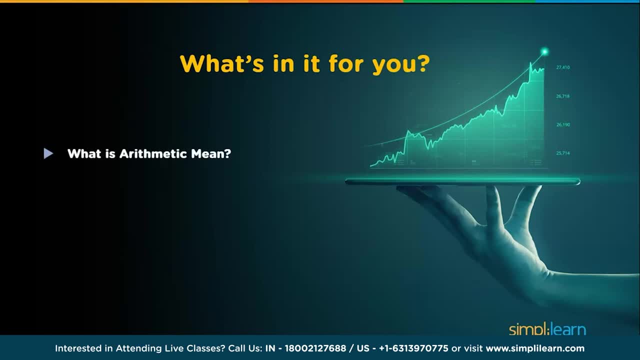 First we will explain the concept of arithmetic mean to you. Then we will move on to what is median and mode. Finally, we will look at two other types of means: geometric mean and arithmetic mean. All of this with the help of worked examples and formulae. 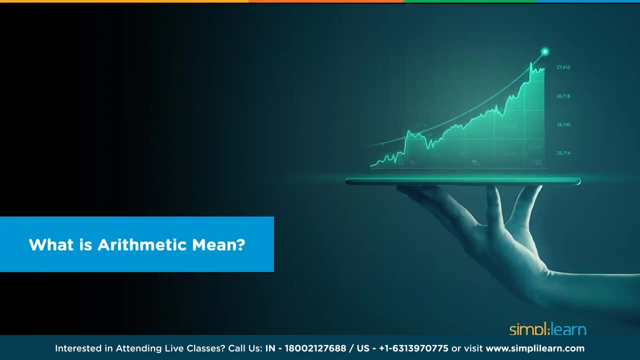 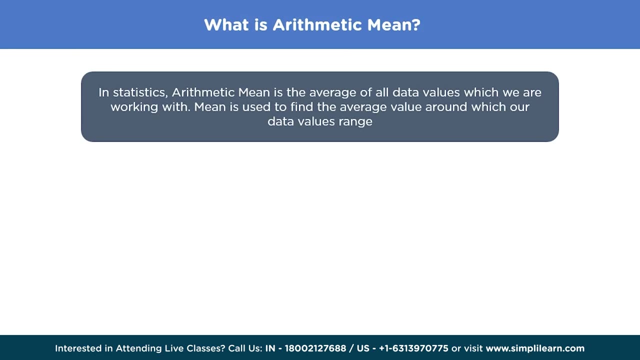 So let's get started. What is arithmetic mean? In statistics, arithmetic mean is the average of all data values which we are working with. Mean is used to find the average value around which our data values range. Mean is the average that you are used to. 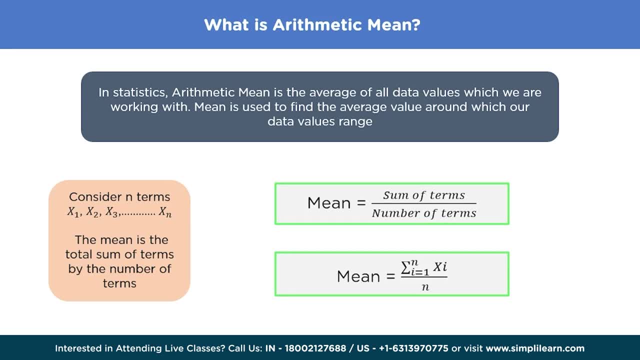 When you add up all the numbers and then divide by the total number of numbers which are present, that gives us the mean. The mean helps us to assess the performance of an investment or company over a period of time, and it has many other uses. 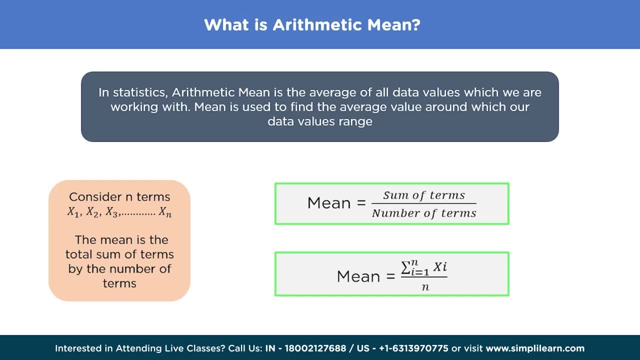 It is a statistical indicator that can be used to gauge the performance of a company's stock price over a period of days, months or years. A company, through its earnings over a number of years. a firm, by assessing its fundamentals such as price to earnings ratio, free cash. 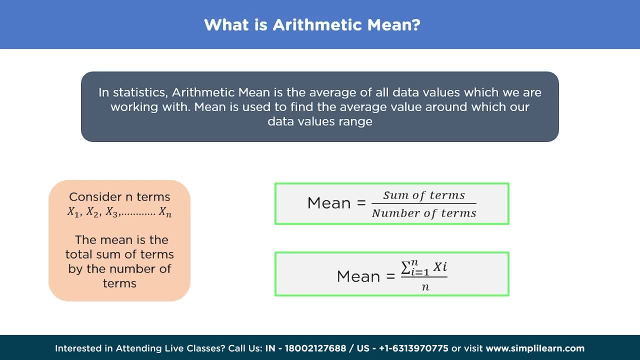 flow and liabilities on the balance sheet and a portfolio by estimating its average returns over a certain period. How do we calculate mean? Consider that we have n number of terms: x1,, x2,, x3 or all the way up to xn. Mean is given by the total sum of. 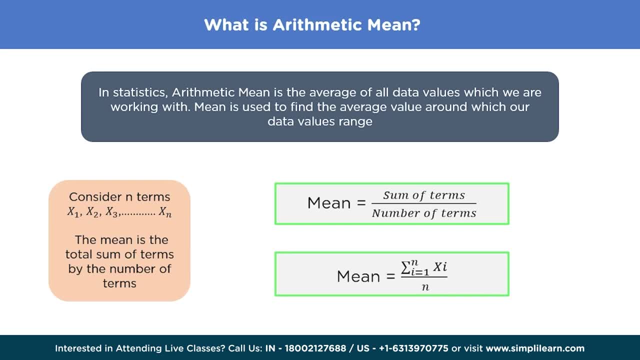 the terms divided by the total number of terms. This can also be represented as summation: i is equal to 1 to n over xi divided by n, where n is nothing but the number of terms and xi are our terms, which range from 1 all the way up to n. 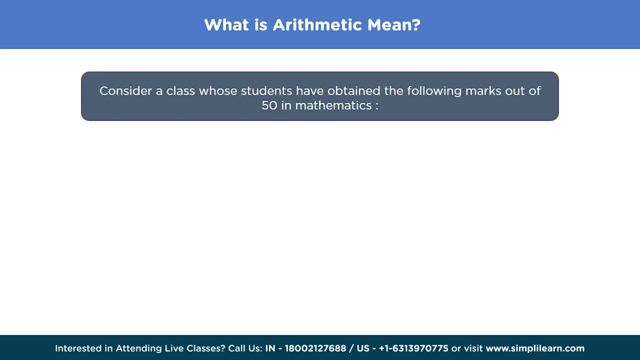 Let's see how mean can be calculated with the help of an example. Consider a class whose students have obtained the following marks out of 50 in mathematics: There are 12 students and the marks obtained by them are 35,, 40,, 45,. 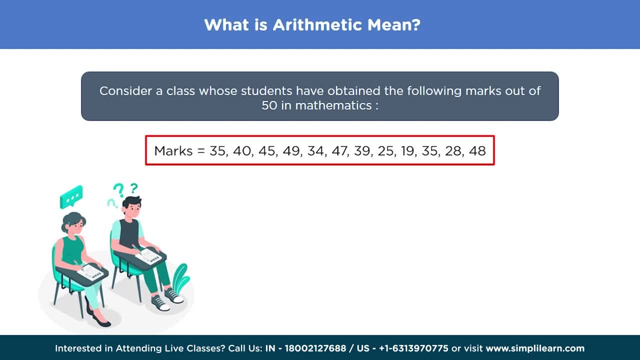 49,, 34,, 47,, 39,, 25,, 19,, 35,, 28 and 48.. Mean is nothing but the average of all the terms which are given to us, divided by the total number of terms. We add all the terms and divide it. 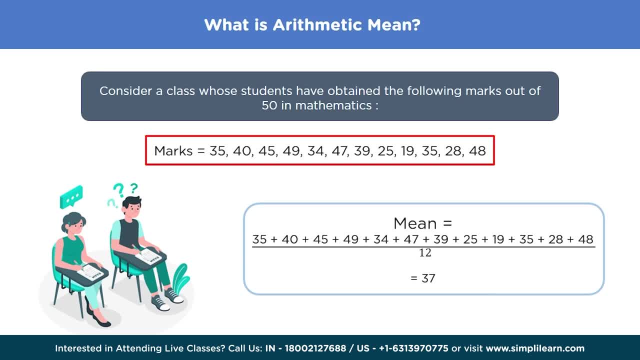 by 12, which is the total number of terms, The mean that we get is 37, which means the average marks of our class is 37.. Note that none of the students actually scored 37 out of 50 in their test In this case. 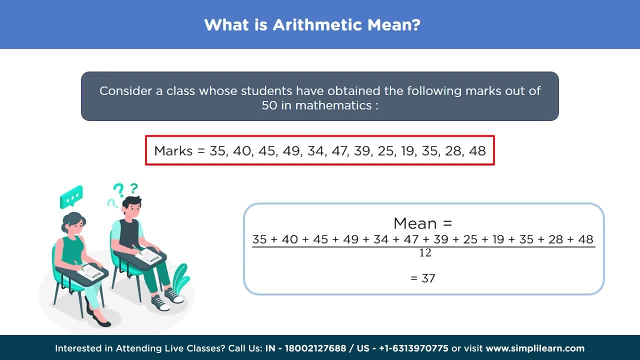 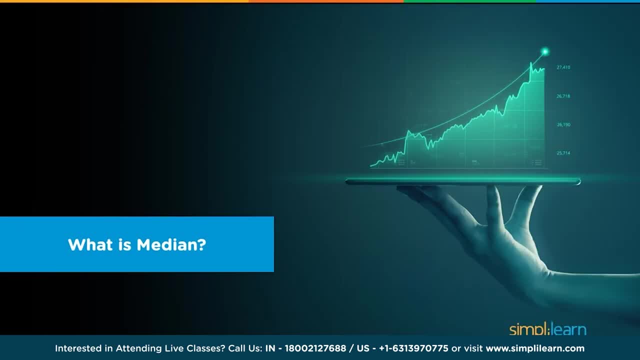 you can see that the mean isn't a value from the original list. This is a common result and you should not assume that your mean will be one of your original numbers. Now let's move on to median. What is median? Median refers to the middle. 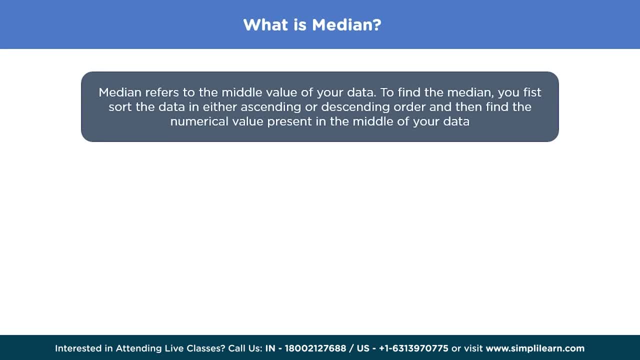 value of your data. To find the median, you first sort the data in either ascending or descending order and then find the numerical value which is present in the middle of your data. The median is sometimes used as a pose to the mean when there are outliers in the sequence. 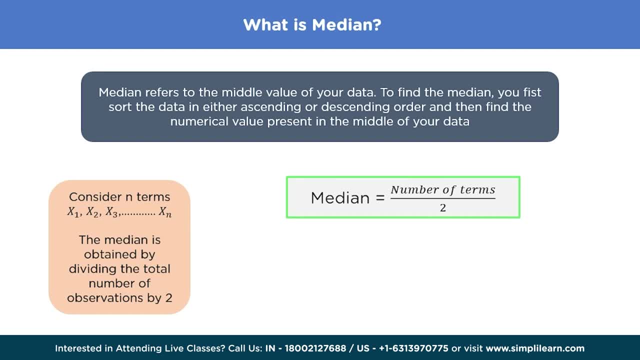 that might skew the average of the values. If there's an odd amount of numbers, the median value is the number that is in the middle, with the same amount of numbers below and above. If there's an even amount of numbers in the list, the middle. 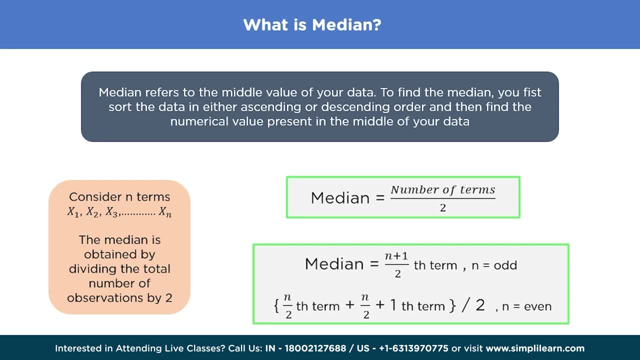 value must be determined, added together and then divided by 2 to find the median value. The median can be used to determine an approximate average or mean, but it should not be confused with the actual mean. So how do you calculate the median? 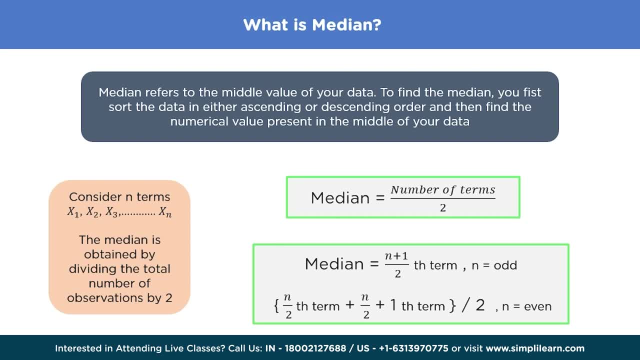 Again. let us consider n number of terms ranging from x1 to xn. The median can be obtained by dividing the total number of observations by 2.. This works out very well with odd number of terms. Suppose you have 11 terms, then obviously, 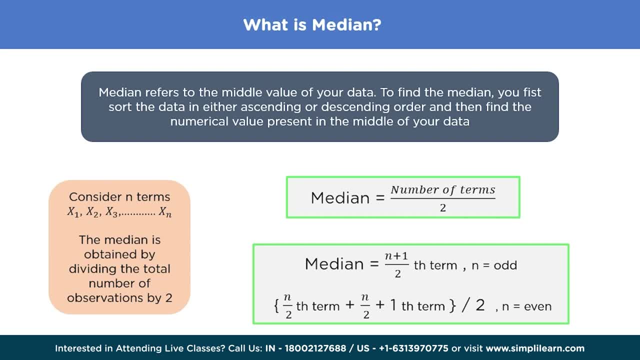 the 6th term will be your median, with 5 numbers above and 5 numbers below. However, when you have an even number of terms, there is no actual middle term To find the median of a series which has even number of terms. 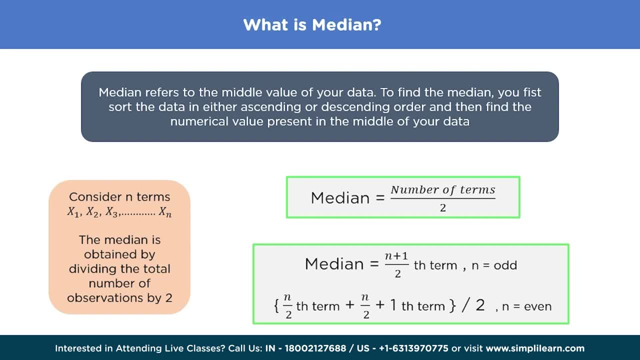 you take the middle term, which is the n by 2 term, and the term after that, which is nothing but the n by 2 plus 1th term. add both of them up and divide them by 2 to get your median. Let's try to understand median with the. 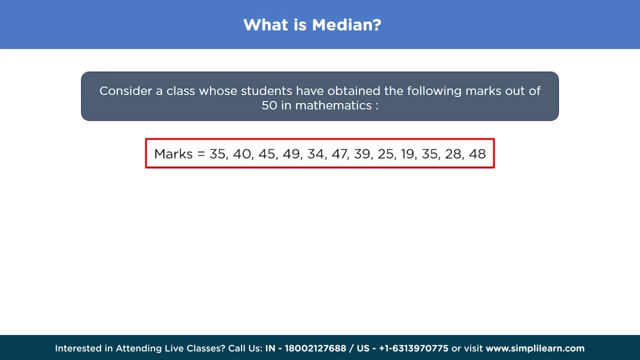 help of an example Again, let's consider the marks obtained by 12 students in mathematics in a class. If there were only 11 terms- like let's assume that the last term was in present, which is 49,, it would be very easy to find the median. 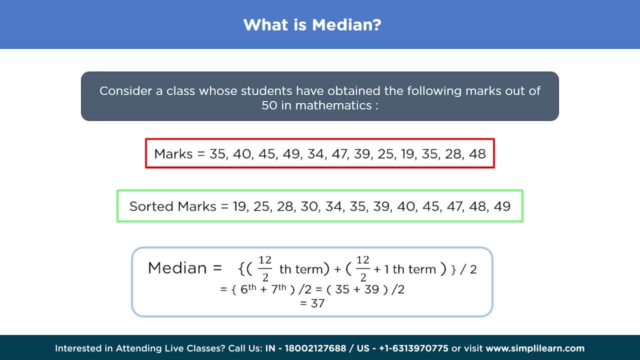 You would just have to consider the middle term or the 6th term here, which is 35. There are 5 terms above it and 5 terms below it. It is clearly in the middle of our range. So this would be our median, But we have 12 numbers here. 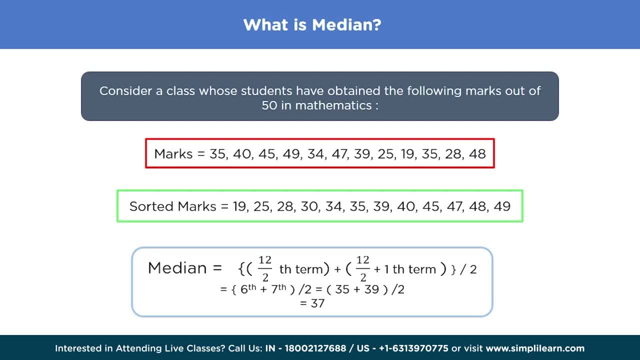 To calculate the median of even number of terms, we take the number of terms by 2, which here is the 12 by 2 term, and the term after that, which is 12 by 2 plus 1th term, which equates to the 6th and 7th term. 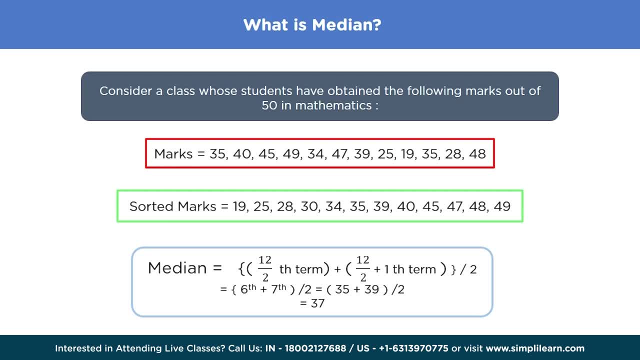 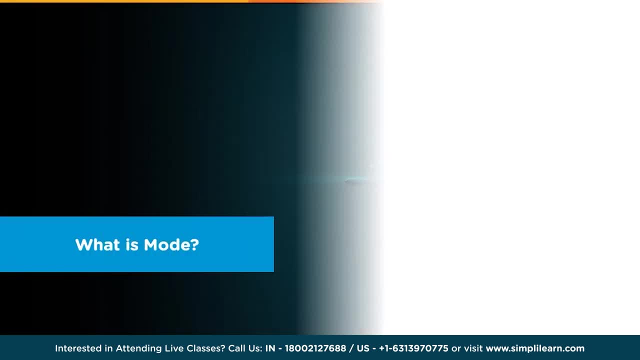 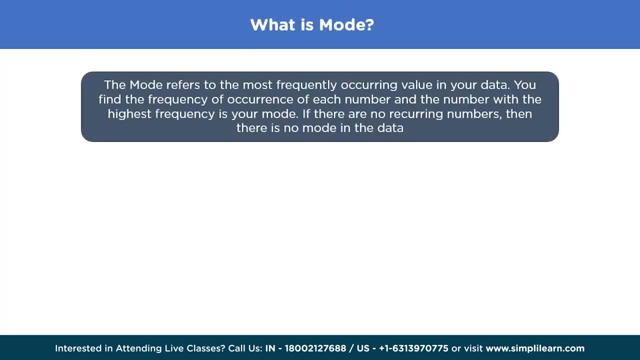 Add both of them up and divide by 2.. 35 plus 39 divided by 2 gives us 37. This would be the median in this case. Now let's answer the question: what is mode? The mode refers to the most frequently occurring value. 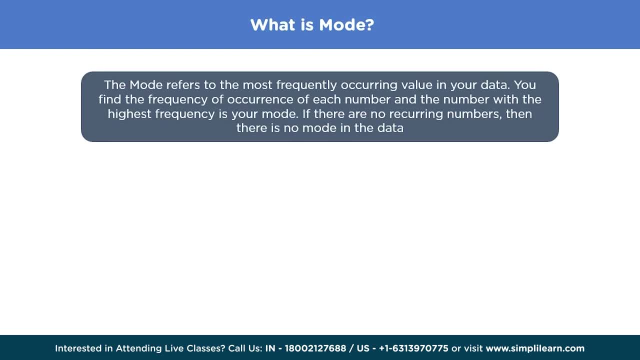 in your data You find the frequency of occurrence of each number, and the number with the highest frequency is your mode. If there are no recurring numbers, then there is no mode in the data. Mode can be obtained by counting the frequency of occurrence of each number. 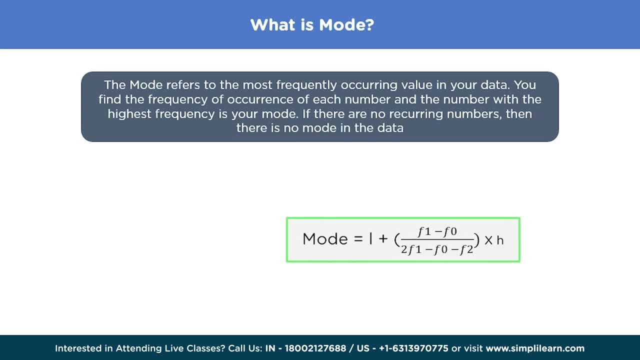 in your range and then choosing the one which occurs the most frequently, or by using the formula L plus F1 minus F0, divided by 2. F1 minus F0 minus F2 into H. What do these terms mean and when do we use this formula? 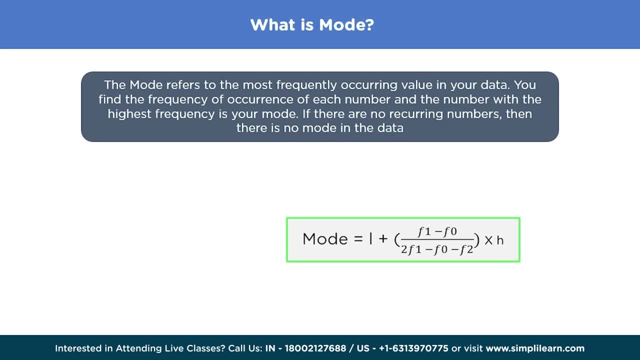 This formula can only be used when our data is in the form of a range of values and the specific values are not given. In this case, L is the lower limit of modal class. Modal class is nothing but the class which has the highest number of terms, H. 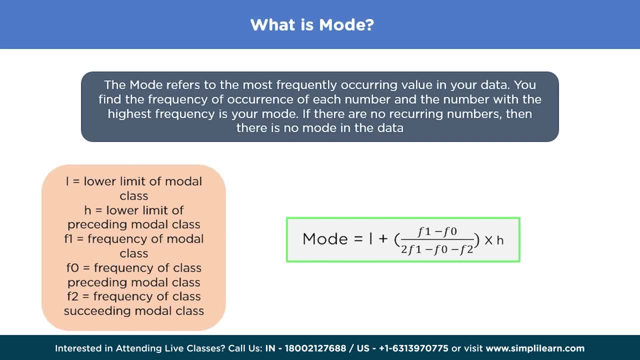 is the lowest limit of the preceding modal class. F1 is the frequency of the modal class. F0 is the frequency of the class which is again preceding the modal class or the class which comes before our modal class. F2 is the frequency of the class which comes after. 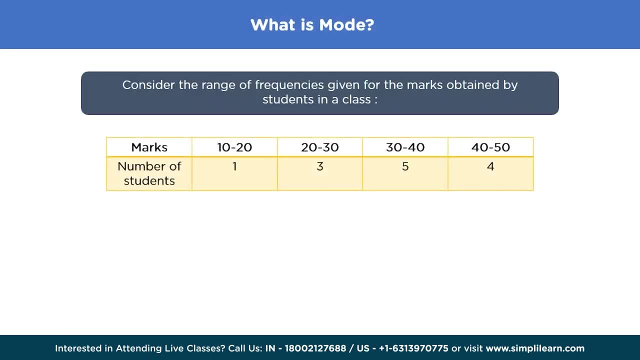 our modal class. Let's try to understand mode with the help of an example. The below table summarizes the data that we have used before and puts it in the form of a range of values. Only one student has obtained marks between 10 to 20,. 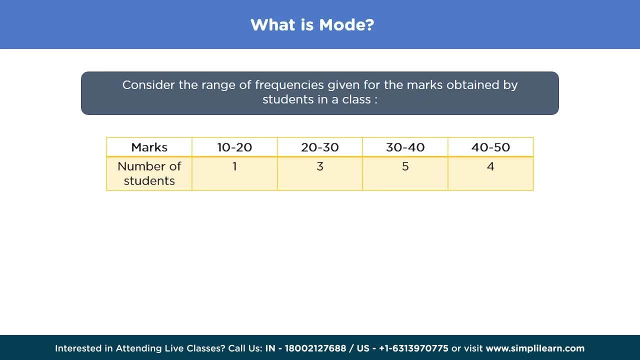 3 have secured marks between 20 to 30,, 5 have gotten marks in the range of 30 to 40, and 4 have gotten marks in the range of 40 to 50.. To find our mode, we're gonna. 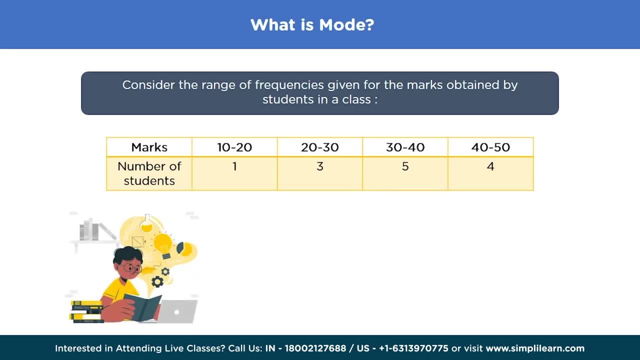 use the formula that we saw. As we can see, the class which has the most number of terms is the class 30 to 40. 5 people have scored marks in the range of 30 to 40. So this is our modal class. 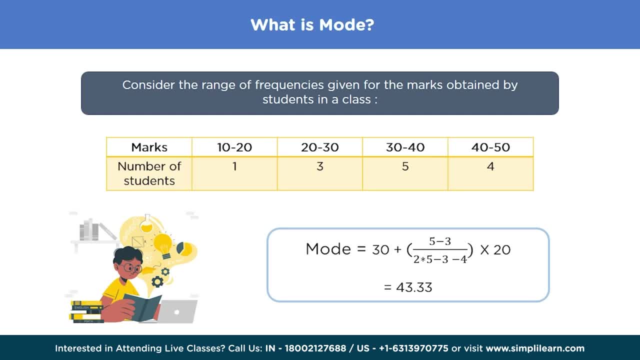 The class preceding this would be 20 to 30, and the class succeeding it would be 40 to 50. So we first have our L term, which is nothing but the lower limit of our modal class, which is 30. We then have the frequency of 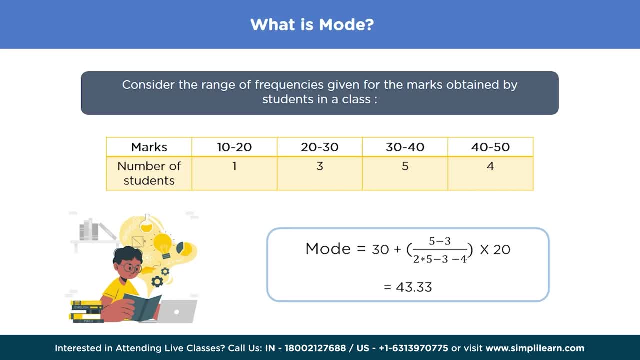 characters in our modal class, which is 5, minus the frequency of characters in the class preceding our modal class, which is 20 to 30, with frequency 3.. Divided by 2 into the frequency of our modal class, again 5 minus F1. 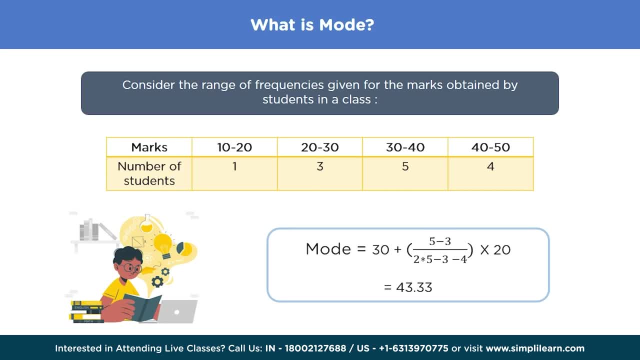 minus F2.. F2 is nothing but the frequency of the class succeeding our modal class, which here is 40 to 50.. We then multiply this fraction by the lower limit of the class preceding our modal class. After solving, we get 43.33. 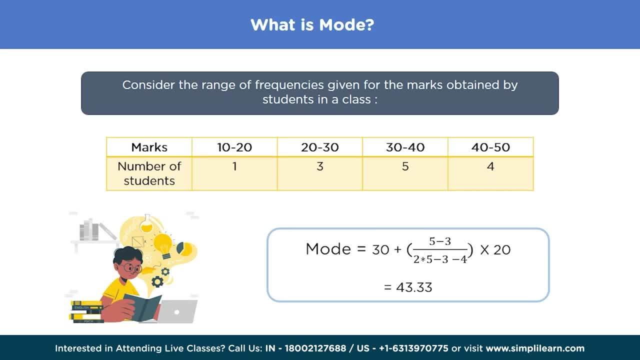 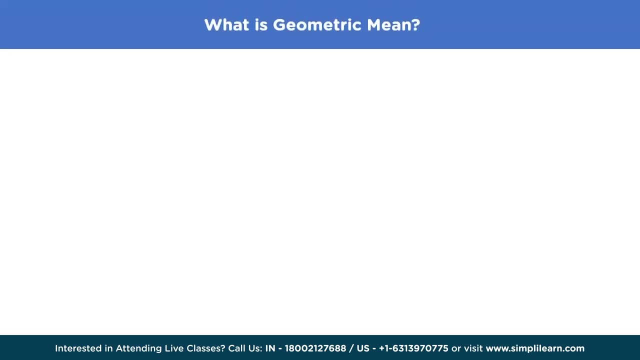 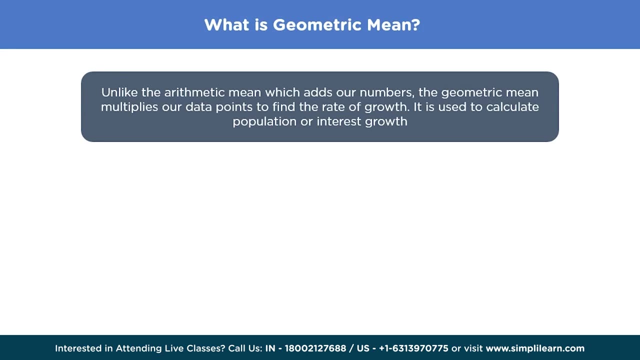 as our mode. 43.33 is the marks here and not the number of students. Next, let's answer the question: what is geometric mean? Unlike the arithmetic mean in which we add our numbers, the geometric mean multiplies our data points to find the rate of growth It is used. 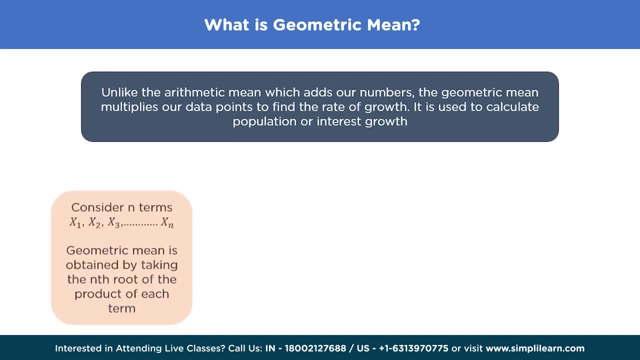 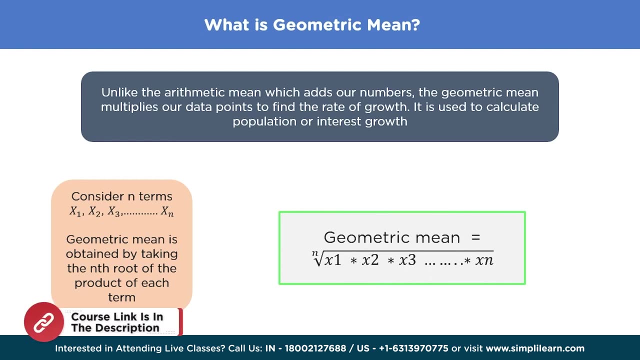 to calculate population or interest growth. The geometric mean factors in compounding and volatility, which makes it a better metric of average returns. In mathematics, the geometric mean is a mean or average, which indicates the central tendency or typical value of a set of numbers by using the product of their 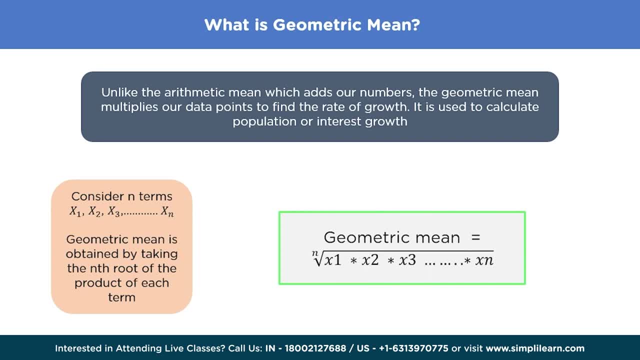 values. as opposed to the arithmetic mean, which uses the sum, The geometric mean is defined as the nth root of the product of n numbers. The geometric mean is often used for a set of numbers whose values are meant to be multiplied together or are exponential in nature. 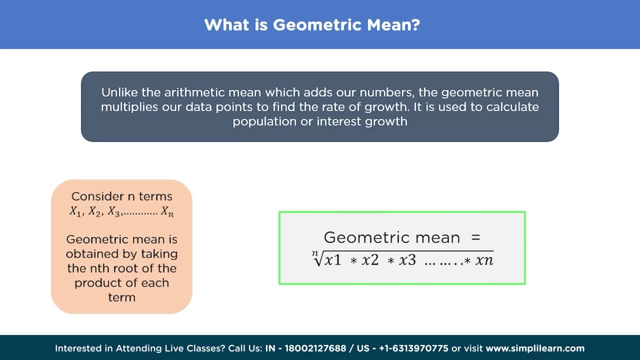 Such as a set of growth figures like values of the human population or interest rates of a financial investment over time. To calculate the geometric mean, let's consider that we have n terms ranging from x1 to xn. The geometric mean can be obtained by taking the. 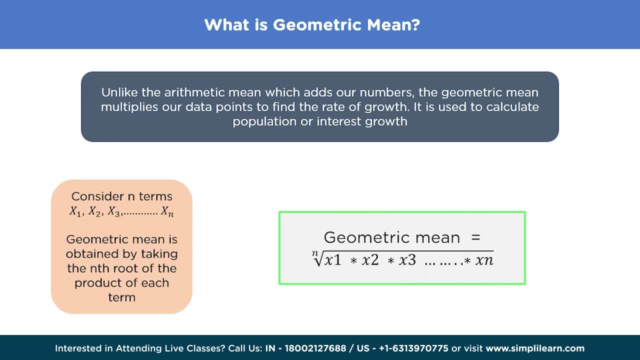 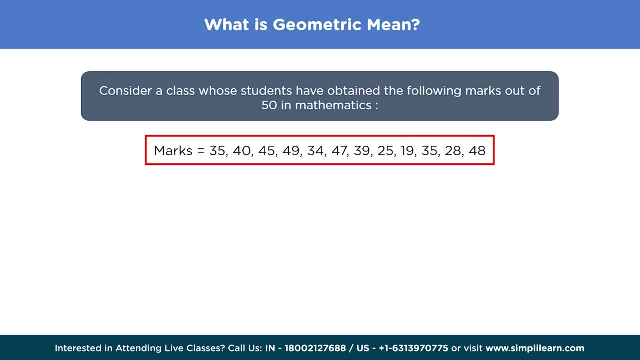 nth root of the product of each term. We multiply all of the terms in our data and we take the nth root of it. Let's again understand this with the help of an example. Let's consider the marks of the student that we've been taking up until now. 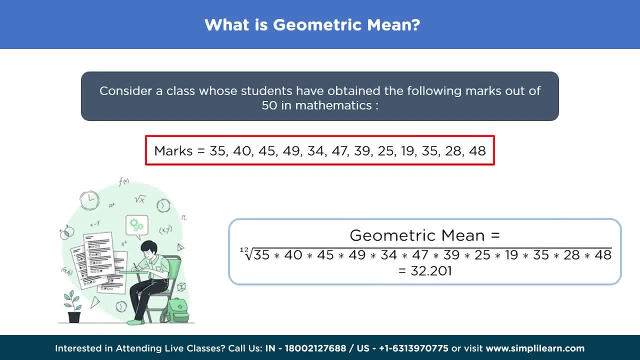 The geometric mean is nothing but the product of all the terms in our data to the nth root of the product. So to find the geometric mean, we multiply all the terms in our data and then take the 12th root of them. The final answer is: 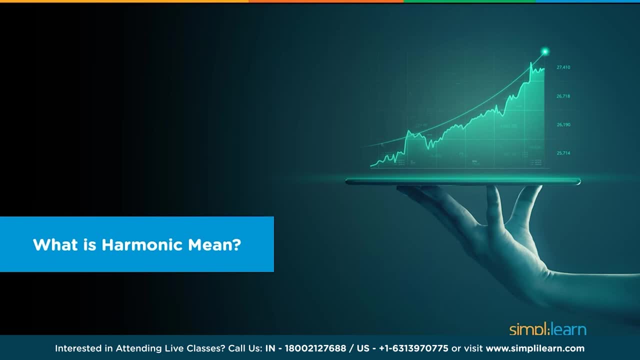 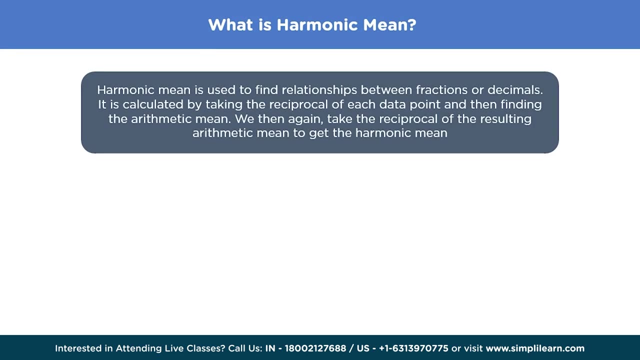 nothing but 32.201.. Now, what is harmonic mean? Harmonic mean is used to find relationships between fractions or decimals. It's calculated by taking the reciprocal of each data point and then finding the arithmetic mean. We then take the reciprocal of the resulting. 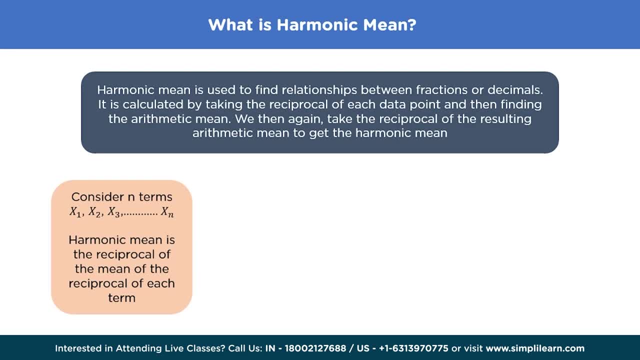 arithmetic mean. to get the harmonic mean Again, let's consider n terms ranging from x1 to xn. To find the harmonic mean, we first take the reciprocal of each one of these terms and then find the mean of the resulting terms. To find the harmonic mean we 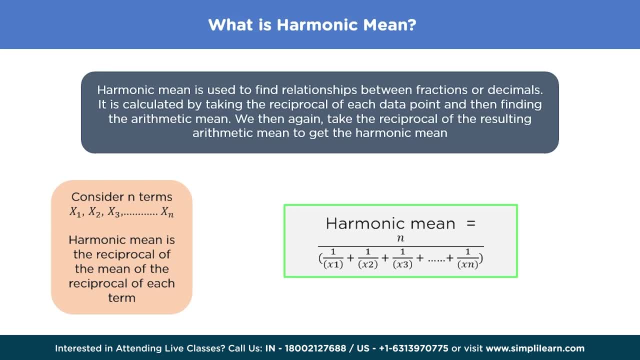 first take the reciprocal of each data term. As you can see, here we have taken the reciprocal 1 by x1,, 1 by x2, 1 by x3, all the way to xn. We then add up all the reciprocals and 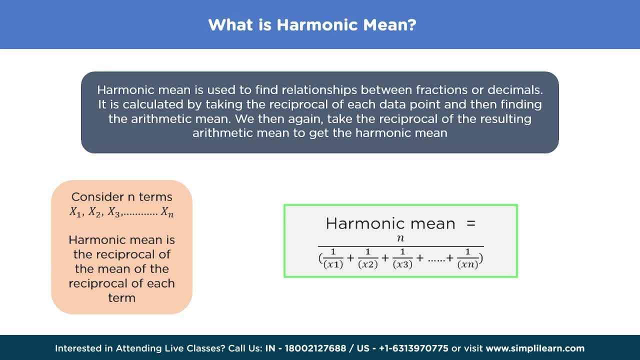 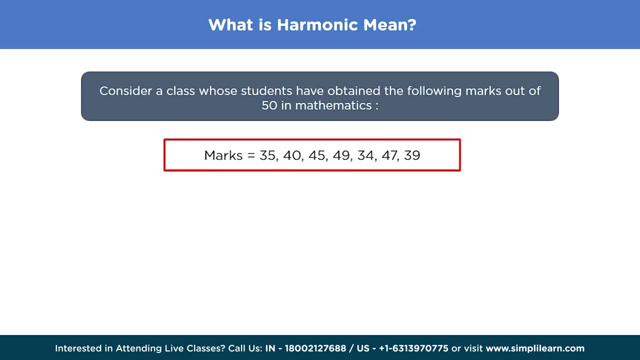 divide it by n to get the mean. We take a reciprocal of the mean to get the harmonic mean. Let's look at how to find the harmonic mean by using the data that we have up until now. Again, consider the marks of the following students out of 50 in mathematics. 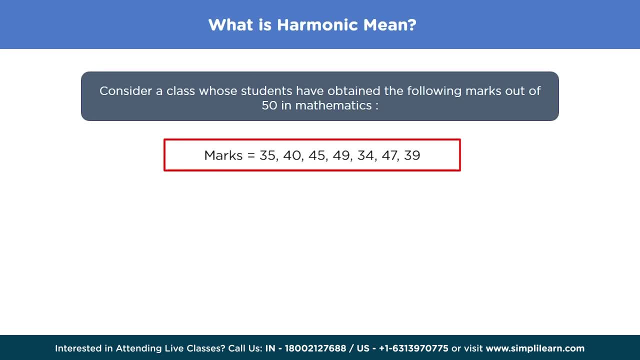 Over. here we are considering 7 terms To find the harmonic mean. we take the average of each one of our reciprocal terms. We have taken the reciprocal of the marks obtained by our students: 1 by 35,, 1 by 40,. 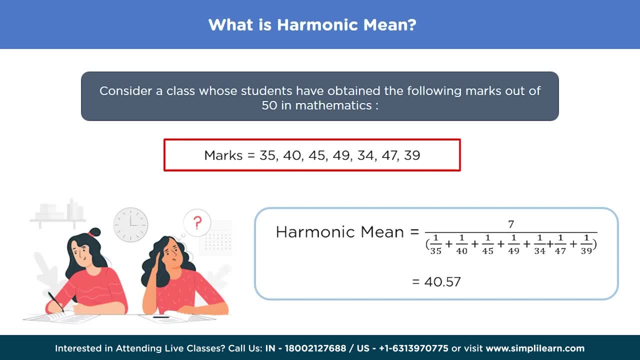 1 by 45,, 1 by 49,, 1 by 34,, 1 by 47 and again 1 by 39. After getting the reciprocal of these terms, we find the mean. So we add up all the reciprocal terms and divide it by 7. 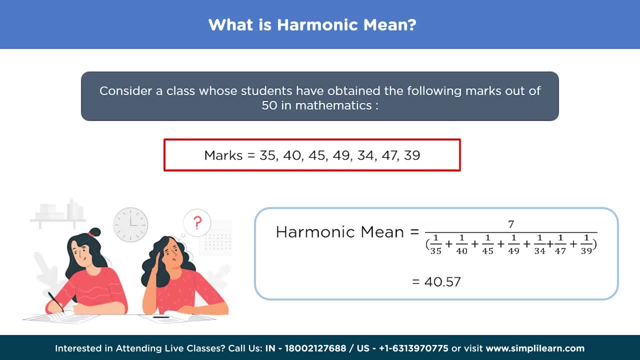 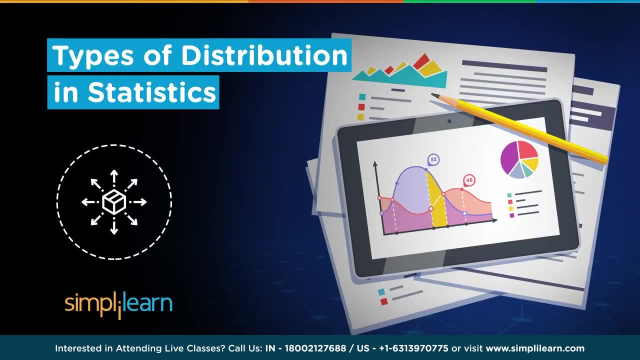 and then take the reciprocal of that term, In the end the harmonic mean that we get is 40.57.. We will discuss the types of distribution in statistics, But before we move ahead, let's have a brief introduction on what is probability distribution. A probability, 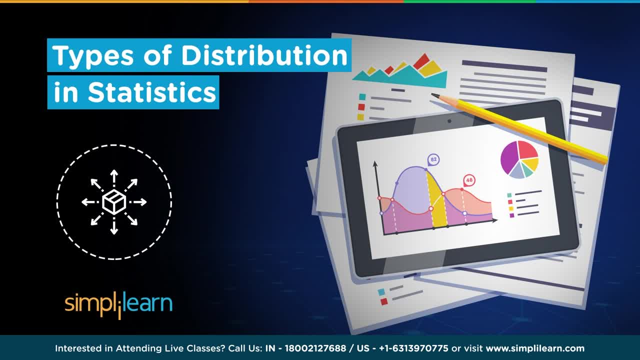 distribution is a list of all of the possible outcomes of a random variable, along with their corresponding probability values, And it is used in many fields, but we rarely do explain what they are. So in this video, we will discuss the three main types of probability distribution. 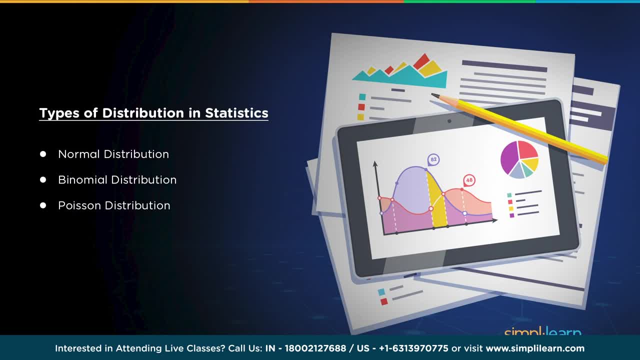 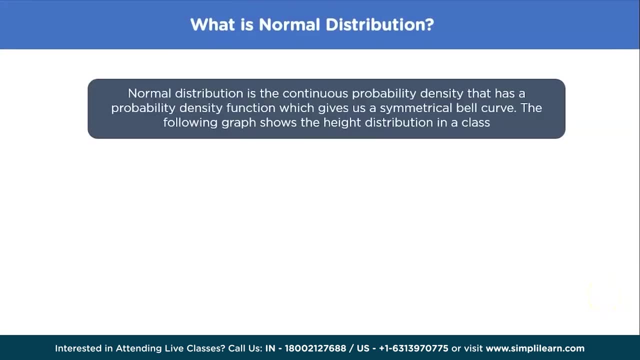 that is Normal Binomial and Poisson distribution. So let's move ahead. So what is normal distribution? Normal distribution is a continuous probability density that has a probability density function which gives us a symmetrical bell curve. Now data can be distributed or 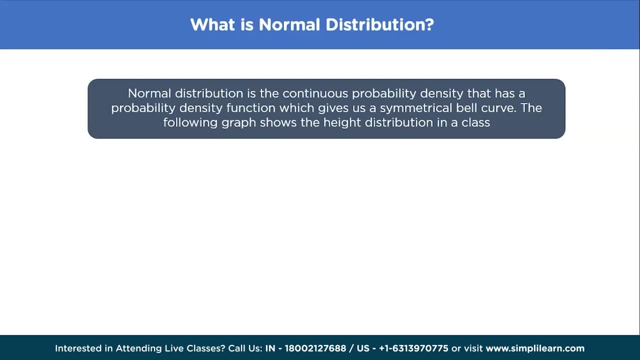 spread out in different ways, But there are many cases where the data tends to be around a central value, with no bias to the left or right, Which means that it doesn't show any particular spikes towards the left or the right And it gets close to a normal distribution. 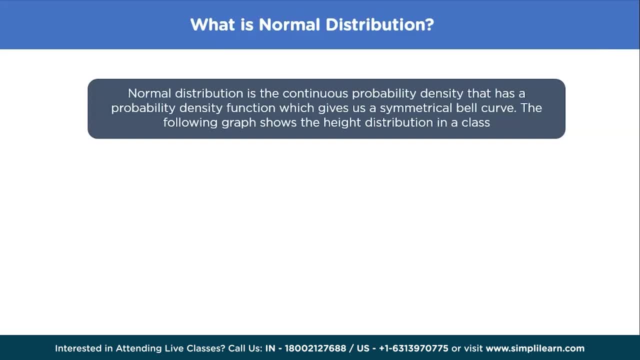 Half of the data will fall on the left of the mean and the other half will fall on the right. Now let's take a look at a graph which shows the height distribution in a class. As you can see, the average height is in the middle and the 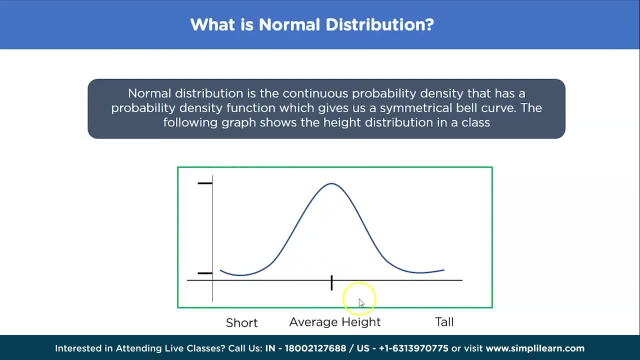 data to the left of the average height represents the short people and the data to the right of it represents the taller people. The y-axis shows us the likelihood of any of these heights occurring. The average height has the most distribution or it has the most number of cases. 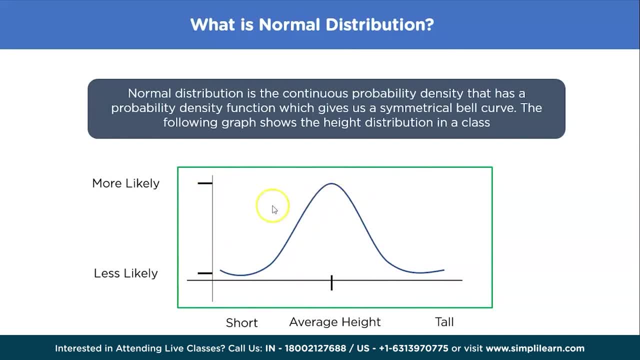 in the class And as the height decreases or increases, the number of people who have that height also decreases. This kind of a distribution is called a normal distribution, where the average or the mean is always the highest point and any other point after that or before that is. 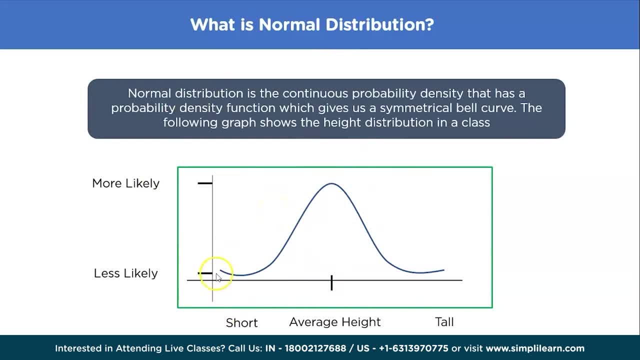 significantly lower. The resulting data gives us a bell curve and, as you can see, there is no abrupt bias or spike in the data anywhere, except for the average height. So this kind of a curve is called a bell curve and it's usually seen in a normal distribution. 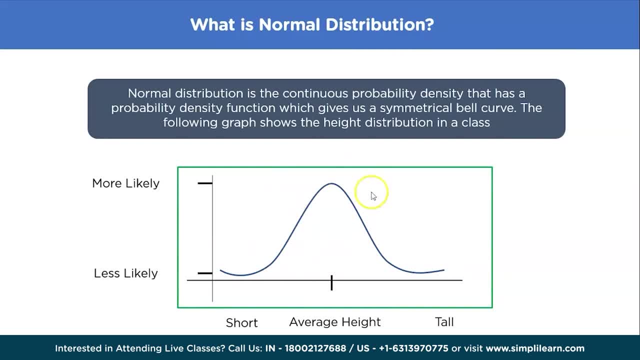 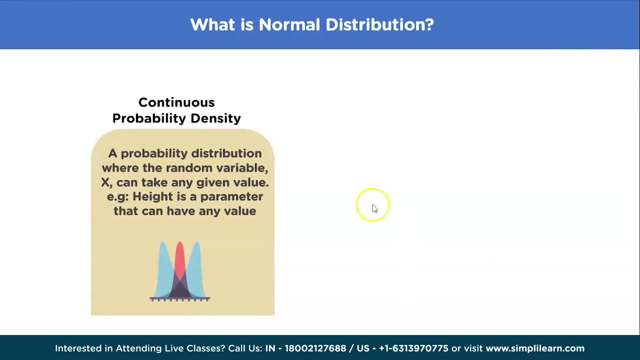 The reason we call this a normal distribution is because the data is normally distributed, with the average being the highest and all the other data points having a lower likelihood. Now we came across two terms which are associated with normal distribution: Continuous probability density and probability density. 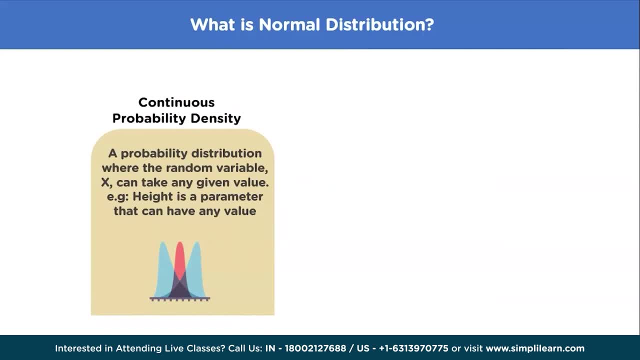 function. What is continuous probability density? Continuous probability density is a probability distribution where the random variable x can take any given value. Because there are infinite values that x could assume, the probability of x taking on any specific value is zero. For example, 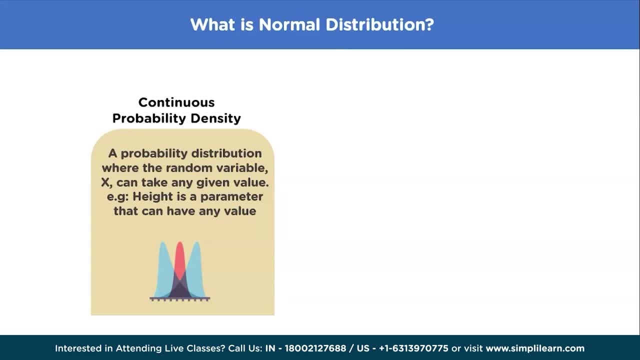 let's say you have a continuous probability density for men's height. What is the probability that a man will have the exact height of 70 inches? It is impossible to find this out because the probability of one man measuring exactly 70 inches is very low. It is. 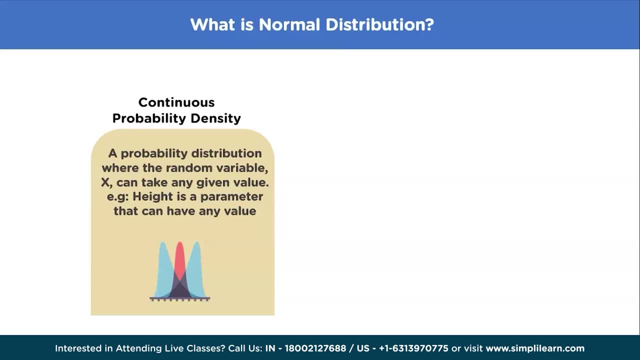 more probable that he will measure around 70.1 inches, or maybe 69.97 inches, and it doesn't stop there. The fact is that it's impossible to exactly measure any variable that's on a continuous scale, and because of this it's impossible to figure out the probability of 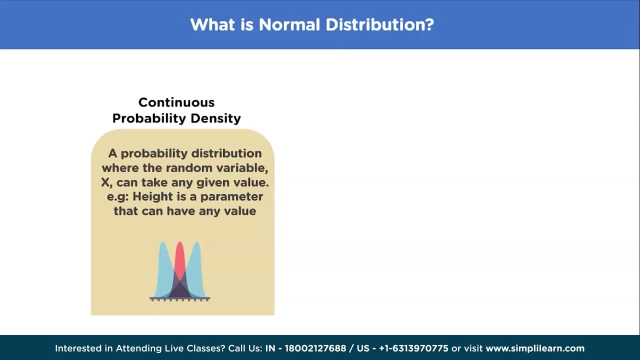 one exact measurement which is occurring in a continuous probability density. Next, we have the probability density function. It's nothing but a function or an expression which is used to define the range of values that a continuous random variable can take. An example of this would be to gauge the risk and reward. 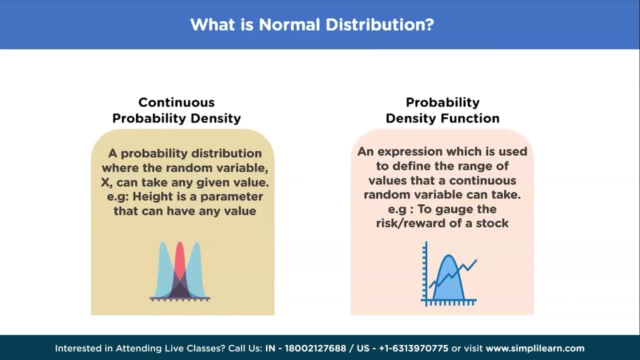 of a stock. A probability density function is a statistical measure which is used to gauge the likelihood of a discrete value. A discrete variable can be measured exactly, while a continuous variable can have infinite values. However, for both continuous as well as discrete variables we can define a function. 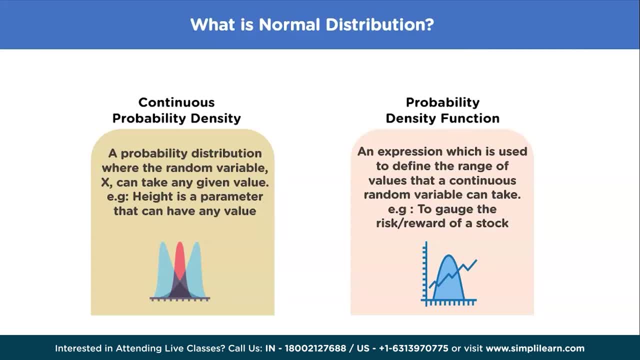 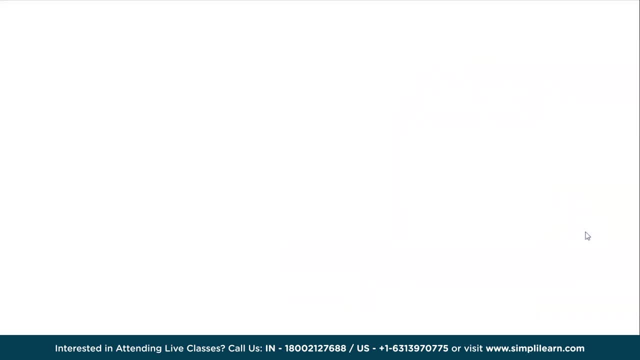 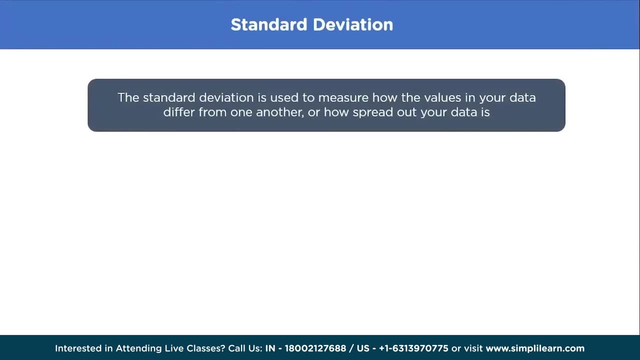 which gives us the range of values within which these variables will fall, And that function is not a probability density function. Now let's take a look at standard deviation. What is standard deviation? Standard deviation is used to measure how the values in your data differ. 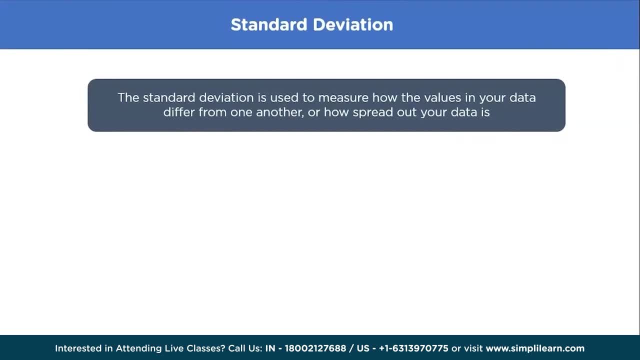 from one another or how spread out your data is A standard deviation is a statistic that measures dispersion of a data set relative to its mean. The standard deviation is calculated as the square root of variance by determining each data point's deviation relative to the mean. 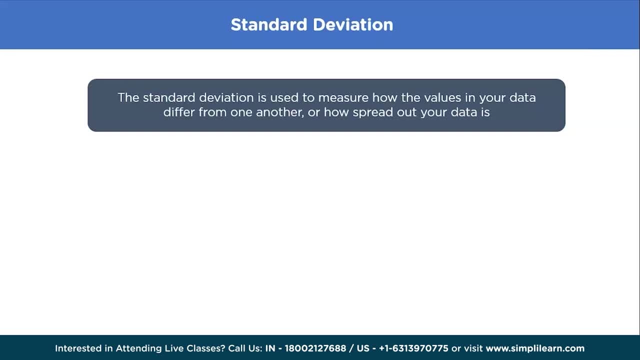 If the data points are further from the mean, that means that there is a higher deviation within the data set, and then the data is said to be more spread out. This leads to a higher standard deviation too. Let's take an example of income in rural and urban areas. 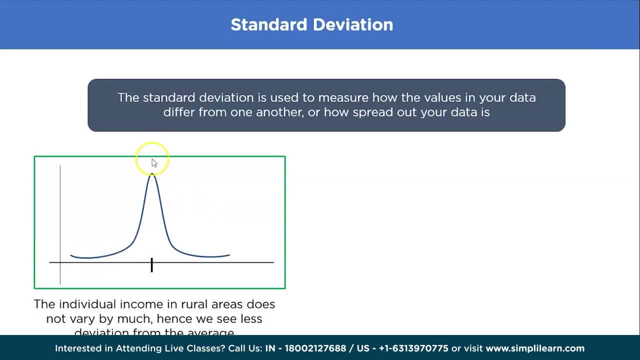 In rural areas, let's say, such as farming areas, the income doesn't differ that much. More or less everyone earns the same. Because of this, our bell curve has a very low standard deviation and it has a very narrow peak. However, 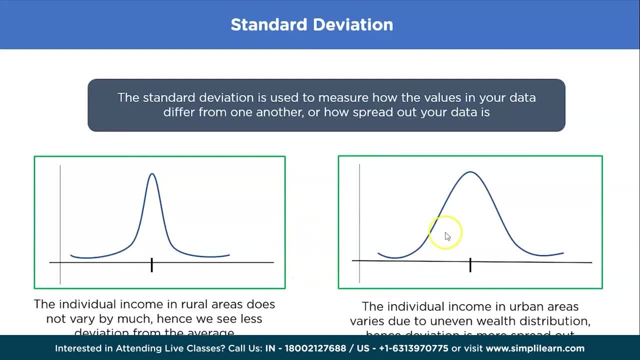 in urban areas, the wealth distribution is very uneven. Some people can have very high incomes and can be earning a lot, while other people can have very low incomes. Furthermore, the data distribution between these two income points is going to be more spread out because 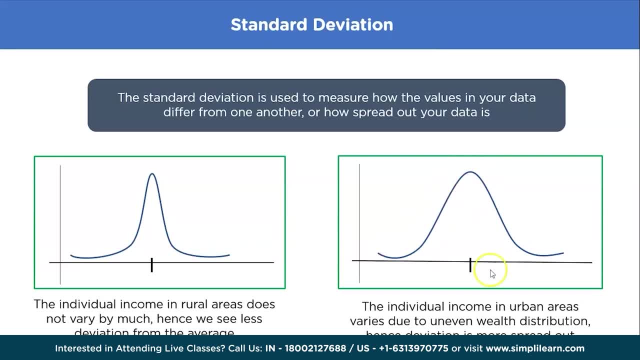 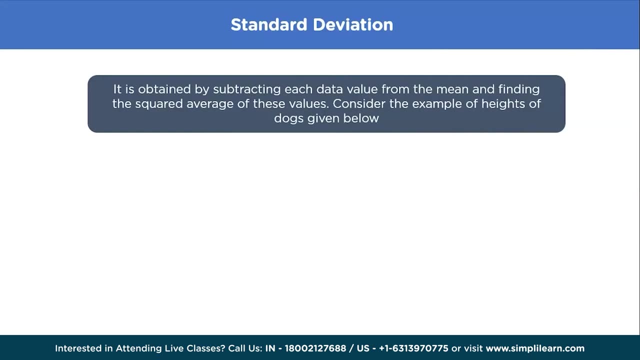 there are lot more people living there who work in various fields and who have various incomes. Because of this, our standard deviation is more spread out and our bell curve will also have a wider peak. Now how can we find the standard deviation? Standard deviation is obtained by subtracting. 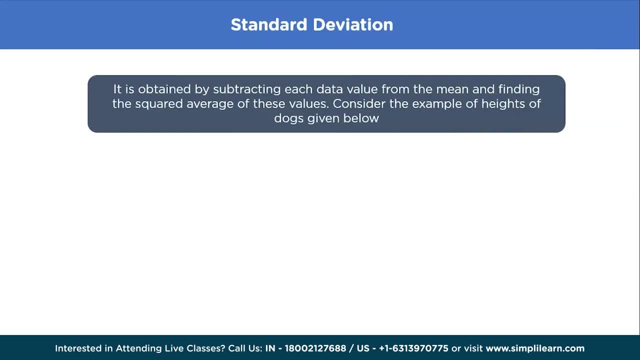 each data value from the mean and finding the squared average of these values. Let's look at how we can do this with the help of an example. These values correspond to the height of various dogs. We can find the mean by finding the average of all these values. 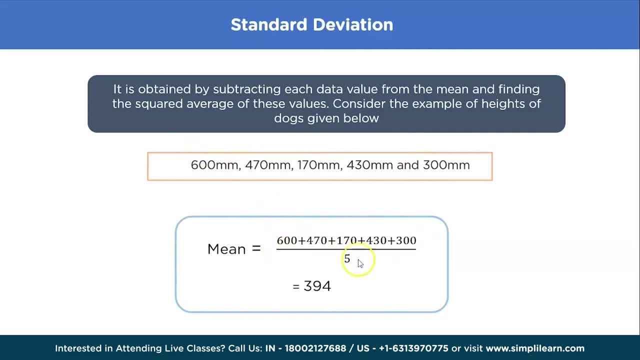 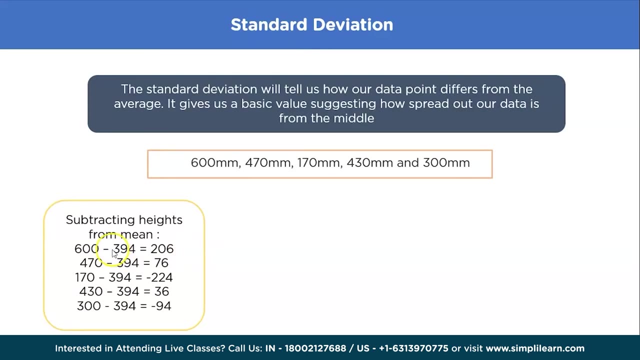 Which is nothing but adding all the values and dividing it by the total number of values. The mean that we get is 394.. This means that the average height of a dog is 394 mm. To find the standard deviation, first we need to subtract the height from the mean. 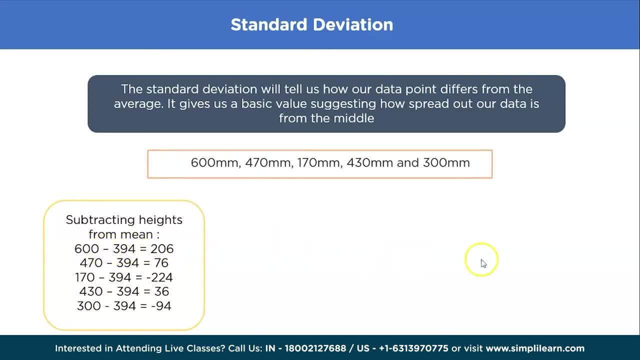 This will tell us how far from the mean our data points actually are. Next, we will square up all of these differences and add them up and again divide it by the total number of values that we have. This is called the variance. The variance. 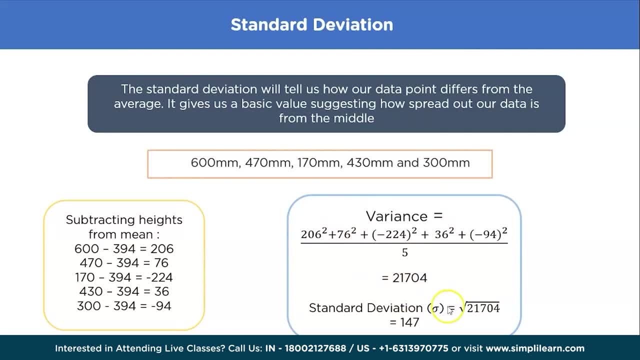 that we get in this case is 21704.. Finally, when we find the square root of this value, we will get the standard deviation. The standard deviation here is 147.. The standard deviation will tell us how our data points differ from the average. 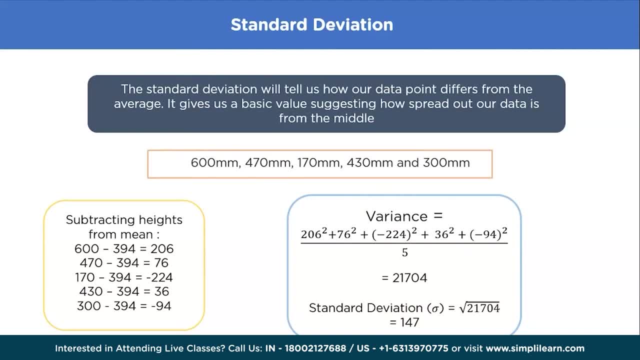 And it gives us a basic value suggesting how spread out our data is: from the very middle or from the mean. So when we plot these values, this value 147 will mean that a curve will have a width of 147 points around the mean. 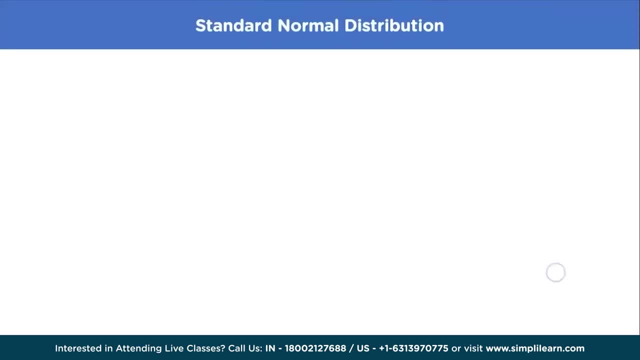 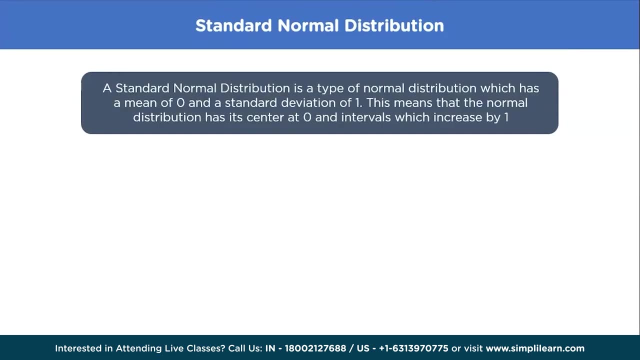 Now, what is the standard normal distribution? The standard normal distribution is a type of normal distribution that has a mean of 0 and a standard deviation of 1. This means that the normal distribution has its center at 0 and it has intervals which increase. 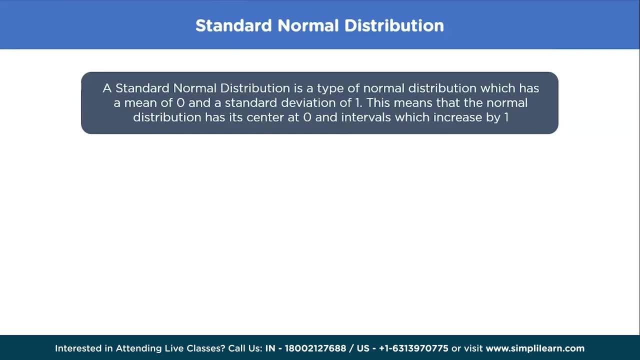 by 1.. All normal distributions, like the standard normal distribution, are unimodal and symmetrically distributed with a bell-shaped curve. However, a normal distribution can take on any value as its mean and standard deviation In the standard normal distribution. however, 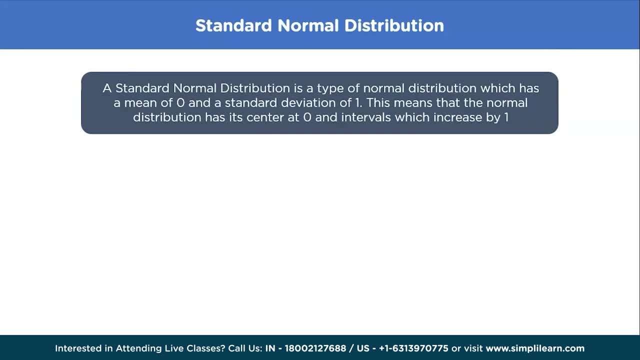 the mean and standard deviation are always fixed. When you standardize a normal distribution, the mean becomes 0 and the standard deviation becomes 1.. This allows you to easily calculate the probability of certain values occurring in your distribution or to compare data sets with different mean and standard. 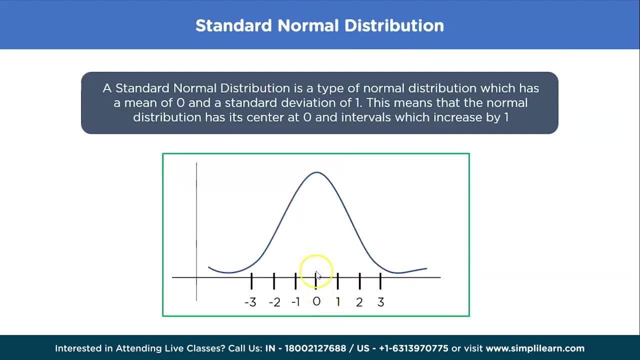 deviations. The curve shows a standard normal distribution. As you can see again, the data is centered at 0.. This does not mean that the data necessarily starts at 0. This means that, after standardizing, this point is where our mean. 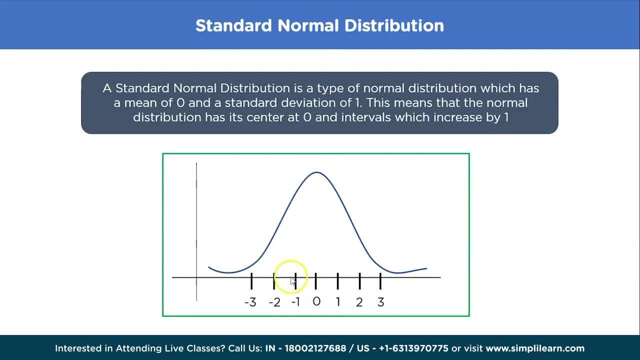 will lie In a standard normal distribution. the standard deviation is 1.. So all the data points will increase or decrease in steps of 1.. Let's better understand a standard normal distribution with the help of an example. Again, as you can see, 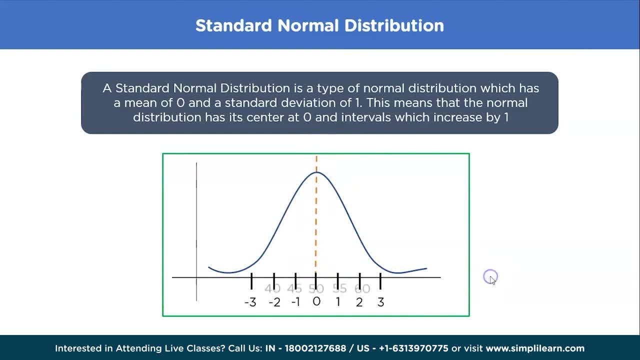 the data is centered around 0,, which is nothing but the mean. Let's again consider the weights of students in class 8.. The average weight here is around 50 kgs and the data increases and decreases in steps of 5.. The data over here: 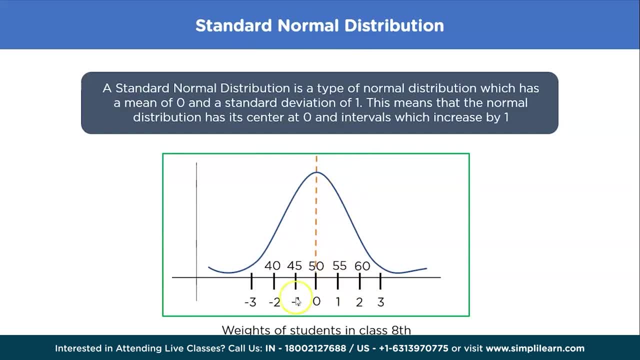 in this curve is evenly distributed along these steps. This is what a standard, normal distribution will look like. We already know that the mean of a data is 50 and because the data is increasing and decreasing in equal steps, we can just standardize it and take. 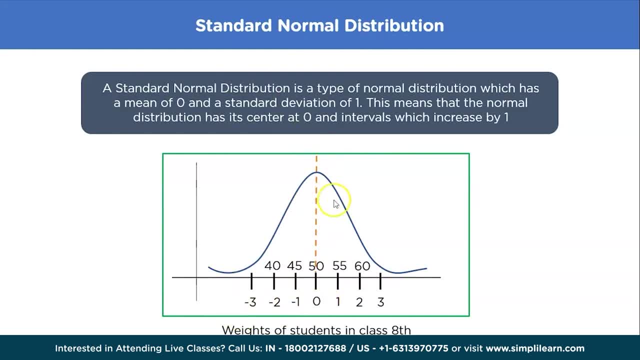 it to mean that the data is increasing and decreasing in steps of 1.. This is what a standard normal distribution looks like, and when you have a data which looks like this, you can always standardize it and convert it into a standard normal distribution. 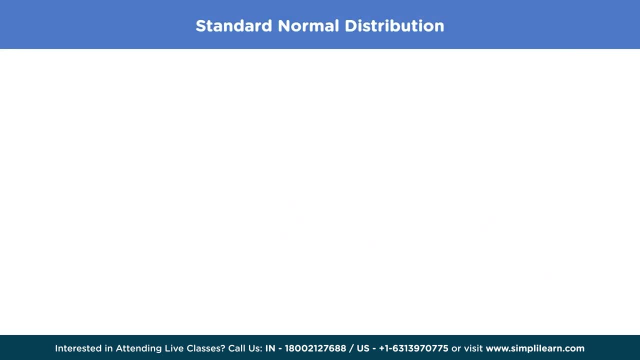 Now, standard normal distribution has a couple of properties which makes calculation comparatively easy. The first one is that 68% of the values fall within the first standard deviation, which means that 68% of all data values on this curve will fall between the range. 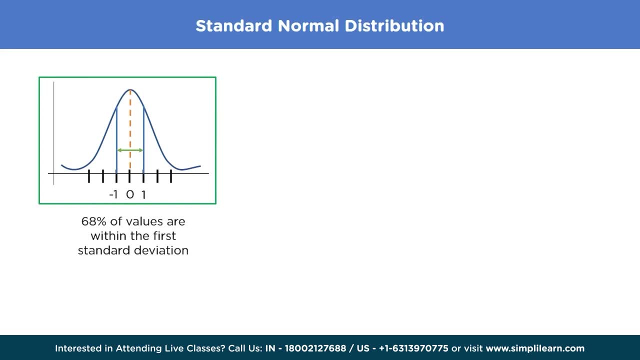 of minus 1 to 1, or the first interval ranging from minus 1 to 1.. The second property is that 95% of the rest of the values are within the second standard deviation, or from the second negative point to the second positive point. 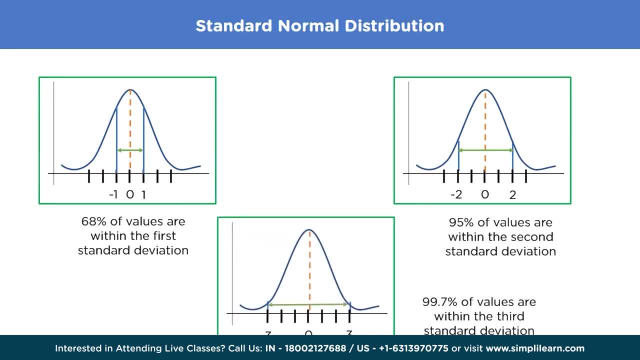 And finally, 99.7% of the values fall within the third standard deviation, or from the third negative point to the third positive point. This makes calculations on standard normal distribution fairly easy. You can compare scores on different distributions with different means and standard deviations. 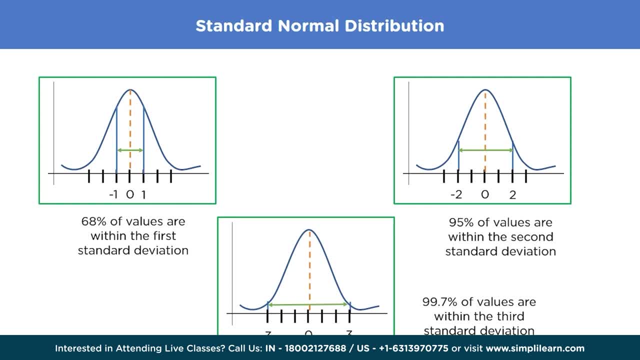 You can normalize scores for statistical decision making using standard normal distribution. You can find the probability of observations and distribution which fall above or below a given value And finally, you can find the probability that a mean significantly differs from a population mean. Now let's 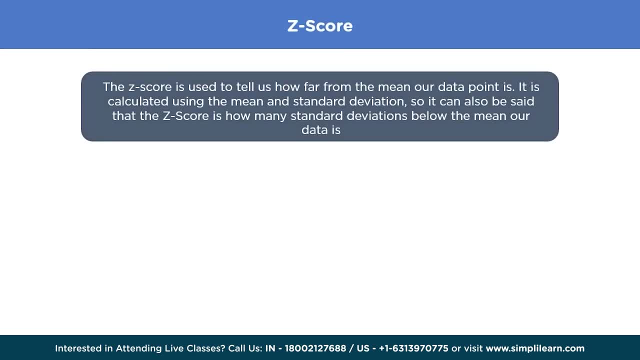 take a look at z-score. So what is a z-score? A z-score is used to tell us how far from the mean our data point actually is. It is calculated using the mean and standard deviation, so it can be said that the z-score is how many standard. 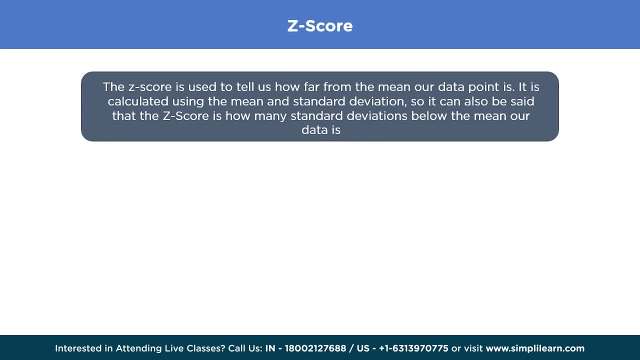 deviations below the mean our data is Basically, by using the z-score, we can get an approximate location of where our data point lies on the graph with regards to the mean. Now, the z-score is given by subtracting the data point from the mean and dividing it by 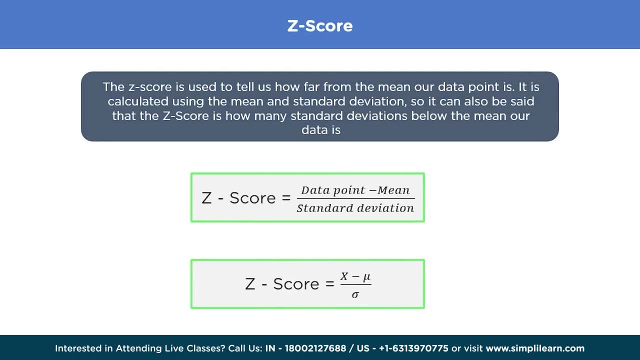 standard deviation. This can also be written as x minus mu divided by sigma. Now any normal distribution can be standardized by converting its values into z-scores. The z-score will tell you how many standard deviations from the mean each values lie, While data points are referred to as x in a. 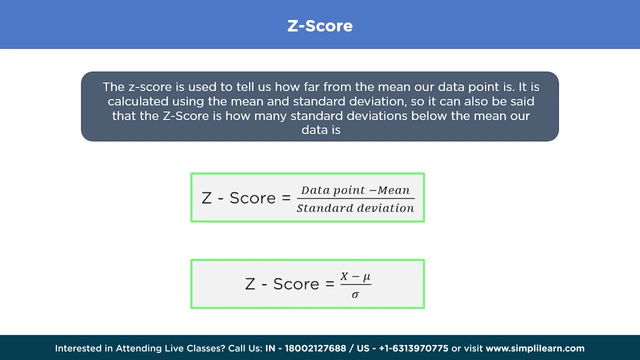 normal distribution they are called z or z-scores in the z distribution. A z-score is a standard score that will tell you how many standard deviations away from the mean an individual point will lie. A positive z-score will mean that your x value is. 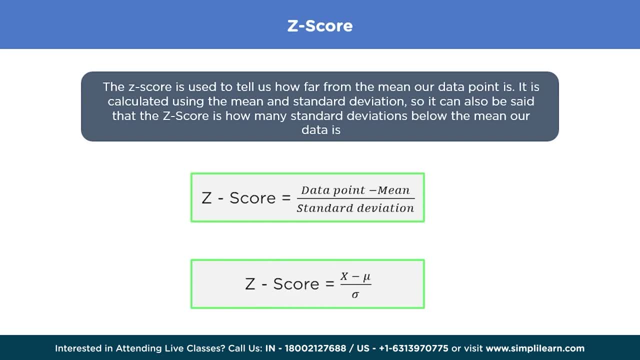 greater than the mean, and a negative z-score will mean that your x value is less than the mean. A z-score of 0 will mean that your x value is equal to the mean. And again, to standardize a value from a normal distribution, all we have. 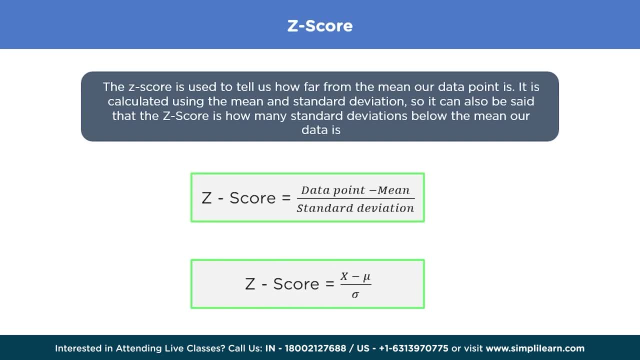 to do is convert it to a z-score by subtracting the mean from our individual value and dividing it by the standard deviation. Now let's see how we can find the z-score from data points with the help of a solved example. Let's do a case. 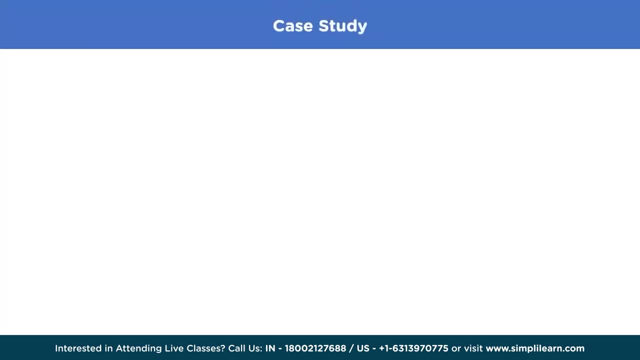 study. In this case study, we'll be taking the summary of daily travel time of a person who's commuting to and from work. All these values are in minutes and using these values we have to calculate the mean, the standard deviation and the 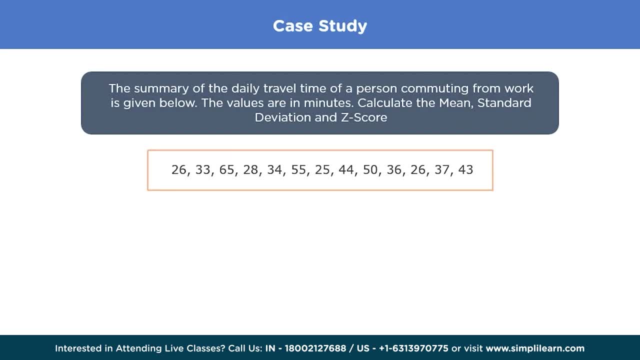 z-score. These values are as shown. As we can see, there are 13 values in total. Let's start by finding the mean. The mean is the average and it can be gotten by adding all of these values and dividing it by the total number of. 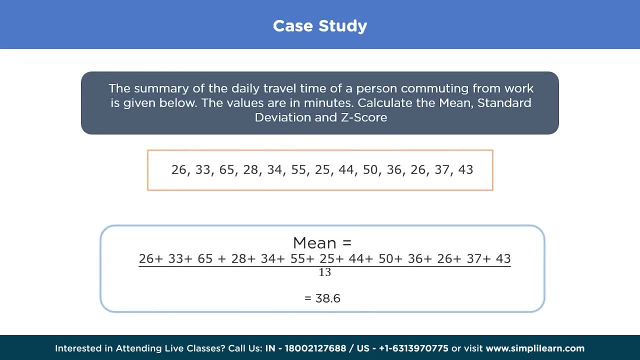 values. This gives us a value of 38.6.. The mean tells us the average of all our data points, which means, on an average, he travels for 38.6 minutes to reach work. Next, let's subtract the individual values. 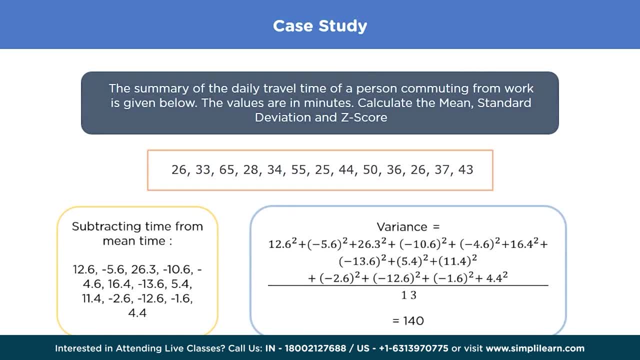 from our mean and calculate the variance and standard deviation. The values on the left give us the values that we get after subtracting it from the mean, and the variance can be calculated by squaring all of these values, adding up all of the squared values and. 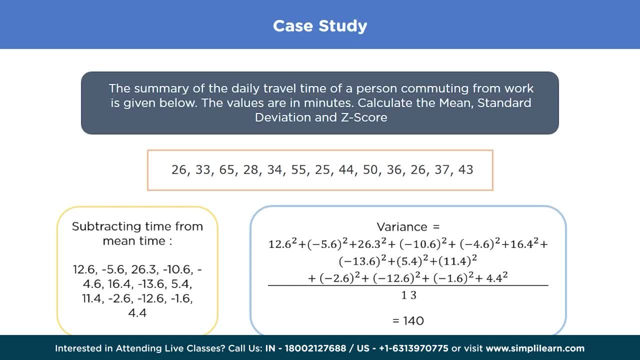 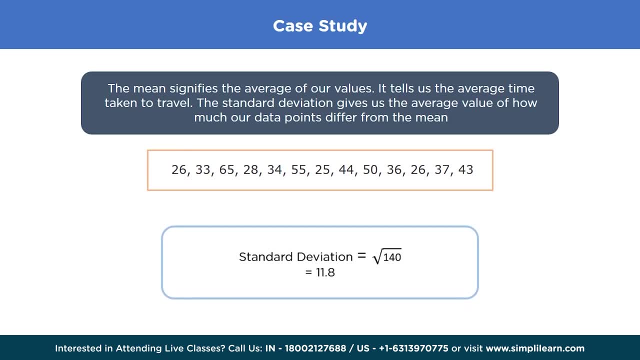 dividing it by the total number of values, At the end of the day we get a variance of 140.. To calculate the standard deviation, all we have to do is take a square root of the variance, which gives us a value of 11.8.. 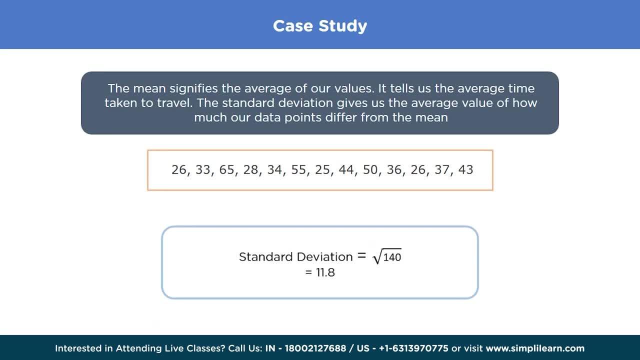 Now, the mean signifies the average of our values and we already know this. It gives us the average time which is taken to travel, but the standard deviation will tell us the average value of how much our data points differ from the mean. It tells us the deviation. 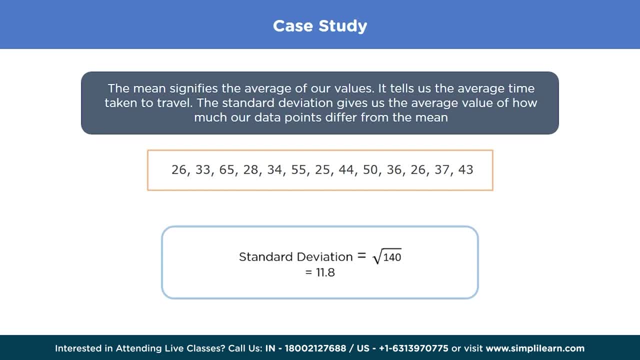 within our own data and it tells us how far away, on an average, a point is from the mean. Now the value that we get is 11.8, which means that, on an average, a single data point is around 11.8 data points away. 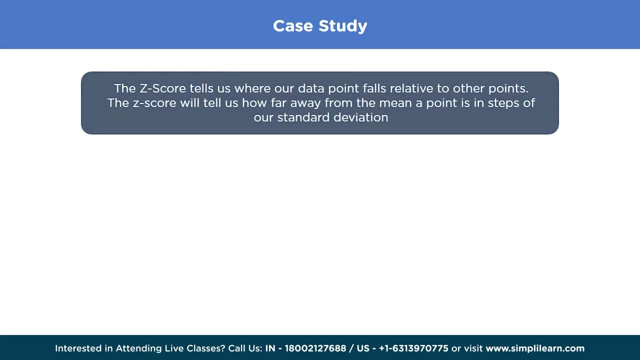 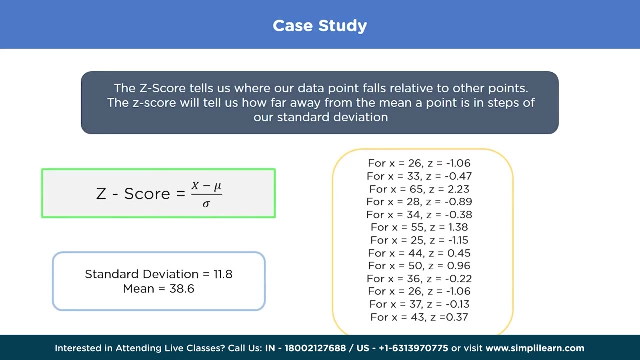 from the mean. Now let's calculate the z-score. The z-score is given by subtracting individual data points from the mean and dividing it by the standard deviation. We know that we have a standard deviation of 11.8, and a mean of. 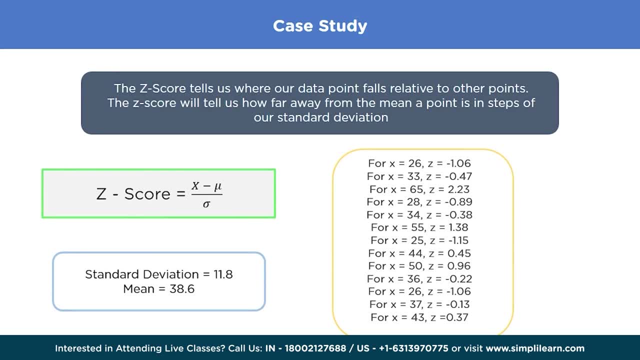 11.6.. Using these values, we can calculate the z-scores for individual x-values. Now we know that a negative z-score means that our x-value is lower than our mean. But what does the number 1.06 mean? 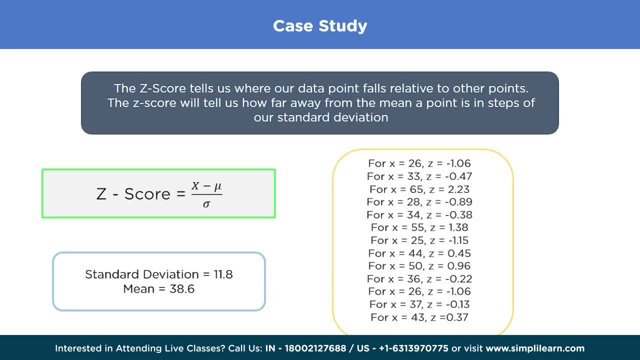 This means that the z-score for 26 is 1.06 standard deviations away from the mean. The negative symbol here means that our x-value is less than the mean. And by how? less 1.06 times the standard deviation. Now we know that. 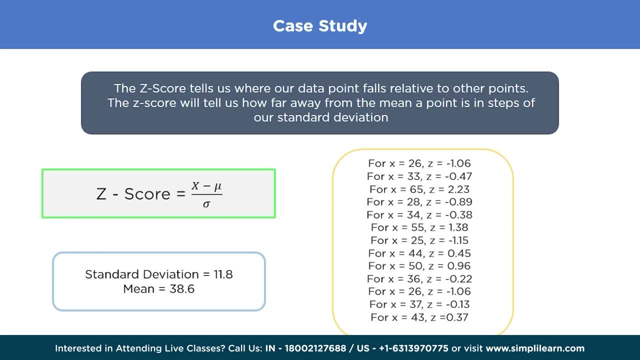 the negative value of a z-score means that our x-value is less than our mean. But what does the number 1.06 mean? This means that the z-score is 1.06 times the standard deviation less than the mean. The same. 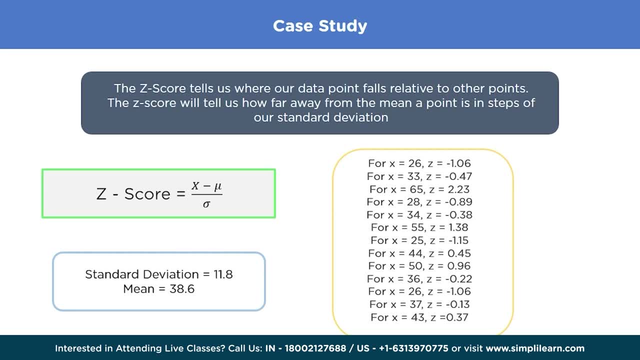 thing can be said for the z-score of 33.. It is 0.47 times the standard deviation, less than the mean. The z-score of 65 is 2.23 times the standard deviation, more than the mean. That means it has to be. 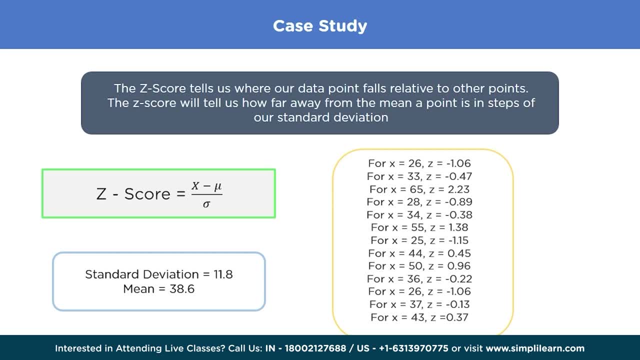 added to the mean. The reason that we know it's more than the mean is because this has a positive value. So this means that, using z-scores, we can know where our data points fall relative to other points on the graph. The z-score will tell us how. 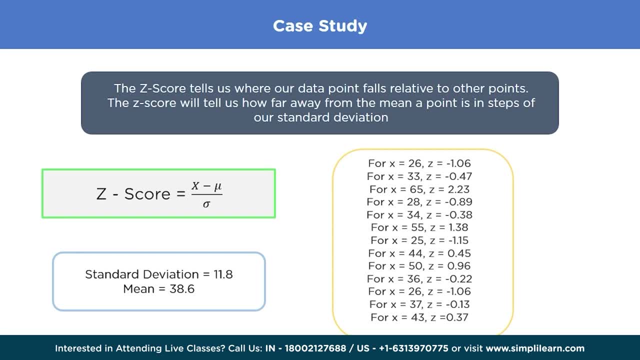 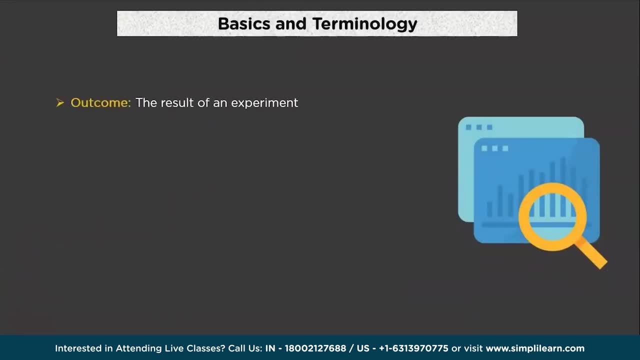 far away from the mean. a point is in steps of our standard deviation Basics and terminology Basics and terminology Basics and terminology. The first one is outcome. Whenever we do an experiment, like flipping a coin or rolling a dice, we get an outcome. For example, if we flip a coin. 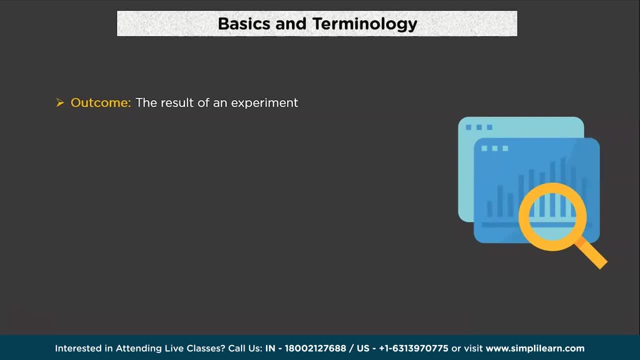 we get an outcome of heads or tails, And if we roll a die, we get an outcome of 1,, 2,, 3,, 4,, 5 or 6. Random experiment: A random experiment is any well-defined procedure that produces. 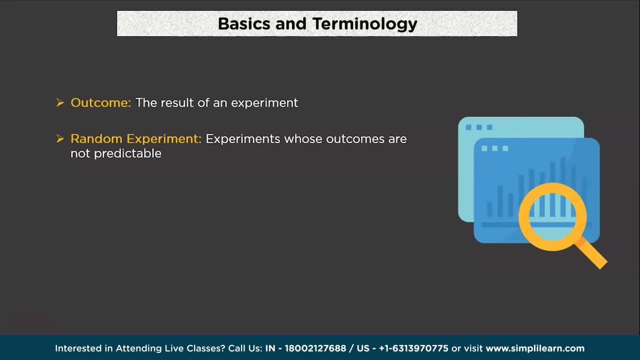 an observable outcome that could not be perfectly predicted in advance. A random experiment must be well-defined to eliminate any vagueness or surprise. It must produce a definite, observable outcome so that you know what happened after the random experiment is run. Random events: Consider a simple. 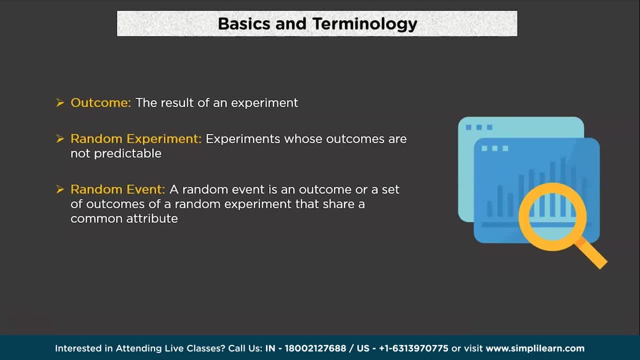 example, Let us say that we toss a coin up in the air. What can happen when it gets back? It either gives a head or a tail. These two are known as outcome, and the occurrence of an outcome is an event. Thus, the event is the. 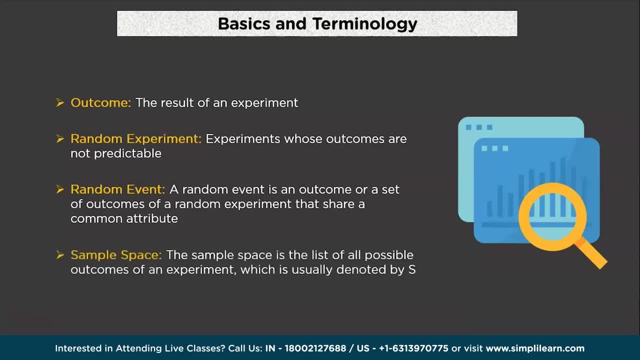 outcome of some phenomenon. The last one is sample space. A sample space is a collection or a set of possible outcomes of a random experiment. The sample space is represented using the symbol S. The subset of all possible outcomes of an experiment is called events, and a sample space may. 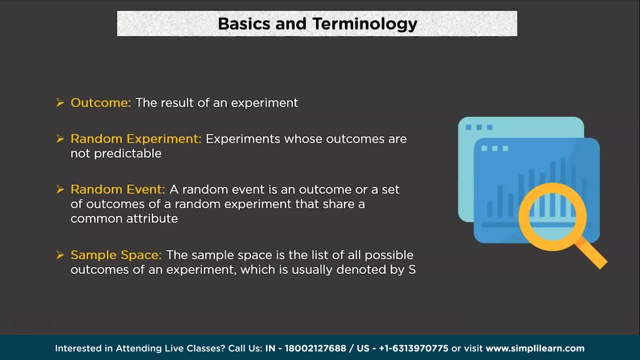 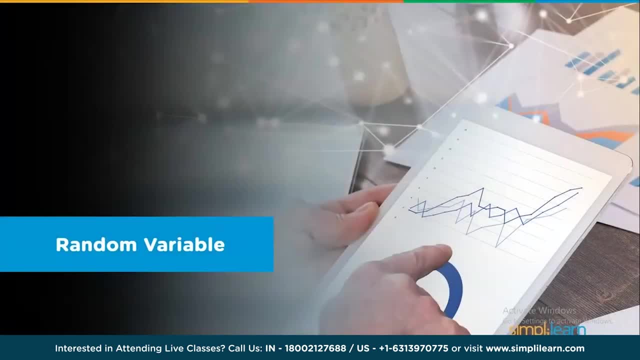 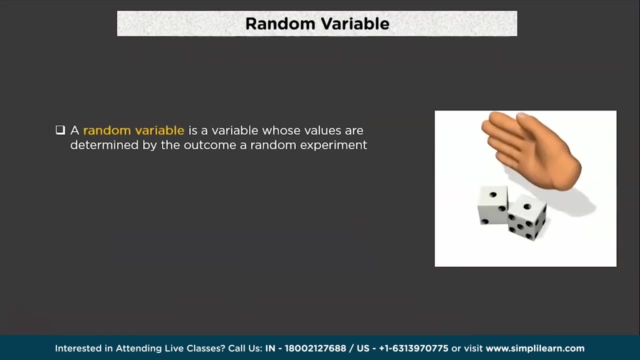 contain a number of outcomes. that depends on the experiment. If it contains a finite number of outcomes, then it is known as a discrete or finite sample spaces. Now let's discuss what is random variable. A random variable is a numerical description of the outcome of a statistical experiment. 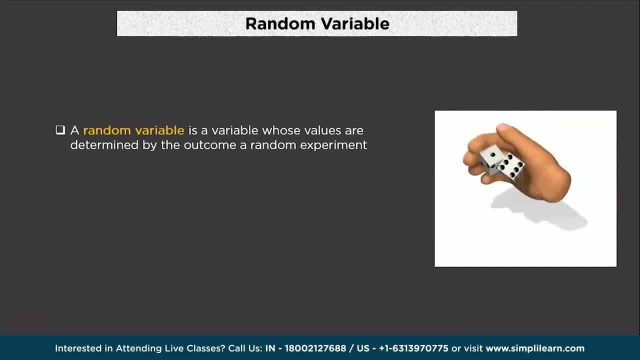 A random variable that may assume only a finite number of values is said to be discrete. One that may assume any value in some interval on the real number line is said to be continuous. Let's see an example. Let X be a random variable defined as the sum of 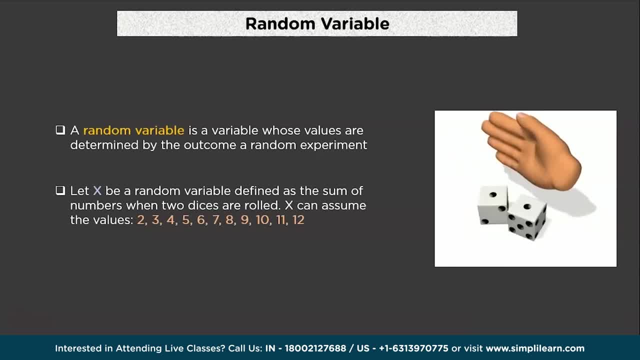 numbers. when two dice are rolled, X can assume the values 2,, 3,, 4,, 5,, 6,, 7,, 8,, 9,, 10,, 11 and 12.. Notice: there is no 1 here. 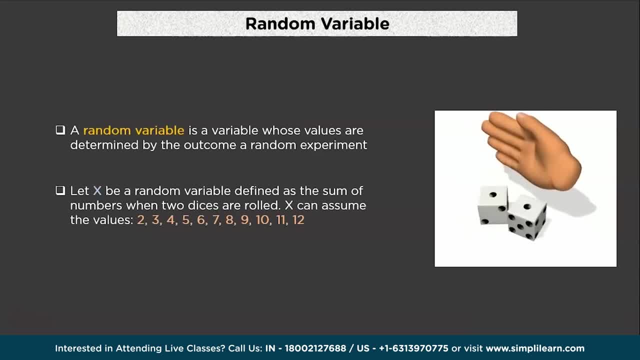 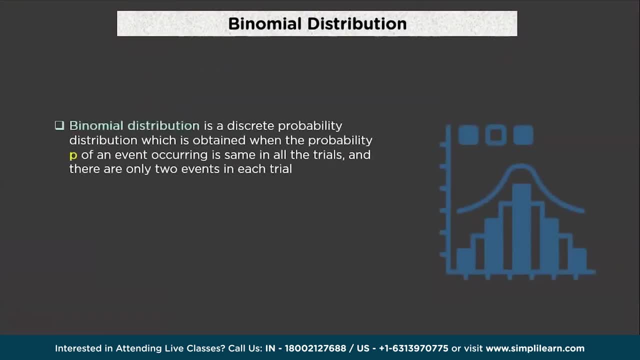 because the sum on the two dice can never be 1.. Now that we know the basics, let's move on to binomial distribution. The binomial distribution is used when there are exactly two mutually exclusive outcomes of a trial. These outcomes are appropriate. 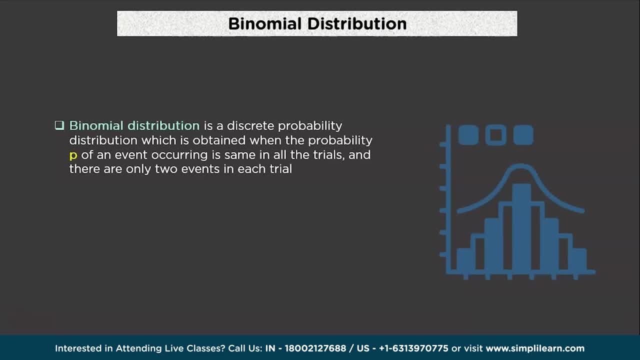 labeled success and failure. The binomial distribution is used to obtain the probability of observing X successes in n number of trials, with the probability of success on a single trial denoted by P. The binomial distribution assumes that P is fixed for all the trials. 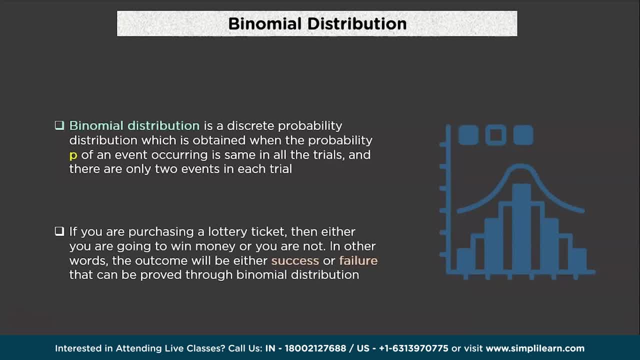 Here is a real-life example of a binomial distribution. Suppose you purchase a lottery ticket, then either you are going to win the lottery or not. In other words, the outcome will be either success or failure. that can be proved through binomial distribution. 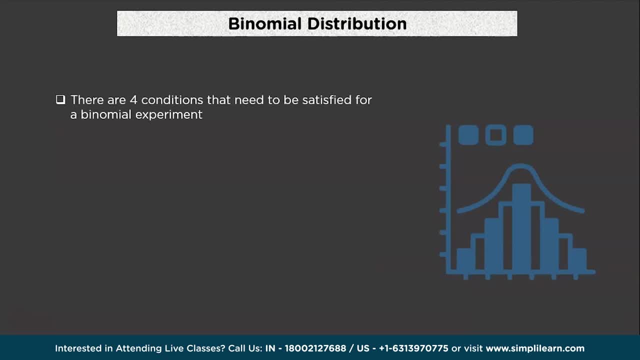 There are four important conditions that needs to be fulfilled for an experiment to be a binomial experiment. The first one is there should be a fixed number of n trials carried out. The outcome of a given trial is only 2, that is either a success or a failure. 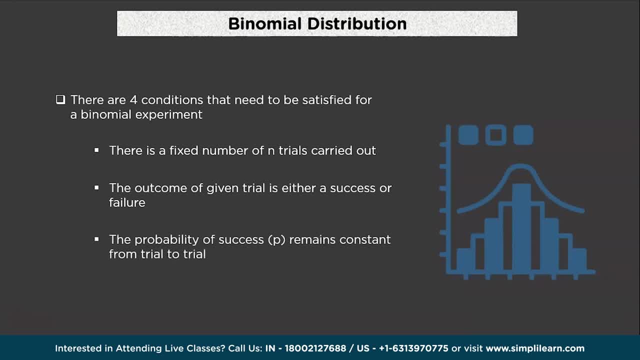 The probability of success remains constant from trial to trial. It does not change from one trial to another And the trials are independent. The outcome of a trial is not affected by the outcome of any other trial. To calculate the binomial coefficient, we use: 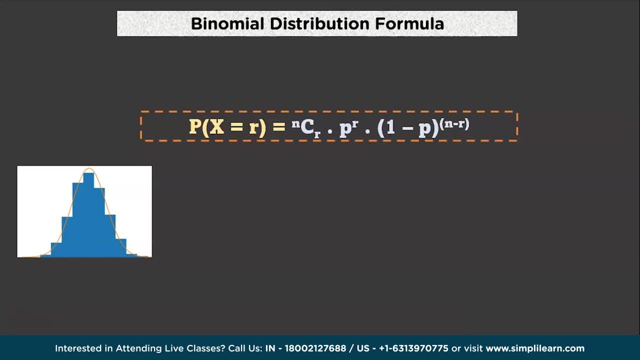 the formula, which is: nCr into P to the power r, into 1-P to the power n-r, where r is the number of success in n number of trials and P is the probability of success. 1-P denotes the probability of a failure. 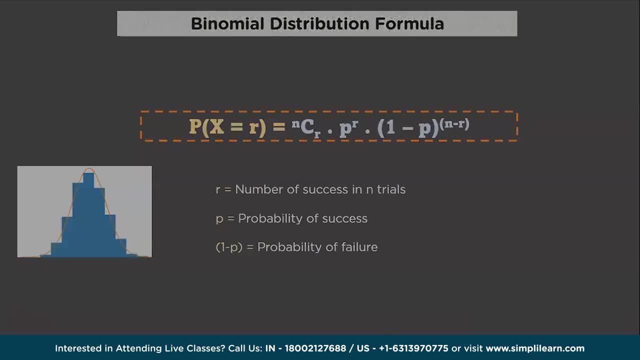 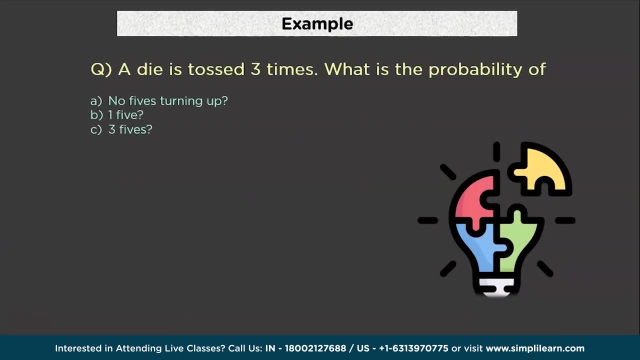 Now let's use this formula to solve an example. Suppose a die is tossed three times. What is the probability of no 5 turning up? 1-5 and 3-5 turning up? To calculate the no 5 turning up here, r is equal to. 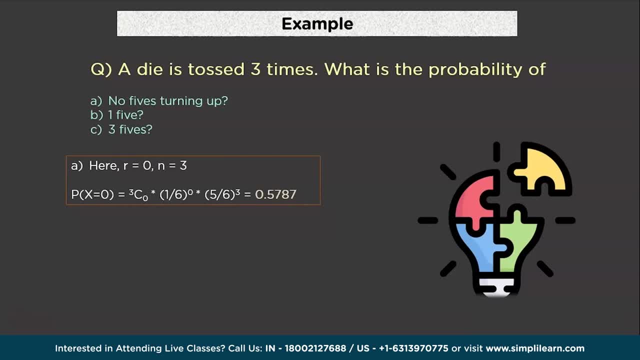 0 and n is equal to 3.. Substituting the value in the formula, we have 330 into 1-6, to the power 0, into 5-6 to the power 3, where 1-6 is the probability of. 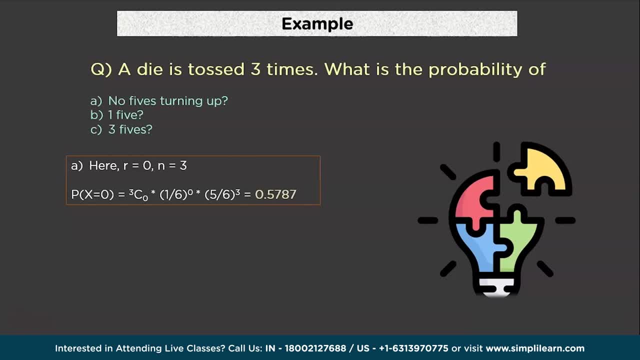 success and 5-6 is the probability of failure. Calculating this equation, we will get the value to be 0.5787.. In a similar manner, to calculate the probability of 1-5 turning up, we will replace r with 1. 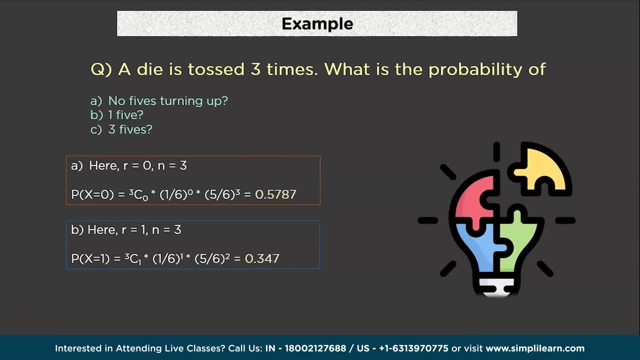 and n will be 3.. So P will be equal to 3C1 into 1-6, to the power 1, into 5-6 to the power 2, which will come out to be 0.347.. And for 3-5, turning up, 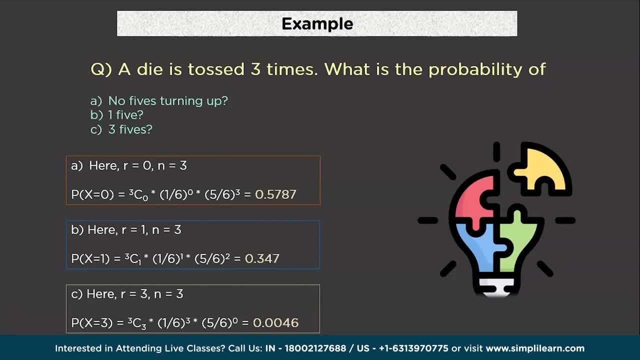 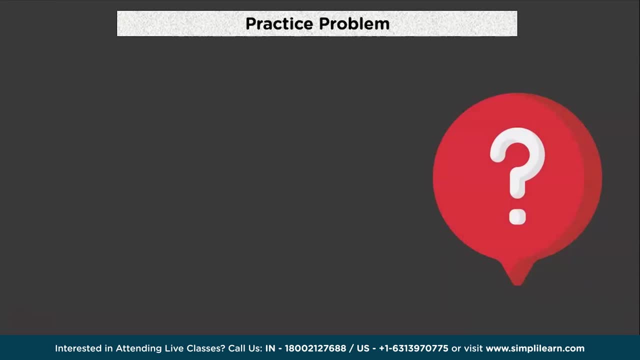 we will substitute r equal to 3 and the formula will remain the same and we will get the value to be 0.0046.. Now that we are done with the concepts of animal probability distribution, here is a problem for you to solve. 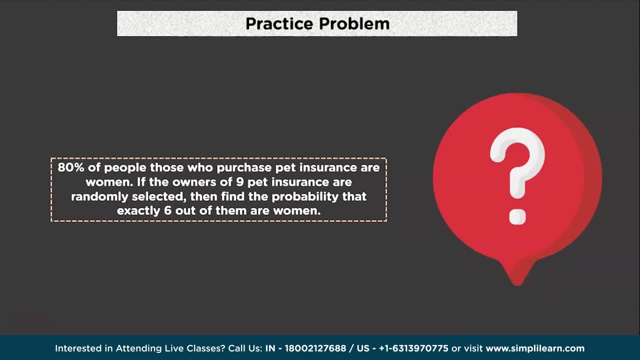 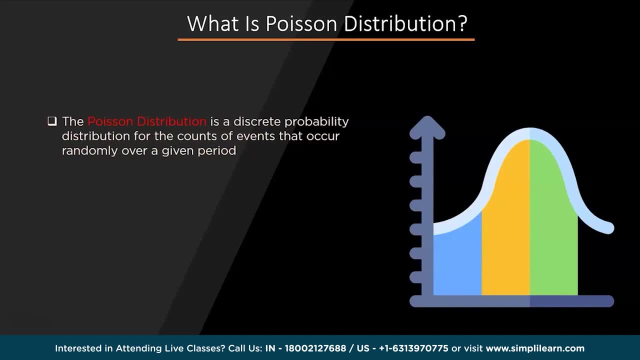 Post your answers in the comment section and let us know. A Poisson distribution is a probability distribution used in statistics to show how many times an event is likely to happen over a given period of time. To put it another way, it's a count. 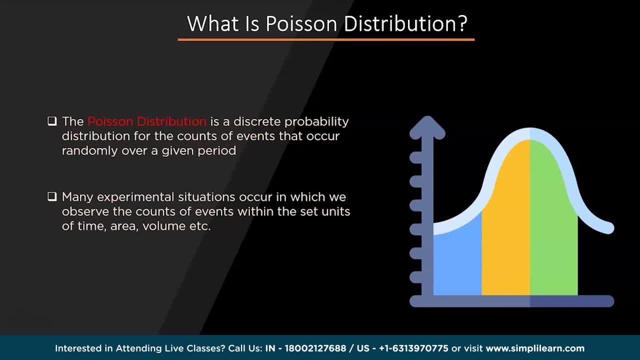 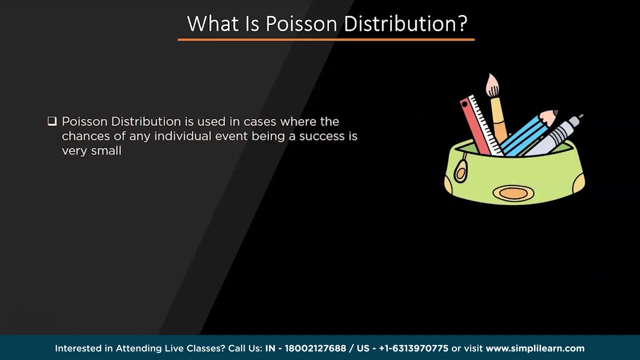 distribution. Poisson distributions are frequently used to comprehend independent events at a constant rate over a given interval of time. The Poisson distribution was developed by French mathematician Simon-Denis Poisson in 1837.. A Poisson distribution is used in cases where the chances of 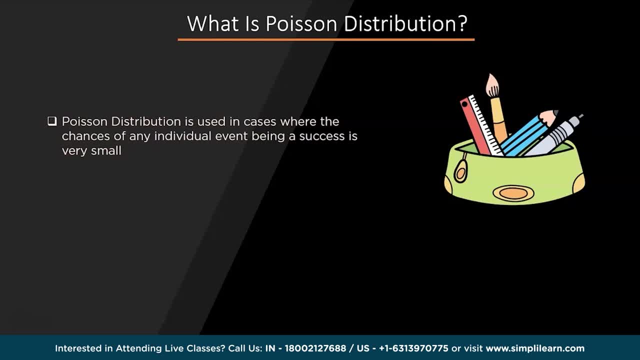 any individual event being a success is very small. The number of defective pencils per box of a 6000 pencil, the number of plane crash in India in one year, or the number of printing mistakes in each page of a book- All of these examples can have use of. 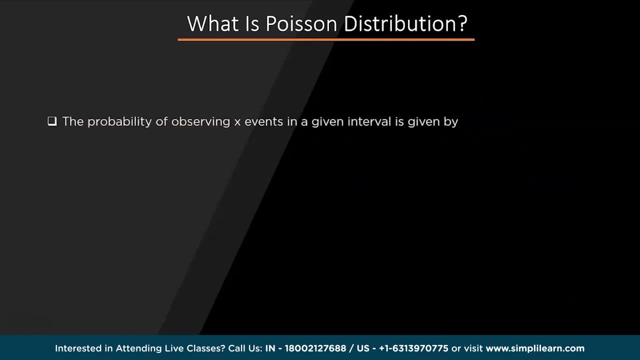 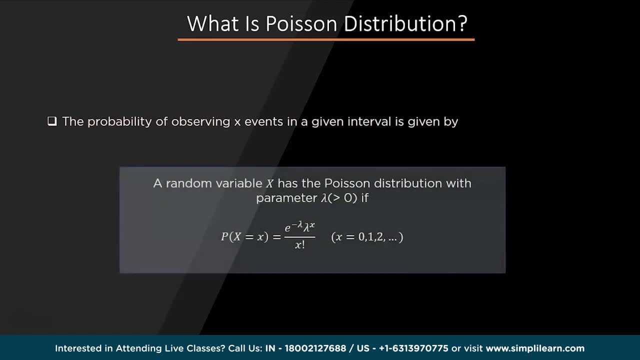 Poisson distribution. The Poisson distribution can be used to calculate how likely it is that something will happen x number of times. A random variable, x, has a Poisson distribution with parameter lambda and the formula for that is: e to the power minus lambda into lambda to the power x divided by. 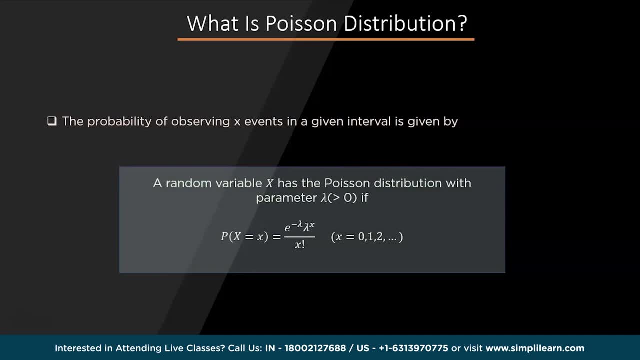 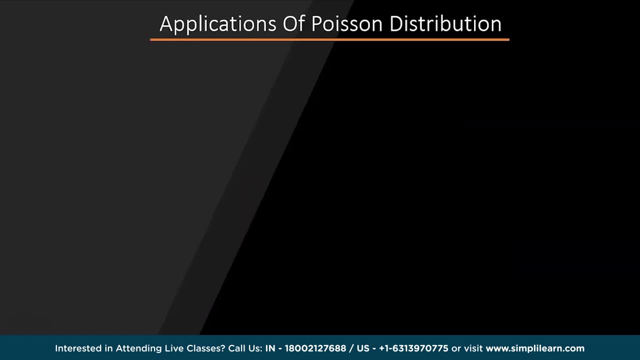 x factorial, Where x can be the number of times the event is happening, The value of e is taken as 2.7182.. Let's discuss some application of Poisson distribution. If you want to calculate the number of deaths per day or week due to rare disease in a 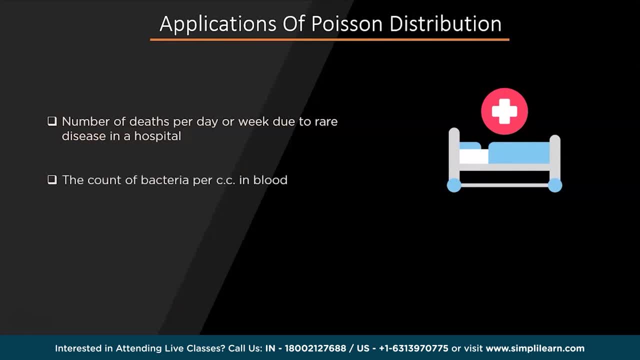 hospital. you can use the Poisson distribution In a similar manner. the count of bacteria per cc in blood or the number of computers infected as virus per week, The number of mishandled baggage per 1000 passengers can also have an application for Poisson distribution. 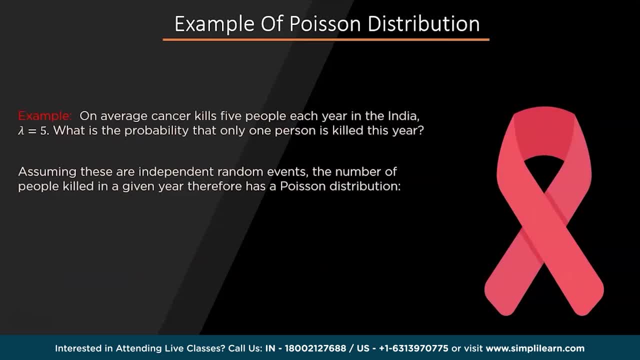 Let's discuss one example to see how we can calculate a Poisson distribution Suppose on an average, cancer kills 5 people each year in India. What is the probability that one person is killed this year? We will assume all these events are independent, random events. 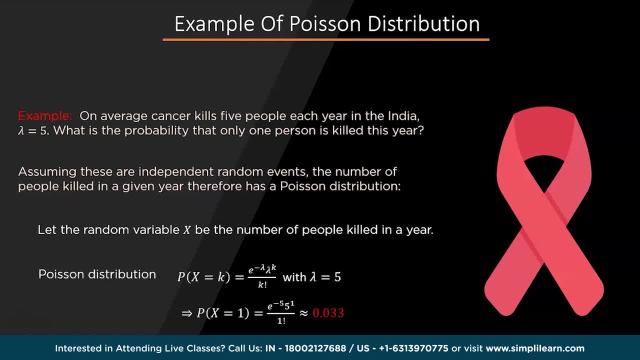 So by the formula we have, x is equal to 1 because we have to calculate the probability of one person that is killed this year. So P will be equal to e, to the power minus 5 into 5, to the power 1 divided by 1 factorial. 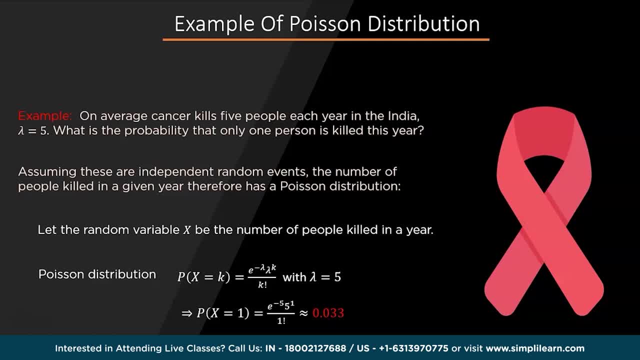 which will come out to be 0.033, which will be near to 3.3%. So the probability that only one person is killed this year due to cancer is 3.3%. Now we have one question for you. Do try to answer. 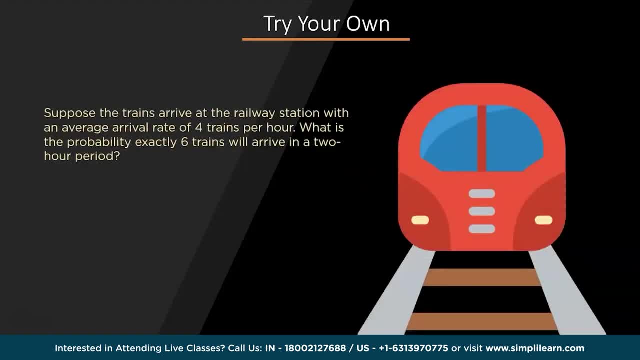 in the comment section. Suppose the trains arrive at a railway station with an average arrival rate of 4 trains per hour, What is the probability exactly 6 trains will arrive in a 2 hour period. And here are your options. Please do let us know your answers in the comment section. 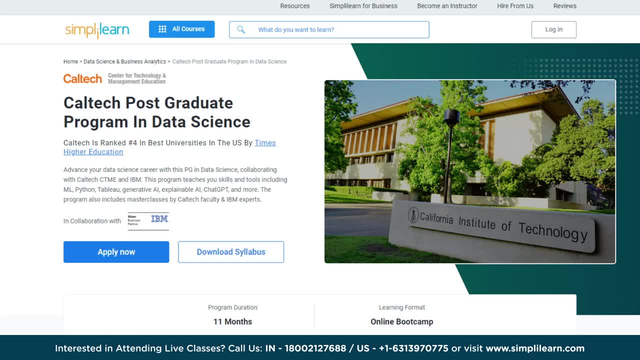 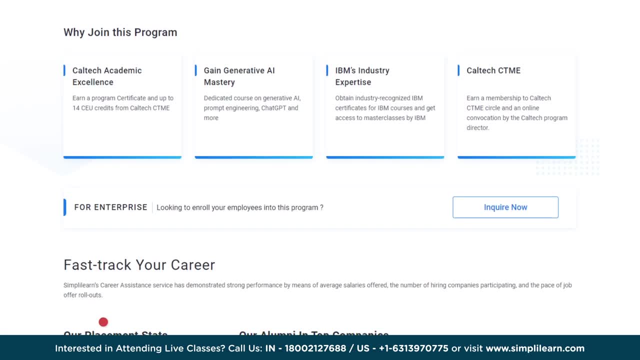 SimplyLearn's post graduate program in data science, offered by Caltech University in collaboration with IBM, is just what you need. For more details, head straight to our homepage and search for data science post graduate program, or simply click on the link in the description box below. 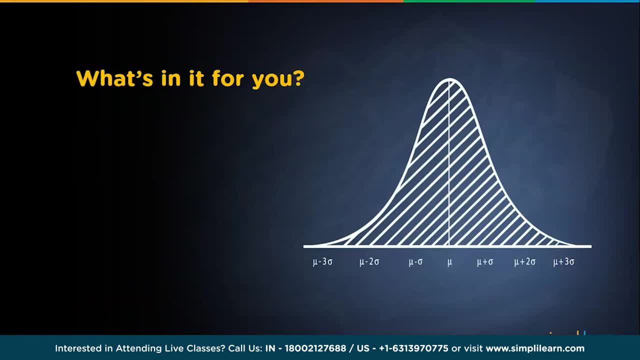 So what can you expect from this video? What's in it for you? First, we will take a look at what is normal distribution. Next, we will look at the concept of standard deviation, Followed by standard normal distribution. A normal distribution. 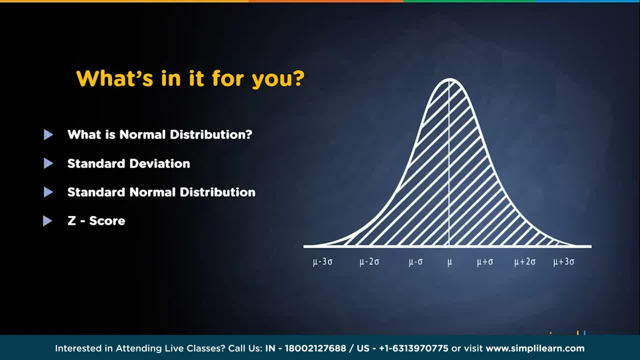 which has been standardized. Finally, we will take a look at what is z-score, And then we will take a look at a solved problem in which we will find the standard, deviation and mean and the z-score of a data set. So let's get. 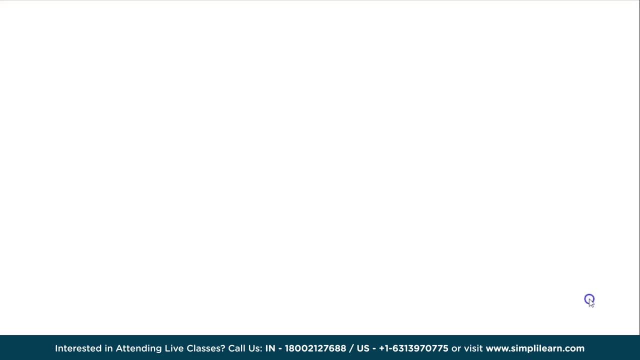 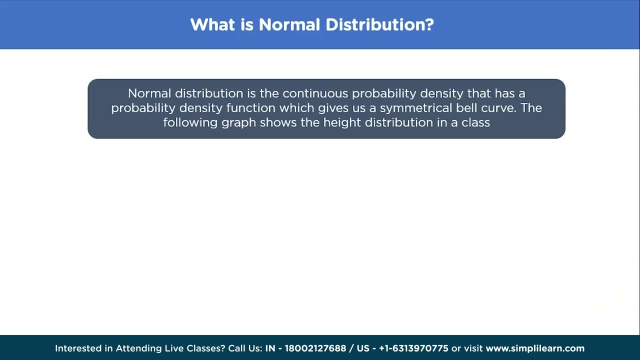 started. So what is normal distribution? Normal distribution is a continuous probability density that has a probability density function which gives us a symmetrical bell curve. Now data can be distributed or spread out in different ways, But there are many cases where the data tends to be. 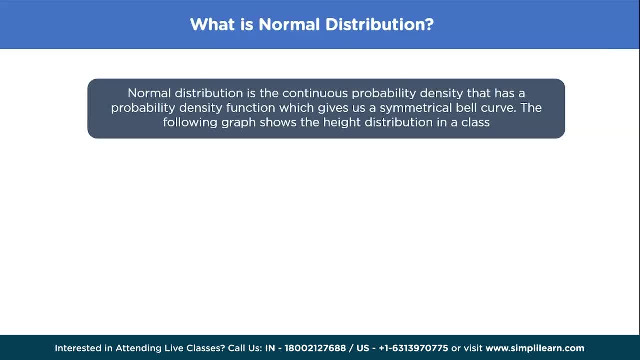 around a central value with no bias to the left or right, Which means that it doesn't show any particular spikes towards the left or the right, And it gets close to a normal distribution. Half of the data will fall on the left of the mean and the other half will. 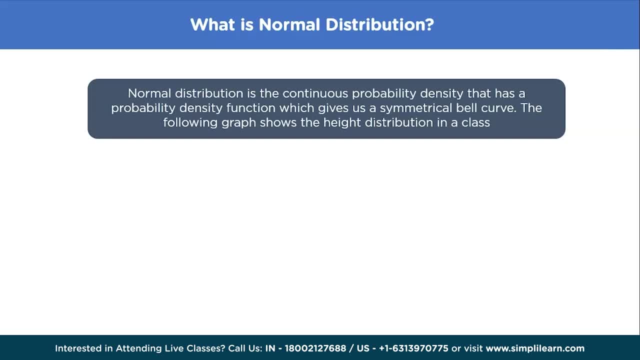 fall on the right. Now let's take a look at a graph which shows the height distribution in a class. As you can see, the average height is in the middle and the data to the left of the average height represents the short people and the data to the right of it represents 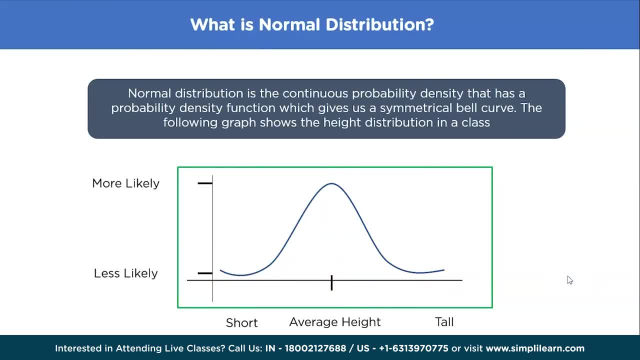 the taller people. The y-axis shows us the likelihood of any of these heights occurring. The average height has the most distribution or it has the most number of cases in the class And as the height decreases or increases the number of people who have that. 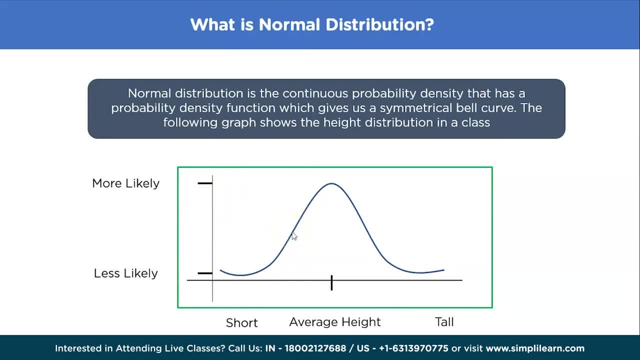 height also decreases. This kind of a distribution is called a normal distribution, where the average or the mean is always the highest point and any other point after that or before that is significantly lower. The resulting data gives us a bell curve and, as you can see, there is no abrupt bias. 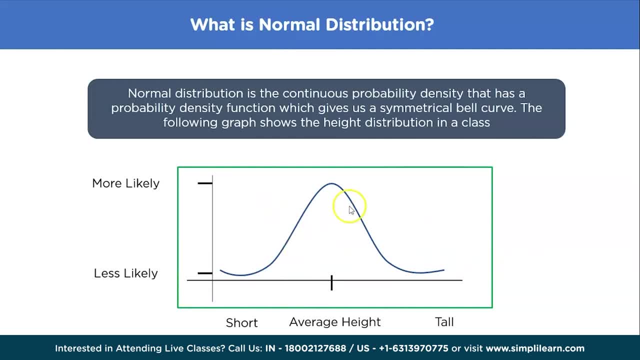 or spike in the data anywhere except for the average height. So this kind of a curve is called a bell curve and it's usually seen in a normal distribution. The reason we call this a normal distribution is because the data is normally distributed with the average being the. 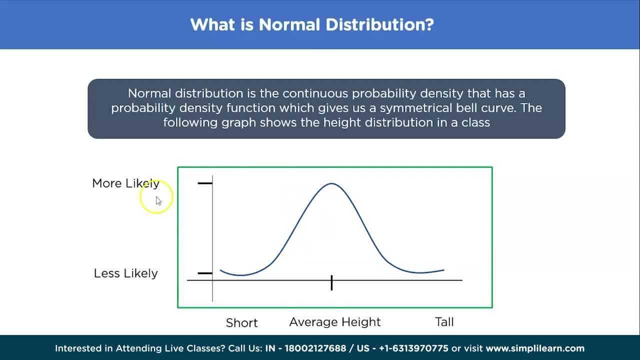 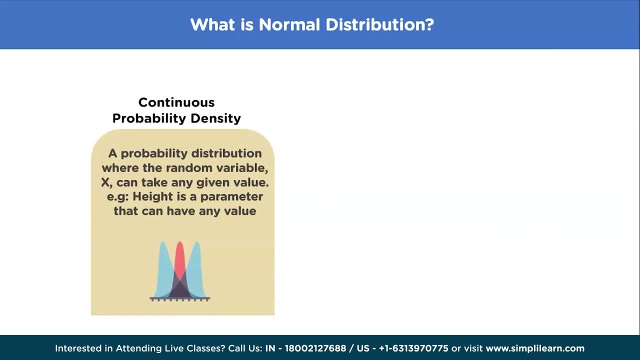 highest and all the other data points having a lower likelihood. Now we came across two terms which are associated with normal distribution: continuous probability density and probability density function. What is continuous probability density? Continuous probability density is a probability distribution where the random variable x can take. 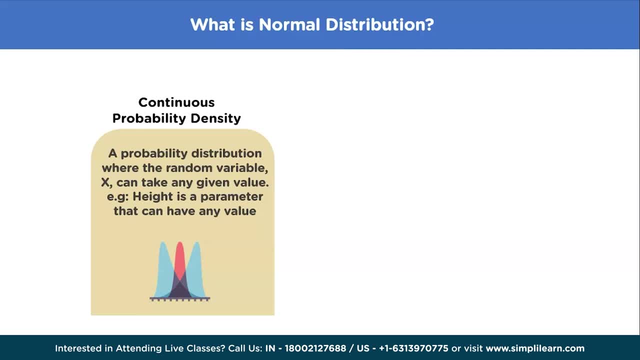 any given value. Because there are infinite values that x could assume. the probability of x taking on any specific value is zero. For example, let's say you have a continuous probability density for men's height. What is the probability that a man will have? 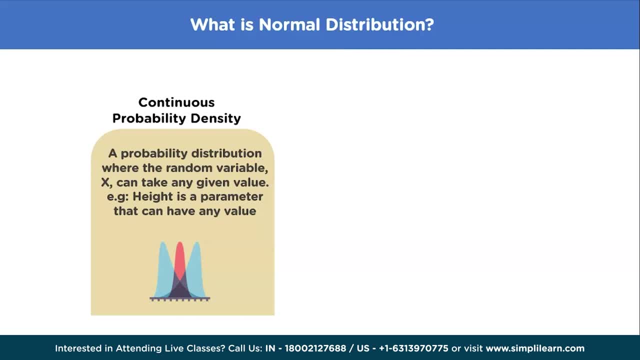 the exact height of 70 inches. It is impossible to find this out because the probability of one man measuring exactly 70 inches is very low. It is more probable that he will measure around 70.1 inches or maybe 69.97 inches. 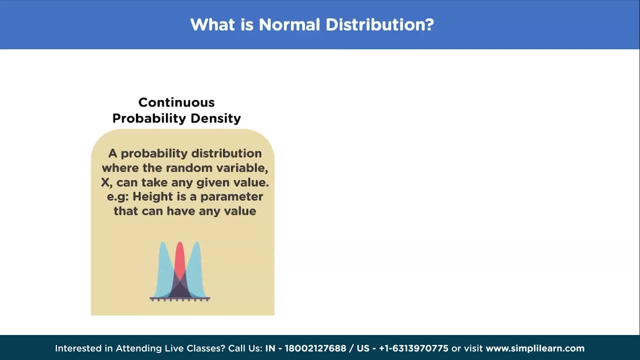 and it doesn't stop there. The fact is that it's impossible to exactly measure any variable that's on a continuous scale and because of this it's impossible to figure out the probability of one exact measurement which is occurring in a continuous probability density. Next we have the probability: 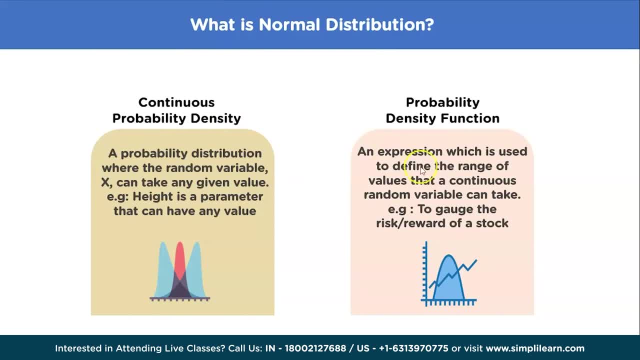 density function. It's nothing but a function or an expression which is used to define the range of values that a continuous random variable can take. An example of this would be to gauge the risk and reward of a stock. A probability density function is a statistical measure which is used. 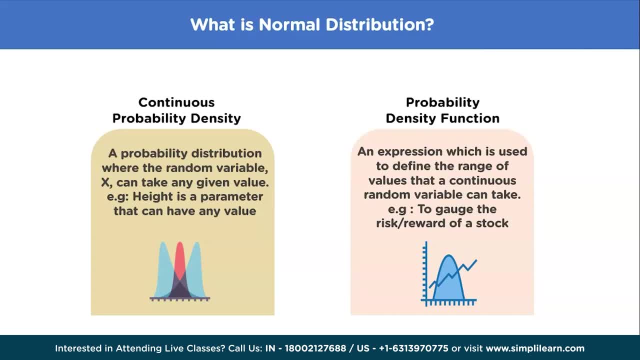 to gauge the likelihood of a discrete value. A discrete variable can be measured exactly, while a continuous variable can have infinite values. However, for both continuous as well as discrete variables, we can define a function which gives us the range of values within which these variables will fall. 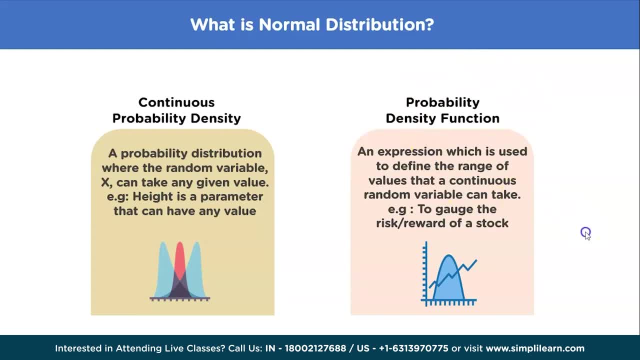 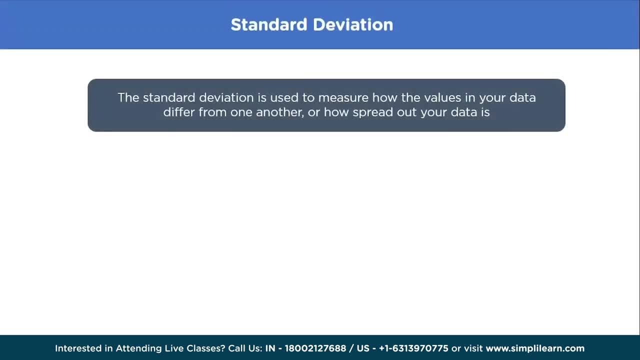 And that function is known as the probability density function. Now let's take a look at standard deviation. What is standard deviation? Standard deviation is used to measure how the values in your data differ from one another, or how spread out your data is. A standard deviation is a statistic. 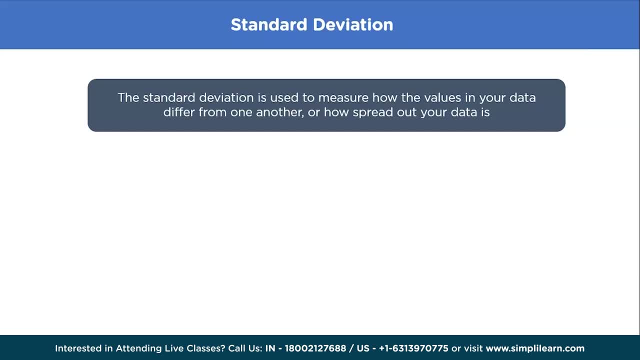 that measures the dispersion of a data set relative to its mean. The standard deviation is calculated as the square root of variance by determining each data point's deviation relative to the mean. If the data points are further from the mean, that means that there is a higher. 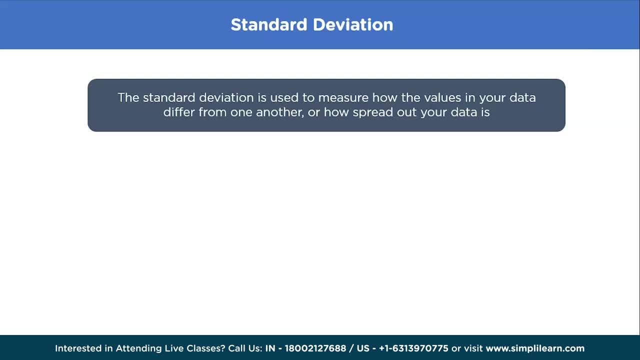 deviation within the data set, and then the data is said to be more spread out. This leads to a higher standard deviation too. Let's take an example of income in rural and urban areas. In rural areas, let's say, such as farming areas, 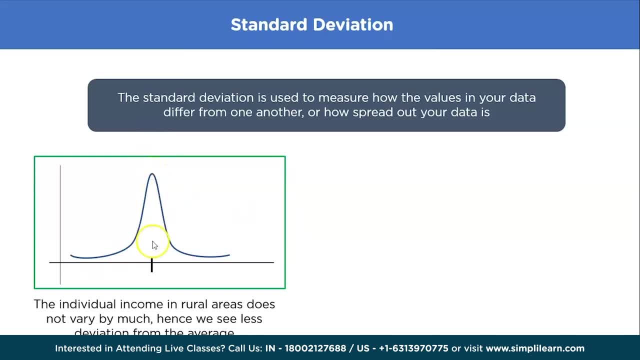 the income doesn't differ that much. More or less everyone earns the same. Because of this, our bell curve has a very low standard deviation and it has a very narrow peak. However, in urban areas, the wealth distribution is very uneven. Some people can have very high incomes. 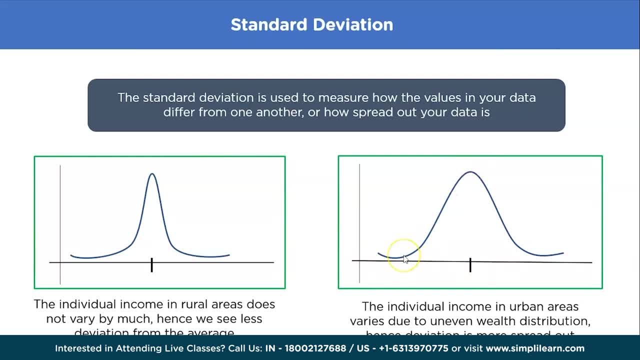 and can be earning a lot, while other people can have very low incomes. Furthermore, the data distribution between these two income points is going to be more spread out because there are a lot more people living there who work in various fields and who have various incomes Because of this. 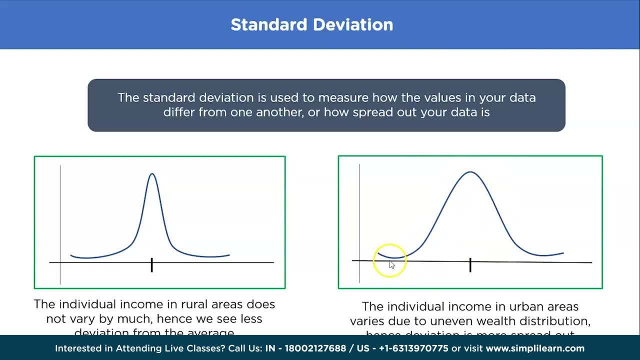 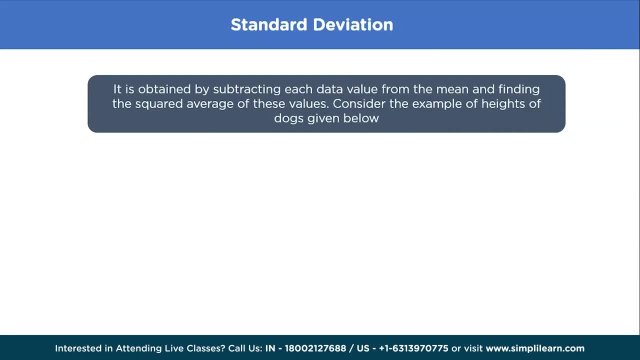 our standard deviation is more spread out and our bell curve will also have a wider peak. Now how can we find the standard deviation? Standard deviation is obtained by subtracting each data value from the mean and finding the squared average of these values. Let's look at how we can do. 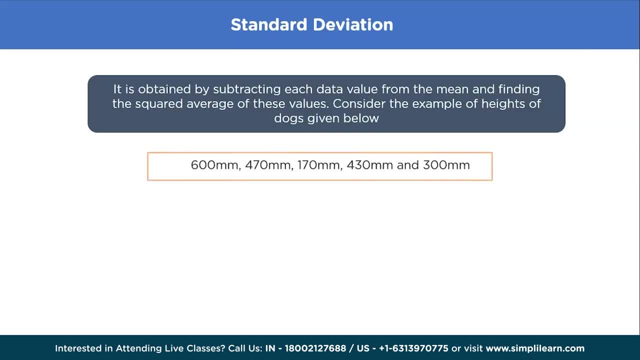 this with the help of an example. These values correspond to the height of various dogs. We can find the mean by finding the average of all these values, which is nothing but adding all the values and dividing it by the total number of values. The mean that 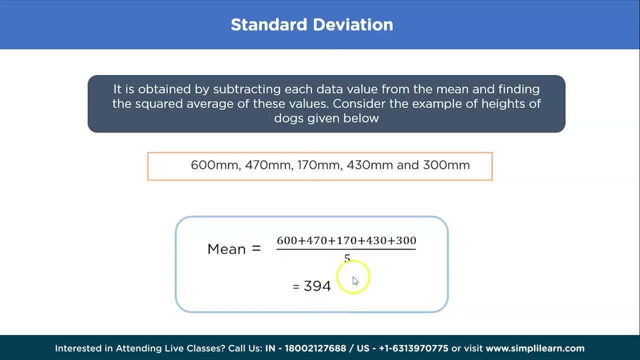 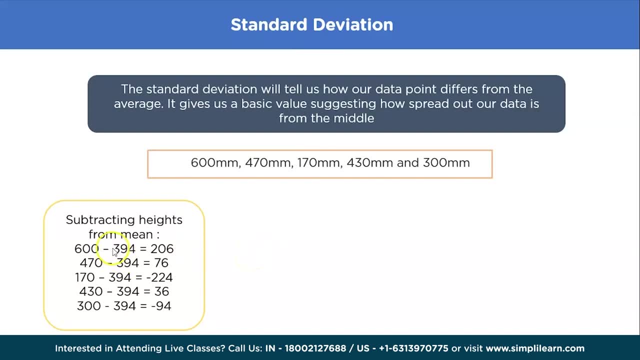 we get is 394.. This means that the average height of a dog is 394,, which means that the average height of a dog is 394 millimeters. To find the standard deviation, first we need to subtract the height from the mean. This will tell us. 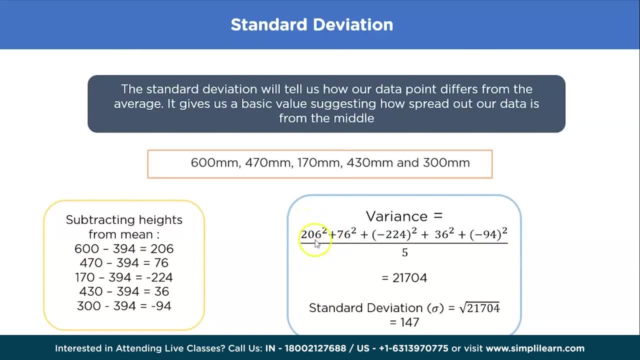 how far from the mean our data points actually are. Next, we will square up all of these differences and add them up and again divide it by the total number of values that we have. This is called the variance- The variance that we get in this case. 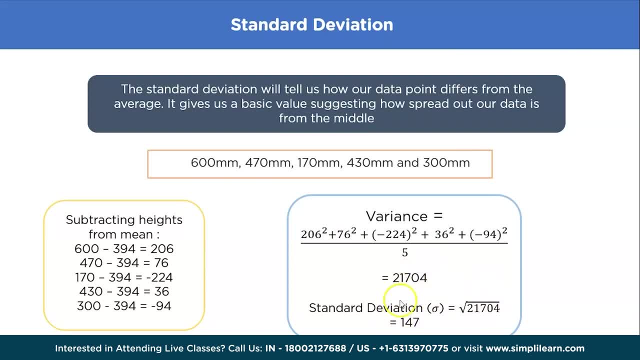 is 21704.. Finally, when we find the square root, the standard deviation here is 147.. The standard deviation will tell us how our data points differ from the average and it gives us a basic value suggesting how spread out our data is from the very middle. 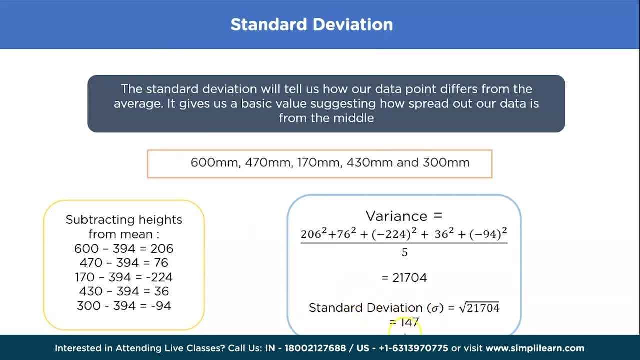 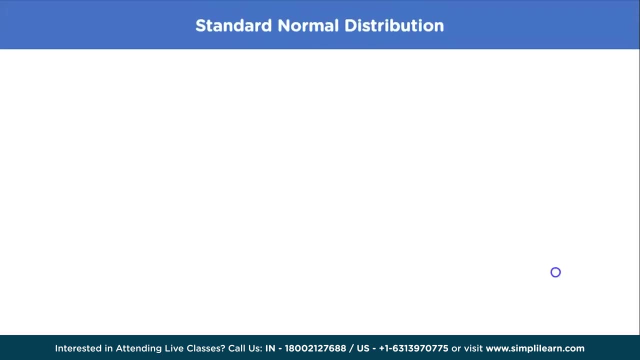 or from the mean. So when we plot these values, this value 147 will mean that a curve will have a width of 147 points around the mean. Now, what is the standard normal distribution? The standard normal distribution is a type of normal distribution that has a mean of 0. 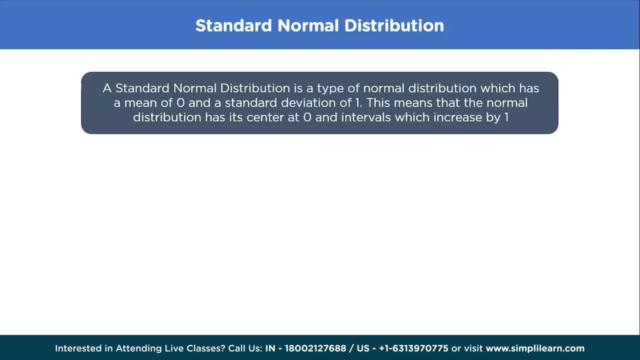 and a standard deviation of 1.. This means that the normal distribution has its center at 0 and it has intervals which increase by 1.. All normal distributions, like the standard normal distribution, are unimodal and symmetrically distributed with a bell-shaped curve. 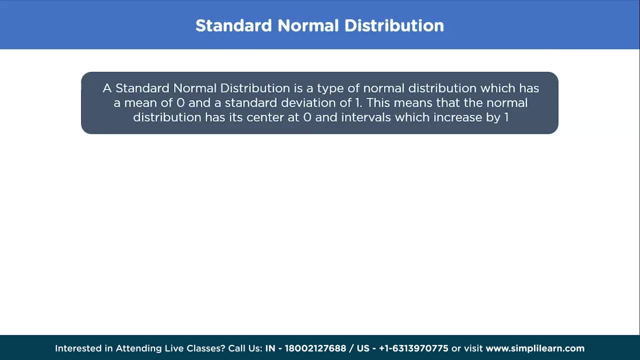 However, a normal distribution can take on any value as its mean and standard deviation. In the standard normal distribution, however, the mean and standard deviation are always fixed. When you standardize a normal distribution, the mean becomes 0 and the standard deviation becomes 1.. 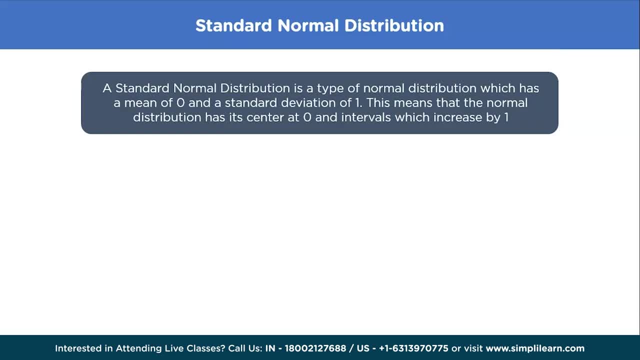 This allows you to easily calculate the probability of certain values occurring in your distribution or to compare datasets with different mean and standard deviations. The curve shows a standard normal distribution. As you can see again, the data is centered at 0.. This does not mean that the data 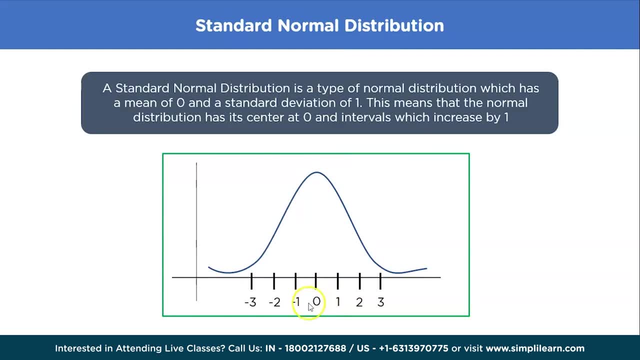 necessarily starts at 0.. This means that after standardizing, this point is where our mean will lie. In a standard normal distribution, the standard deviation is 1.. So all the data points will increase or decrease in steps of 1.. 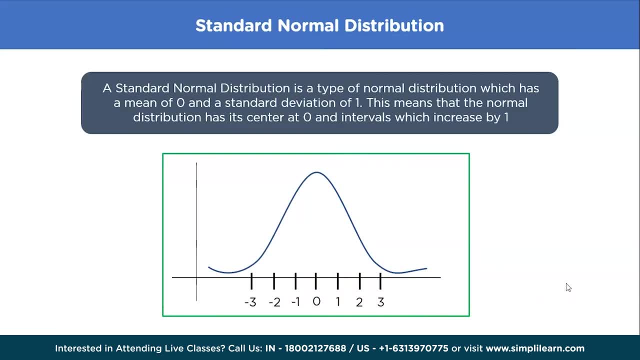 Let's better understand a standard, normal distribution with the help of an example Again, as you can see, the data is centered around 0, which is nothing but the mean. Let's again consider the weights of students in class 8.. The average weight here is around 50 kgs. 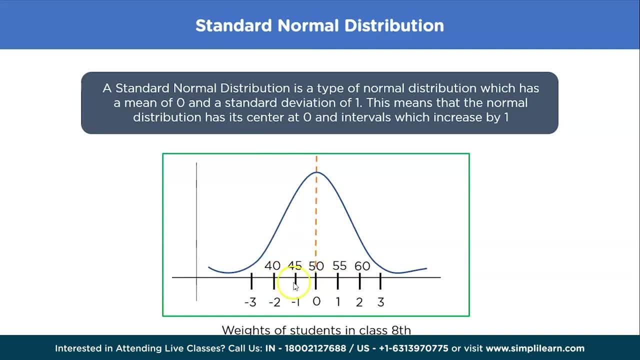 and the data increases and decreases in steps of 5. The data over here in this curve is evenly distributed along these steps. This is what a standard, normal distribution will look like. We already know that the mean of our data is 50 and because the data is increasing, 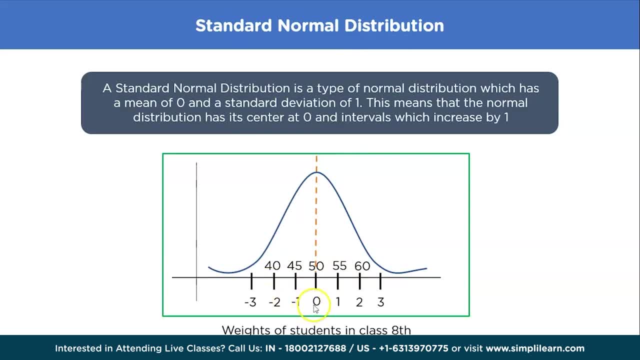 and decreasing in equal steps. we can just standardize it and take it to mean that the data is increasing and decreasing in steps of 1.. This is what a standard, normal distribution looks like, And when you have a data which looks like this: 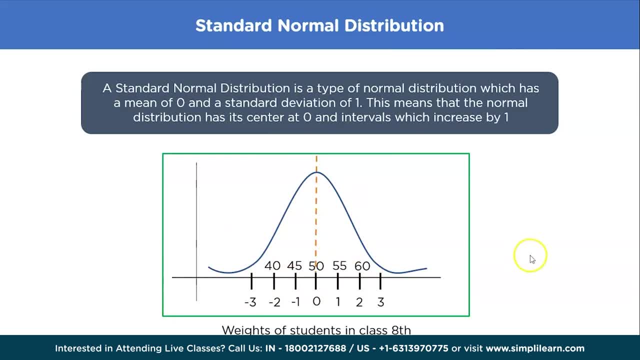 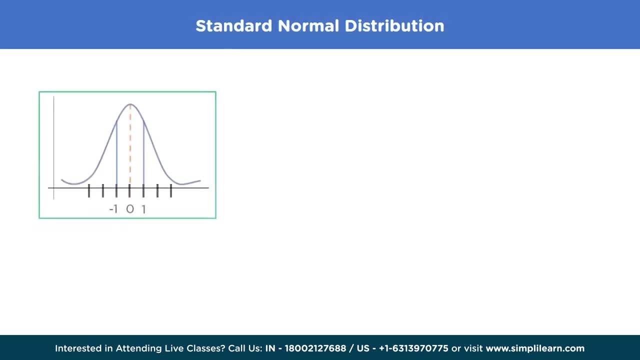 you can always standardize it and convert it into a standard normal distribution. Now, standard normal distribution has a couple of properties which makes calculation comparatively easy. The first one is that 68% of the values fall within the first standard deviation, which means that 68% of 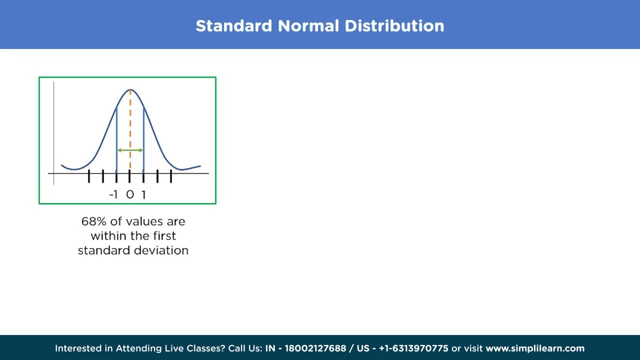 all data values on this curve will fall between the range of minus 1 to 1 in the first interval, ranging from minus 1 to 1.. The second property is that 95% of the rest of the values are within the second standard deviation. 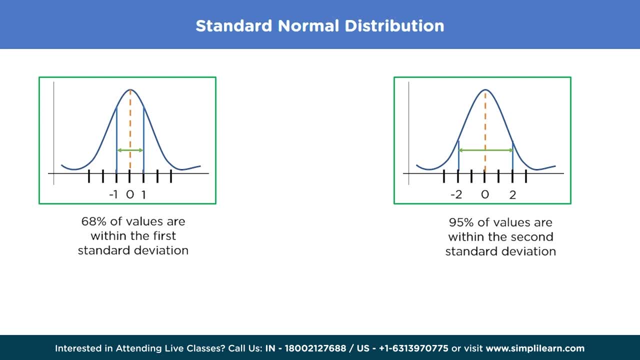 or from the second negative point to the second positive point. And finally, 99.7% of the values fall within the third standard deviation, or from the third negative point to the third positive point. This makes calculations on standard normal distribution fairly easy. 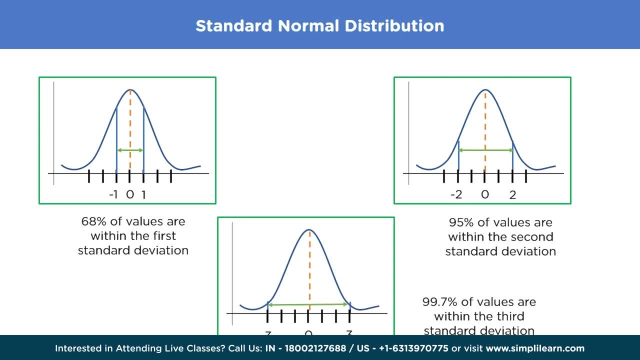 You can compare scores on different distributions with different means and standard deviations. You can normalize scores for statistical decision making using standard normal distribution. You can find the probability of observations in a distribution which fall above or below a given value And finally, you can find the probability. 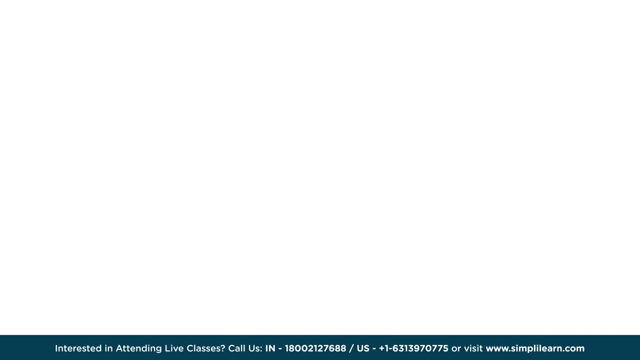 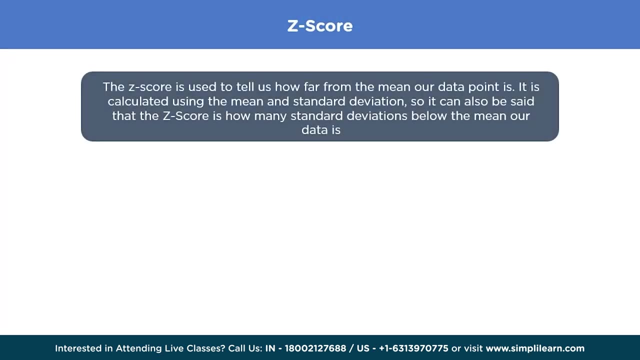 that a mean significantly differs from a population mean. Now let's take a look at z-score. So what is a z-score? A z-score is used to tell us how far from the mean our data point actually is. It is calculated. 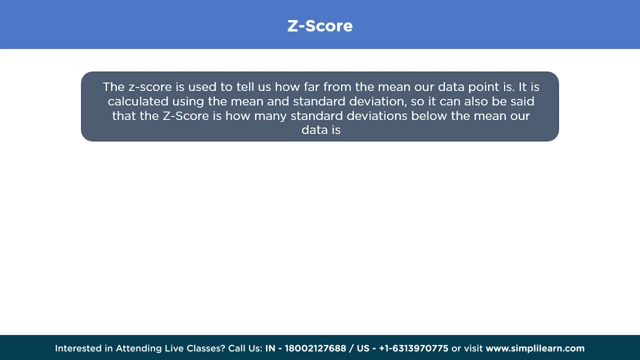 using the mean and standard deviation. so it can be said that the z-score is how many standard deviations below the mean our data is. Basically, by using the z-score, we can get an approximate location of where our data point lies on the graph with regards to the mean. 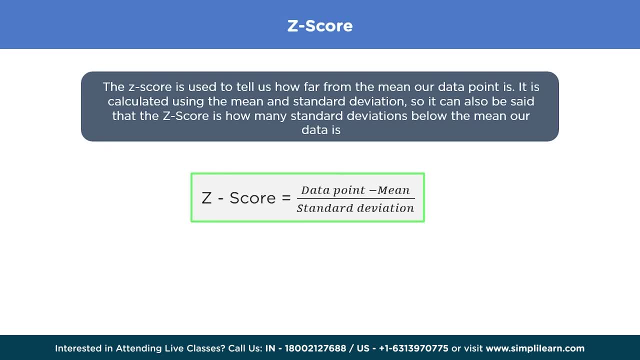 Now the z-score is given by subtracting the data point from the mean and dividing it by standard deviation. This can also be written as x minus mu divided by sigma. Now any normal distribution can be standardized by converting its values into z-scores. 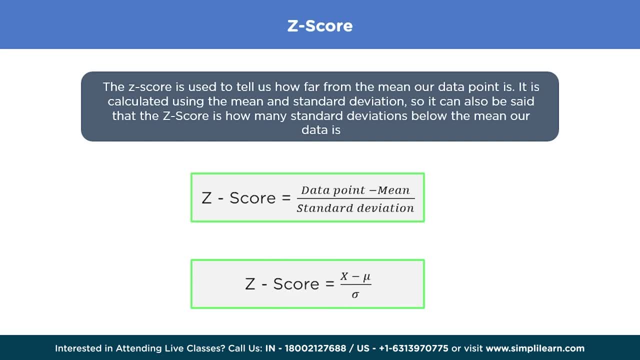 The z-score will tell you how many standard deviations from the mean each values lie. While data points are referred to as x in a normal distribution, they are called z or z-scores. in the z distribution. A z-score is a standard score that will tell you how many standard deviations. 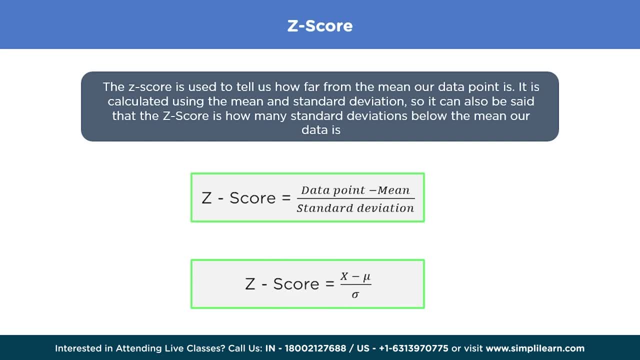 away from the mean, an individual point will lie. A positive z-score will mean that your x value is greater than the mean, and a negative z-score will mean that your x value is less than the mean. A z-score of 0 will mean that your x value. 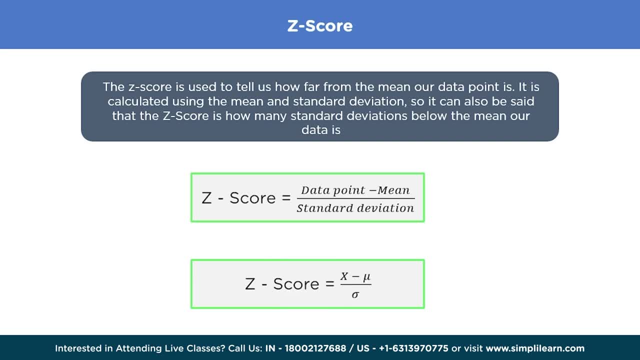 is equal to the mean. And again, to standardize a value from a normal distribution, all we have to do is convert it to a z-score by subtracting the mean from our individual value and dividing it by the standard deviation. Now let's see how we can find. 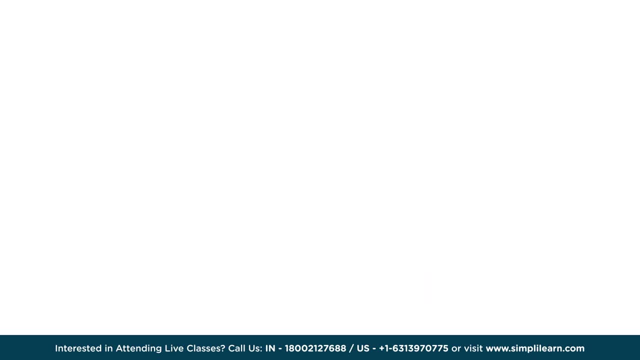 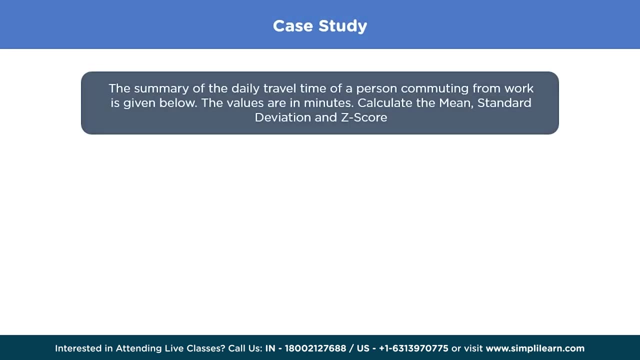 the z-score from data points. with the help of a solved example, Let's do a case study. In this case study, we'll be taking the summary of daily travel time of a person who's commuting to and from work. All these values are in minutes And using these, 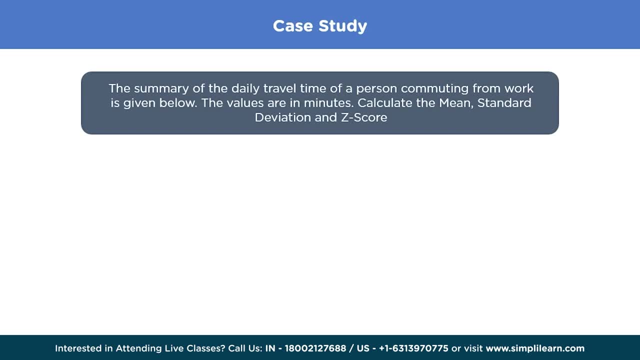 values. we have to calculate the mean, the standard deviation and the z-score. These values are as shown. As we can see, there are the 13 values in total. Let's start by finding the mean. The mean is the average and it can be. 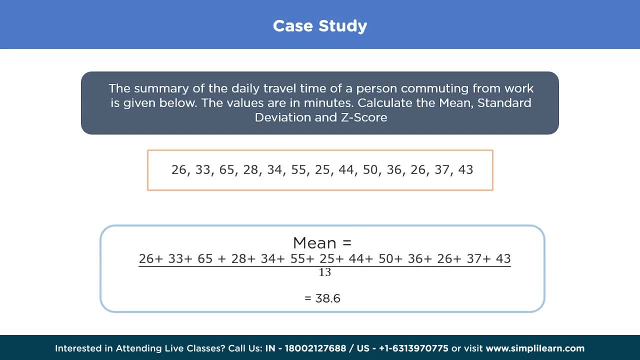 gotten by adding all of these values and dividing it by the total number of values. This gives us a value of 38.6.. The mean tells us the average of all our data points, which means, on an average, he travels for 38.6 minutes to reach work. 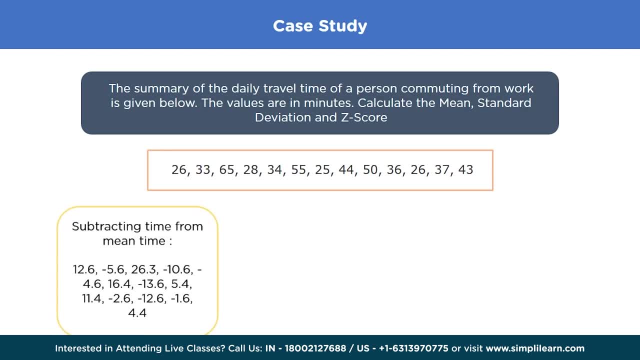 Next, let's subtract the individual values from our mean and calculate the variance and standard deviation. The values on the left give us the values that we get after subtracting it from the mean, and the variance can be calculated by squaring all of these values, adding up. 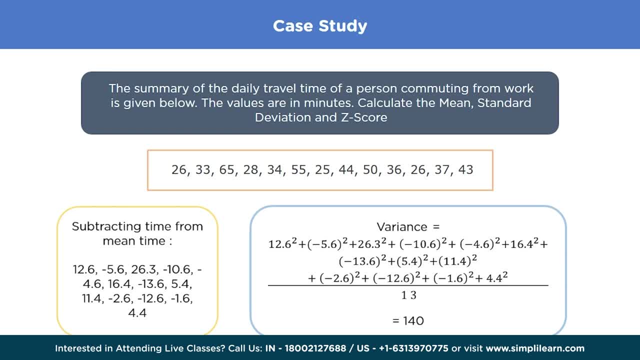 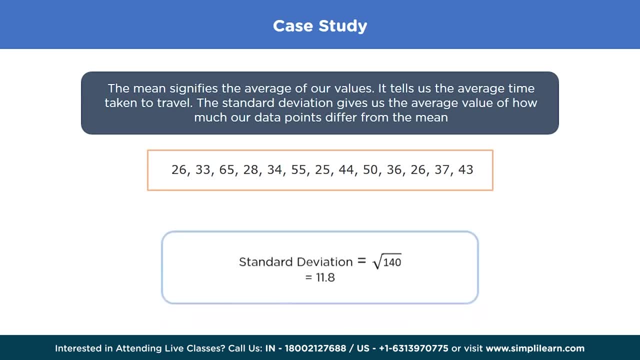 all of the squared values and dividing it by the total number of values, At the end of the day we get a variance of 140.. To calculate the standard deviation, all we have to do is take a square root of the variance, which gives us a value. 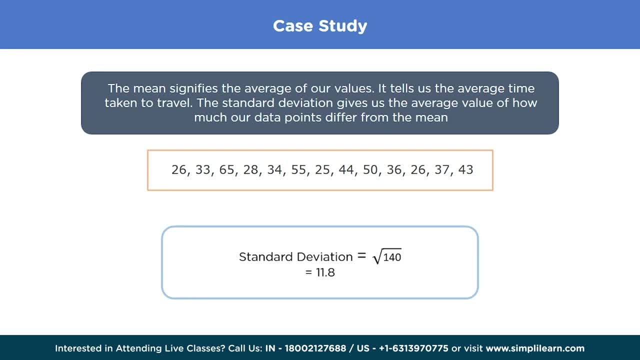 of 11.8.. Now the mean signifies the average of our values, and we already know this. It gives us the average time which is taken to travel, but the standard deviation will tell us the average value of how much our data points differ from the mean. 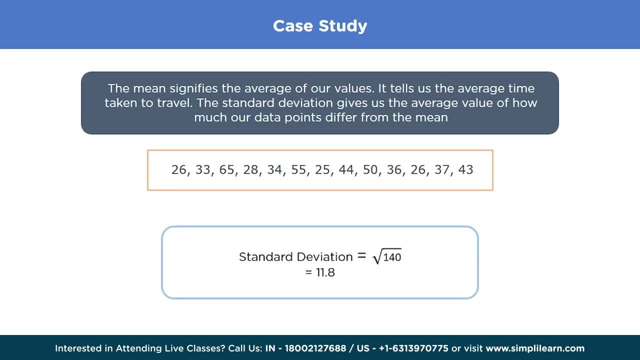 It tells us the deviation within our own data and it tells us how far away, on an average, a point is from the mean. Now the value that we get is 11.8,, which means that, on an average, a single data. 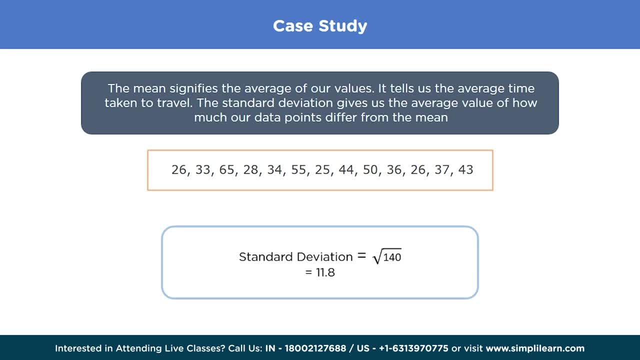 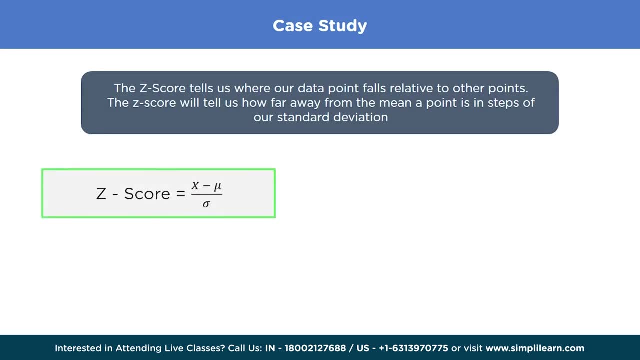 point is around 11.8 data points away from the mean. Now let's calculate the z-score. The z-score is given by subtracting individual data points from the mean and dividing it by the standard deviation. We know that we have a standard deviation of. 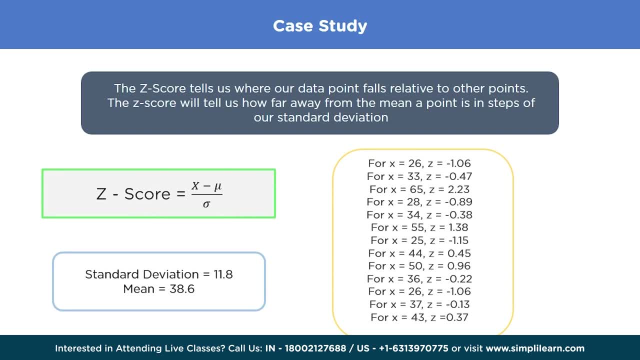 11.8, and a mean of 38.6.. Using these values, we can calculate the z-scores for individual x values. Now we know that a negative z-score means that our x value is lower than our mean, But what does the number 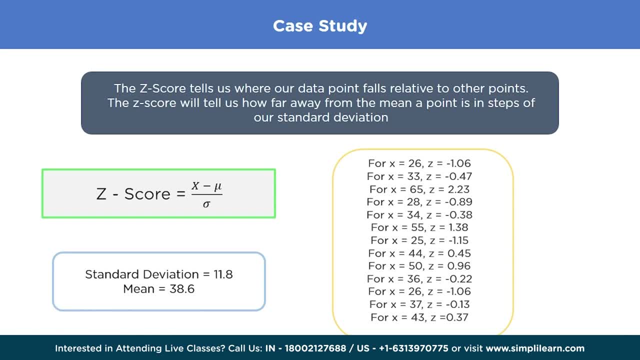 1.06 mean. This means that the z-score for 26 is 1.06 standard deviations away from the mean. The negative symbol here means that our x value is less than the mean. And by how? less 1.06 times the standard. 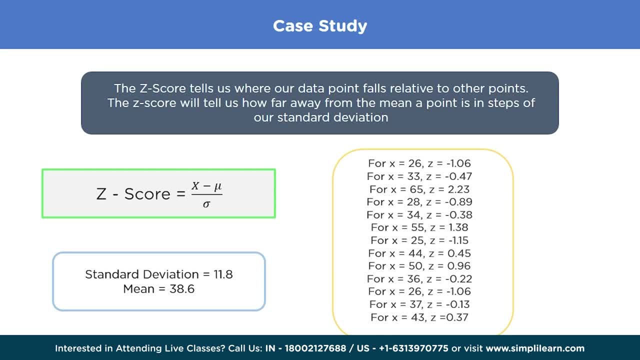 deviation. Now we know that the negative value of a z-score means that our x value is less than our mean. But what does the number 1.06 mean? This means that the z-score is 1.06 times the standard deviation less than the mean. 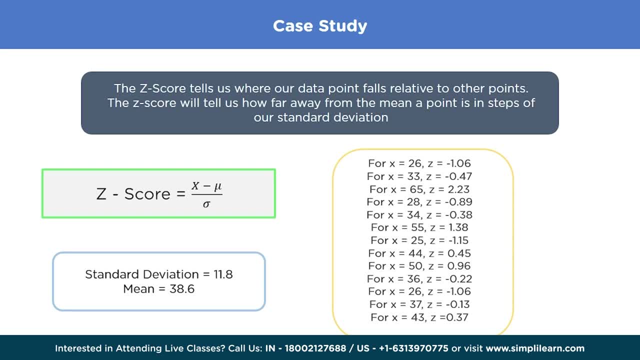 The same thing can be said for the z-score of 33.. It is 0.47 times the standard deviation, less than the mean. The z-score of 65 is 2.23 times the standard deviation, more than the mean. That means it has to be added. 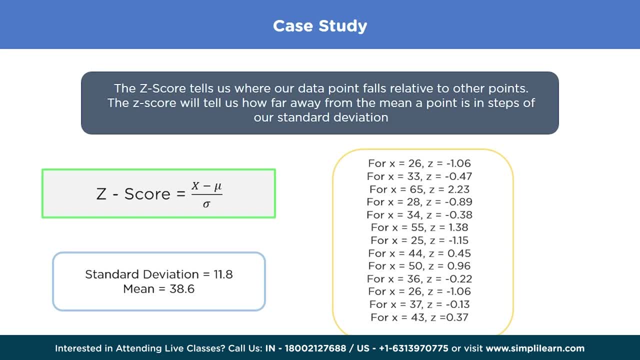 to the mean. The reason that we know it's more than the mean is because this has a positive value. So this means that, using z-scores, we can know where our data points fall relative to other points on the graph. The z-score will tell us how far 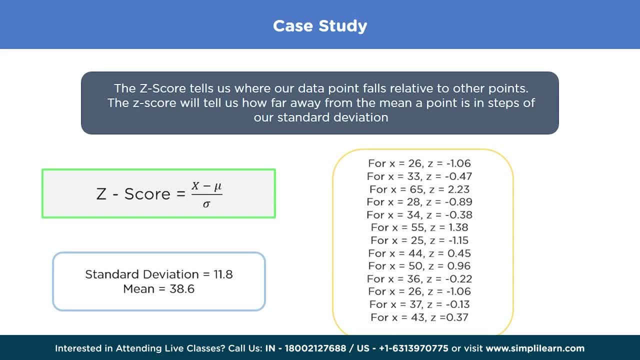 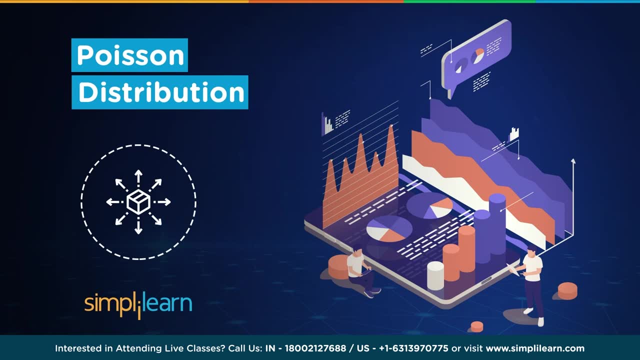 away from the mean. a point is in steps of our standard deviation. Data science has grown in popularity as an interdisciplinary field. It extracts facts and insights from structured, semi-structured and unstructured datasets using scientific approaches, methods, algorithms and tools. 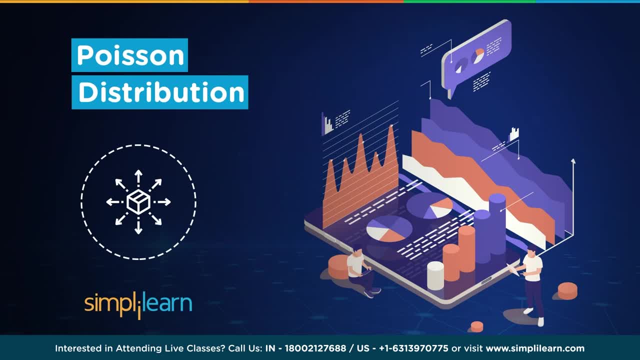 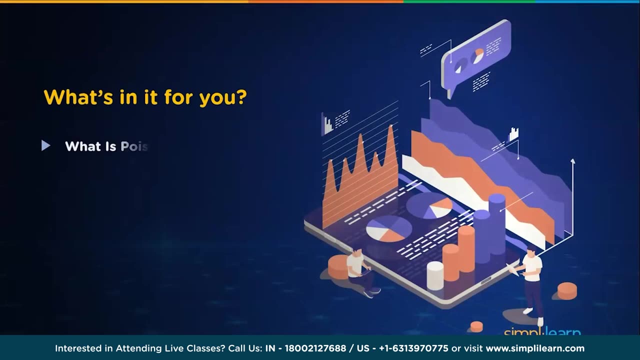 The probability distribution isn't important when performing data analysis and preparing a dataset for model training. In today's session, we'll discuss one such probability distribution, that is, poison distribution. So let's see what's in it for you. We'll start this session by discussing 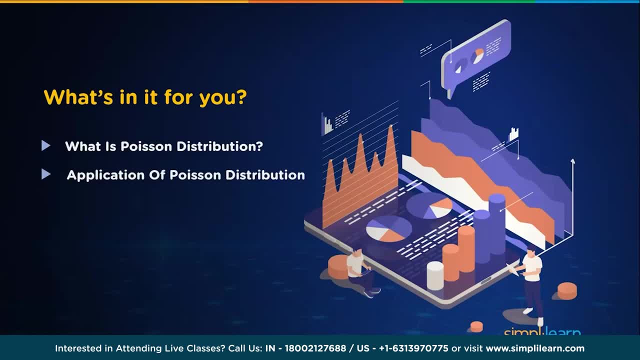 what is poison distribution? Then we'll move on to the applications of poison distribution and we'll work on some examples to understand it. Finally, we'll have a question for you so that you can write your answers in the comment section. 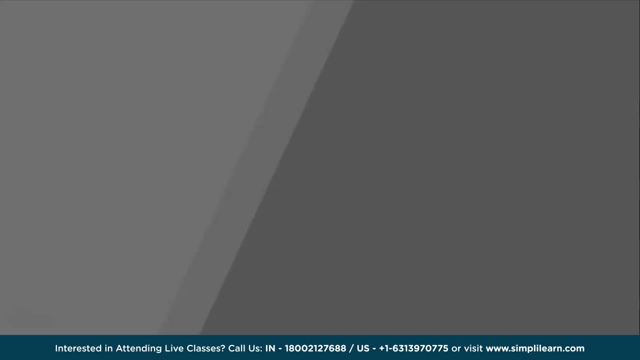 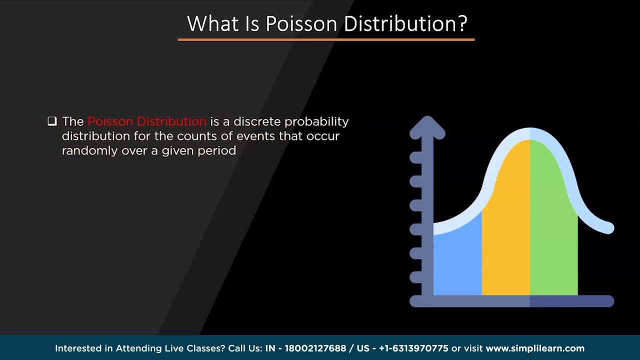 So let's begin. A poison distribution is a probability distribution used in statistics to show how many times an event is likely to happen over a given period of time. To put it another way, it's a count distribution. Poison distributions are frequently used to comprehend independent events. 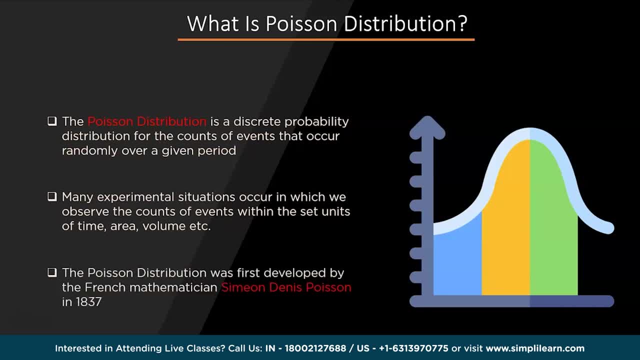 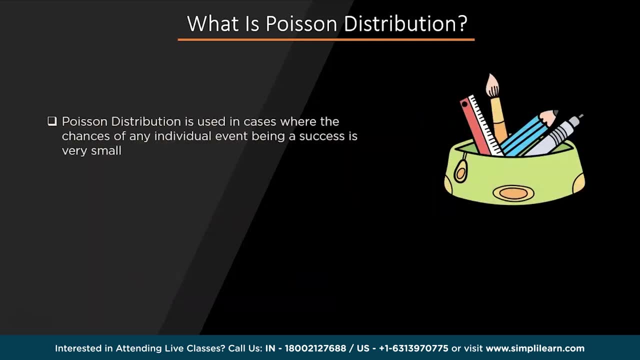 at a constant rate over a given interval of time. The poison distribution was developed by French mathematician Simon Dennis Poisson in 1837.. A poison distribution is used in cases where the chances of any individual event being a success is very small. The number of defective pencils per box. 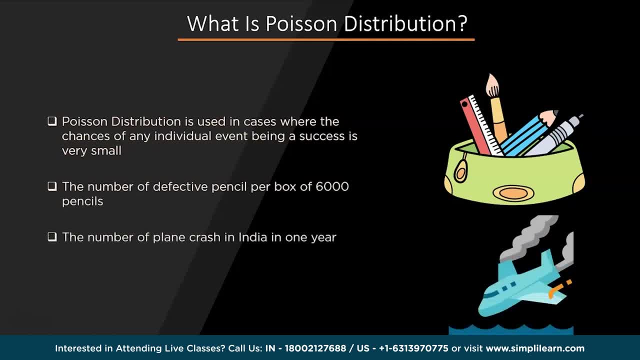 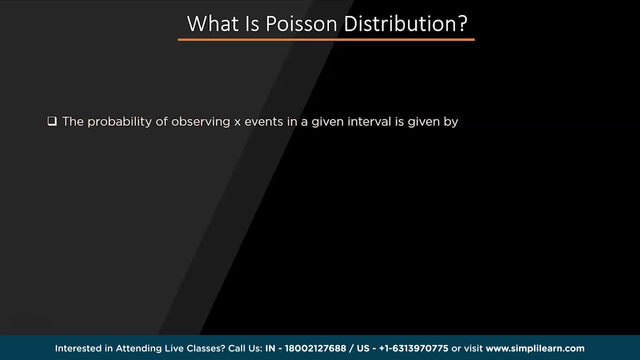 of a 6000 pencil, the number of plane crashes in India in one year, or the number of printing mistakes in each page of a book- All of these examples can have use of poison distribution. The poison distribution can be used to calculate how likely it is that something will happen. 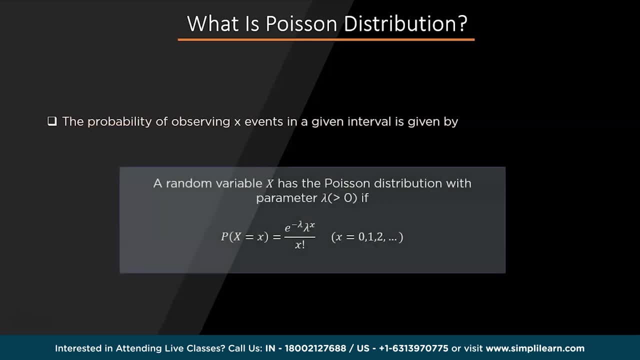 x number of times. A random variable x has a poison distribution with parameter lambda and the formula for that is: e to the power minus lambda into lambda to the power x divided by x factorial, Where x can be the number of times the event is happening. 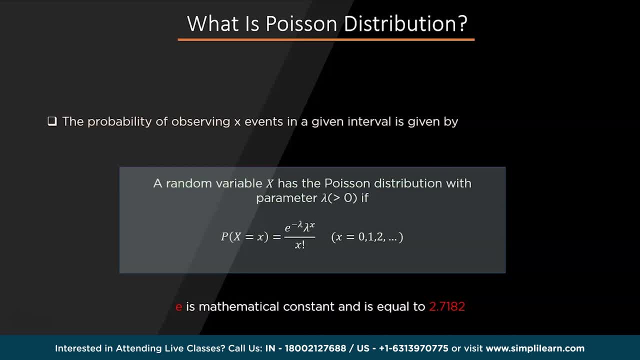 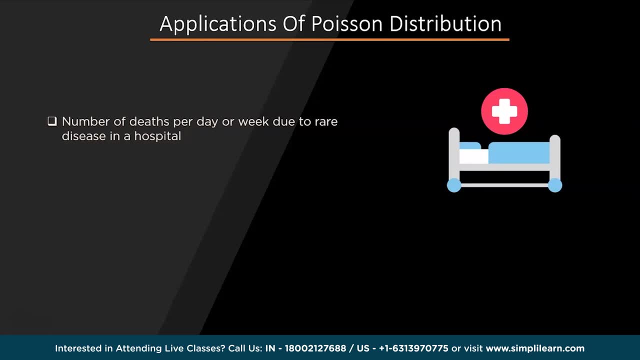 The value of e is taken as 2.7182.. Let's discuss some application of poison distribution. If you want to calculate the number of deaths per day or week due to rare disease in a hospital, you can use the poison distribution In a similar manner. 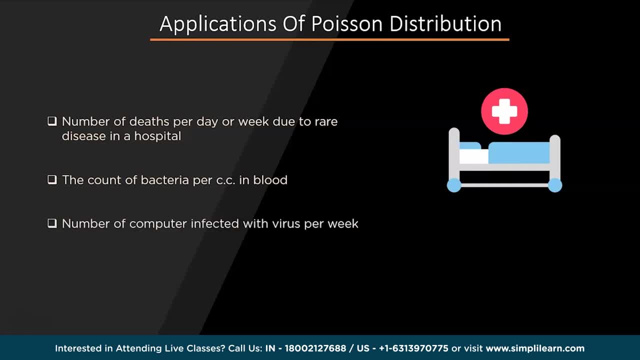 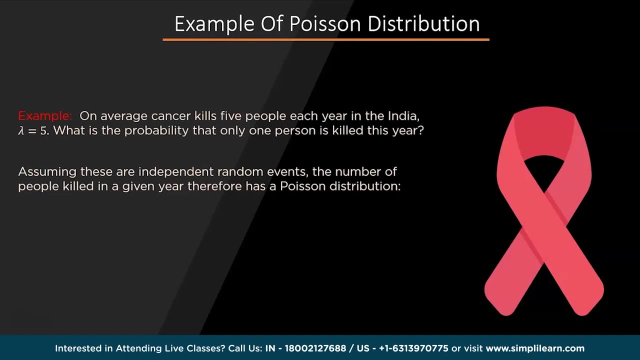 the count of bacteria per cc in blood or the number of computers infected with virus per week. The number of mishandled baggage per 1000 passengers can also have an application for poison distribution. Let's discuss one example to see how we can calculate the poison distribution. 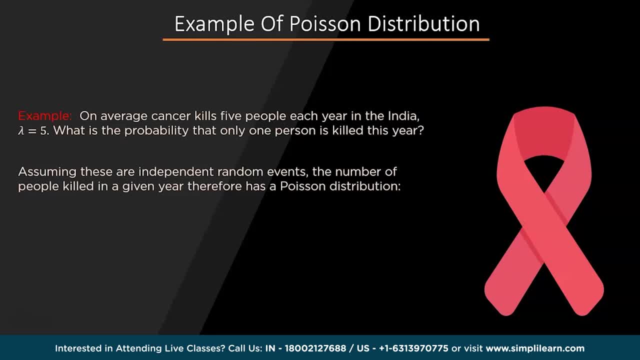 Suppose, on an average a cancer kills 5 people each year in India. What is the probability that one person is killed this year? We'll assume all these events are independent, random events. So by the formula we have, x is equal to 1, because we have to calculate the probability of one. 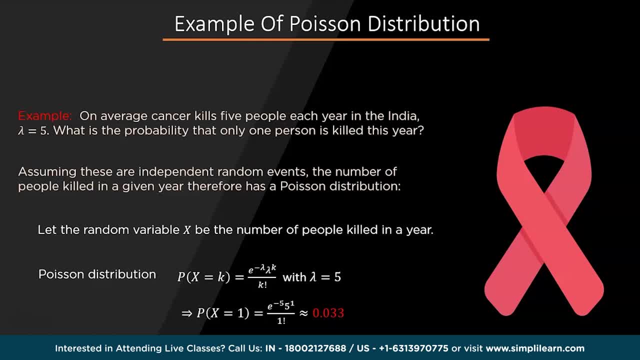 person that is killed this year. So p x equal to 1 will be equal to e, to the power minus 5 into 5, to the power 1 divided by 1 factorial, Which will come out to be 0.033, which will be near to 3.3%. 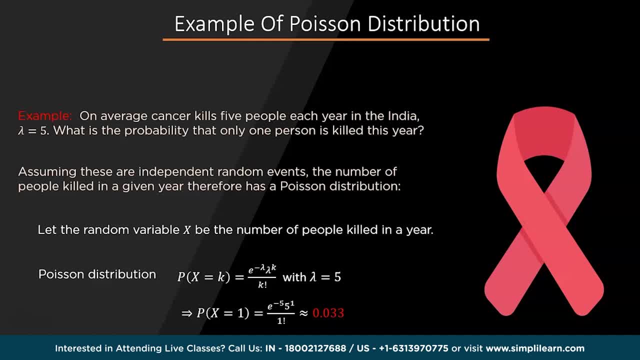 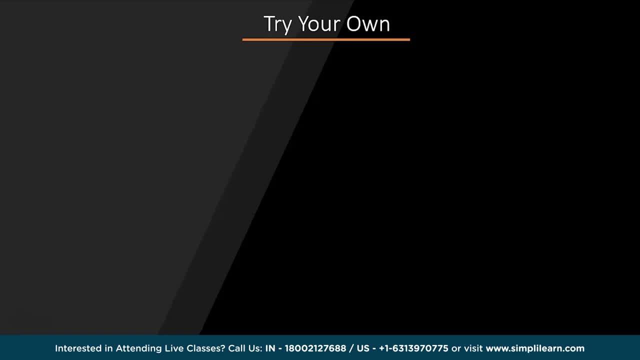 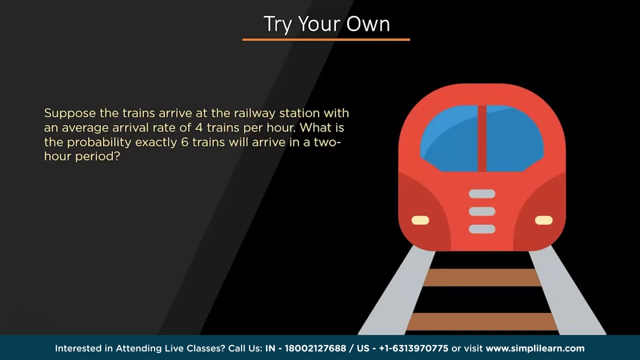 So the probability that only one person is killed this year due to cancer is 3.3%. Now we have one question for you. Do try to answer in the comment section. Suppose the trains arrive at a railway station with an average arrival rate of 4 trains per hour. 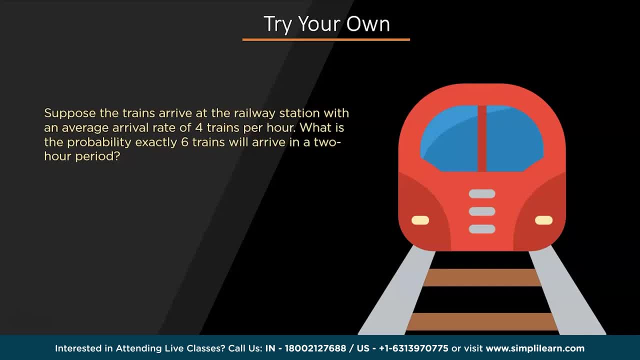 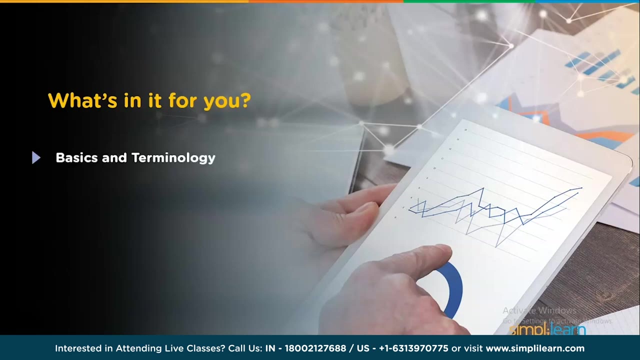 What is the probability? exactly 6 trains will arrive in a 2 hour period, And here are your options. Please do let us know your answers in the comment section. Let's discuss what's in it for you. We'll start this tutorial by discussing the important terms. 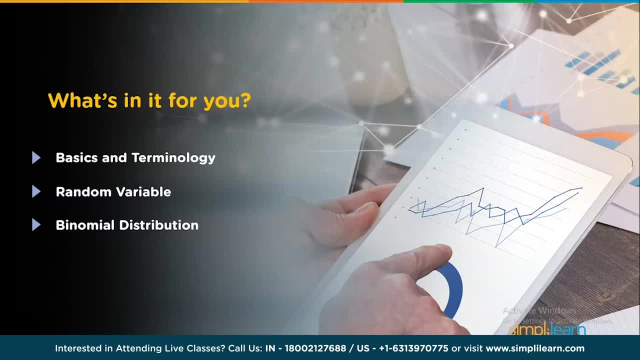 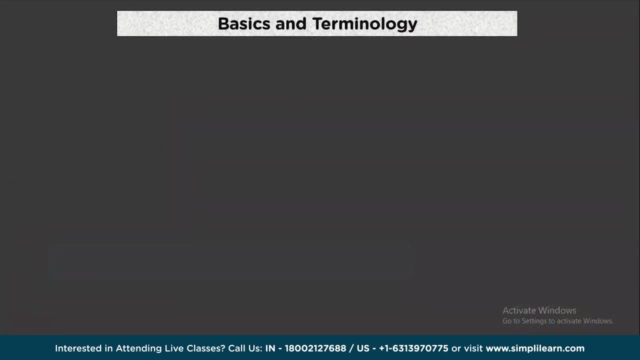 that you should know. Then we'll move on to discuss binomial distribution and the formula for calculating the binomial coefficient. Then we'll work on an example to get the clear understanding of the topic. So let's get started. Basics and Terminology. 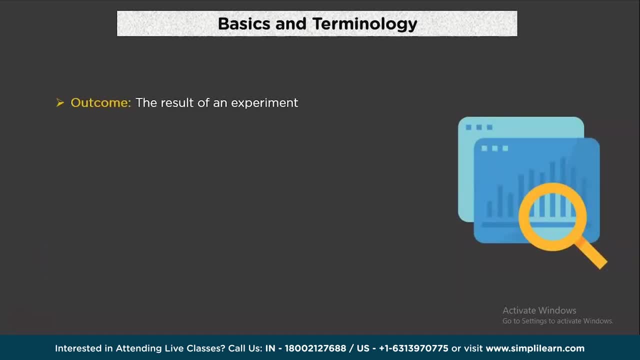 The first one is Outcome: Whenever we do an experiment like flipping a coin or rolling a dice, we get an outcome. For example, if we flip a coin, we get an outcome of heads or tails, And if we roll a die, we get an outcome of. 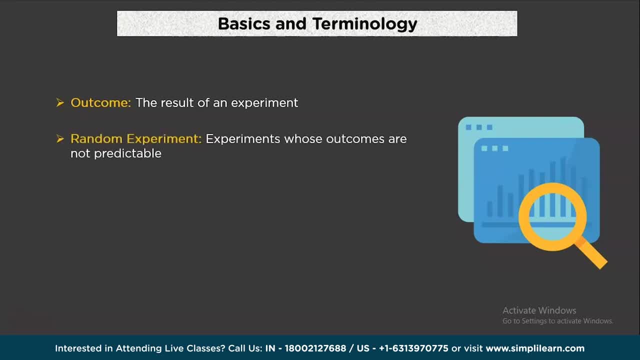 1, 2,, 3,, 4, 5 or 6.. Random Experiment: A random experiment is any well-defined procedure that produces an observable outcome that cannot be perfectly predicted in advance. A random experiment must be well-defined to eliminate any 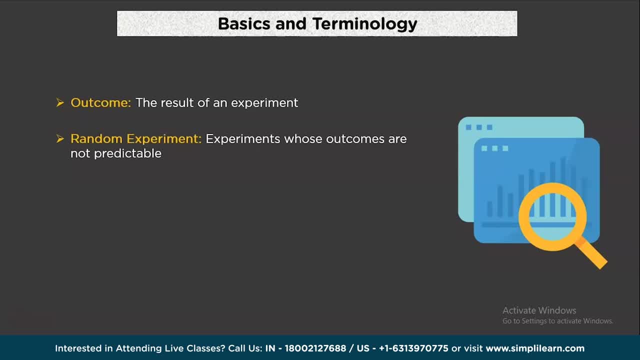 vagueness or surprise. It must produce a definite, observable outcome so that you know what happened after the random experiment is run. Random Events. Consider a simple example. Let us say that we toss a coin up in the air. What can happen when it gets back? 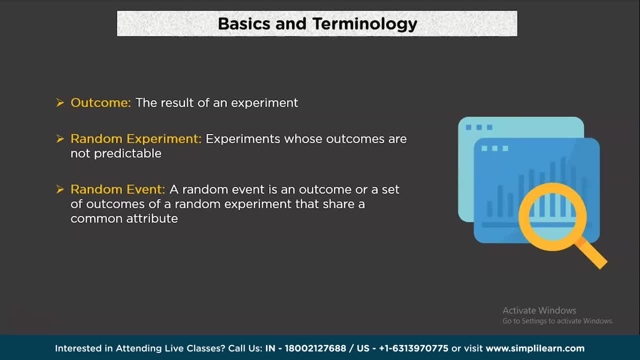 It either gives a head or a tail. These two are known as random events. A random event is an event. Thus, the event is the outcome of some phenomenon. The last one is Sample Space. A sample space is a collection or a set of possible outcomes. 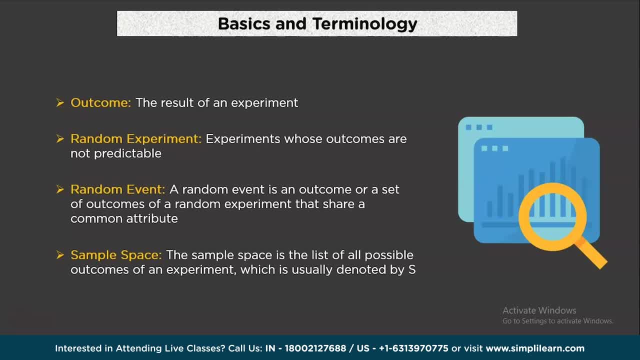 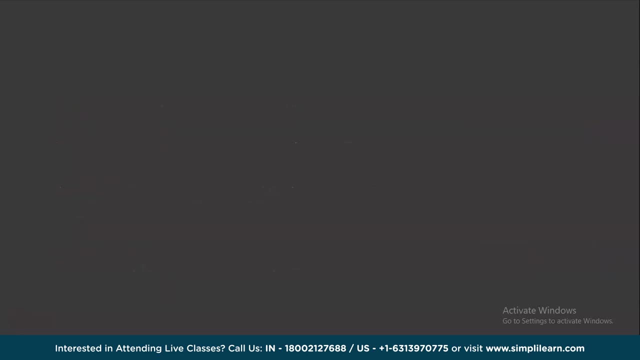 of a random experiment. The sample space is represented using the symbol S. The subset of all possible outcomes of an experiment is called events, and a sample space may contain a finite number of outcomes. Then it is known as a discrete or finite sample spaces. 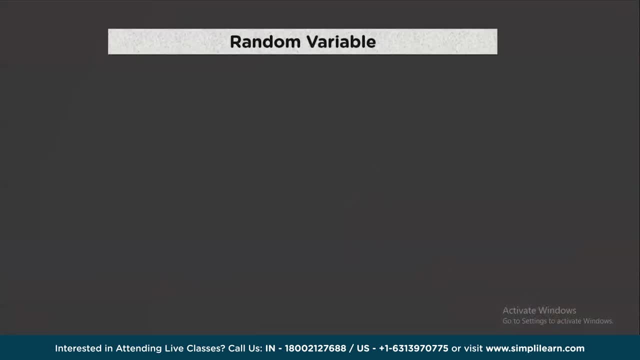 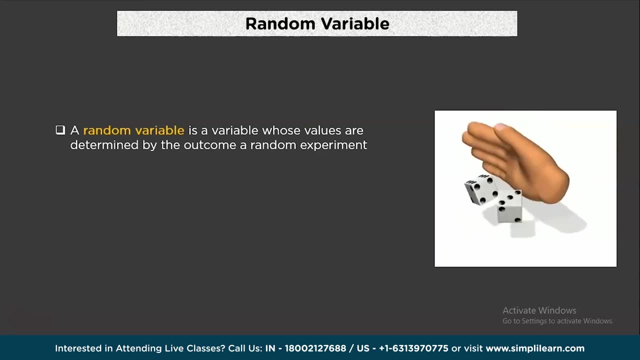 Now let's discuss what is random variable. A random variable is a numerical description of the outcome of a statistical experiment. A random variable that may assume only a finite number of values is said to be discrete. One that may assume any value in some interval on the real. 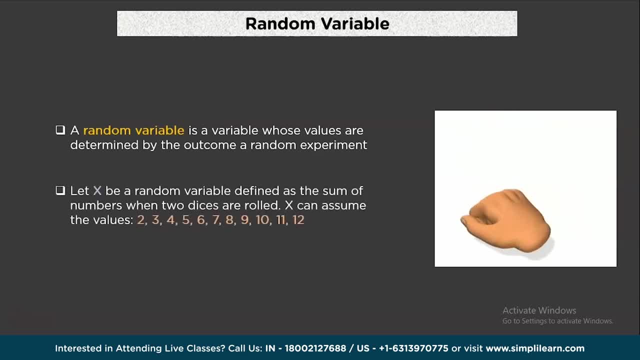 number line is said to be continuous. Let's see an example. Let X be a random variable defined as the sum of numbers when two dices are rolled. X can assume the values 2,, 3,, 4,, 5,, 6,, 7,, 8,, 9,, 10,, 11 and 12.. 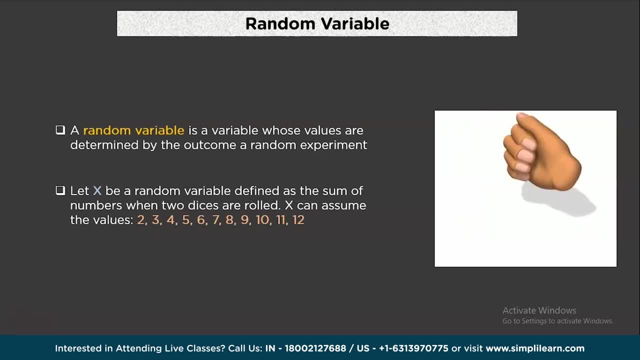 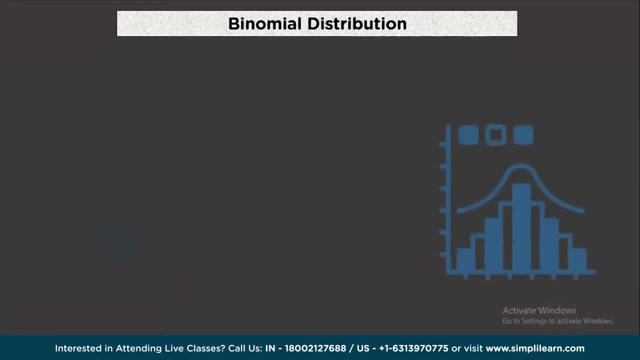 Notice there is no 1 here, because the sum on the two dice can never be 1.. Now that we know the basics, let's move on to binomial distribution. The binomial distribution is used when there are exactly two mutually exclusive outcomes of a trial. 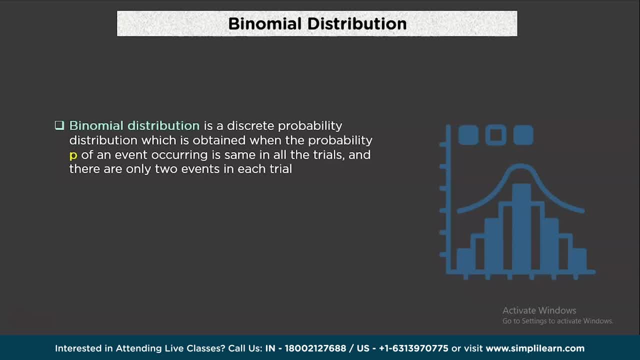 These outcomes are appropriately labeled: success and failure. The binomial distribution is used to obtain the probability of observing X successes in n number of trials, with the probability of success on a single trial denoted by p. The binomial distribution assumes that p is fixed. 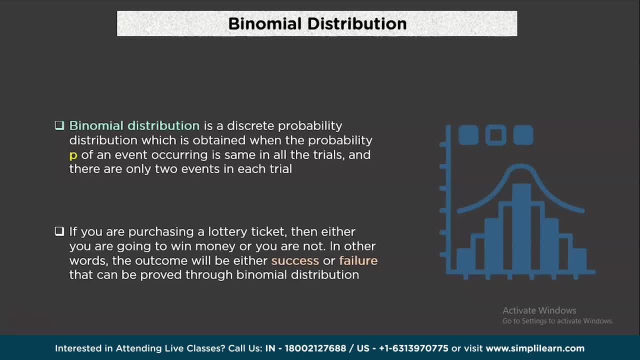 for all the trials. Here is a real-life example of a binomial distribution. Suppose you purchase a lottery ticket, Then either you are going to win the lottery or not. In other words, the outcome will be either success or failure. that can be. 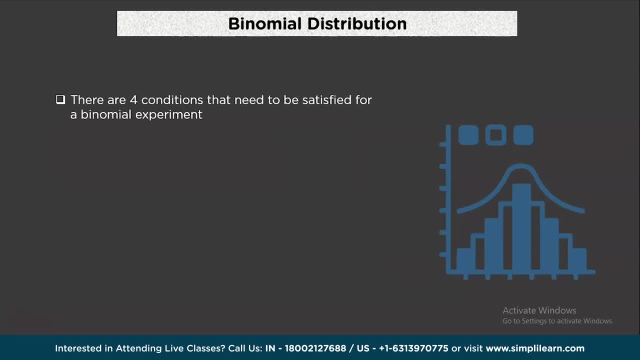 proved through binomial distribution. There are four important conditions that needs to be fulfilled for an experiment to be a binomial experiment. The first one is there should be a fixed number of n trials carried out. The outcome of a given trial is only two, that is. 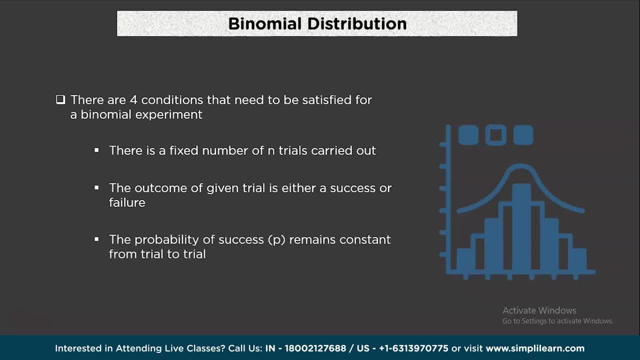 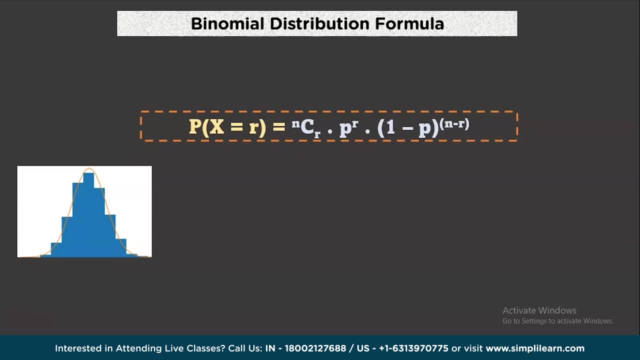 either a success or a failure. The probability of success remains constant from trial to trial. It does not change from one trial to another And the trials are independent. The outcome of a trial is not affected by the outcome of any other trial. To calculate the binomial coefficient: 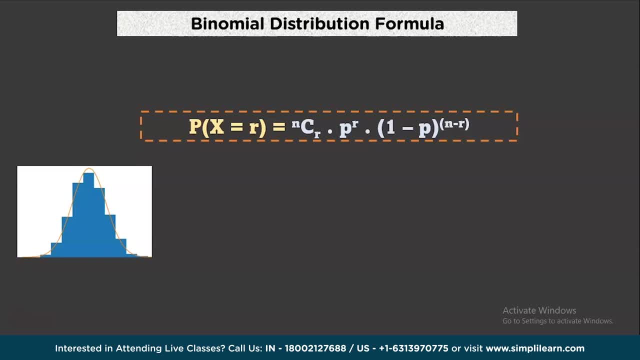 we use the formula which is nCr into p to the power r, into 1 minus p to the power n minus r, where r is the number of success in n number of trials and p is the probability of success. 1 minus p denotes the probability. 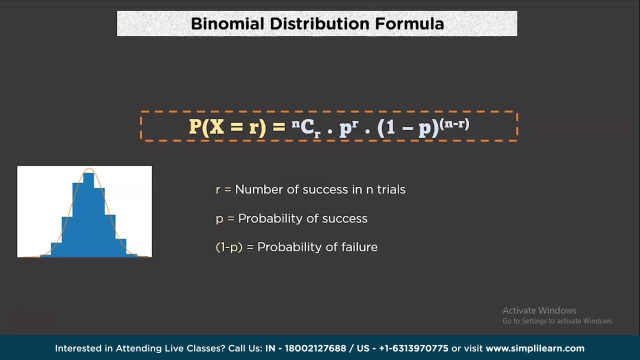 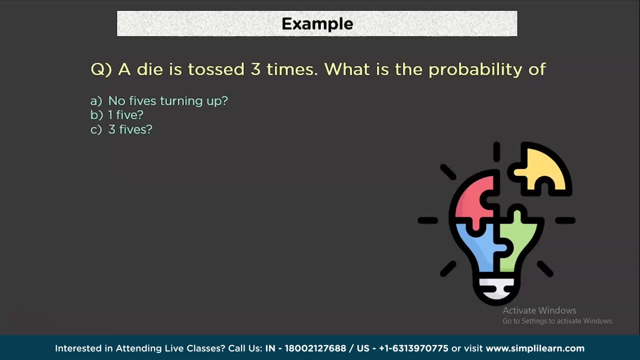 of a failure. Now let's use this formula to solve an example. Suppose a die is tossed three times. What is the probability of 1 by 5 turning up, 1 by 5 and 3 by 5 turning up? 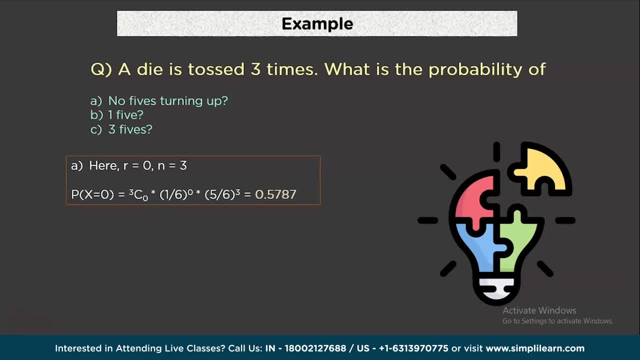 To calculate the no 5 turning up here: r is equal to 0 and n is equal to 3.. Substituting the value in the formula we have, 3, 3, 0 into 1 by 6 to the power, 0 into. 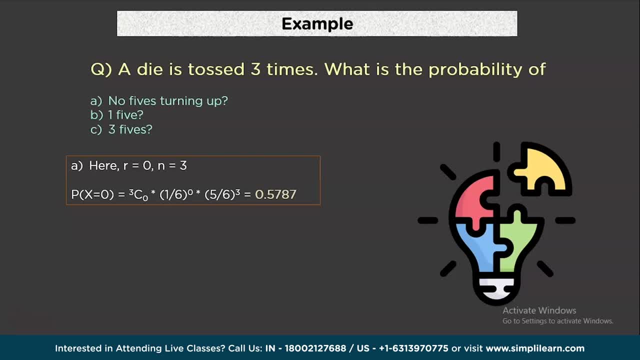 5 by 6 to the power 3, where 1 by 6 is the probability of success and 5 by 6 is the probability of failure. Calculating this equation, we will get the value to be 0.5787.. 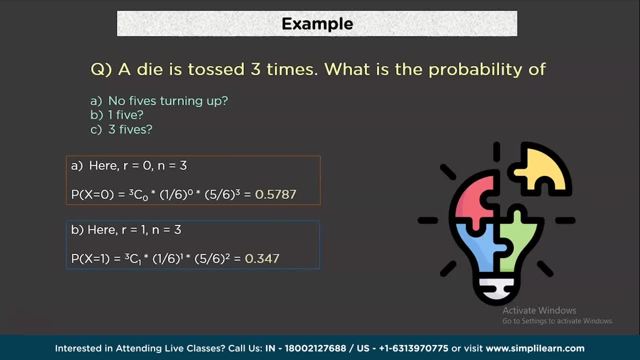 In a similar manner to calculate the probability of 1 by 5 turning up. we will replace r with 1 and n will be 3.. So p will be equal to 3, c 1 into 1 by 6 to the power 1. 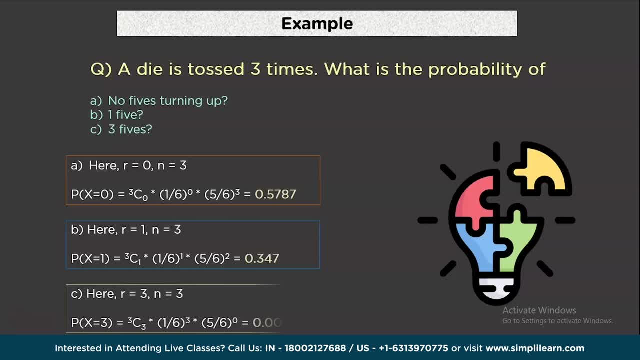 into 5 by 6 to the power 2, which will come out to be 0.347. And for 3 by 5 turning up, we will substitute r equal to 3 and the formula will remain the same and we will get the value to be. 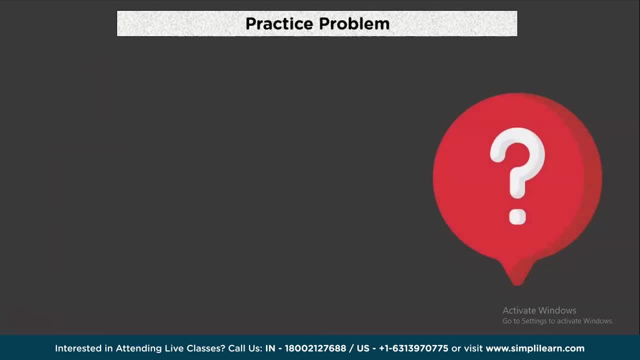 0.0046.. Now that we are done with the concepts of animal probability distribution, here is a problem for you to solve. Post your answers in the comment section and let us know. We will start this tutorial by discussing what is empirical rule. 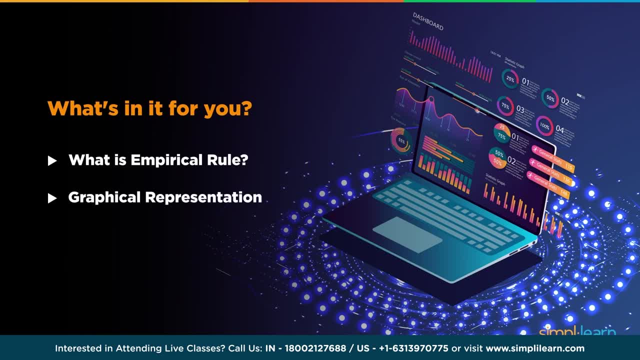 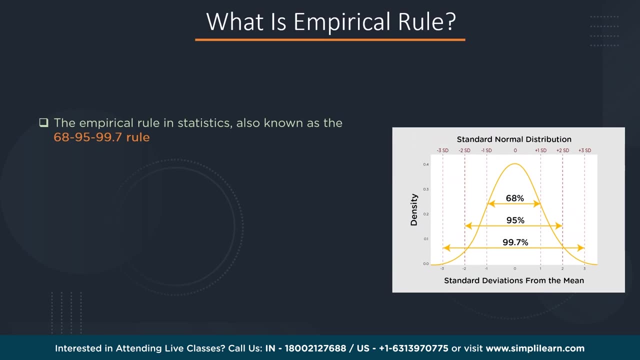 and we will see the graphical representation of the empirical rule. Then we will work on an example to understand the empirical rule more comprehensively. So let's move ahead. What is empirical rule? The empirical rule. it is also known as the 68-95-99.7 rule. 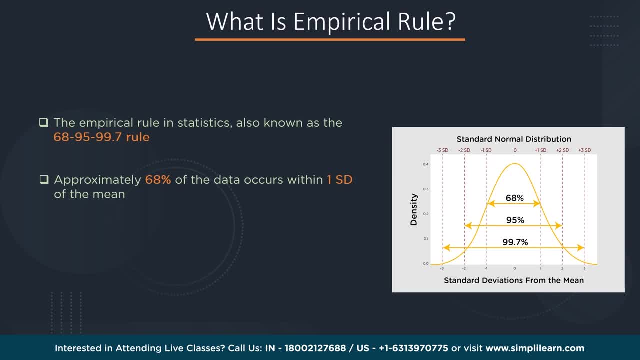 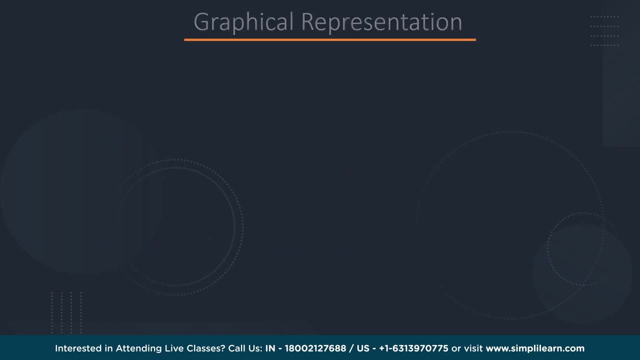 states that 68% of the data occurs within the one standard deviation of the mean and 95% of the data occurs within the two standard deviation of the mean. Similarly, the three standard deviations covers 99.7% of the total data. 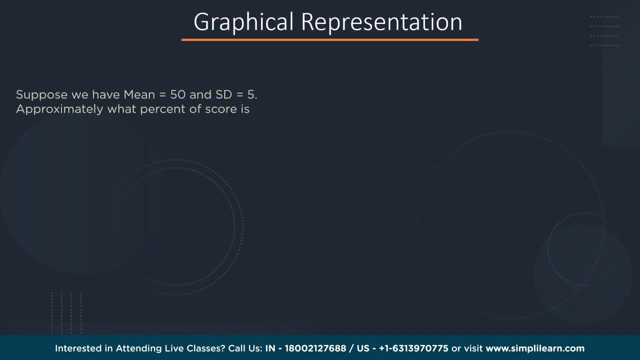 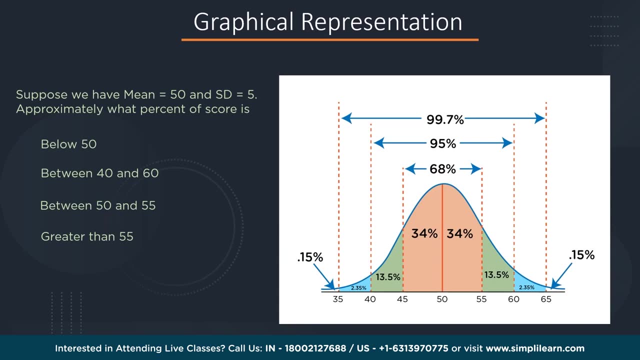 Suppose we have a bell-shaped distribution with mean value 50 and standard deviation 5.. We want to answer the following questions. Since the mean is 50, one standard deviation to the right will be 55,. two standard deviation will be 60,. 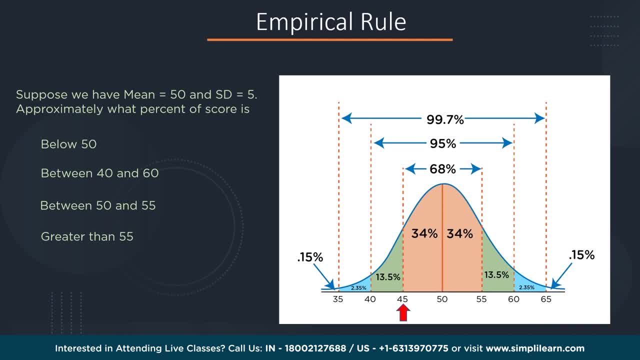 and three standard deviation will be 65.. In a similar manner, one standard deviation from the left will be 45,, two standard deviation will be 40, and three standard deviation will be 35.. Since 50 represents the mean value, all the values below 50. 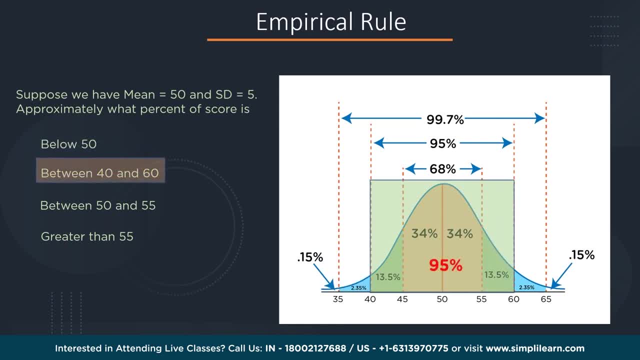 will cover the 50% of the total data. The value 40 and 60 are within two standard deviations of the mean, which covers 95% of the total data. The value 50 and 55 represent exactly 34% of the total data. 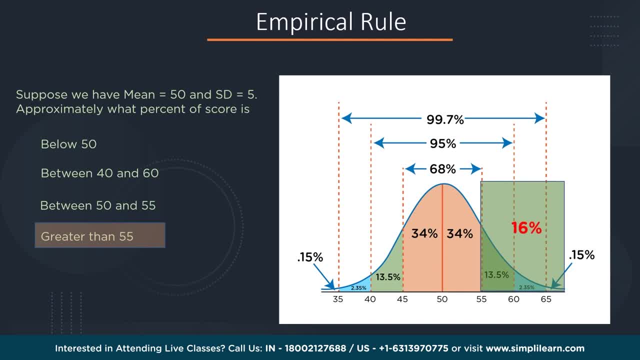 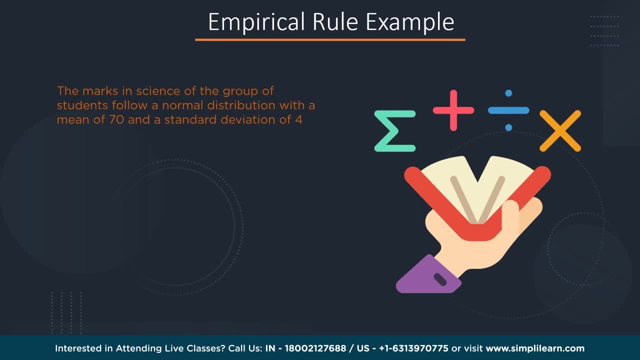 and greater than 55 represents 16% of the total data. Consider the following example: The marks and signs of a group of students follow a normal distribution with a mean value of 70 and standard deviation of 4.. We want to find a range around the mean. 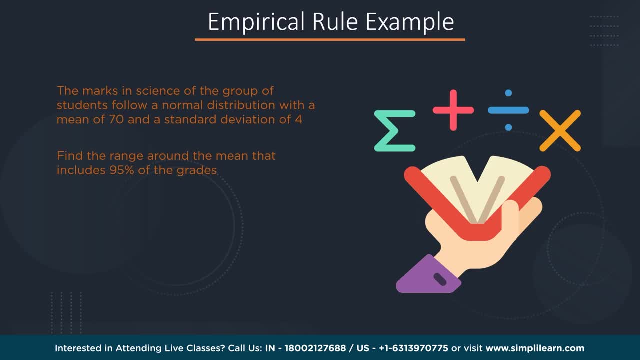 that includes 95% of the grades. So let's first note down the important data. We are given a mean value of 70 and standard deviation of 4.. In this slide we know that the 95% of the data means the two standard deviations. 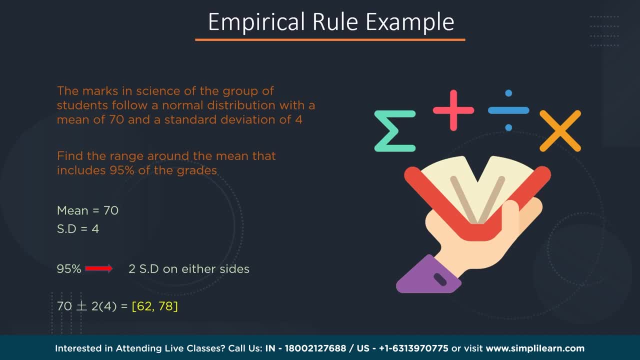 on either side of the mean. We will add and subtract the two standard deviations from 70 on either side, which will give us the value of 62 and 78 respectively. This means that 95% of the total grades lies between the marks 62 and 78.. 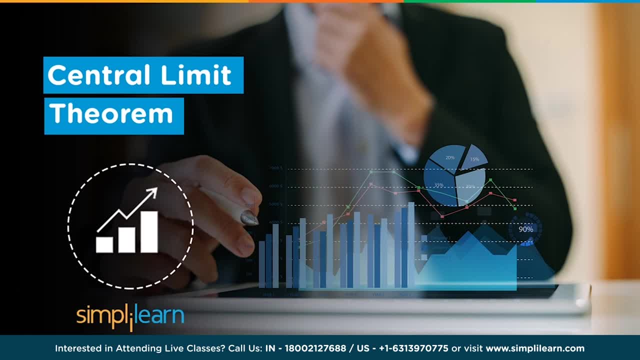 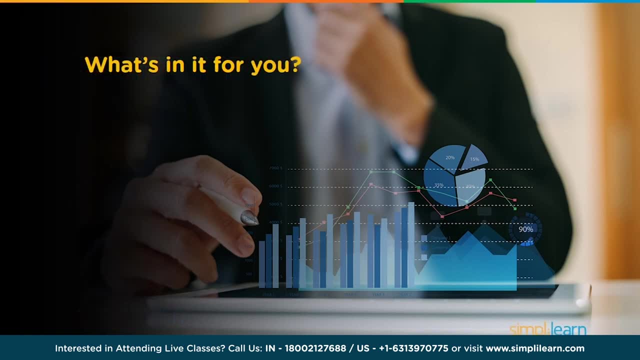 And yet it is often confused by a spying data scientist. Yes, I am talking about the central limit theorem. So in this video we will discuss all there is to know about the central limit theorem. So let's start by discussing the agenda for today. 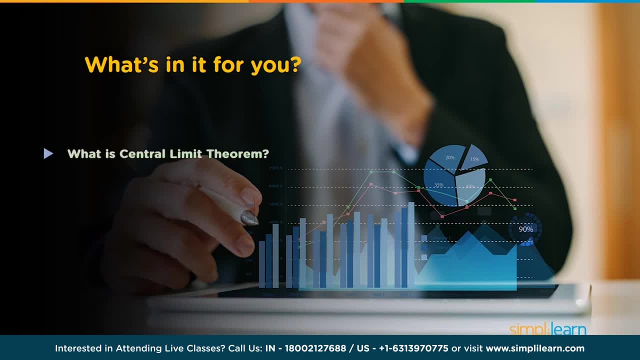 We will start with the definition of central limit theorem and then discuss the mean and standard deviation associated with it. Then we will take a real-life example to understand where you can use the central limit theorem. Then we will discuss some assumptions that are taken for effective use of central limit theorem. 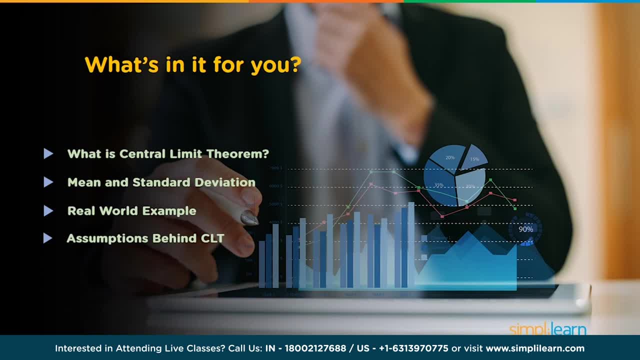 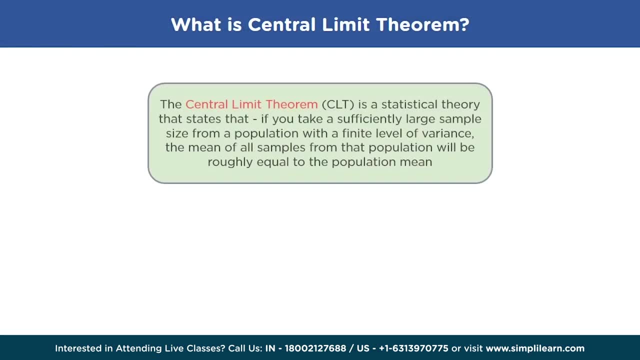 We will end this tutorial with a demonstration of the central limit theorem in Python. So without further ado, let's get started. So what is the central limit theorem? The central limit theorem is a statistical concept that states that the sample means of the distribution of a random variable. 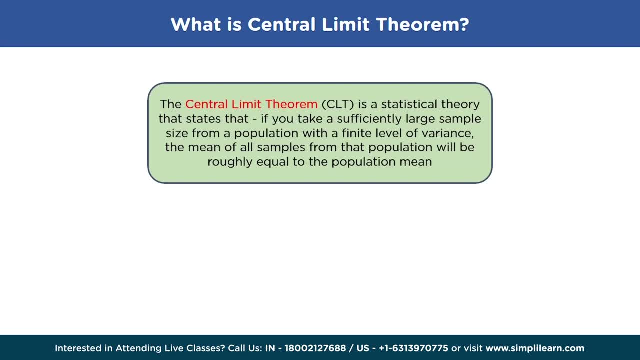 will approach to a normal distribution if the sample sizes are large, respective of the shape of the original population distribution. We take the population and we take the sample out of them. Let's discuss the mean and standard deviation associated with it. Suppose we are sampling from a population. 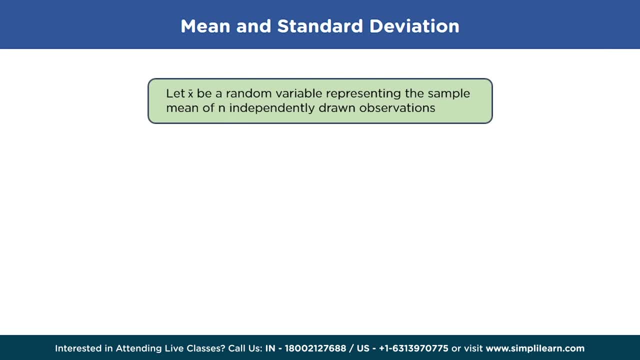 with mean mu and a standard deviation sigma. Let x be the random variable representing the sample mean of n independently drawn observations. Then we can say that the mean of the sampling distribution of the sample means is equal to the population mean, which is mu. x bar is equal to mu. 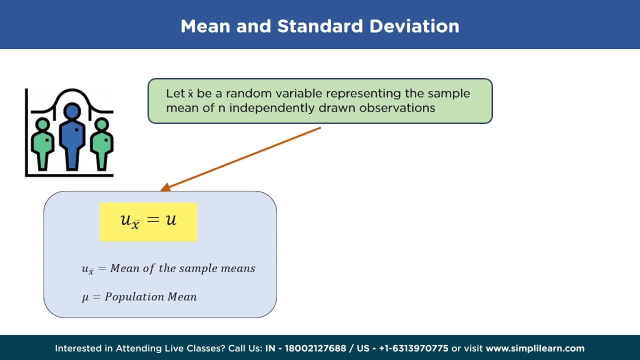 where mu x bar represents the mean of the sample means and mu represents the population mean. On other hand, the standard deviation of the sampling distribution will be equal to the population of the total standard deviation upon the under root of sample size. Let's understand this more. 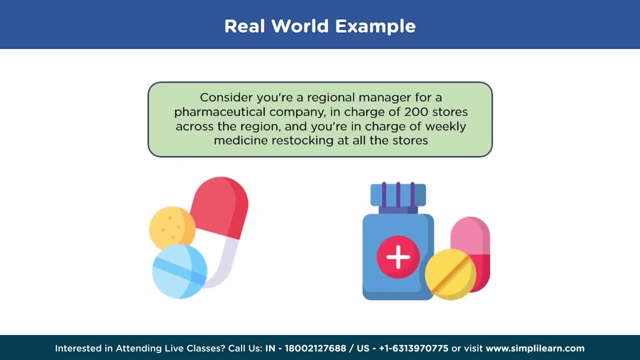 clearly by taking a real world example. Suppose you are a regional manager of pharmaceutical company in charge of 200 stores across the region and you are in charge of weekly medicine restocking at all of them. You need to know how many cases to order weekly for each store in order. 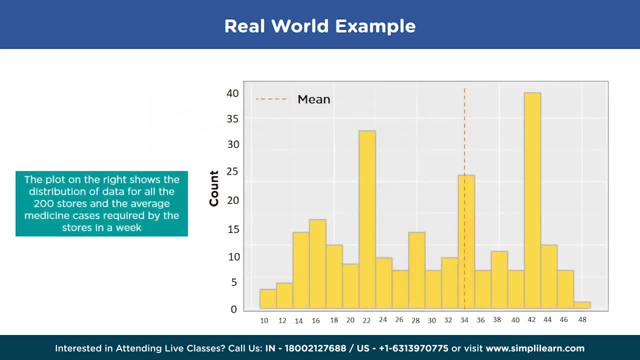 to reduce the amount of inventory that expires. The plot on the right hand side shows the distribution of all the 200 stores and average medicine cases required by each of the stores in a week. The red line represents the average cases required, which is equal to 34.. 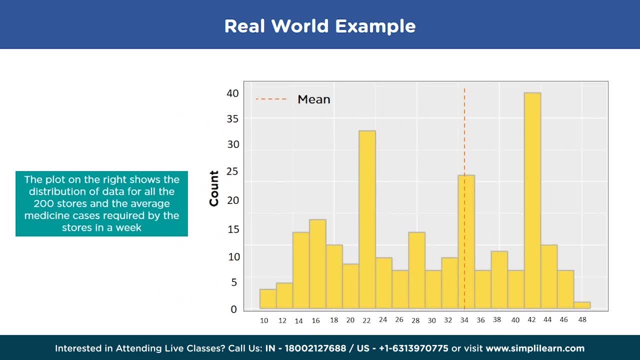 You know there has to be a better way to arrive at a reasonable answer that doesn't entail visiting every single store in your area and obtaining their weekly sales figure. You can apply the central limit theorem to this problem. not that you understand the concept. 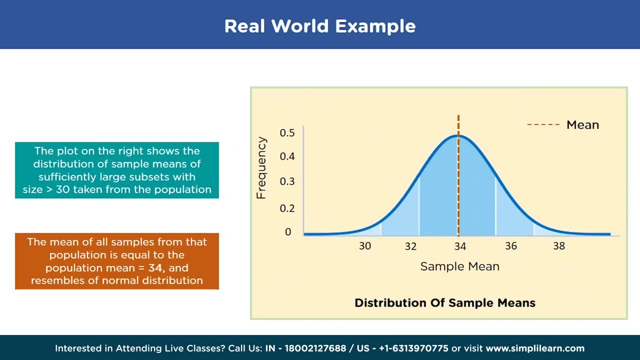 You already knew, the central limit theorem, When applied to a real world problem, aids in balancing the time and cost of gathering the data required to draw the conclusions about the data. So here you can see. the plot on the right hand side shows the distribution of sample means of the 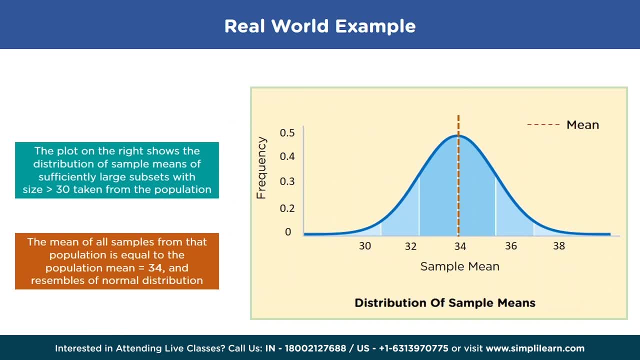 sufficiently large subsets taken from the population Sample size greater than 30 will be sufficient enough to get the normal bell curve. The mean of all the samples taken from that population mean is equal to 34, which is equal to the sample mean of the subset. 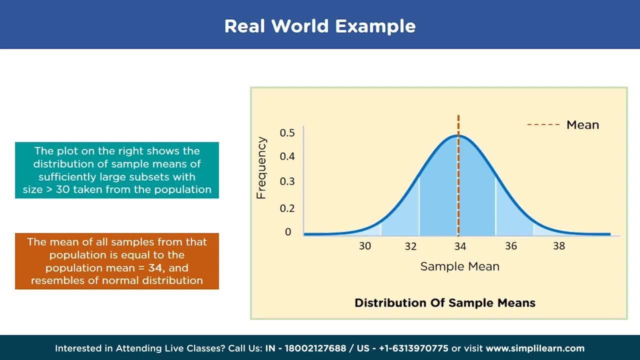 If you plot the sample means, you will get a normal distribution which is a form for bell curve. If these samples meet the central limit theorem criteria, you can assume the distribution of the sample means can be approximated to the normal distribution. Now you know how to apply the central limit theorem. 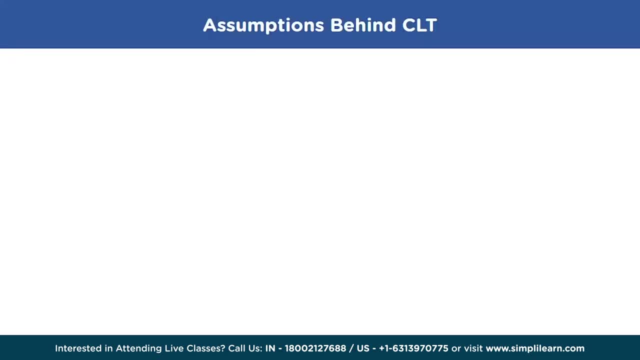 in a real world problem. Let's discuss some assumptions behind the central limit theorem. The first one is the randomization condition. The data must be sampled at randomly and it must adhere to the randomization rule. The second one is the independence assumption. 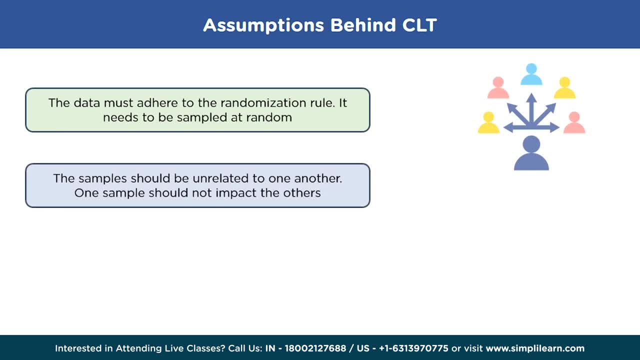 The sample value must be independent of each other. This means that the occurrence of one event has no influence on the next event. Usually, if we know that people or items were selected randomly, we can assume that the independence assumption is met. The third and the last one. 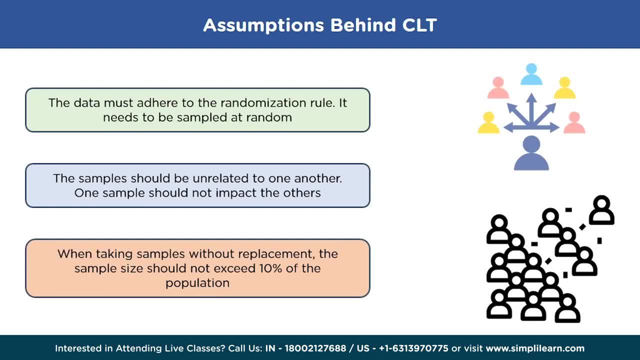 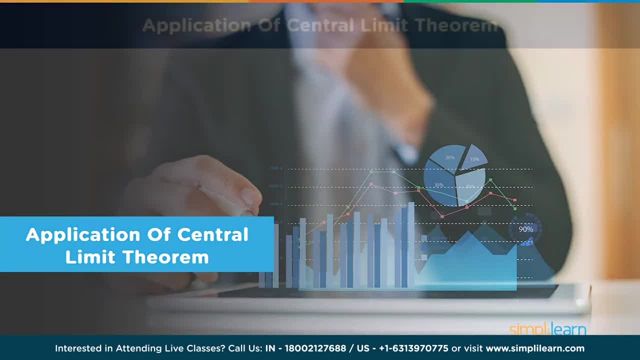 is the 10% condition. This states that when the sample is drawn without replacement, the sample size, which is n, should be no more than the 10% of the population. Let's now discuss some application of the central limit theorem. Sample and election polling is a great example to show. 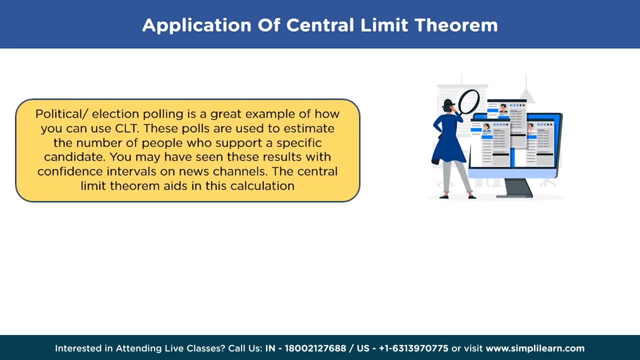 how you can use the central limit theorem. These post results are used to estimate the number of people who support a specific candidate, To calculate the confidence interval, which is shown on the news channel. the central limit theorem is very useful in this. One more place where you can use the central limit theorem. 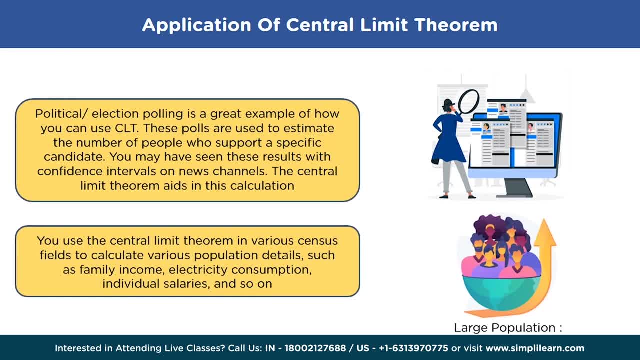 is the census data. You use the central limit theorem to calculate the various population details, such as family income, electricity consumption, individual salaries and so on. Now that we have a good understanding of the central limit theorem, its theories and application, let's see. 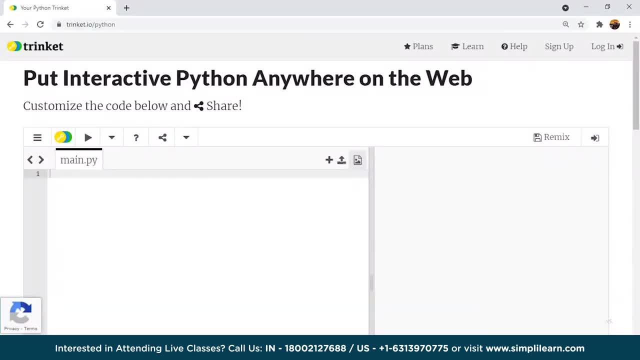 a demo in Python to understand it more clearly. Here we are on an online compiler. We'll discuss the CLT by taking a dice example. A dice is a different number on each side, ranging from 1 to 6.. Each number has a 1 in. 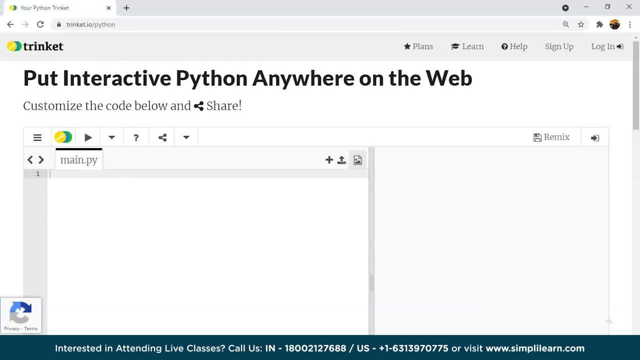 6 chances of appearing on a roll. Given all the equal likelihood, the dispersion of the numbers that come up from a dice roll is uniform. Let's start by importing some necessary libraries. We'll import the numpy first From numpyrandom. we'll import the. 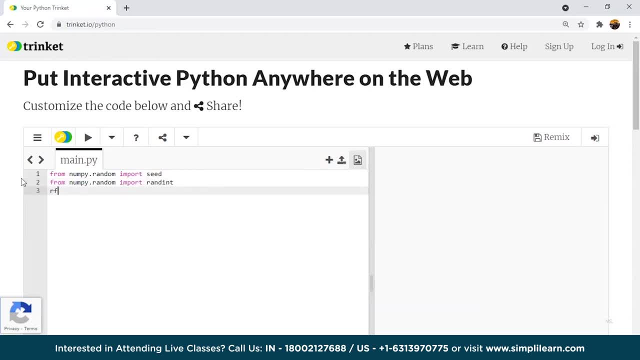 random function which will be used to generate the random integers. We'll also import the mean function from the numpy. We'll set the seed to 1.. Now we'll write the function to generate the random numbers. The randit function will generate a number. 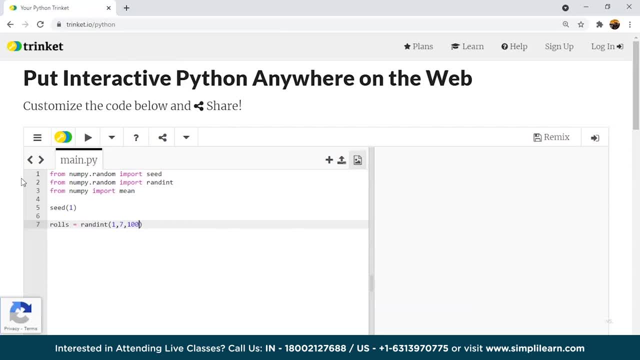 ranging from 1 to 6.. We have taken the 100 because the example will generate the print samples of 100 dice rolls along with the mean Print the rolls and then we'll print the mean of the rolls. So when you run this code, you'll get the following: 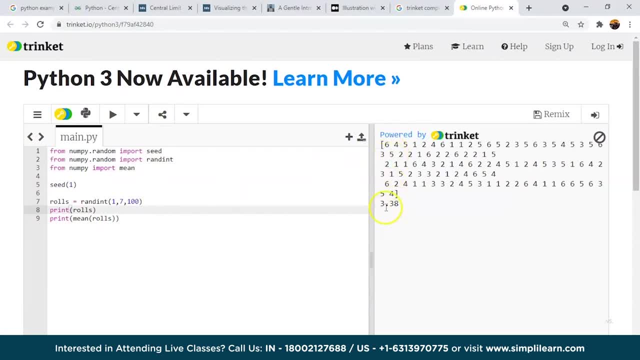 result. You see, we have the 100 numbers and the mean of this number is 4.38.. Now we'll repeat the process 1000 times. This will give you the result of 1000 sample means. According to the CLT, the result of the sample means. 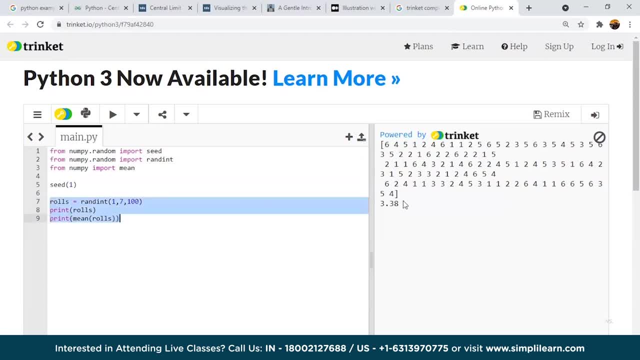 will be Gaussian, So we'll change this code. from here. Means will be equal to mean of this random integers. We'll take from 1,7,100 and this will be 4 in range of 1000.. Now we'll plot this distribution. 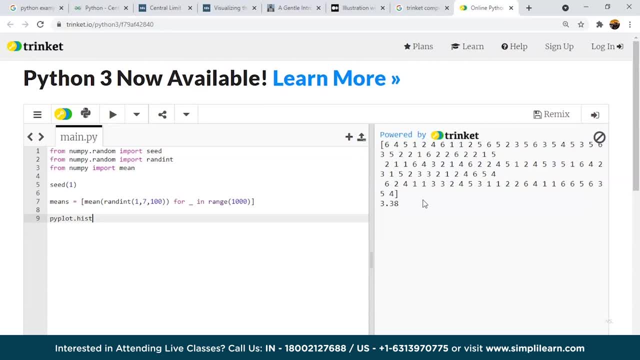 We'll use the pyplot function. We'll get the graph as a histogram graph, So we'll plot it in that Means and pyplotshow. Let's recheck our code. We have the random integer function. We have the feed. We have imported the mean. 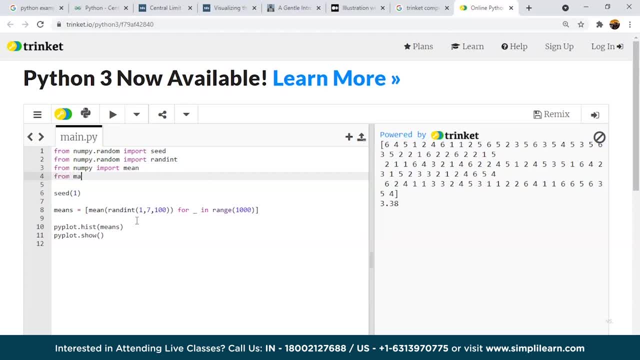 We have not imported the matplot library, So from matplot library we'll import pyplot Now. I think everything is in place. Now let's try to run this code. Yep, you can see. this graph is a histogram graph In the shape of a bell curve. 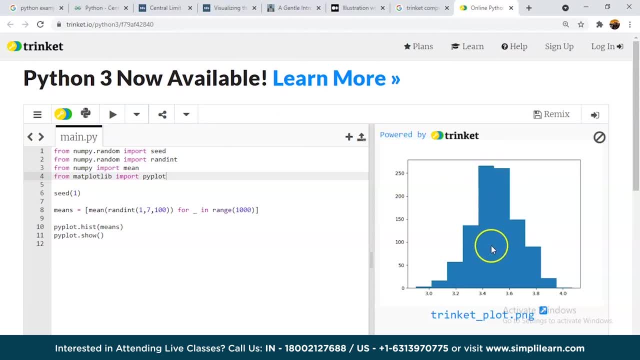 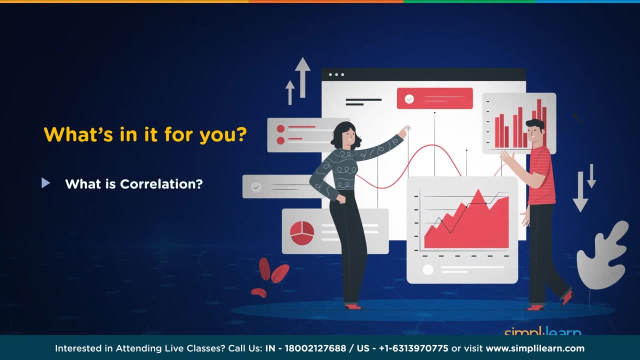 And if you see closely, the mean is closely to 3.4.. We'll start by discussing what is correlation and correlation coefficient. Then we'll move on to discuss PSN's rank correlation and its formula. Then we'll move on to Excel and Python. 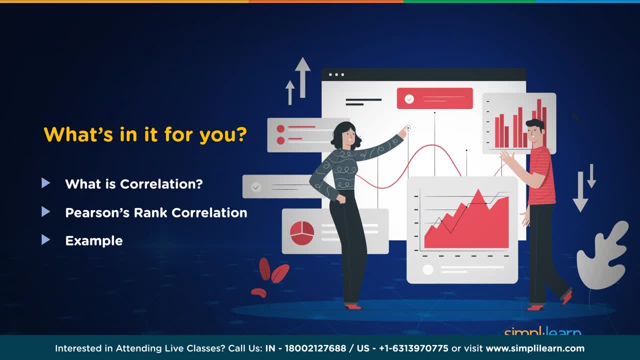 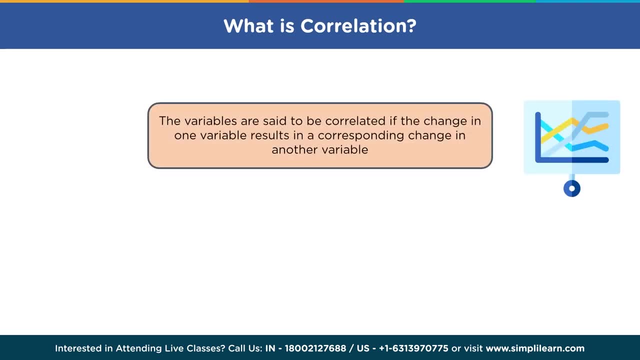 to see how you can calculate the PSN's rank correlation coefficient. So what is correlation? The two variables are said to be correlated if the change in one variable results in the corresponding change in another variable. It can be positive or negative, For example. 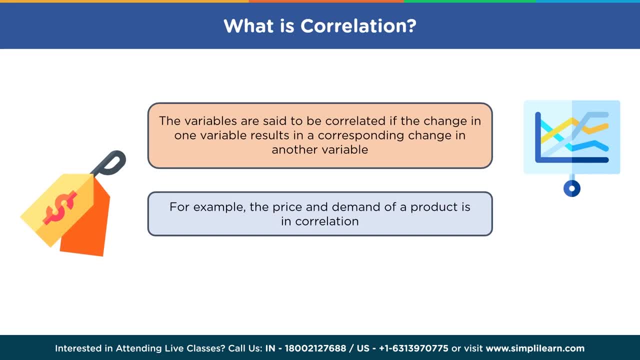 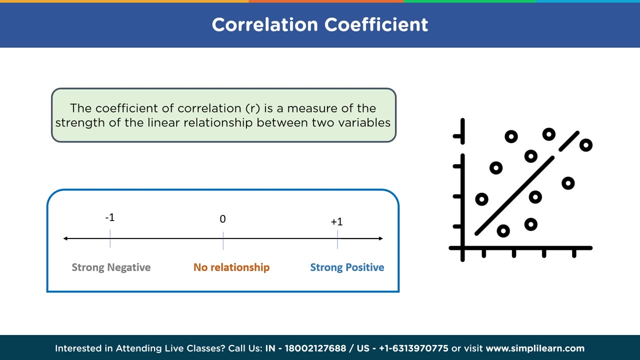 the price and demand of a product are in correlation. As the demand of a product increases, the price increases simultaneously. The value of the correlation always lies between minus 1 to plus 1.. Minus 1 shows a strong negative correlation. 0 shows 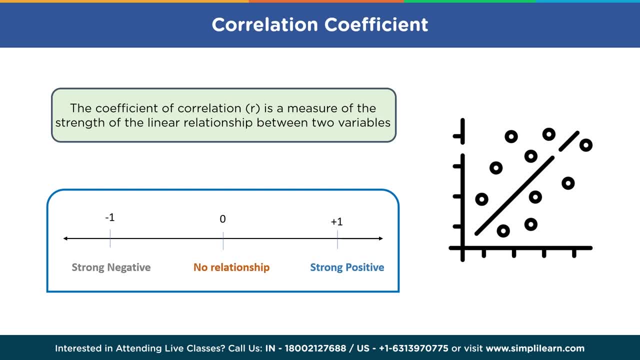 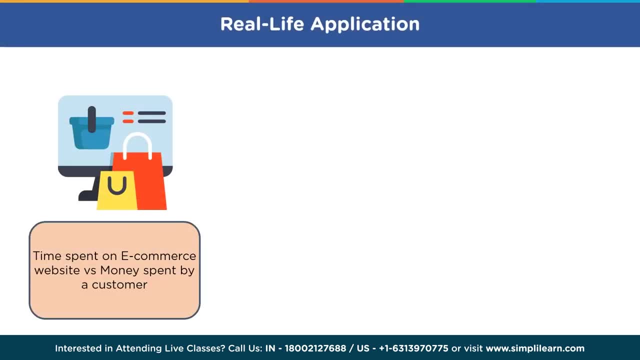 that there is no relationship between the two variables And plus 1 shows that there is a very strong correlation between the two variables. Some of the examples can be the time spent on e-commerce website versus the money spent by the customers. It can be taken as an example of positive. 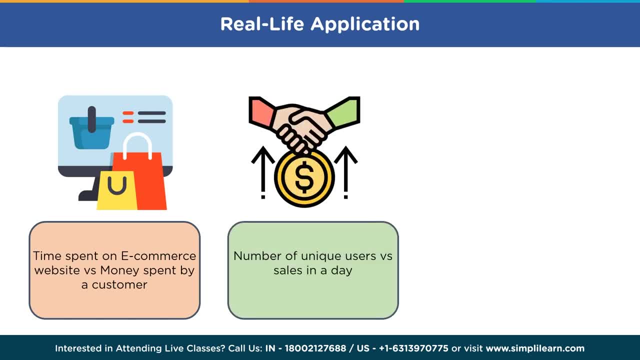 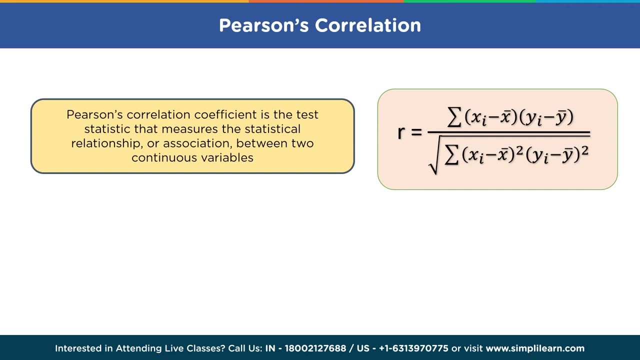 correlation. Number of unique users versus sales in a day are also correlated. Correlation can also be used to measure the patient's blood pressure and the medication used. Now let's discuss what is PSS correlation? PSS correlation coefficient is a statistical test that measures 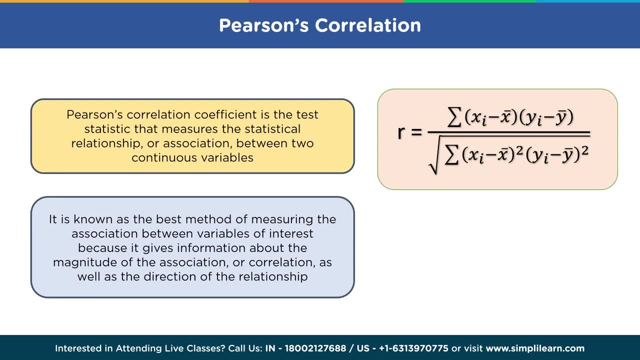 the relationship or association between the two continuous variables. It is known as the best method for measuring the association between the two variables because it gives the relationship between the magnitude of the association as well as the direction of the relationship. The formula to calculate the PSS rank correlation is: 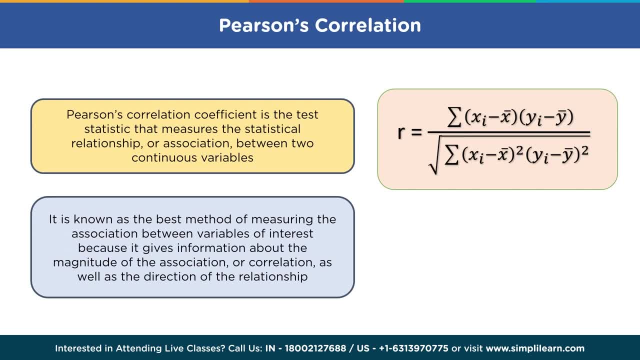 r is equal to sigma xi minus x bar bracket, yi minus y bar, divided by under root of sigma. sigma xi minus x bar whole square. yi minus y bar whole square. In this case, r is the coefficient of correlation, x bar is the mean of x variable. 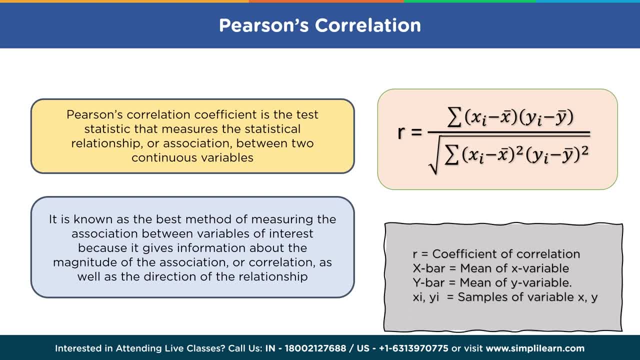 and y bar is the mean of y variable, And xi and yr are samples of the variable x and y. Now that we know the PSS rank correlation, let's move on to excel and then python to see how you can calculate these rank correlation coefficient. 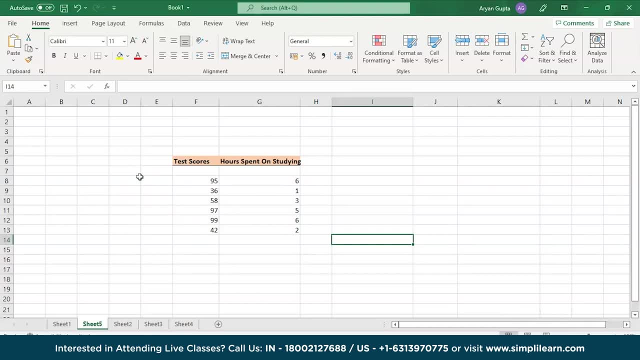 So here we are on our excel workbook. As you can see, we have two columns. One is test scores and other is hours spent on studying. We have to find the correlation between the two. That means how the test scores and the number of hours. 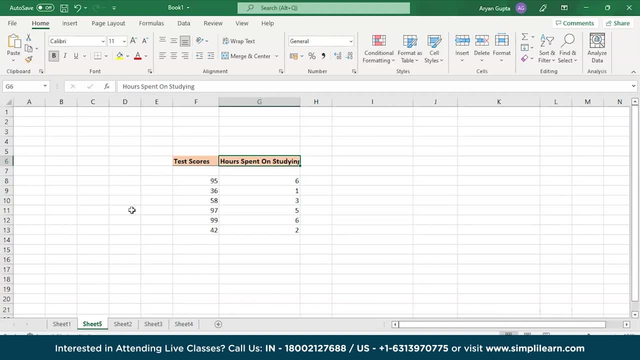 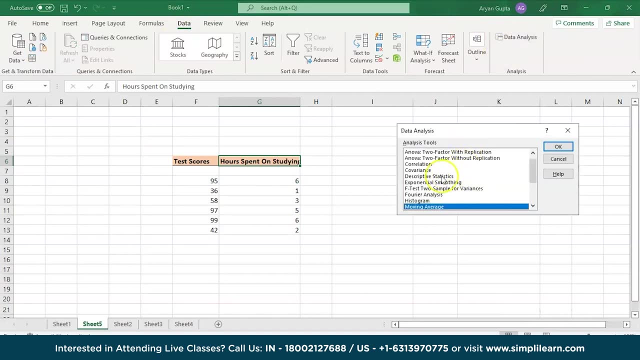 spent on studying affect each other. So to do that, we will first move on to data tab and we will say data analysis. Here we will go on to correlation and click ok. Now it is asking for input range. So here we will select both the columns. 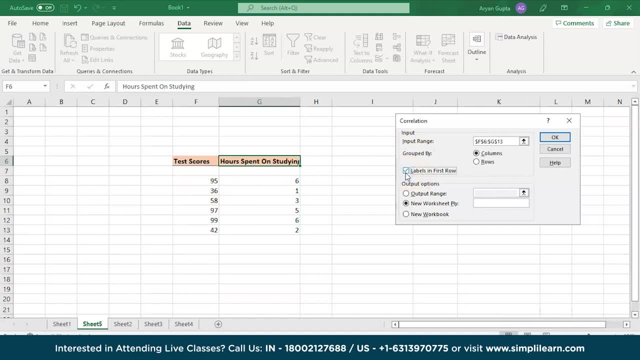 as an input range. We have the labels in our first row, so we will check on the labels. Now for the output range. we will give the output range in the same sheet. So we will select these cells for our output range. We click ok. 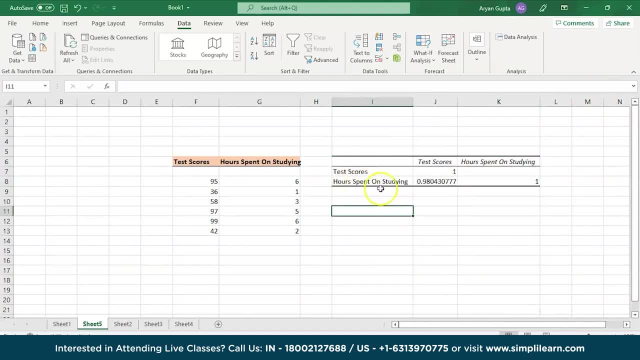 and now you will see: the test scores and hours spent on studying are very positively correlated. That is 0.98, which shows a very strong correlation. It means as the number of hours spent on studying increases, the test score will definitely increase. There is one more way to. 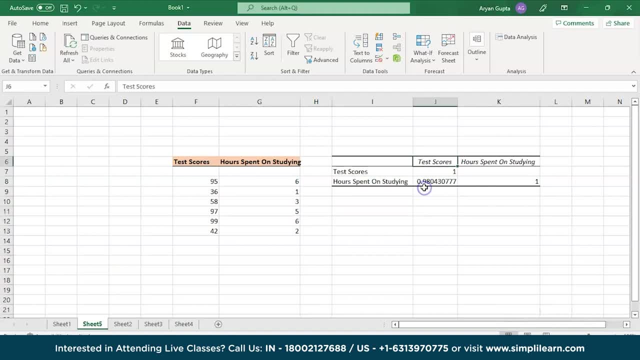 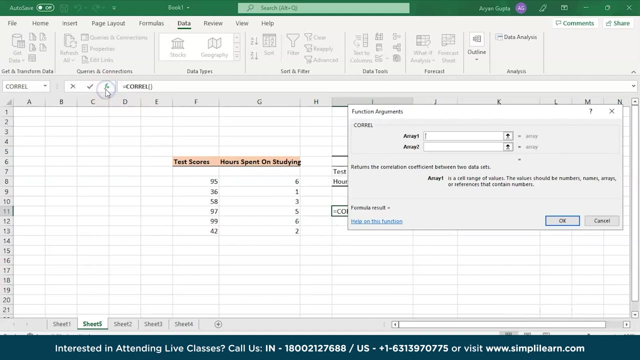 calculate the correlation using function. So to calculate the correlation between test scores and hours spent on studying, we will type equal to tab. and now it is asking for array 1 and array 2.. Let's open this function. So this is asking for array 1.. 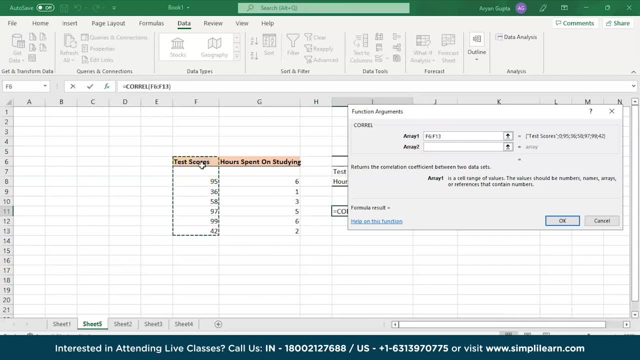 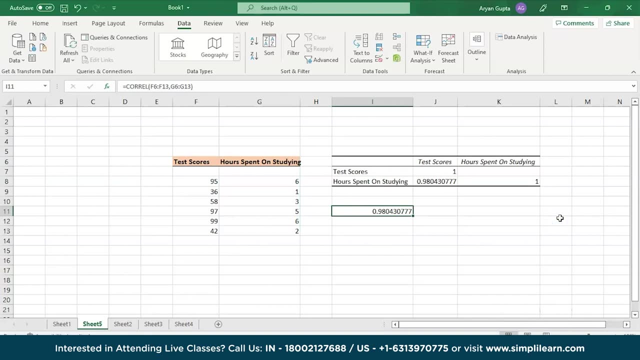 So our array 1 is this range and our array 2 is hours spent on studying. When you click ok, you will get the same value, which is 0.98.. So there are two ways by which you can calculate the correlation. That's it, I hope. 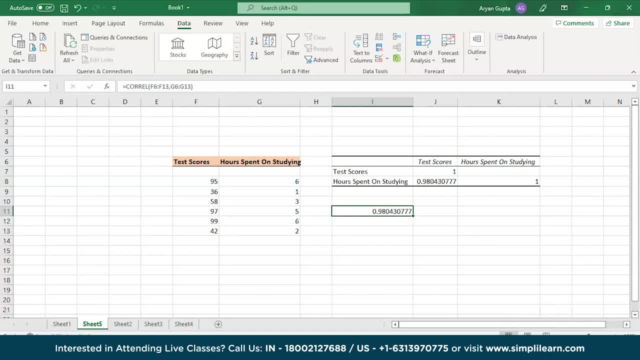 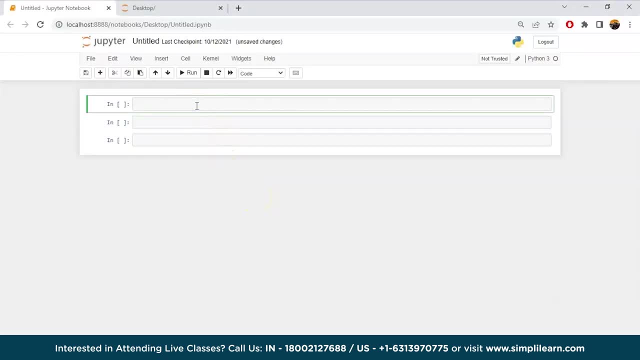 you understood this example. Now let's move on to python, to see how you can calculate the correlation using the python. So here we are on our Jupyter notebook. Let's see how you can use the Jupyter notebook and python to calculate the correlation coefficient. That is: 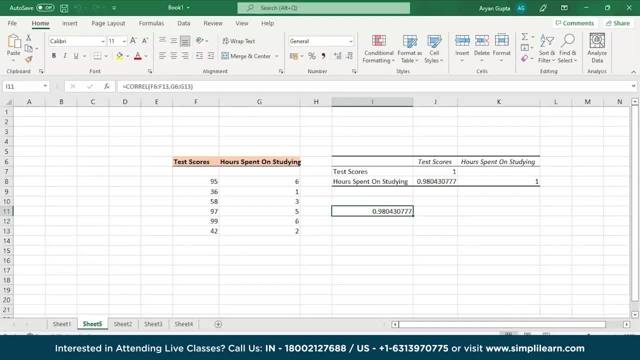 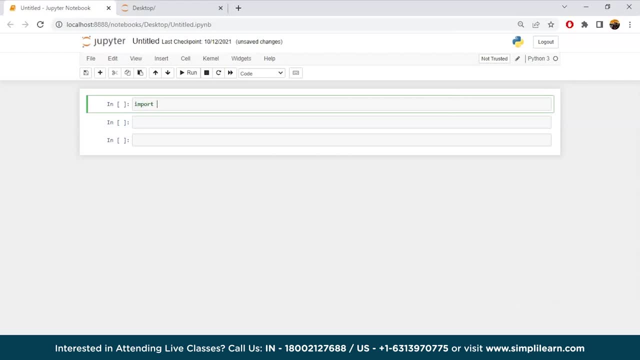 Pearson's correlation coefficient. So first we will feed the data that we have used for our excel example. Let's start by importing numpy. Now in our data sheet we had the test scores, So we will write test scores, and the scores were 95,, 36,, 58. 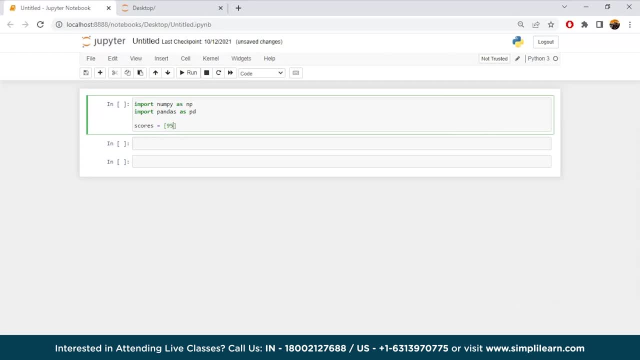 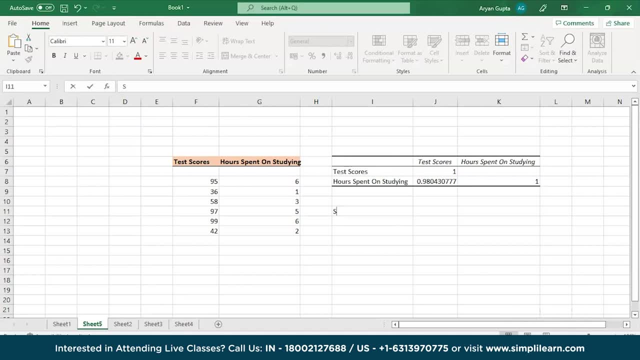 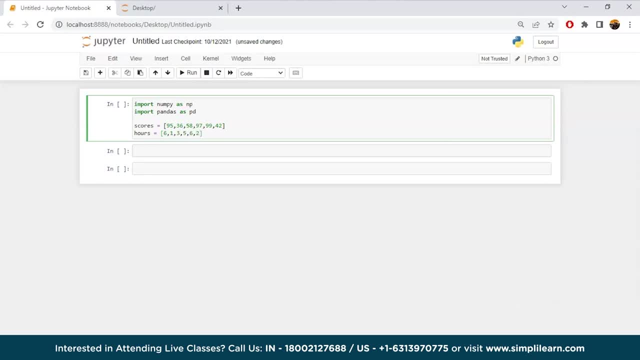 6, 1, 2, 5, 6, 2- 6, 1, 2, 5, 6, 2. So we have entered both the data of scores and hours. Now to calculate the correlation coefficient, we will use the function. 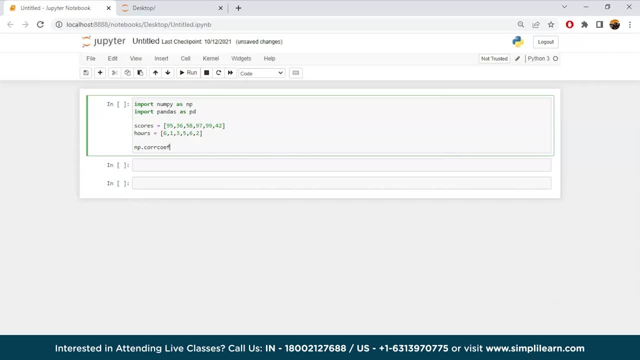 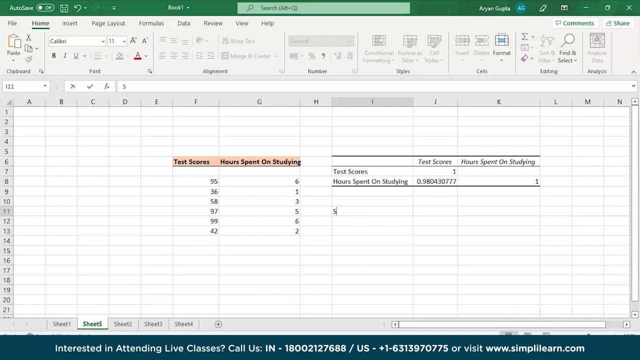 corl correlation coefficient and we will mention both the data sets, that is, scores and hours. Now let's run to see if we get the same value as in excel. So you can see we have the same value of 0.980 as our correlation coefficient and it matches with our excel data. 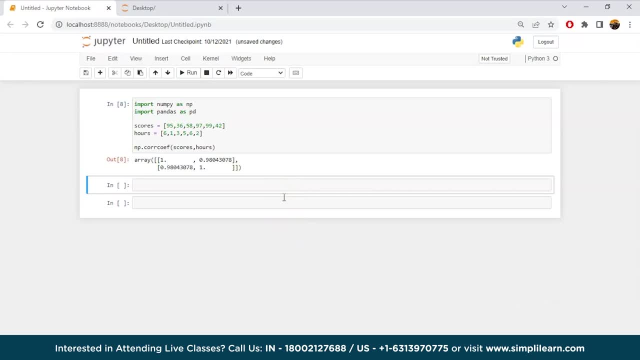 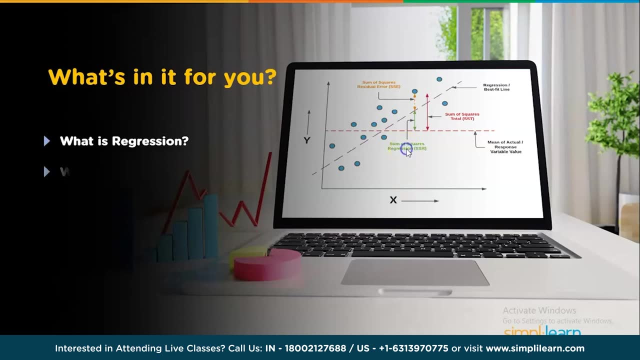 So in this way you can calculate a correlation coefficient using python. We will explain the concept of regression using a machine learning algorithm to you. Next, we will take a look at the r squared error, which can be used to calculate the error in regression models. Next, we will teach you how to calculate. 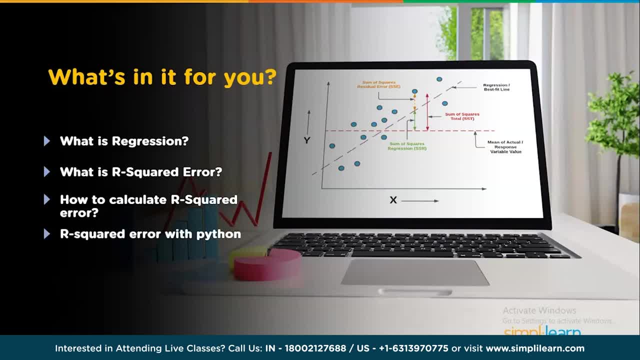 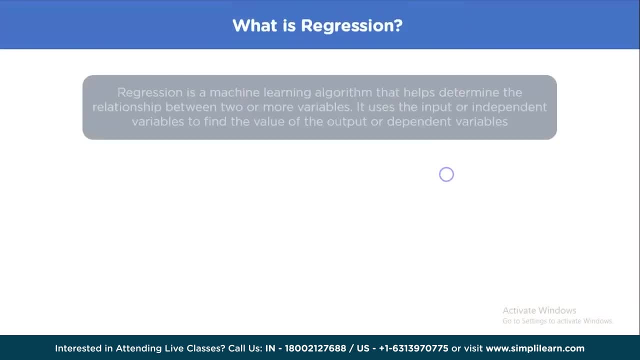 the r squared error. and finally, we will implement the r squared error with the help of python. So what is regression? Regression is nothing but a machine learning algorithm that helps us determine the relationship between two or more variables. It uses input or independent variables to find the value of the output. 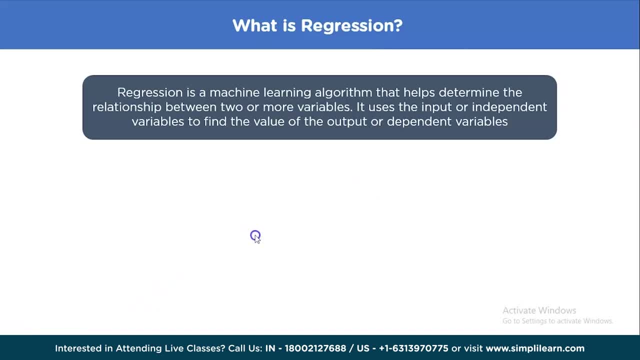 or dependent variables. Regression is a prediction algorithm which means that, given some variables, we can predict the value of an output variable. The predicted value is not going to be from a set of values, but is going to be a unique value in itself. Now let's understand what exactly regression is. 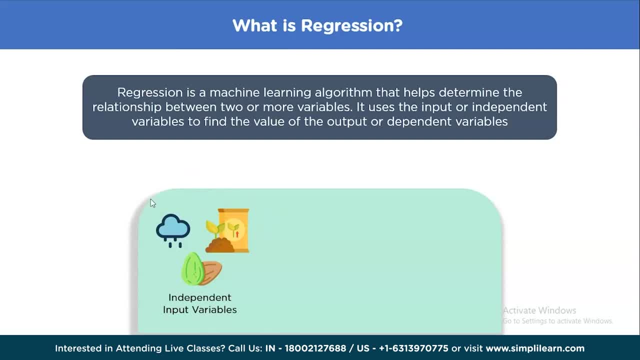 with the help of a few independent input variables. In this case, the variables that we will be looking at is rainwater, fertilizer and seeds. When we pass these independent input variables through a regression model, we are going to get a predicted output. The output predicted is that a crop. 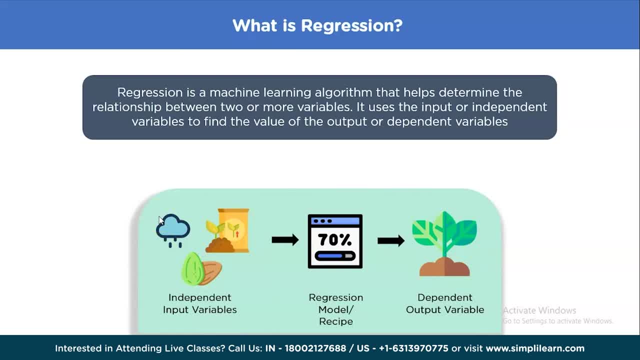 will germinate when all three of these components are put together in certain quantities. So with the help of regression or input data, we can find out the dependent output variable that we will get when all of these input variables are more or less combined. Regression is nothing but a statistical method. 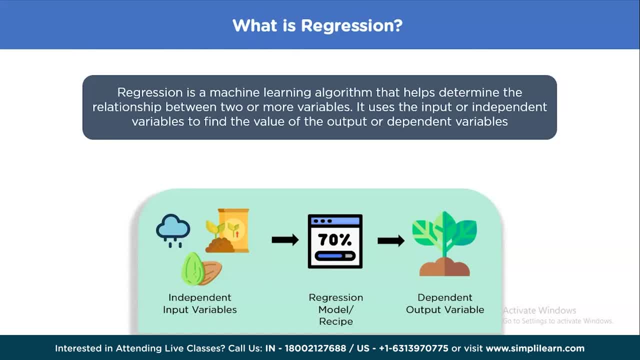 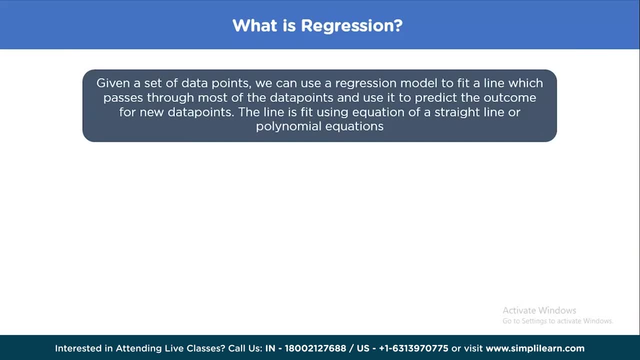 which is used to determine the strength and character of the relationship between a dependent variable and a series of other variables. Now, using regression, if we have a set of data points, we can use a regression model that passes through most of these data points and use it to predict the outcome. 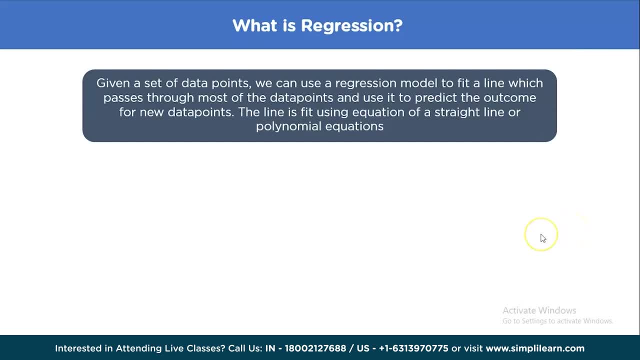 for new data points. The line is fit using equation of a straight line or a polynomial equation. Now, in this graph, consider that we have our dependent variable, or the output y, and our independent variable, or the output x. For a certain value of our independent variable, we are going to get a certain value. 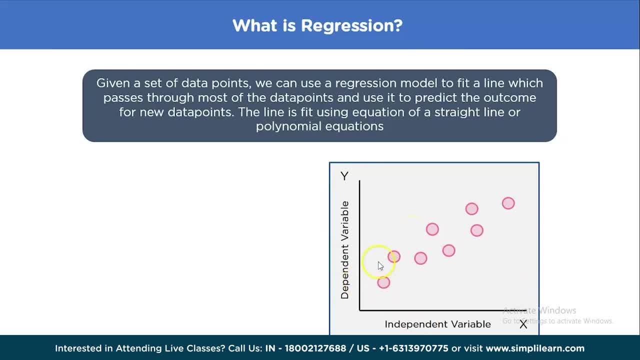 of our dependent variable or our output. Using the data given here, our output varies when our input varies. To predict the value of our outcome y we are going to need to find a relationship between all of these data points. To do this, we are going to plot a straight line through it. 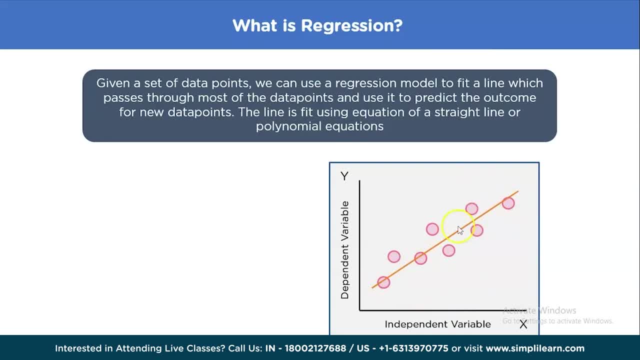 because, as you can see, all the data points lie more or less along a given straight line. Now, using this straight line, for any value of x, we can find the approximate value of y. So suppose you want to find the value of y for a point x, which is given here. 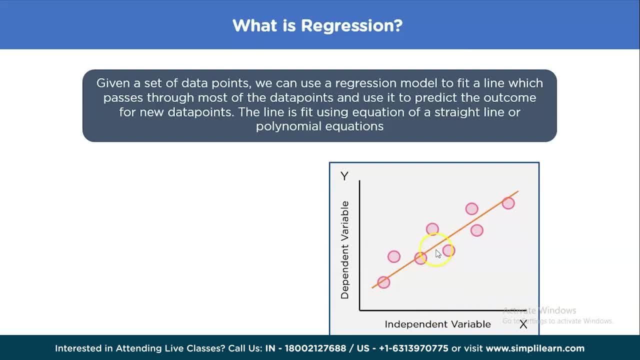 then all you have to do is extend a line from this point onto a predicted model, which is this line here, and then we can see where this point on the line coincides with the y-axis and get the approximate value of the outcome. The equation of a straight line. 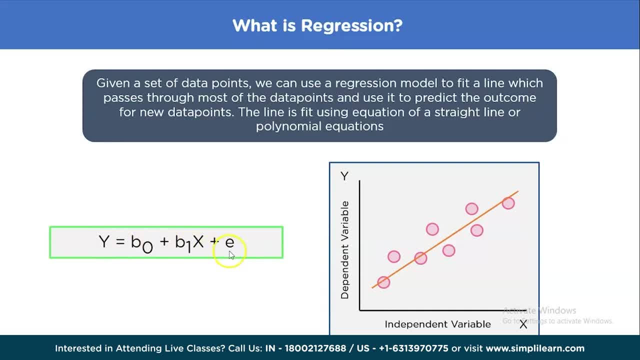 is given as: y is equal to b0 plus b1x plus e, where b0 is a constant y-intercept of our line, or basically, where the line intersects on the y-axis, b1 is the slope of our line and x is the point for which we want to find the output. 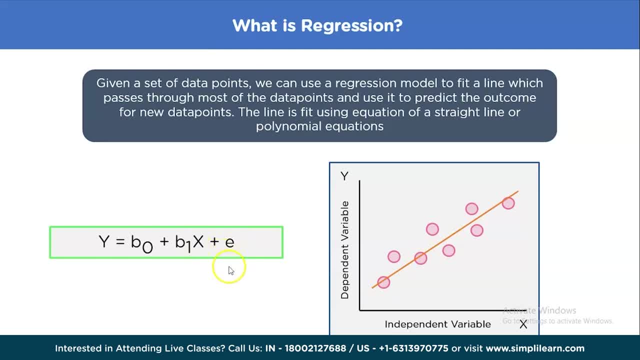 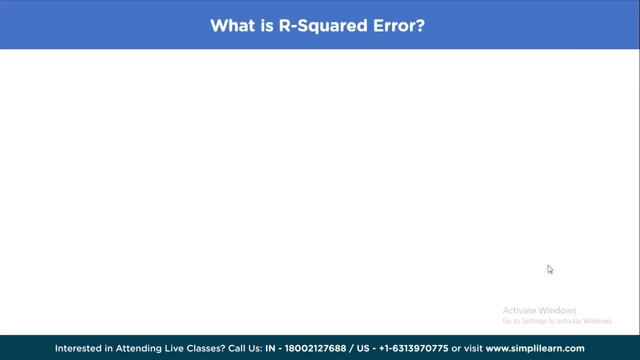 e in this case, is nothing but an error correcting term. So this is basically how regression works and this is how prediction takes place in our regression model. Next, we will explain the concept of the r-squared error to you. So what is r-squared error? 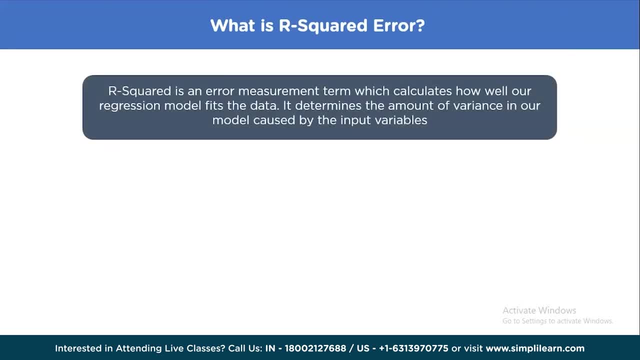 r-squared error is nothing but an error measurement term which calculates how well our regression model fits the data. It determines the amount of variance in our model caused by the input variables. Now, r-squared is a statistical measure that represents the portion of variance for a dependent 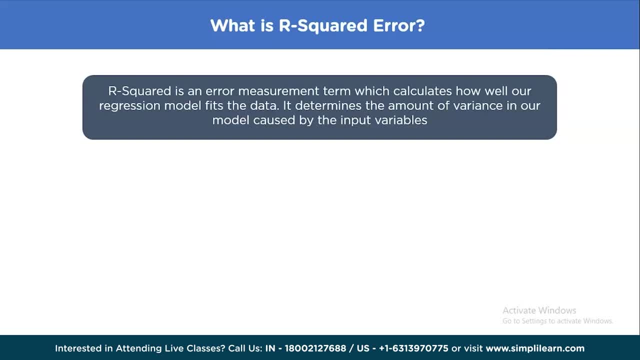 variable that's explained by an independent variable of variables. in a regression model, r-squared is used to explain to what extent the variance of one variable affects the variance of a second variable. So if the r-squared of a model is 0.5, then approximately. 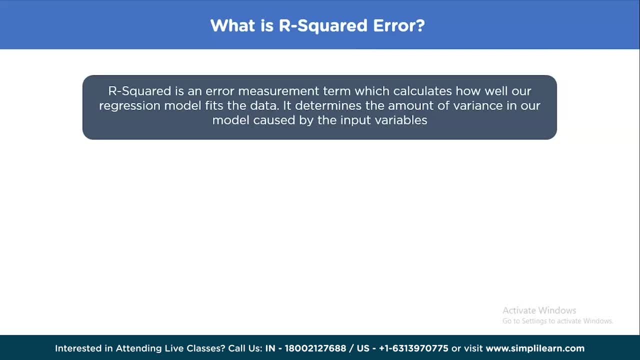 half of the observed variation can be explained by the model's inputs. In other words, an r-squared of 60% reveals that 60% of our data fits our regression model exactly Now, in this case, in this graph, if we have a variance of 60%, 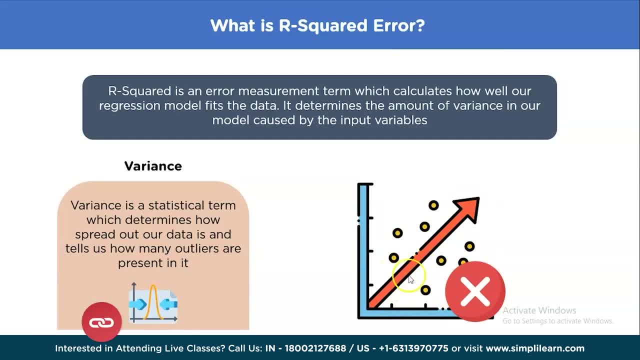 it means that 60% of our data points fall exactly on our regression line. However, it is not always the case that a high r-squared is good for a regression model. The quality of this statistical measure depends on many factors, such as the nature of the variables employed. 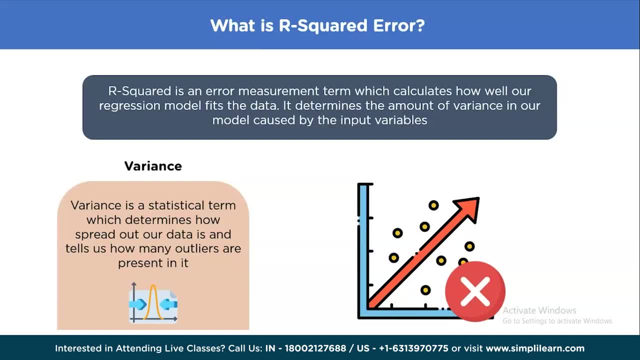 in the model, the unit of measure of variables and the applied data transformation. Thus, sometimes a high r-squared can indicate the problems with the regression model. A low r-squared figure is generally a bad sign for predictive models. Now, all this time we've been 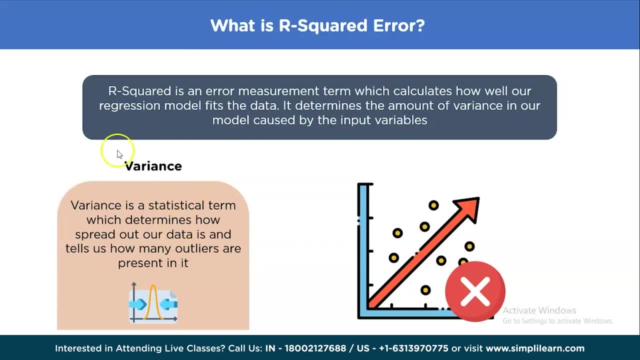 talking about variance in our model. What exactly is variance? Variance is nothing but a statistical term which determines how spread out our data is and tells us how many outliers are present in it. Basically, it's a measure of how far a set of numbers is spread out from. 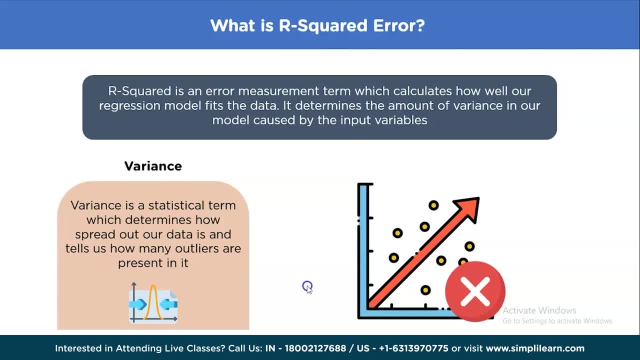 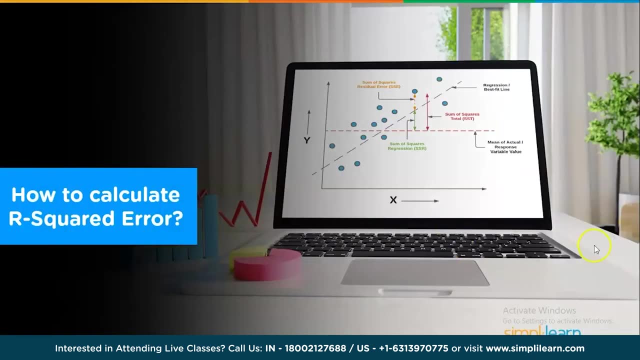 their average value. Using variance, you can basically figure out where your data is centered and how spread it is from the mean, and also you can find out how many outliers it has. Now how can you calculate the r-squared error? Let's start by considering the data. 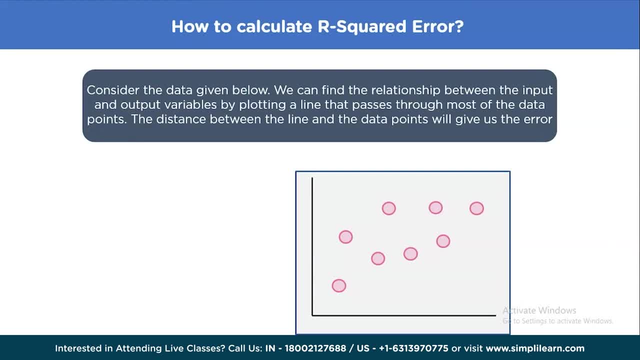 that we have been given, as shown below. Now we can find the relationship between the input and the output variables by plotting a straight line or a regression model that passes through most of the data. To get the perfect fit for our model, we don't necessarily need to have 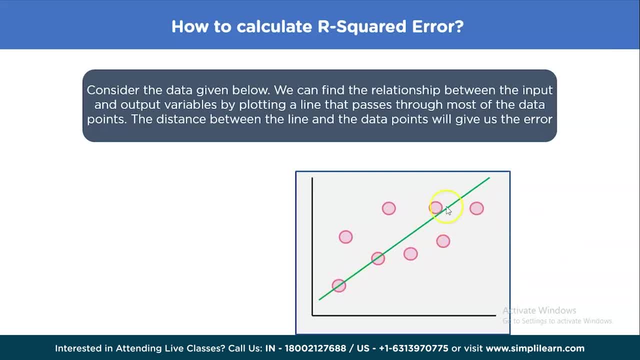 the line passing through as many data points as possible. A true measure of a good model is that we reduce the error which is present in our model. Now, how do you find this error? The error present in our model is given by nothing but the distance between our predicted line. 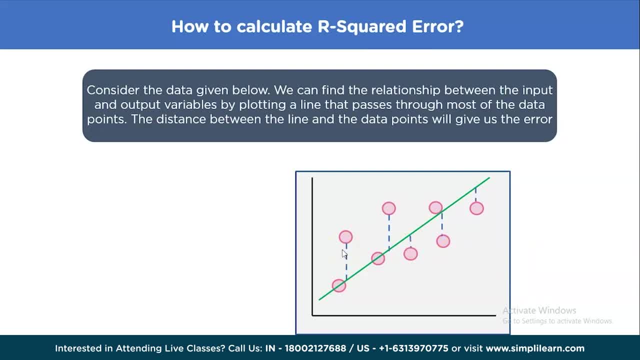 and the data points which do not fall on the line that we have to minimize. The distance between our data points and our line can be calculated by subtracting our data point from the point at which it coincides on our regression line. We square this just to get rid of. 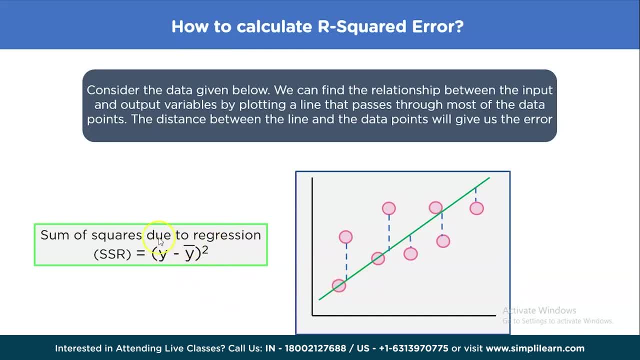 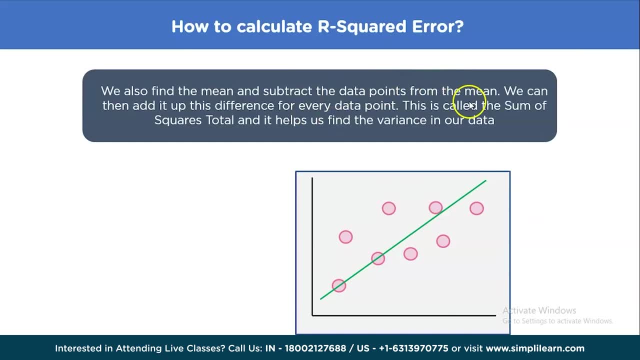 any negative coefficients that may occur due to finding the difference between the two points. Now to find the variance in our data, we are going to find the mean and subtract the data points from the mean. This will basically tell us what our data point is from the average value. 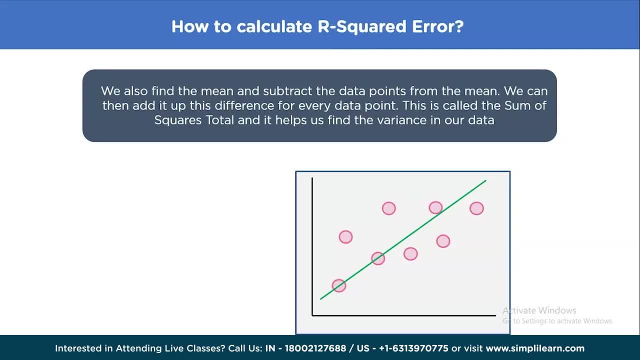 We can then square these differences and add up the result to get our total variance. This is also known as the sum of squares total, and using this we can find the total variance in our data. The mean is nothing but the average of our data, and using the mean, 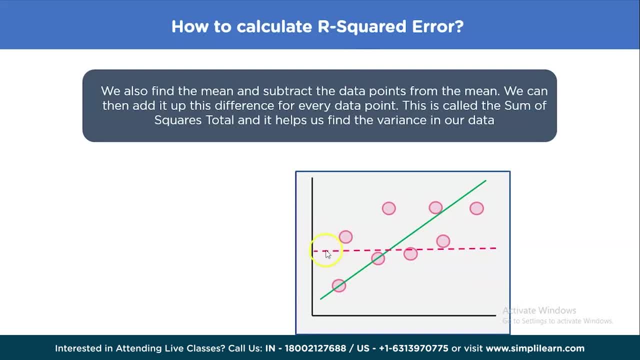 we can find the center of our data. So this is exactly where our data is centered. This is the average value that occurs in our data. This is nothing but the distance of all of our data points from the mean. If we do this, we are basically going to find out. 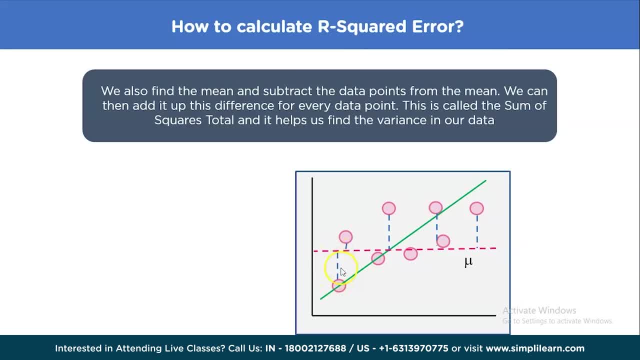 how spread apart our data is from the average value or how far all of our data points lie from each other. When we subtract the position of our data points from our mean and square it and add all of that up, we get something known as the sum of squares total. 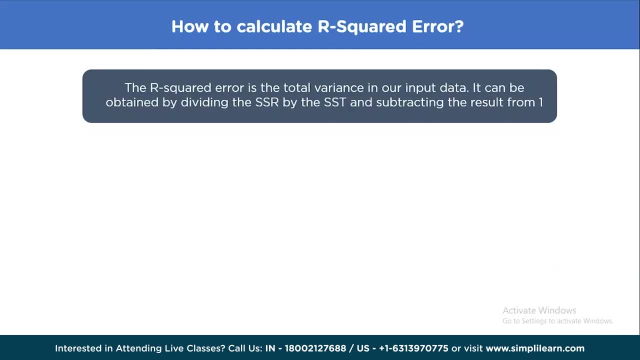 Now, the R squared error is the total variance in our input data. It can be obtained by dividing the SSR by the SST and subtracting the results from 1, So the R squared error totally becomes 1, minus the sum of our squared errors divided by the sum of. 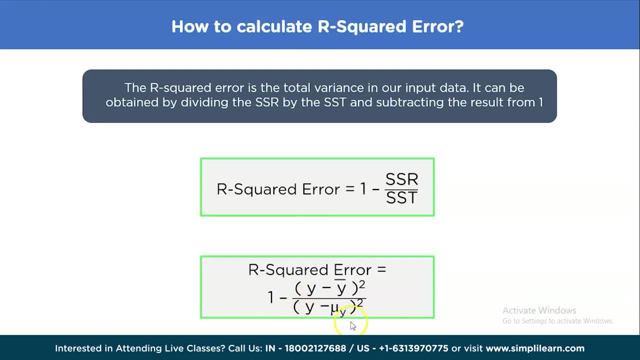 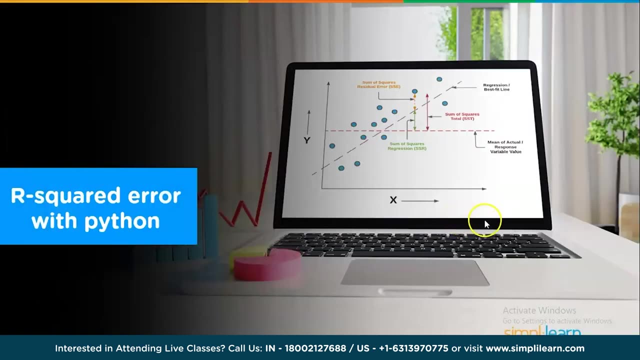 the squared difference between our data points and the mean. Now this value gives us the variance and this is why we can say that R squared is used to find the portion of variation in our data. Now how can you implement R squared error with python To calculate R squared error? 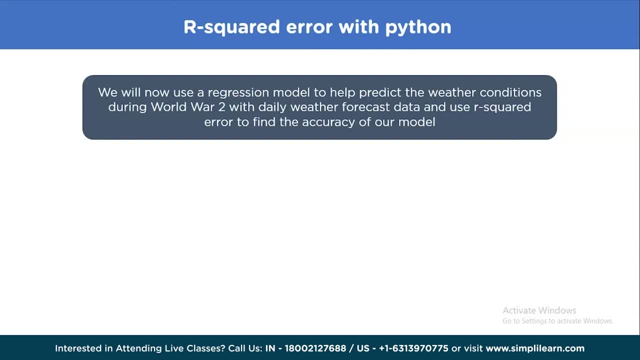 with python, we are going to look at the data which depicts the weather conditions which were present during world war 2 and, using the variables which are present in our data, we are going to create a model which predicts the daily weather forecast during world war 2. 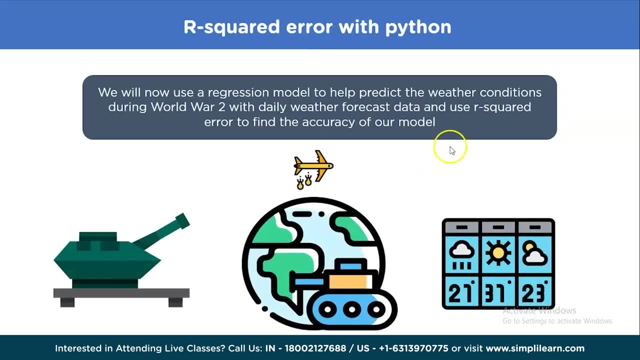 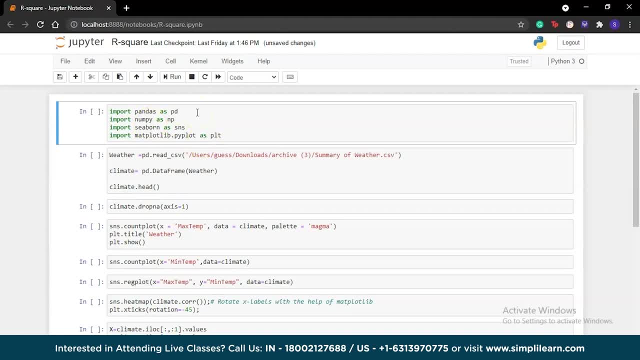 and then we are going to use R squared error to find the accuracy of our model. So this is our R squared error model. So we are going to start off by importing all of our necessary modules. We are going to use the model numpy to perform numerical calculations on our database. 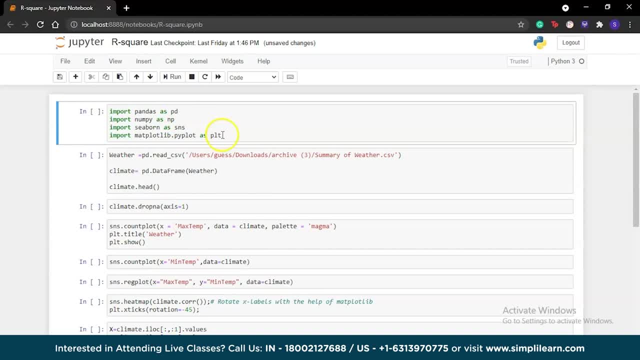 and arrays, and we are going to use cbon and matplotlib to plot our data. So now we have managed to import all of our data sets, Let's also load our data by reading in the csv file that it is stored as in the form of a data frame. 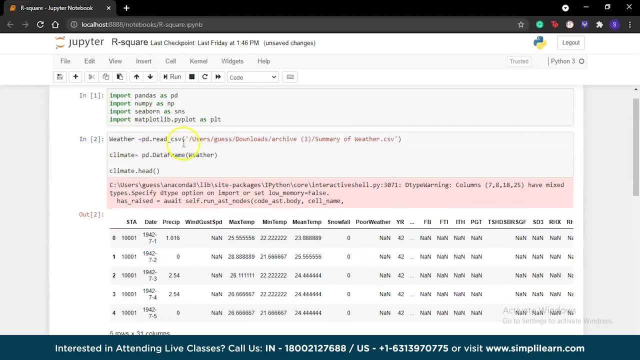 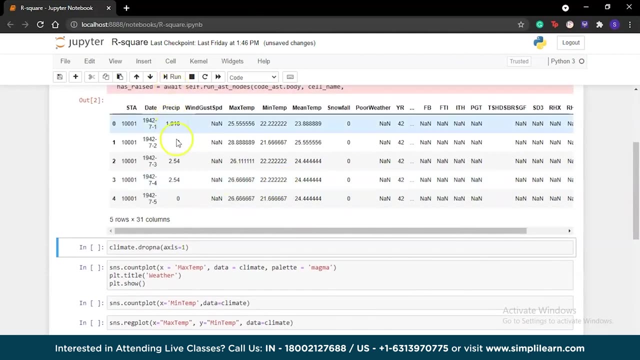 So over here, as you can see, we have read in the csv file into a variable called weather, and then after that we are changing weather into a pandas data frame called climate. This is what our data frame finally looks like. So, as you can see in our data frame, 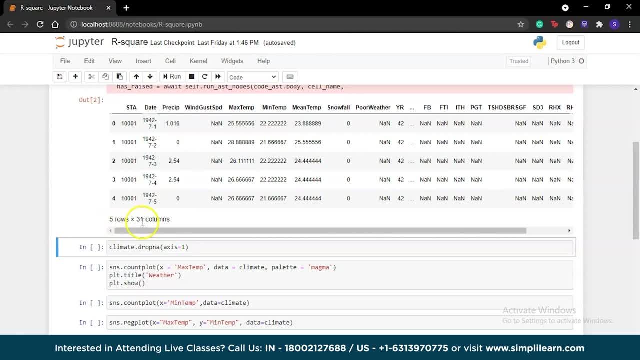 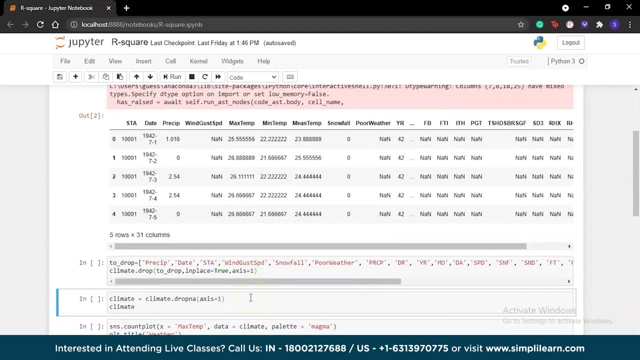 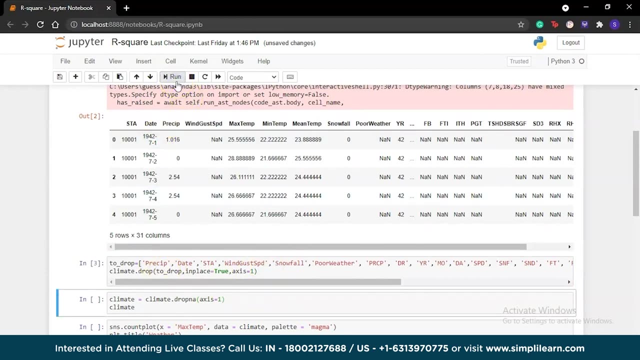 we have 5 rows, because we are only looking at the top 5 rows, and we have 31 columns. So these are variables which are not required and which are basically going to increase our error value. So let's drop them and get rid of them Now. let's also drop 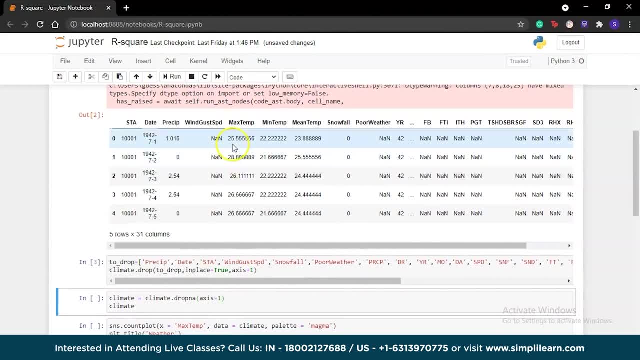 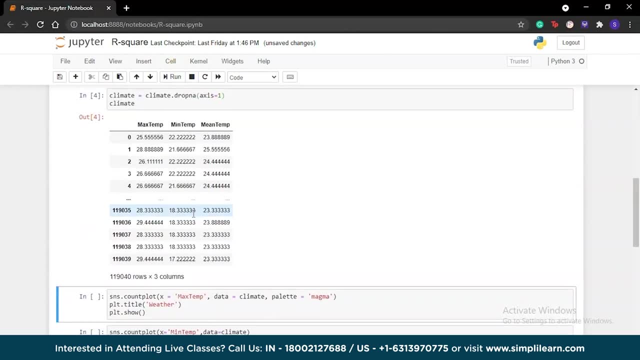 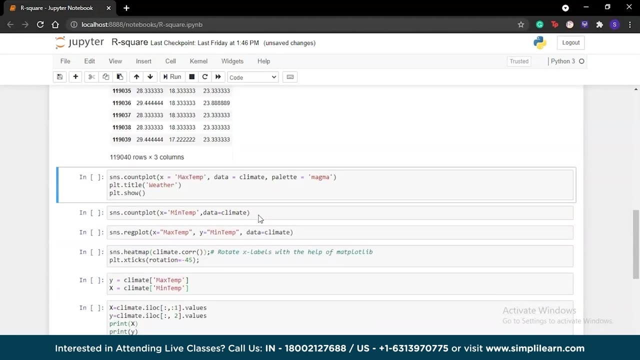 any empty values which may occur in the remaining columns of our data set and see what the final data set looks like. So this is our final data set We have. at the end, we are only left with max temperature, minimum temperature and mean temperature. Now let's plot. 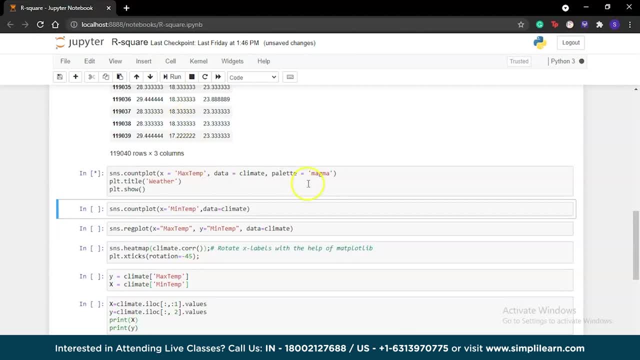 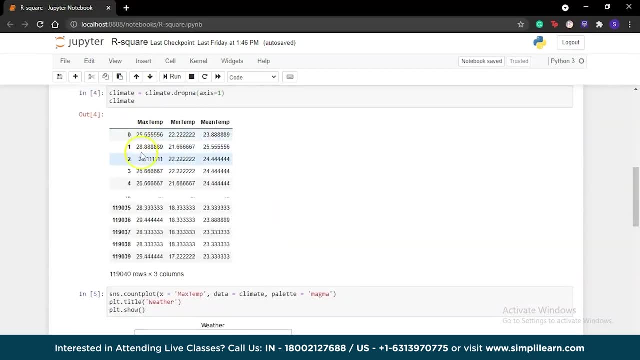 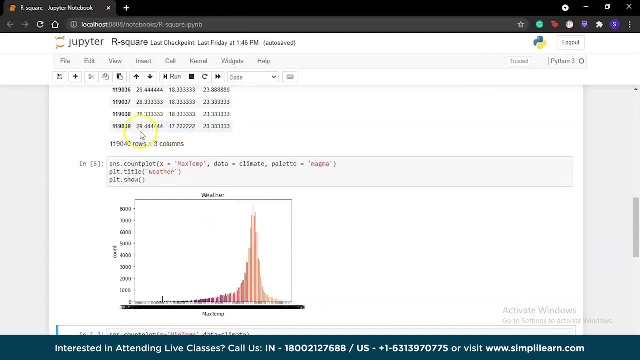 a count plot of our max temperature. A count plot is basically going to go through the entire max temperature column and figure out how many times every temperature value occurs. So it's gonna figure out how many. it's gonna count how many times 29.44444 has occurred. 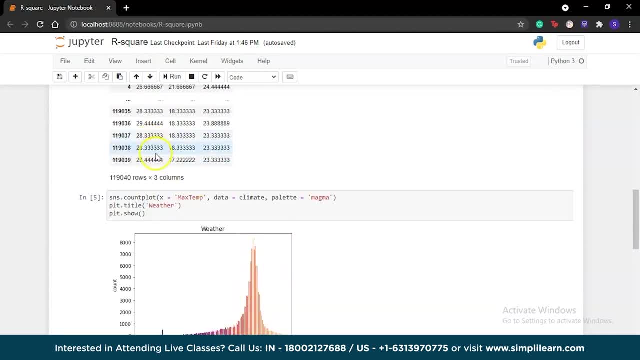 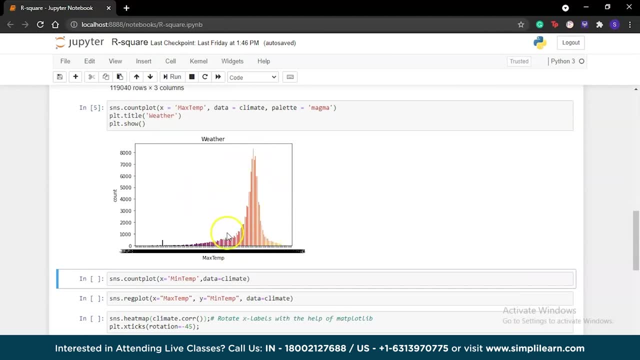 and it's gonna plot that on this graph and it is going to do that for every unique temperature value which is present in our column. So, finally, this is the value that we get, So over here, as you can see, the majority of our temperature values are concentrated within: 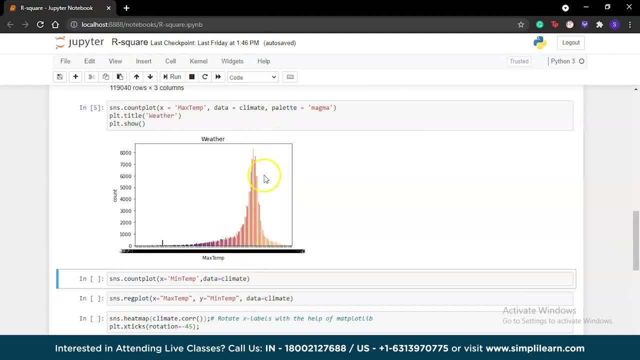 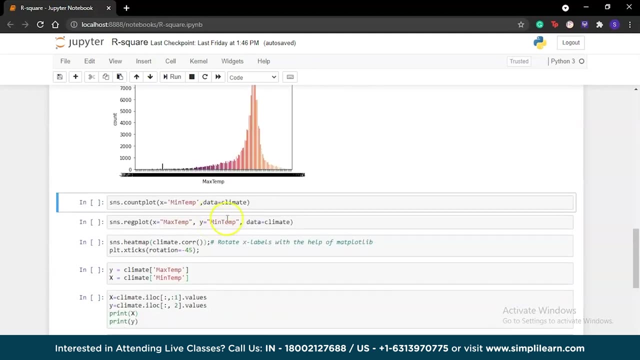 this range. This means that these temperature values are the ones which occur most frequently. The other ones can be considered as outliers, because they rarely are seen in our data and they can further skew the output that we are gonna get. Now let's do the same with minimum temperature. 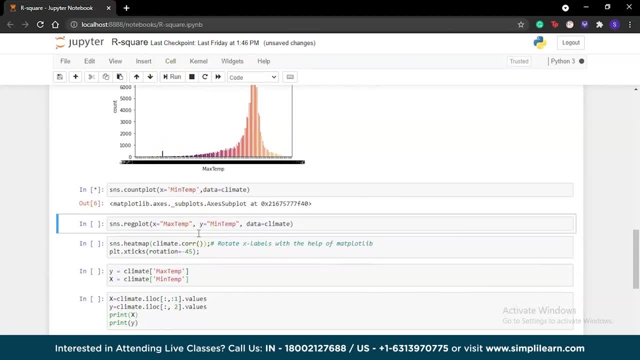 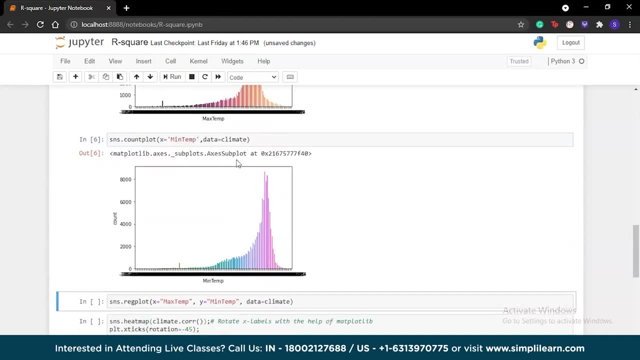 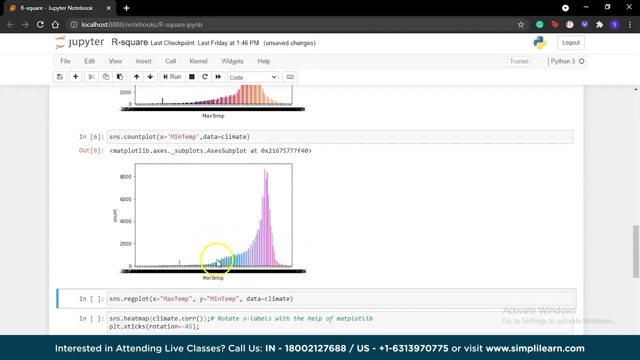 Let's plot a count plot for minimum temperature. So for the minimum temperature we can see a very similar plot to the one that we got for our maximum temperature. Most of the values are concentrated around this region, but the outlier values here are way fewer. Now let's plot a regression plot. 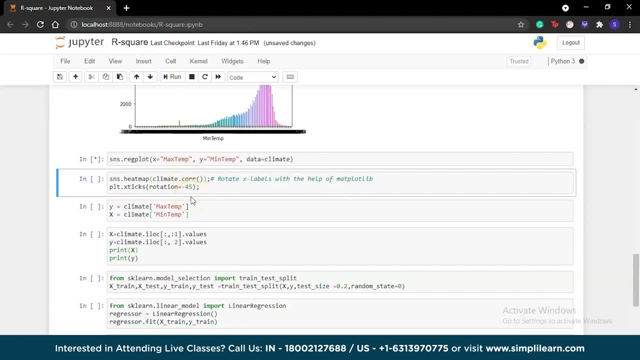 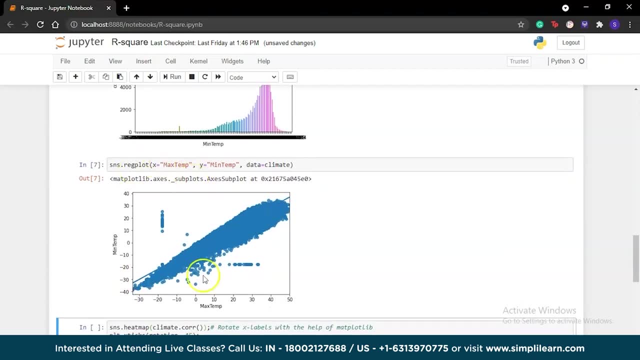 between our maximum and our minimum temperature. So, using the regression plot, we can plot a regression line for the two variables in our x and y axis. So this is our x axis and this is our y axis. This is basically going to plot a straight line which best fits the 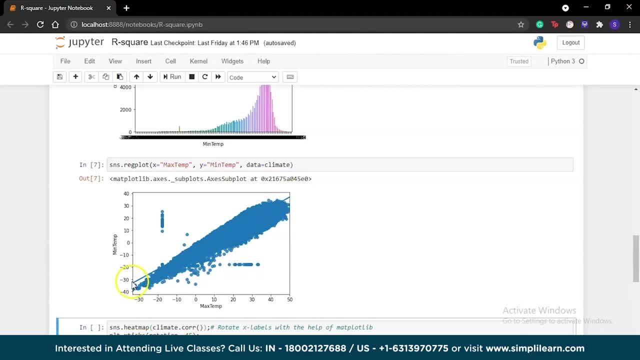 data that we are getting here. So, over here, as you can see, this is our regression line. This thin blue line is our regression line, which intersects our minimum temperature at a value which is between minus 30 and minus 40, and it passes through our entire data. 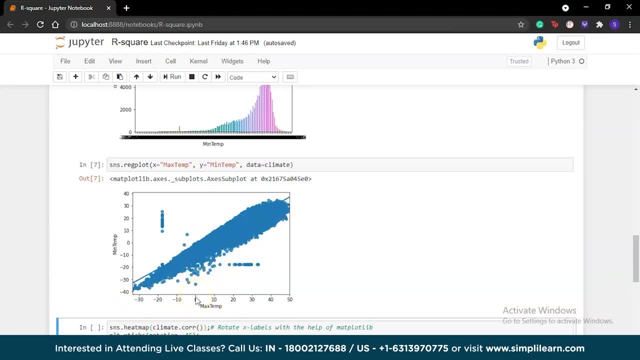 So for a value of maximum temperature which is zero, using this we can predict the minimum temperature that would have occurred on the same day. So for zero, it will be somewhere around minus 10 degree Celsius. So if we sum maximum temperature of zero degrees on that day, we would have seen a. 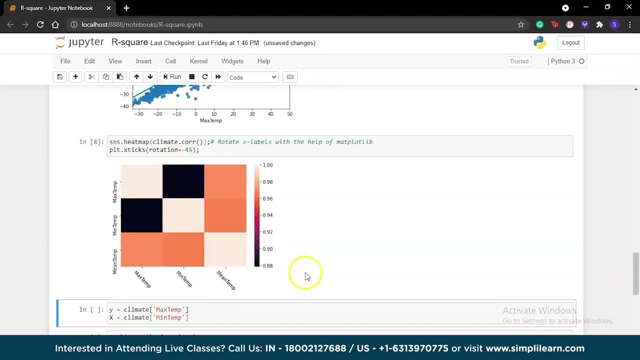 minimum temperature of minus 10 on the same day. Now let's plot a heat map to see how these values are correlated with each other. So the correlation is basically used to find which values affect each other linearly or which values when change will also affect the change in other values. 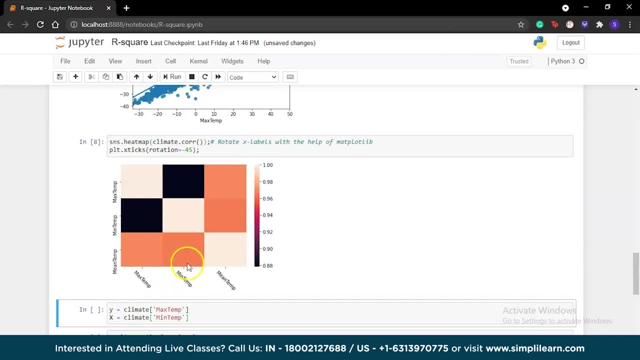 So over here, as you can see, minimum temperature and maximum temperature and maximum temperature have a correlation of 0.88, which means if minimum temperature changes, then the maximum temperature will also change to 0.88. Now the best correlation is obviously going to be between the mean temperatures. 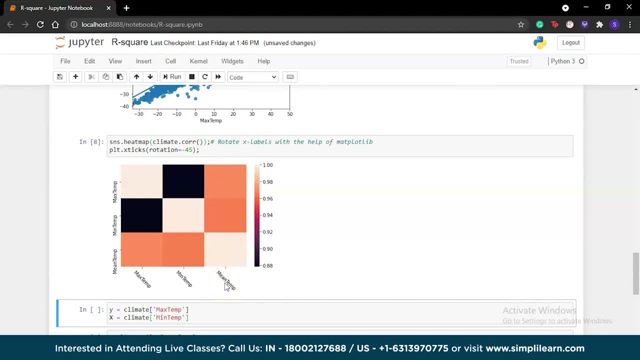 and the minimum and maximum temperatures. The mean temperature is nothing but the average temperature value that we have, So this is basically going to lie in the middle of all of our temperature values, which is why we are going to have a better correlation for mean temperature, but minimum temperature. 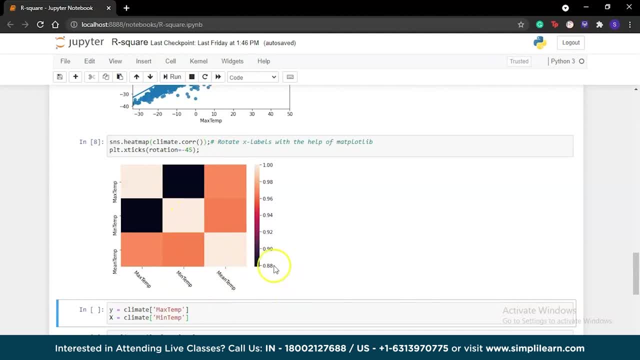 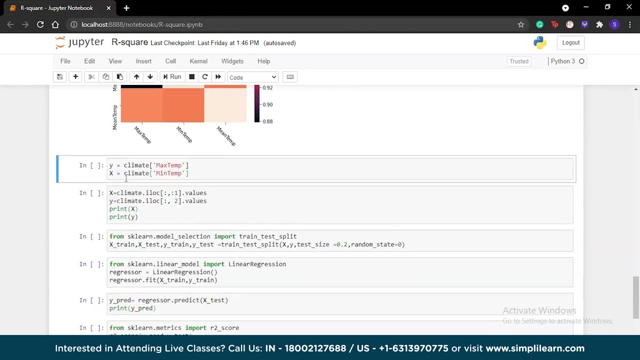 and maximum temperature are also pretty well correlated, with a correlation value of 0.88. This means that if our minimum temperature fluctuates, our maximum temperature will also fluctuate proportionately. Now let's separate our input and output values. We are going to predict the maximum temperature. 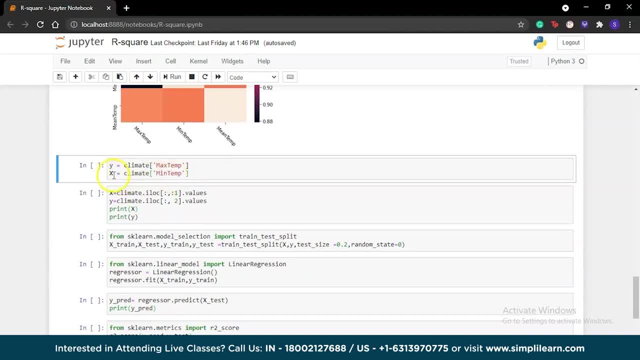 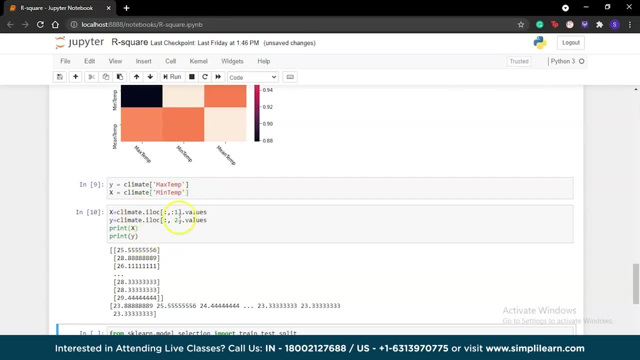 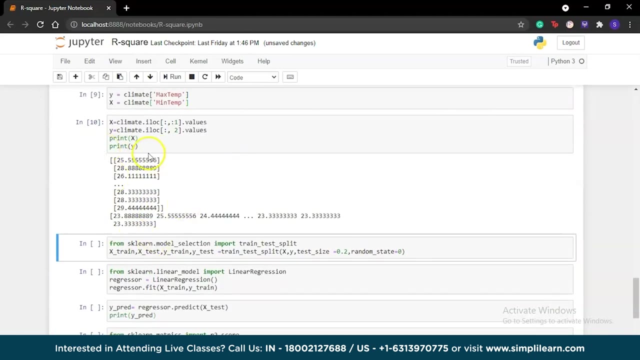 given our minimum temperature. Here, x is our input variable and y is our output variable. So now we are basically just going to get all the important values in our x and y data sets. So after that, this is what our x and y data sets are going to look like. 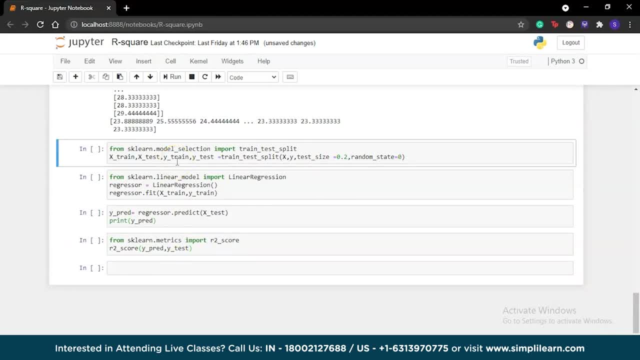 Now let's split our data set into training and testing sets. The training set will be used to train our regression model and the testing set will be used to predict how well our regression model is performing. The training data is the data which will be visible to our model, or the. 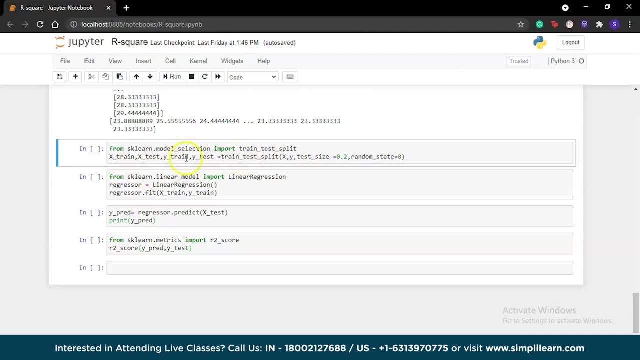 data which our model is allowed to have access to. Testing data will be data which the model has never seen before or which it doesn't have access to, and hence it will be made to work on completely new data to better test how well we've fit it to our data. 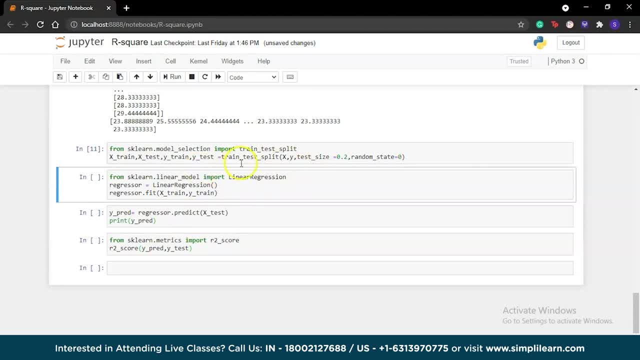 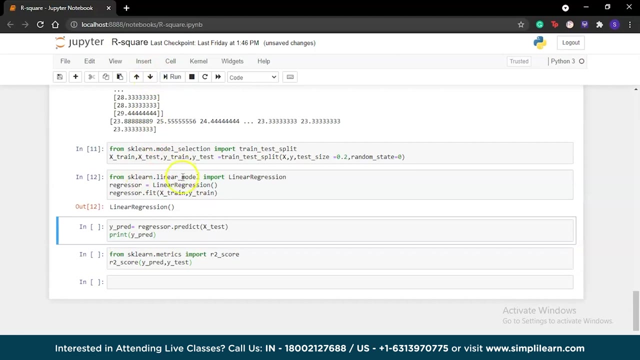 set. Now we can split our data set into training and testing sets by using the train test split functionality from our sklearnmodel selection library. Now, finally, from our scikit-learn library, let's import a linear regression model. We are going to initialize a linear regression model to a 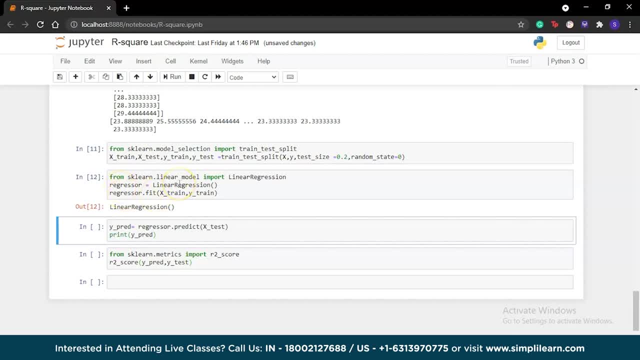 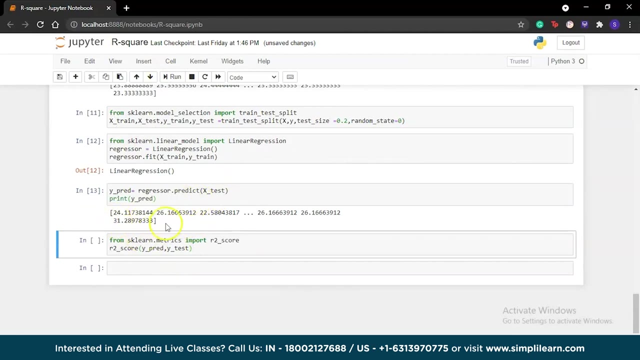 variable called regressor, and then we are going to fit a linear regression model to our training data set. So we finally got a trained linear regression model. Now let's use this model to perform predictions on our testing data set. So these are the values that we've gotten after running. 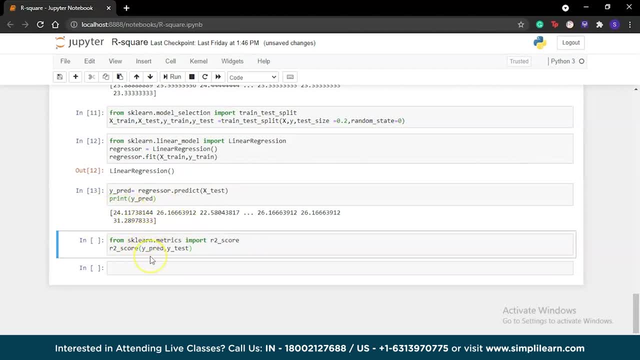 a linear regression model on our testing data set. Let's see how well we've performed. We are going to import the R2 score from our sklearn metric Now. the R2 score will directly perform R squared error on our prediction and testing data set and see how well our 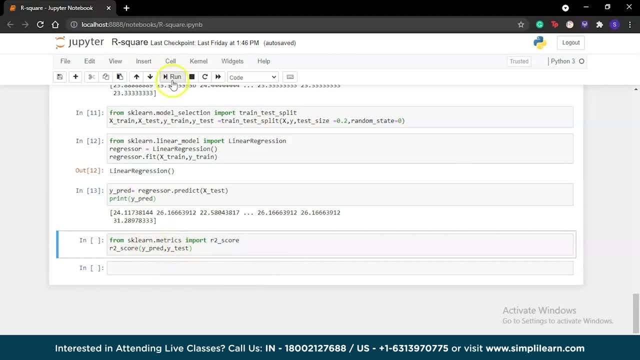 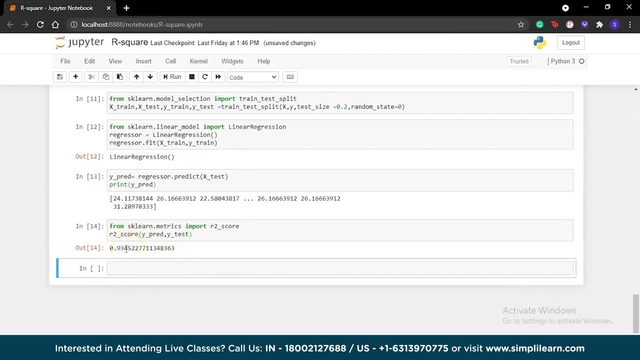 testing data set matches our prediction data set. So now we've gotten an R squared error of 0.9345, which basically means that 93% of our output values are influenced by our input values. This also means that our model is 93% accurate. 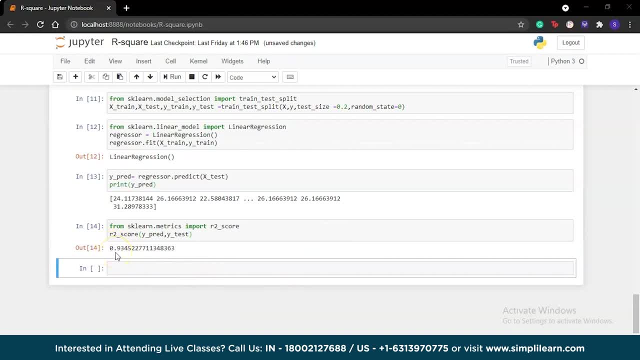 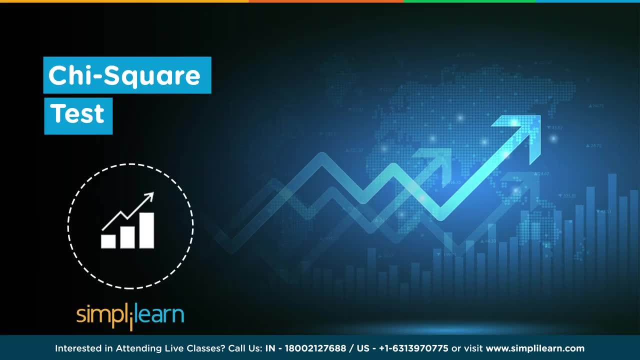 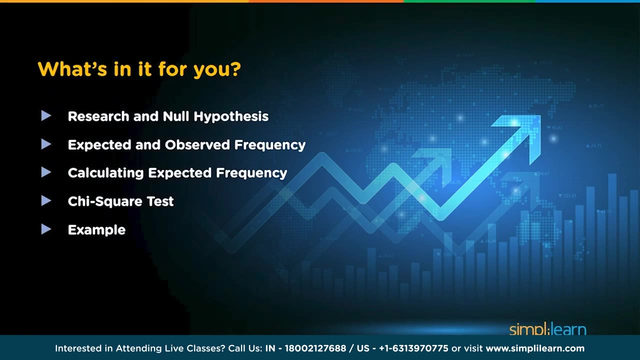 and that approximately 93% of our observed variation can be explained by the model's inputs. We'll be discussing the chi-square test. We'll start by defining what is research and null hypothesis. Then we'll move on to learn about observed and expected frequencies. You'll see how you can calculate. 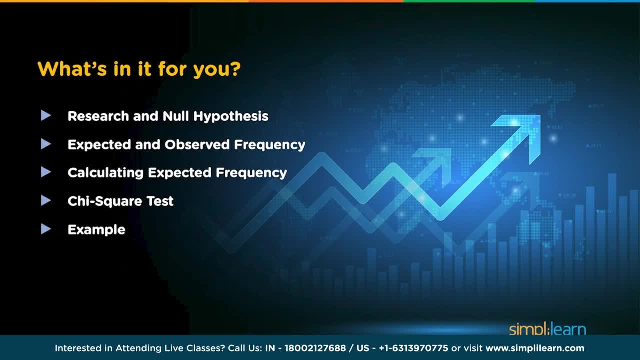 the expected value using a formula. Then we'll move on to chi-square statistics. We'll learn its limitations, its formula and its basic concept. After grasping every theoretical knowledge, we'll discuss an example, step by step, to see how you can calculate the chi-square statistics and the conclusion. 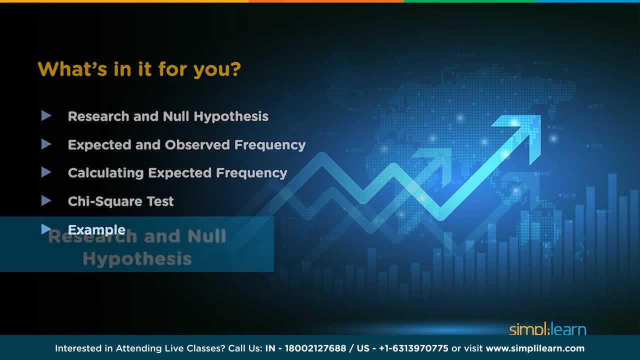 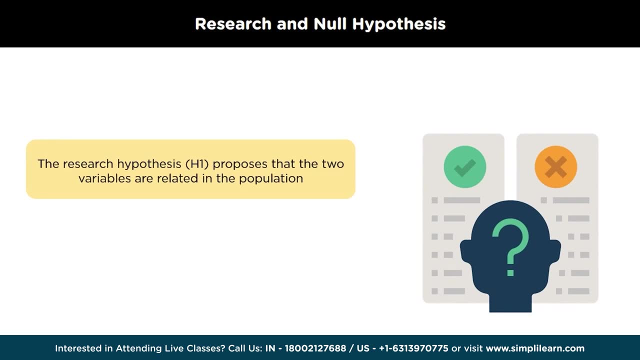 you can draw from the calculated value. So let's get started. Research and Null Hypothesis. The research hypothesis, which is also denoted by H1, says that the two variables are related in the population. The acceptance of the research hypothesis follows the rejection of the null hypothesis. 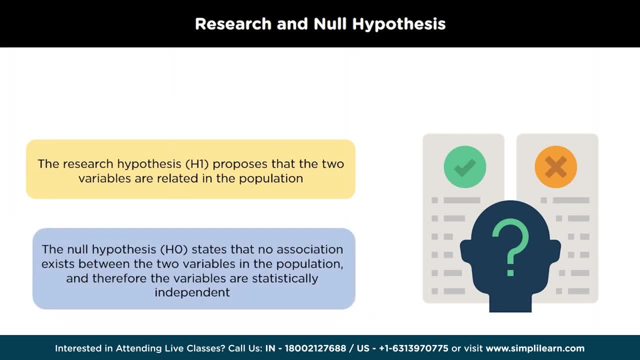 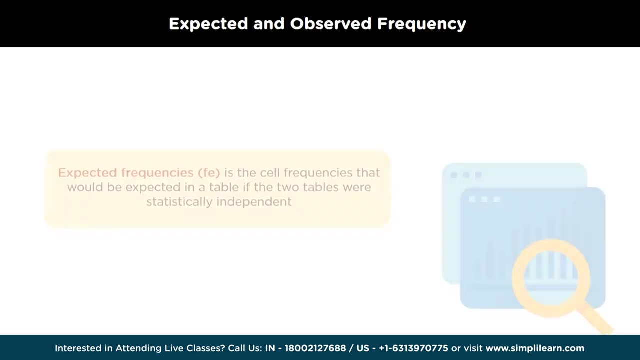 The null hypothesis H0 says that there is no association between the two variables and they are statistically independent. The null hypothesis has no bearing on the study's outcome, unless it is rejected. Now let's define expected and observed frequencies. Expected frequencies are the value that we would get. 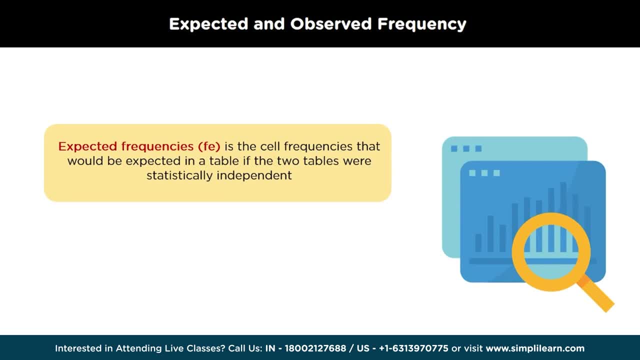 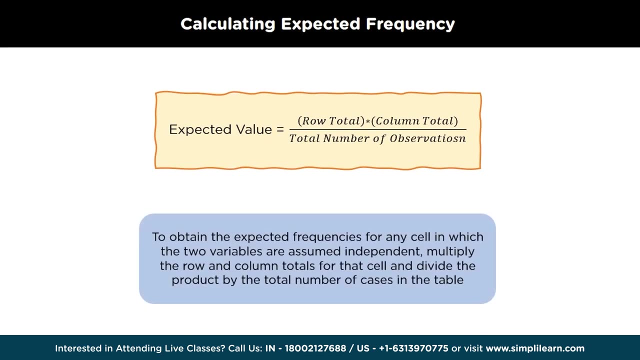 if the two tables were statistically independent. The expected values are calculated based on our null hypothesis. The observed frequencies are those frequencies that we gather ourselves from our observation. To calculate the expected frequency, we have a direct formula: We multiply the row total by the column total and divide the whole value. 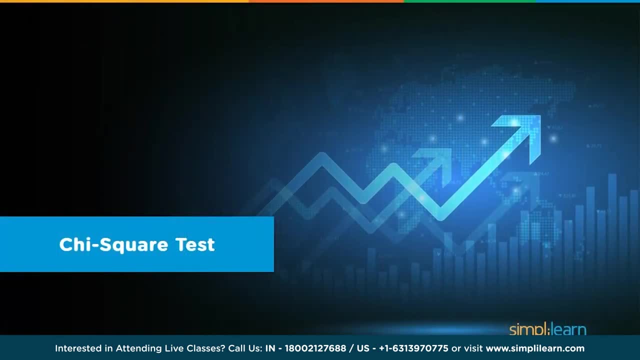 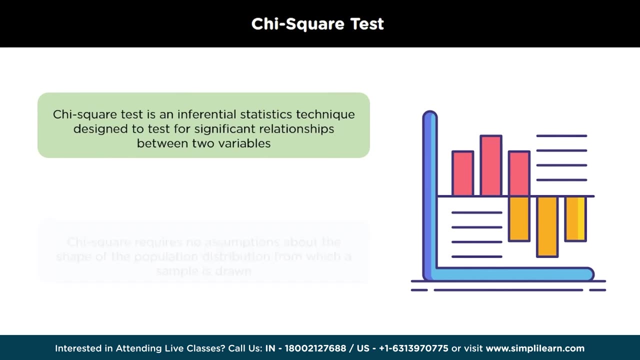 by the total number of observations. Now let's move on to chi-square test. The chi-square test is a statistical procedure for determining the difference between observed and expected data. This test can also be used to determine whether categorical variables in our data are correlated. It helps to find out. 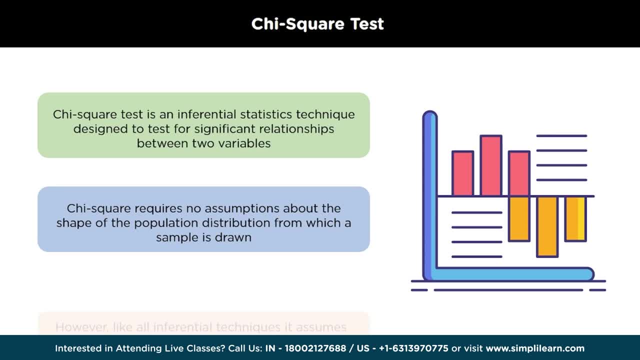 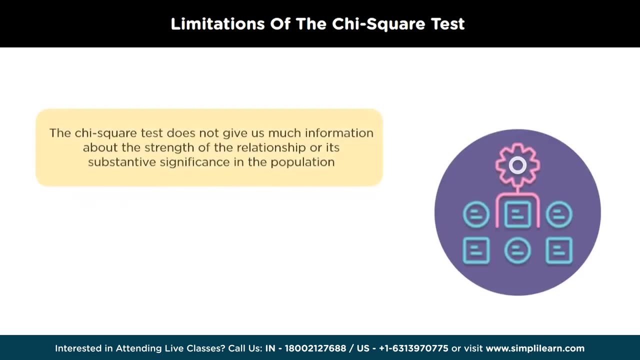 whether a difference between two categorical variables is due to chance or a relationship between them. The chi-square test requires no assumptions about the shape of the population distribution from which the sample is drawn. However, like all inferential techniques, they assume the random sampling. The chi-square test. 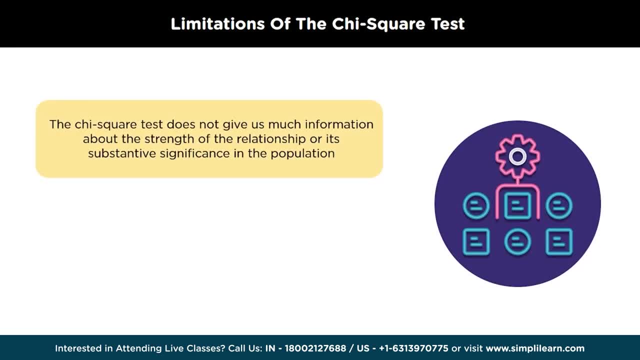 do have some limitations. Firstly, the chi-square test does not give much information about the strength of the relation or its significance in the population. The chi-square test is also sensitive to sample size. The calculated chi-square statistics is directly proportional to the size of the sample. 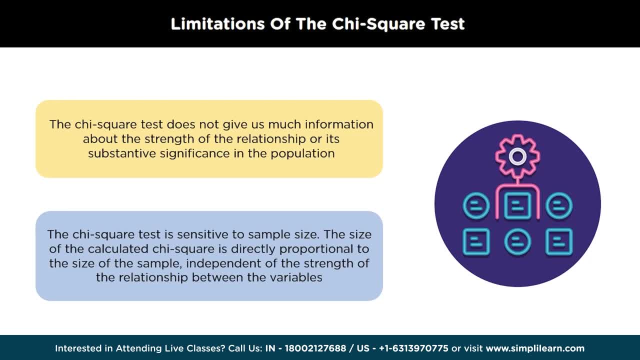 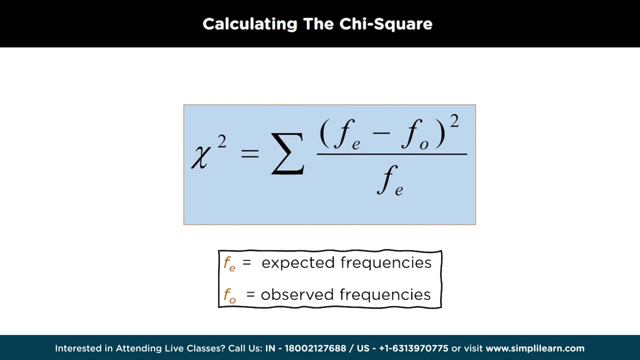 which is independent of the strength of the relation between the variables. So to calculate the chi-square statistics we have a direct formula. The chi-square statistics, which is also denoted by x-square, is equal to summation of expected frequencies minus observed frequencies, whole square divided by expected frequencies. 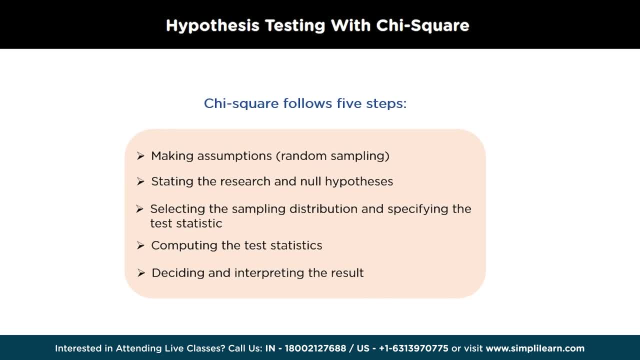 The chi-square test statistics follow five steps. First we make assumptions about random sampling and state its research and null hypothesis. Then we select the sampling distribution and specify the test statistics. and after that we compute the test statistics. The value we get is used to decide and interpret the results. 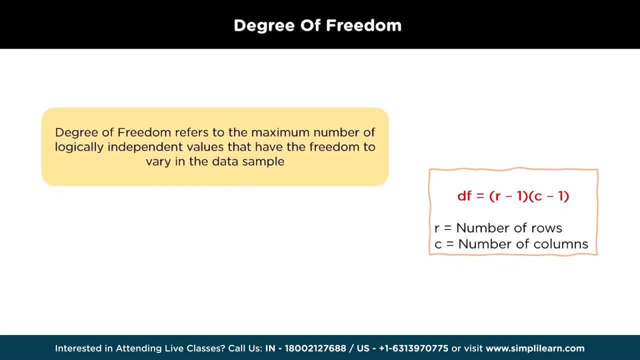 Degree of freedom. The degree of freedom is a statistical calculation which represents the number of variables that can vary. in a calculation, The degree of freedom can be calculated to ensure that the chi-square tests are statistically valid. These tests are frequently used to compare observed data with the data that would be expected. 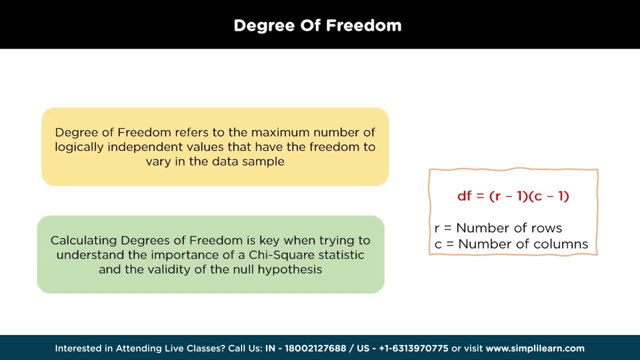 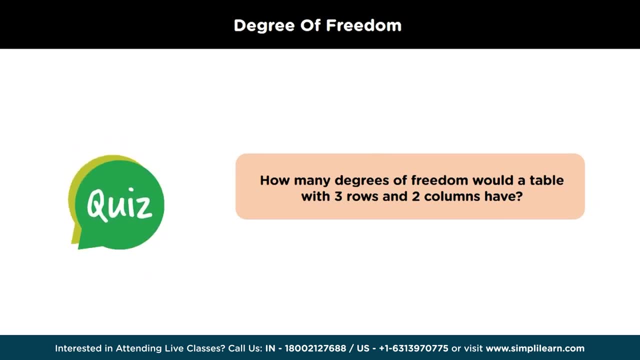 to be obtained if a particular hypothesis were true. The formula to calculate the degree of freedom is number of rows minus one multiplied by number of columns minus one. So, after knowing the formula, we have a question for you: How many degree of freedom would a table with three rows and two columns would have? 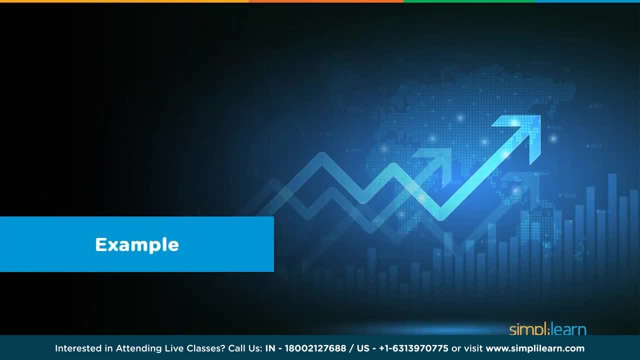 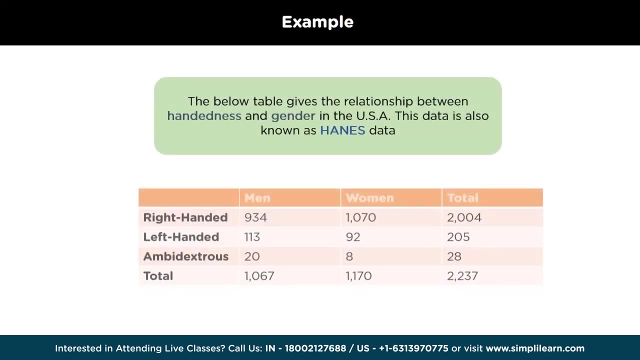 Post your answers in the comment section. Now that we have learnt all the theoretical concepts regarding chi-square tests, Let's understand this more clearly with the help of an example. Let's say we want to know if the gender has anything to do with hand-handedness. We have the data of 2237 people. 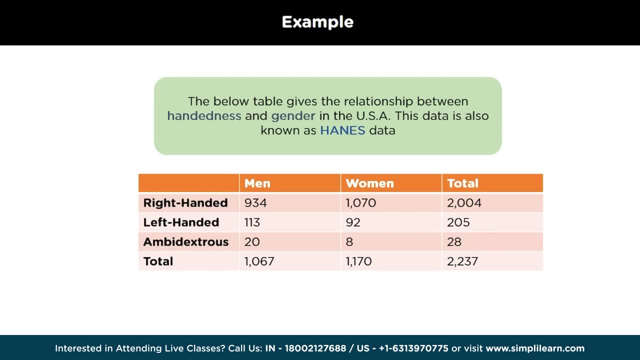 in a simple random sample to find out if they are left-handed, right-handed or both. The results of the survey are shown in the table below. To see if the gender is linked to hand-handedness, we perform a chi-square test. The first step is to define the null hypothesis. 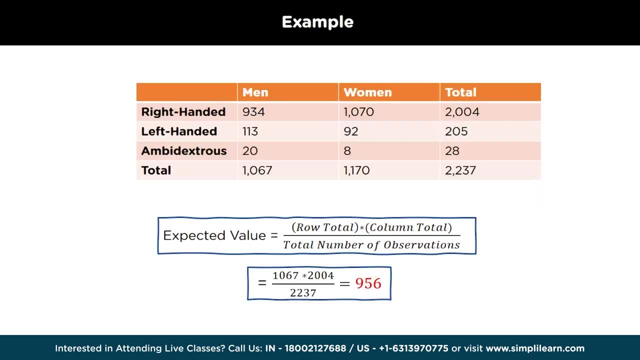 The null hypothesis says that the gender and hand-handedness are independent to each other. The next step is to calculate the expected values, which is row total into column total divided by the total number of observations. For example, the expected value of a right-handed man can be calculated. 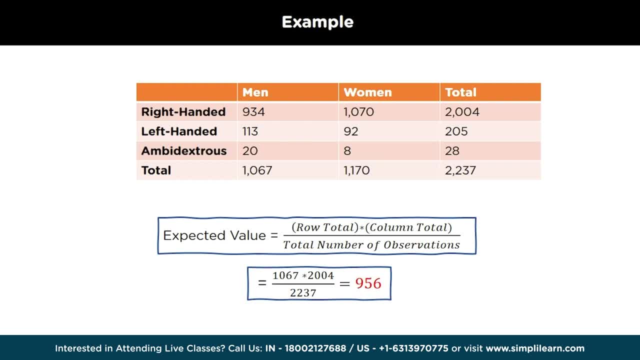 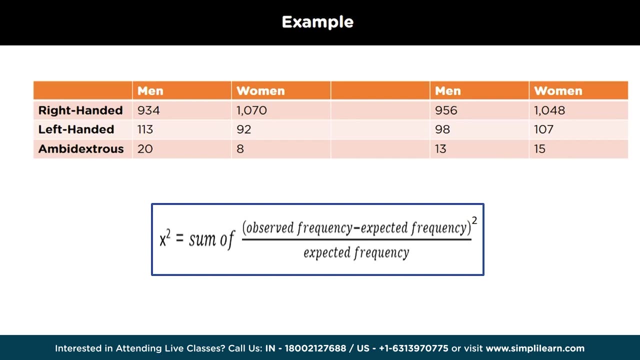 by multiplying 1067 into 2004, divided by 2237, which comes out to be 956. In a similar manner, you can calculate the expected value for each of the cell. After calculating the expected value, we calculate the value of x-square. x-square is calculated by. 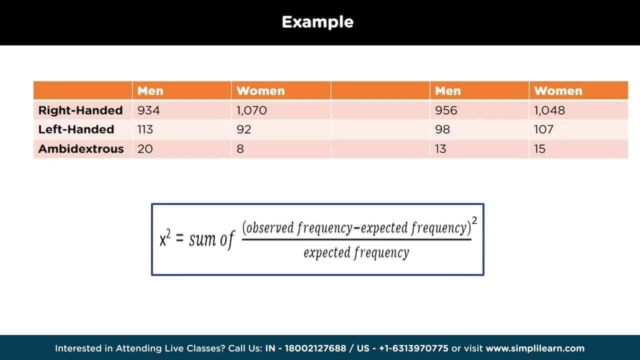 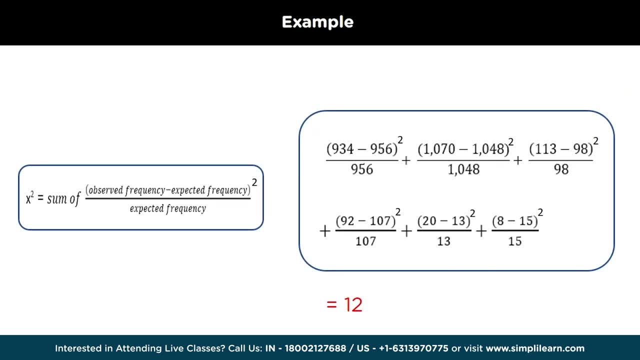 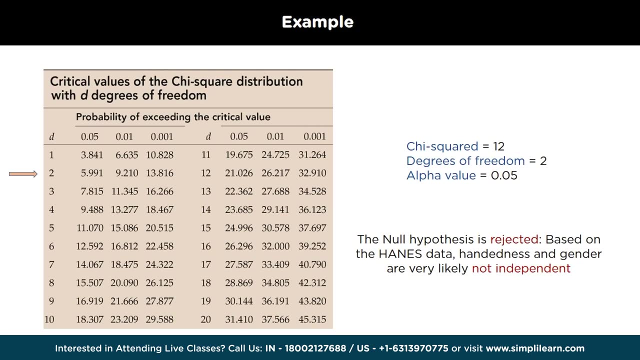 the following formula: observed frequency minus expected frequency, whole square divided by expected frequency. So by putting the values in the formula, we get the x-square value to be 12. Now we got our x-square, which is chi-square value, to be 12 and the degree of freedom is equal to 2. 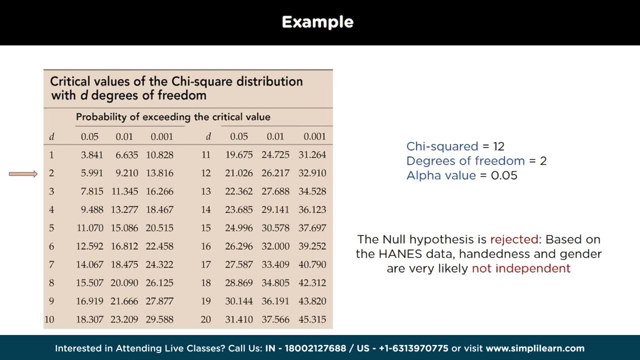 which is calculated by R-1 into C-1. where R and C were rows and columns respectively, The alpha value was assumed to be 0.05. We compare our chi-square value with the critical values of the chi-square distribution with the degree of freedom. 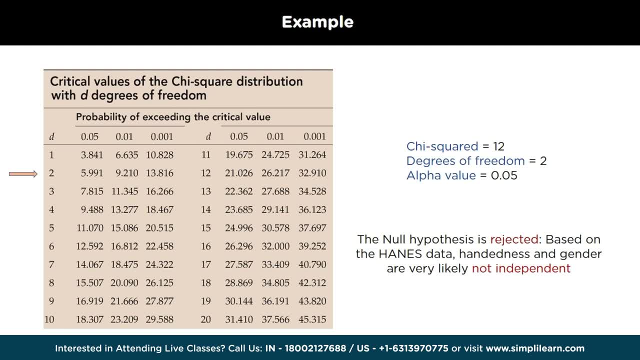 So for degree of freedom 2 and alpha level 0.05, the value was 5.991, which was lower than our chi-square value. This states that handedness and gender are not very likely to be independent. Simply Learn's post graduate program in data science offered by 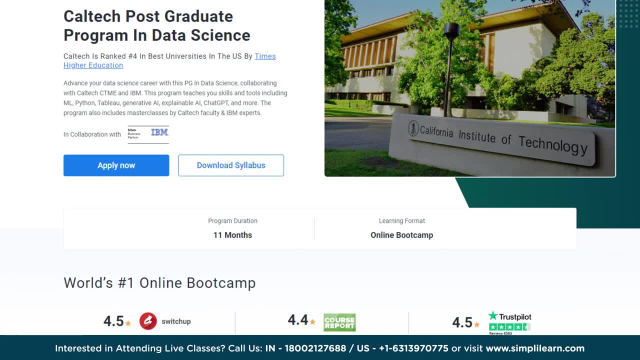 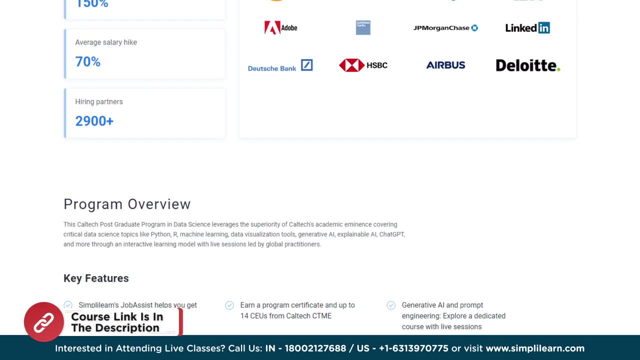 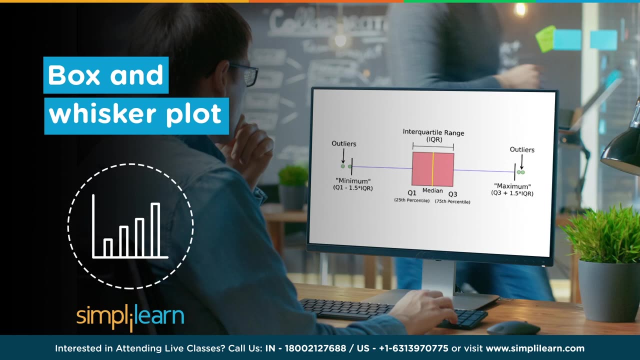 Caltech University, in collaboration with IBM, is just what you need. For more details, head straight to our homepage and search for data science post graduate program, or simply click on the link in the description box below. As you know, the graphic visualization of data constitutes a discipline within the data science universe. 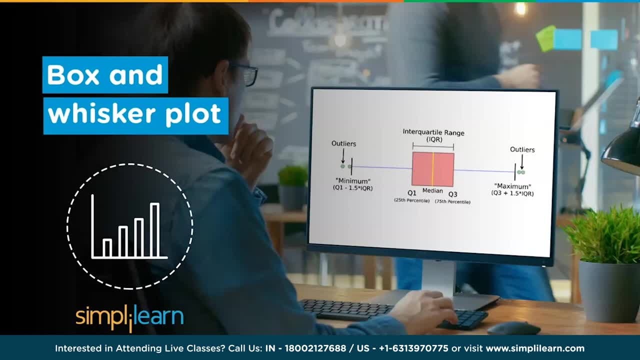 This practice has become an important milestone throughout the history in data analytics, So, keeping that in mind, in this video we are going to discuss an important graph that is a Bosc and a Risco plot. But before we begin, if you love watching tech videos, 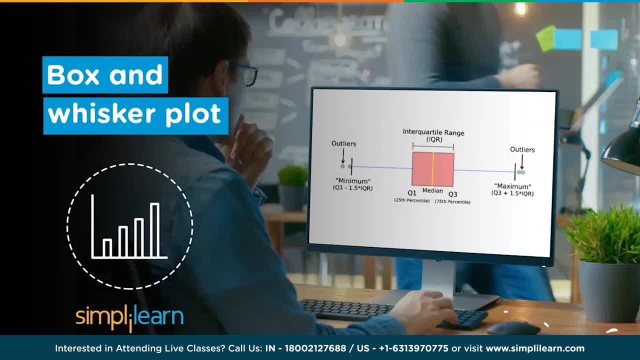 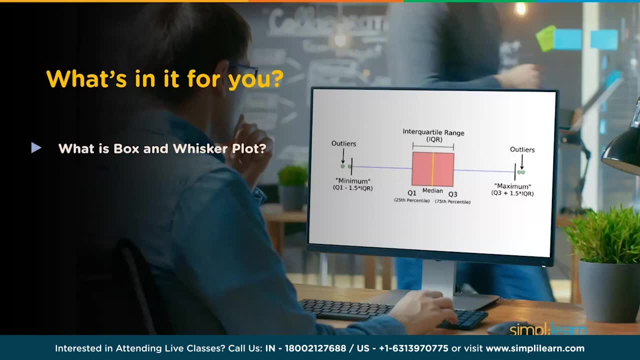 subscribe to our channel and hit the bell icon to never miss an update. So let's discuss the agenda for this tutorial. We'll begin this video by discussing what is Bosc and Risco plot and some important terms involved with the Bosc and Risco plot. 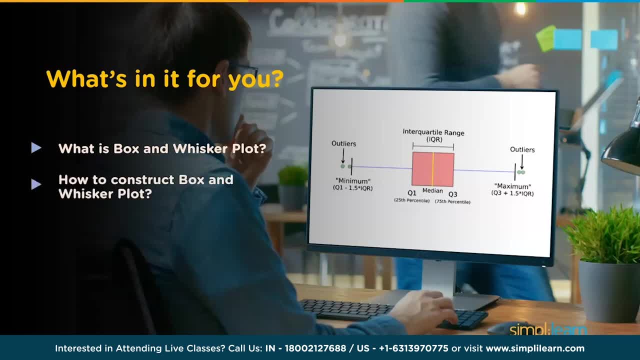 After this, we'll look into the way in which you can construct a Bosc and a Risco plot by taking an example. After this, we'll move on to the python and see how you can create a Bosc and a Risco plot. So, without further ado. 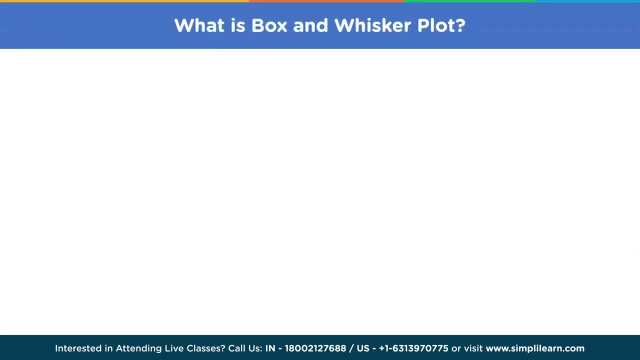 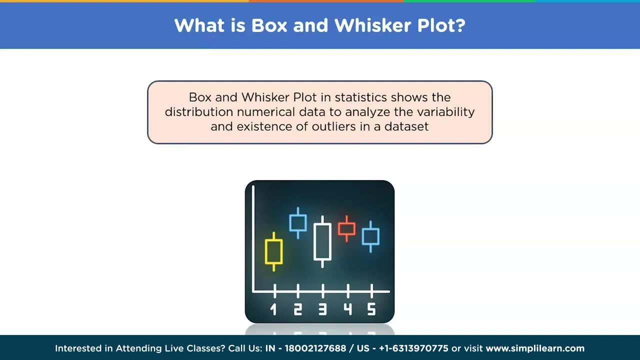 let's get started. So what are Bosc and Risco plot? A Bosc and a Risco plot is a graphical representation of variation in a set of data. A histogram analysis is usually sufficient, but a Bosc and a Risco plot can add more detail. 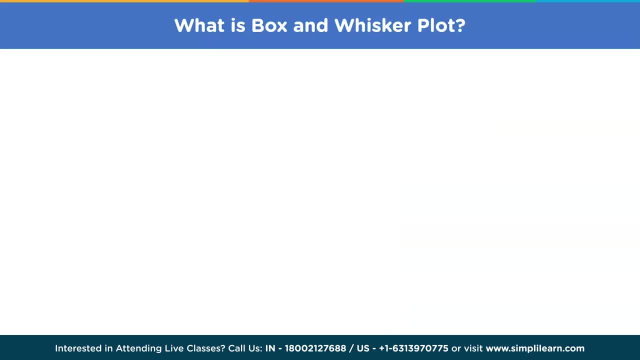 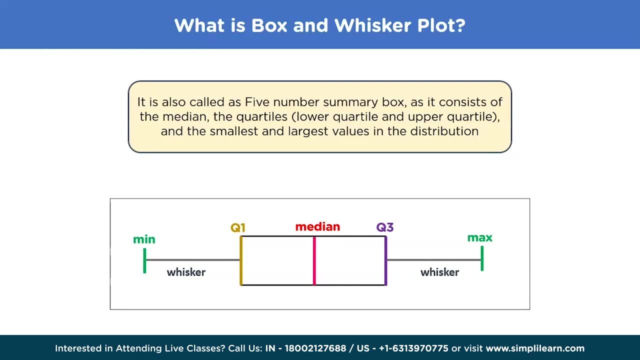 while also allowing multiple sets of data to be displayed in the same graph. Let us understand the terms involved here. So the first one is the minimum value, which is the smallest value in the data set. The Q1,, which is the lower quartile, is the value below which the lower 25%. 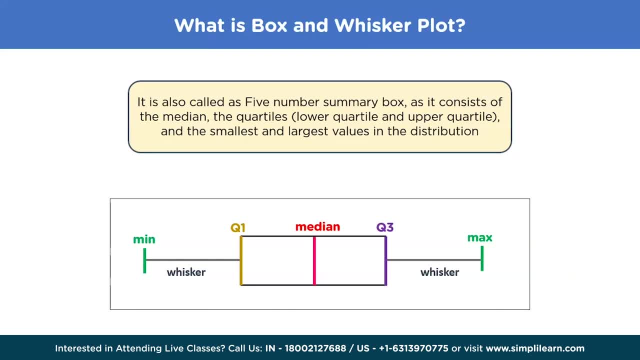 of the data are contained. The median value is the middle number in a range of numbers, and the third quartile is the value above which the upper 25% of the data are contained and, at last, the maximum value, which is the largest value in the data set. 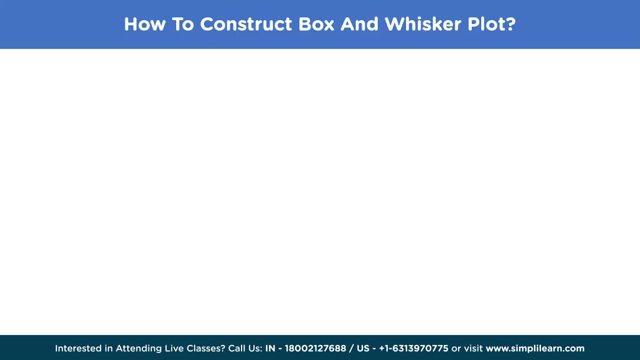 Now that we know about what is Bosc and Risco plots and the key terms that are required to construct a plot, let's move on to an example to see how you can construct a plot in a systematic manner. Here we have a sample age of 10 students. 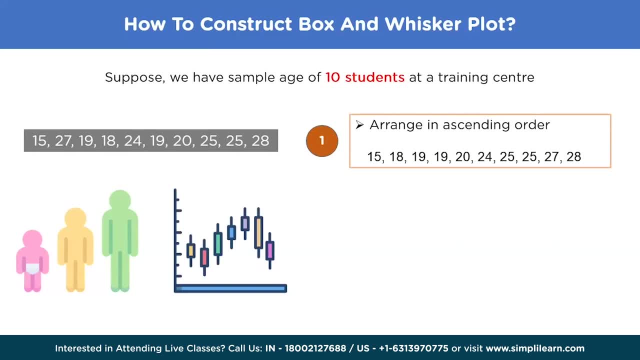 at the training center. So the first step would be to arrange the data in the ascending order of the data set. Since there are even number of terms, we will find the average of the middle two terms to find the average of the data set. So adding 20 plus 24 and dividing it by 2. 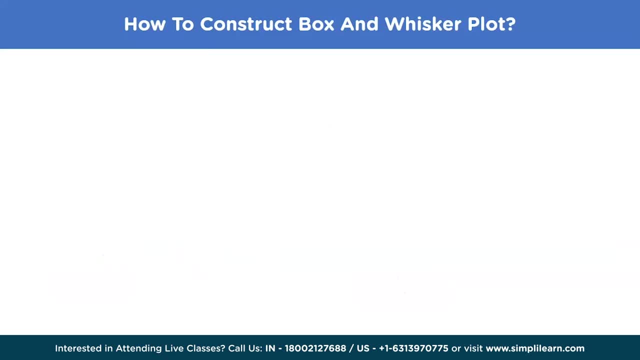 we get the average as 22, which is also the median of our data set. Now that we have find our median of the data set, let's move on to the next step. So the next step is to find the median of the lower half and the upper half. 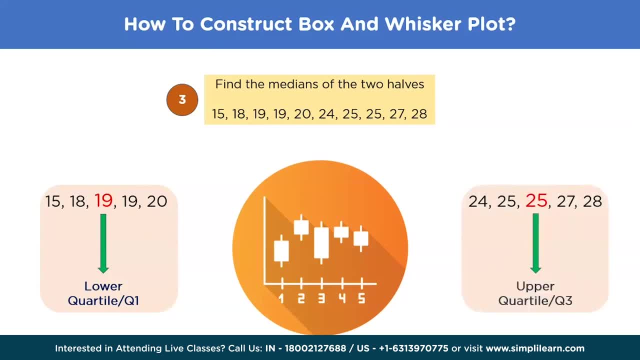 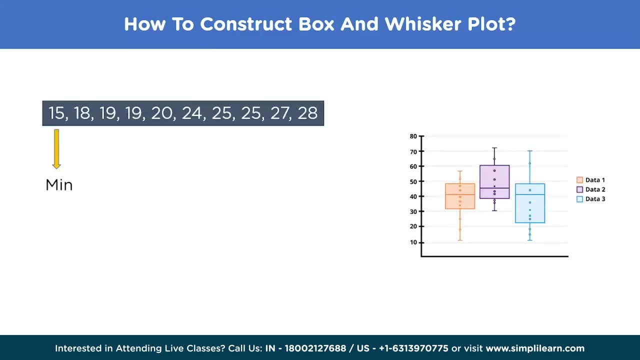 The lower half median is 19, which is also the Q1 of the data set, and the upper half median is 25. So our five number summary will look like this: The minimum value is 15, The Q1 is 19, The median, which is also the Q2, is 22. 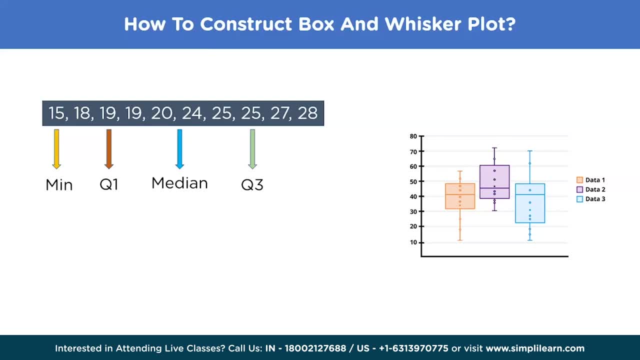 and the upper half median is 25, and finally the maximum value, which is 28. Now we have all the required values to make a box plot, So let's go ahead and create one. So to create the box plot, the first step would be to make a number line. 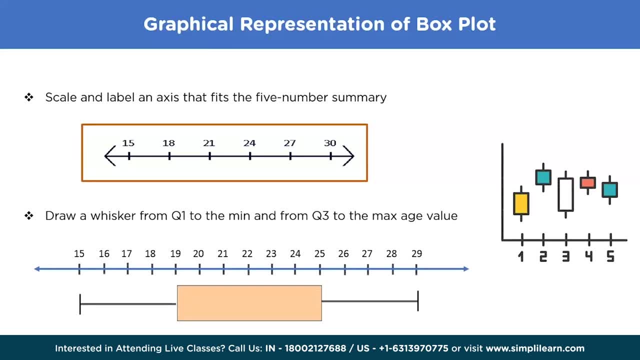 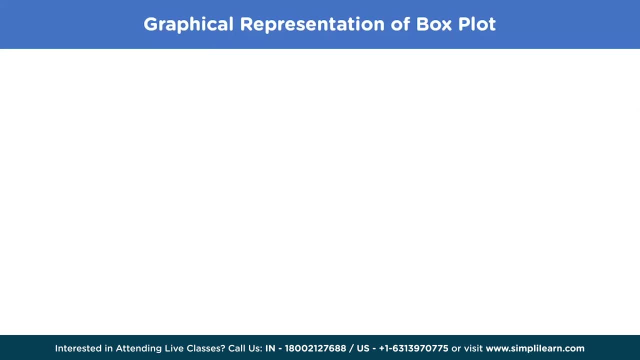 with a proper scaling. After this, we just have to draw the whisker to the minimum and Q3 to the maximum age value. Now that we have created the box plot, let's understand what these values actually mean. So the lowest age among the students at the training center is 15. 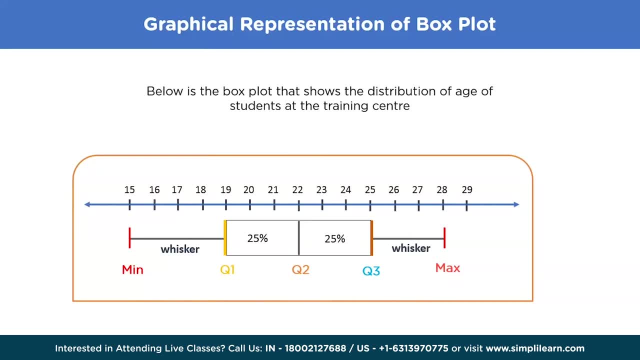 excluding the outliers, About 25% of the students are under 19 years of age and close to 50% of the students are between 19 and 25 years of age. Nearly 75% of the students have an age less than 25 and the maximum age among the students is 28. 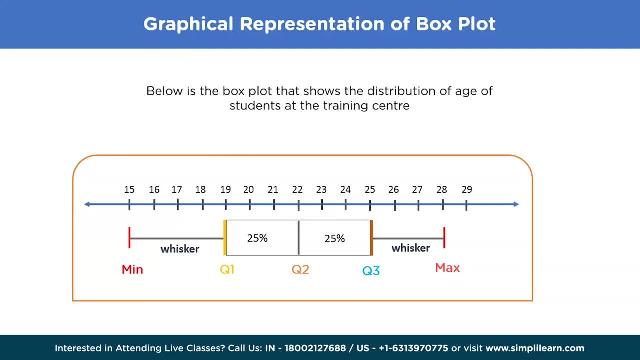 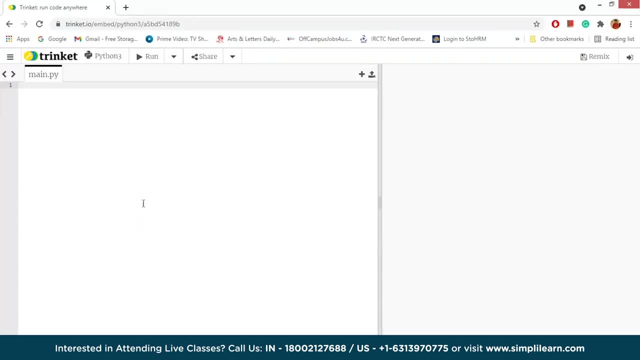 excluding outliers. Now that we know how to create a box plot, let's move on to python compiler to see how you can create a box plot using a matplot and a numpy library. So here I am on an online compiler. So let's start by importing. 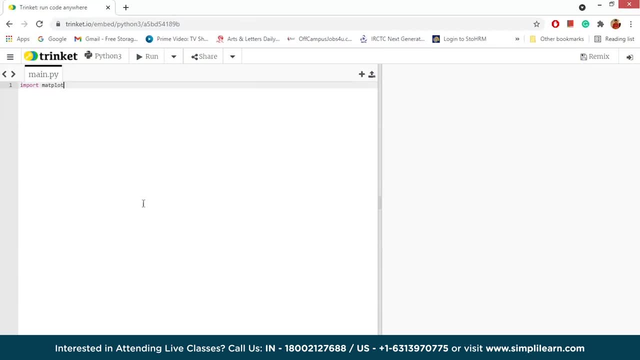 matplotlib and a numpy library. matplot as plot, import, numpy as np. Now that we have imported both the libraries, let's generate some random numbers. For that we will use the function random nprandom and we will name it randomIntegers. So the first value we are going to enter. 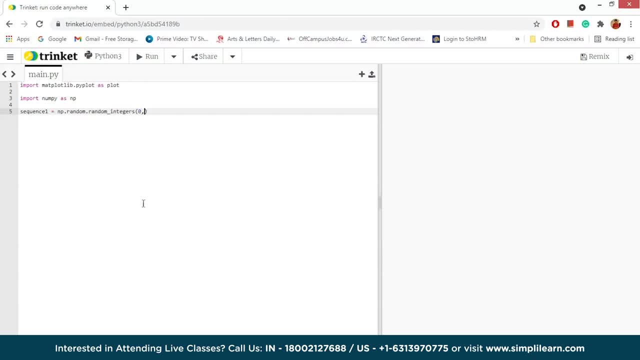 is the lowest value a dataset can have, So 0- The 100 will be the maximum value we can have, and there should be 100 terms in our dataset. Now To make a box plot, just use the plotboxplot function and pass it to sequence. 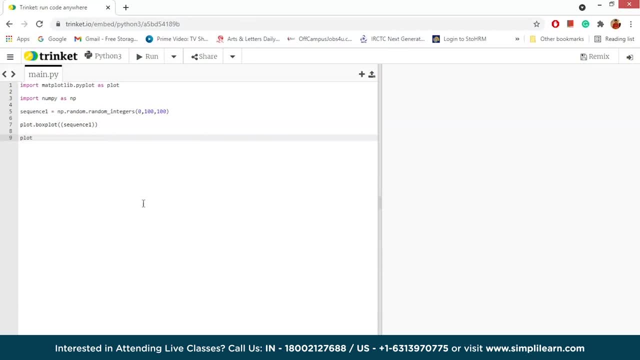 Make sure you spell it right Now. To get the graph, use plotshow Now. just run it. You can see we have a box plot ready. So in this way you can create a box plot in a python To simply learn. Bias and variance are important part of 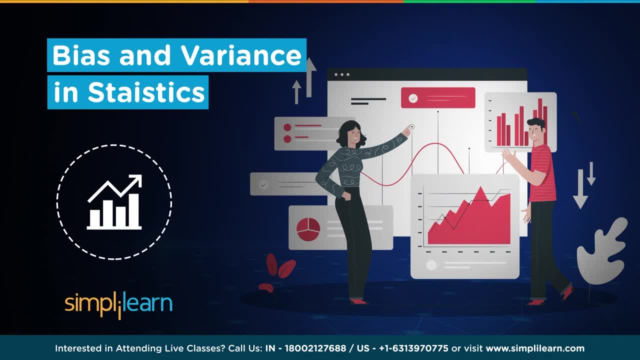 statistical analysis and is used in several places, such as research, machine learning, data science, data analytics and many more. It has a wide range of applications. So in this video we will discuss what is bias and variance and we will try to understand it with the help of an example. 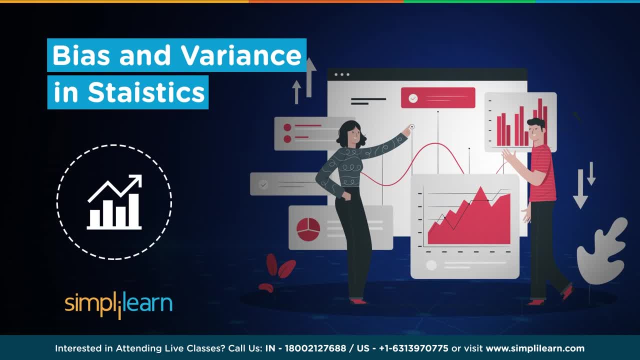 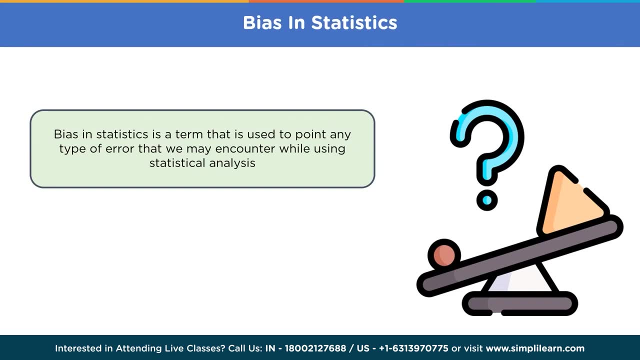 So, without further delay, let's move ahead. What is bias in statistics? What is bias in statistics? What is bias in statistics? Bias in statistics is a term that is used to refer any type of error that we may find when we use the statistical analysis. 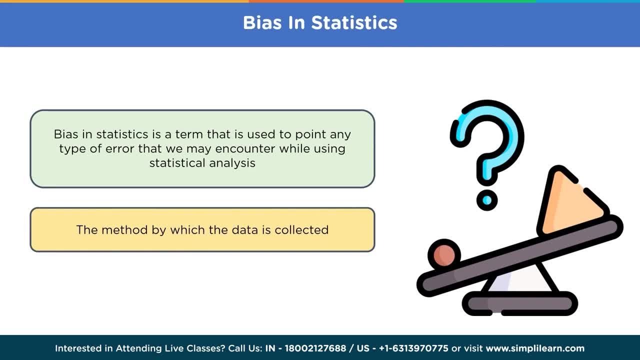 We can say that it is an estimator of a parameter. that may not be confusing with its degree of precision. The reasons for this bias may be that the method by which the data is collected may be faulty or the question is phrased may be not accurate. 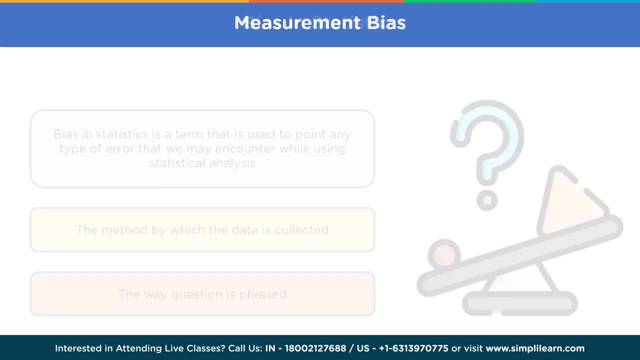 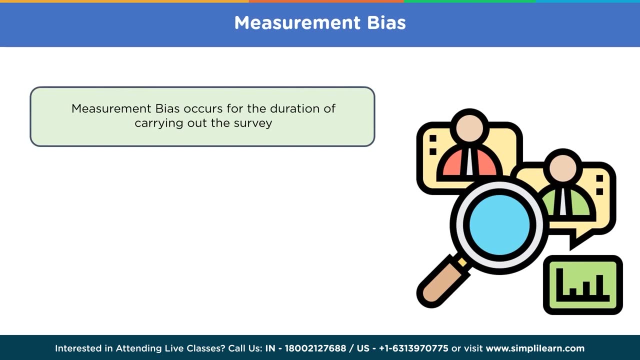 Let's see what are the types of biases. The first one is the measurement bias. Measurement bias refers to any systematic or non-random error type that occurs in the collection of data in a study. Another term that is used for this type of bias is the detection bias. 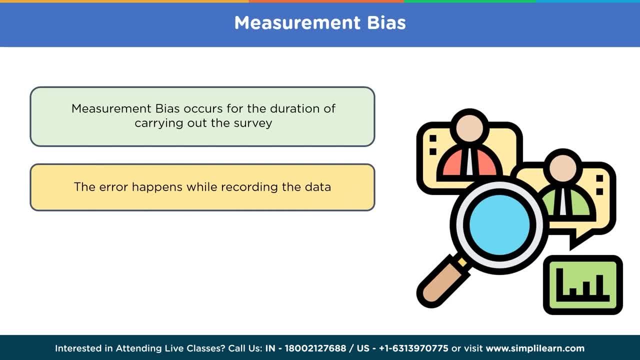 This difference in observation might be because of an unseen reason. Some of them can be the error that happens while recording the data or the leading questions that follows after the data. The error can also occur because the respondents gave the false answers. Suppose you conduct a survey to determine whether or not someone voted. 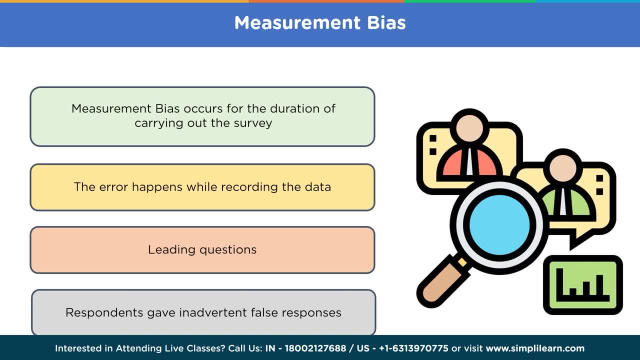 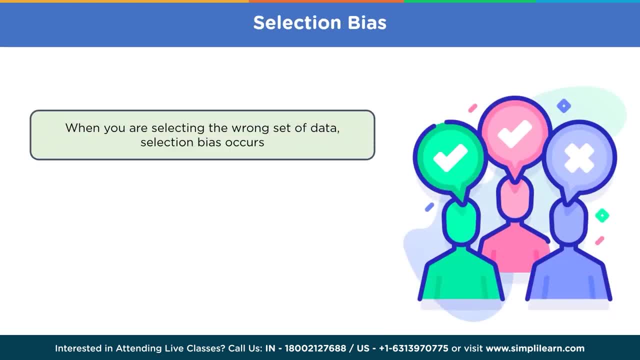 for President Obama. Some may have voted for him, but the way the question was put confused the respondents and they answered wrong. In this case, the measurement bias can occur. The next type of bias is the selection bias. When you choose your sample or data incorrectly, selection bias occurs. 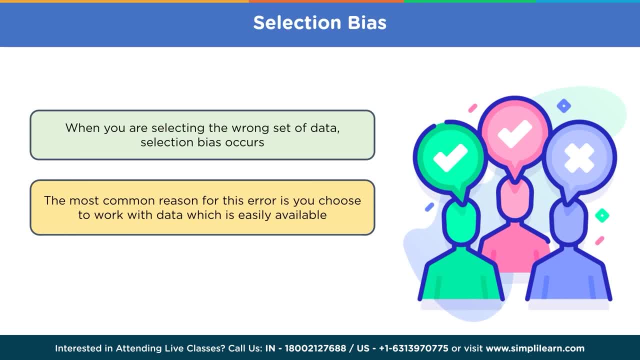 There can be many reasons for this, but the most common reason is that people try to work with the data that are easily available, and because of that, the respondents gave the false response. Let's try to understand this concept with the help of an example. Suppose you are conducting a poll. 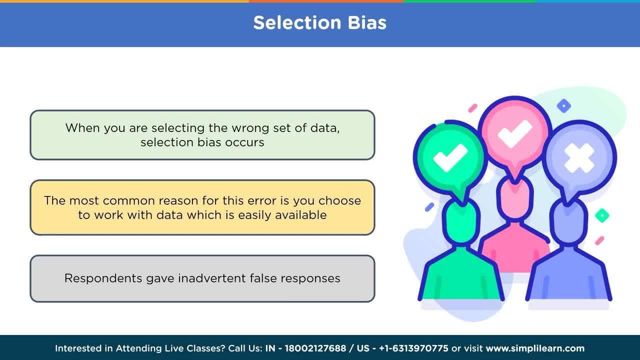 to determine how people feel about the current ruling government. You have gathered all the information that you need. Unfortunately, many of them say that Twitter is the primary source for the information. Now, social media is not considered trustworthy because it is in public opinion, but their friends' opinion. 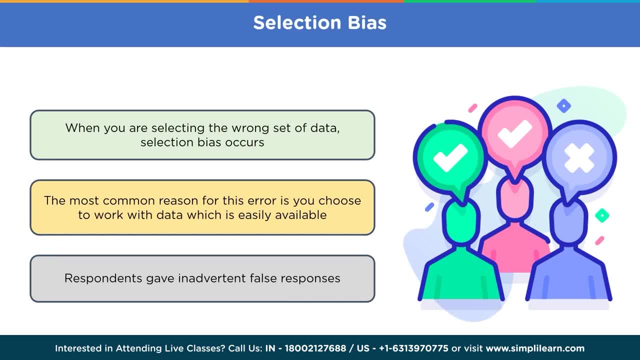 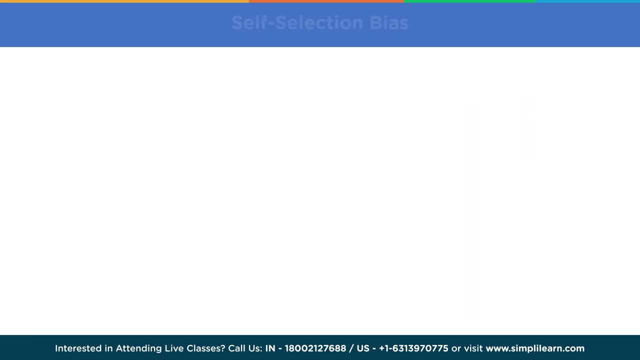 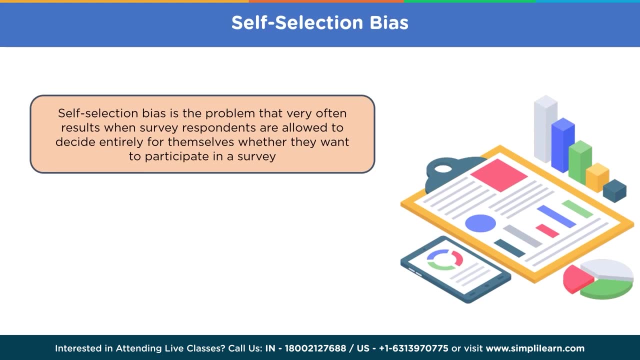 As a result, this type of data can be classified as a traditional selection bias, easily accessible, but not for unrepresentative and specific subsets of the overall population. The next type of bias is the self-selection bias. Self-selection bias occurs when the respondents are allowed to decide entirely. 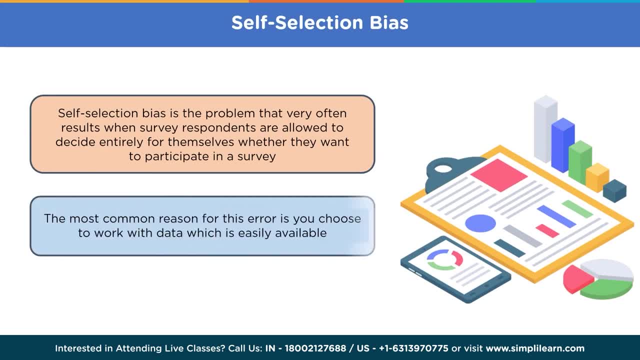 for themselves whether they want to participate in the survey or not. The reasons for this error may be same: that the data may be collected which are easily available. Let's try to understand this type of bias with the help of an example. Suppose you want to assess a program. 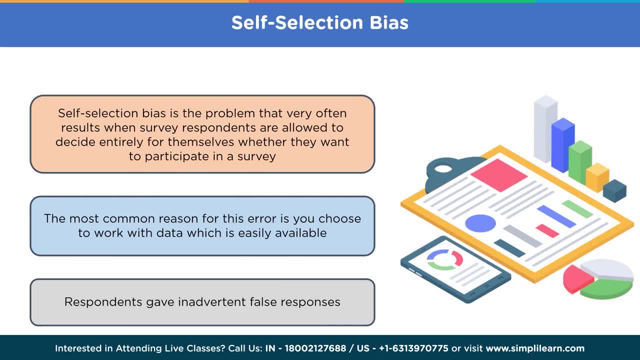 for improving the eating habits of the shift workers. You put up posters where many workers nice shifts and invite them to participate. However, those who sign up may be different from those who don't. They may be more health-conscious to be with, which is why they are interested in a program. 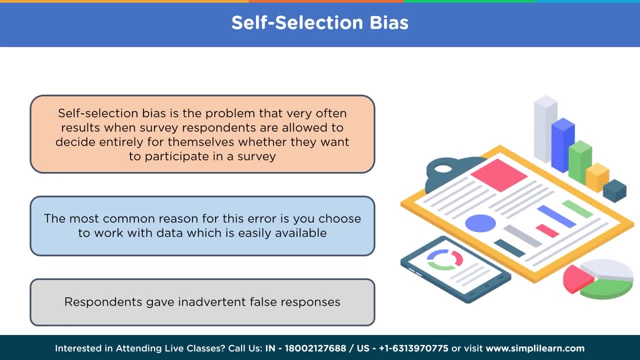 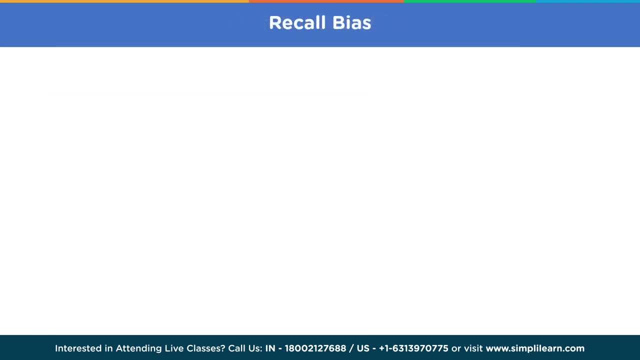 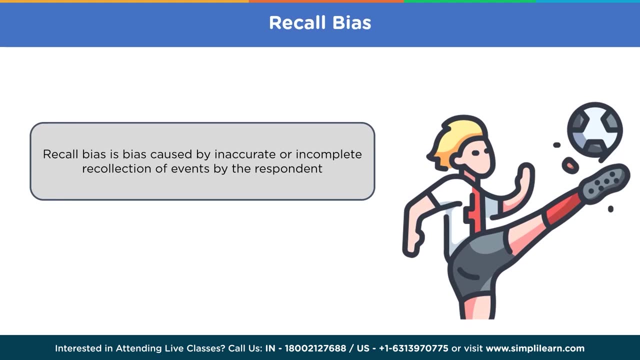 for improving eating habits. If this was the case, it wouldn't be fair to conclude that a program was effective or not. In this case, a self-selection bias occurs. Recall that. Recall bias occurs when respondents' recollection of events is inaccurate or incomplete. It's especially problematic. 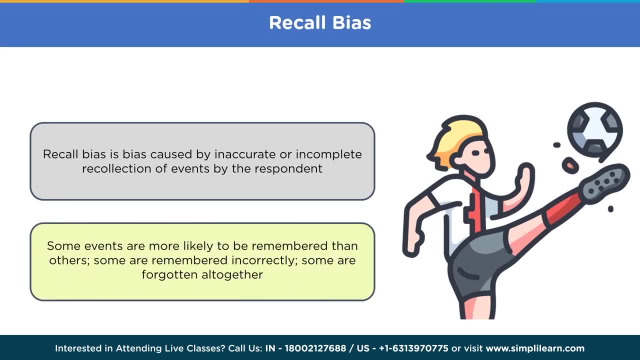 when it comes to retrospective survey questions. For example, Suppose you are asked for a football match that happened 3 years back Now. you may remember the goals and the good moments of the football match, but might not be able to recall the bad moments or the fouls or the mistakes. 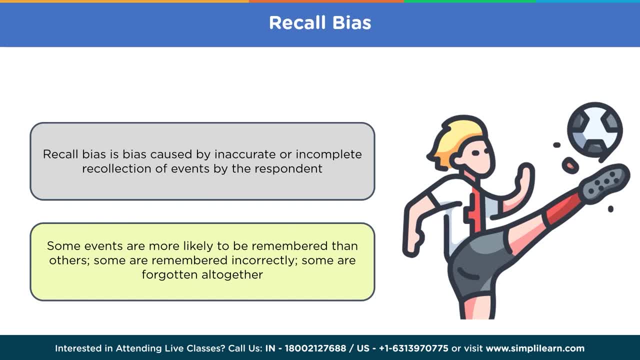 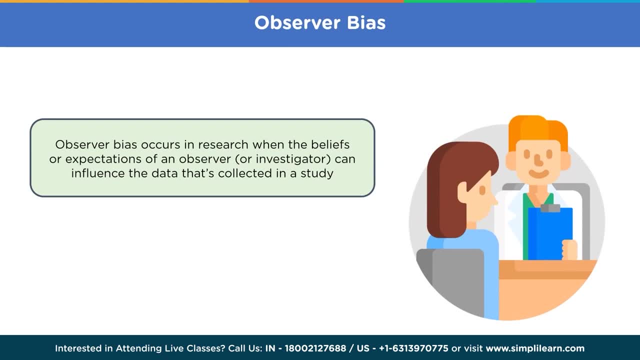 that happened in that match. So if you try to guess work here, In this case a recall bias can occur. Another one is the observer bias. When a researcher subconsciously projects their expectation onto the research, this is known as the observer bias. In this case, 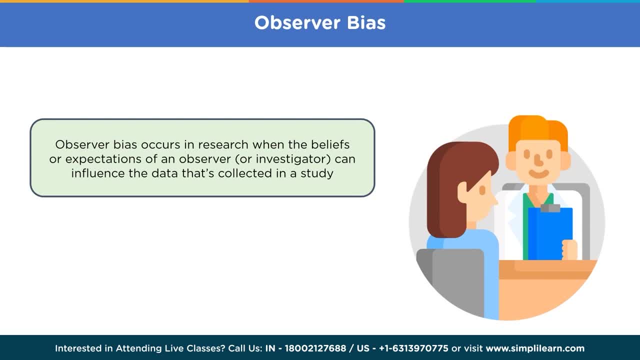 the beliefs or expectations of an observer can influence the data that is collected for the study. Let's try to understand this observer bias with the help of an example. Suppose there is a certain news channel. Now in the race of TRP, certain news might not be accurate. 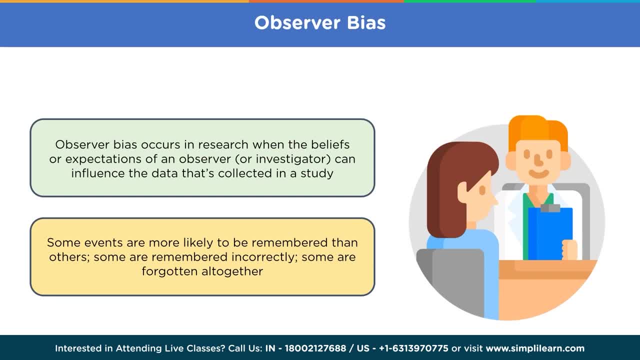 or may be even false, but to prove his point, he may try to prove that this news is correct and the data that are given are accurate. In this case, the observer, which is the news channel, is trying to force his opinion on the data and in this case the observer- bias can occur. 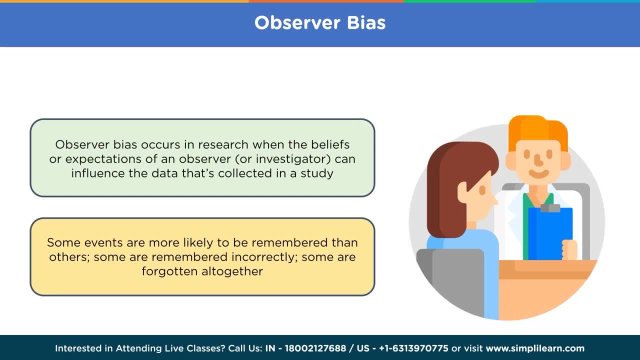 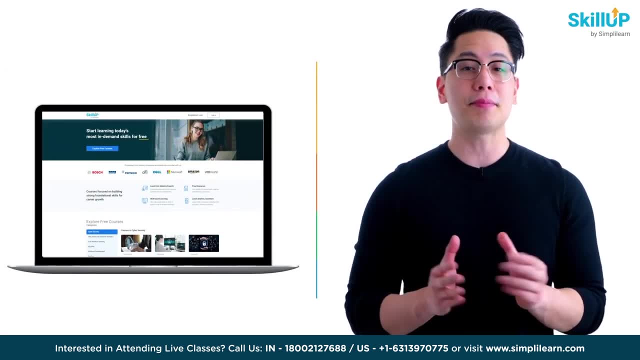 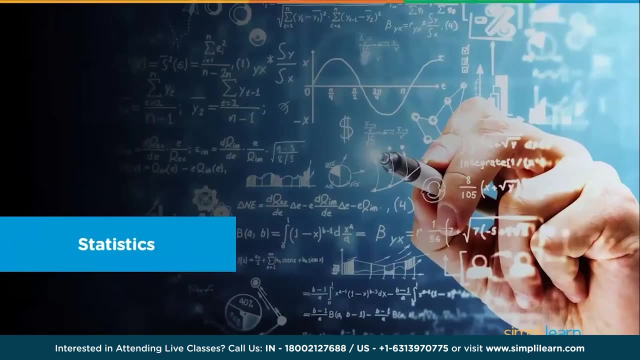 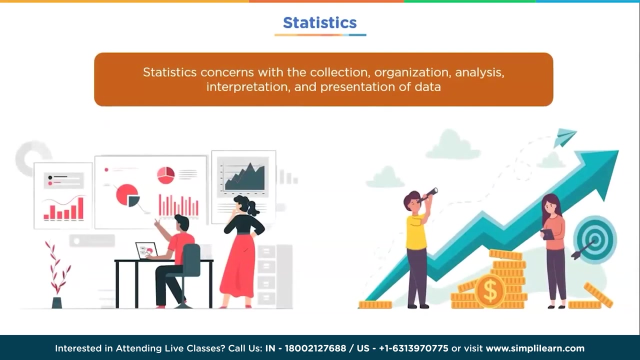 So with this we have discussed all the types of biases with the help of an example. So what is statistics? Statistics is a science concerned with developing and studying methods for collecting, analyzing and interpreting the empirical data. Statistics is a highly interdisciplinary field. Research in statistics finds applicability. 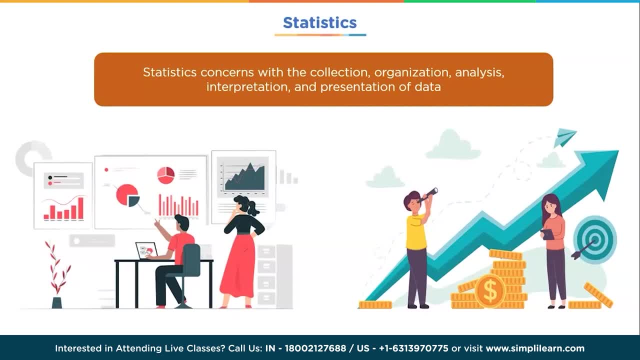 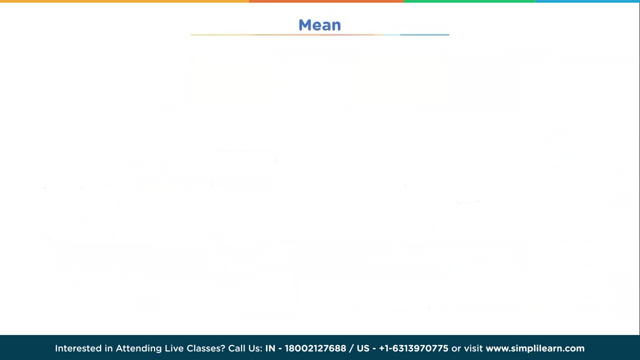 in virtually all scientific fields and research questions in the various scientific fields. In developing methods and studying the theory that analyze the methods, statisticians draw on variety of mathematical and computational tools. Now let's discuss about some of the important terms related to statistics. The first one is mean. 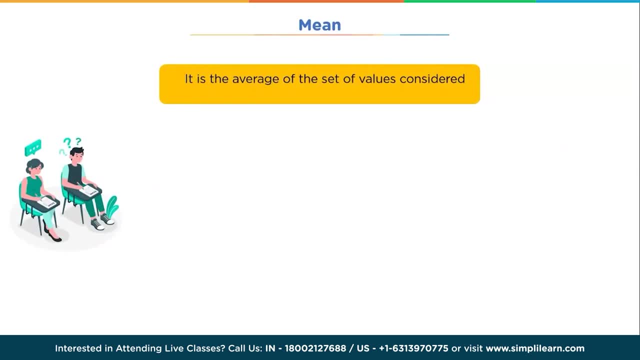 The mean, or the average, is the most popular and well known measure of central tendency. It can be used with both discrete and continuous data, although used is most often with the continuous data. It is the average of all the set of values that are considered To understand better. 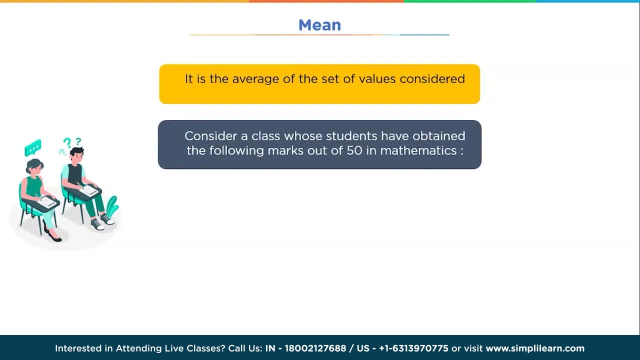 let's take an example. Suppose we have a class whose students have obtained the following marks out of 15 mathematics. Here are the following marks: So to find the mean of these marks, we will add all the marks and divide it by the number of marks there are. 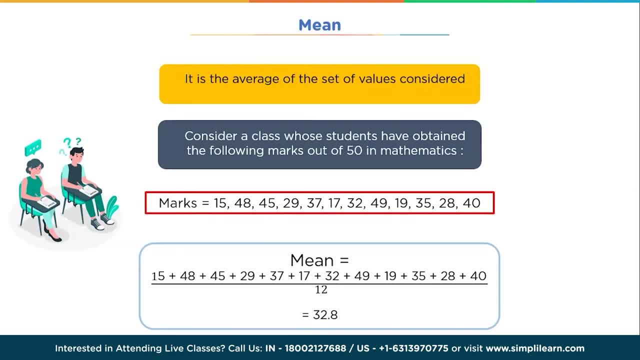 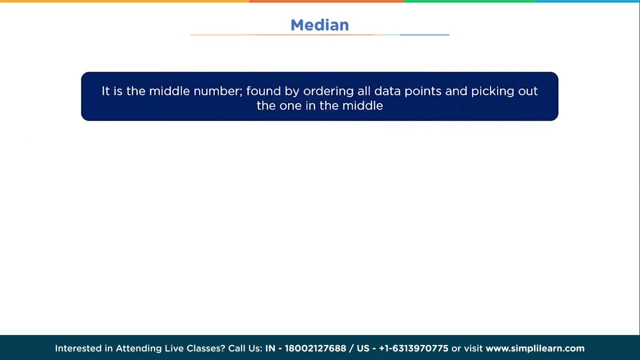 So we have the total of 12 marks. So the mean of these numbers are 32.8. The next term we are going to discuss is median. The median is the middle score for all the set of data that have been arranged in order of magnitude. 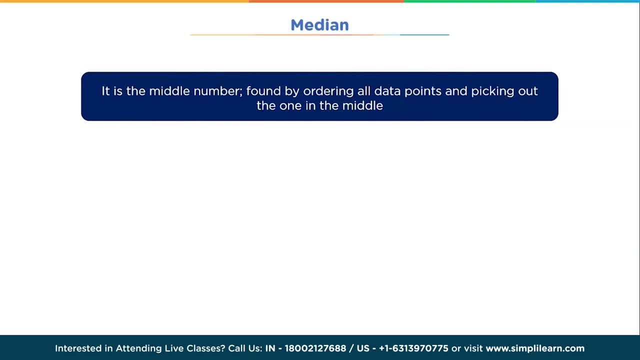 The median is less affected by the outliers and skewed data. In order to calculate the median, suppose we have the following data below: So these are the marks that we took in the previous example. We will first arrange these marks in the ascending order. So to find the median, 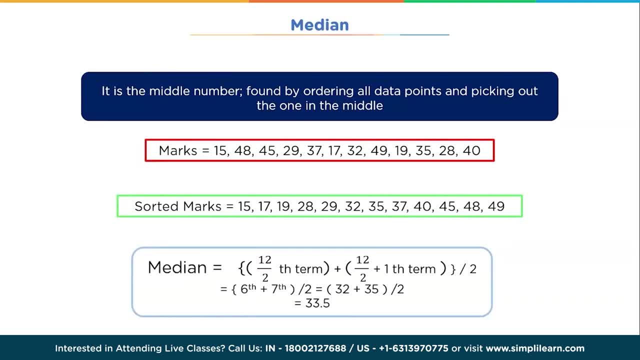 we will find the middle point of the two middle terms in the given data. So here the two middle terms are the sixth and the seventh term, which is 32 and 35. So adding the 32 and 35 and dividing it by 2, 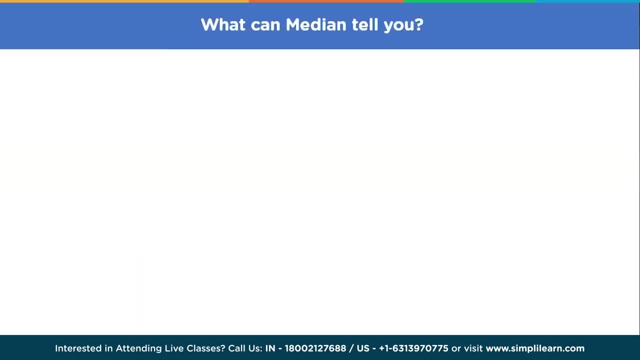 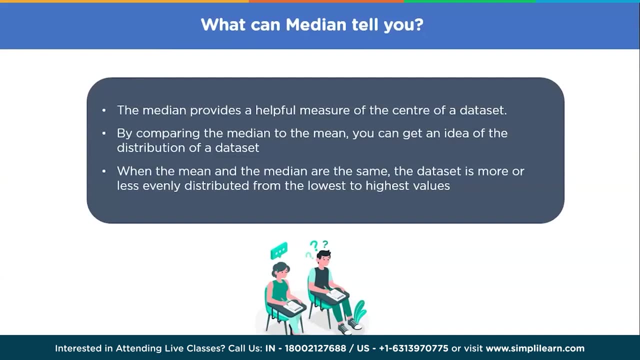 we will get 33.5. So what can the median tell you? The median provides a helpful measure of the center of the data set. By comparing the median of the mean, we can get an idea of the distribution of the data set. When the mean and the median 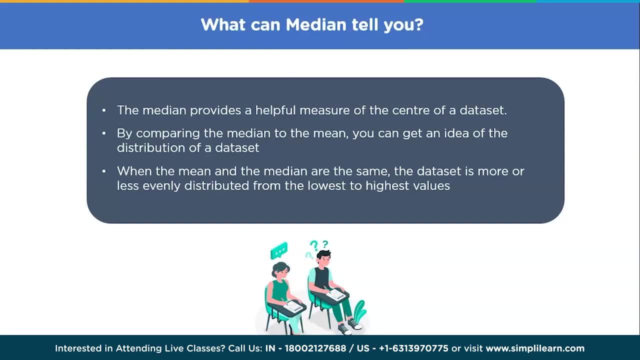 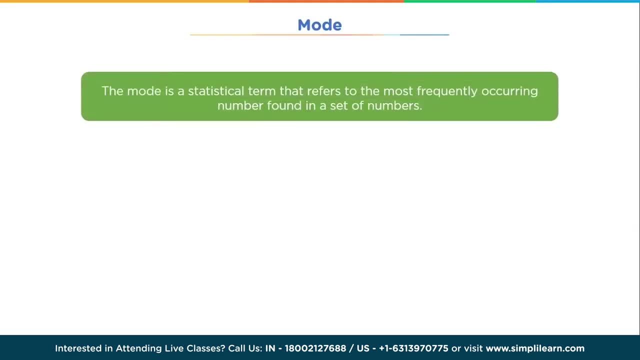 are the same. the data set is more or less evenly distributed from the lowest to highest values. The next term is mode. The mode is the most frequent score in our data set. So suppose we have this following example: Here you can see the mark 70 is occurring three times. 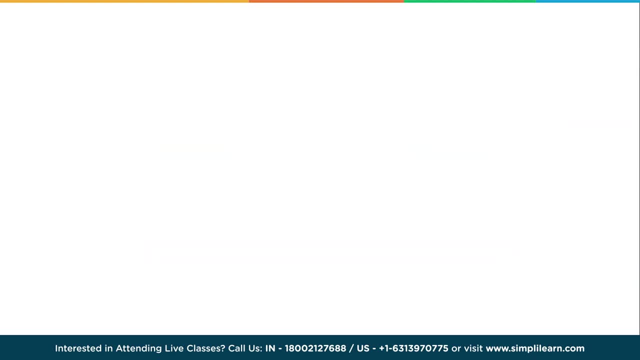 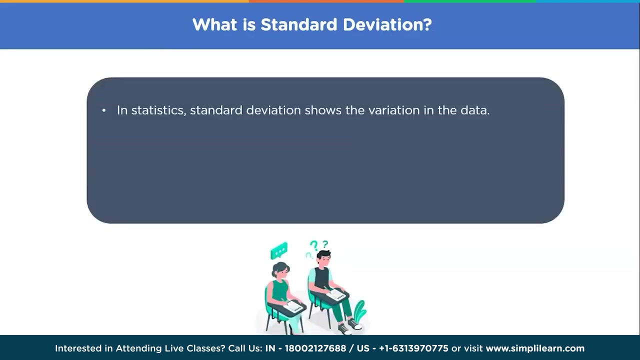 So this is our mode. Now that we have discussed all the terms related to statistics, Let's move on to standard deviation. So what is a standard deviation? A standard deviation is a statistics that measures the dispersion of a data set relative to its mean. The standard deviation is calculated. 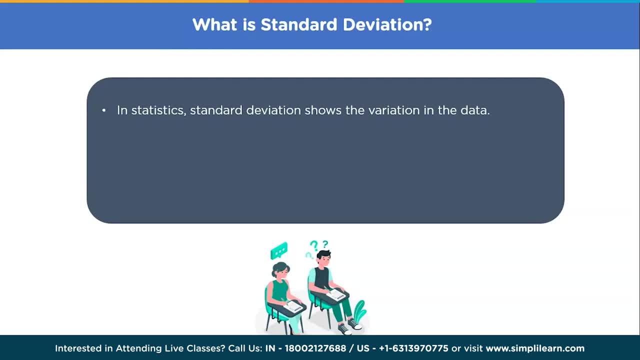 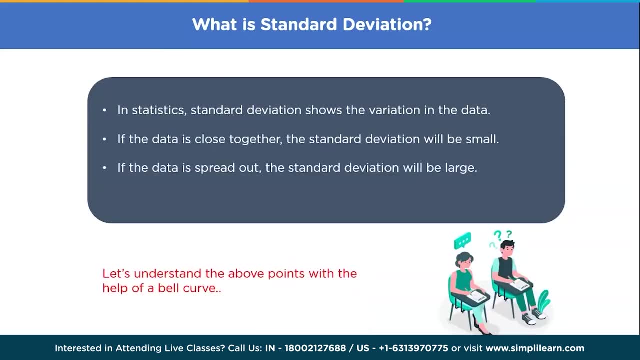 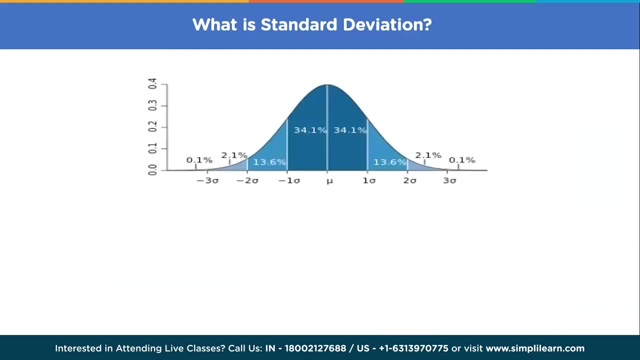 as the square root of variance, by determining each data point's deviation relative to the mean. If the data is closed together, the standard deviation will be small, And if the data is spread, then the standard deviation will be large. Let's understand these points with the help of a bell curve. 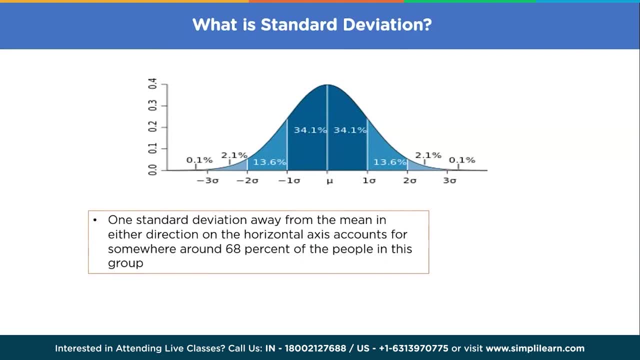 A bell curve's bit is defined by its standard deviation, which is calculated as the level of variation of the data in a sample around the mean. One standard deviation away from the mean in either direction on the horizontal axis accounts for some around 68.8% of the people in this group. 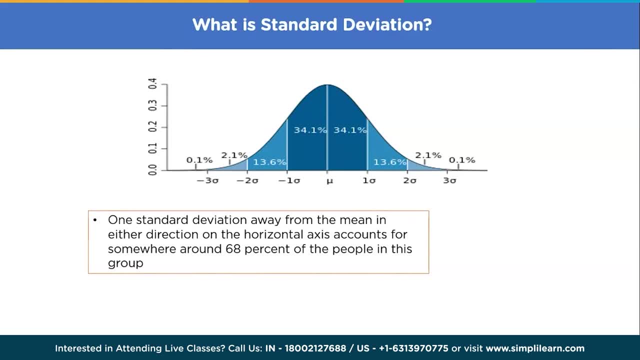 Suppose a 34.1 on the left side and a 34.1 on the right side. Moving two standard deviations away from the mean should include 95% of the total data. Moving three standard deviations away from the mean should represent 99.7%. 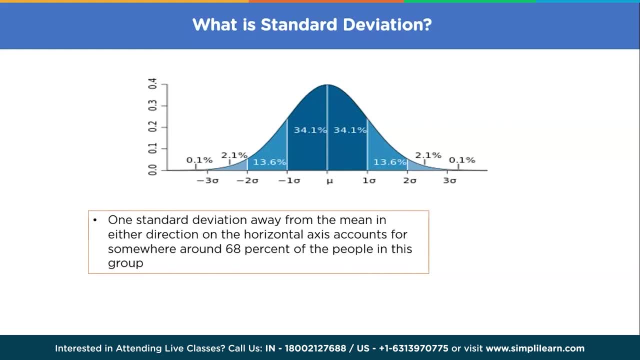 of the total data While interpreting a bell curve. the points nearest to the center of the bell curve are those which are most likely to occur, whereas the points closest to the left and right edges are the outliers. Bell curves are used across the wide variety of disciplines. 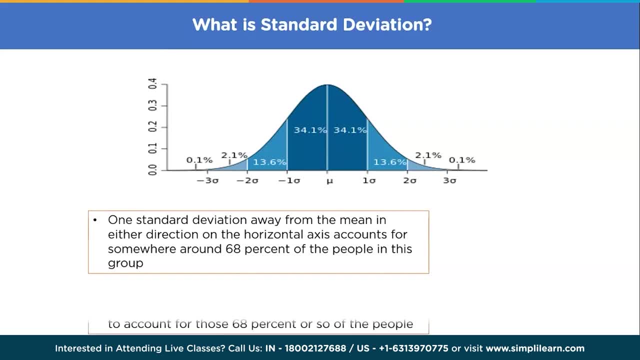 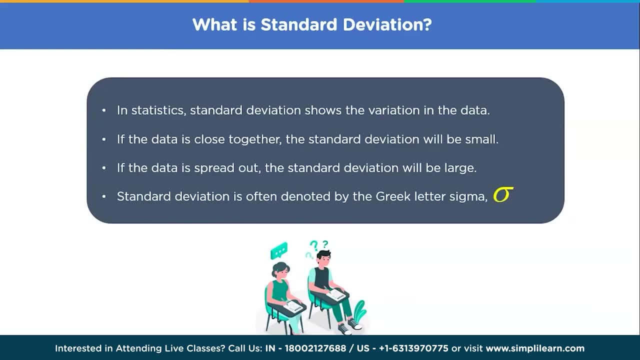 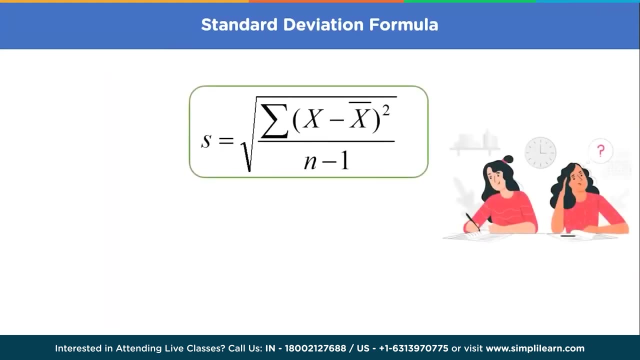 including finance and economics, social science and the natural science. Standard deviation is often denoted by the Greek letter word σ. Now that we know what is the standard deviation, let's see how we can calculate the standard deviation. So, to calculate the standard deviation, we have this formula: 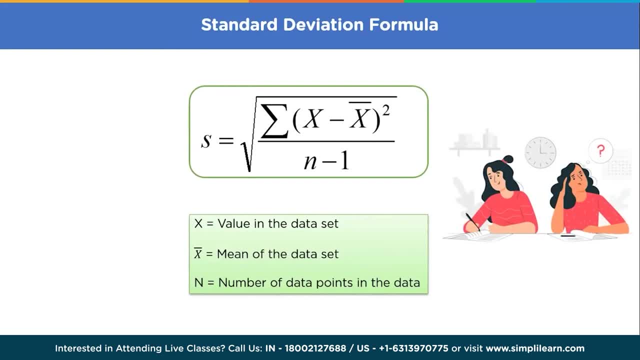 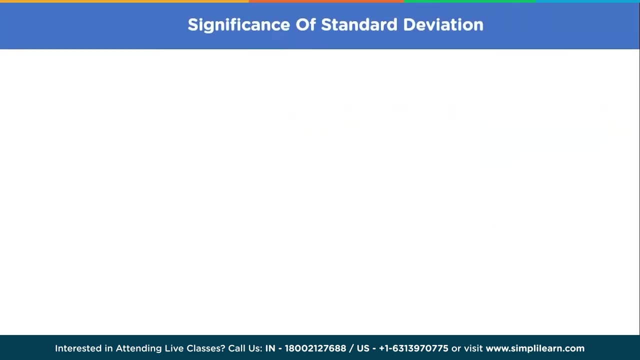 It is the under root of x minus x bar, whole square divided by n minus 1, where x is the value in the data set, x bar is the mean of the data set and n is the number of data points in the data. Now let's understand the significance. 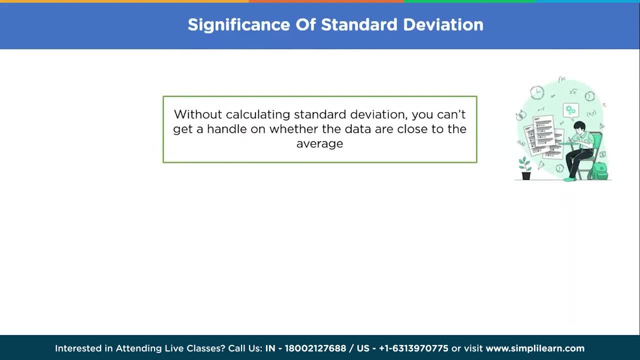 of standard deviation. To get the insights on a large data set you need this standard deviation. Suppose you are the owner of a car company where you manufacture the car parts and you want to keep check on the accuracy of the diameter of the car parts that are being manufactured in your company. 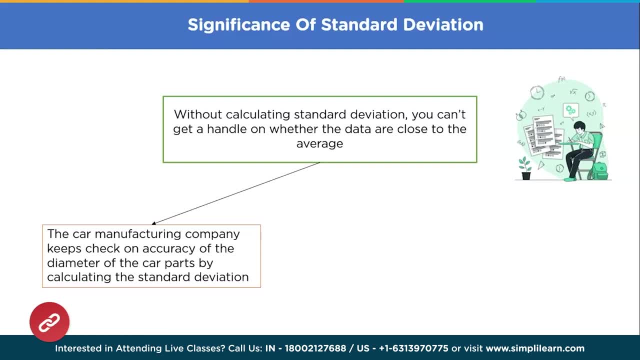 Standard deviation can be very helpful in this. You can calculate the deviation from the mean of the car parts that are being manufactured. The second example you can think of is the spread of the data, such as in case of house price or the average income levels in the US mortgage. 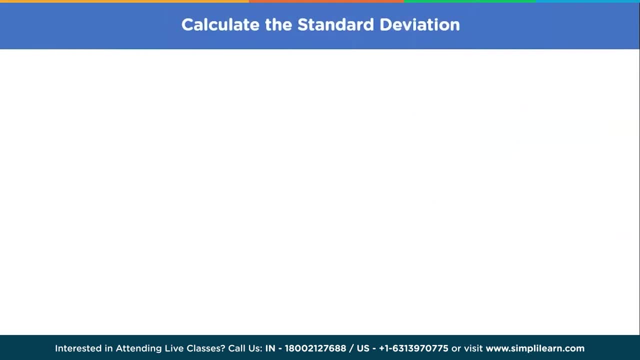 through the standard deviation. Now, this is all about the theoretical aspect of the standard deviation. Now let's learn how you can calculate the standard deviation. To calculate the standard deviation, we have taken this example. This is the marks of 6 students out of 100. 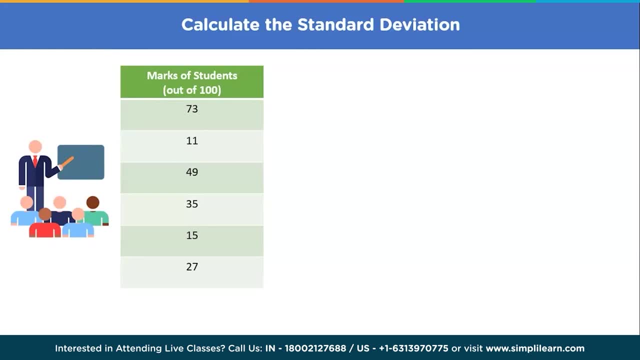 73,, 11,, 49,, 35,, 15 and 27. Now the first step is to find the mean of the given data. So to find the mean, as we have learnt in the previous slide, you just have to add. 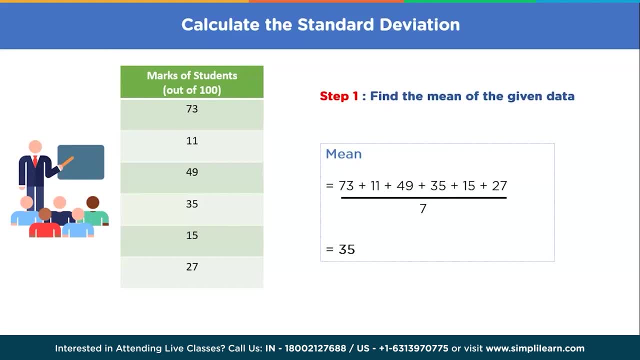 all the marks and divide by the total number of data. So here the mean is 35. Now the second step will be to calculate the square of the difference between each score and the mean. So we got the mean as our 35 and we will subtract the marks with the mean. 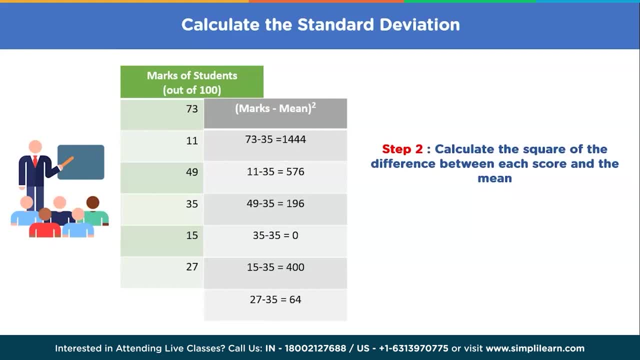 When we divide 35 from 73, we will get the answer as 38, and squaring the 38, we will get the answer as 144. In a similar manner, we have calculated the marks minus mean whole square. for all the cases, We get 576,. 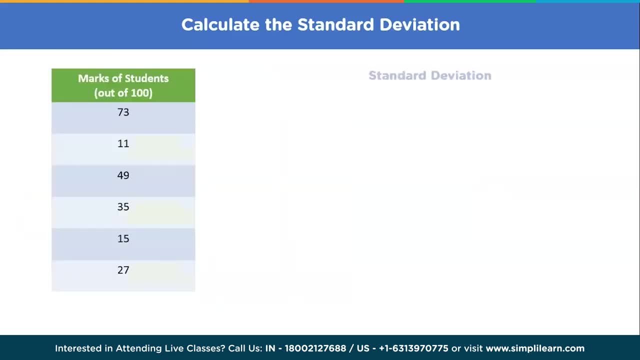 196, 0, 464. Now that we have all the data, we just need to put the data in our formula. So the formula was under root: marks minus mean whole square divided by total observations minus 1. Here the marks minus mean whole square will add. 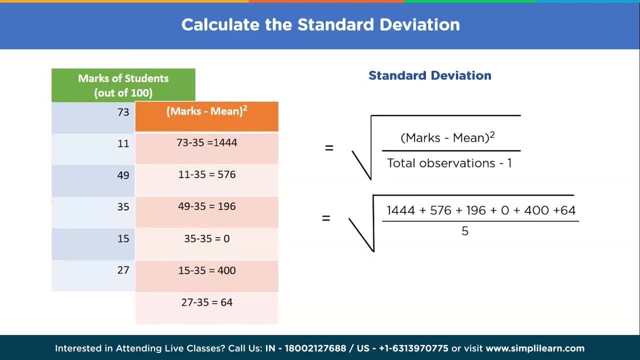 all the data and will divide it by the total observations data: 6 minus 1.. So this is the standard deviation we will get as 23.15. Now you might be wondering why we are calculating the standard deviation. What is the use of the standard deviation? 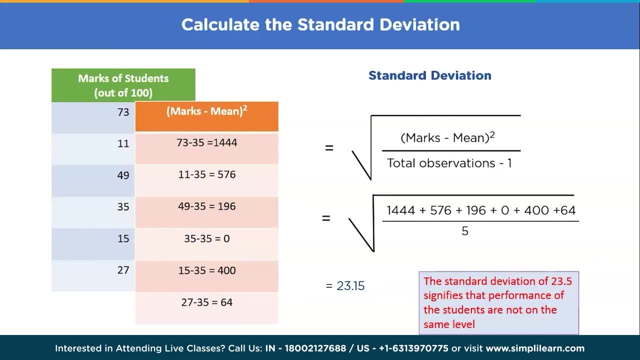 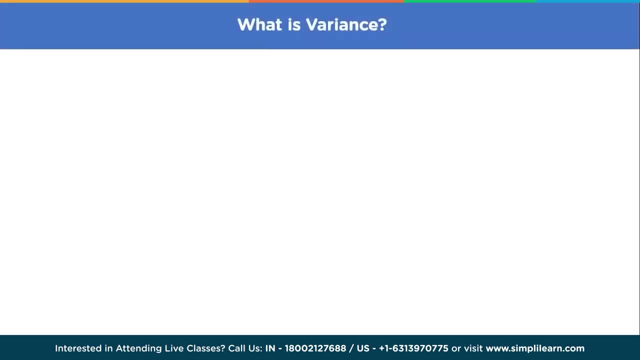 So the standard deviation of 23.15 defines that the performance of the students are not on the same level. They are deviating all over the place. Now that we have learnt about the standard deviation and have seen how to calculate the standard deviation, 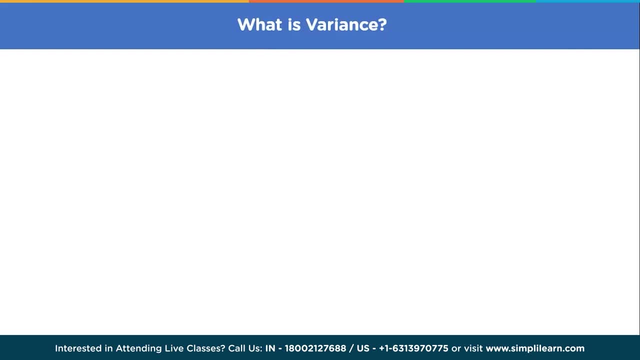 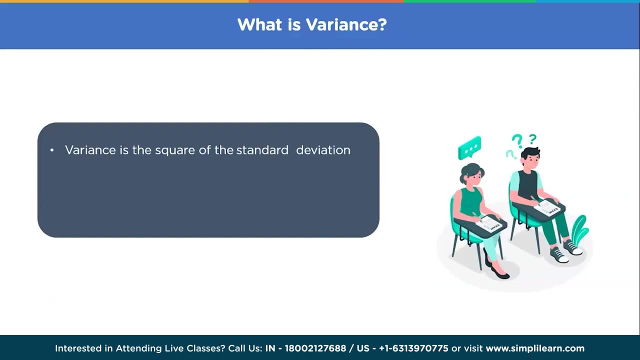 by taking an example. let's move further and learn about variance. So what is a variance? You can say variance is the square of the standard deviation. It is a statistical concept whose purpose is to measure the dispersion of observation around the mean or the average value. 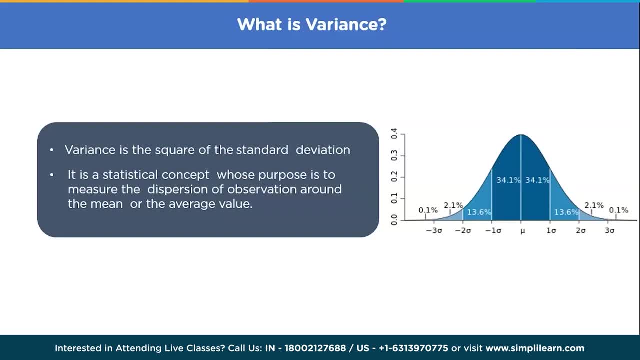 Variance tells the degree of spread in your data set. The more spread the data, the larger the variance is in relation to the mean and you can see with the graph Our central line, mu is the mean and on the either side of the mean you can see the spread of the data. 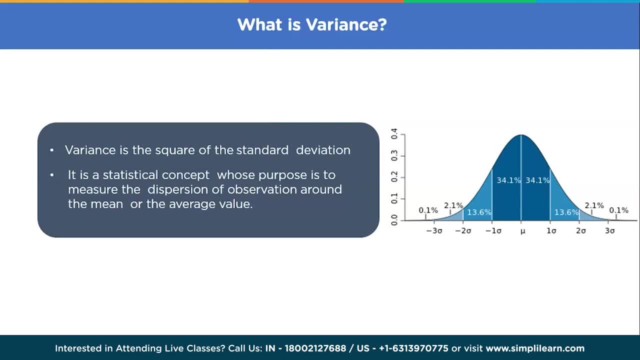 The major difference between the standard deviation and the variance is that stringent deviation is expressed in the same units as the original values, suppose exact meters. Variance is expressed in much larger units- Example meters squared- Since the units of variance are much larger than those of a typical value of a data set. 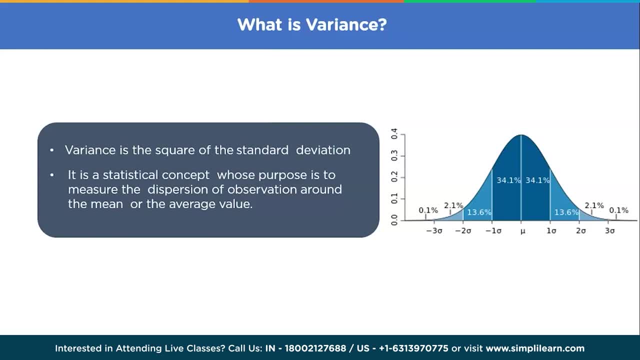 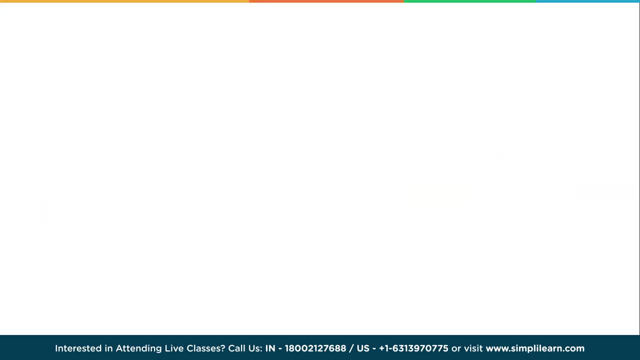 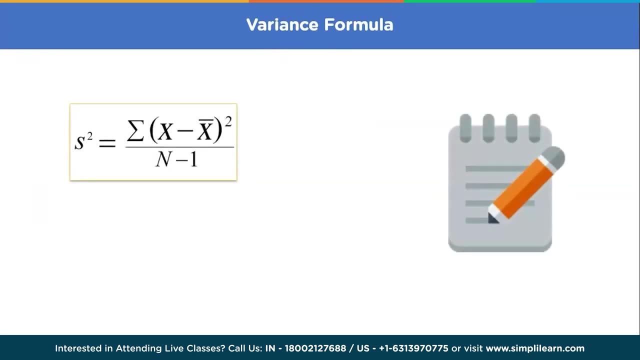 It's harder to interpret the variance number accurately. That's why standard deviation is often preferred as the main measure of variability. So to calculate the formula we just have to square the formula that we have seen in the standard deviation. So the formula of the variance is: 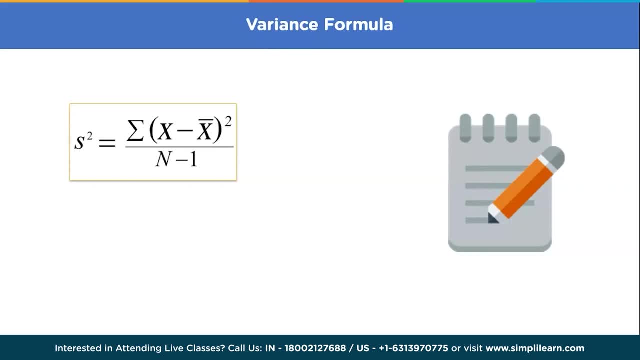 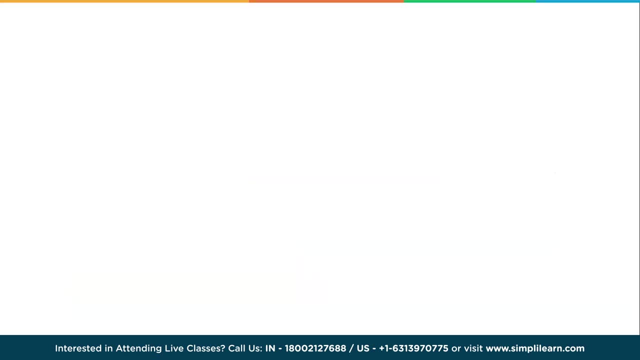 sigma x minus x bar: whole square divided by n minus 1, Where x is the value in the data set, x bar is the mean of the data set and n is the number of data points in the data. Let's see some example where variance is used in the real life. 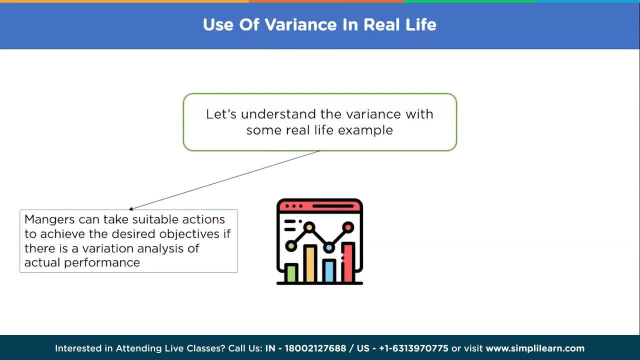 In a real life situation, managers can take suitable actions to achieve the desired objectives. if there is a variation analysis of the actual performance, You can compare the variation of the performance in the different quarter against the mean of the performance of all the employees. The second example you can think of. 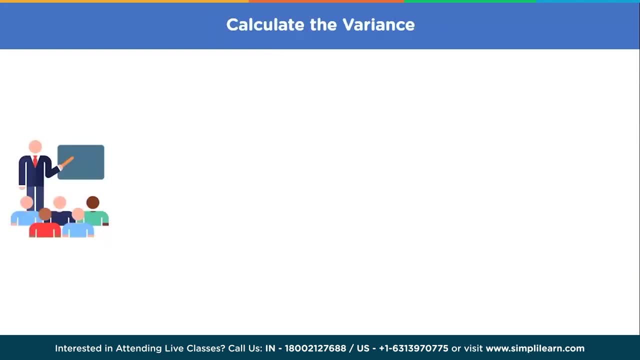 is the analysis of the performance of the different organization. So how to calculate the variance? So this is the same previous example. We have the marks of student out of 100. So the first step would be to find the mean of the given data. 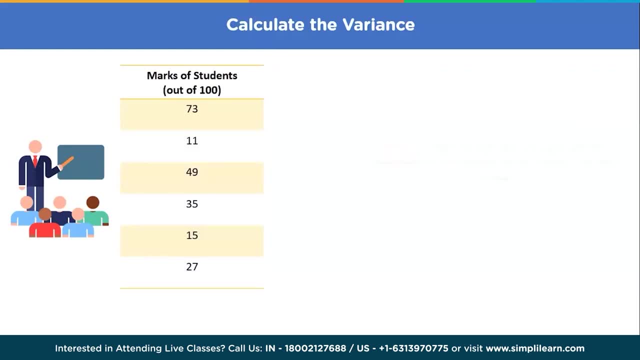 So, as calculated before, the mean of the given data was 35. Step 2 will be to calculate the square of the difference between each score and the mean. So this is the same as the previous step, where we have calculated the marks minus mean whole square. 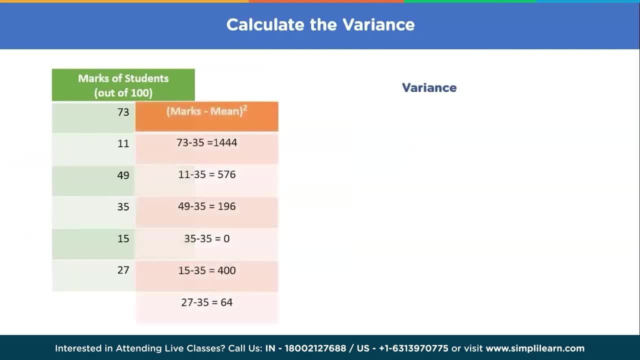 The change comes here. The variance formula is the square of the marks minus mean whole square divided by observation, minus n. So when we add all the marks minus mean whole square and divide it by 5 we will get the variance as 536 Majorly variance is used. 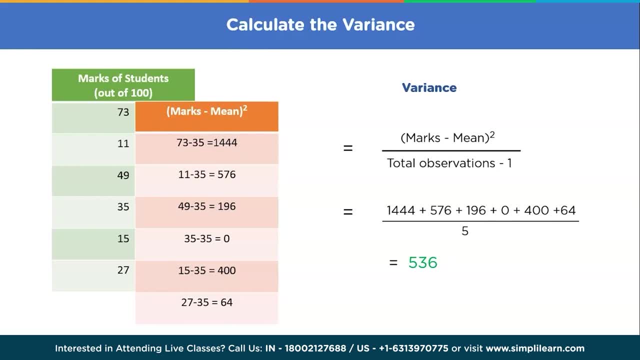 to calculate the standard deviation, since it is the square root. When we calculate the square root of 536, we will get the answer as 23.5. This is the same as the standard deviation. So you must be thinking: Why does variance matter? So variance matters for two main reasons. 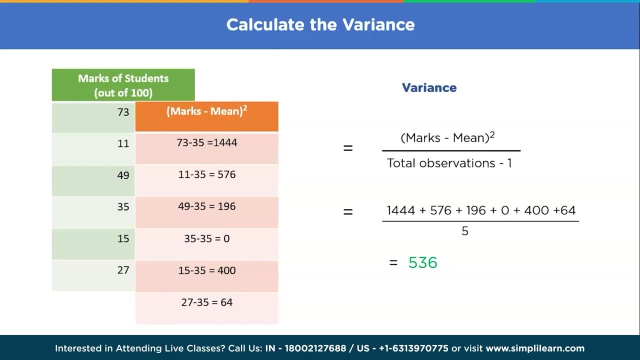 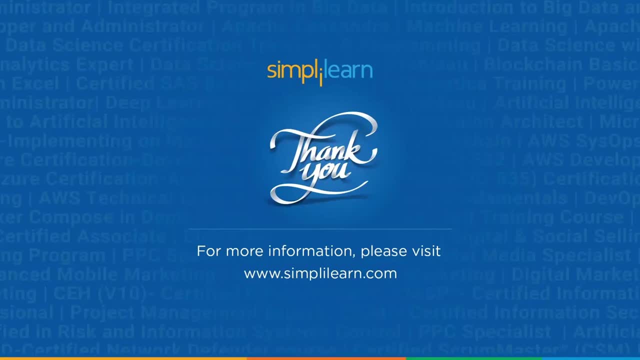 First, the parametric statistical tests are sensitive to variance. Comparing the variance of sample helps you to assess the group differences. And with that we have reached to the end of this session on statistics for data science full course. Should you need any assistance, PPT. 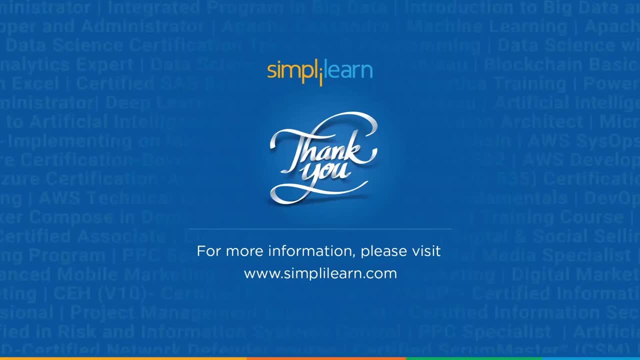 or any other resources used in this session, please do let us know in the comment section below, and our team of experts will be more than happy to help you as soon as possible. Thank you for watching and stay tuned for more from Simply Learn: Staying ahead in your career.